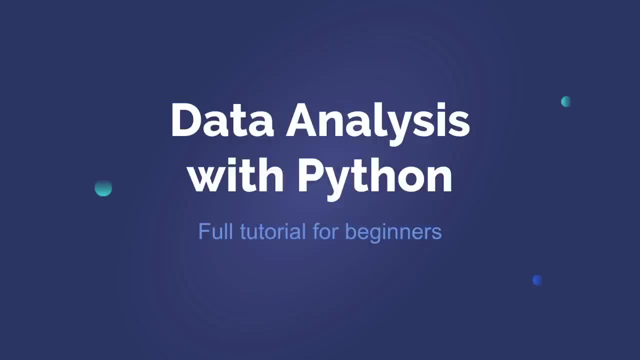 Welcome to our data analysis with Python tutorial. My name is Santiago and I'm an instructor at Remotercom, an online data science academy. This tutorial is a result of a joint effort by Remoter and FreeCodeCamp and it's totally free. It includes slides, Jupyter, notebooks. 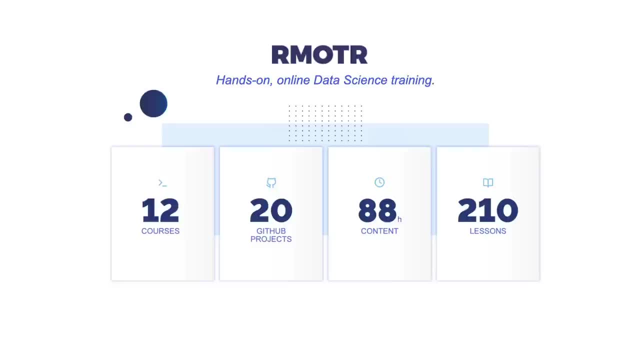 and coding exercises. Let me tell you a little bit more about Remoter. We're an online hands-on data science academy. We specialize in data science, including data analysis, programming and data analysis. We're also an online hands-on data science academy. We specialize in data science, including data analysis, programming and data analysis. 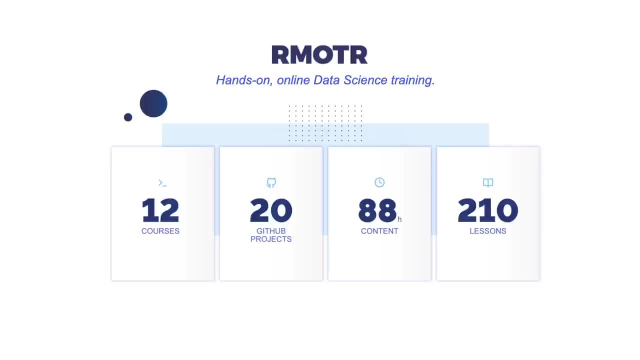 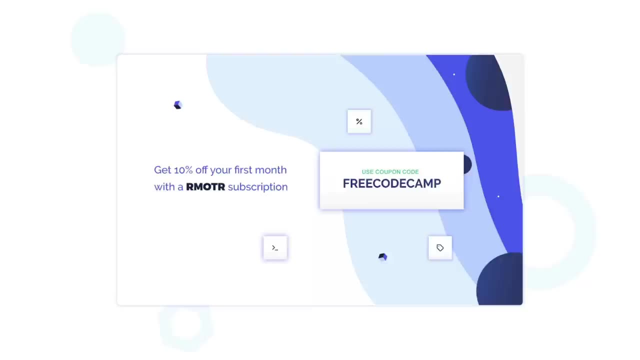 and machine learning. We have a complete course catalog and we're adding more content every month. If you're interested in learning data science or data analysis, check us out. As part of this joint effort between FreeCodeCamp and Remoter, you can get a 10% discount in your first month by using the following discount coupon: 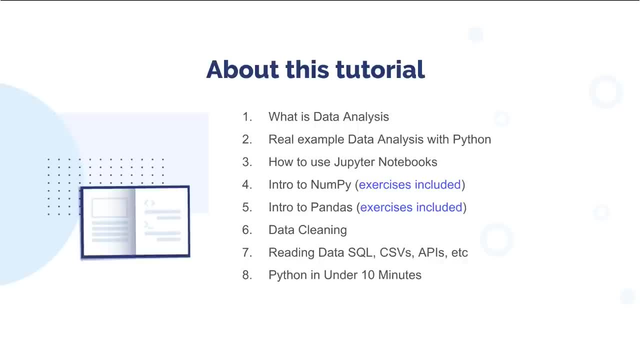 Let's quickly review the contents of this tutorial. In the description of this video, we have included direct links to each section so you can jump between them. This is the first section, and we are going to discuss what is data analysis. We'll also talk about data. 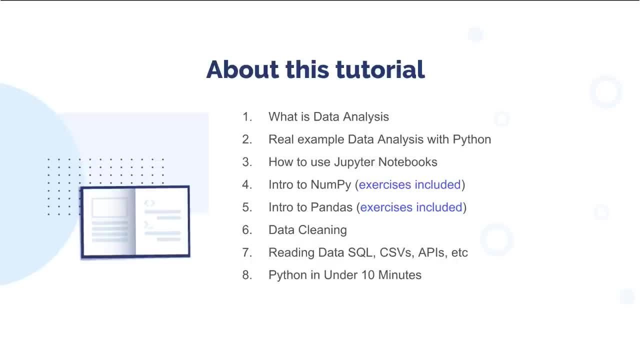 analysis with Python and why programming tools like Python, SQL and Pandas are important. In the following section we'll show you a real example of data analysis using Python so you can see the power of it. We'll not explain the tools in detail. 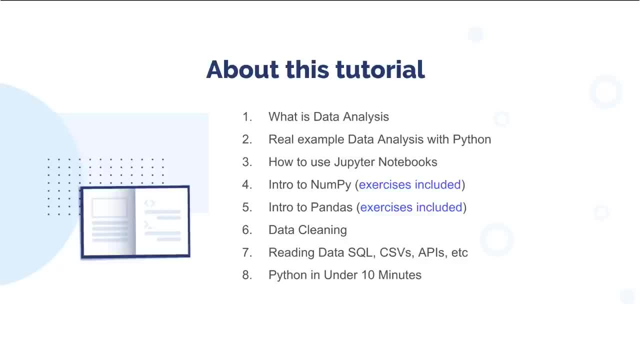 It's just a quick demonstration for you to understand what this tutorial is about. The following sections will be the ones explaining each tool in detail. There are two more sections that I want to specially point out. The first one is section number three, Jupyter tutorial. This is not mandatory. 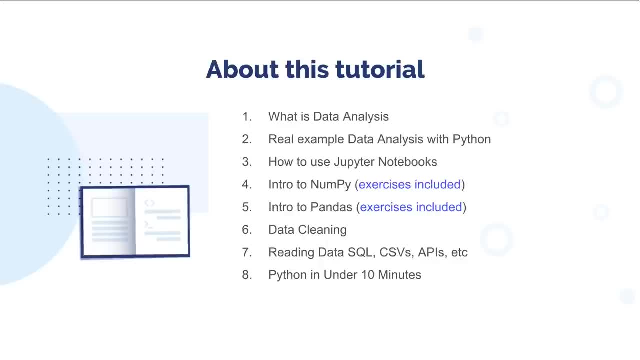 and you can skip it if you already know how to use Jupyter notebooks. Also, the last section: Python, in under 10 minutes. This is just a recap of Python. if you are coming from other languages, You might want to take this first. if that's the case, Again, you can use the. 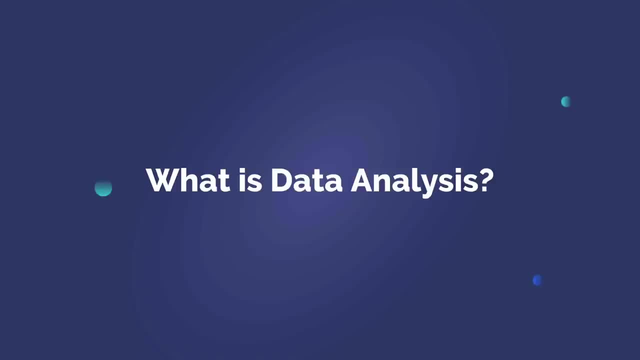 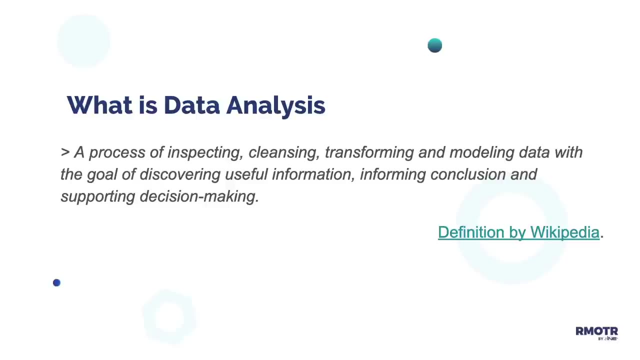 links in the video description to jump straight to it. Alright, now let's define what is data analysis. I think the Wikipedia article summarizes perfectly the process of inspecting, cleansing, transforming and modeling data with the goal of discovering useful information, informing conclusions and support decision making. Let's analyze this definition piece by 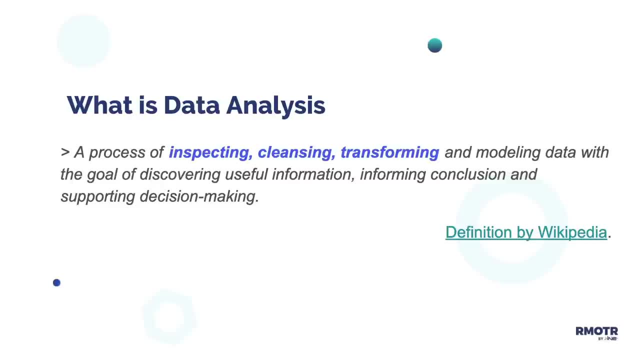 piece. The first part of the process of data analysis is usually tedious. It starts by gathering the data, cleaning it and transforming it for further analysis. This is where Python and tools excel. We're going to be using pandas to read, clean and transform our data Modeling. 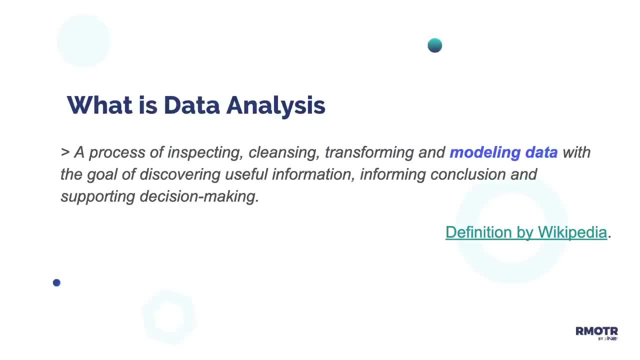 data means adapting real life scenarios to information systems, using inferential statistics to see if any pattern or model arise. For this we are going to be using the statistical analysis features of pandas and visualizations from Apple, Live and Seaborn, Once we've processed the data. 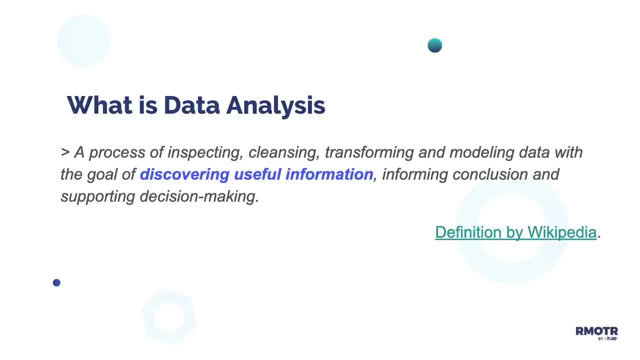 and created models out of it. we'll try to drive conclusions from it so we can see if there are interesting patterns or anomalies that might arise. The word information here is key. We're trying to transform data into information. Our data might be a huge list of all the purchases made in Walmart in the last year. The information will be 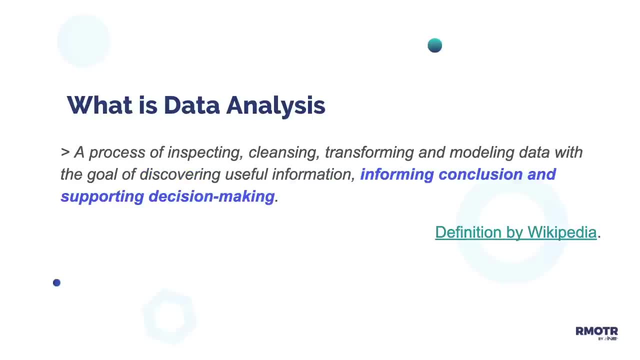 something like Pop-Tarts sell better on Tuesdays. This is the final objective of data analysis. We need to provide evidence of our findings, create readable reports and dashboards and aid other departments with the information we've gathered. Multiple actors will use your analysis: Marketing, sales, accounting executives, etc. 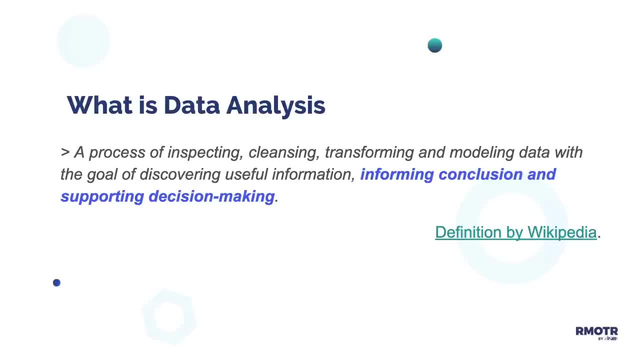 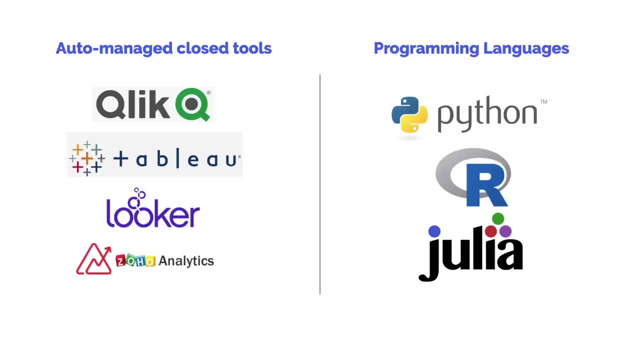 They might need to see a different view of the same information. They might all need different reports or level of detail. What tools are available today for data analysis? We've broken these down into two main categories. Auto-managed tools are closed products, Tools that you can buy and start using right out of the box. 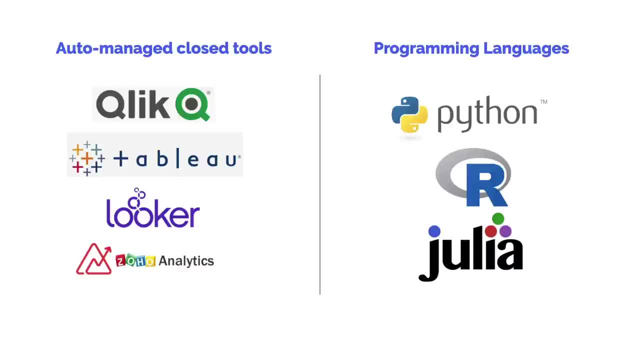 Excel is a good example. Tableau and Looker are probably the most popular ones for data analysis. In the other extreme, we have what we call programming languages, or we could call them open tools. These are not sold by an individual vendor, but they are a combination of languages. 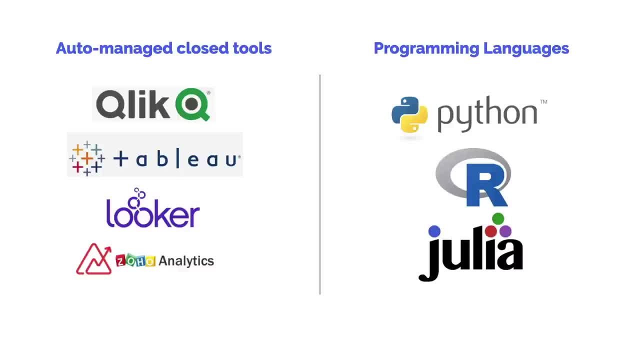 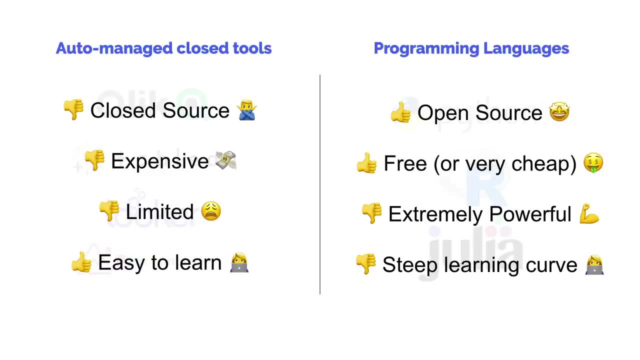 open source libraries and products. Python, R and Julia are the most popular ones in this category. Let's explore the advantages and disadvantages of them. The main advantage of closed tools like Tableau or Excel is that they are generally easy to learn. There is a company. 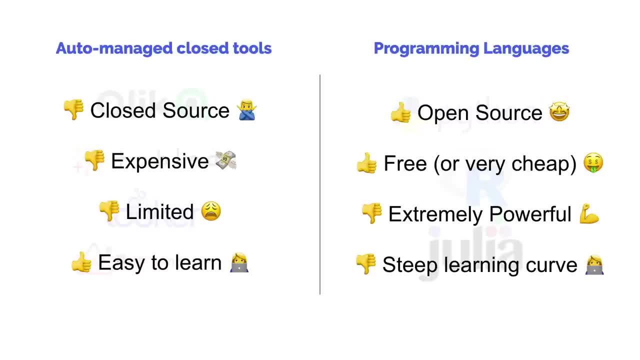 providing support and driving the creation of the product. The biggest disadvantage is that the scope of the tool is limited. You can't cross the boundaries of it. In contrast, using Python and the universe of Pydata tools gives you amazing flexibility. Do you need to read data from a closed API using secret key authentication? You can do it. 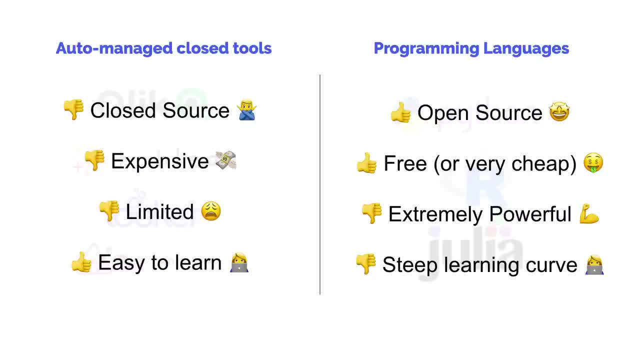 Do you need to consume data directly from AWS Kinesis? A programming language is the most powerful tool you can learn. A programming language is the most powerful tool you can learn. A single prospect is one of the main reasons this school is spoken In the. 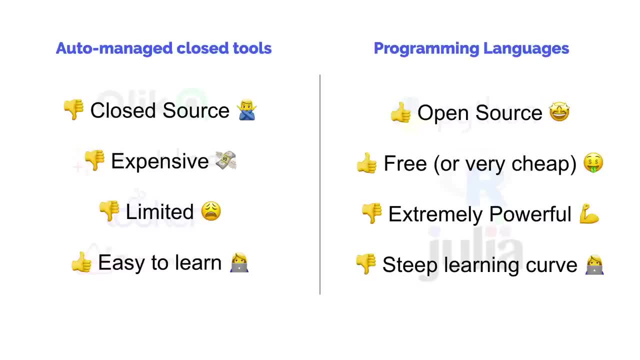 learn. Another important advantage is a general scope of a programming language. What happens if Tableau, for example, goes out of business or if you just get bored from it and feel like your career is stuck? you need a career change: Learning how to process data using. 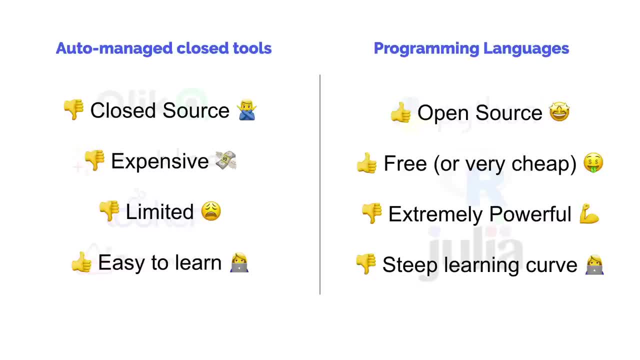 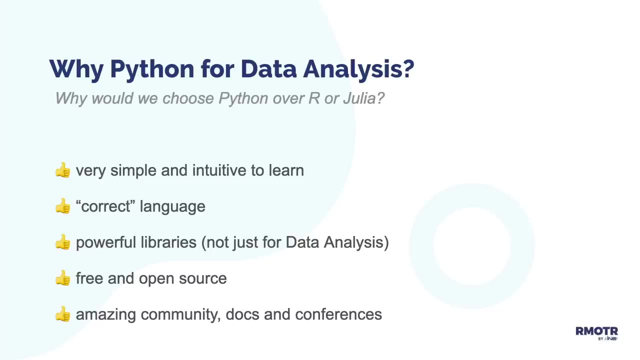 a programming language gives you freedom. The main disadvantage of a programming language is that it's not as simple to learn as with a tool. you need to learn the basics of coding first, And it takes time. Why are we choosing Python to do data analysis? Python is the 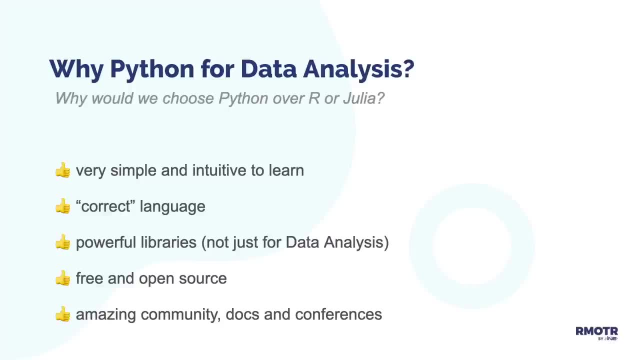 best programming language to learn to code. It's simple, intuitive, unreadable. It includes 1000s of libraries to do virtually anything from cryptography to IoT. Python is free and open source. That means that there are 1000s of eyes, very smart people, seeing the internals. 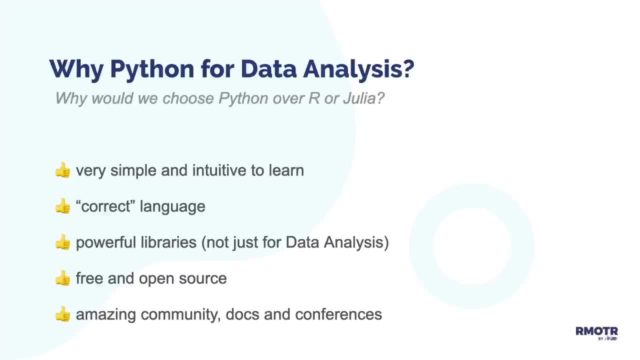 of the language on the libraries. From Google to Bank of America, major institutions rely on Python Every day, which means that it's very hard for it just to go away. Finally, Python has a great open source spirit. The community is amazing. the documentation is exhaustive. 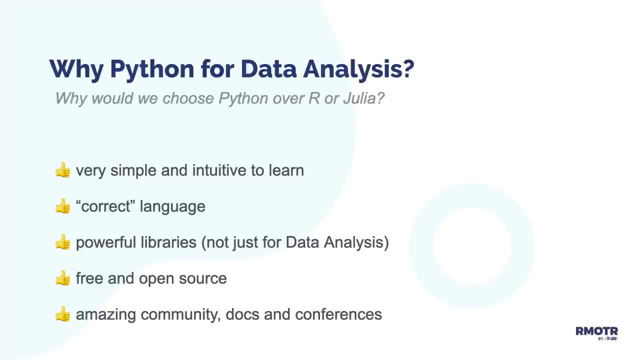 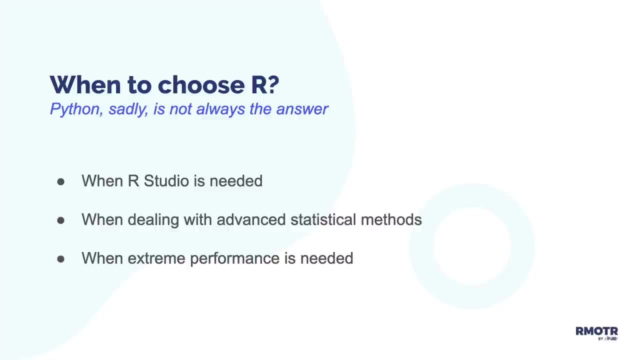 and there are a lot of free tutorials around. Check out for conferences in your area. it's very likely that there is a local group of Python developers in your city. We couldn't be talking about data analysis without mentioning R. R is also a great programming language. 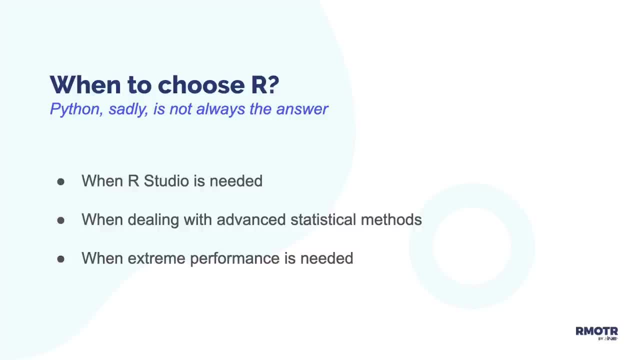 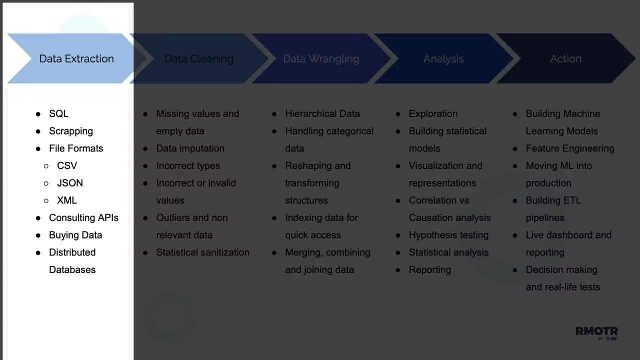 We prefer Python because it's easier to get started. R has a huge library of statistical functions and if you're in a highly technical discipline, you should check it out. Let's quickly review the data analysis process. The process starts by getting the data Where 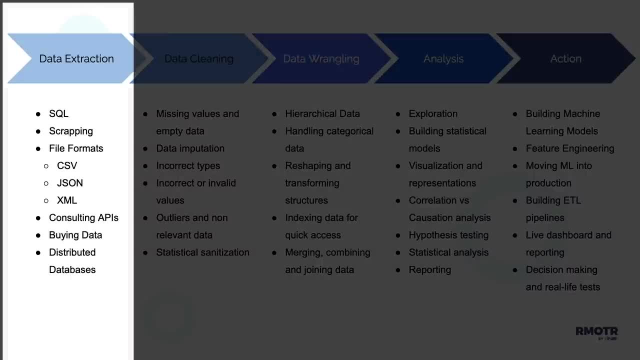 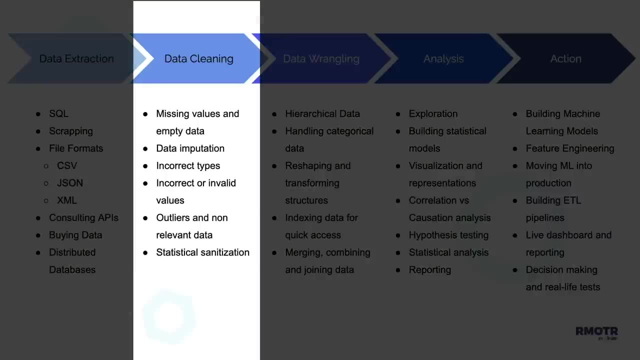 is your data coming from? Usually it's in your own database, but it could also come from file store in a different format or a web API. Once you've collected the data, you'll need to clean it. If the source of the data is your own database, then it's probably already in shape. If you're. 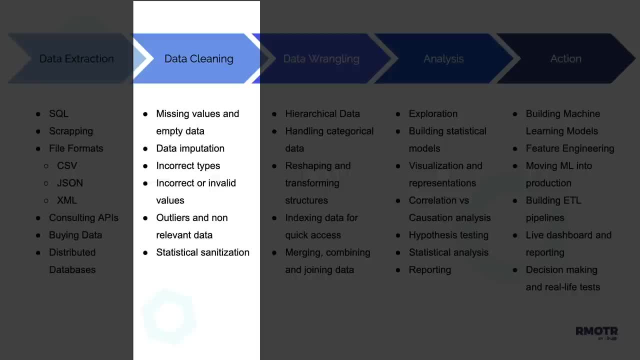 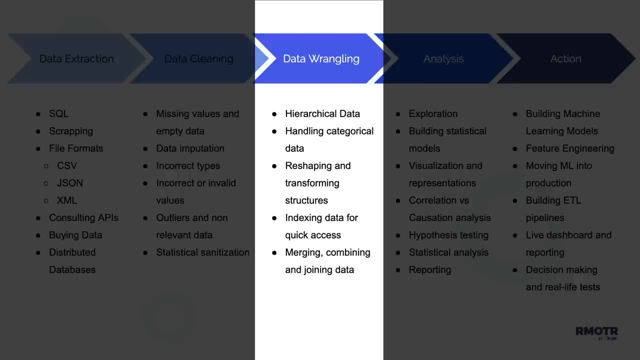 using more extreme sources like web scraping, then the process will be more tedious. With your data cleaned, you'll now need to rearrange and reshape the data for better analysis: transforming fields, merging tables, combining data from multiple sources, etc. The objective: 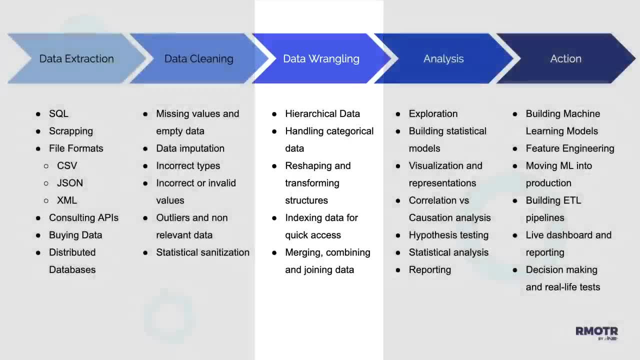 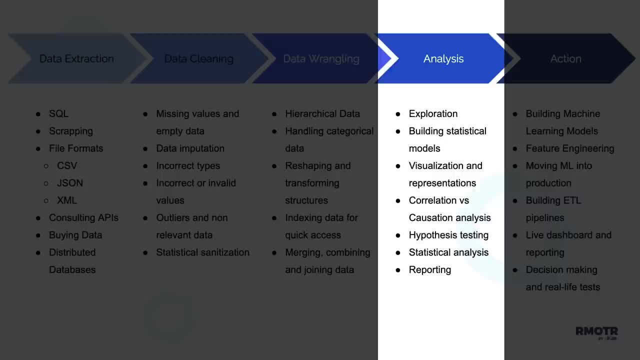 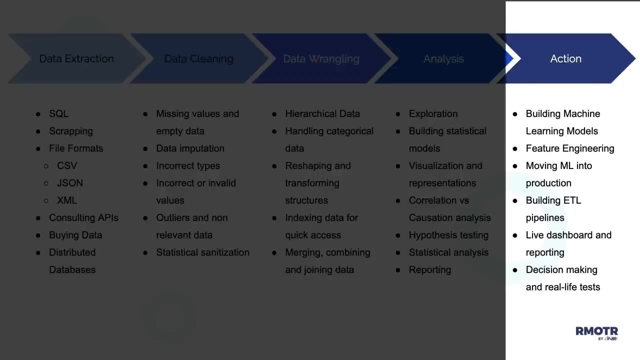 of this process is to get the data ready for the next step. The process of analysis involves extracting patterns from the data that are already in shape. If the data is already in shape, then it's time to do something with the data analysis. If this was a data science. 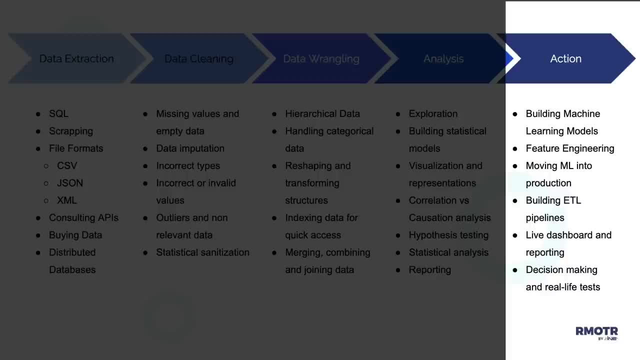 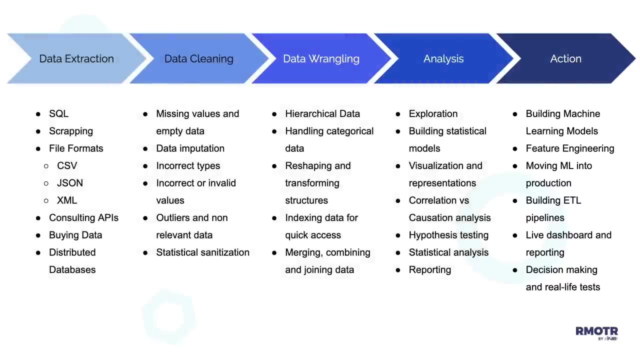 project, we could be ready to implement machine learning models. If we focus strictly on data analysis, we'll probably need to build reports, communicate our results and support decision making. Let's finish by saying that in real life, this process isn't so linear. We're usually. 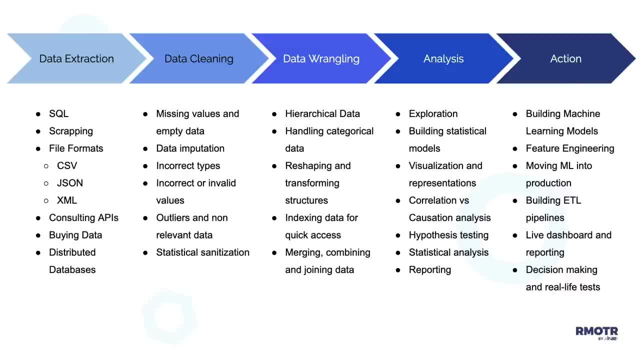 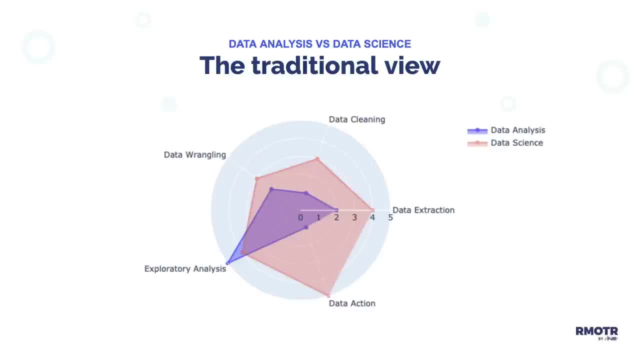 jumping back and forth between the steps and it looks more like a cycle than a straight line. What is the difference between data analysis and data science? The boundaries between data analysis and data science are not very clear. The main differences are that data scientists 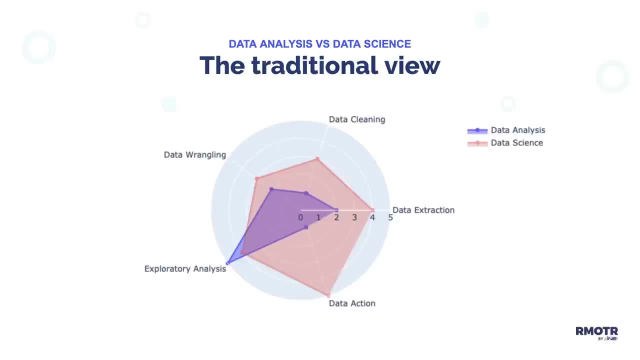 usually have more programming and math skills. They can then apply these skills in machine learning and ETL processes. Data analysts, on the other hand, have better communication skills, creating better reports with stronger data analysis. Data analysts, on the other hand, have better communication skills, creating better reports with stronger data analysis. 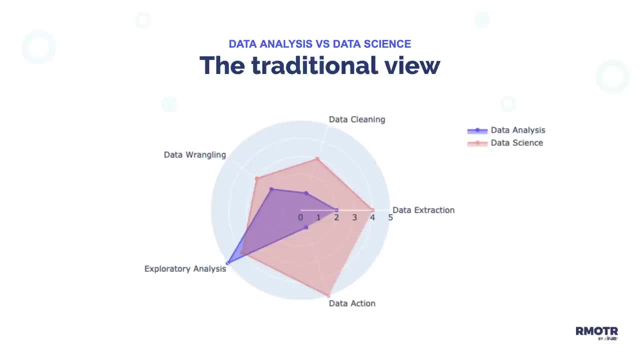 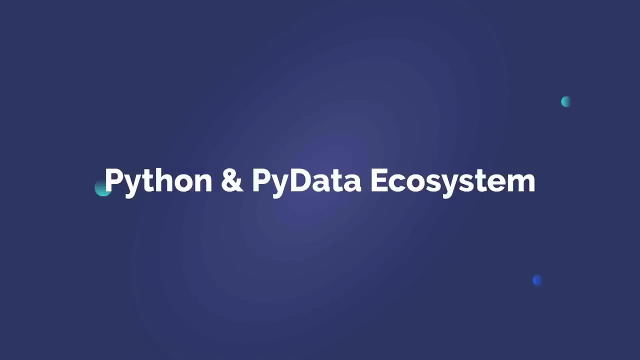 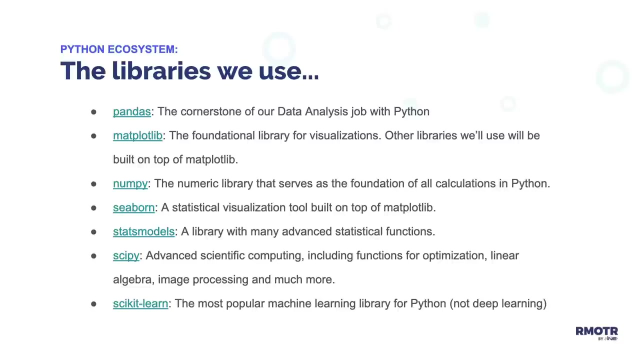 These are all subtle points ofganisation, value sharing and communication. After we have choose to succeed in our調べar and collect data, we'll all pull together and form down stronger story-telling abilities. By the way, this radar chart is available in. 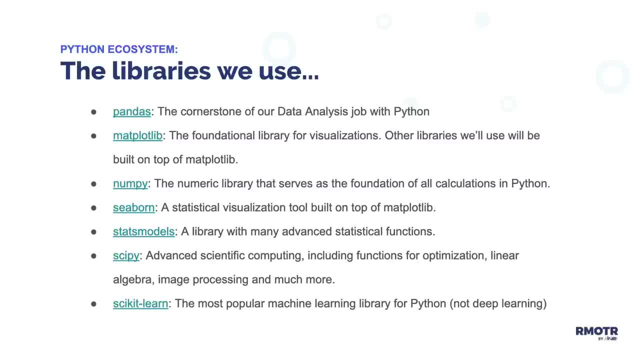 the notes. if we want to choose our source code, Let's explore the Python and PyData ecosystem, all the tools and libraries that we will be using. The most important libraries that we will be using are Pandas for data analysis and Map, Bow, Live and Seaborn for visualizations. but the ecosystem is large and there are many. 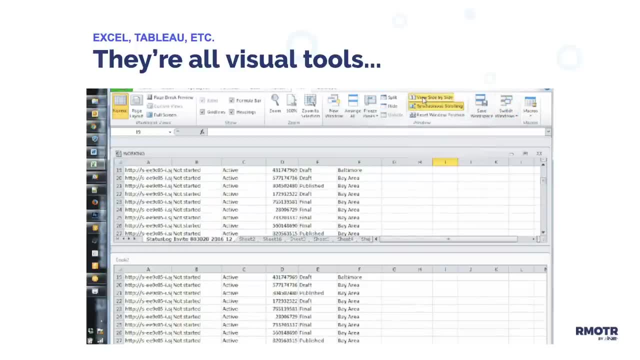 useful libraries for specific use cases: forward777.270.4radas-p. 3721-2324.7777,. coming from a traditional data analysis place using tools like Excel and Tableau, you're probably used to have a constant visual reference of your data. All these tools are point and. 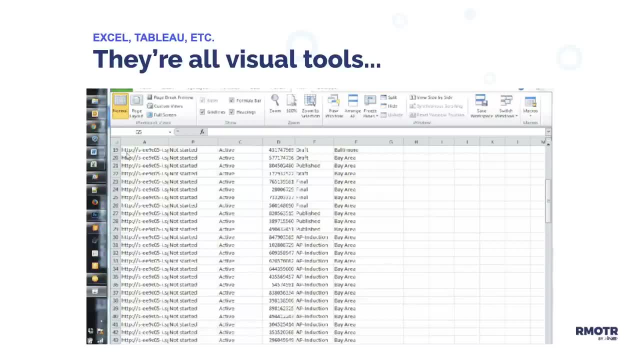 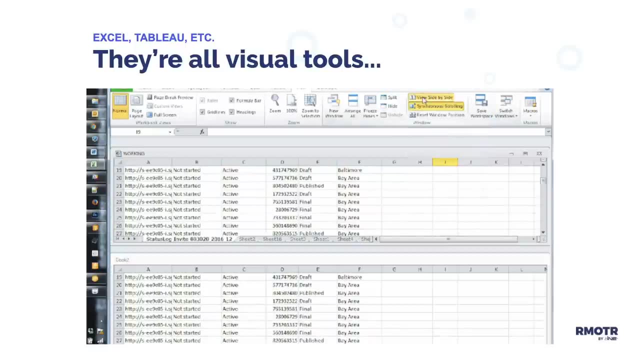 click. This works great for a small amount of data, but it's less useful when the amount of records grow. It's just impossible for humans to visually reference too much data, And the processing gets incredibly slow. In contrast, when we work with Python, we don't. 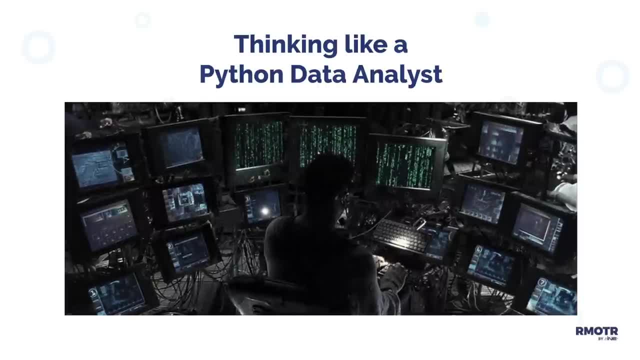 have a constant visual reference of the data we're working with. We know it's there, we know how it looks like, we know the main statistical properties of it, but we're not constantly looking at it. This allows us to work with millions of records incredibly fast. This 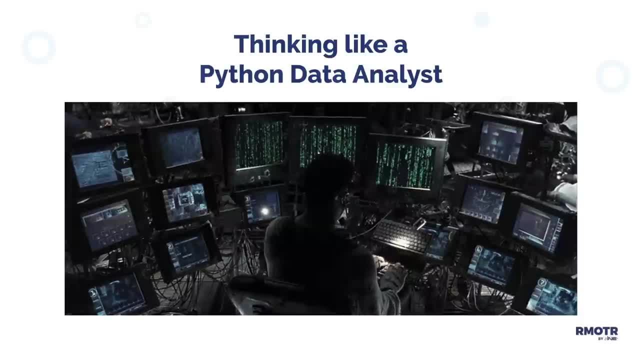 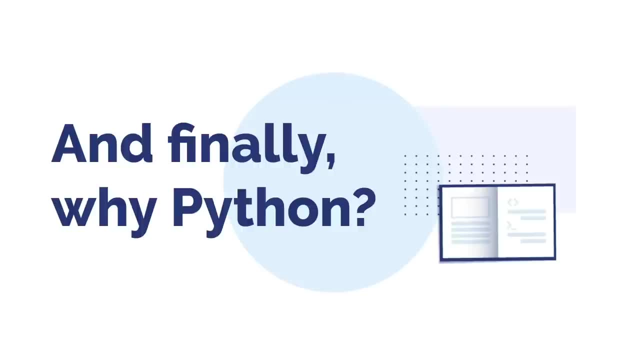 also means you can move your data analysis processes from one computer to the other and, for example, to the cloud, without much overhead. And finally, why would you like to add Python to your data analysis skills? Aside from the advantages of freedom and power, 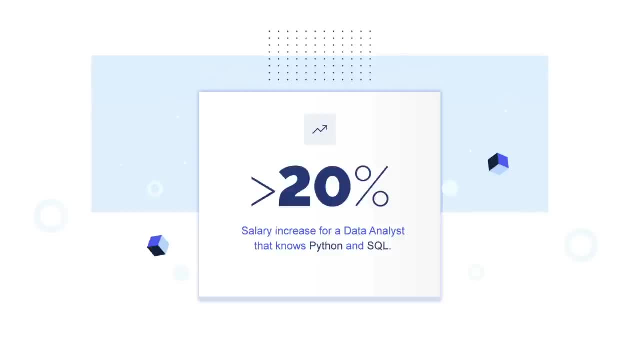 there is another important reason: According to pay scale, data analysts that know Python and SQL are better paid than the ones that don't know how to use programming tools. So that's it. let's get started. in our following section, we'll show you a real world example. 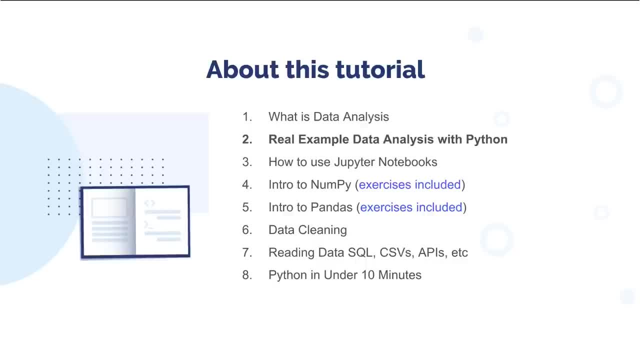 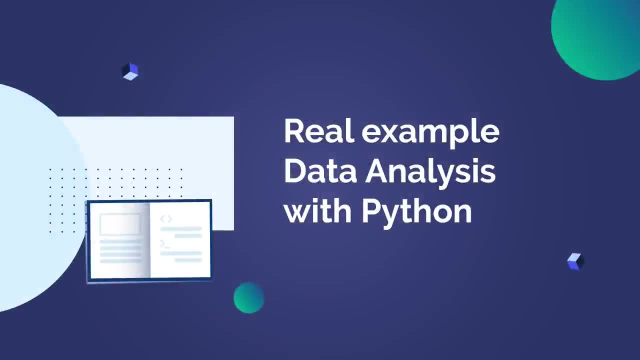 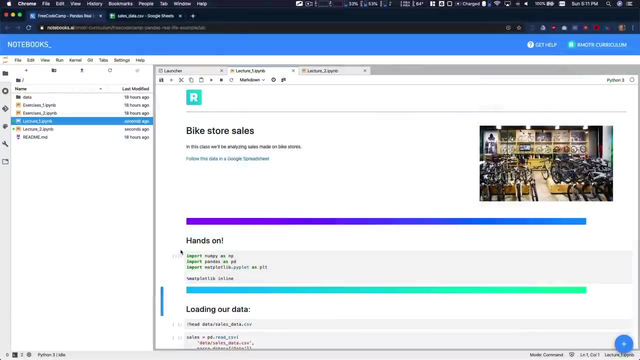 of data analysis with Python. we want you to see right away what you will be able to do after this tutorial. We're gonna start with the first example of data analysis with Python. we're going to to start this tutorial by working with a real example of data analysis and data processing. 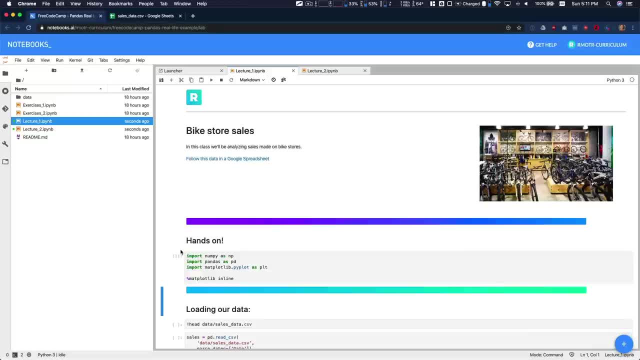 with Python. we're not going to get into the details yet. the following sections will explain what each one of the tools does and what is the best way to apply them, combining and the details of them in general. This is just for you to have a quick and high level reference. 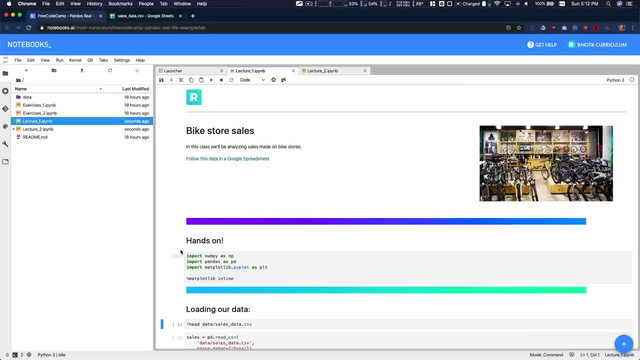 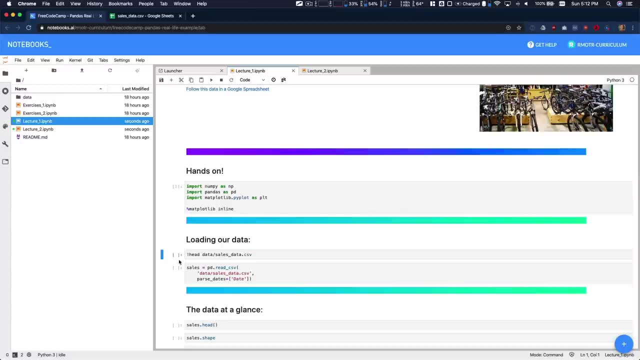 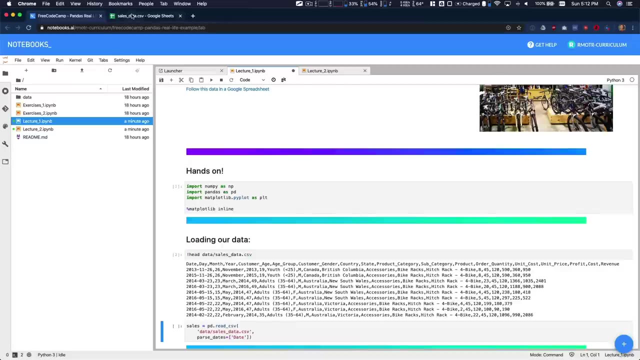 of our day to day process as data analysts, data managers, data scientists, using Python. So the first data set that we're going to use is a CSV file that has this form. you can find it right here under the data directory. The data that we're going to be used is this: 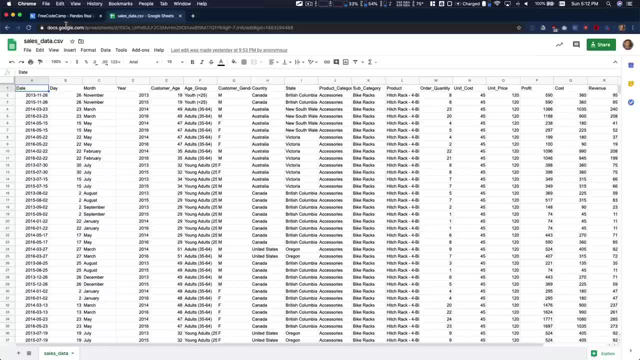 I have just transform it into a spreadsheet So we can pretty much look at it from a more visual perspective. But remember, as we said in the introduction, as data analysis we're going to be using Python. So we're going to be using Python. 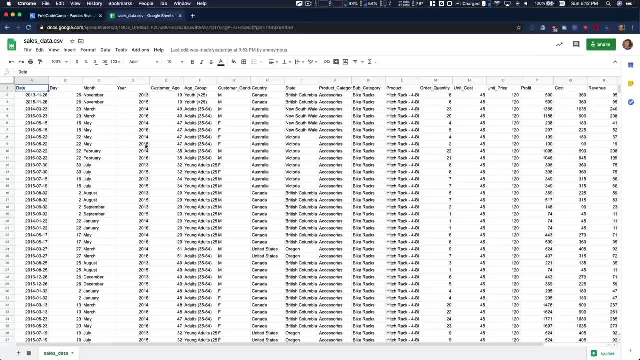 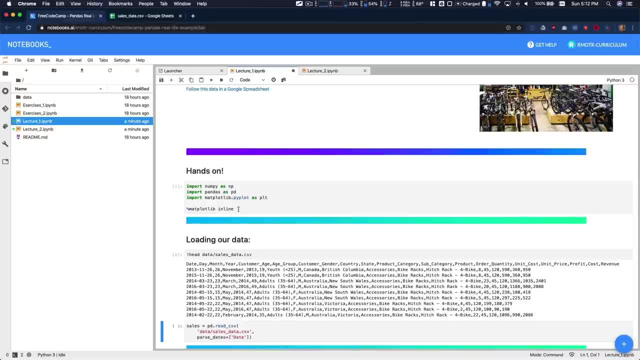 we are more driven by the understanding of the data right in the back of our head. we understand how, what the data looks like, what's the shape of it, And that's what it's conducting our analysis. So the first thing we're going to do is we're going to read it. 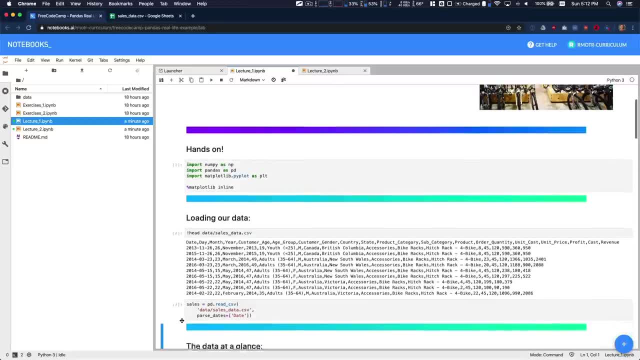 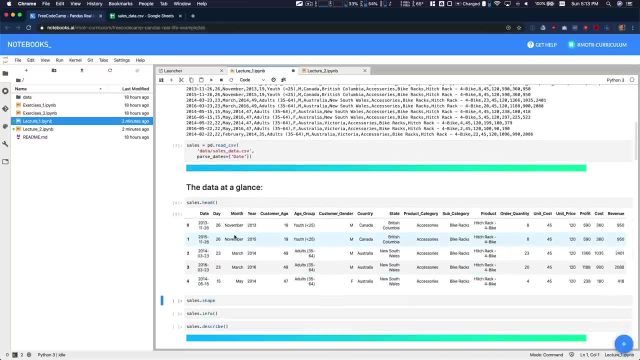 this CSV into Python And you can see how simple it is. just one line of code gets us the CSV read into Python. we're going to give a quick reference reference And this is what the data frame that we have created looks like: data frame. 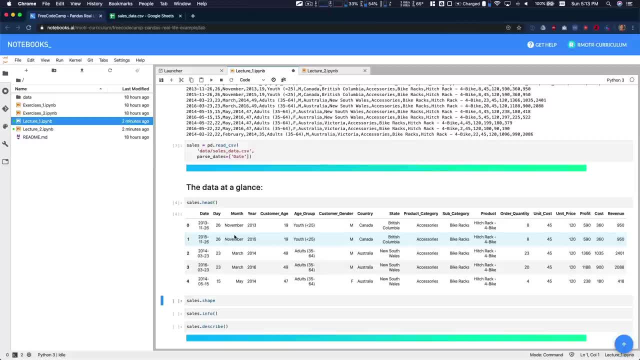 is a special word- is a special data structure that we use in the pandas tool, And again we're going to see that in detail in the pandas part of this tutorial. The data frame is pretty much the CSV representation but it has a few more enforced things like, for example: 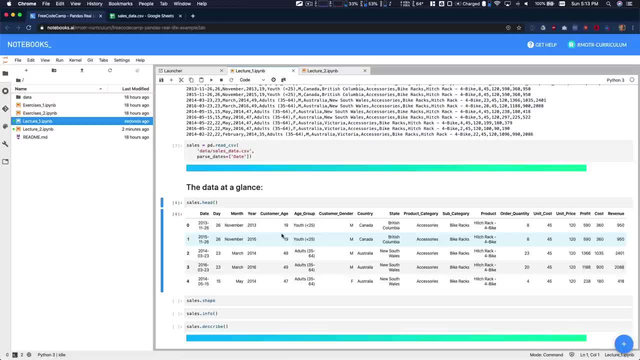 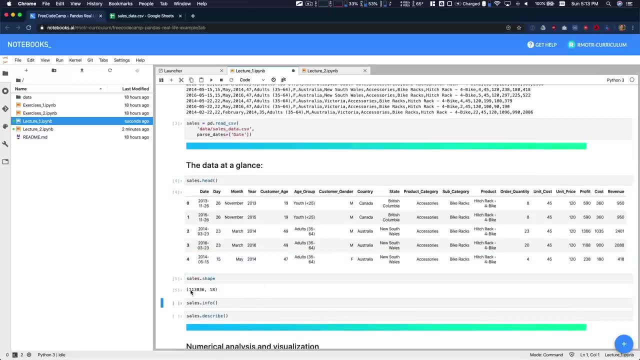 each column has a strict data type and we will not be able to change it, etc. It's a better way to conduct our analysis. the shape of our data frame tells us how many rows and how many columns we have, So you can imagine that with these amount of rows, it's not so. 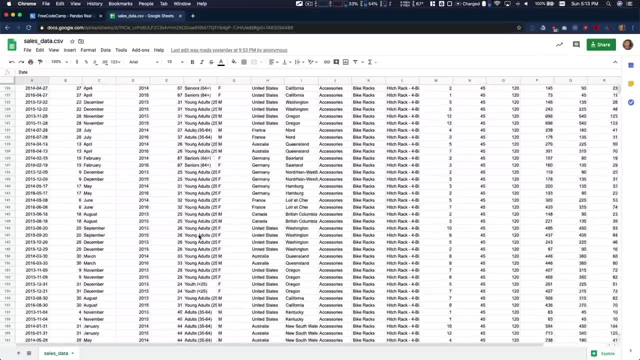 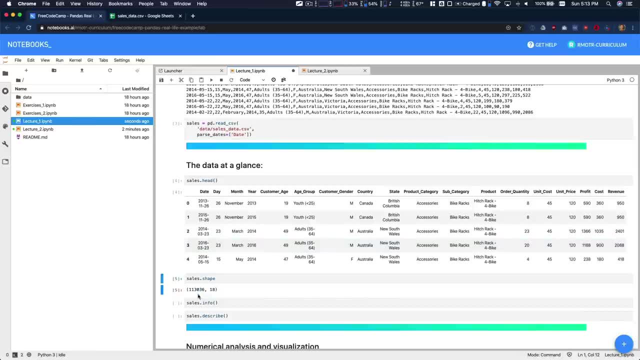 simple to gain. follow a visual representation of it's like it's pretty much infinite, scrolling in this point: 100,000 rows. But the way we work, we're going to be able to do a lot of different things. We're going to be able to. 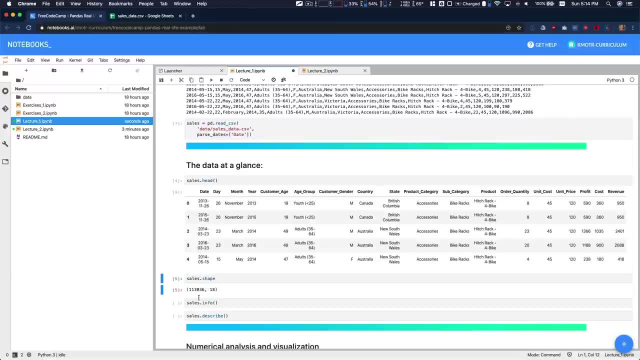 do a lot of different things. We're going to be able to do a lot of different things. We're going to work is by, immediately after we load our data, we want to find some sort of reference in the shape and the properties of the data that we're working with, And for that we're 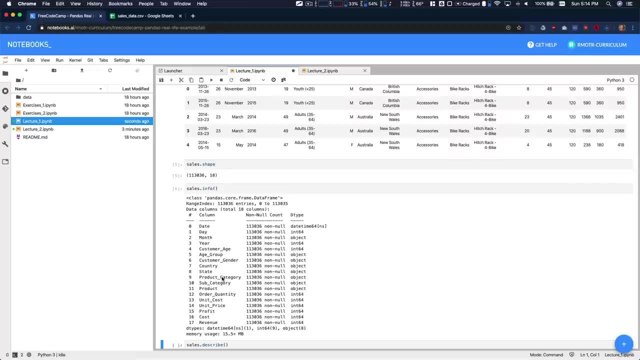 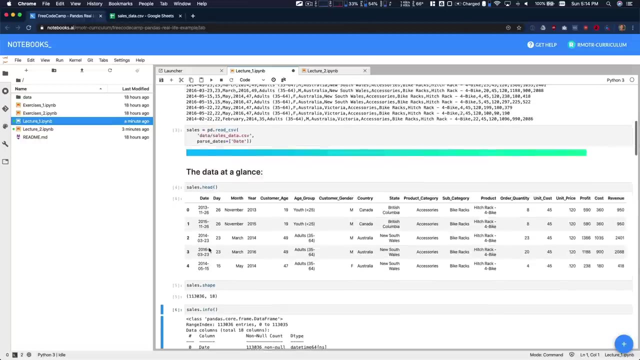 going to do first an info to quickly understand the columns we're working with. In this case. we have date, which is a daytime field. we have day, month, year and that are just complementary to the date. we have the customer age, which is an integer which makes sense, right age. 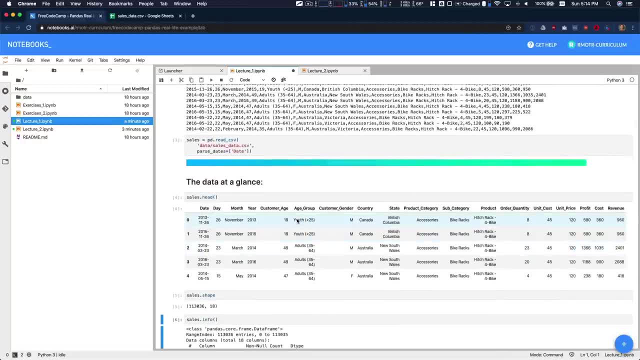 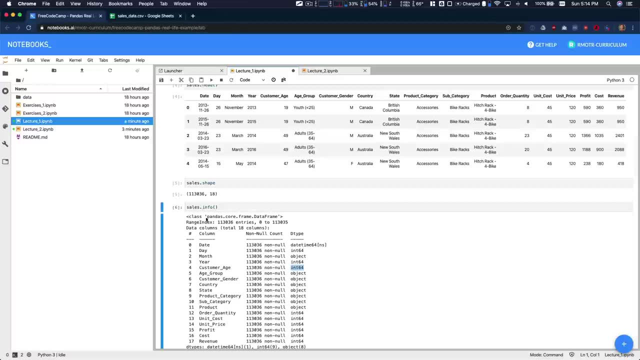 group. you can see it right here: it's age group, youth, customer gender. we have an idea again of the of the entire data set. we know the columns we have, But we also know how large it is And we don't care what's in between. we will be claiming it probably. 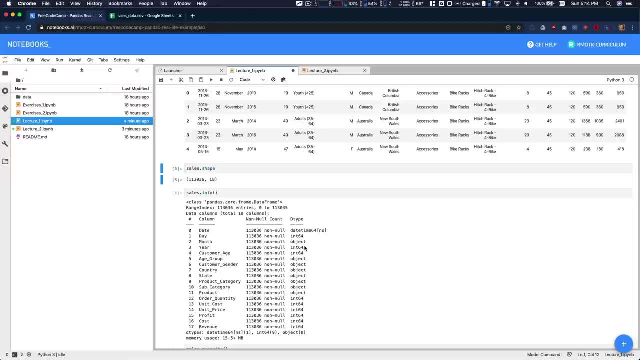 but we don't need to actually start looking bro per row right, just with our very limited eyes. we have a better understanding of the structure of our data in this way- And you know we're going one step further- we will also have a better understanding of the statistical. 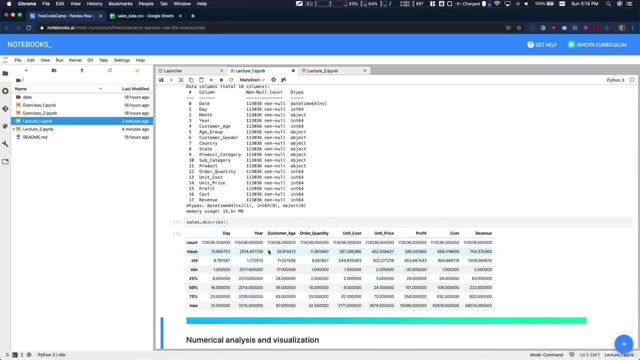 properties of this data frame. with a describe method For all those numeric fields, I can have an idea of the statistical properties of those. So, for example, I know that the average age of these data set is 35 years old. I also know that the maximum age in this 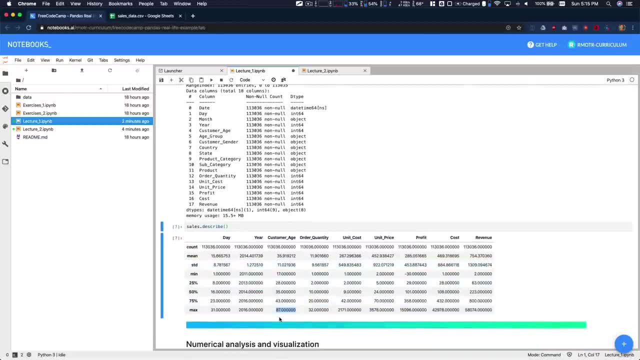 case- if these are, is a sales data- is 87 years old Now the minimum is 17 years old And again I can start building right at my understanding of the statistical properties of it. So in this case the median of my age is very close. 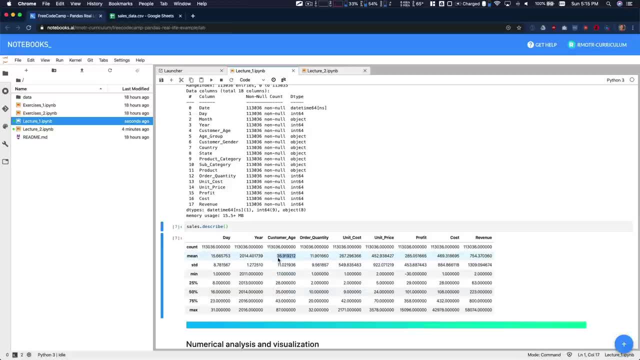 to the mean. So this is telling me, all this telling me something, and the same thing is going to happen for each one of the columns that we are using. For example, we have a negative profit here And we have very large values here. are these correct? Is this correct? 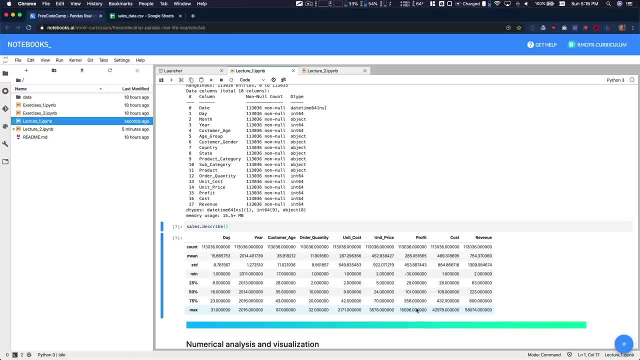 Is maybe this a mistake? Again, it's by having a quick statistical view of our data, we're going to be driving the process of analysis without the need of constantly looking at all the rows that we have. it's a. it's a more generalistic overview, So we're going. 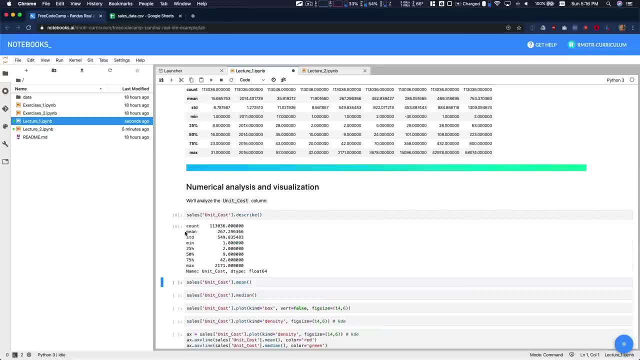 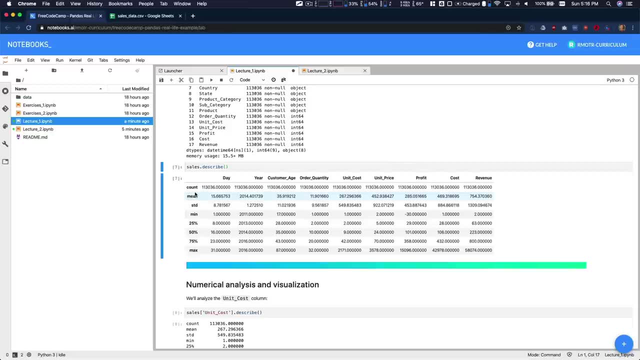 to start with unit cost, let's- let's see what it looks like And we're going to do- describe only a few net cost, which is pretty much what we have right here In the previous in this line, what we did was for the entire data frame, for the entire data In this case, 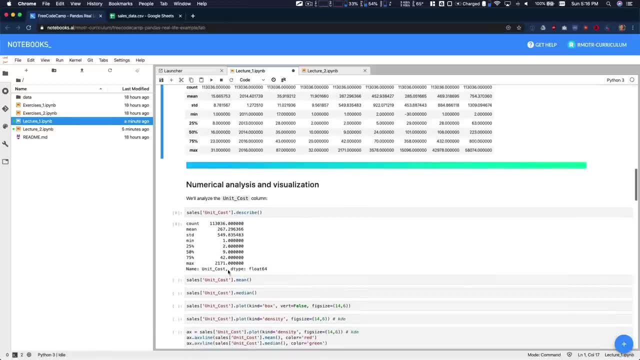 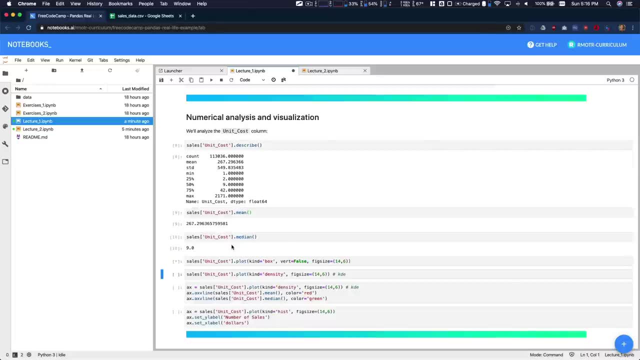 it's focusing in the unit cost. cost, sorry, column, the mean the median- all fields. we know already pretty much from this And we're going to quickly plot them. we're going to use these tools to visualize them. And it's the same tool, it's pandas that it's. 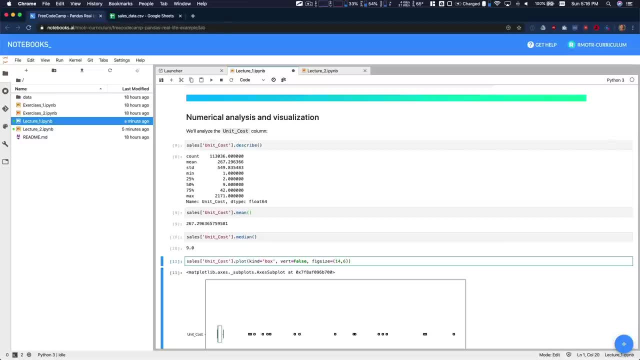 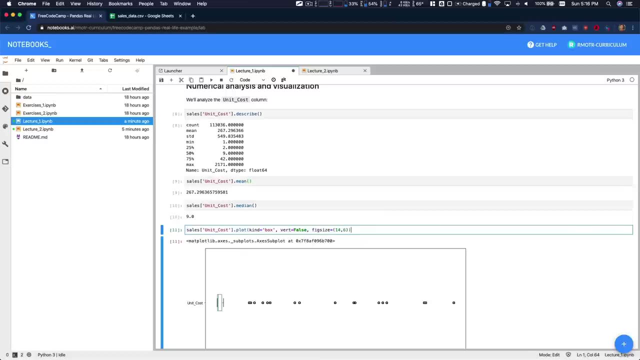 using on top right, It's using matplotlib, So the visualization is created with matplotlib, But we're doing it directly from pandas. And again, don't worry, this is all explaining the pandas lessons. So this is unit cost, right? This is what this is the, the, the. 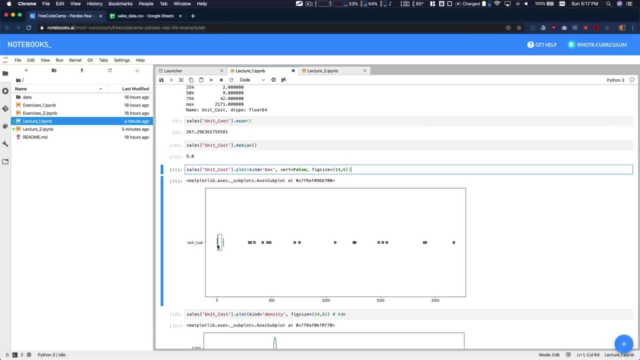 box but we have just created. we have the whiskers. that mean that shows us the first and third quartile, the, the median, And then we see all the outliers that we have right here. So we see that a product that is around $500 is considered to be an outlier And the 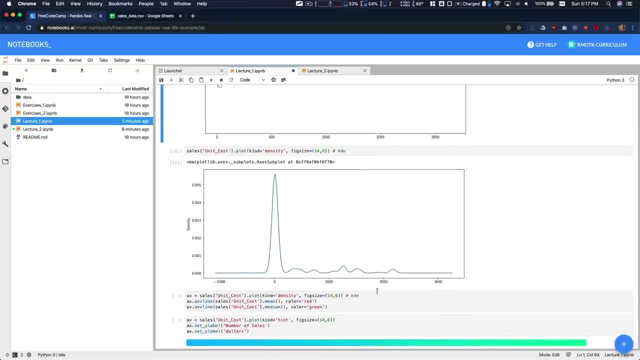 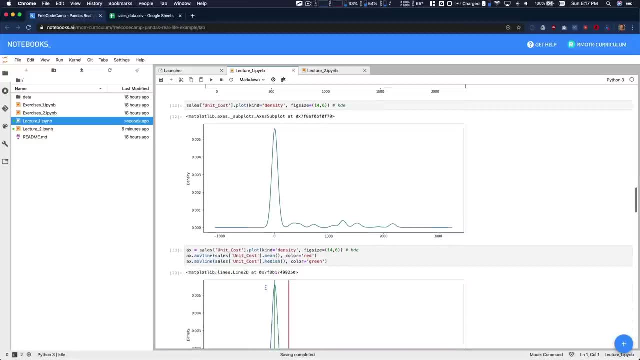 same thing if we do a density plot right. so this is what it looks like. we're going to draw two more charts right in which we're going to pretty much point out the mean and the median right in the distribution chart, And we're 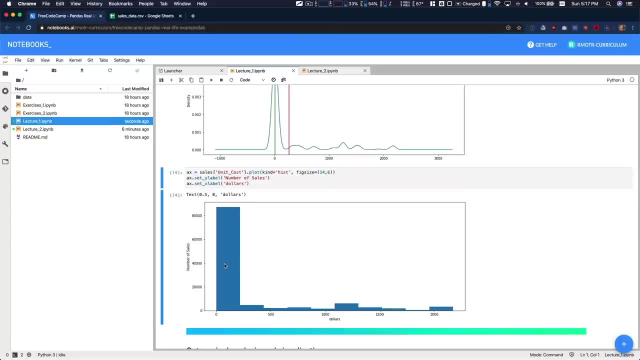 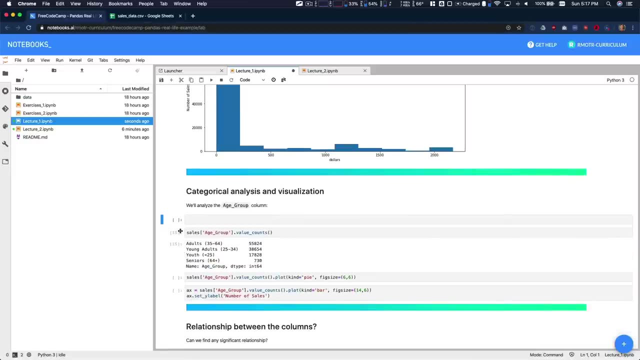 going to do a quick histogram of the costs of our products. Moving forward, we're going to talk about age groups, with the age of a customer And at any moment we can always do something like sales dot head to give a quick reference. We know that the the age 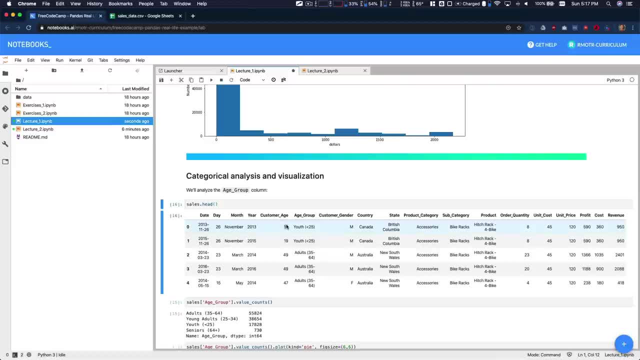 of the the customer is expressed in actual years old they were, but also they were the. they have been categorized with three of four, actually four age groups: seniors, youth, young adults and adults. right, So they we have given categories, were creative, right. 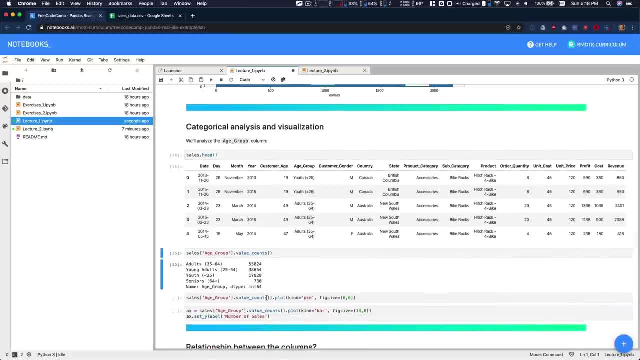 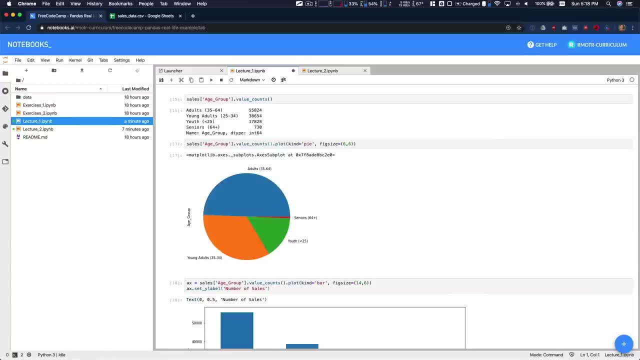 to better understand these groups, And we do that with values, value counts. we can quickly get a pie chart out of it, or we could get a bar chart out of it. As you can see, right here we're doing an analysis of our data. 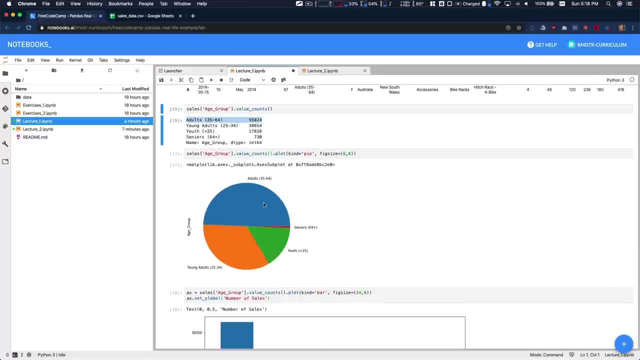 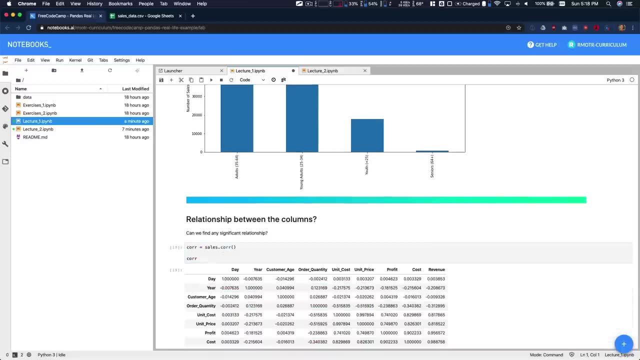 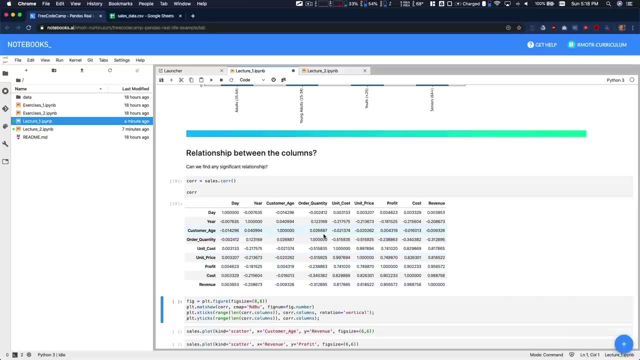 Yeah, we see that adults right here are the largest group in our, for our data at least. So, moving forward, what about a correlation analysis? What is the correlation between some of our properties? we will probably have high correlation, for example, between profit. 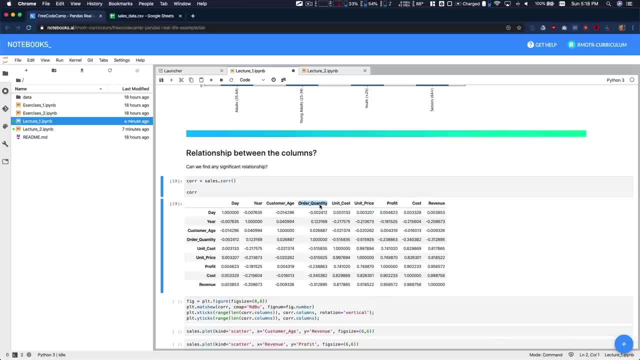 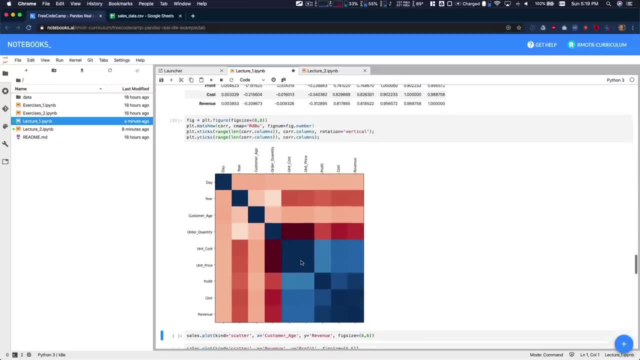 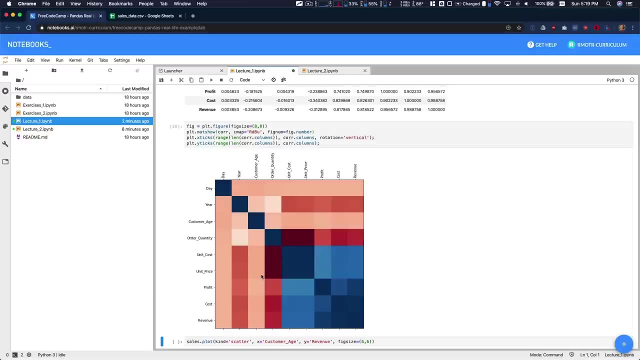 and unit cost, for example, or the quantity. that's kind of expected, but that's all something that we can do right here. This is a matrix right of correlation showing in red high correlation. So order quantity and unit cost, or where is profit right? here profit is right. 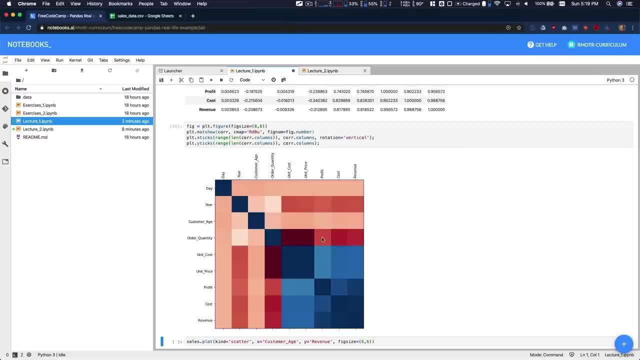 here. So we see high correlation with unit, with cost, with profit, not with profit. Actually it's the opposite. blue is high correlation. I'm sorry, the diagonal which is blue is correlation is equals one. So high correlation is blue And we see that profit has huge core, has a lot of correlation, positive correlation. 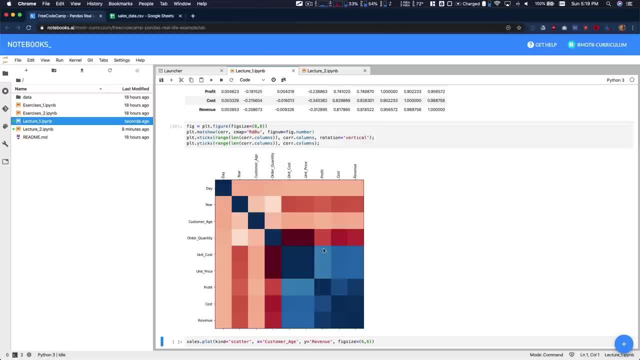 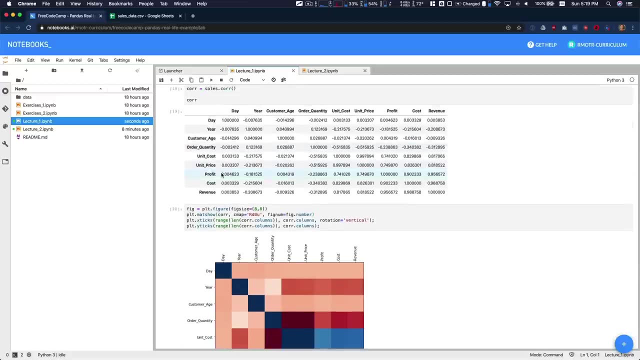 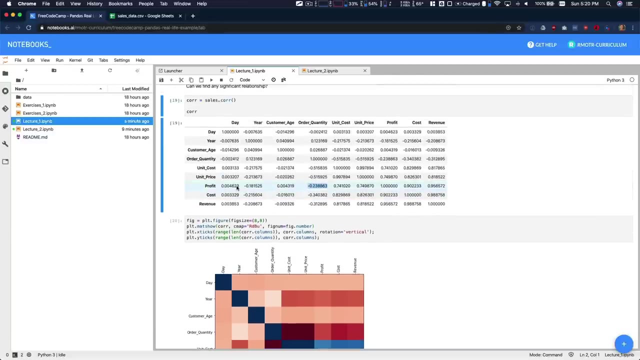 with unit cost and unit price, and negative correlation is with dark red. So we again can have a quick idea. Let's see, for example here: profit: it has negative correlation with order quantity, which is interesting, right It's. we want to dig deeper into that. 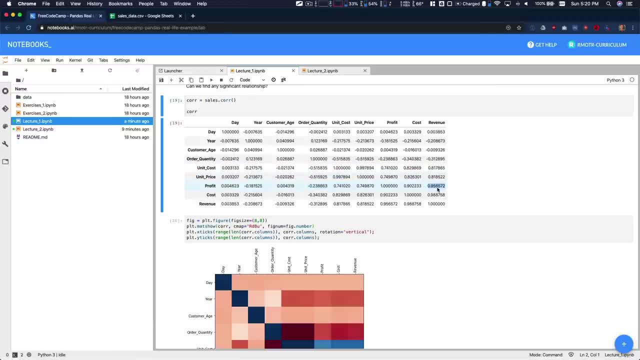 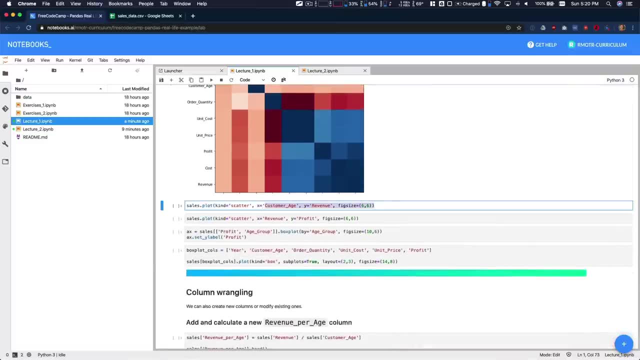 of course the profit has a high correlation positive with red Revenue right. And again, it's just a quick correlation analysis. we can also do a quick scatterplot to analyze the customer age and the revenue right to see if there is any. 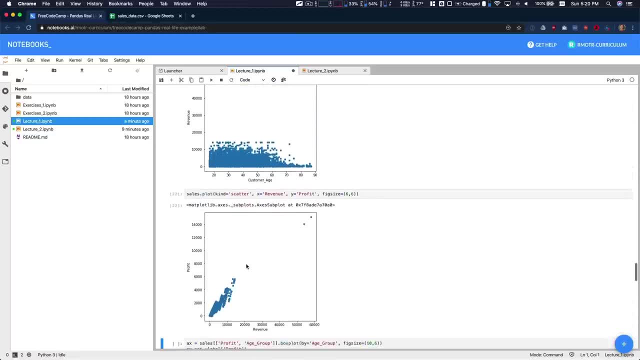 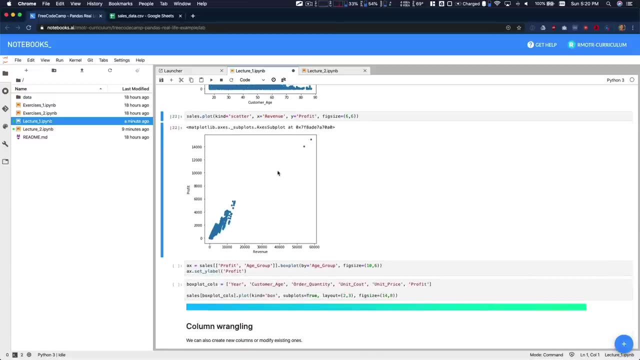 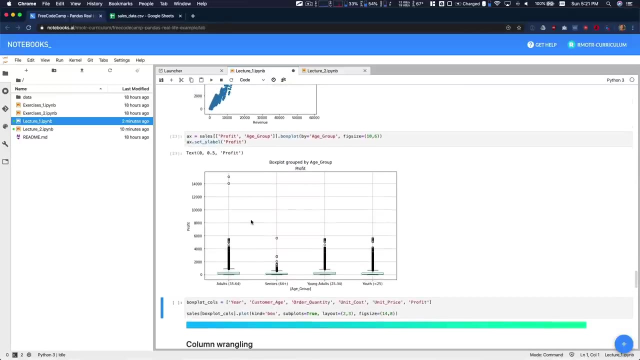 any correlation there, Right. And the same thing for revenue and profit. This obvious, right we can. we can quickly draw a diagonal here, right? so there is a lot of linear dependency between these variables. form a few more box plots, in this case understanding the profit per age group. right, so we can. 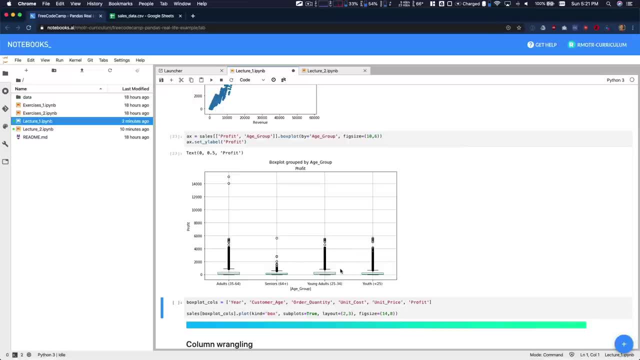 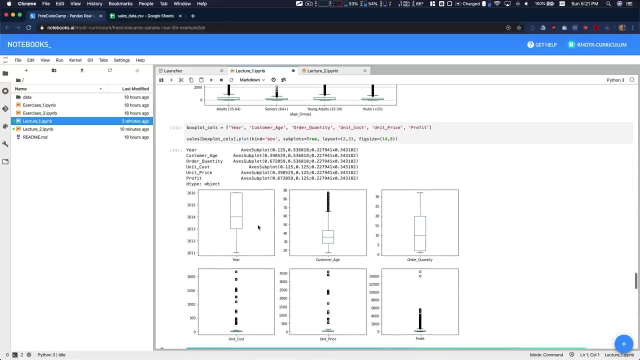 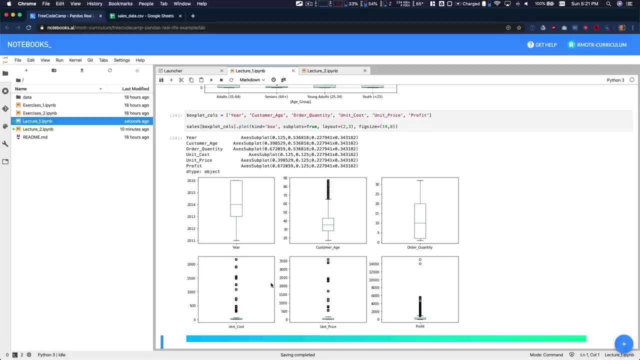 see how the the profit will be will change depending on the customer's age and a few more box plots, And we're creating these this grade of year, customer age, unit costs, etc. for multiple things. So moving forward, something that we can quickly do when we're working. 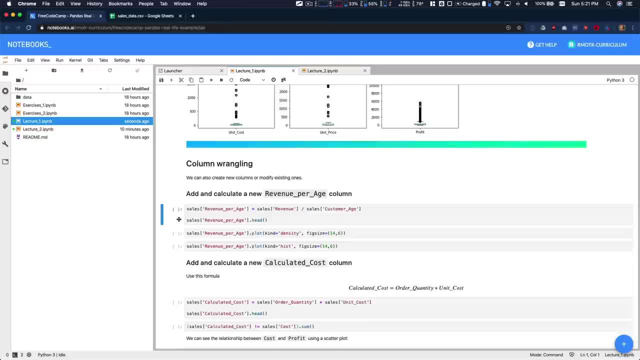 with Python, especially with him. this is to reshape our data or derive it from other columns, right? So this is pretty common in Excel. we can create these revenue per age column. if you're here in Google Spreadsheets, you're going to do something like revenue. 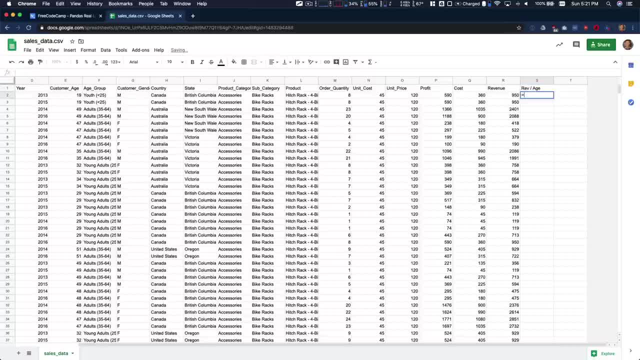 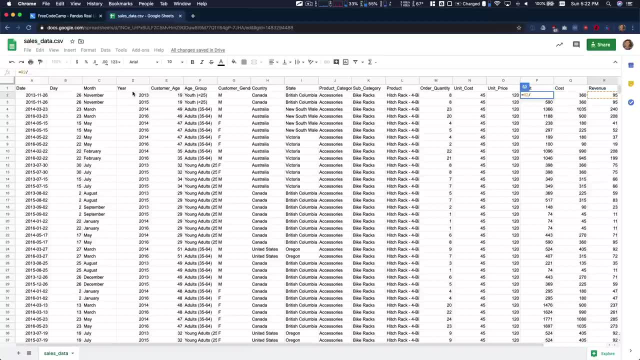 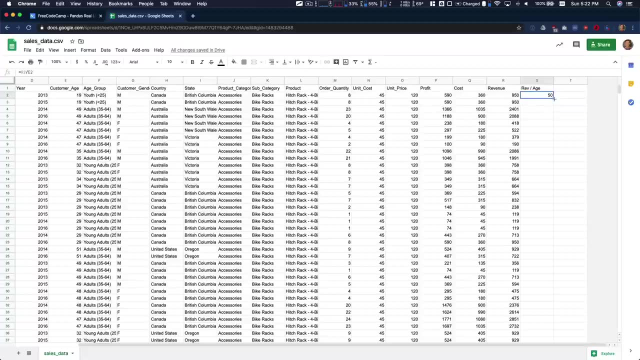 per age and you're going to do something like equals right, equals revenue per age, revenue divided. I don't remember this correct formula we're using, but just for you to have a reference, And we're going to pretty much extend this whole thing. There you go Well. 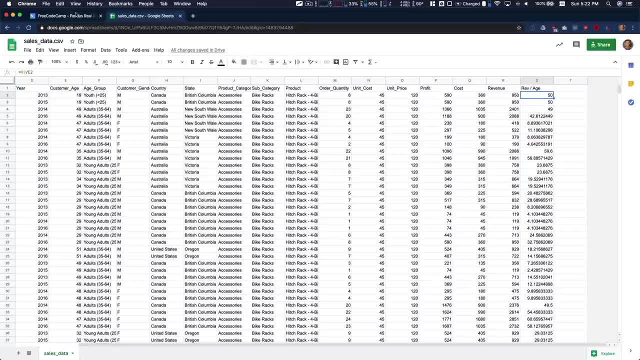 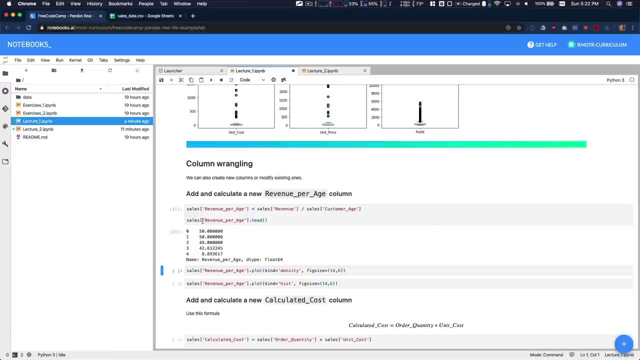 it's processing. I have 100,000 rows, so you can see how slow it is, And let's compare that just to the way Python works. I'm going to execute this thing. It was instant, you know, extremely fast, And it was all kind of. 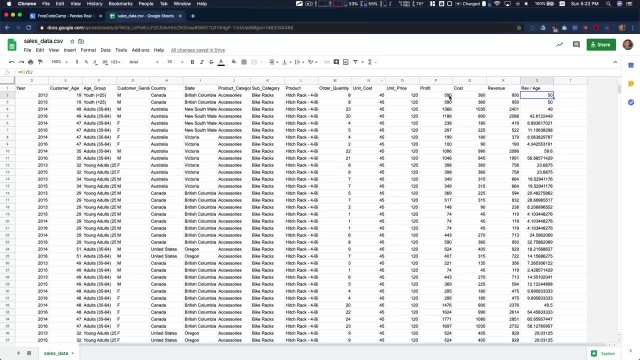 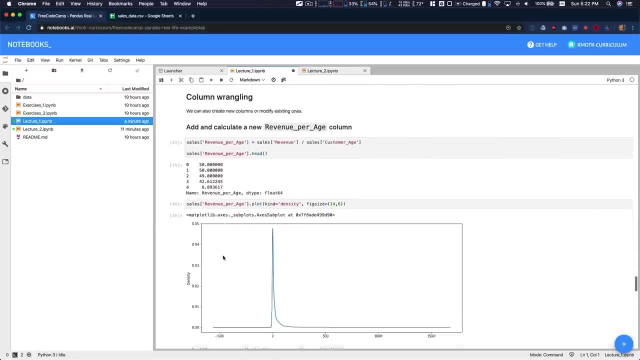 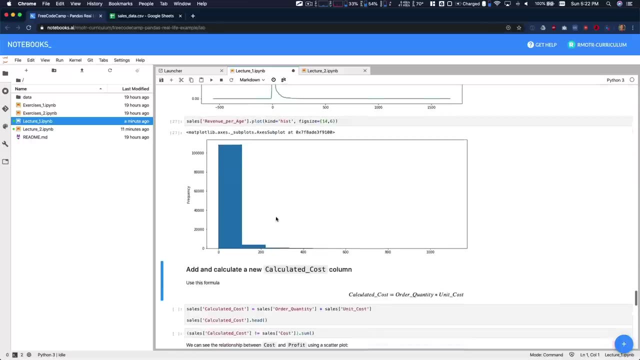 calculated, since we have the same results as expected. same results as expected, And we can quickly plot both the in a density plot and in a histogram. as you can see right there, not that revenue per age is going to be relevant In any case, it's just to show. 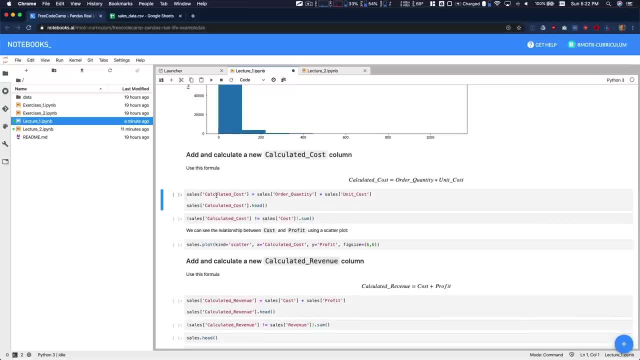 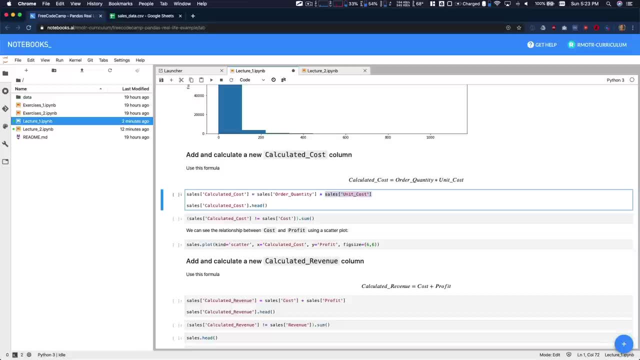 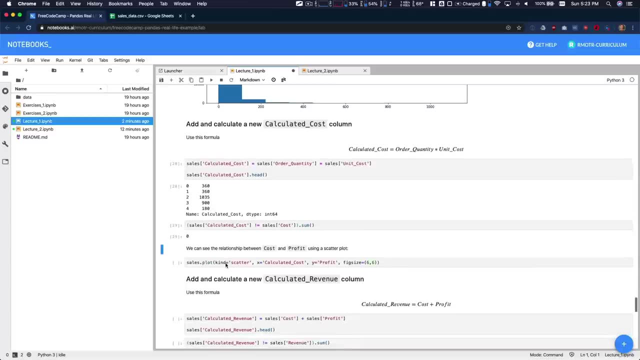 the total, the quantity of the order times, the cost right. extremely simple formula, very fast process, And we're gonna get right here how many rows had a different value than what was provided by cost. So what we're doing right here is like we're quickly checking. 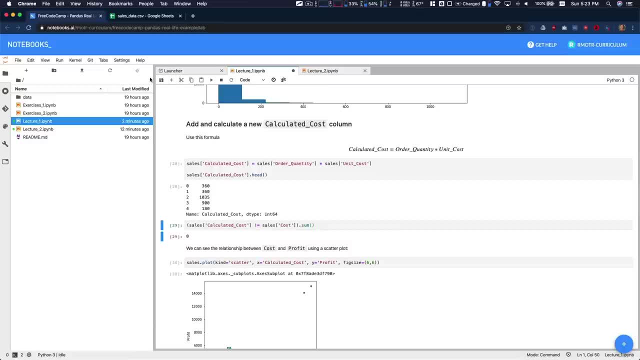 if the cost provided by the data set at some point doesn't align with the actual cost we are calculating. So is there any mistakes that were made by the- I don't know- the original system or people doing a data entry? If these new column is different from cost, we want to know about. 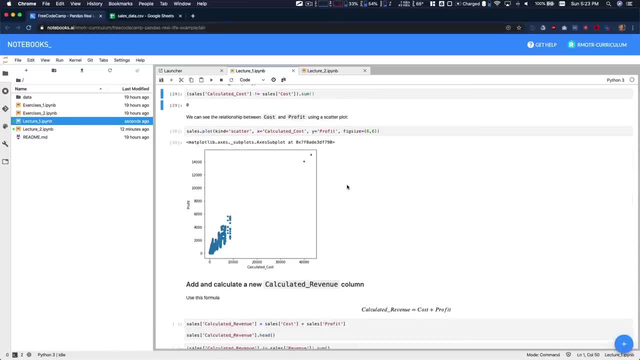 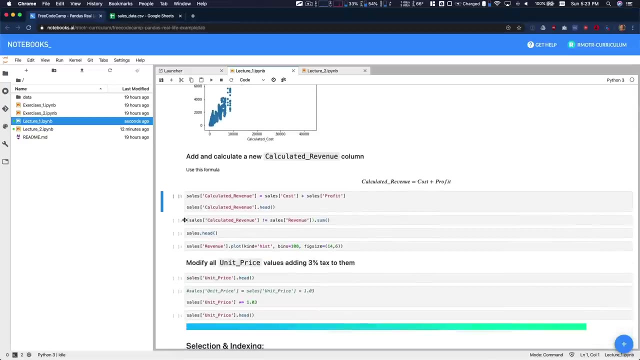 that And that doesn't happen. So again, quick, quick regression plot. In this case it's very obvious that there is some linear dependency between calculated cost and profit. So more formulas in this case cost cost plus profit. So we're gonna adding a little bit more. there is no difference with revenue and the calculated 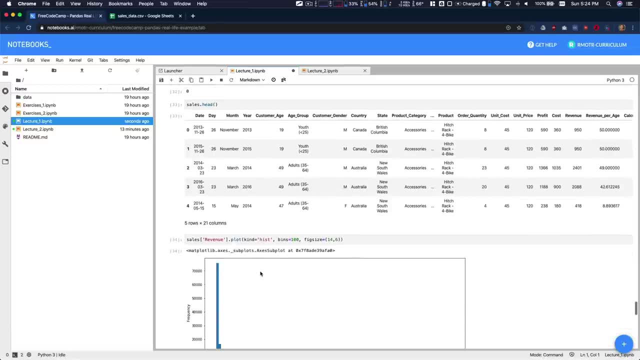 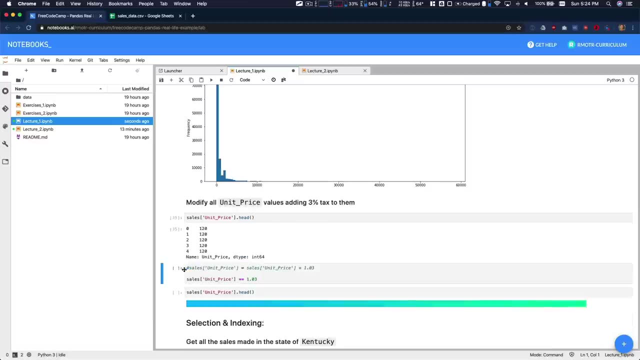 revenue that we are having. So that all makes sense. We're going to do a quick histogram of the revenue. We can, for example, on 3% to all the prices that we are using. we need to increase prices. how are you going to do that? Well, it's very simple, with Python. 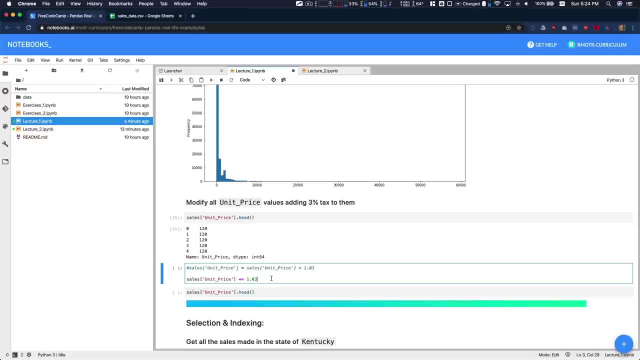 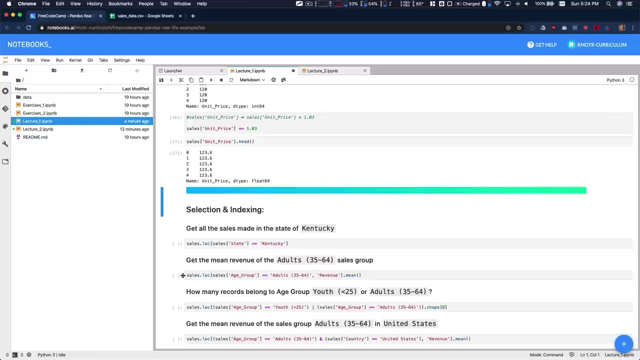 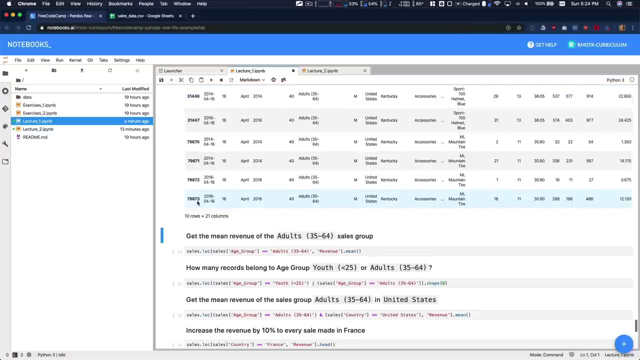 we're just going to do: increase everything by point zero three, And now we're going to see- now all the prices have changed- What else we're going to be able to do. quick filtering: let's get all the sales from the state of Kentucky, right? So these are all the sales. 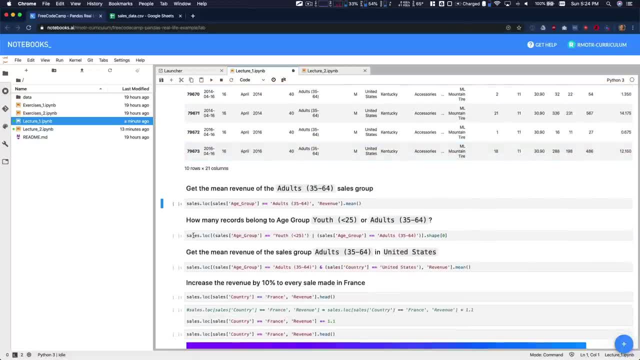 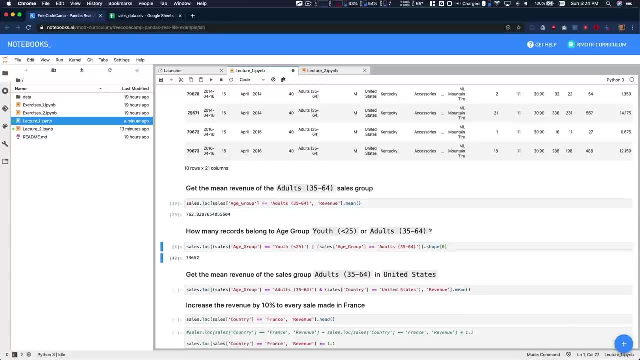 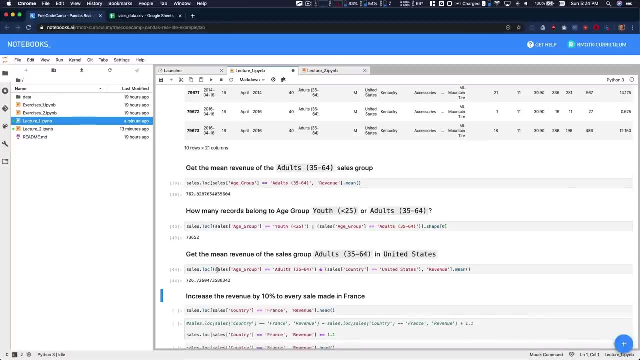 from the state of Kentucky. we can get only the average of the sales by these age group on only revenue, right? So these, all these filtering options are extremely simple to get with Python. In this case, we say: give me all the sales from these age group and also from this country, right, and we're. 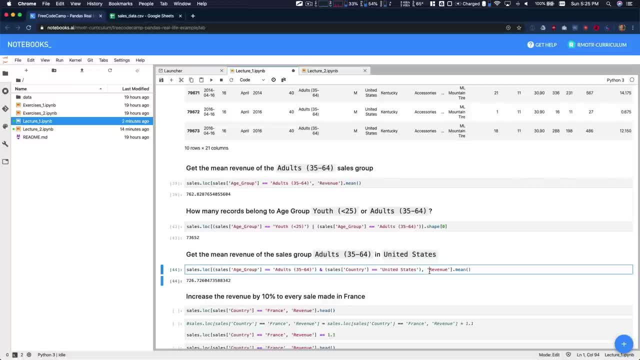 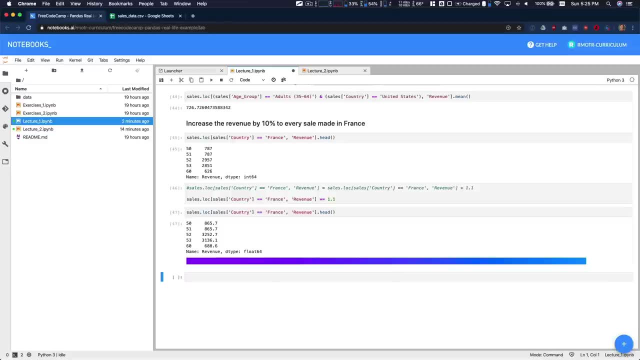 going to get the average revenue from these group that we are selecting And again, to modify the data. we can make just a few quick modifications, Like in this case: we're going to say all the sales from country, right, the revenue, we're going to increase it by. 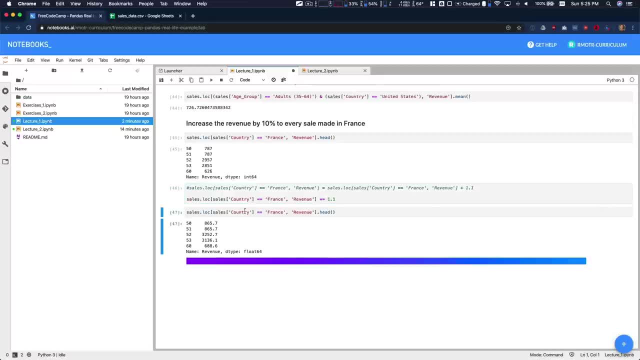 1.1.. I don't know why we're just doing it arbitrarily. It's just for me to show you how it works. So far, so good. Again, we've done a couple things you don't need to know about the details. 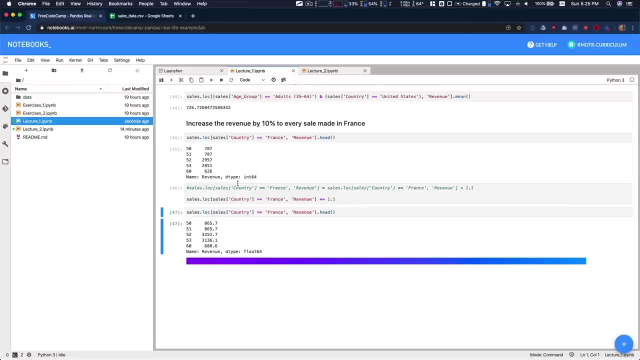 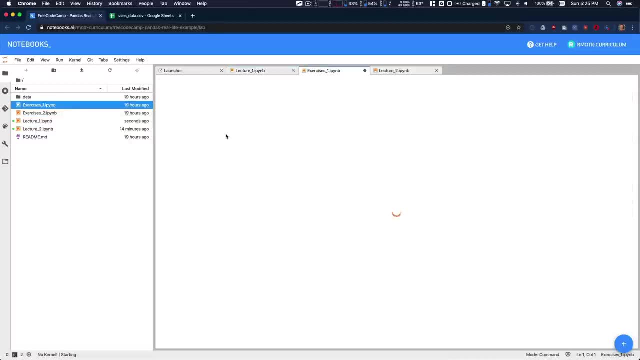 we will actually go through that in the NumPy independent sections in this tutorial. So just for you to have a quick reference of it, there are exercises associated with these given lecture. So if you want to pause right now and get into the exercises, that's going. 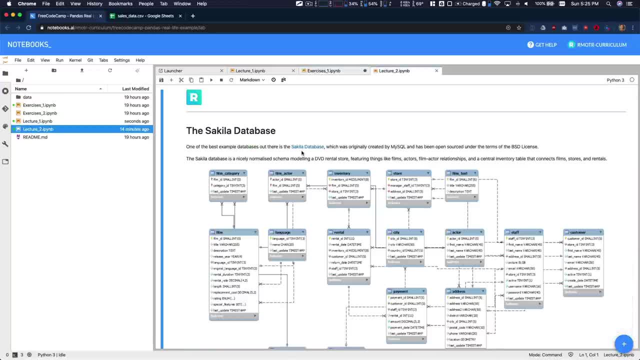 to be very helpful. We're going to move forward now with the second lecture, in which we will be using a database. There's a killer database and we're going to be reading data instead of from a CSV file as we did before. we're going to read data now from a database. Reading data from. 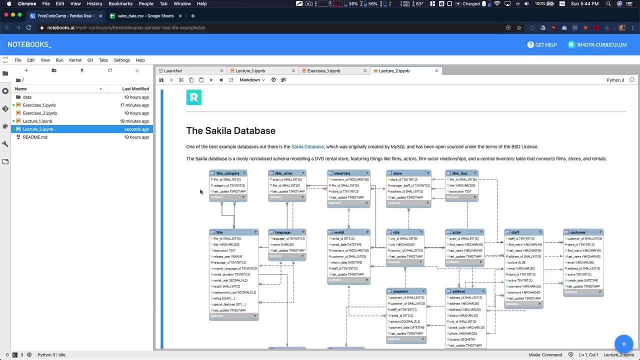 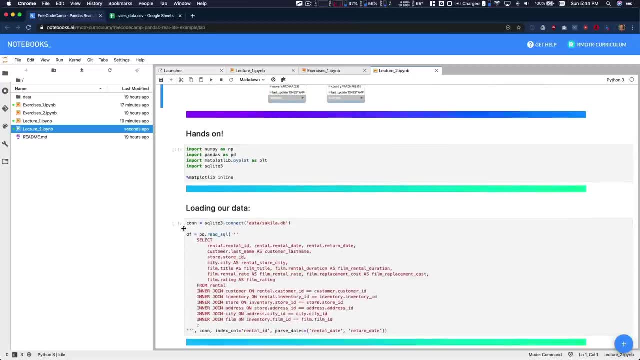 a SQL database is as simple as it is from an Excel file or a CSV file, as we were doing with our previous example, And once you've read the data, as we're going to do now. the process is the same. So what we have right here is a query, a SQL query. If you don't, 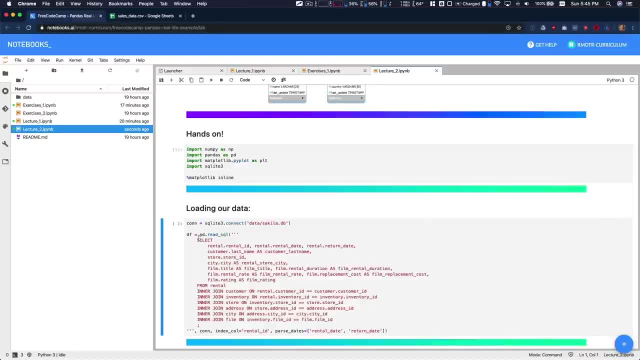 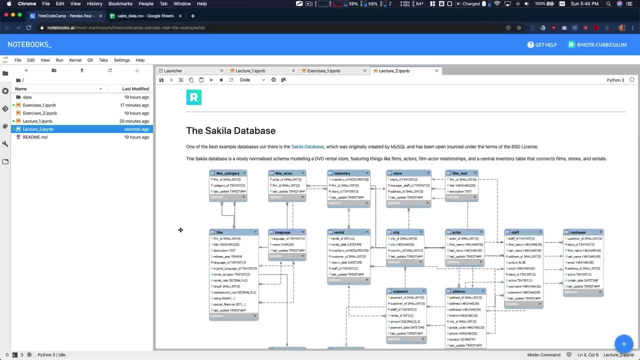 know about SQL. you can check our courses or other courses online And then you can see the process online. Basically, we're pulling the data from the database. This is one of the advantages of Python, it's not. there are connectors for pretty much every. 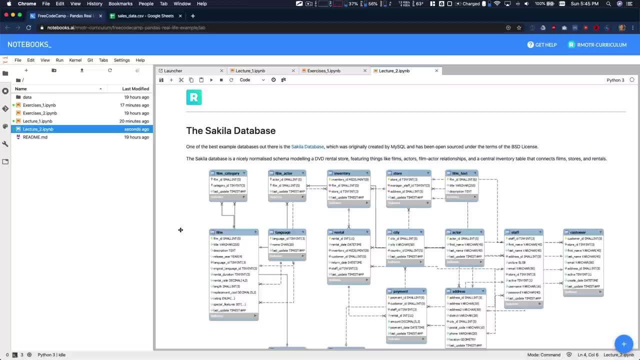 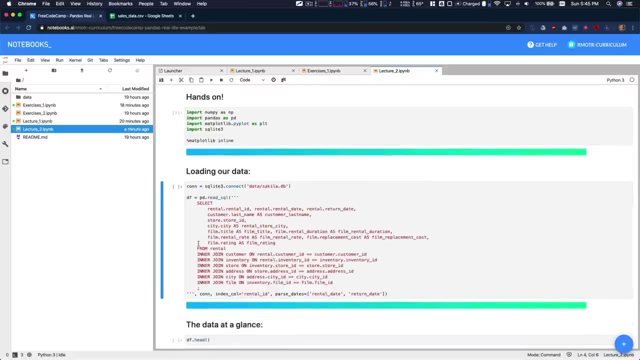 database provided out there- Oracle, Postgres, MySQL, SQL Server, etc. In this particular example, we're going to be using MySQL, So once you construct the query and you pull the data from the database, then the process is the same. we have just converted these. 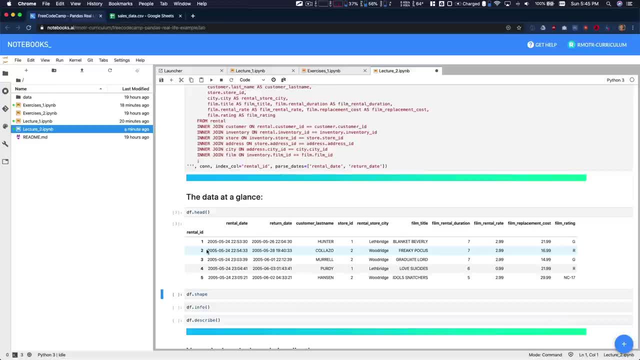 outside data into data frame that we can use with our Python skills. First step, as usual, is to check the shape, information, description of our data, of our data frame. In this case, we want to again understand the structure of it, So we want: 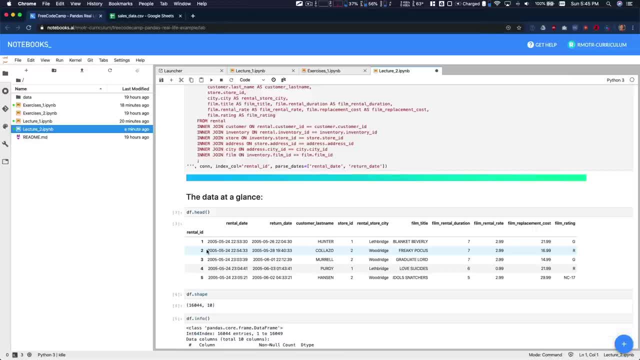 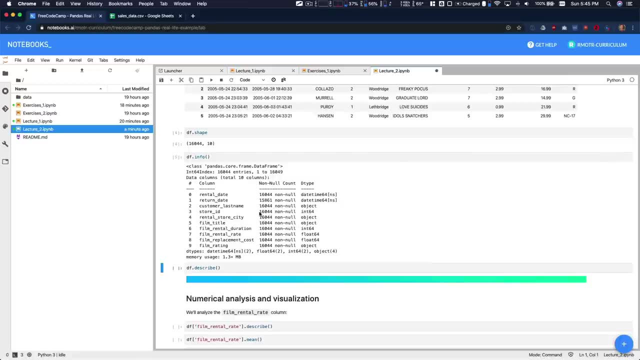 to know how many rows we have- 16,000,. we want to know a little bit more about our rows. we want to know about a little bit more about our columns and how many rows, how many records we have for each one of them and the type of each one of these columns, And we also 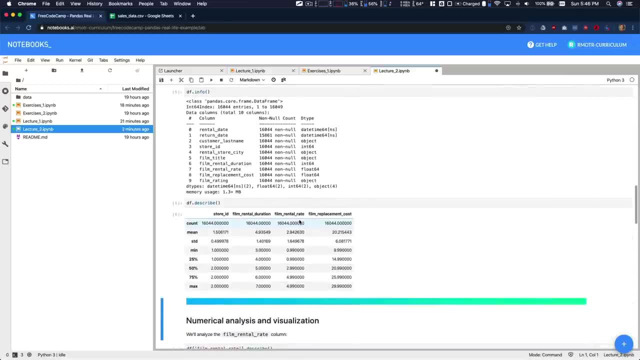 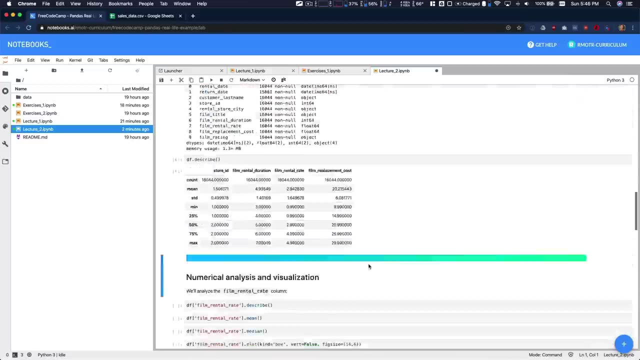 want to have a better statistical understanding of our data, So we do a quick describe and we have more details about it. If we want to focus in individual columns, right, we can just do that by. in this case, we're going to focus in film rental rate, right, pretty much how much you pay. 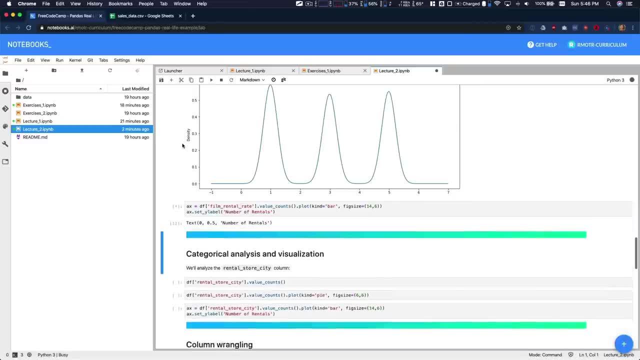 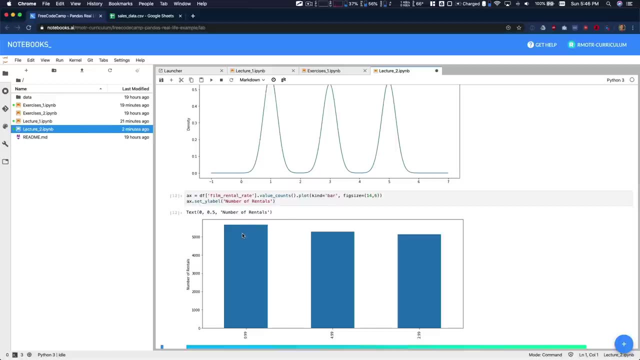 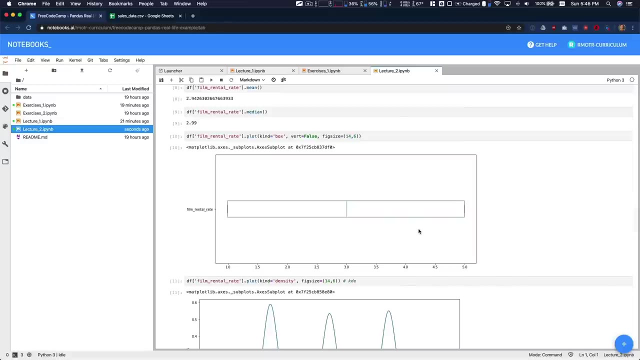 to rent a film and we're going to see the kind of distribution we have. we can call it distribution. it's pretty much a categorical field in this case. But basically the rentals are divided in three main categories or prices: 099, 299, 499.. So that's this box. plot is pretty. 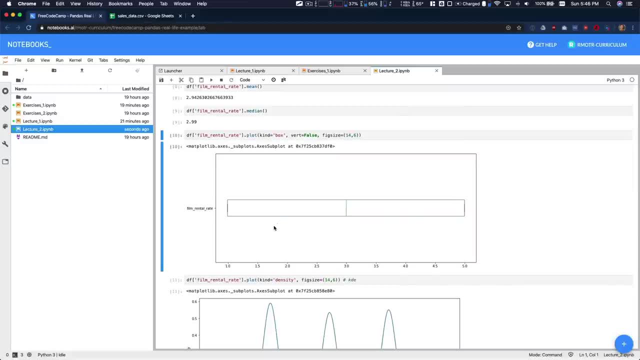 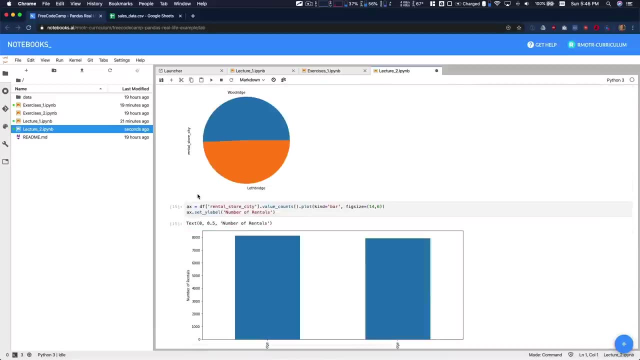 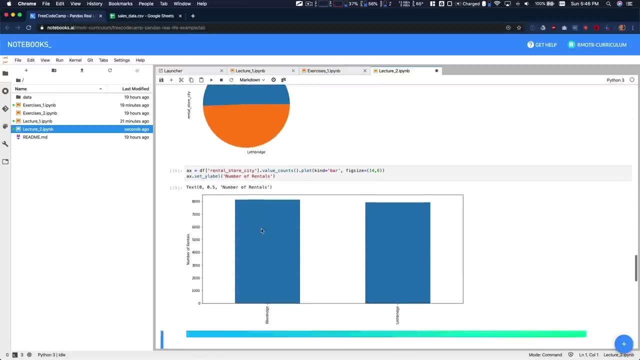 much perfect, never seen in real life. plot box plot gives you those prices And, moving forward, we can also check very quickly a categorical analysis understanding the distribution of rentals between cities. So we have two cities and it's pretty much even, as you can see. 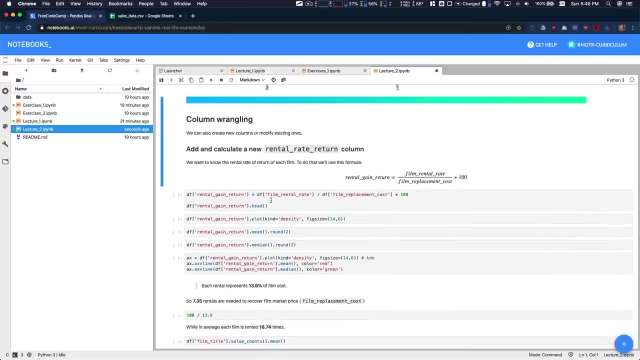 right here. creating new columns and reshaping the data for further analysis, etc. is relatively simple. In this case we're going to analyze their return in rentals, right which you know which films are going to be more profitable for the company dividing the rental rate. 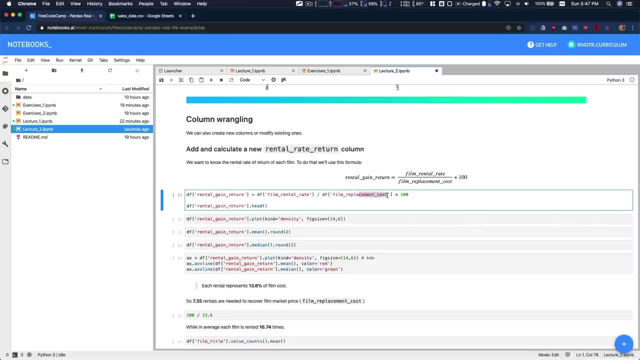 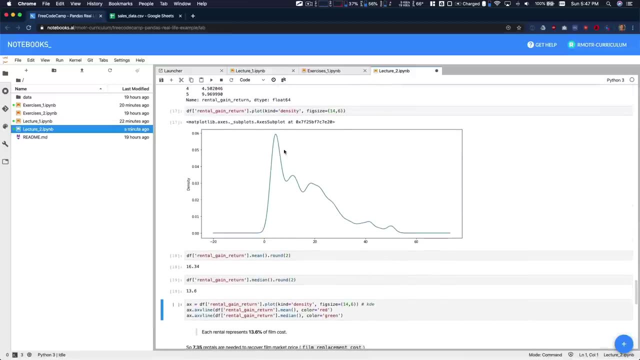 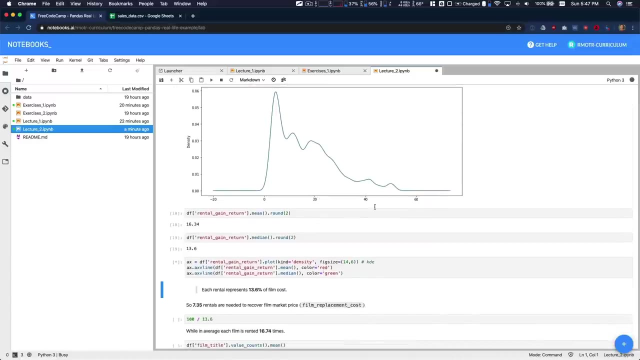 how much we charge divided by the cost, how much it costs us to acquire the film. So in this case we can see the distribution of that right. So most rentals are here in the beginning, and then we have more profitable rentals. we're making up to 60% above the. 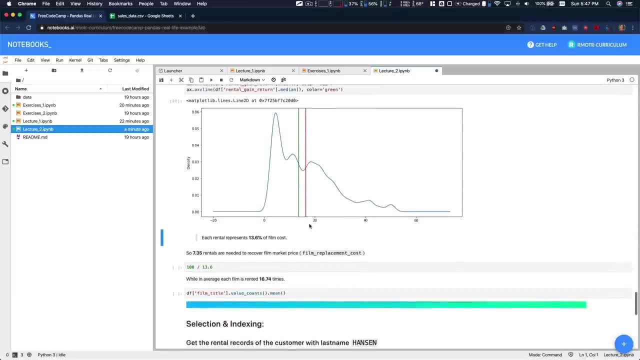 rental And we can quickly analyze the median rentals. So we can quickly analyze the median rentals. And we can quickly analyze the median rentals. And we can quickly analyze the median rentals. So we can quickly analyze the median and the median of it. right to to have a quick. 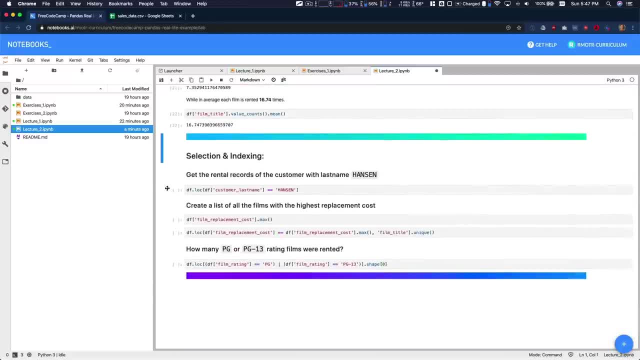 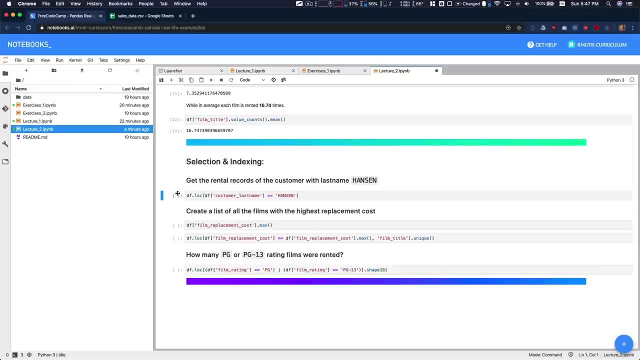 idea of all that. Finally, selection and indexing. if you want to start focusing, if you want to go in the data right, you want to zoom in, you want to have a better understanding, so you start filtering. In this case, we can filter by customer. but if you want to do, 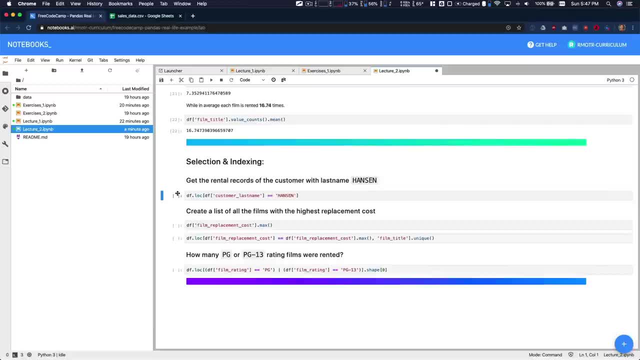 it per city, if you want to do it per state, if you want to do it per film, per price category, etc. it's very simple to fill, to filter and zoom in. just real quick. Thank you. one particular characteristic of your data so you can perform a more detailed analysis. 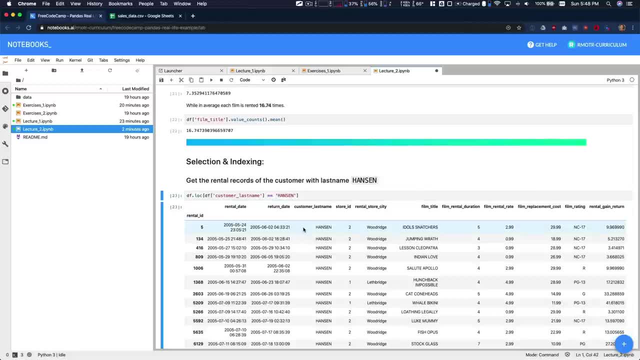 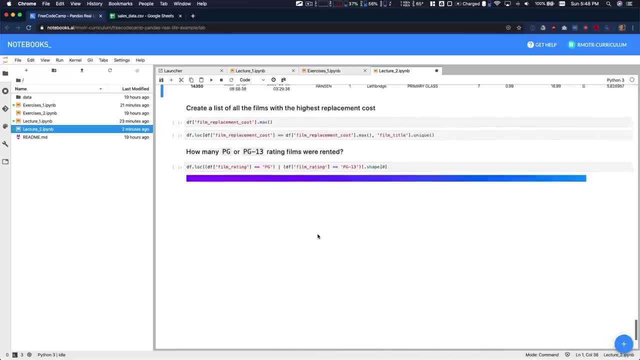 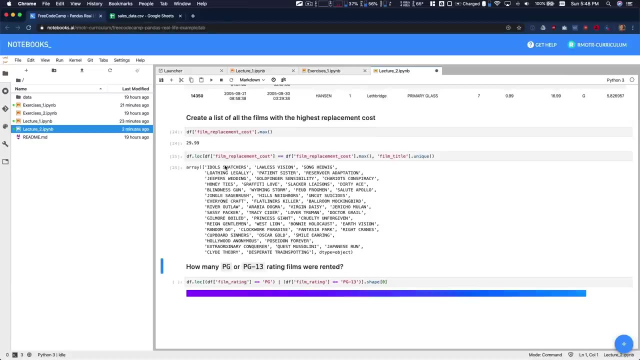 So in this case we have all the the films that were rented by the customer last name Hansen, which doesn't mean it's the same person. But again, it's very simple to filter that And here we can do. we can very quickly see which ones are the prices, the films, sorry. 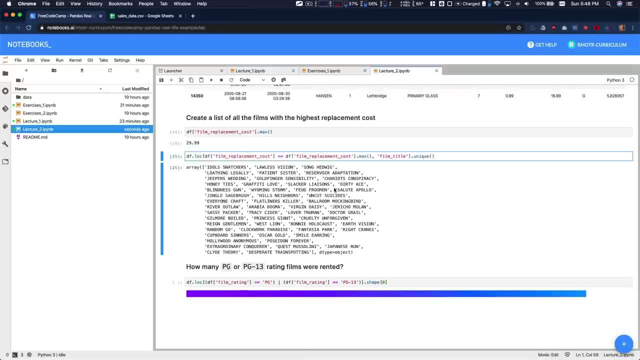 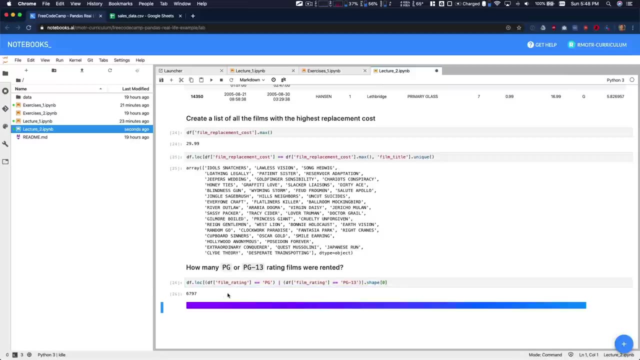 that have the highest replacement cost, right? So basically, what we're doing is we're going to isolate those films that have the highest replacement cost And also we can see right here, just for you to have an idea, all the films that are in the category PG, all the. 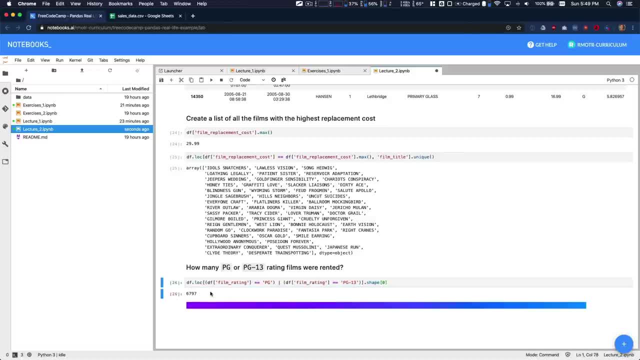 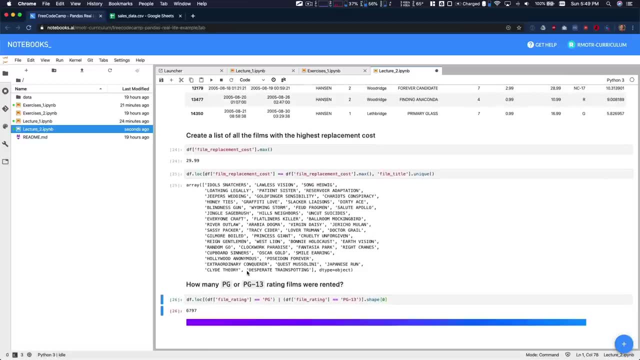 films or PG 13,. it's very simple also to filter that data. So this is the process we usually follow: we import the data, we reshape it somehow, create columns. there is an important process of cleaning, but we're not highlighting this part of the tutorial we're going to 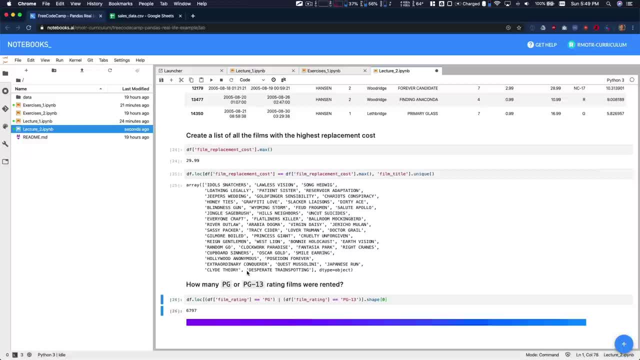 talk about it in the tutorial itself. There's the process of cleaning, then reshaping, creating new columns, combining data and creating visualizations. This is the process, right, that we're following here with our Python skills. there is a ton more to add, as you. 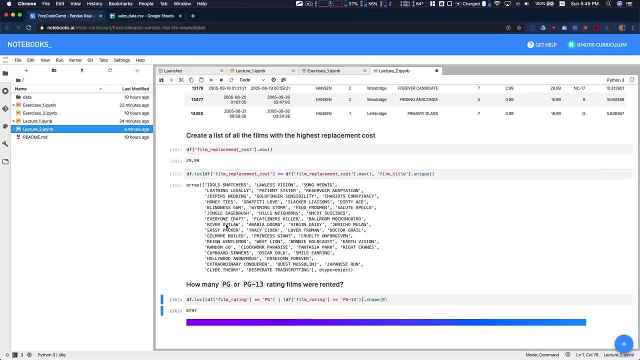 might imagine, From creating reports to running machine learning processes, creating linear regressions, etc. For now, this is just a quick understanding of the process we follow And now, starting now, we're going to move forward with more details of each one of the individual tools. 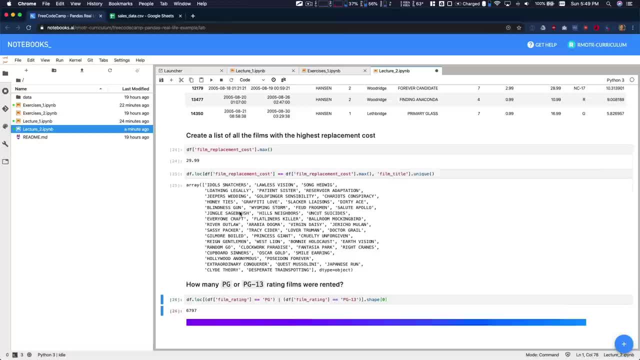 we're going to talk about. We're going to talk about Jupyter notebooks. we're going to talk about NumPy. we're going to talk about pandas. we're going to talk about matplotlib, seaborn, etc. Starting now, right, the first thing you're going to see is: what is this whole thing that? 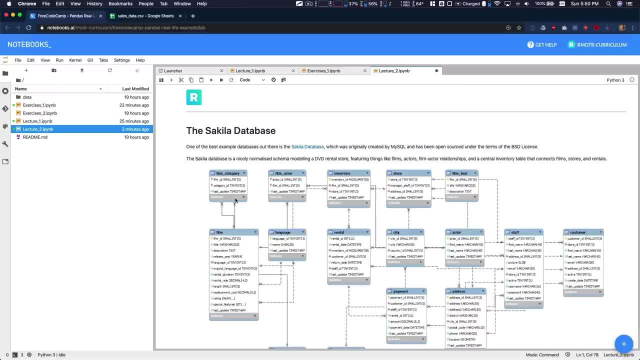 I've been using this Jupyter notebook. I want you now to. if you want, if you, if you don't have experience with it, I want you to have an idea of how it works And then we're going to move forward. the individual tools: NumPy pandas, etc. Remember, there are exercises. 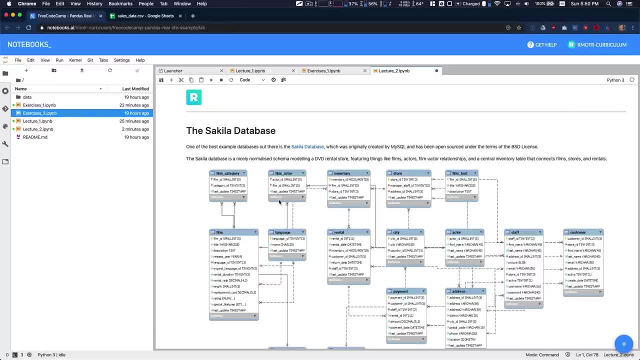 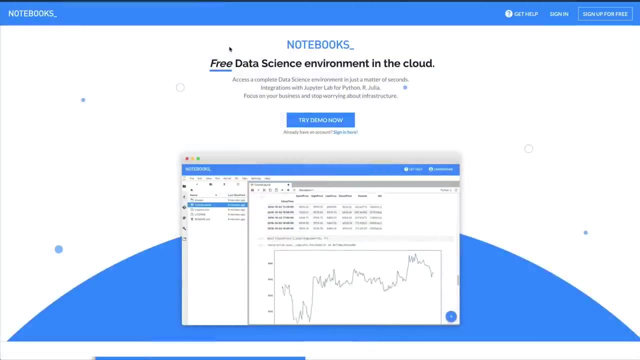 also associated with this particular lecture, So you can always go back again and work with them once you get more a better understanding of the tools we are using Before we jump into the actual data analysis course and we start talking about Python. 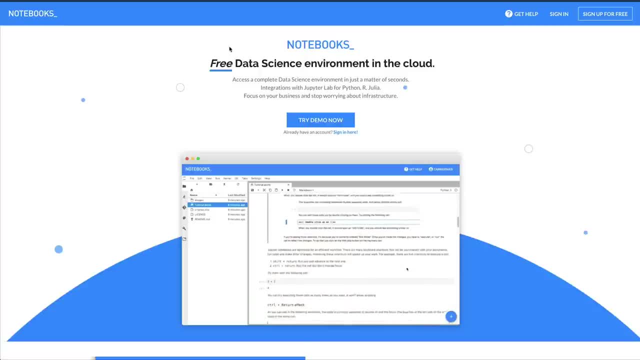 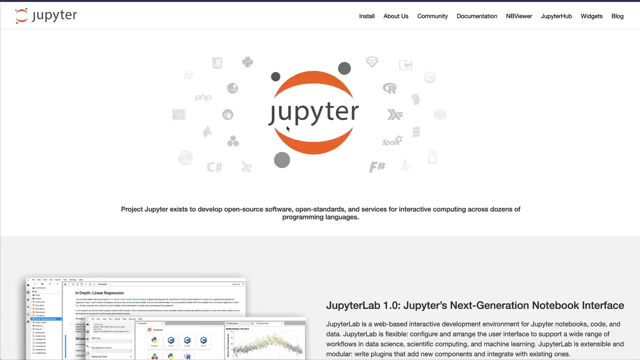 pandas, all the tools we're going to use: import files, read data from databases, etc. I want to show you the environment that we work with. It's our primary environment, it's the tool that we use 99% of the time and it's Jupyter notebook. There are a couple. 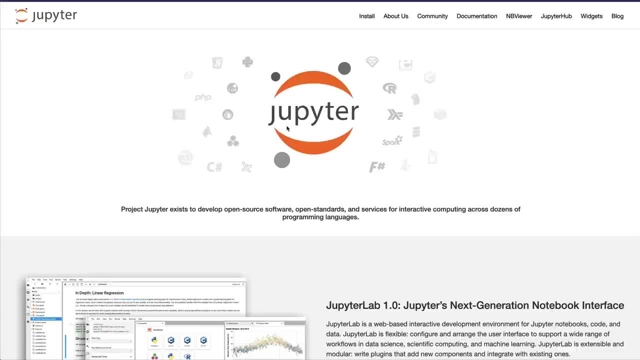 of different terms here. I'm going to be referring to it as Jupyter notebook. But, as you're going to see in this, in this part of the of our tutorial, you're gonna see the Jupyter is actually a whole ecosystem of tools And it's a very interesting project. Jupyter is a free. 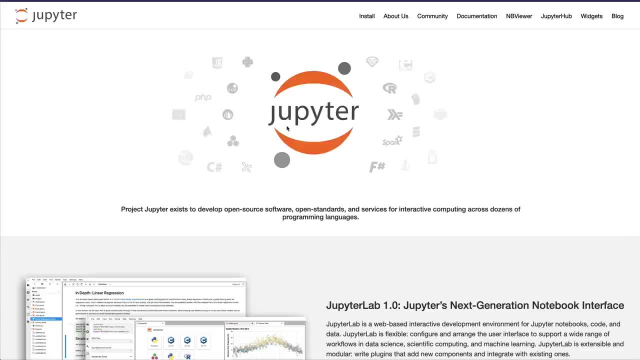 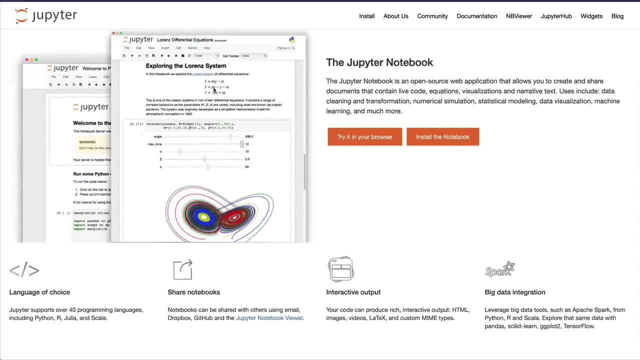 and open source again, ecosystem of multiple tools, And primarily we're going to talk about first what is a Jupyter notebook, what you're seeing right here and you're going to see what is a Jupyter notebook, what you're seeing right here and you're going to see. 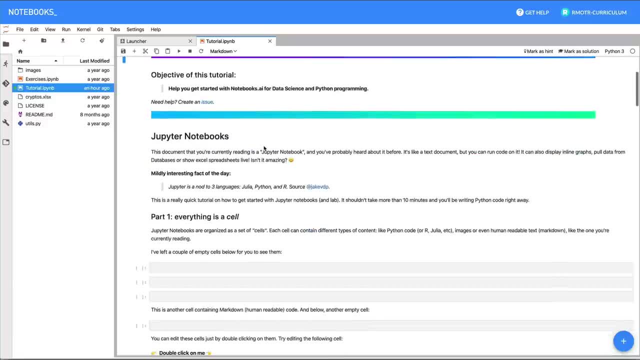 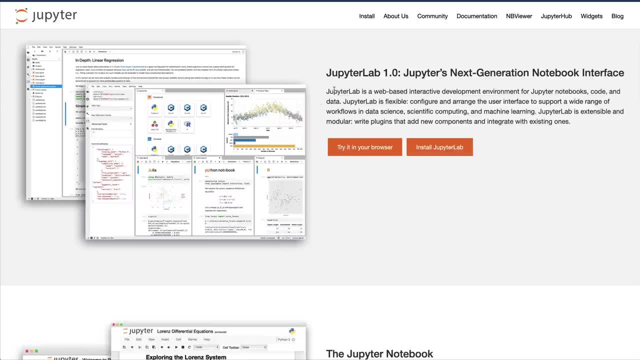 live in a second I can actually show it to you- is this thing we're going to use- And we are also going to talk about Jupyter lab. okay, which is the evolution of the regular Jupyter notebook. So I think this could be familiar to you already. Usually the questions: 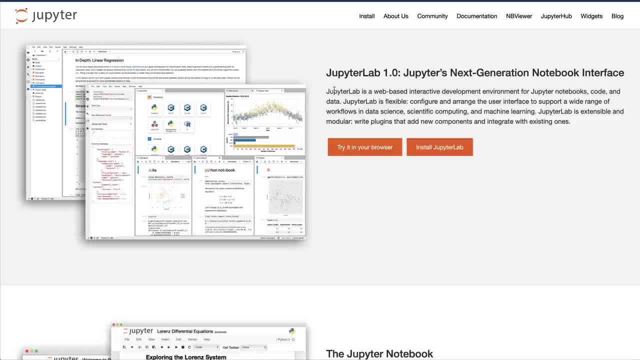 is. the question is: what's the difference between Jupyter notebook and Jupyter lab? Well, the difference is that Jupyter lab is just a nicer interface on top of Jupyter notebooks. it's not just the plain notebook. this is a notebook, but I'm scrolling right. 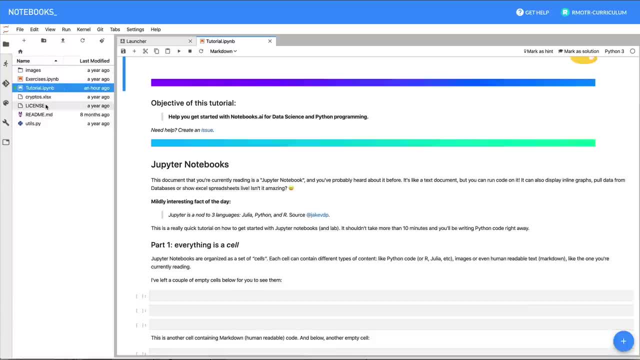 now. It's also the addition of a tree view, it's an addition of get tools and it's an addition of command palette and multiple other things. you can open some files with a nice preview in it, etc. So Jupyter lab, Jupyter notebook, they are similar, Jupyter. 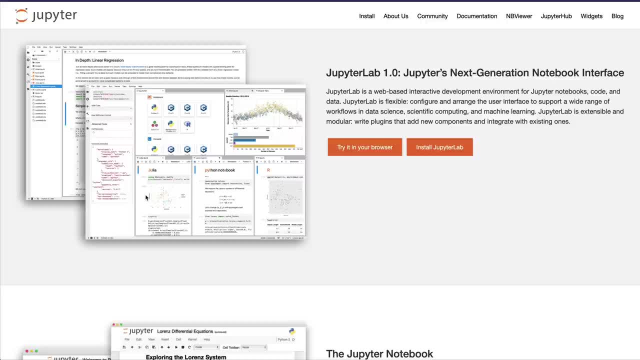 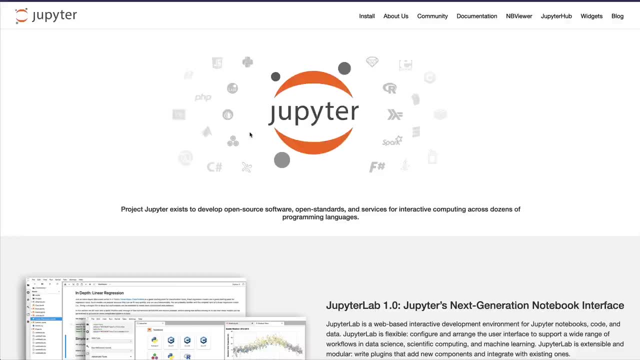 lab is the again the evolution of a Jupyter notebook, And that's what we're using Again. Jupyter is a free and open source project, So anybody can install it, anybody can download it. it's very simple to get it set up in your local computer. In this case, we're using 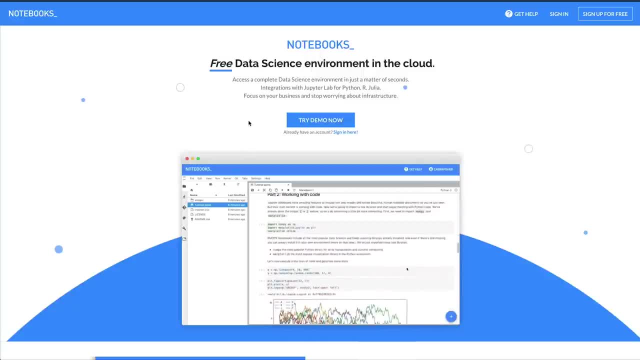 something we call notebooks AI. It's a project that provides Jupyter environments for free in the cloud, So you don't need to install things locally. you don't need to put things in sync in your own hard drive, right? You? that means you don't need to buck it up for. 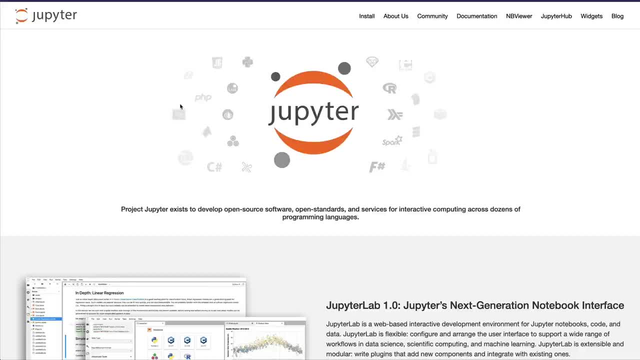 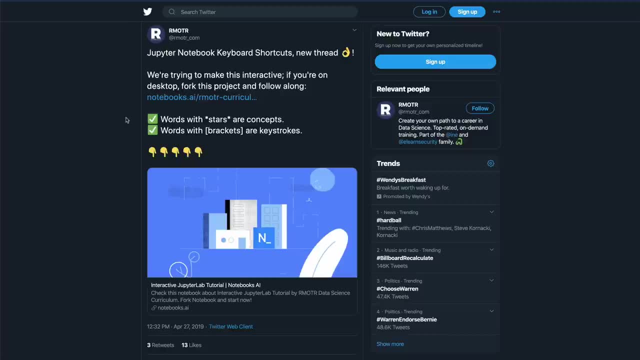 example, because it's just a service And it's all worked in the cloud. So, said that, I want to tell you that we have compiled a very quick list of everything we're going to talk in this part of the tutorial, In this list of tweets- just a thread with 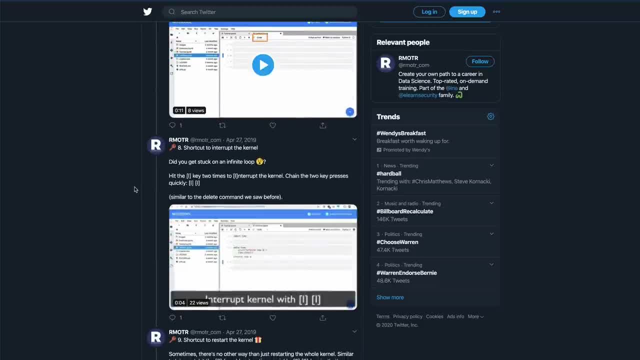 multiple, multiple hints of how to use Jupyter notebooks. So, after the video, after the course, if you forget some of these concepts, you can always go back to this, to it. it's a quick reference for you to have. So let's get started. 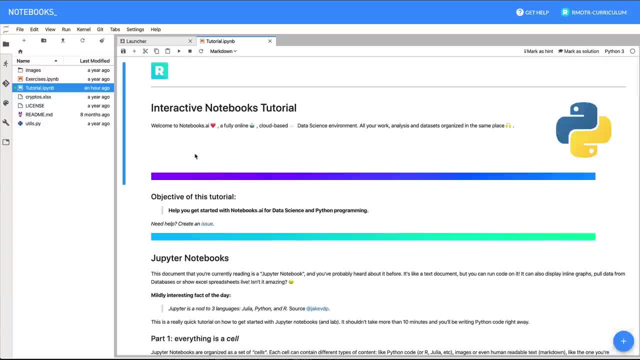 Why do we use a Jupyter notebook? because it's an interactive, real time environment to produce our or to explore our data and to do our data analysis. It's a tool. you're going to fire commands and it will immediately respond with something back. It's a very interactive. 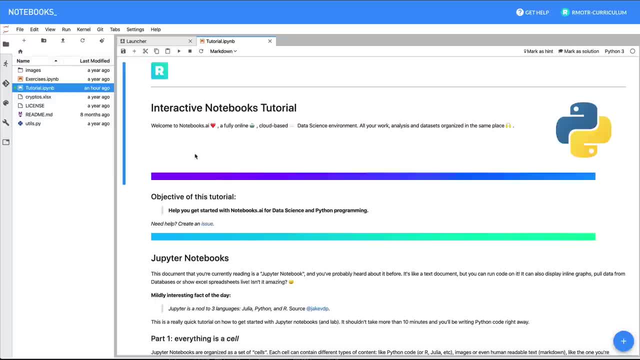 tool When we're working with data analysis, and this is mainly the main difference with some other tools like, for example, Excel, Tableau, etc. is that we are not constantly looking at the data. there is no visual reference like 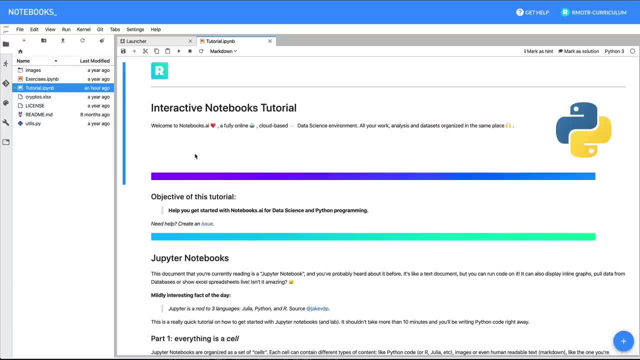 for example, you have in Excel, right? So in Excel you're constantly looking at the data. you have it in front of you. there are 100,000 cells and you can scroll and see them. The problem is that that's not scalable, right? It's like nobody can work with 100,000. 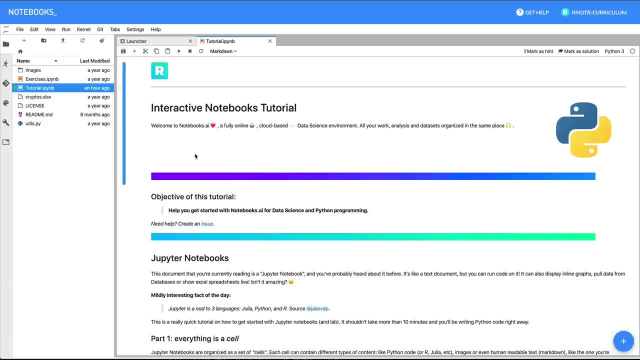 rows in their, in their, in their mind. we will always forget something. So the way we're going to work with Python in data analysis is by always having a reference of how our data looks like, But always at the back of our head. we're not constantly looking at. 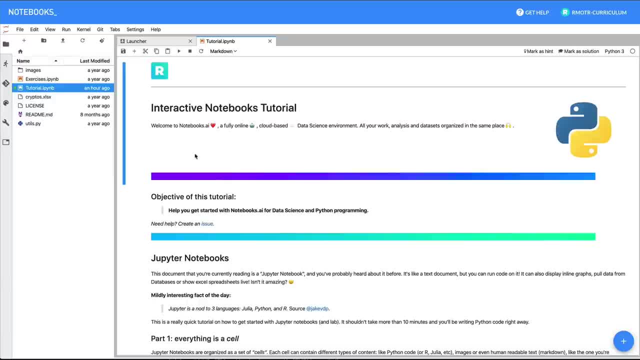 it. we're like this person from the matrix, you know the, the, the commander of the matrix that commands people to get, get in and out. We're basically telling people up, telling people that, basically asking data right Asking questions, right Asking questions. 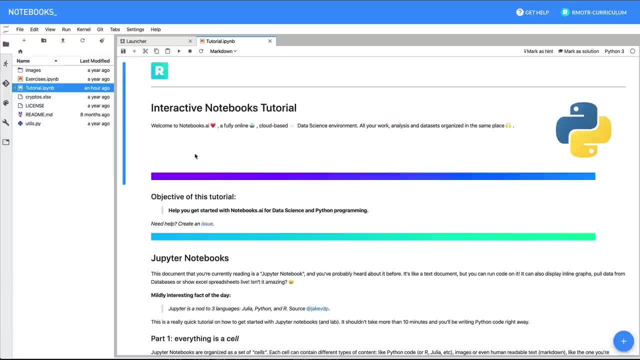 questions to the data and having a picture in our mind of how that's going to work. We're not constantly looking at it, we're just having a reference in our in the back of our heads, of what our data looks like. So that's why this tool is very useful. This tool is useful. 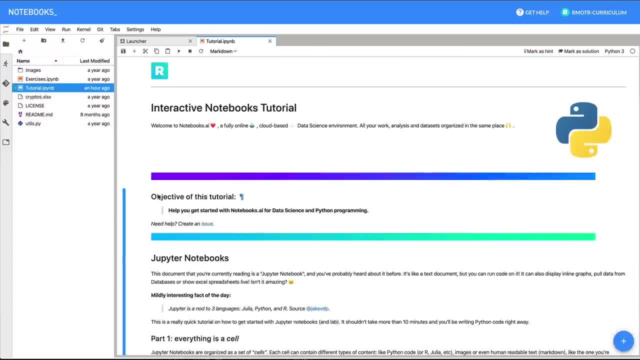 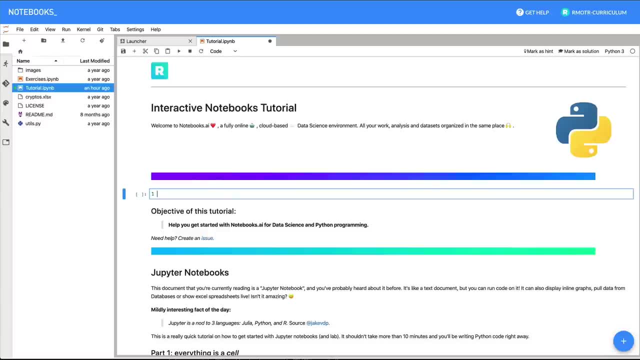 also, if you're just training your Python skills and or their programming languages skills, because what you're going to see is that it's just a regular Python interpreter. In this case, I can execute some code. let's do one times, actually one. 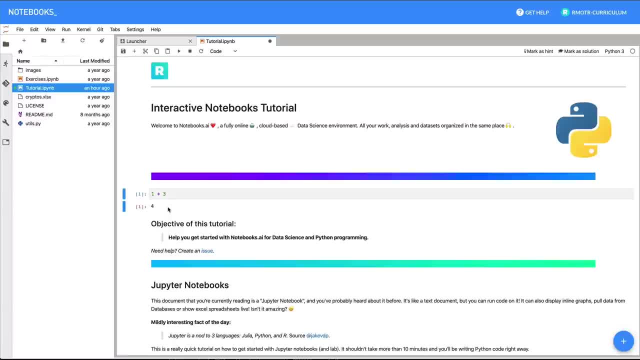 Plus three. there we go And the result is four. right, So this is a Python, is a fully featured Python interpreter. The good thing is that, again, it's gonna respond to us pretty much immediately. I create a command and I immediately get a response. I can do something. 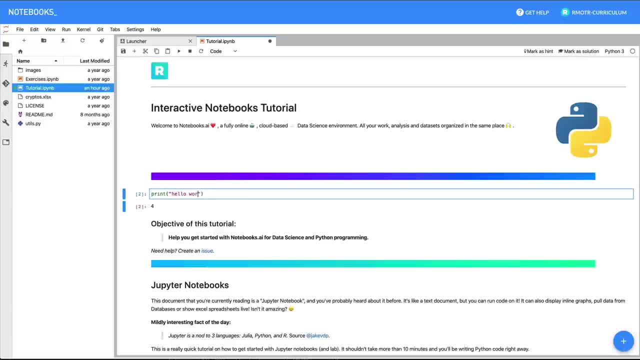 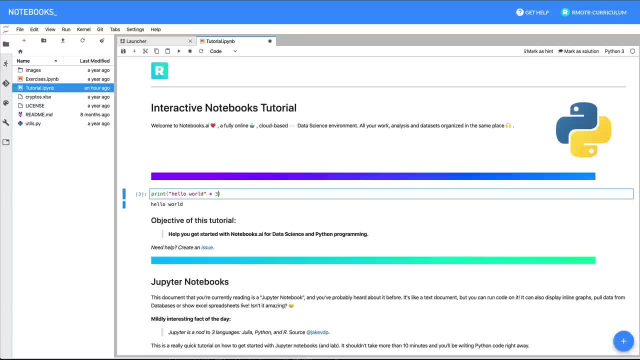 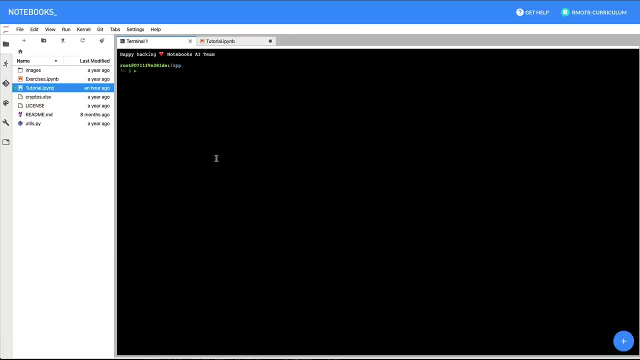 a print here, hello world, I immediately get a response. I can do Hello world times times three. Again, it's a Python interpreter, a fully feature Python interpreter, but it's not being accessed from a terminal which you can write. this is the good thing about Jupyter lab: to have a terminal. 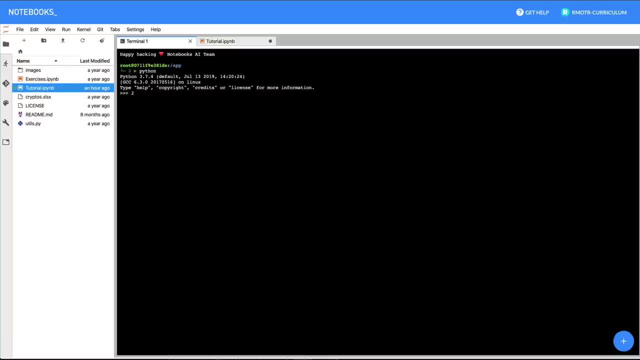 I can do Python right and I can do two times three and I get an answer back. But this is not convenient. to work with our data we need something a little bit more interactive. we can also mix with documents. that's going to be the advantage of a Jupyter Notebook. 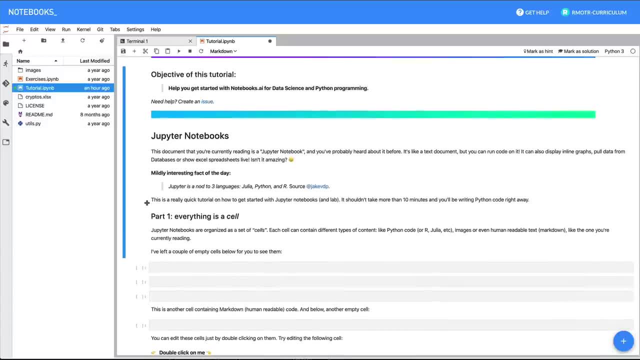 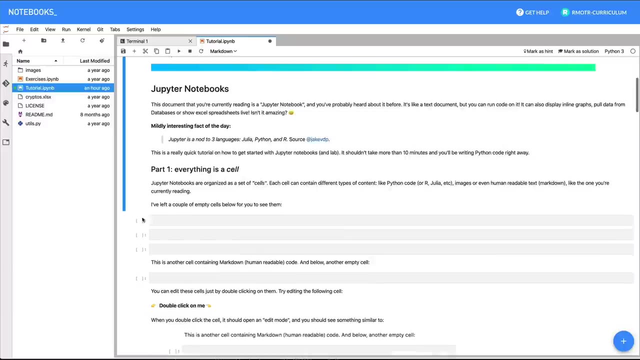 So what? what's the way we work with Jupyter Notebooks? there are a few concepts, very important concepts, that we are going to follow. A Jupyter Notebook is just a sequence of multiple cells. okay, everything is a cell And, as you can see when I click on these cells, 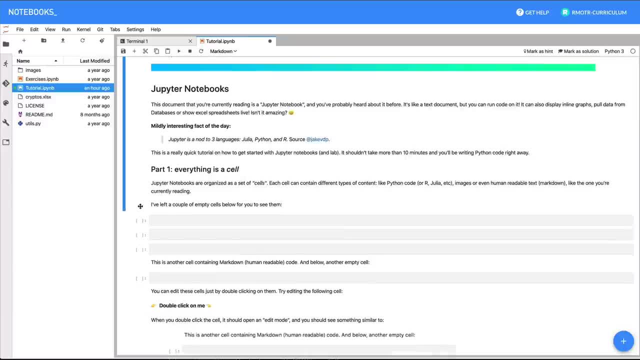 even if, even if it doesn't look like being a cell, it is. you will see that this blue thing right here right is pretty much following me. because I'm clicking on the cell right and I'm selecting that particular cell, everything happens within a cell if I want to execute. 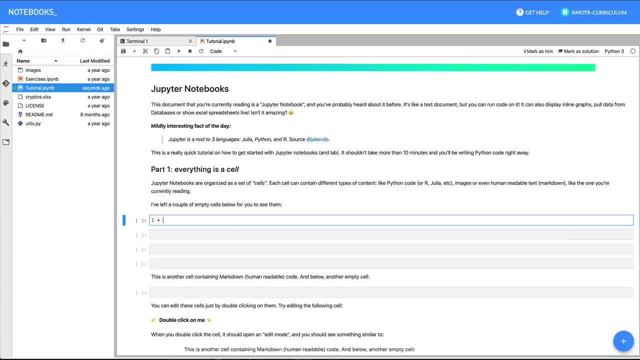 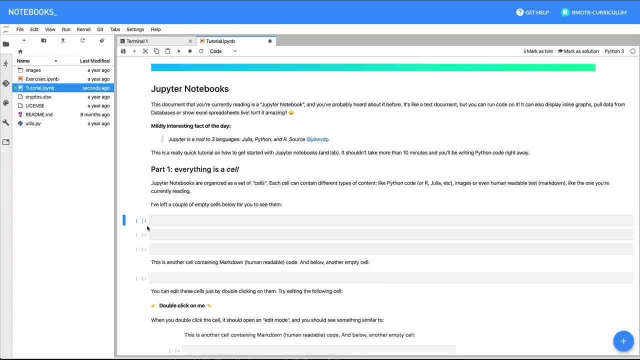 some code. I can do again one plus five and I get a result or a result back. right, that's, that's how it works. So I'm creating a cell, I'm deleting a cell, I create another cell again. So it's, everything happens with a cell, And I'm going to tell you how to add. 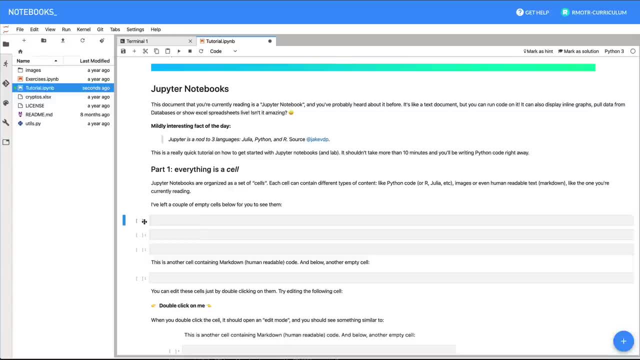 the cells, how to remove them, how to execute code, etc. The interesting thing about a cell is that it can either be Python code or any other programming language. you're using in this case is a Python data analysis course you. it can be Python code, as we're we were doing before, one plus. 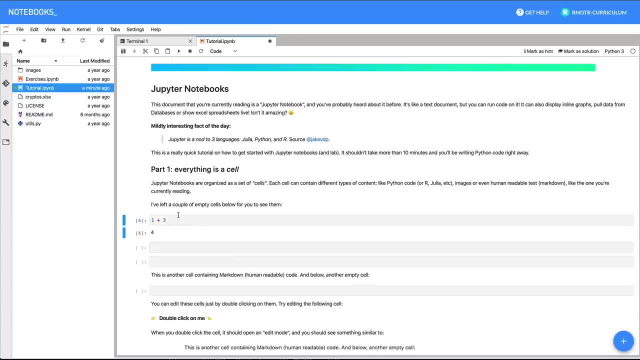 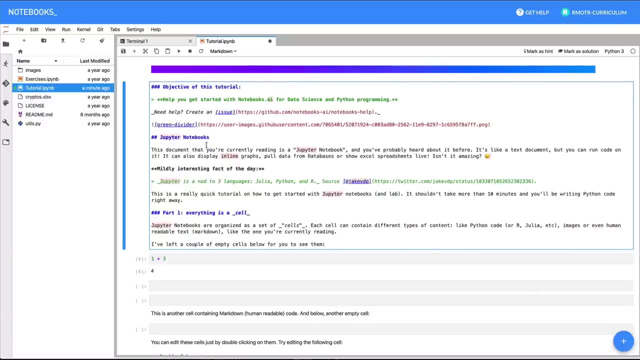 three, this is Python code, or it can be what we call markdown, okay, which is a formatting format right to create text. that will be a render with sort of HTML at the at the output. So in this case, this is what the source code of: 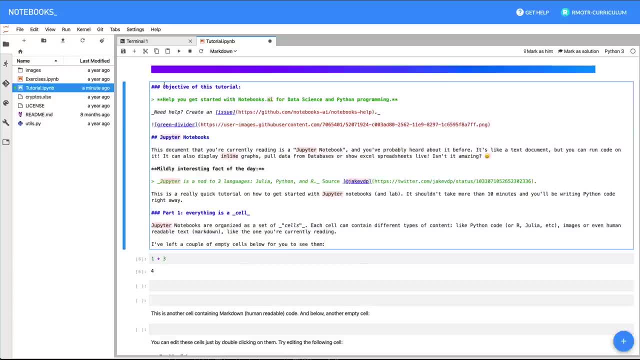 the markdown looks like: in markdown, any line that starts with this parts it's going to be a title. in this case, it's going to be the largest. the biggest title you can have is just one pad, And then you keep adding to reduce the size, in this case, a level three. 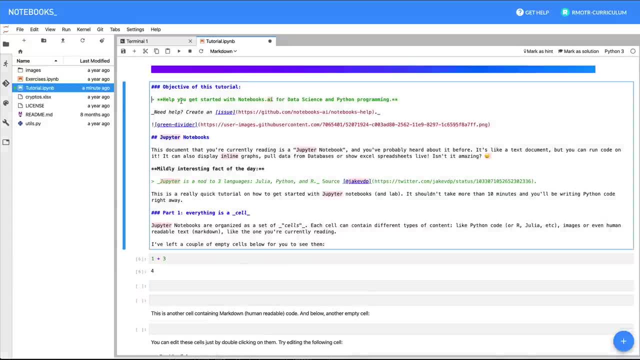 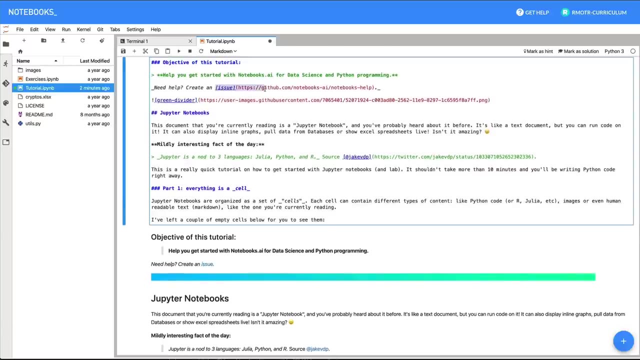 title And then you can have, for example, this is a quote, this is bold, And then you can have: this is italics. this is a link right. So let me- actually I could copy the cell and open the source code. There we go. So this is a link, right issue. issue is created. 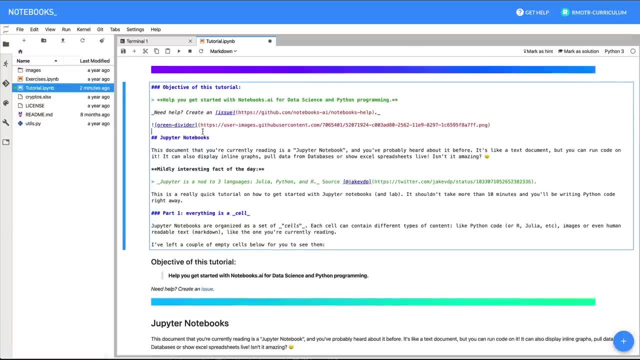 or it's rendered as a link. So markdown what is is a is a text formatting tool, right or protocol. we could say that in this case we just specify us. we have some, some rules to use in our, in our text. 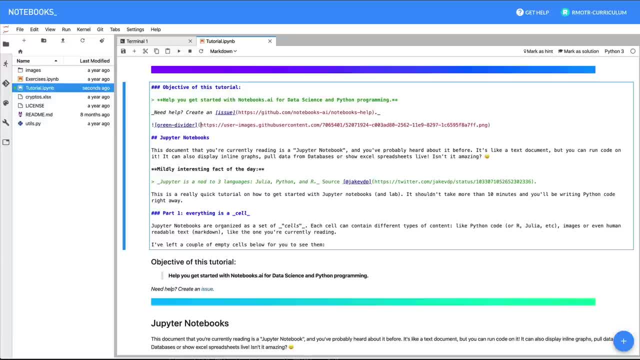 And markdown, knows how to interpret them and format right or return a formatted document after them. So, for example, here we have green divider, which is a picture, And we know it's a picture because it starts with an exclamation marks, And that's that what. 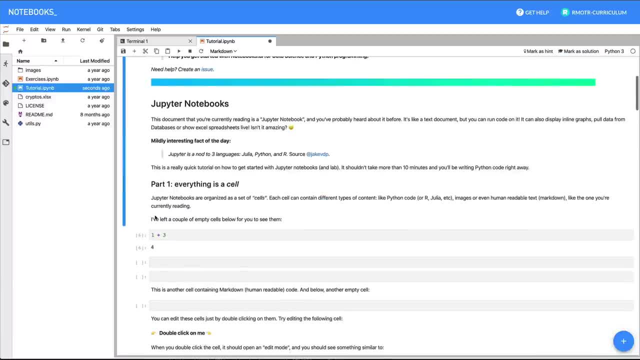 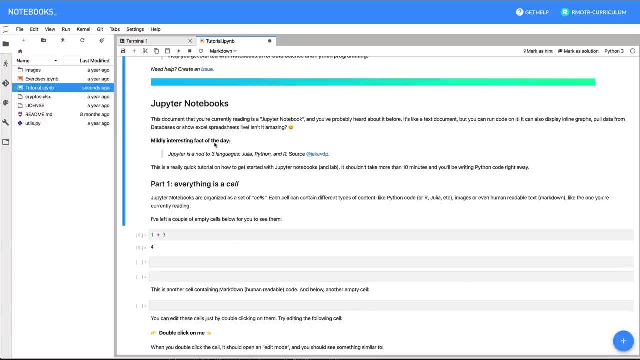 can get any tutorial online. you can get any tutorial online. you can get any tutorial online free. it's fairly simple to get started with And it's also very important because when you're formatting your reports right, when you're creating your reports, you want 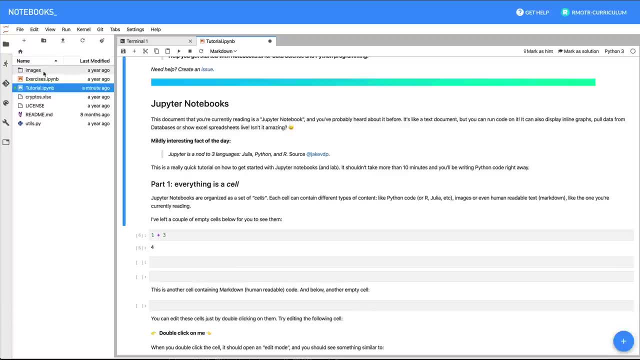 them to look pretty. you can use markdown for not, And what we're going to see later is that you can export these notebooks and they will generate PDFs, Right. so this whole thing can be a PDF or an or an HTML page. So, after you're done with your data analysis, 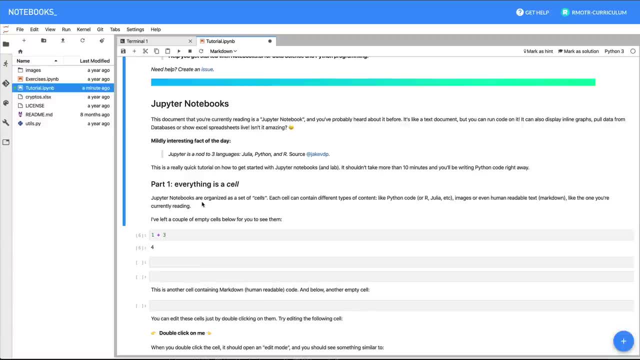 you can hand over to whoever asked for the analysis A PDF report, which is pretty neat. So, moving forward again, any cell is going to be either markdown or it's going to be code right here. So this one is code And you can switch the. 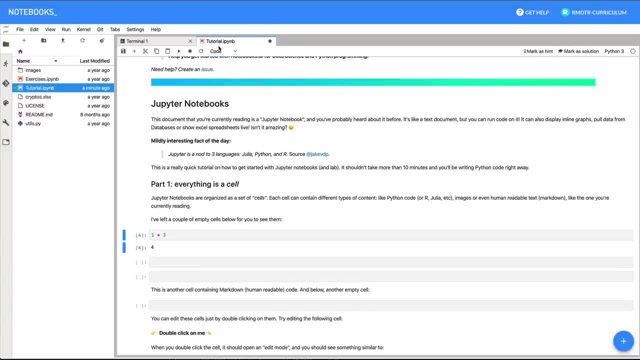 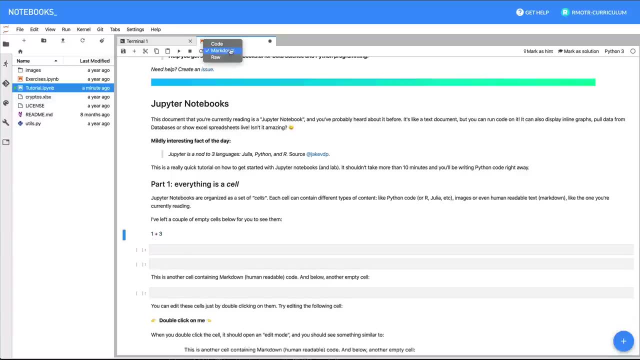 modes. you can say: this cell is code or actually let's make it markdown. So right now, if it's a code, it doesn't, doesn't matter at all, or just it's not executing anything because the cell is interpreted as markdown. So now I'm switched back to code And now it works. 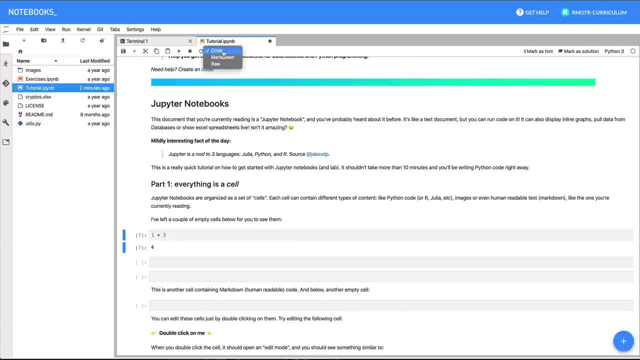 again as it should. It can also be raw, But, to be honest, we don't use raw very often. So again you have this, this general cell type, this cell we're using. what type is it? Is it code? Is it markdown? 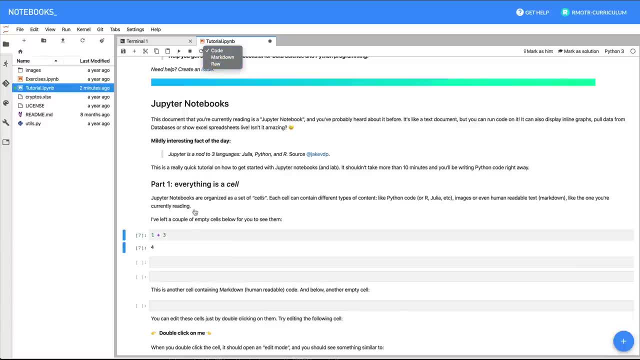 you can switch it with these, with this selector right here. So a few more things that I have to tell you right away so you can start internalizing them, and it's going to take some time to get used to it, But once you get used to it, you're going to move very fast in your data. 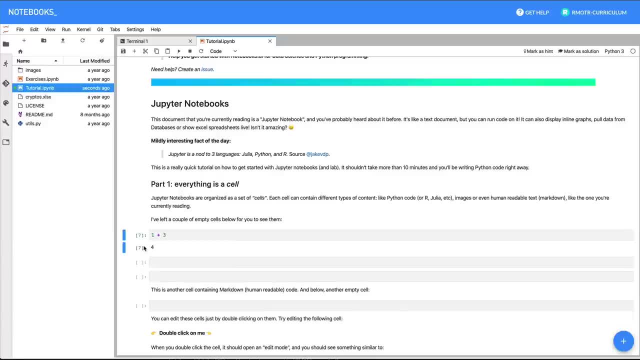 analysis with Python, Jupyter and Python notebooks. The first thing is that, as you're seeing right here, every cell has been given an execution number. So any the cells will be moved. right, they will be moving around. you will be moving them around, But you will always know which one executed before another. 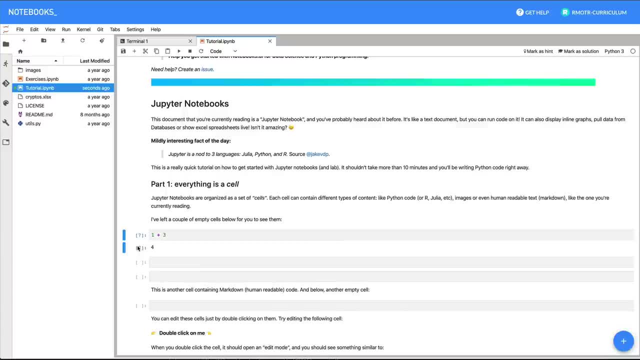 one, And that's because every execution you run will be assigned an execution number. In this case, this is the seventh time I have executed code, But execute code again, for example, I don't know- two times two. this is the eighth time. 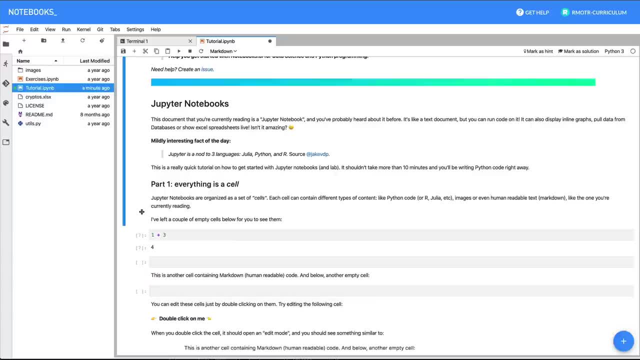 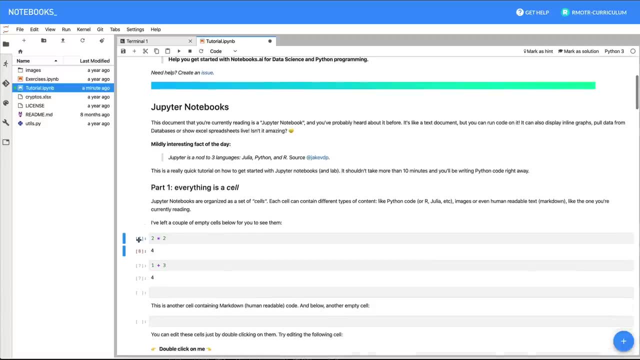 that I've executed code And if I move this thing right here, if you're reading this thing top down, you will not be fooled. right, you will understand this thing. it was moved, the cell was moved, the structure of the notebook changed, But this thing was executed after. 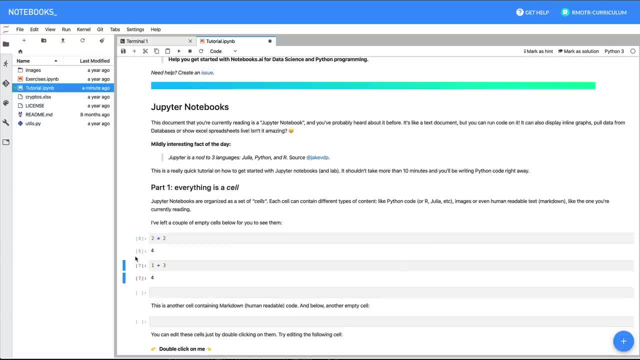 this other cell right. this is eight and this is seven, So the execution- this is eight- order is always preserved. So that's an important thing. Something else: that you're seeing me change the structure and do things with the notebook without using any menu, And that's. 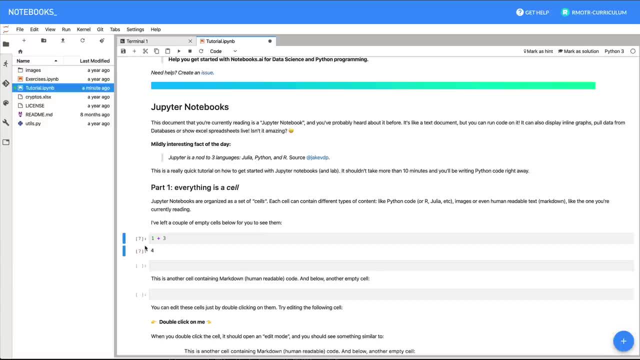 because I know how to use keyboard commands, keyboard shortcuts, to run most of these commands. So, for example, how can I add a new cell? I have this is a markdown cell and there's a code cell Before this one. what's? what's that command that I'm going to issue in order to create? 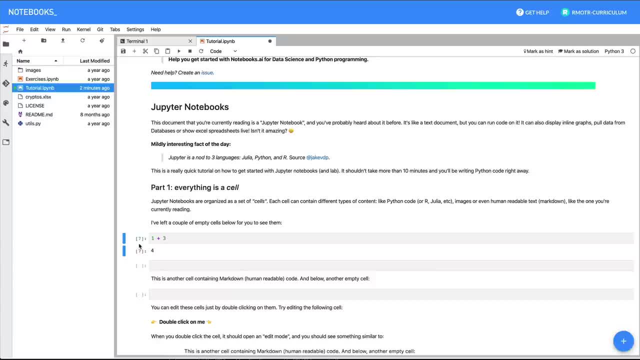 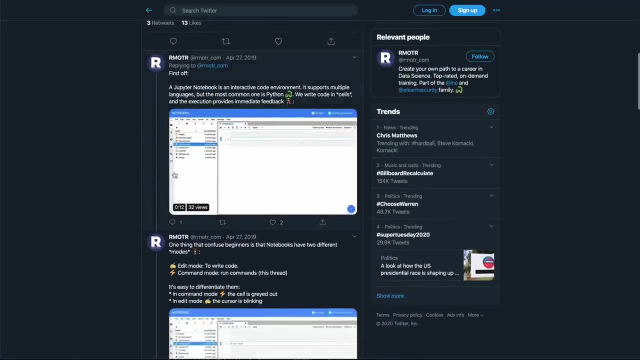 the cell. In this case, the command is going to be the letter A. I just type a under is a new cell creative? how can I delete the cell? it can be two times the D key, two times the D key And again, this is all in this reference with built. So, for example, right. 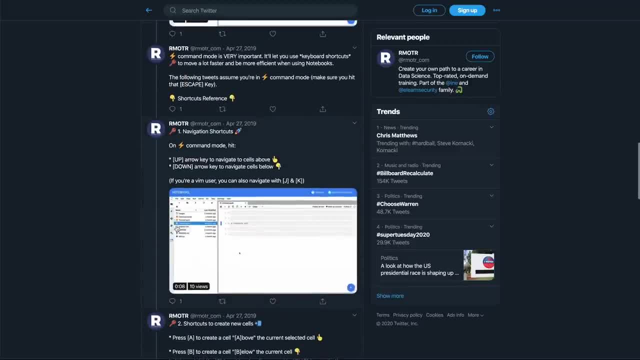 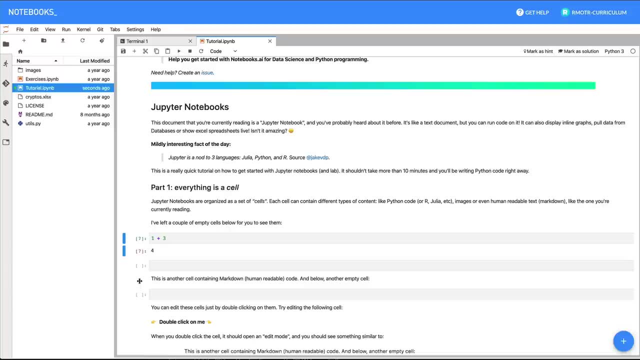 here. where is it At some point? you can Here, you can type, you can press A to create a new cell, you can press B to create a new cell, but we call below. So let me put something here. this is a reference And I'm going to put here the letter B: it's: 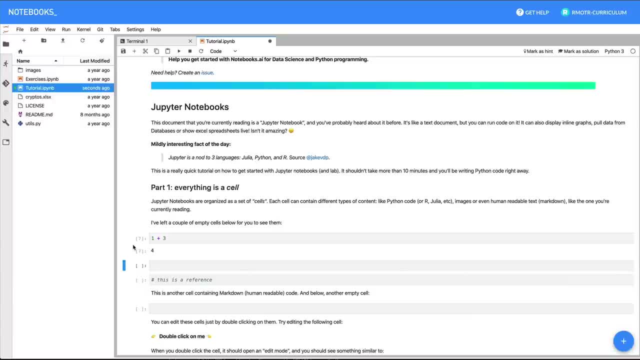 going to create a cell below the currently selected one. So the selection here is here in the blue. I hit- let me delete this one. I hit B and you're gonna. it's going to create a cell below the previously selected one if I hit a. 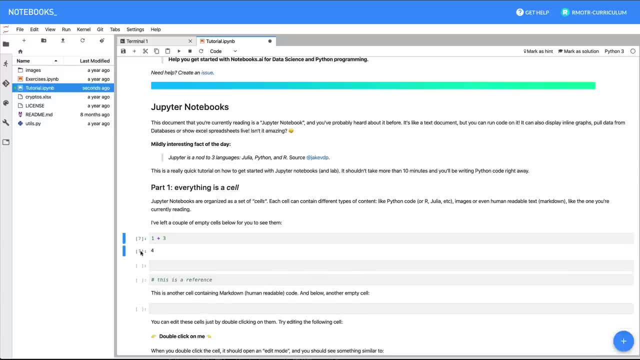 it's gonna create a cell above the previously created one. So these, these are the mnemonic ccs of the creation. something else that it's very important, Why when I'm in this cell and I hit the letter a liter, literally it just. 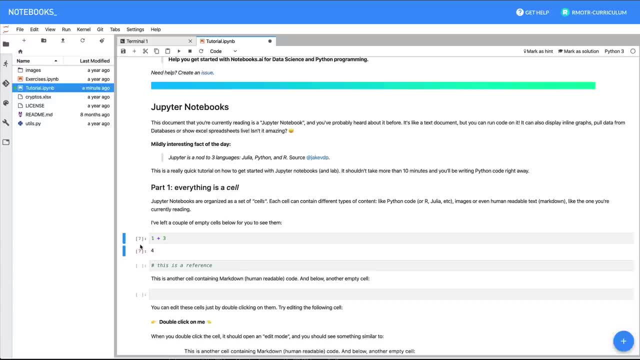 hits the letter A in my keyword- no control, no command, just a. it creates a new cell and it doesn't type a inside the document. right, So right here, if I type a, it's adding at an actual a character in in the cell. Why didn't that happen before? And you're going. 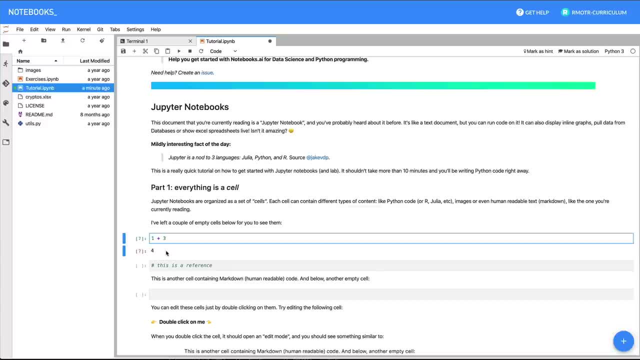 to notice that when I change what I'm going to call the mode in a second, you're going to see that the content of the cell is grayed out. So what now? when I, when I, press on the letter A, it actually creates the cell and it's not adding content to the cell itself. 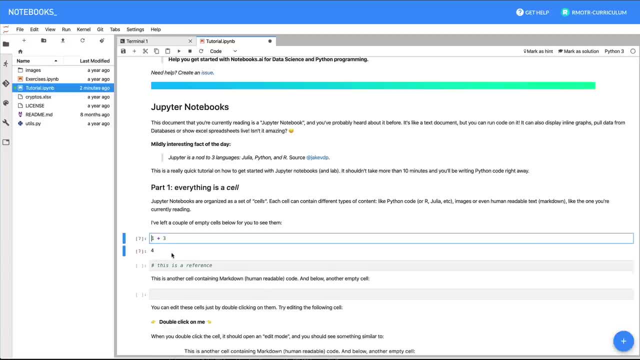 If I go back again to the other mode and I'm going to give you a better explanation. a second: if I take anything in this case, a, it's actually appended to the text within it. So this is my introduction to cell modes And this is very important. The Jupyter Notebook. 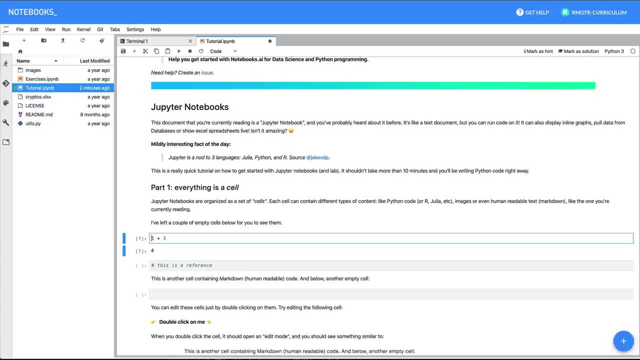 is a mode based editor, right? So there are multiple editors or for example, Vim or V VI. those are mode based editors which basically the behavior of your work will change depending on the mode that it's currently activated. So, for example, in this case I am in edition mode because any character that I type will 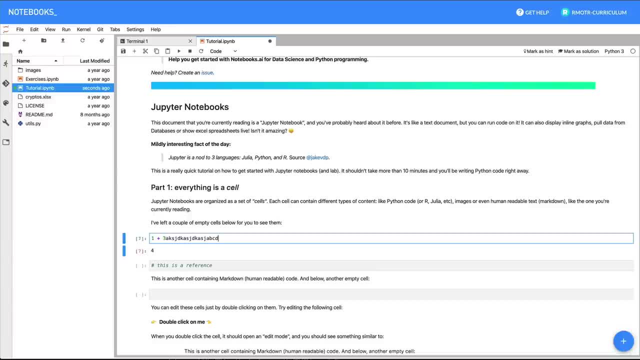 be appended to the cell a, b, c, d, etc. If I switch out of editing mode to what we're going to call command mode, I switch out out of that mode. Now the cell is grayed out And any key that I hit it's gonna do something. 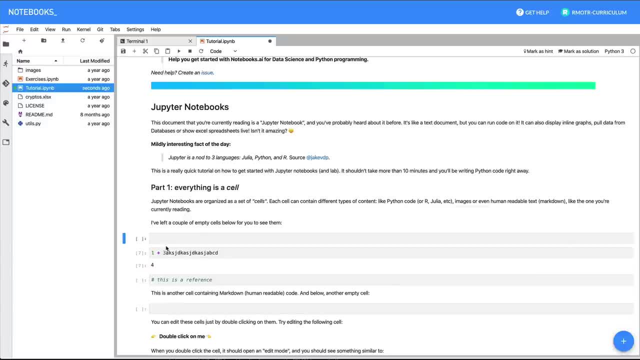 different associated with that key. So A is going to create a new cell above, B is going to create a new cell below. double D is going to delete the cell right. So that's, that's the important part of that's one of the most important parts in order to understand how. 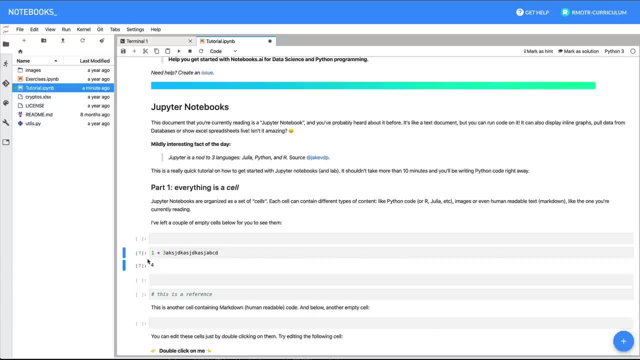 to work with Jupyter notebooks, the mode that you're currently working with- And there are only two modes, So it's fairly simple. This is command mode And we recognize command mode because the cell is grayed out When we get into edit mode. there is a regular. 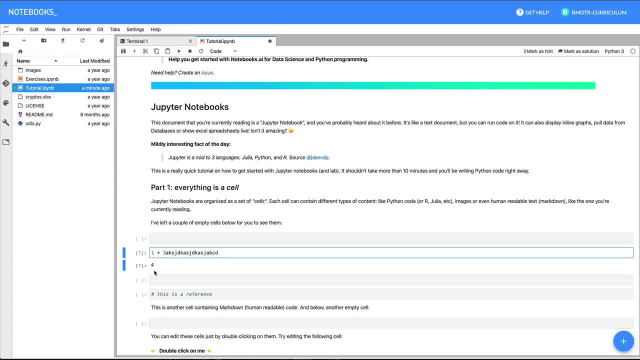 prompt. as you're seeing before, the number one on the cell is actually subject of addition. So that's the way we can realize that. How are you going to? So that's the way we can realize that. How are you going to solve this problem? Well, 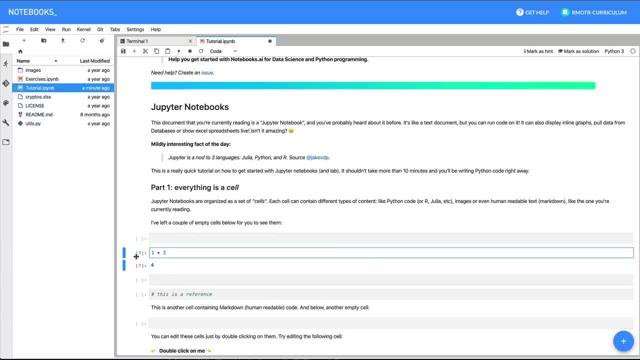 let's switch from modes. In this case I'm in editing mode. if I'm using my mouse just pointing, I can click outside. I'm going to get out of the edit mode into command mode. If I point inside, I'm going back again to the edit mode. But let me tell you something. 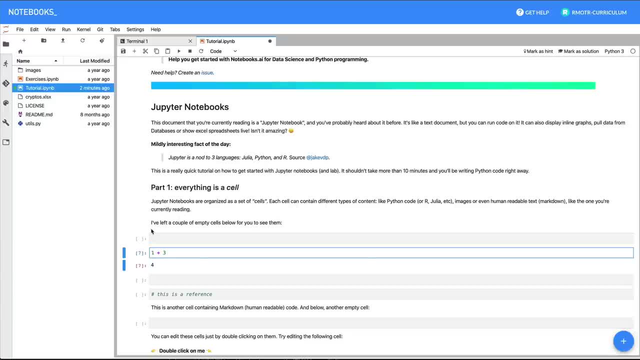 right away And it's like we don't like to use our mouse. we don't like to point and click because that's very slow. We like to use our keyboard. we move very fast, We are keyboard. So how are you going to switch from from editing mode back to command mode? 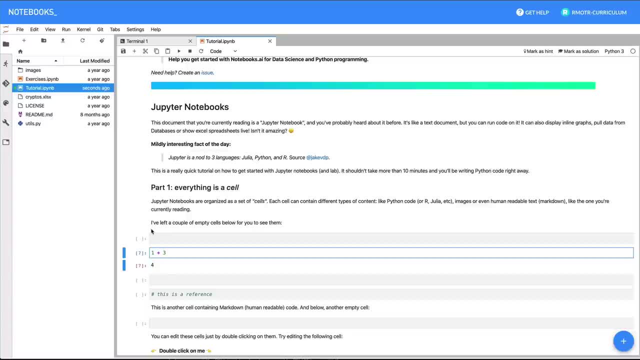 that's going to be with the escape key to go from editing to command. edit escape key is going to switch out of editing back to command mode And if you actually want to make modifications to the cell, basically you want to get into edit mode, you're going. 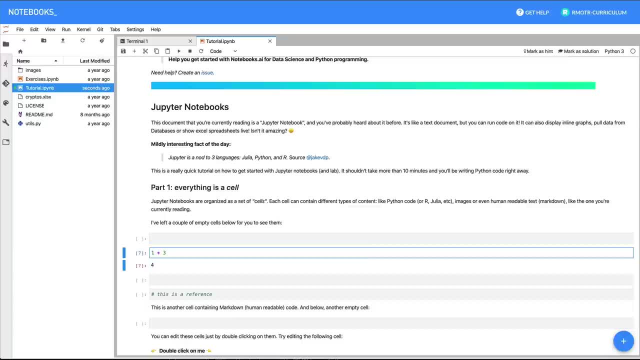 to hit the return key. that's going to get you into edit mode again. So we have tackled multiple things already. Again, we said in Jupyter notebooks we're going to use Python code very quickly to interact with our data. we need a real time. you know I'm asking. 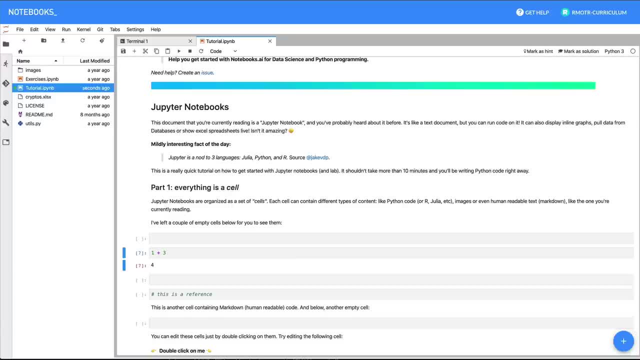 a- you're answering- type of editor. that's what the Jupyter notebook is. The Jupyter notebook has these two modes: edit and and a command mode, And then the cells, which is pretty much everything's the most fun. that's a fundamental part of the notebook. 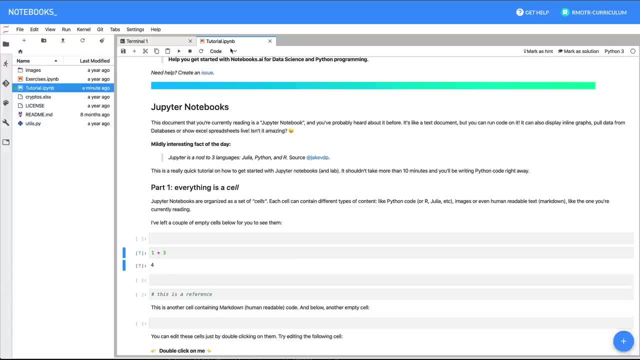 the cell is going to have two types. it's going to be either code or it's going to be marked down right. And now I'm going to start showing you more features And I'm going to show you I'm going. 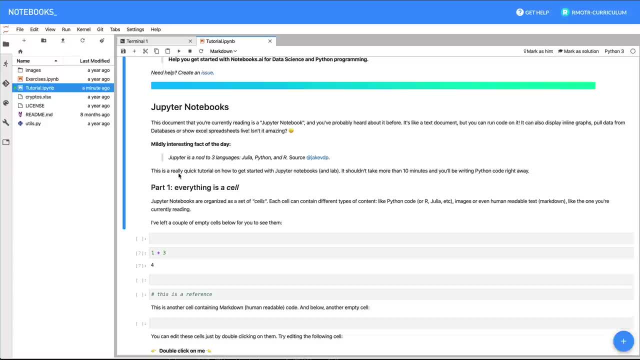 to show you the most important commands And, of course, how the what the keyword shortcuts for those commands are, so you can move freely and and work with Jupyter notebooks in the most efficient way. So let's get started. First of all, for for from the most important. 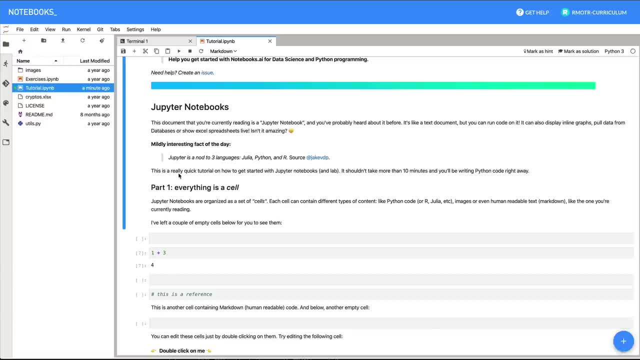 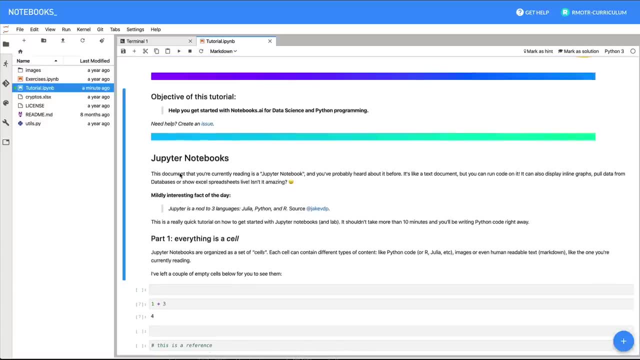 commands is moving right, So navigating. it's very simple to navigate: just use your arrow keys up and down, up and down, and you're going to move around in your notebook. If you want to switch the type right, going from markdown to code, etc. you can switch. 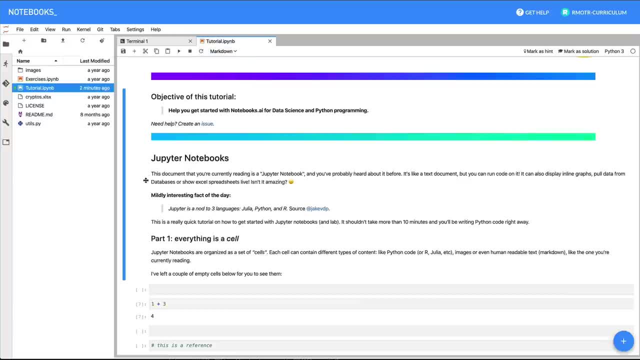 use these drop down or you can press the specific keys to switch to either markdown or Python. So for my markdown you're going to switch. sorry, hit the M key. that's going to make it markdown. For Python, you're going to hit the Y key. you're going to hit the. 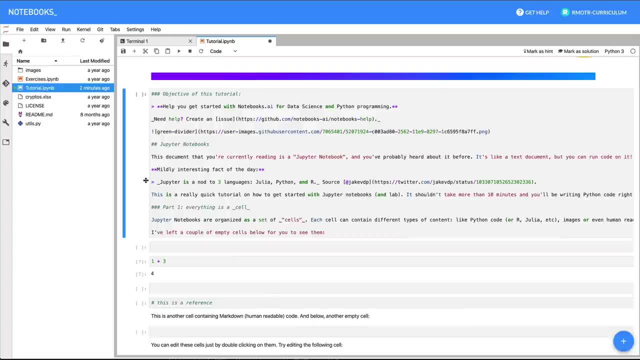 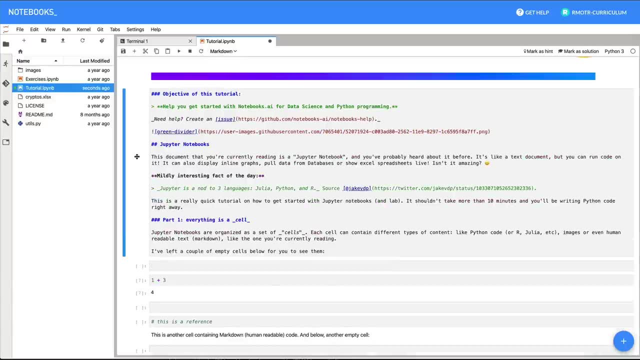 Y key. That's going to make it Python code, So M and Y are going to switch you back and forth. Keep an eye on the selector. I'm going to hit Y, M, Y M. it's going to switch it from. 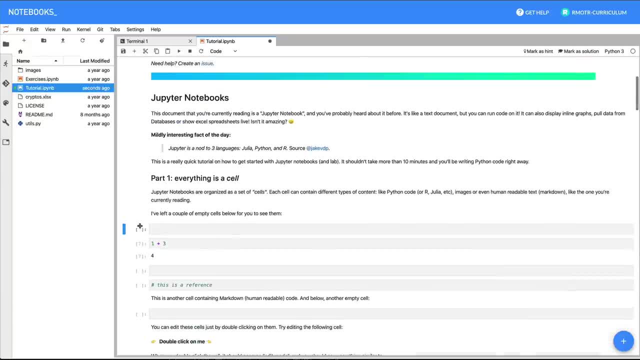 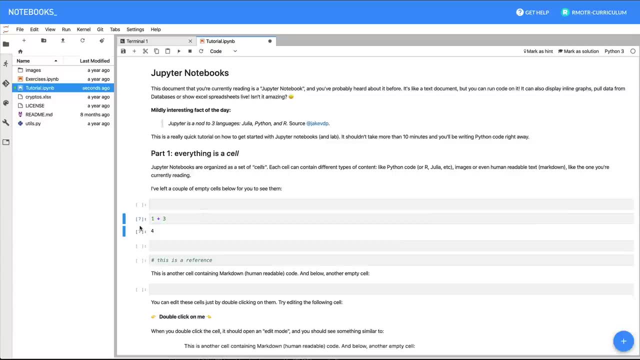 code to markdown What else? How can you execute code once you are within your typing code and you want to execute it? there are two types of executions you can run. The first one is going to keep the selection, the currently selected and active set. 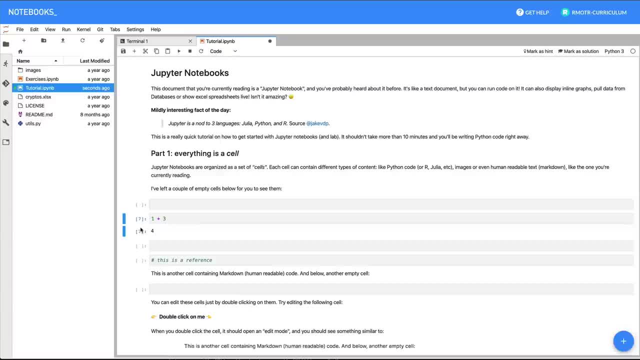 It's going to stay at the same place you are And that's going to be my- by keeping pressed the control key and hitting return. So that's going to run decoder And this, the prompt, or the current selected cell, will remain being the same. So I'm running this thing a couple 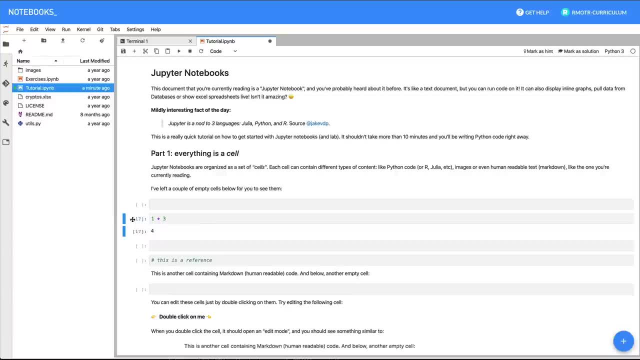 of times already And the selection or the currently highlighted cell stays the same. I can change that by using shift return. So I keep the shift key pressed And I hit return and is going to execute the code, but it will immediately switch the. 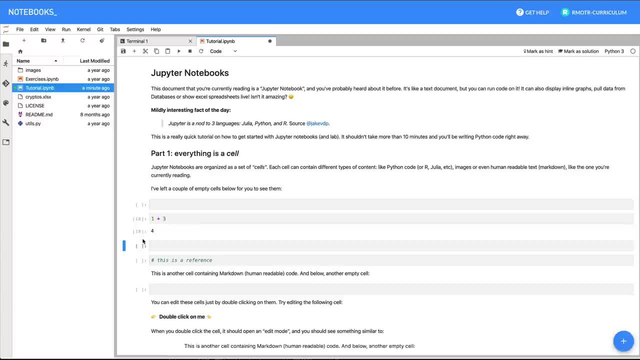 prompt or the currently selected cell to the following one. And that's useful when you have multiple cells. you want to execute one after the other So you can keep hitting shift, return, return, return, return, and it keeps you moving right from top to bottom. Alright, 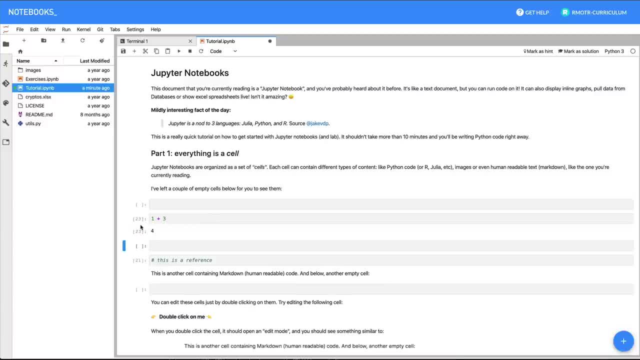 so control return or shift return to change the execution is the same. It's just what's going to happen with the currently selected. So we already saw how to create cells. With the A key, we create a cell above, with the B key, we create a cell. 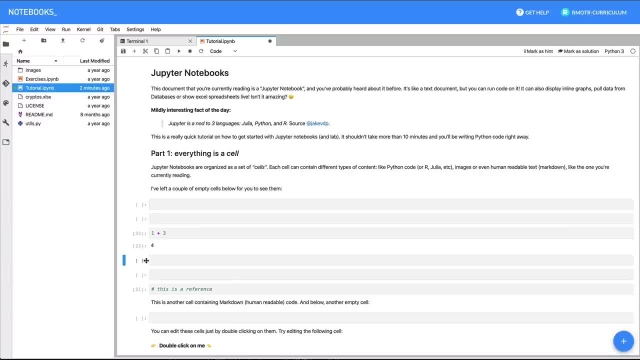 below To delete a cell. you're going to hit the D key, the D key, two times, one after the other, very quickly. DD is going to delete this, the cell. what happens if you made a mistake and you want to undo the previously issued commands? 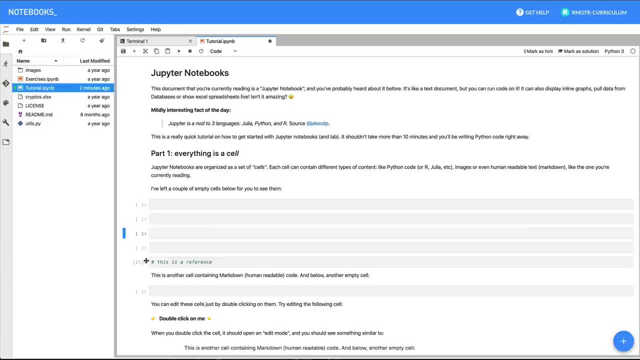 Well, the mnemonic here is going to be Ctrl Z. you know the mnemonic, it's not the command, it's going to be Ctrl Z. you only need to press the Z key. no, you don't need control, just Z And it's gonna undo whatever you did in your previous command. Alright, so A B. 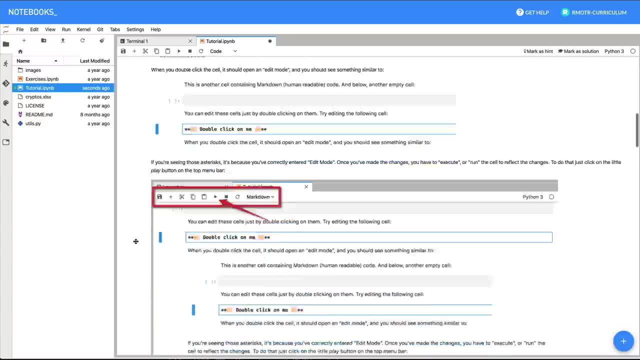 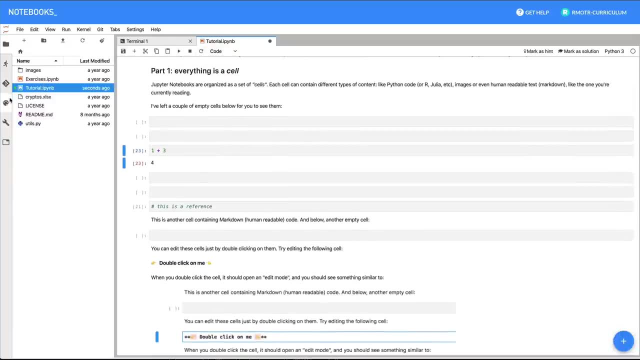 D- deletion, and then Z to undo The all the commands we're saying. they all have a correspondence in this toolbar or in this command Palette. So, for example, right here I could run this code by pressing these play button. right here you see it, the execution is changing. There are multiple ones and you can search. 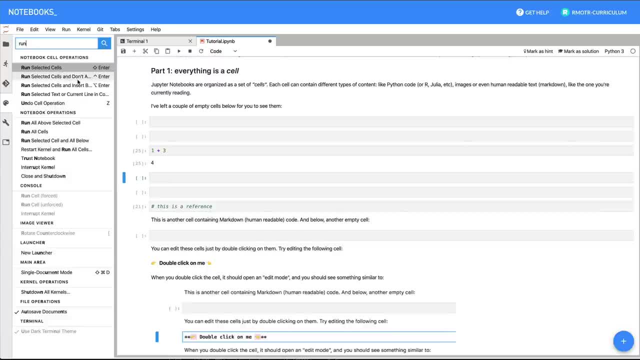 them if you don't remember right here- And the neat thing about it is that you actually have the shortcuts to to issue the same command. So let's say you don't remember how execute and stay, stay in the same cell or move whatever. 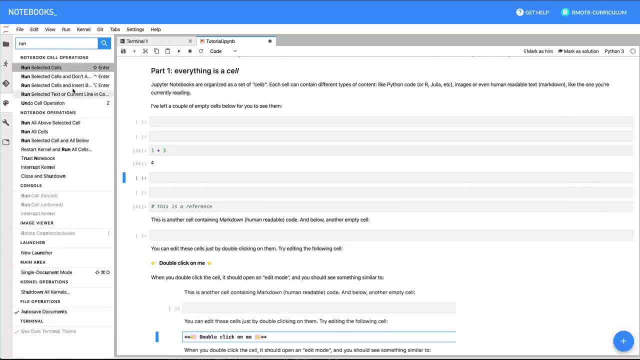 So you can search for run And you can see what's the name and what's the actual command that you have right there, right, So you can, at least for your first- I don't know- month working with Jupyter notebooks, you will usually need to go back to these commands. 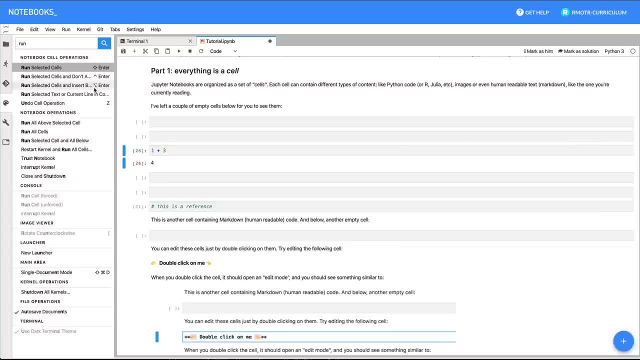 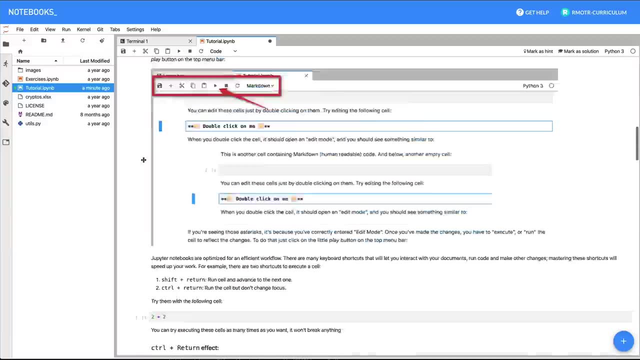 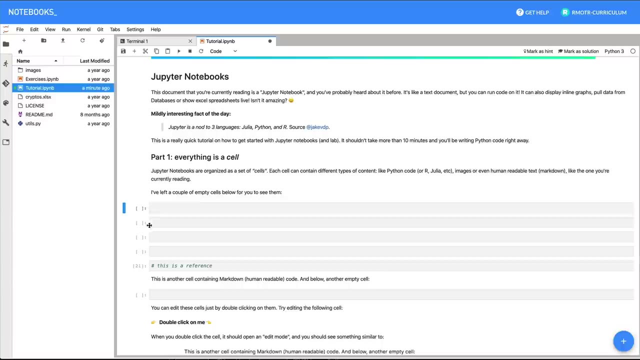 and try to remember the, the quick shortcuts, And with time and practice those will just come naturally. So, moving forward, what else? we have a few other commands. In this case we have Something to cut and paste the cell somewhere else. cost cut and paste, that's going to be. 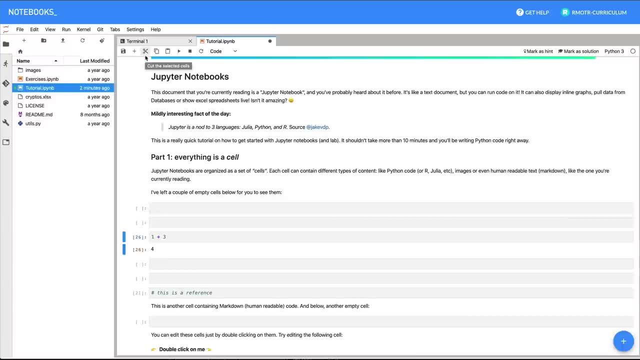 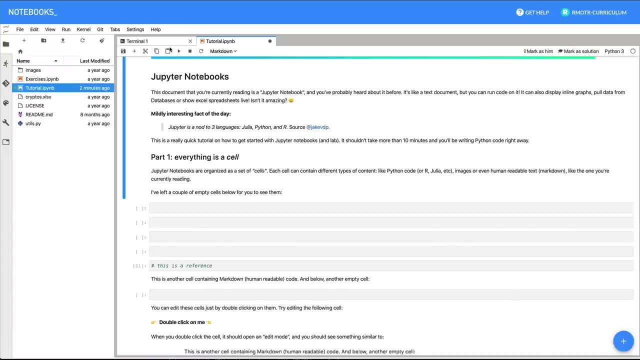 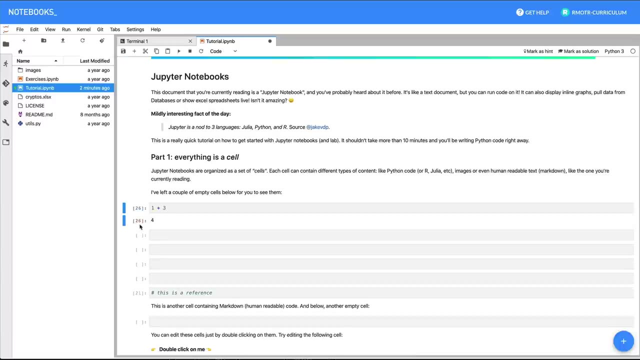 x to cut it. Or you can also use the scissors here- x to cut it And to paste it. you can use this button- or actually this button, sorry- Or you can just press the V key. V is going to paste it wherever you are currently standing at, So I'm going to cut it, I'm going to remove. 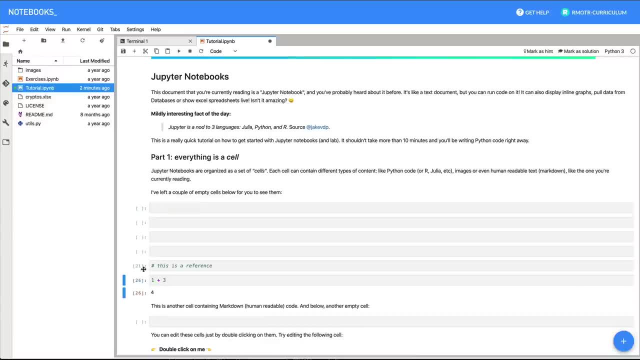 it from here And I'm going to paste it below there, Or you can also copy it. So, instead of cutting it, you can press the C key is going to cut, sorry, copy. And then you can actually say where you want to paste it. In this case, 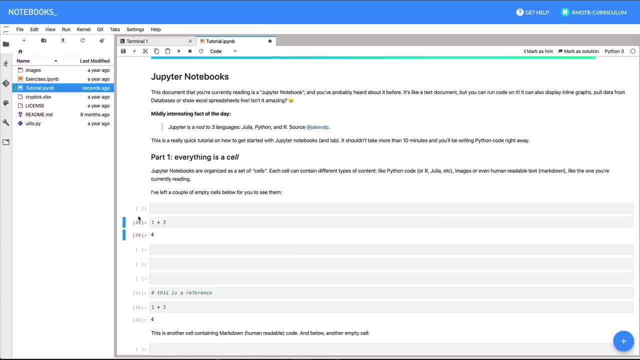 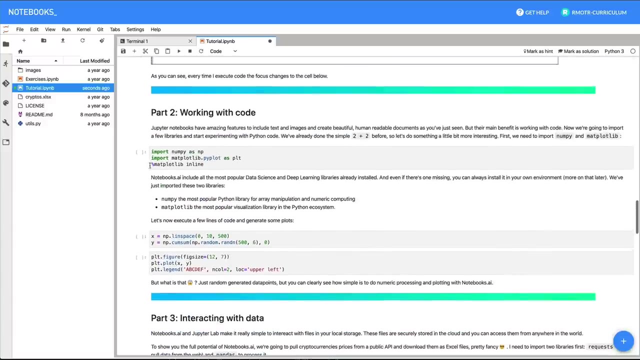 we have duplicated the same cell and look something interesting here: the execution count remains the same. So again, there is, like this, unique identifier for your executions, which means that you know when and where something was executed Moving forward. we're going to use some code here. 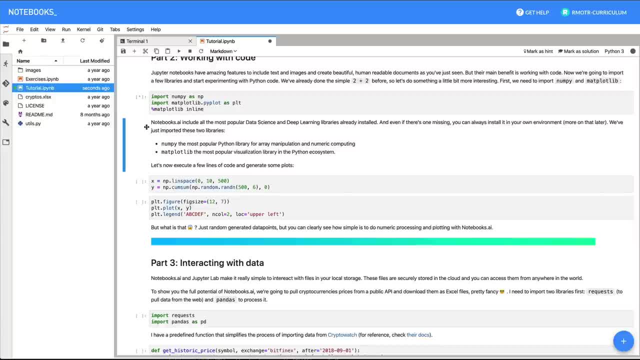 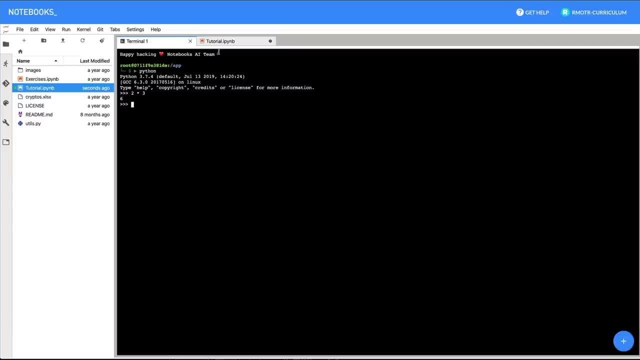 Here we're going to import some tools. you can see some characteristics or advantages of Jupyter notebooks and why we use it so often compared to, for example, the regular Python terminal. One very important thing is visualizations. we, as data analysts, we're 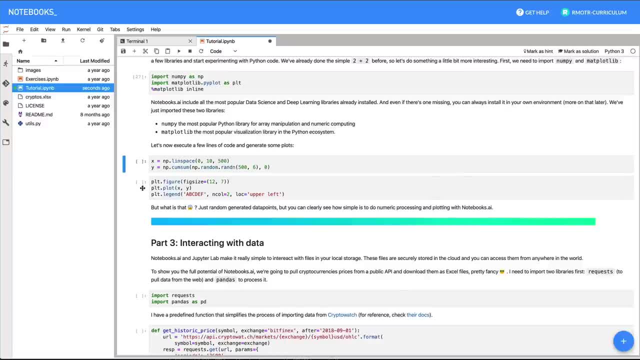 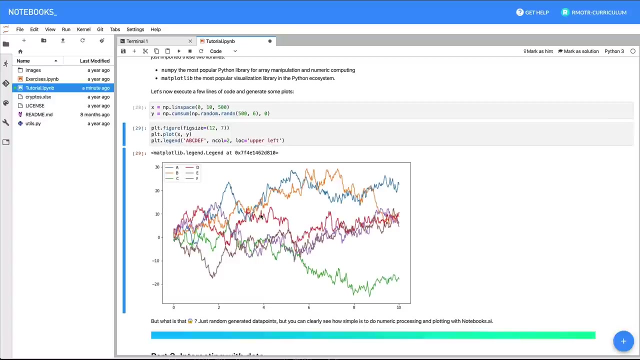 constantly getting data and expressing it through images or animated animations, right, but most commonly images. the main library we use in Python is matplotlib, And matplotlib is a first class citizen in Jupyter notebooks, which means that you can just run the figures from matplotlib And they will just show up directly. 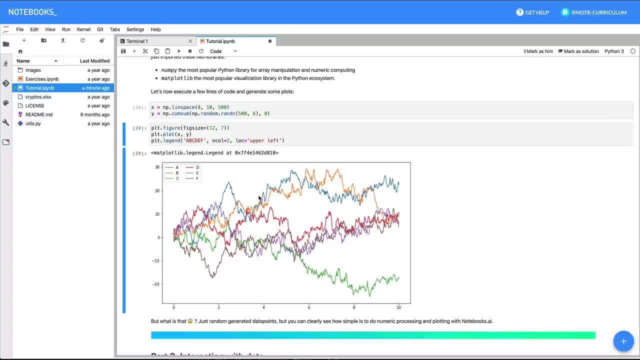 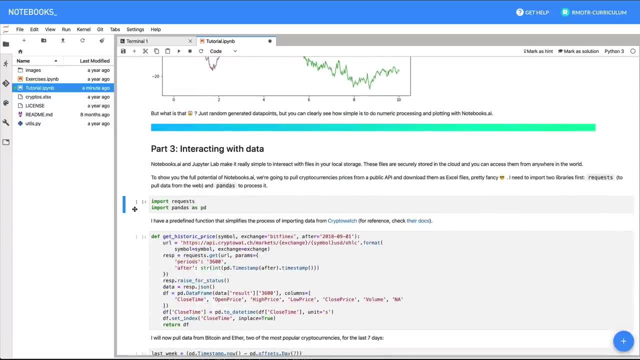 in your notebook without the need of doing anything crazy. So can you imagine showing these, these beautiful picture, in this terminal? That's, that's very hard, of course. So again, that's one of the main advantages of a Jupyter notebook Moving forward we're going to use 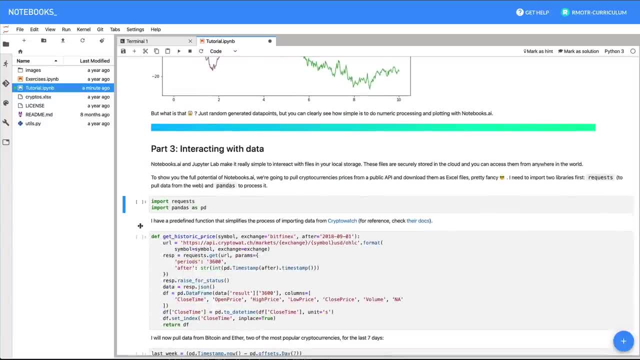 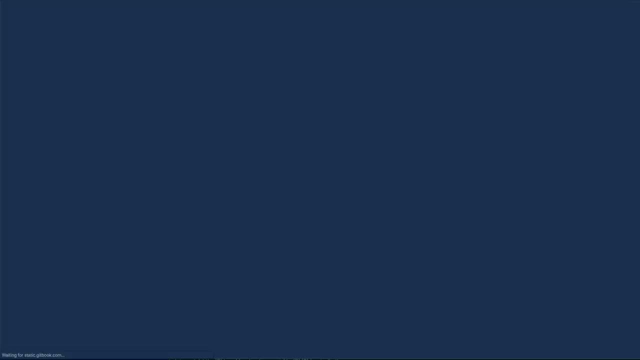 a public API. So what we're going to do is we're going to first, we're going to get some data from a public API. So there is this crypto watch service, which basically has crypto information, Bitcoin, ether, etc. And you can check the docs. we can actually open them. 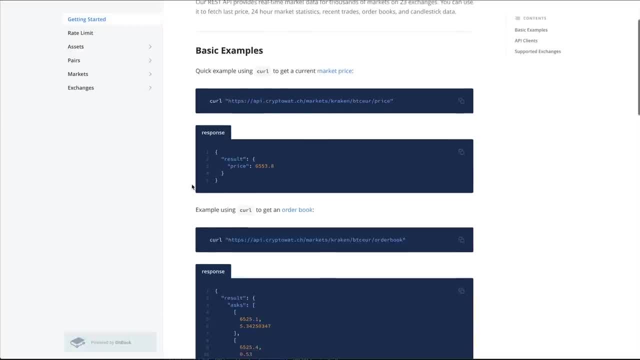 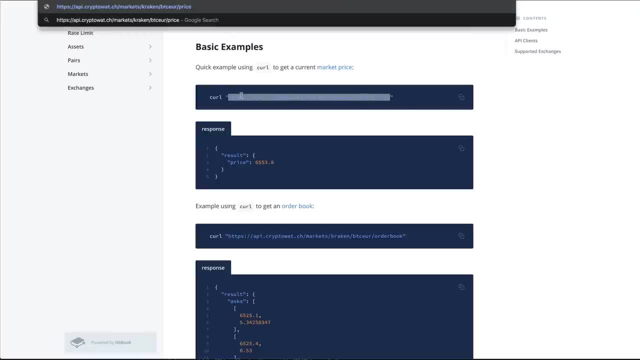 It's going to give you market data, etc. You can check the docs and how you can get- in this case it's BDC Bitcoin to Euro. it's actually. let's see if we can change it to USD, USD, USD. 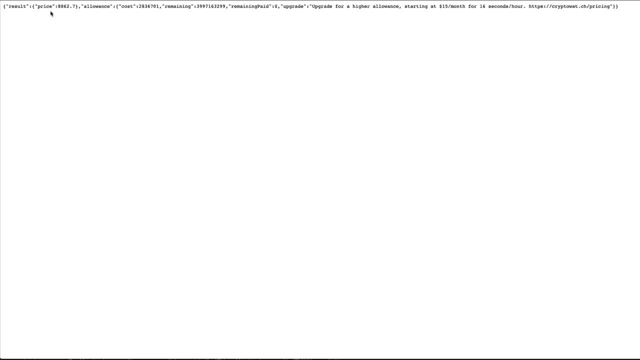 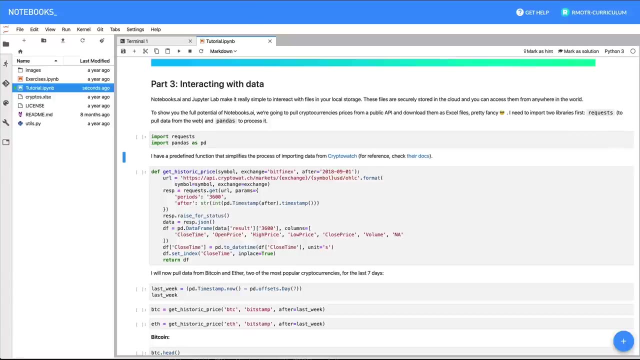 USD price. there you go. So this is the current price of Bitcoin, results, the price, etc. And we're actually going to do markets. do we have crack and BDC used? And let's do. let's actually issue the same query we're going to use, which is open, high, low, close, OHLC. 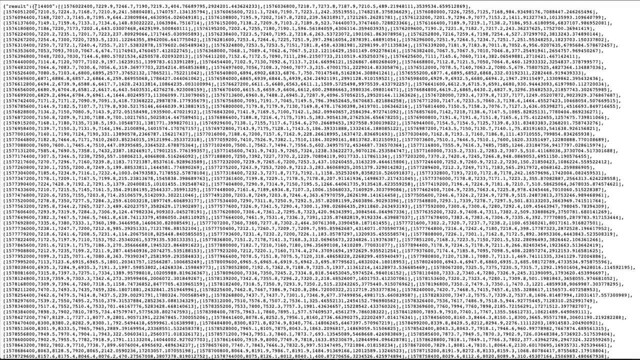 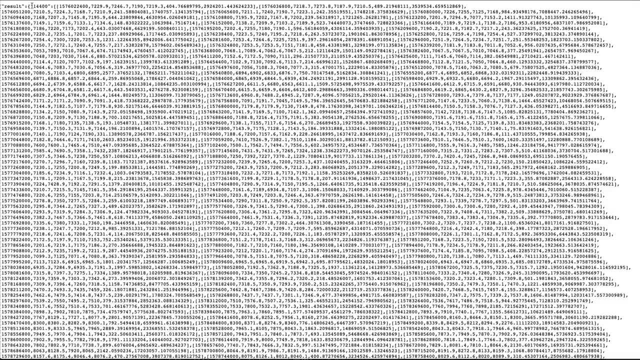 And, don't worry, this looks ugly, But this is actually what we're using. is a list of results right? All different candles, we call them. we get the idea of the open price, close price, high price and low price. So we're going to issue those, we're going to issue these requests. 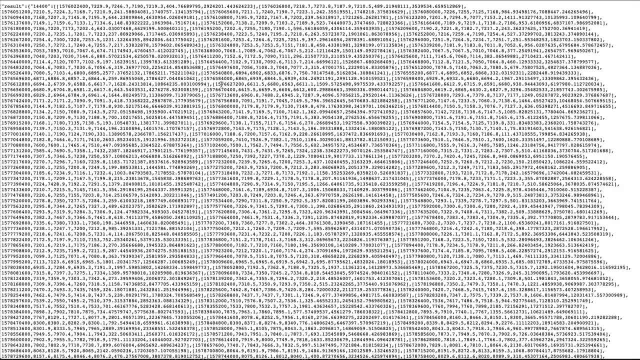 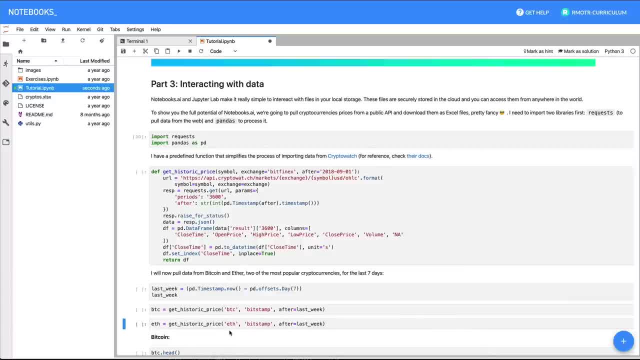 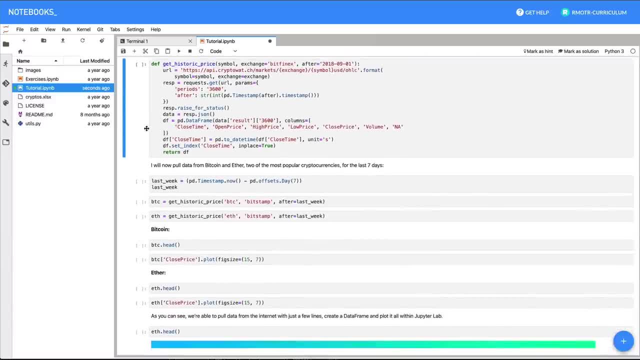 to the internet, to these API- the crypto, the crypto watch API- So you can get information about Bitcoin to do some analysis. I say Bitcoin, you can actually get it from ether for for ether for all other different types of crypto or currencies. So the function we're defining. 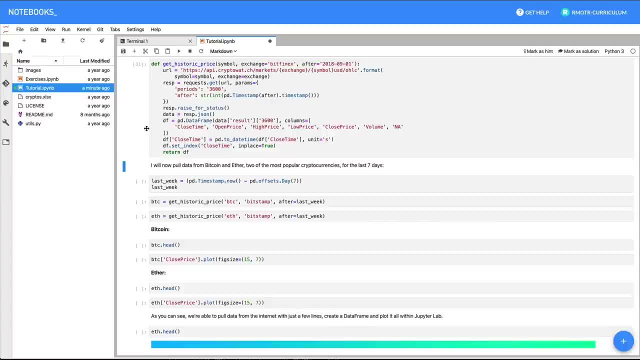 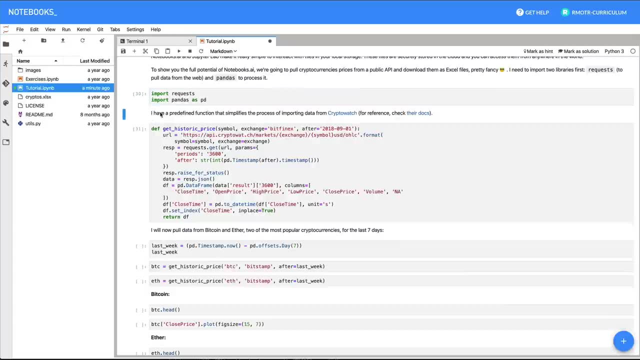 is: get history, get historic price. It's a very simple function that uses pandas, one of the most important tools we're going to be using this course, and the requests library, which is also very famous library for Python, And what we're going to do here is we're going 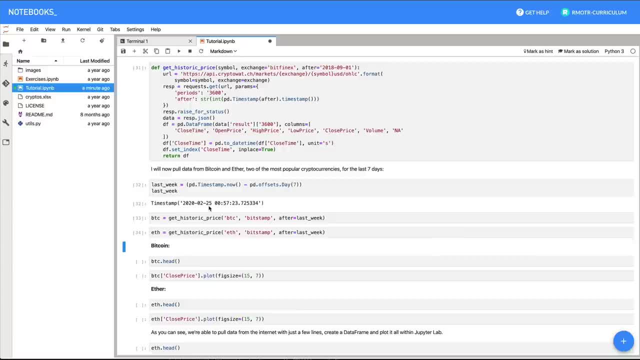 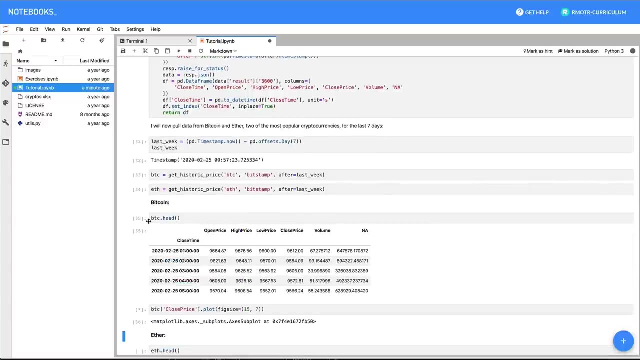 to get Bitcoin on ether price for an entire week, right? So, from a Faraday that the second February- sorry, February 25, up to today, right? So, depending on when I'm shooting this video and we're going to get a quick reference of the prices, open, high, low, close. So in 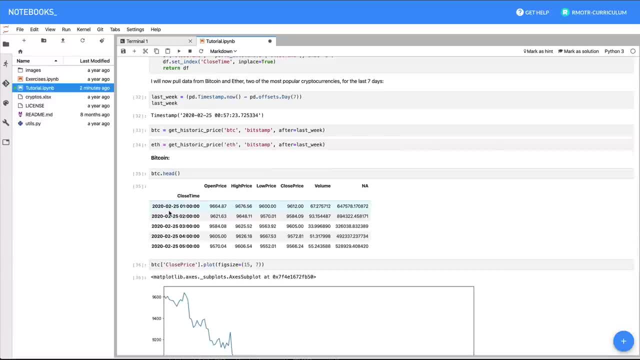 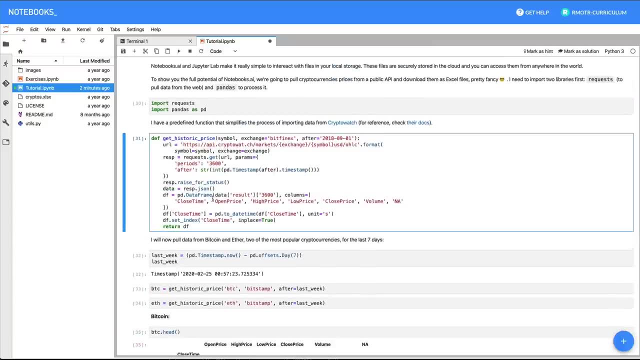 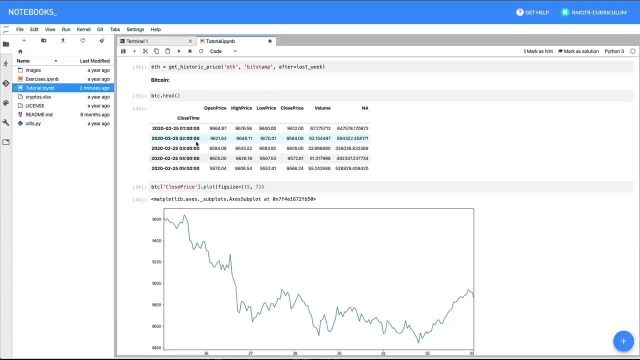 this case we have for information per hour. okay, so this is something you can actually change in the, in the, in the request you're making to the API, you can reduce the candle size. In this case we're keeping it per hour, So we have, by the hour, information about Bitcoin. 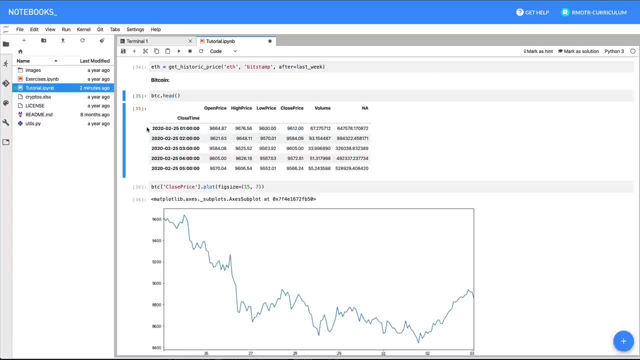 in this particular market, which is bitstamp. Here we have this day, this day- and these are right when I am in the morning- open, close, highest price and lowest price and also the volume that was operated within this time period. 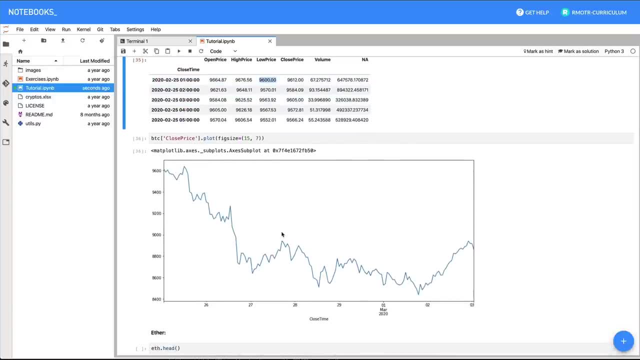 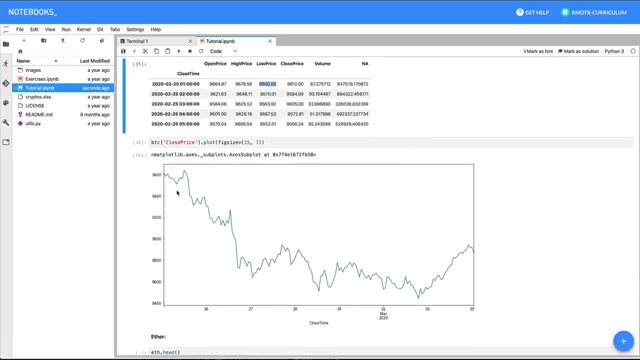 And we're going to immediately plot the price. So we see that in this time, which I think is an entire day, we the price dropped. it's actually a few days, like an entire week. the price dropped from $9,600, below right 9000. So it was a pretty significant drop. 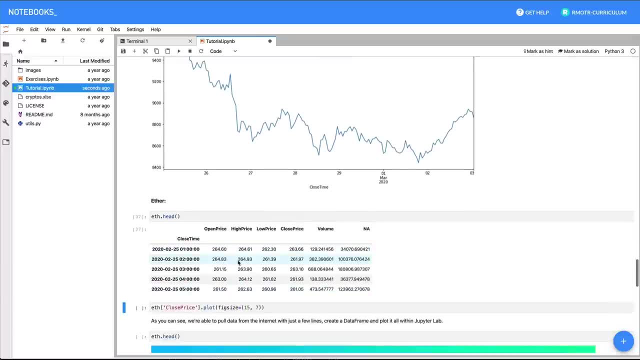 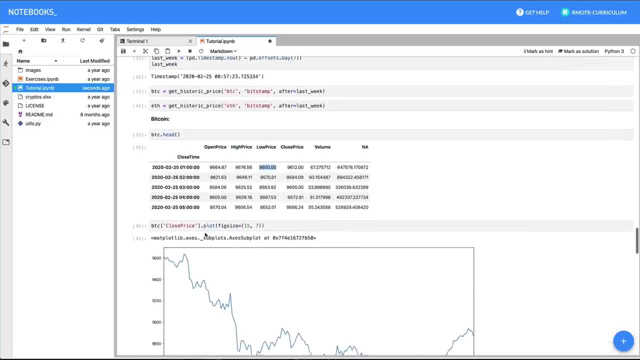 Let's see ether, how it performed- We have here all the records- and how it moved. So this is what I told you: that when you're doing data analysis with a programming tool like Python or R, you're not constantly looking at the data. So what I'm showing you right? 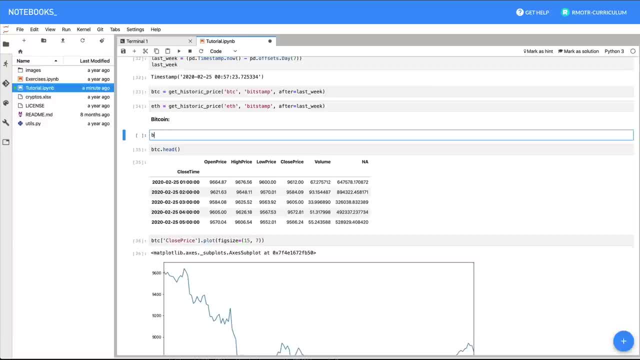 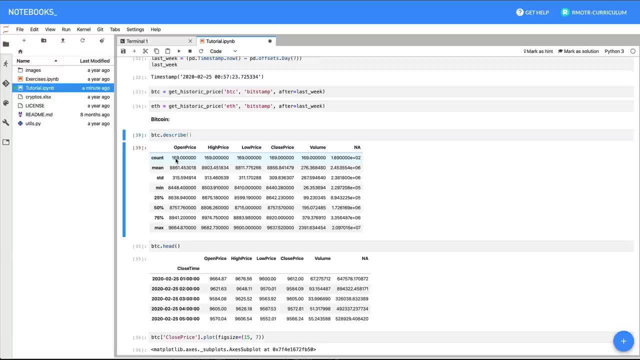 here are the first five records we actually have. Let's do that. We actually have 169 records. okay, 169 records And this per hour. So if we do 169 hours divided by 24 hours, we have seven days, right? So 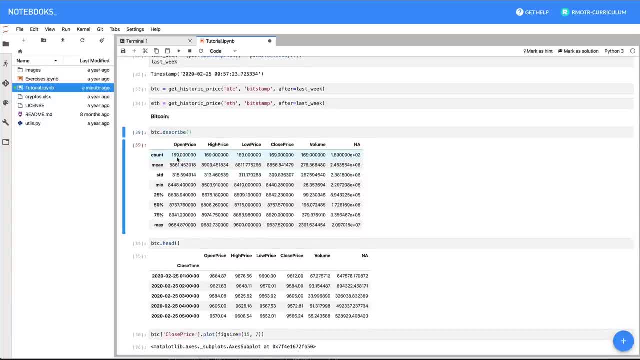 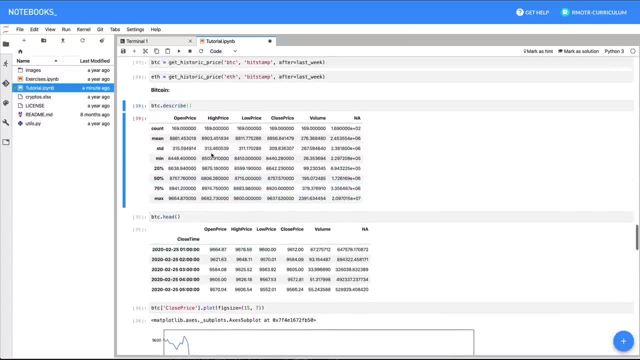 we have seven days of data, 169 records, And then we have a little bit more information here, statistical, I'm gonna get to that in a second- But basically this is what I tell you: 169 records, to be honest, something you could be seeing in a spreadsheet, but I want. 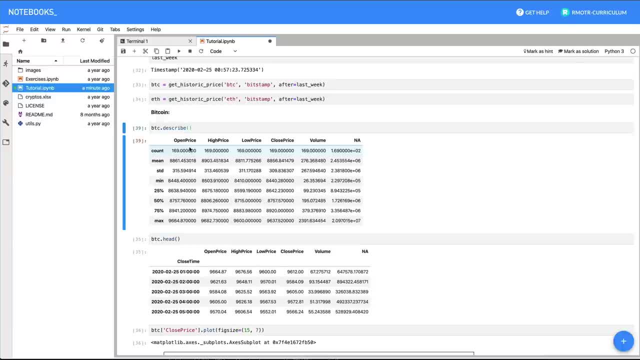 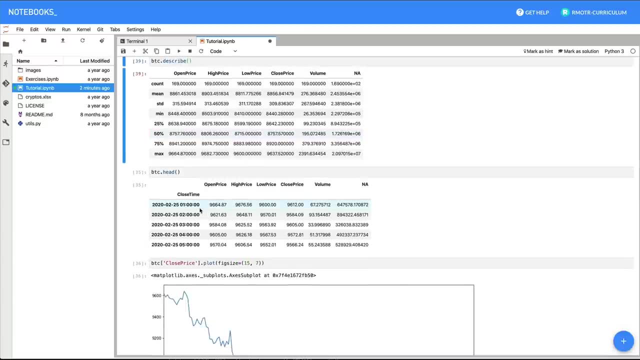 you to get the concept here. We're not just looking at our data, we have it in our brain, we know what it is, we know what shape it has, we know how many records it had. we know information standard deviation. what's the mean of that right So close price was the 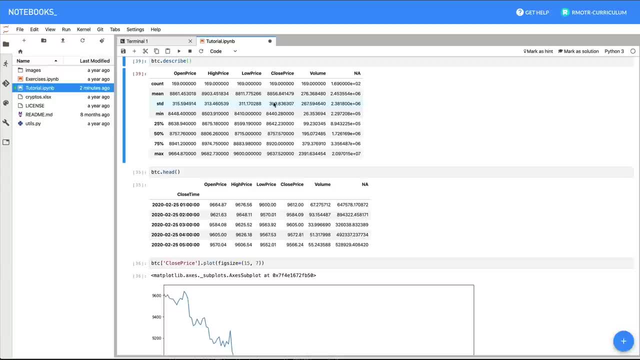 standard deviation Right. What's the, the average, the mean, the median right? So we have information about our data. it's sitting behind, you know, in our brain, but we're not looking at it. And that's because the very simple example with only 169 records, but in real life we're. 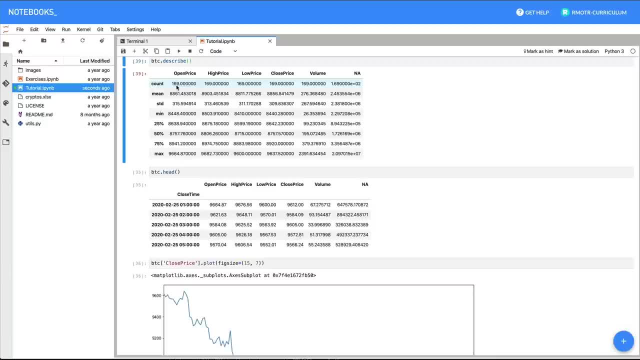 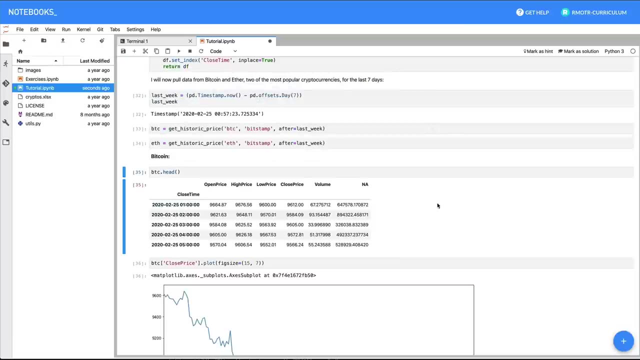 dealing with millions of records, So it's impossible to see it. Have you ever tried scrolling in an Excel spreadsheet through millions of records? It's crazy, It's not possible. It's just unusable. That's again the way we work with data analysis in Python and R and other tools. we don't 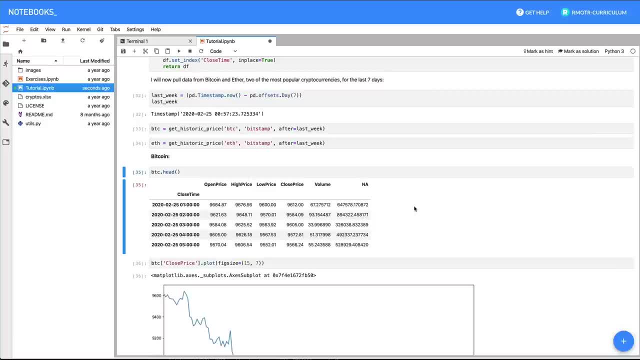 constantly keep an eye on the data. we know the shape of it And we just have these quick references like: show me the first five records, I mean the last five records, show me this chunk here, that there, but that's it. So, again, these are the visualizations we're. 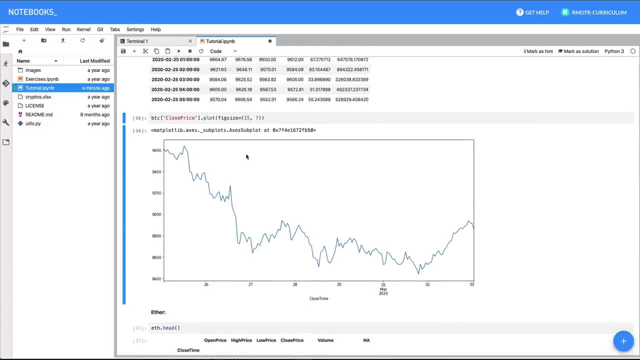 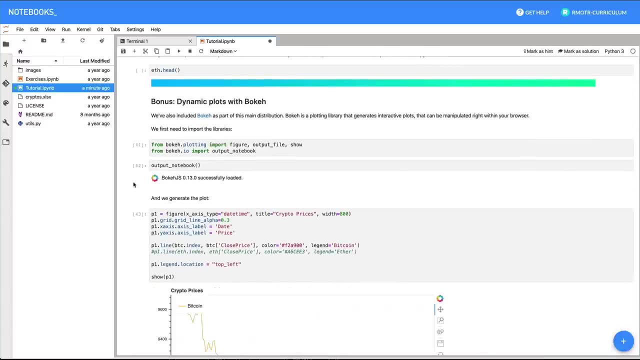 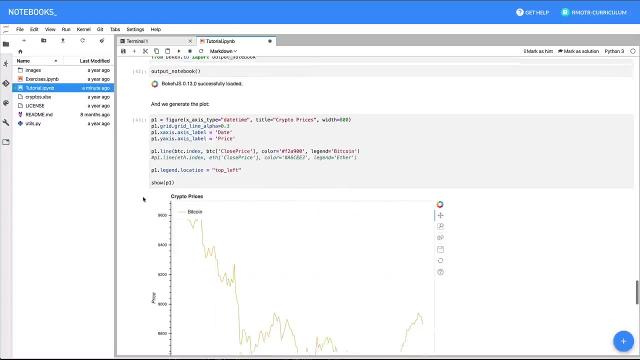 creating on Jupyter notebooks. Again, it's just very simple to get the plot done right there. And you also see in Jupyter notebooks a few other pretty neat things. The first one is that we can use another library which is called bokeh, And the difference that bokeh 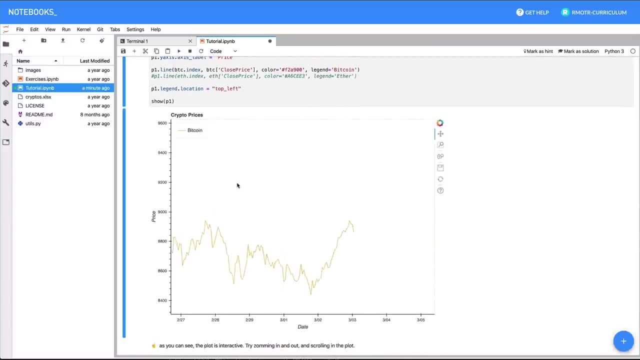 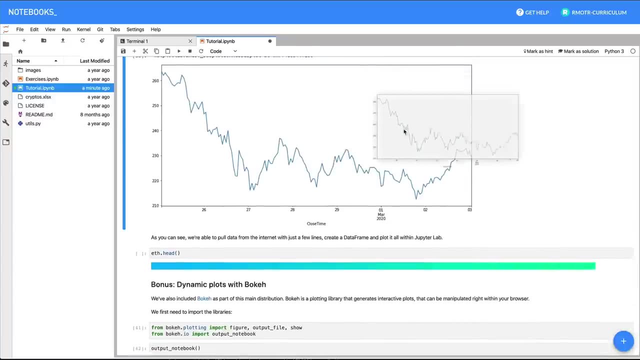 will have charts that are interactive, so I'm moving it right here. has JavaScript And it's in drag. if you look back again to what we had here, this is static chart. it's just a PNG. you can actually export it as a PNG. there is nothing you can do with it With 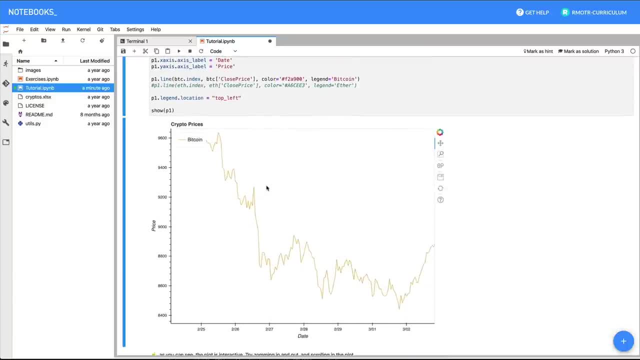 bokeh, It's actually a dynamic chart. It's a dynamic, dynamically generated interactive chart. So I can. I can zoom in pieces of data. right, they can move it around. I can just do whatever I want with it. I can refresh. 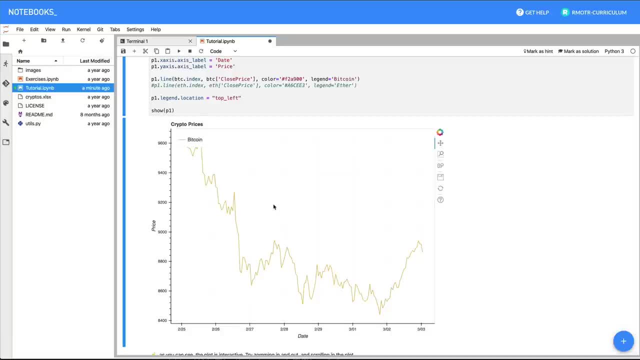 and reset it to whatever it was, And it's a dynamically generated chart. The difference is, if you're working with data dynamically in your analysis, sort of in your exploration, then bokeh is a pretty neat tool because you can zoom in right. So what's going on? 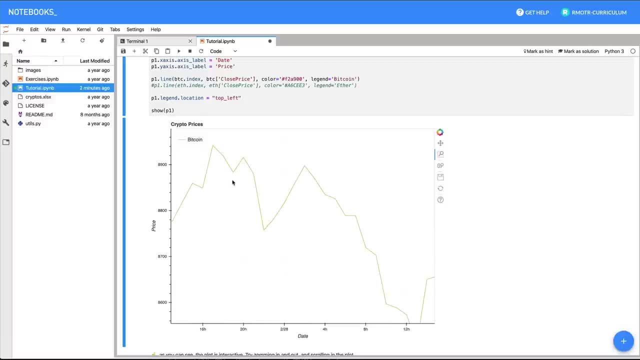 here, let's. let's look at this thing. If we're working on a mean reverting strategy, for example, we see a high value, we see a low value. the mean is going to be here, So we see some mean. 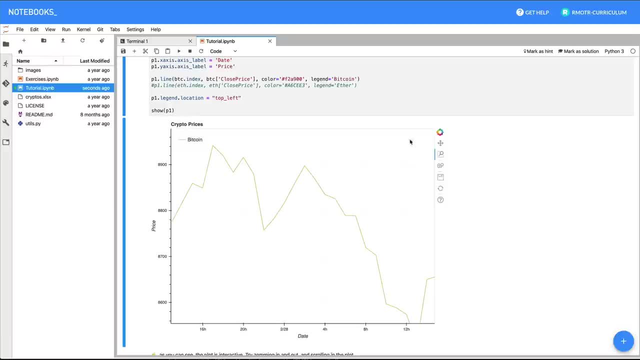 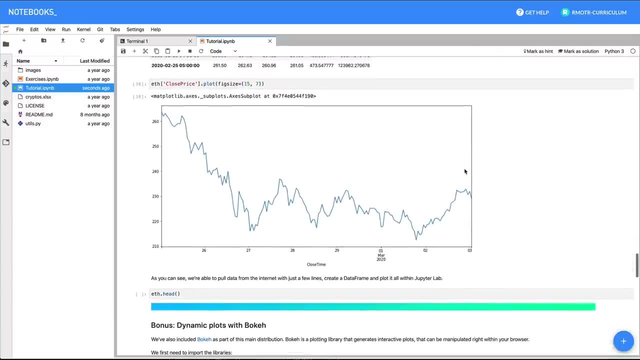 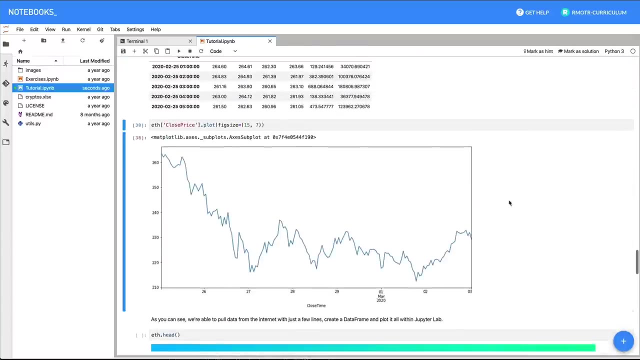 reversion in there. It's very interesting. If you need to, for example, export a PDF, export a huge HTML file, then static images are going to be probably better. So that's the difference between them. To be honest, model live is a lot more popular than bokeh. 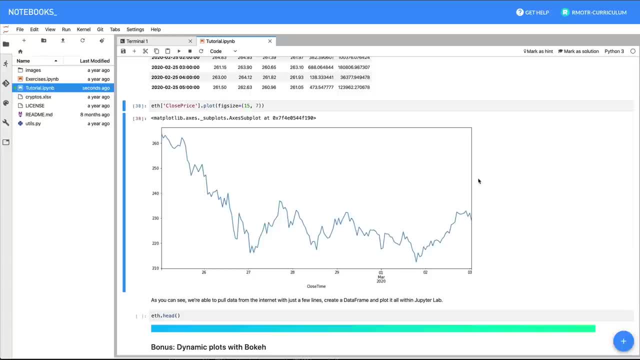 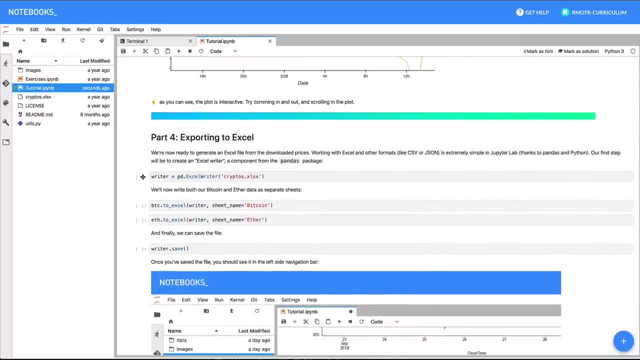 we use maplo live a lot more because it's we actually have a few other tools like seaworn that make it very easy to access and use it. What else? Jupyter Notebooks work very well with some Excel, Excel files, with other file formats- CSVs, XMLs, Excel files, etc. And 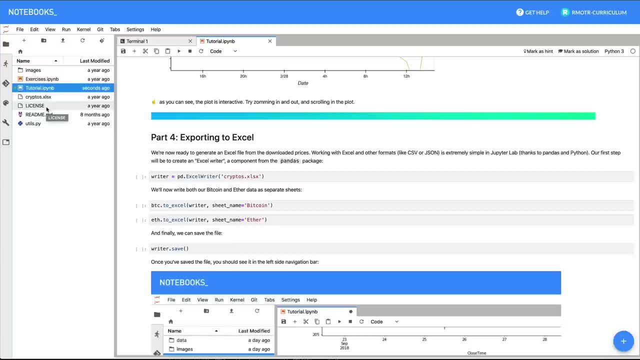 that's also the the availability of Jupyter lab. So Jupyter lab can immediately interpret an open CSV file. It can open, with some extensions, XLS files, XML files, JSON files. has a very nice editor and tree view for JSON. So the Jupyter lab environment combined with Python, Jupyter notebooks. 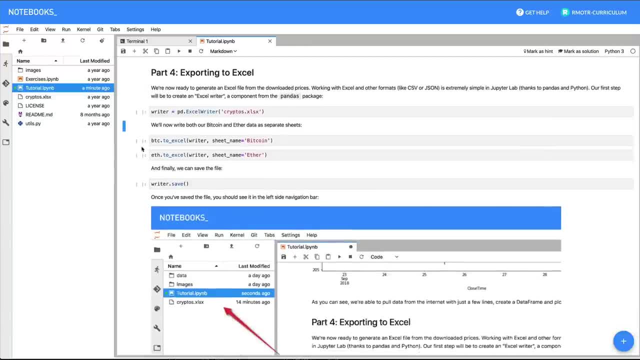 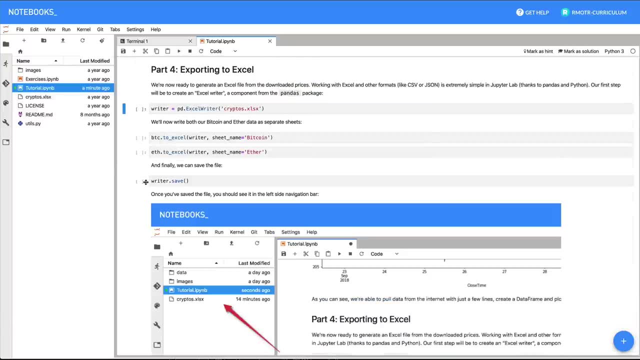 will give you a good idea of Jupyter in general. So in this case we have just saved. I'm not going to execute this. you can try it out, But you can execute and run what we have just done and export this crypto file as an Excel file. 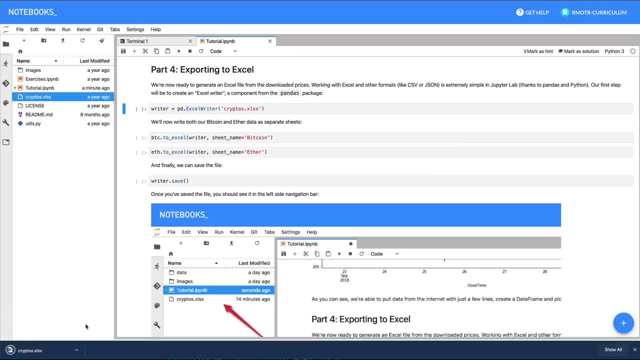 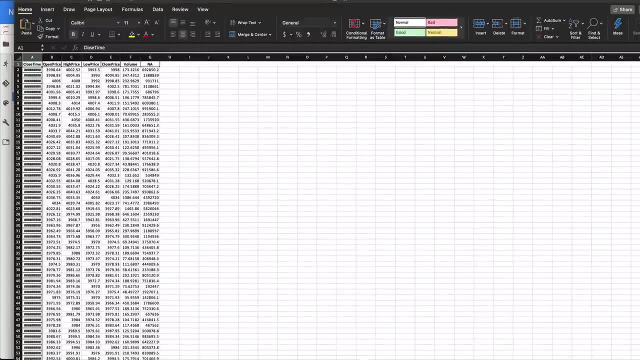 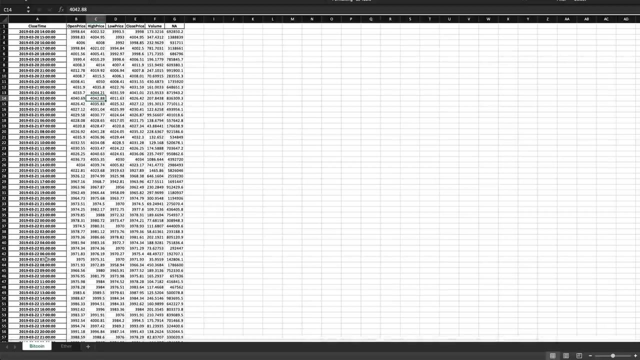 spreadsheet So you can just click on here and you can basically download it. I'm going to open it and see what has. there we go, So let me reduce the size of this thing. There we go, So you can see that we have just exported to spread to sheets, in this case, Bitcoin. 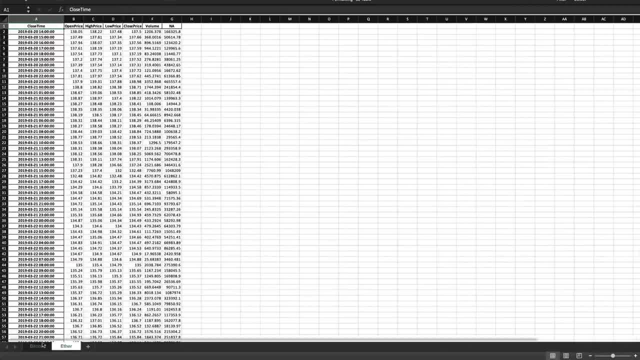 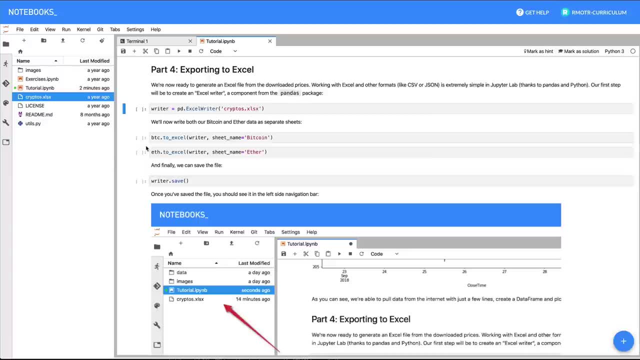 on ether, right, Right With the data that we had in our previous notebook, right. So that's all again. the combination of Jupyter, the combination of Python, the combination of Jupyter lab, which are tools, just work very well together. So we're going to keep moving forward in this. 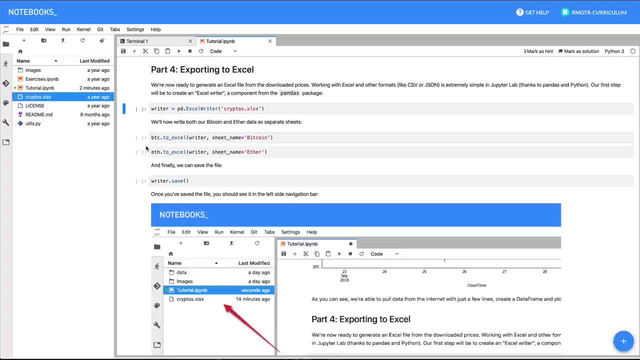 video, this tutorial, talking about more data analysis In general. we're going to talk about Python. we're going to do a quick review of Python. maybe when we, when I was running these commands- you fail, you've you felt a little bit lost. 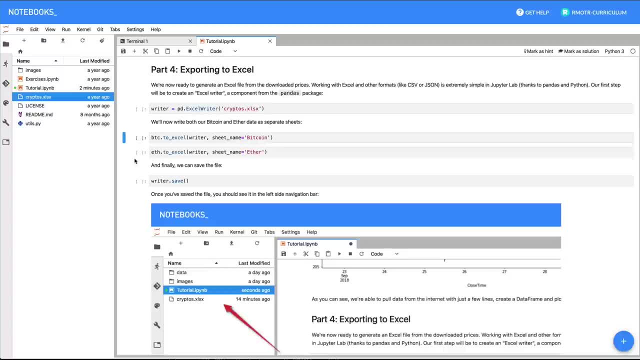 What I was doing with it. So we're going to do a quick review of Python and all that And, of course, we're going to get directly deep into data analysis with pandas, with some other tools. I want to tell you something before we finish this chapter, and it's that. 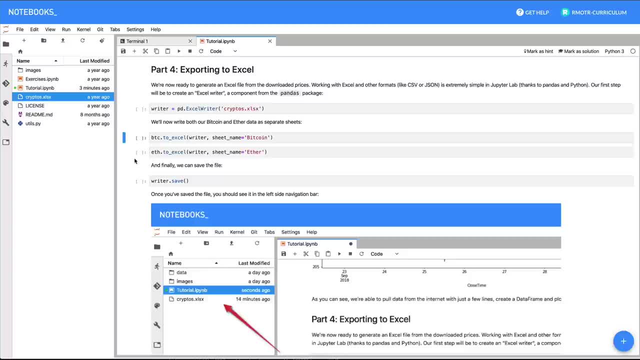 is very important for you to get familiar with data analysis, with- sorry, with- Jupyter notebooks, because you're gonna spend a ton of time with it And it's a very, very valuable skill you can get if you get proficient, comfortable with. 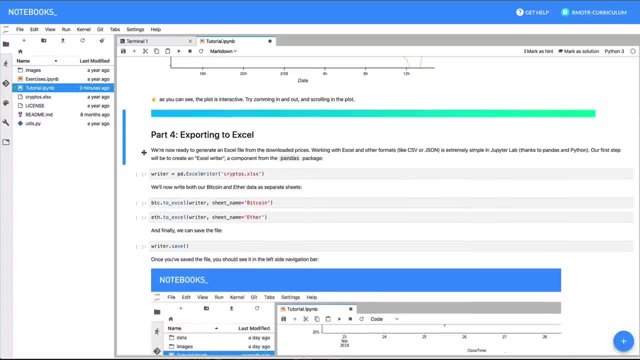 Jupyter notebooks, you know, like creating cells, deleting cells, cutting, pasting, moving things around, etc. For you to generate reports. Jupyter notebooks are going to be excellent, So keep an eye on it, keep practicing. it's the only way to learn it to you, to analysis. 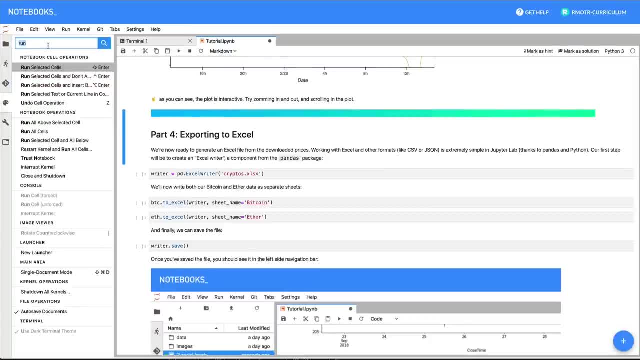 keep practicing it, keep open the command palette So you can always, if you forgot, how can it cut a cell? Well, there is here this command x. right, it's gonna just tell you upfront And keep an eye on it, keep working with it and practicing it And once you get familiar, 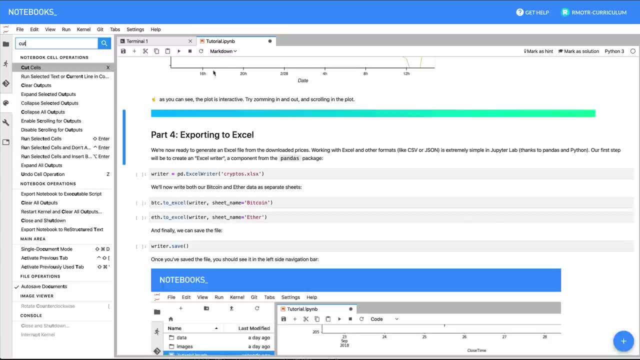 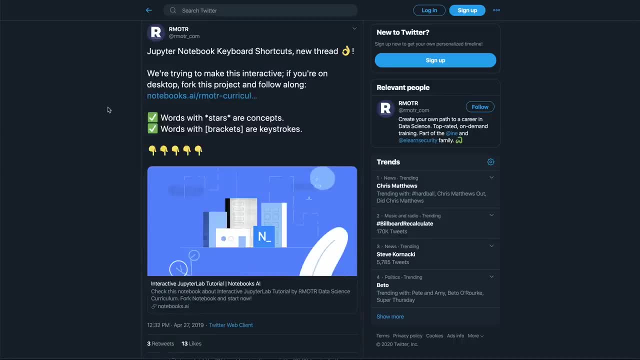 with Jupyter notebooks, you're going to move very, very fast. Remember, they have these nice list of compiled commands and reference you can always access if you need extra help. And we're going to keep moving forward now with more data analysis, And now it's time. 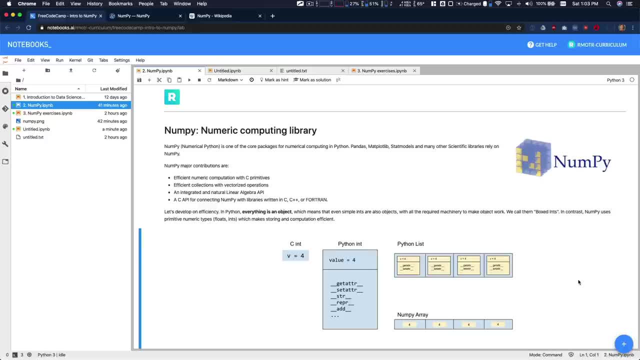 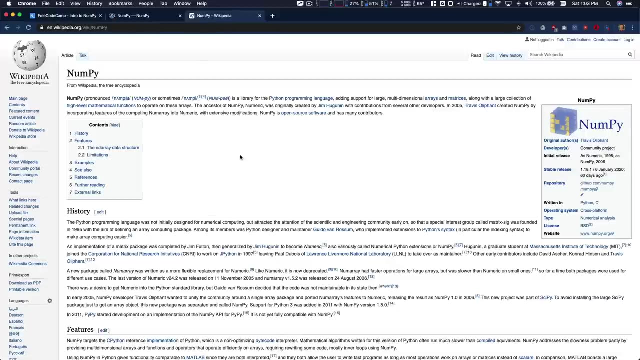 to talk about NumPy, One of the most important libraries in the Python ecosystem for data processing in general. it's the one that got pretty much everything started And if you trace back NumPy, it's. it's a very old, developed library- 20 years maybe it's. it's an extremely popular library. 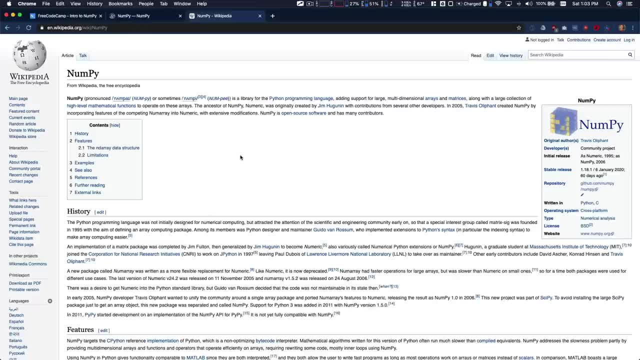 an important library. I'm not gonna say popular, and I'm gonna explain why in just a second, But it's an a very, very important library In the Python ecosystem for data processing. NumPy is a library that will let you. it's a. 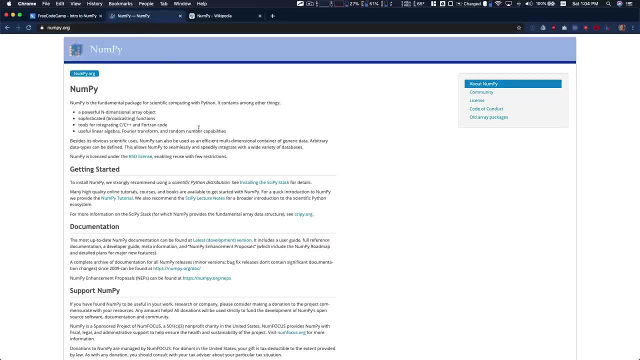 numeric computing library. it's just to process numbers, to calculate things with numbers, And that's it. So NumPy has a very limited scope. we could say- and this is on purpose, a very simple library when you look at it And when you look at the API, which is very 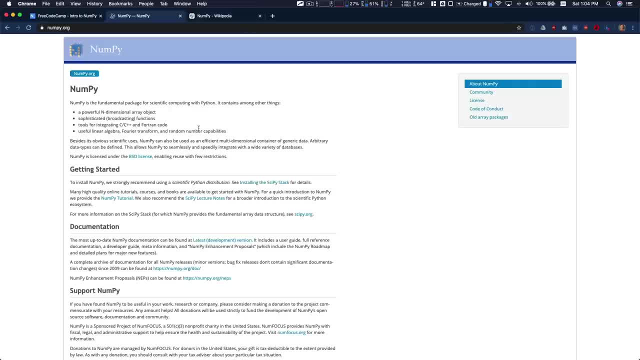 consistent. by the way. Why is NumPy so important? Well, in Python, numeric processing, in just pure Python, processing numbers is very slow. Okay, Python is not slow as itself, compared to other programming languages, But when you go down right to two very deep levels of performance, when you 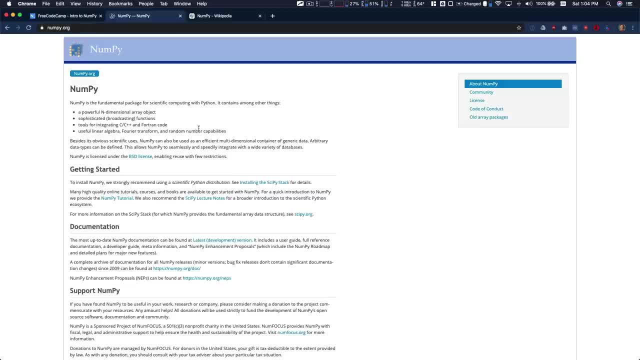 are processing large amounts of data, right, and you need to squeeze even you know, that tiny bite at the end of your pipeline. you need to squeeze every flop from your CPU, then Python is not the right tool for that. Python as as a 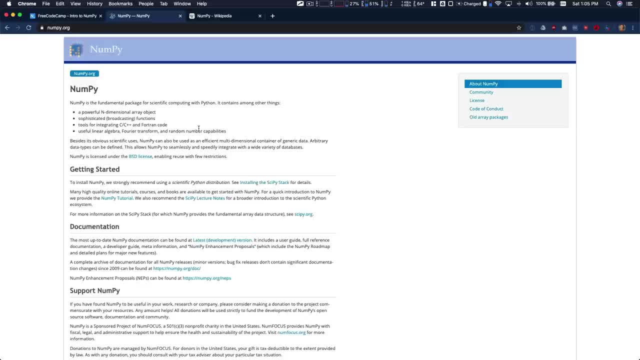 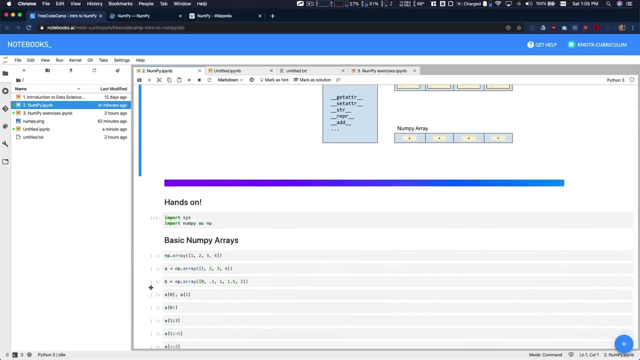 pure Python programming language. NumPy is actually solving dot. NumPy is a very efficient numeric processing library that sits on top of Python and gives you the same API as you're going to work with with just writing Python code, as you're saying here, but low level. 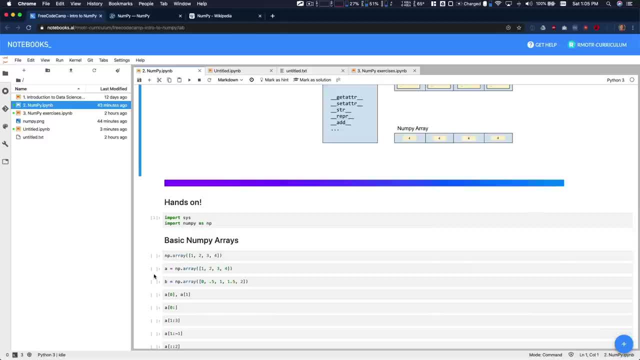 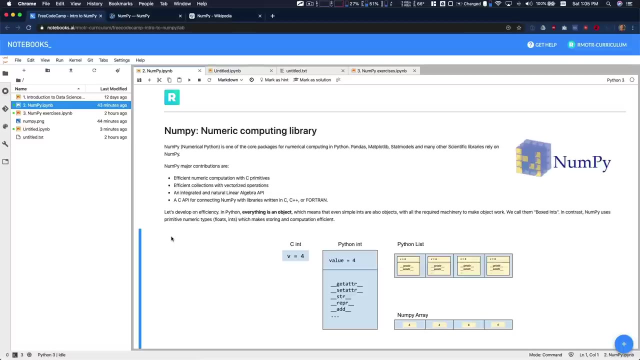 it's going to be using high performance code, performant numeric computations and and arrays and numbers and representations, etc. That's it. that's it for Python NumPy. It's extremely simple from from an API perspective, but it's extremely powerful. Why did I say that it's not so popular? but yes, it's so. 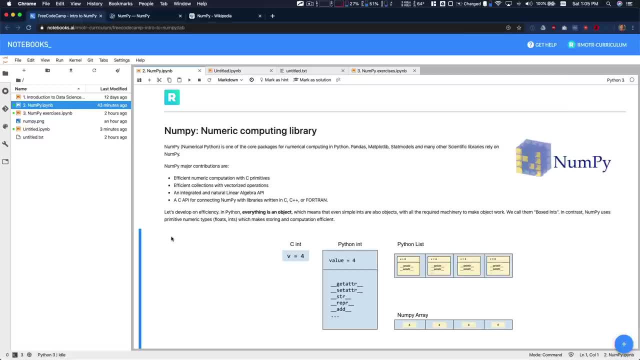 important? Well, because in reality we don't usually employ NumPy directly. you will not see yourself using NumPy so often, but you will be using other tools in Python, like, for example, painless and maplo lib, And they are all working on top of NumPy. They're all relaying on, relying 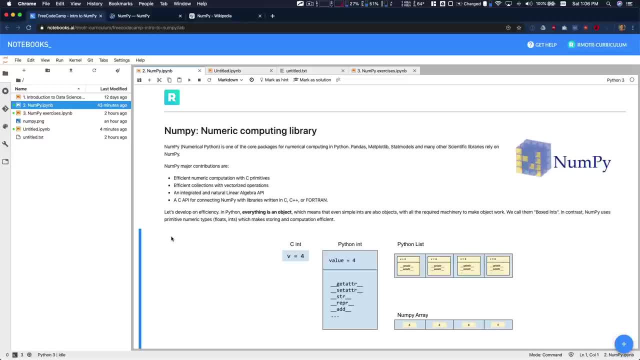 on NumPy for their numeric processing. So that's why NumPy is so important. So the for, at least for this part of the tutorial, NumPy- I'm going to divide it into pieces. The first one is going to be a very detailed low level explanation. 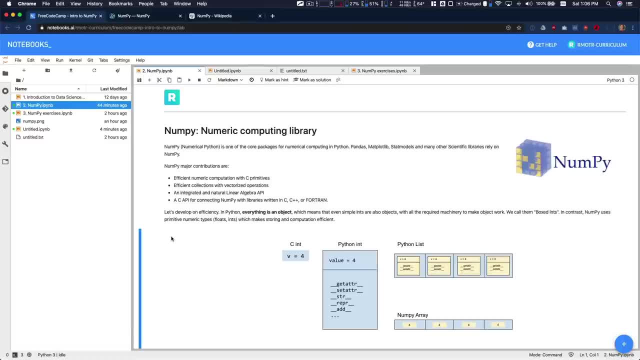 So the first one is going to be a very detailed, low level explanation. So the first one is going to be a very detailed, low level explanation of how NumPy works, why we need to use NumPy And what are the differences between different. 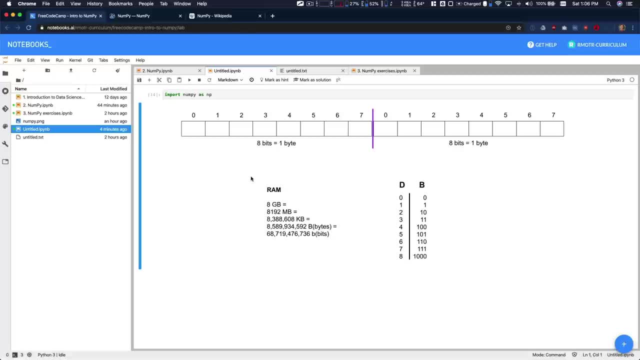 byte sizes for numbers. we're going to talk about integers, but this is going to apply for decimals and datetimes also- and why you need a very low level optimized tool as NumPy. Now you can- you can- skip this part you're going to find in the description of this tutorial. 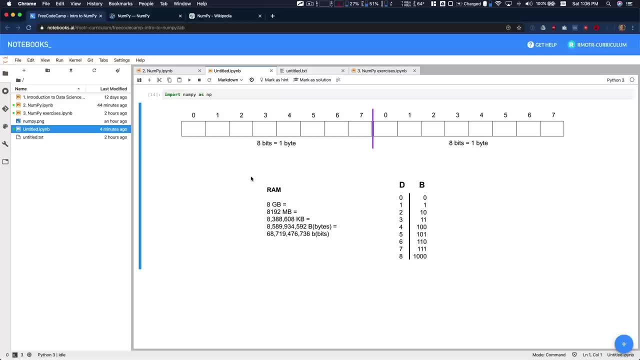 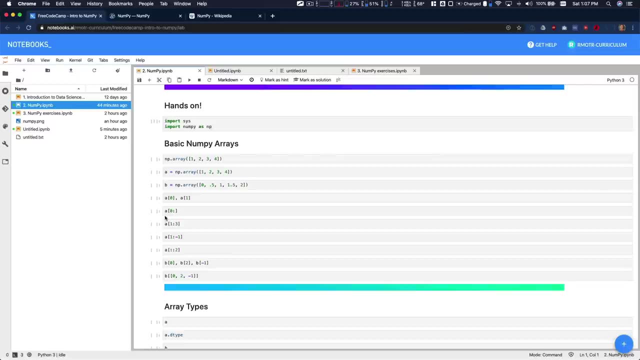 the precise moment in time. so you can just skip and go directly to NumPy, go directly to the second part, which is when we actually start using NumPy And I show you how to create arrays, how to make computations, etc. So for now we're going. 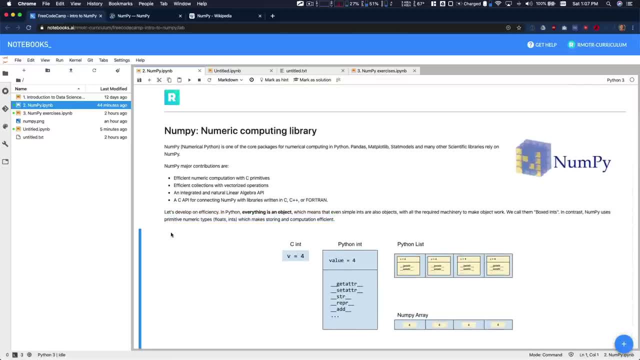 to divide it in two parts. we're going to start first with the low level explanation, which you can escape if you want, because it's not going to be crucial. you can easily use NumPy without it. We've found that for some of our students it's it's important. 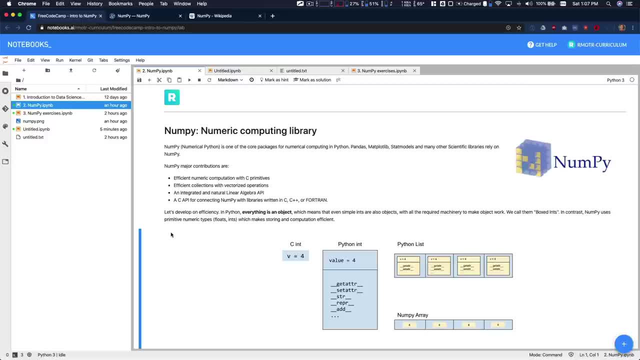 to understand the low level basics of it, especially if you didn't have a computer science background. it can help you get you know, raise your right, your level of understanding of computers and how to make your computations more efficient. But don't worry if you if 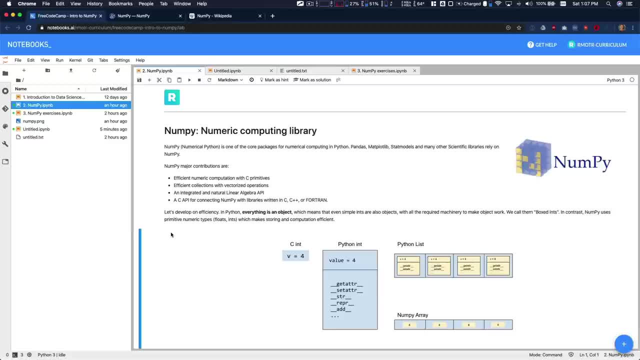 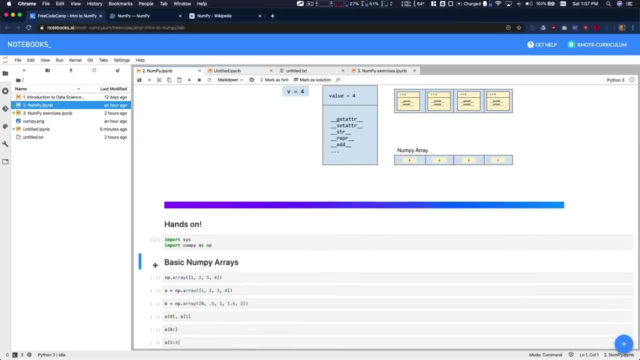 you don't want to go through that now, it's fine. you can skip this part and come back later or any other at any other moment. you don't need these to use NumPy Seriously. you don't need it. it's going to be beneficial but you don't absolutely need, so you can just. 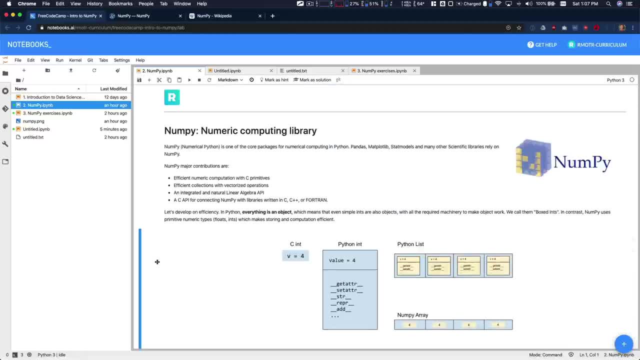 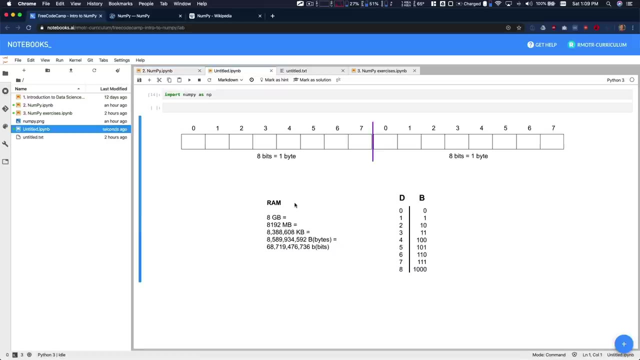 skip and come later. That said, let's actually go into a into a deep understanding and explanation of how computers store integers, numbers, in memory, and what are bytes, bits, etc. In order to understand why NumPy is so important, we have to go back again to the basics. What are numbers? 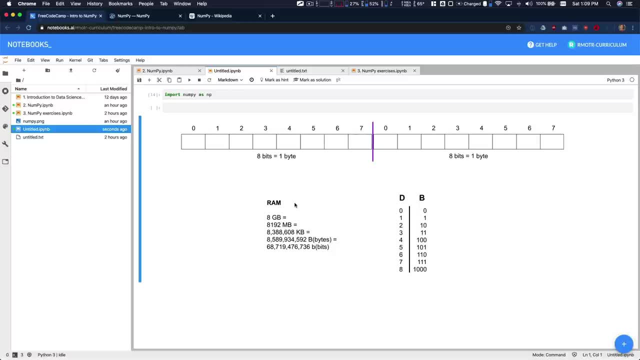 how they are represented in computers, etc. As you might know already, a computer can only process ones and zeros bits. it can't process numbers, Or just decimal numbers to be more correct. sorry, it only can process ones and zeros. 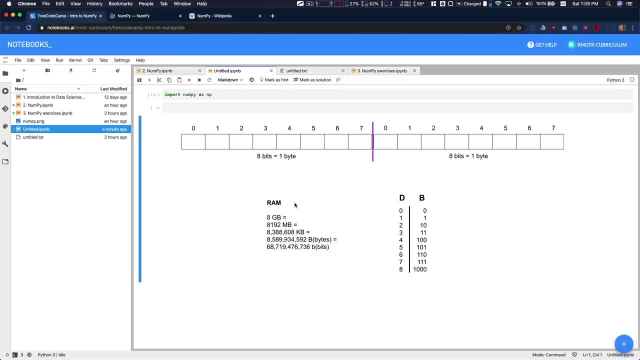 a computer is just always storing and processing ones and zero. it's a binary machine. Your memory is the central place around the random access memory in your computer is the central place where your computer is storing the data that it's actively processing. right So you? 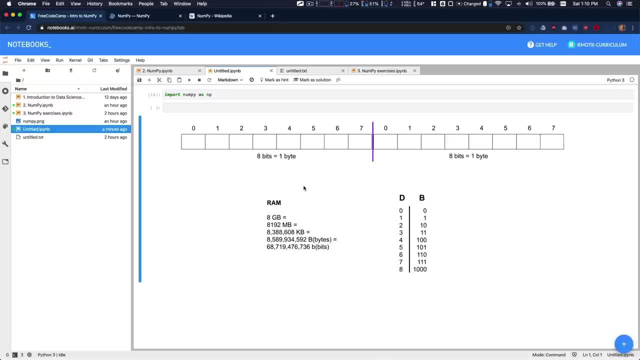 have, for example, a hard drive which stores long term data, but the computer can't process data directly from the hard drive. Before doing that, it has to load it into your RAM, into your random access memory. again, usually, right, a computer is going to have what? eight gigabytes, 1632, doesn't matter, let's say you. 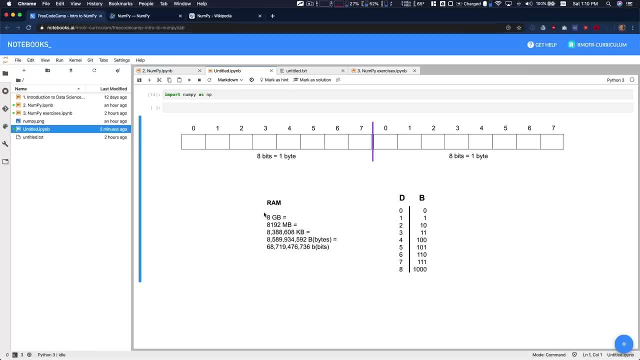 have eight gigabytes of memory. that at some point is going to translate to number of bits that your computer can store. So if you follow, if you follow these we have right here, you can see the total number of bits available in a regular computer with eight gigabytes of memory. Why? 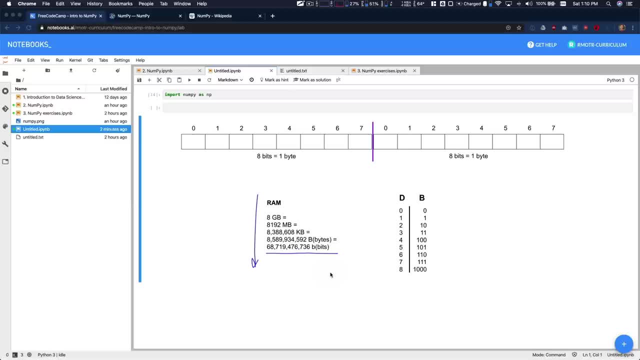 is this important? Because, again, the objective of these of these tutorial is the objective of this part at least- is to explain how you can squeeze out of every single bit you can in your computer, right? How can you make it more efficient for your numeric processing, both in storage? use less. 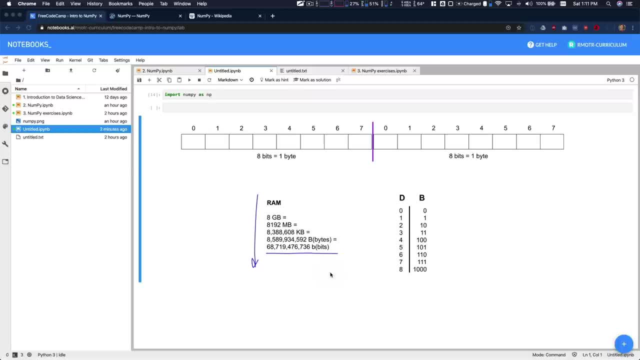 memory for the same data and also how to make it faster. right for your calculations. So, in terms of physical storage or actually memory storage, right, How can we make it, How can we optimize to use the least amount of memory for this given problem? That's objective. 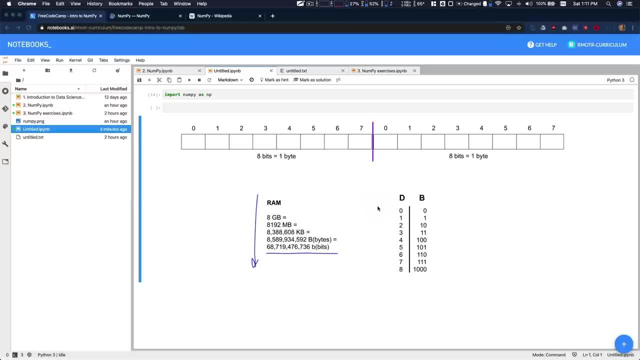 of optimizing it. we need to understand how numbers, Decimals or sorry, integers in the decimal numeric system are represented in binary right. So this table right here shows you the first nine numbers, 01234, etc. And their binary representation in your computer. let's say you want to store the age of user age. 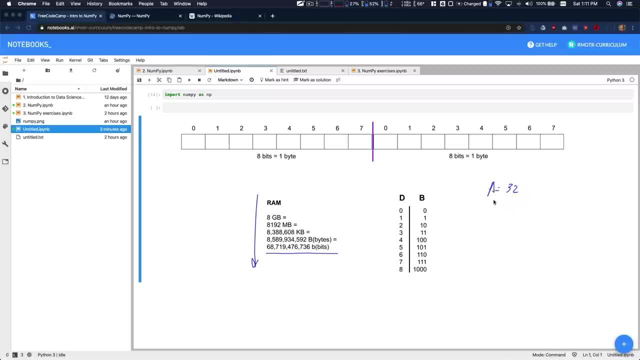 of a user, which is I don't know 32. You can't store 32. In here, because your computer, again, doesn't know about decimals, it only knows about binary. To do that, you will need to find the correct representation in ones and zeros of 3030.. Right, sorry to which. 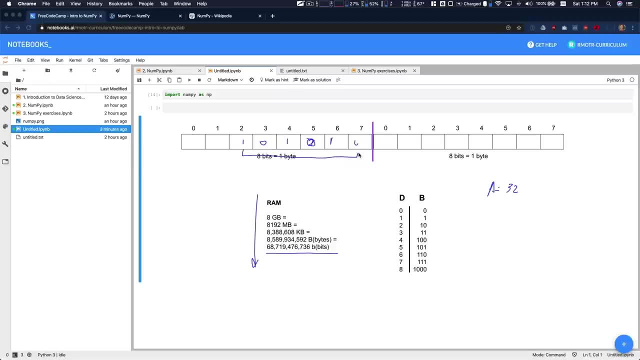 is not this one, to be honest. I'm just making it up as we go. But again, you need to know the correct binary representation of these number in order to store that data. How can you know that? Well, there's a whole binary arithmetic, right, There's a whole part of math dedicated to 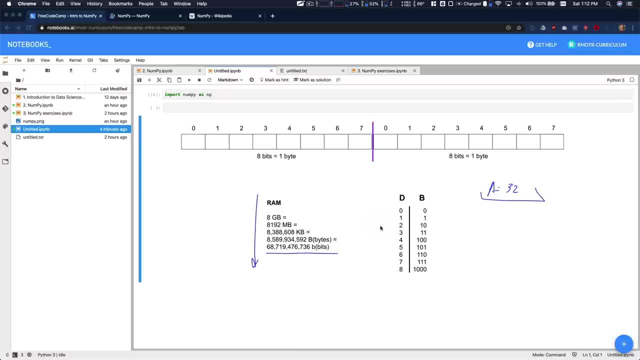 binary doesn't matter for now, But I'm going to just drive the intuition of it So you can have a better understanding And if you're interested you can dig deeper later. So, basically, any decimal number needs to be stored in a binary format, which of course only takes. 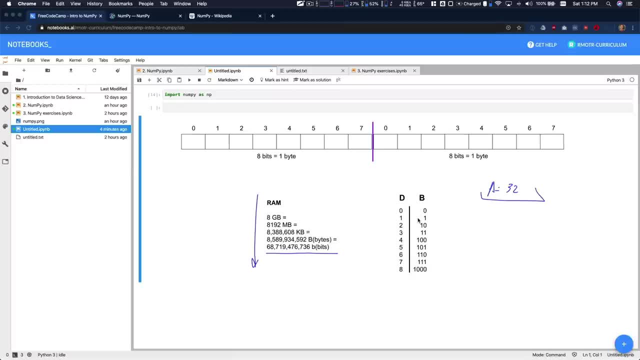 ones and zeros, And what we usually do is just we keep increasing zeros and ones in positions, right? So in this case we have the number zero, the number one. that's fine. Once we need to store the number two, we need now to increase the number. 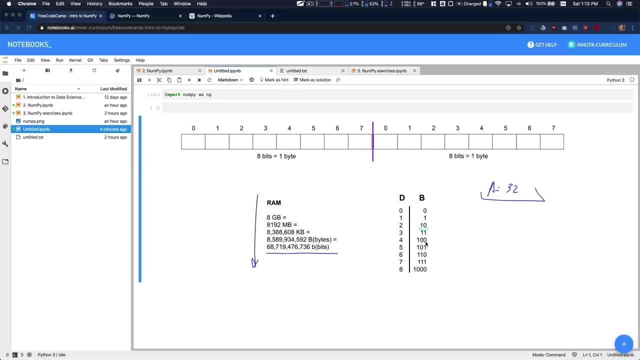 the position. right here we need to increase right. we need to go from two to one zero. we go to the number three: it's 11.. And then, when we need to go to number four, we need to increase positions again, because we only have two symbols: zero and one. So, as you're, 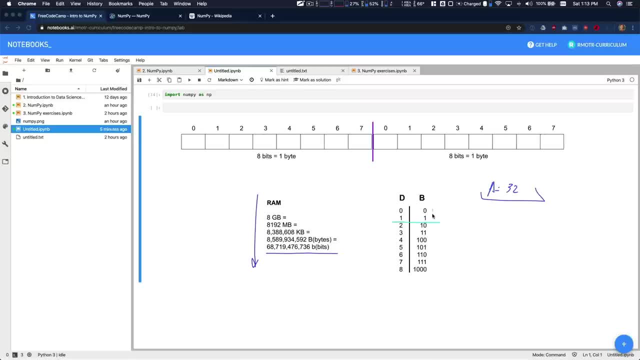 seeing right here: up to this level, we need only one position. Up to this level, we need two positions. this level, we need three positions, And this level is going to need four positions, And you'll see how the size of these is increasing. 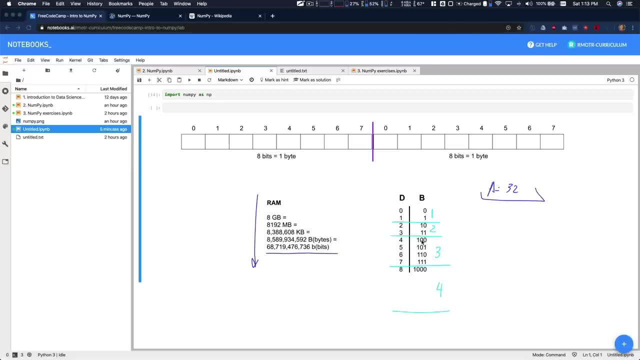 And it's good. It has a an explanation behind it that we're going to see in a second. So the question is how many decimal numbers you can store with Bytes and bits- sorry bits. So let's say we have n bits And let's say n is equals. 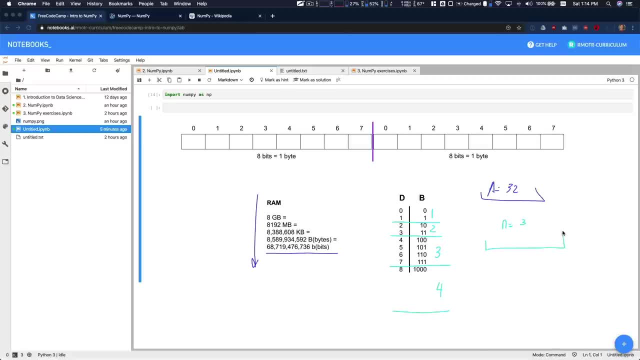 to three. That means that you only have three positions right, three bits, how many total decimal numbers you can store with it. Well, we can store zero, zero, zero, we can store zero. we can store one zero, zero, we can store stores. are you one zero, right? So? 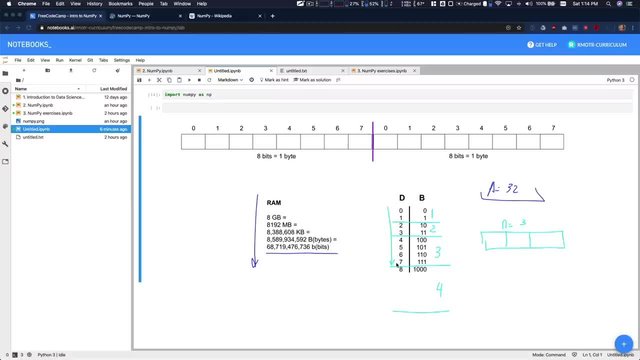 in these case, we can store up to here. we can store up to seven numbers. one one- one is equals to seven- was, once we fill all the positions right, we've reached the limit right. the largest number, the largest binary for this amount of symbols or positions, That's the. 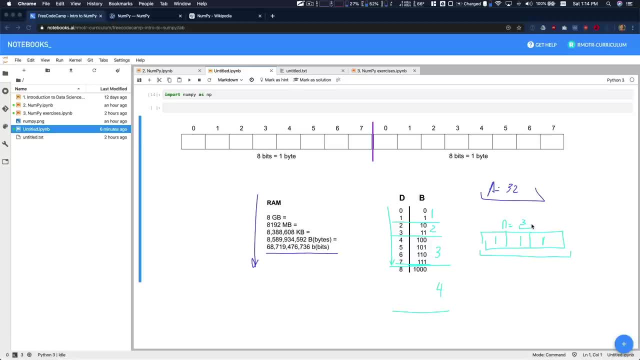 number seven. So this means that with three numbers you can store from zero from zero. from zero- here zero- up to 111.. In total you can store eight decimal numbers. Here you have eight decimal numbers: 012345678 total decimal numbers from zero to seven. The equation: 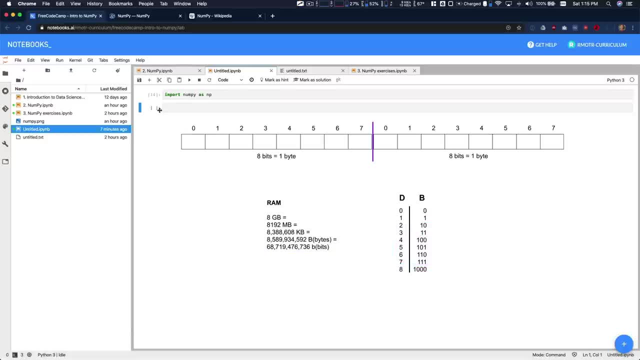 if you want. behind this is as follows: If you have n equals three and one bits, in order to know how many decimal numbers you can store with those bits, it's two to the power of n. in this case is total eight bits. So if we go back into our drawings, 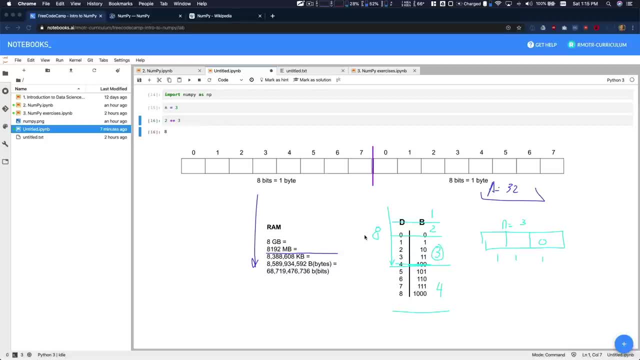 we said that with three bits we can store up to eight decimal numbers, And again the equation is two to the power of n. it's going to give you how many decimal numbers you you need. you can always do the opposite process using logarithm, and get how many bits you're going to need. 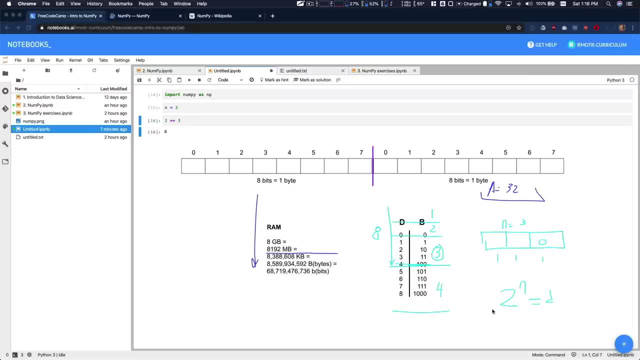 to create, to store a given decimal number. I'm I'm not going to get into that, So we don't complicate it. But again, the math behind it is extremely simple. So now, moving forward, we're going to delete this whole thing. Moving forward, why is this important When you're 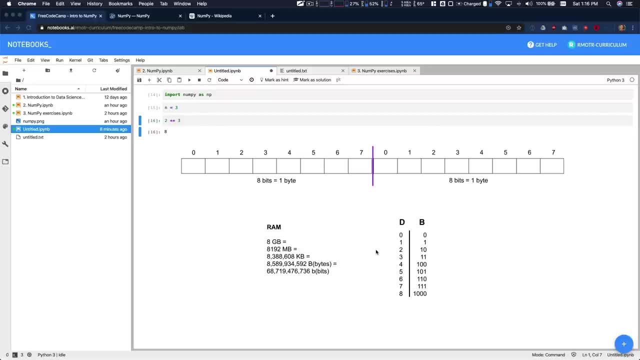 working with your data. when you're doing your data analysis, you know what, what data you're, what type of data you're working with. they're all numbers, but numbers all usually have a connotation behind right, So let's say that you have here- it's a table of people. 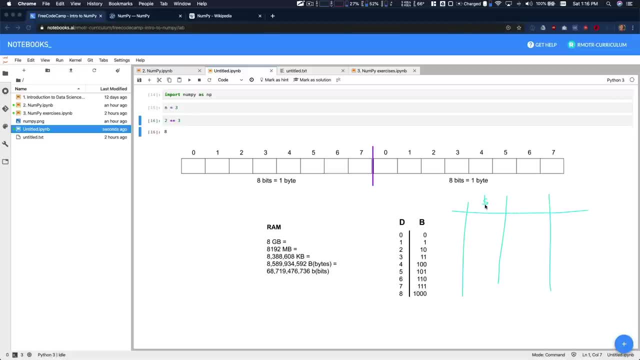 And you have the total net worth of the person And also you have the age of the person. The age is is a value that will range between what zero, right, just born to I don't know- 120,. we can say: 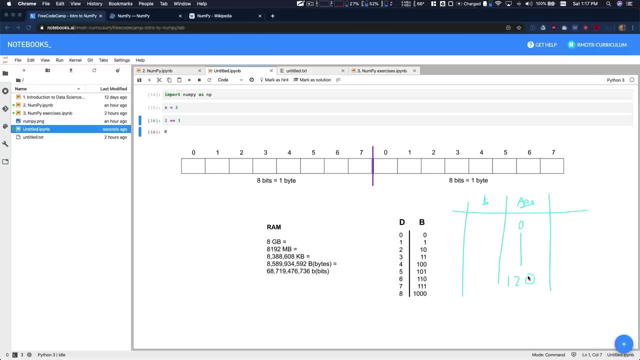 I don't know what's the maximum age registered right now- the oldest human being- but zero to 120 is seems, seems reasonable. In your other column, net worth for this person, the range is it's completely different. we can go from something like $0.. 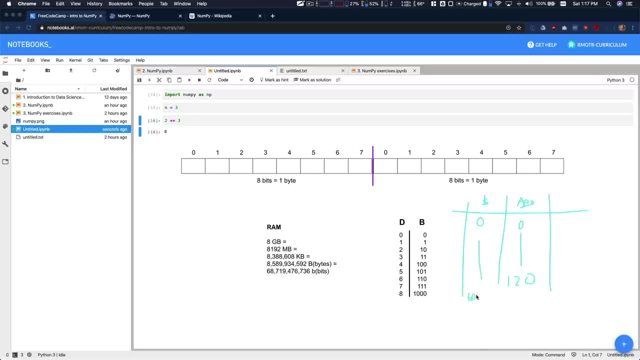 to I don't know $60 billion. I think Mark Zuckerberg or Jeff Bezos or one of those. So what? we go from zero to 60 billion. In this case, if there are dollars, what happens if this is a highly 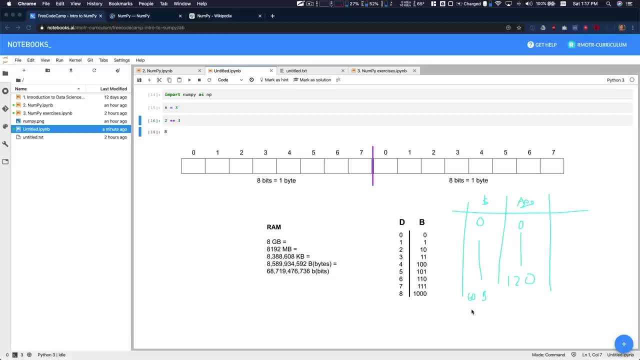 devaluated currency would have we have to go to trillions, right? So these two, even though they are just plain numbers and we can say there are integers, even though these are plain numbers, they have an integers, they have a different connotation. 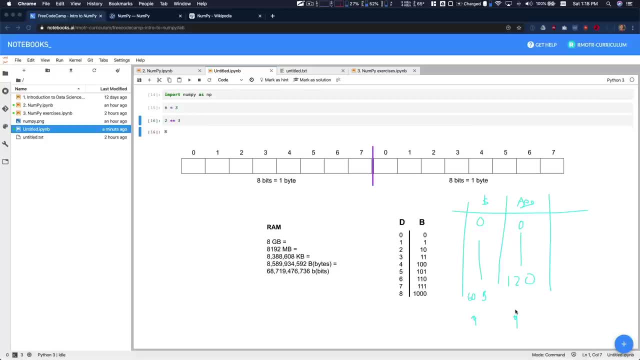 and they will need different requirements in terms of storage size, right? So if we say that an age goes from zero to 120, we don't need so many, so many bits to store it in memory, right? We can do the math. actually, how many bits do we need in order to store? 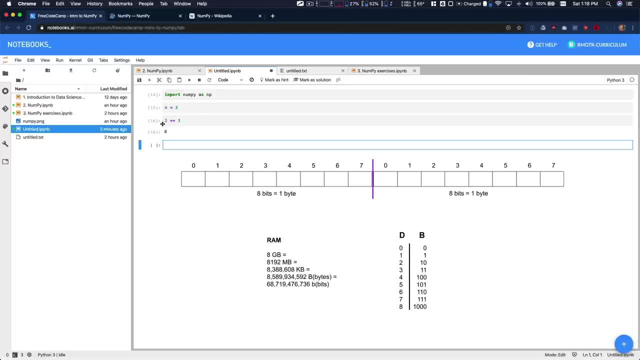 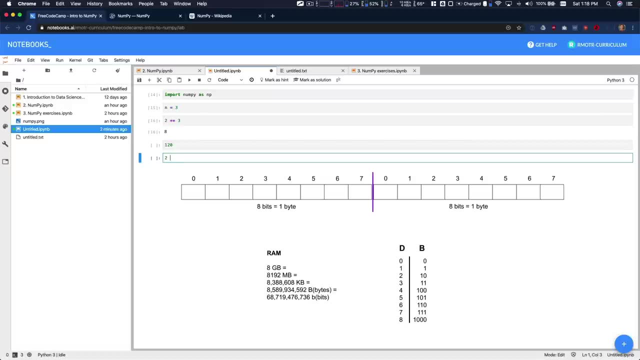 120? 100?? And what do we say? 120? Right? Well, if you do the math, you will see that two to the power of two to the power of seven is 128.. So if you have, if you have seven, 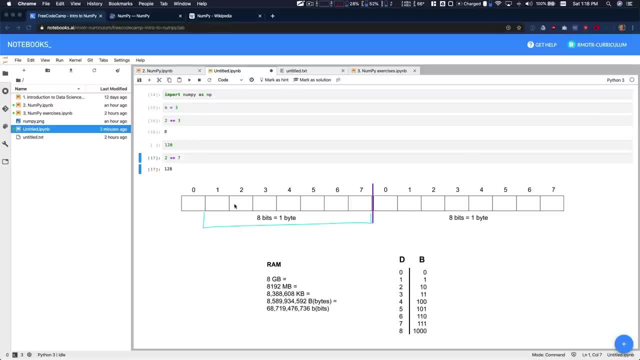 bits here, seven bits. you're going to store from zero up to 11111.. One, one, one one, which is actually 127.. Okay, these number, or once seven ones, in binary is equals to 127.. In decimal, in total we can store 128 numbers. zero, zero matters. 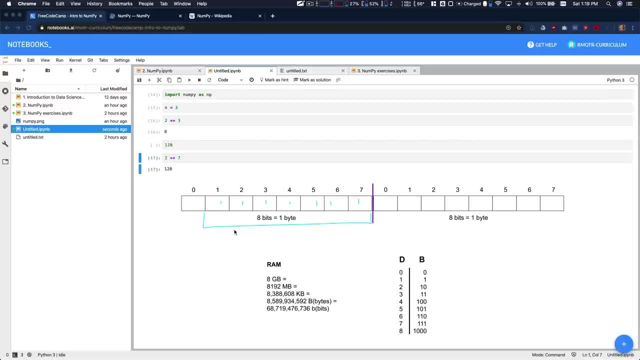 up to 127.. So that means that for our column right, the column age here, age we, only we can use. the size of the memory that we need to use is going to be seven bits per user or customer or person, whatever. What about these number right here if we? 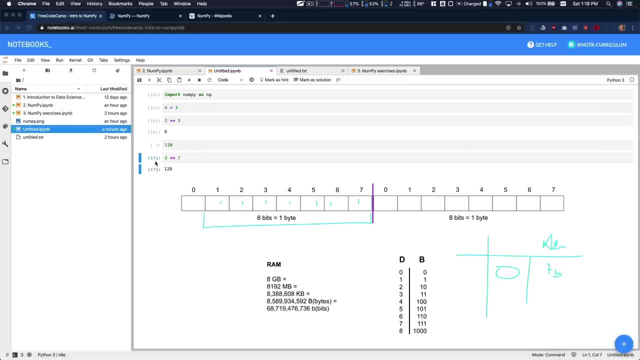 have to go up to a couple billions. Well, in that case, the the number is a little bit more complicated. we're going to need, for example, we can say 64. Or 3232, it's actually 64, probably, But with 32 bits, right, you can store up to from. 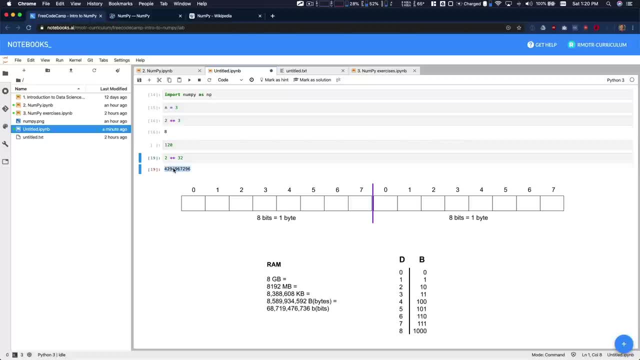 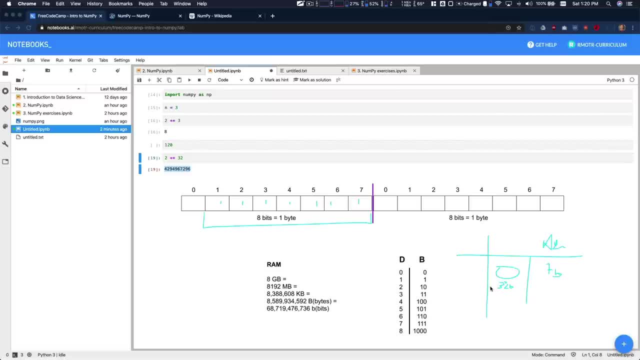 this data, How many records do you have? If you have only 1000 records, that's not significant. you can use whatever. you can use 64 bits here to store the age and you're not going to have a problem. But what happens if you have more? What happens? What happens if you? 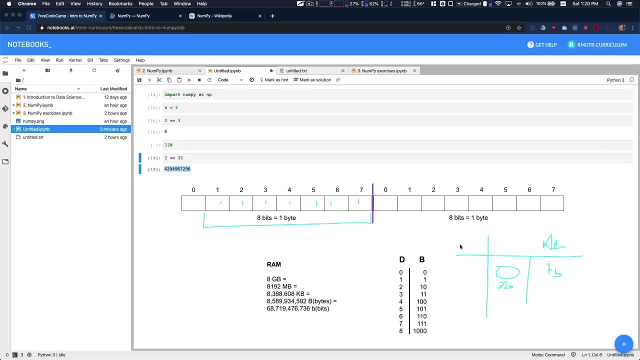 have the entire population of the earth. you have 7 billion records here, 7 billion records. then every bit that you're saving in these columns is going to be important, Because it's going to take a ton of data And, of course, you have a ton more columns. 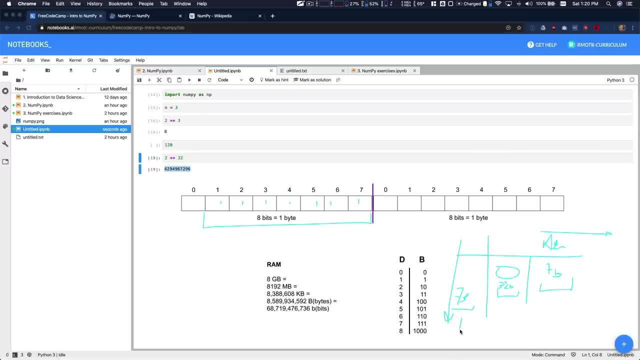 right, What happens if you're processing trillions of records from financial transactions? right, you want to be very, you want to be very efficient and optimize every single bit you have, And that means, again, selecting the correct number of of a bit per the column you're currently. 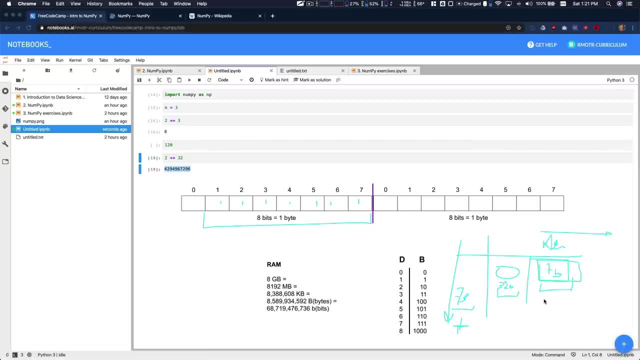 processing. So so far, so good. Again, we understand that the the the number in decimal that we need to store has a correspondence with in bits. right Eight bits is one byte, And the more we can optimize that, the less memory we're going to use for our applications. Where does 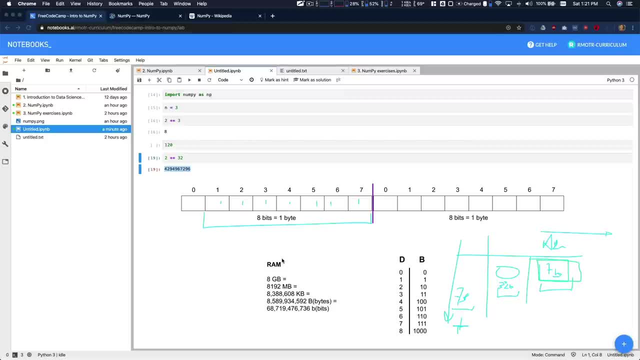 NumPy come in place. Why are we talking about this in this NumPy lesson? Well, the the idea is that NumPy is a library that will let you has a very advanced numeric processing in order to let you select the number of bits you want to take for an integer Even more. let's say you forget about NumPy, you want. 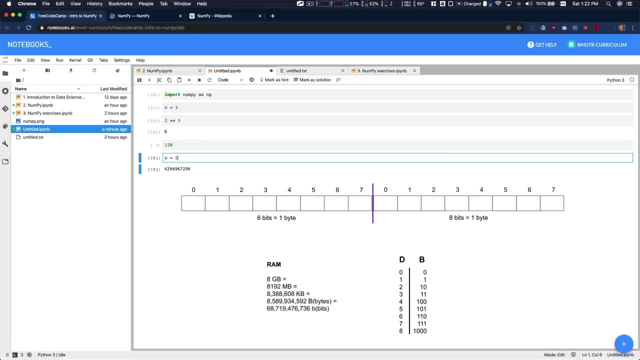 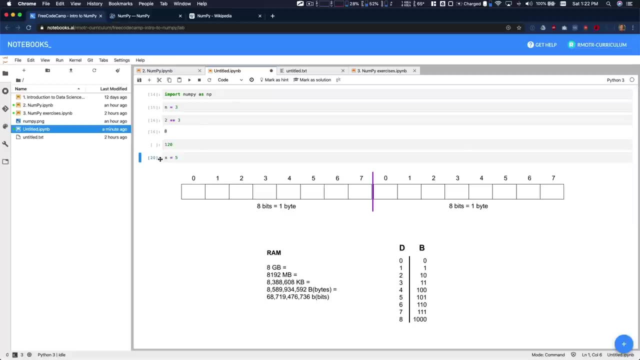 to process this thing with pure Python. So you do: x equals five, for example. working with Python, you create a number we're storing: age is a five. How many bytes? How many bits Do you think This A simple variable takes in memory? How many? Well, in reality, even though we think it, 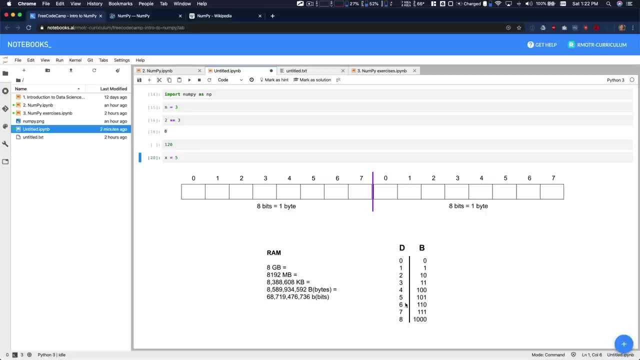 should be around what? three, three bits, eight, let's say big. to be simple, to simplistic. In reality, for Python, this is going to take around 20 bytes. Okay, so we are wasting a ton of memory in order to store this number, And why is that? 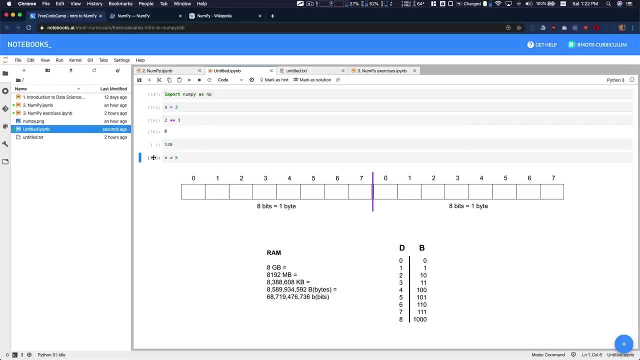 Well, Python, it's a high level object oriented programming language. The reasoning behind it is that Python is simple to write, a right, simple to also read and code on top of it. But again, in order to create that simplicity, it needs to wrap all the numbers in objects. 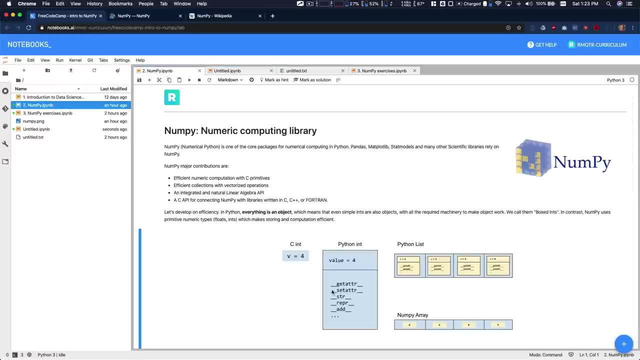 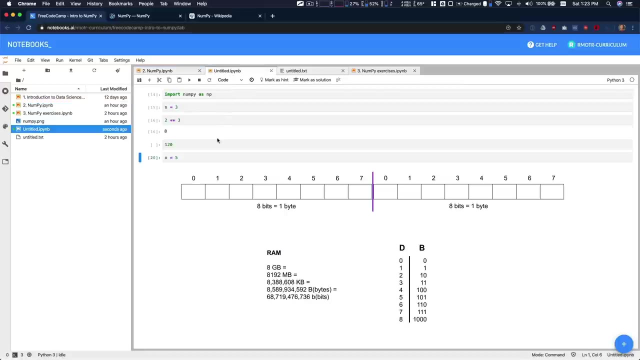 which have all these attributes that if you know advanced Python you're going to recognize that are not necessary. So these is taking a ton of memory, And a regular, very simple number in Python ends up consuming 100 times more memory than what it should be consuming. This one, NumPy, comes. 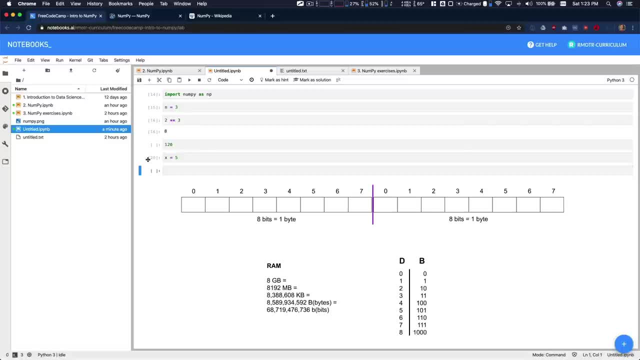 in place In NumPy, you can create numbers that are, for example, you can control the size in terms of bits. you can say: I want to create a number that has only eight bits And that's it, that you're going to create a one byte integer. 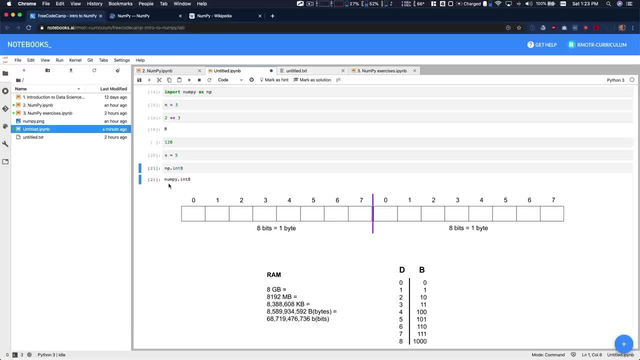 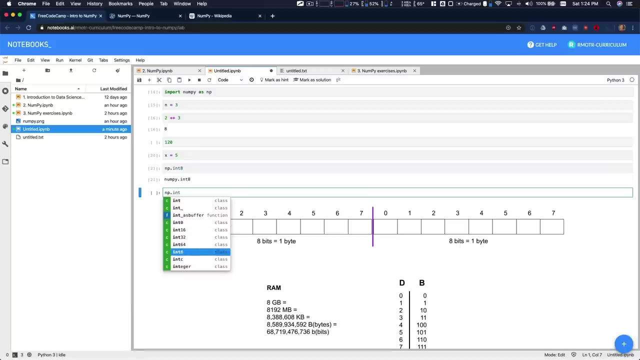 And you're very precise and how much memory it takes. you can create a number that it's actually need a little bit more space. we're going to do MP int And we can here use a tab key. you're going to get auto completion 6016 bits or eight, or 32 or 64.. Right so? 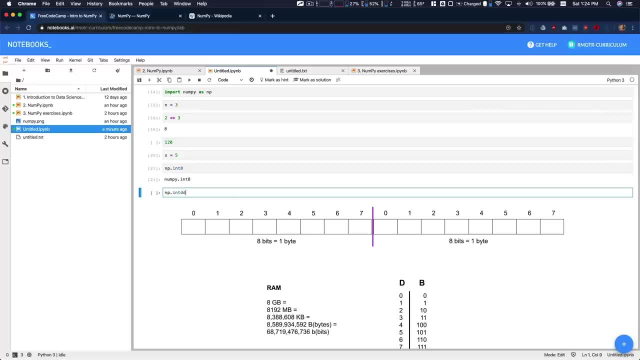 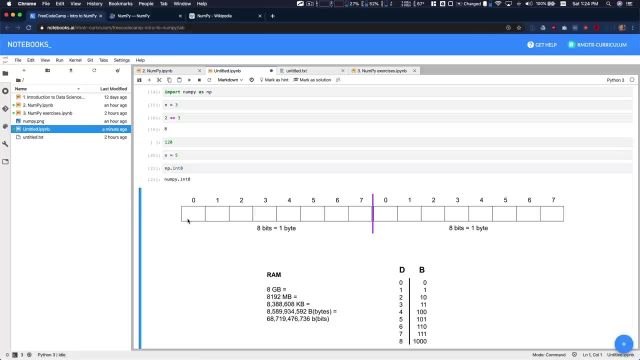 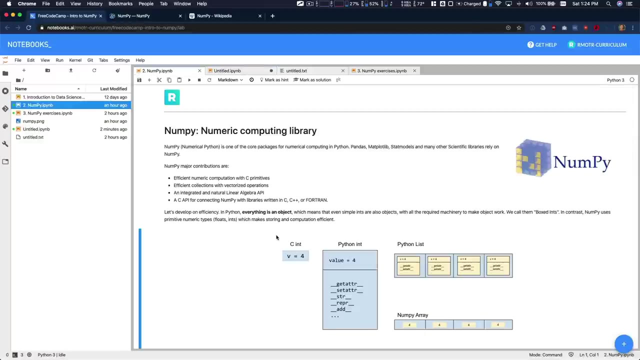 we can actually be a lot more precise in the number of bits that we need, And this is extremely important And, for again, our high level processing. On top of that, NumPy is a array processing library. NumPy is 99% about processing arrays, constantly processing arrays, the data structures. 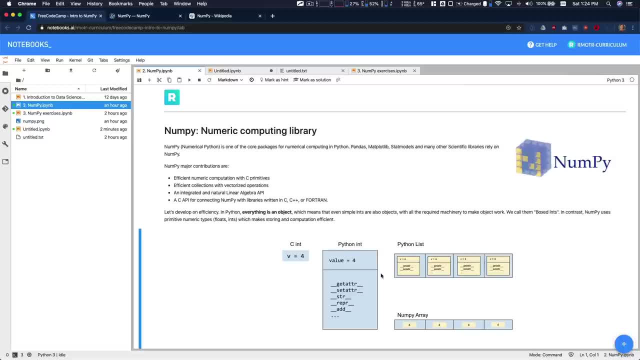 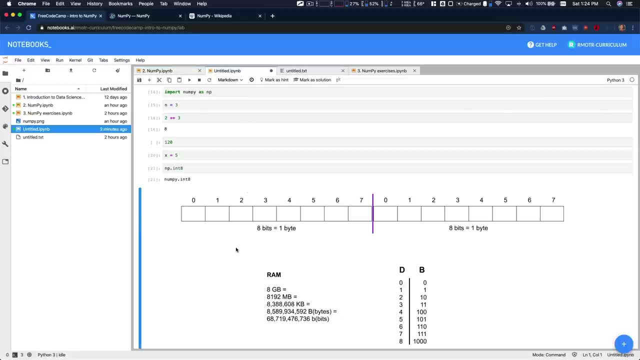 we have in Python the built in data structures. we have in Python, for example, the list dictionary. they are not optimized for high level computing. So if you have a list of numbers in Python, let's say you have. I don't know. 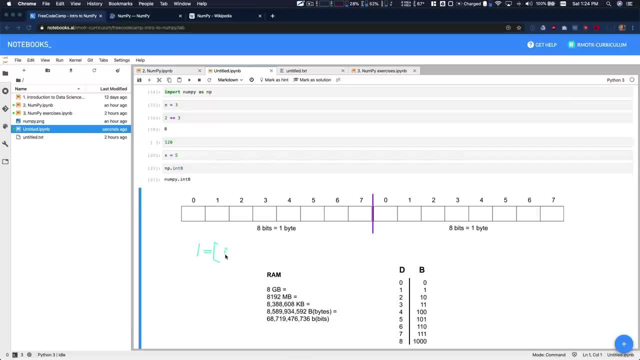 L equals three, two, two, four. right, you have three numbers in your list. In Python it's not guaranteed that the least the list is going to contain all the numbers three to four in contiguous positions is gonna. it might put them in separate positions in. 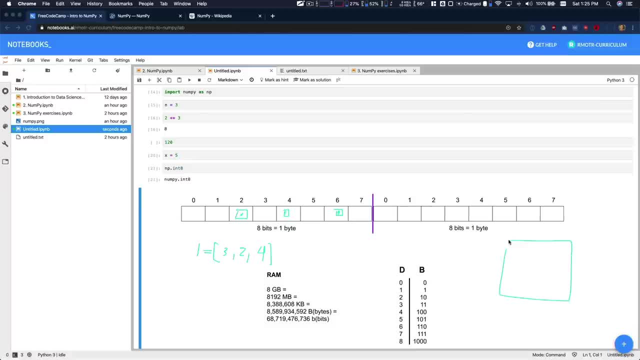 memory. On top of that, you can't rely on advanced CPU directives and instructions for processing matrix matrices- sorry, because Python again is wrapping these things in objects, So there is no access to these high, performant, low level instructions. With NumPy that changes, because when you create an array 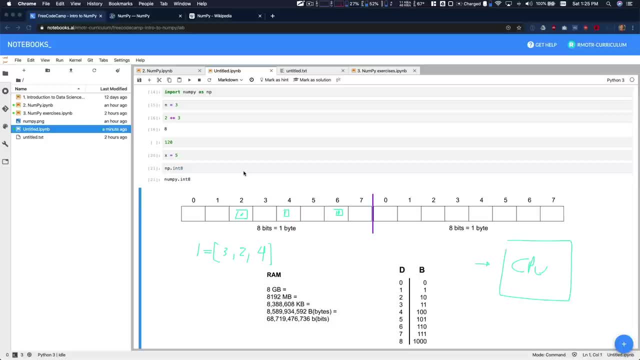 NumPy you say I want to create an array of three numbers and they are all into eight and imposition. Forget about, this is not. these are not bytes. I am, I'm using this drawing as a general representation of memory. So in that case, in Numpy, when you create these, 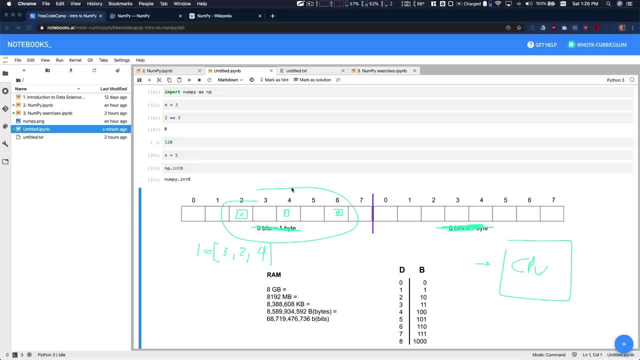 three element in eight array. it's going to create those three elements in contiguous positions in memory three to four and they are only going to take that amount of memory that we said they were going to take And of that we can rely on a bunch of very efficient low level instructions from your CPU for matrix. 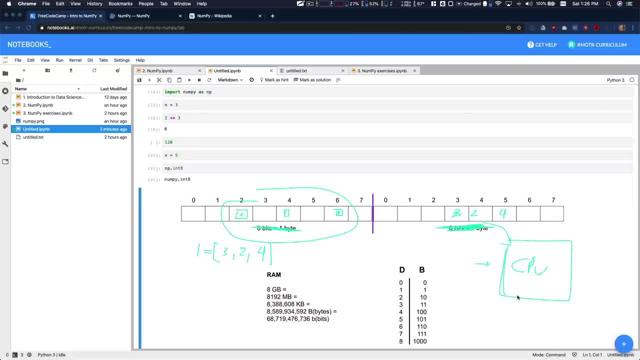 matrix calculations is something that it's a little bit more advanced And it's something that has exploded in the past 10 years: CPS with more, with richer instruction sets, And the same thing for GPUs, you might have heard, especially with machine learning and all that. 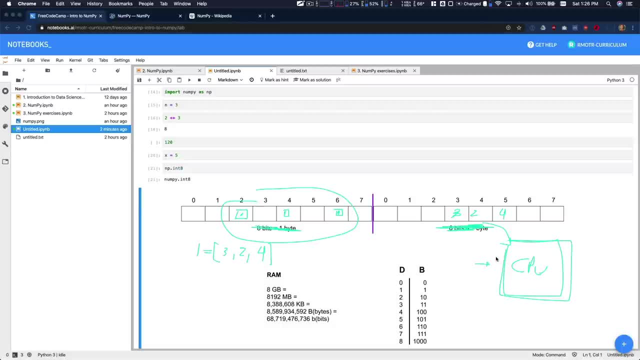 we need. we need fast array processing when we are sorting features and weights, and all that's a topic for a for different tutorial. But again, the idea is we need right, a ton of week, sorry. we can use all these important and very efficient low level directives from: 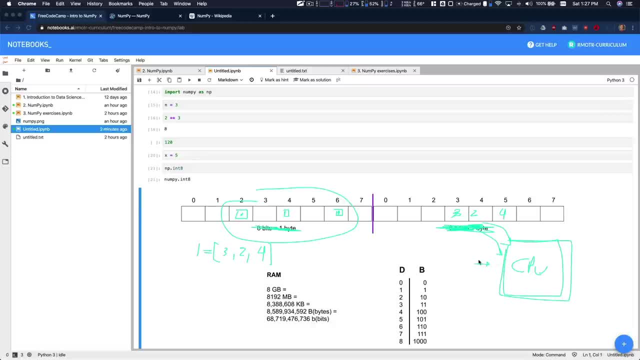 our CPU, which makes our computations a lot faster. So, again as a recap, you don't need to know all these to work with NumPy. That's a fact, First thing. second, you don't need to get extremely, extremely conscious about all the 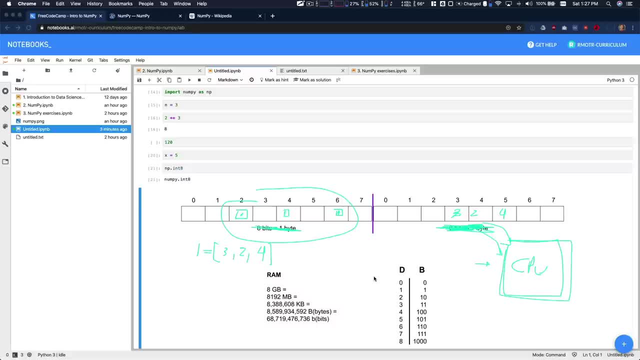 numbers you use At the beginning. you're just going to use NumPy as it is and you're going to use just the default types that it picks in 38. And- sorry, in 32,, in 64,. that's fine, But then with when you get into bottlenecks, when you're working with with larger amount, 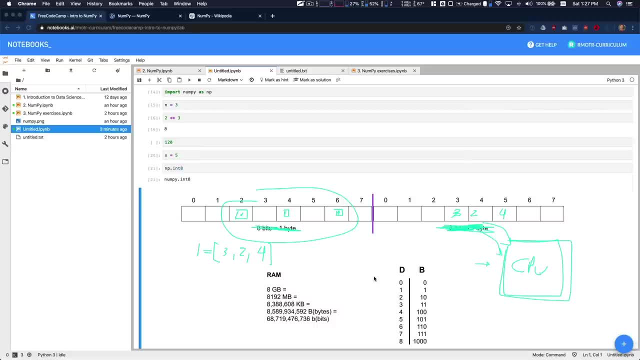 of with more amount of data, then you might need to get into the details of the size of the integers that you're using, And this all applies to floats. So I'm just using integers because it's simpler but is all applies to floats. 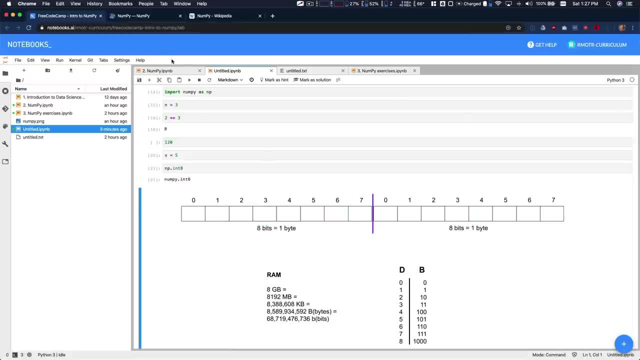 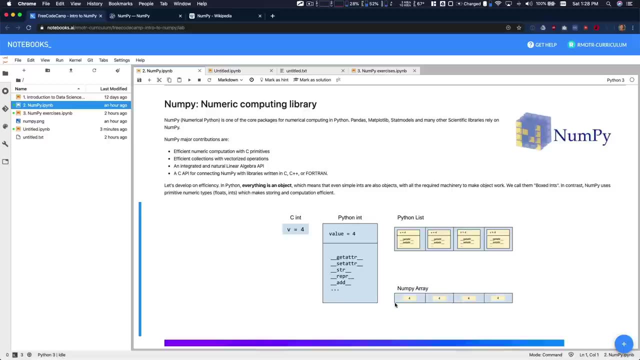 So again, NumPy, the main advantage is that it's it has built in very fast and arrays can take advantage of CPU instructions for matrices and arrays and all that, And then it also has a very efficient representations of numbers right, that are not the regular. 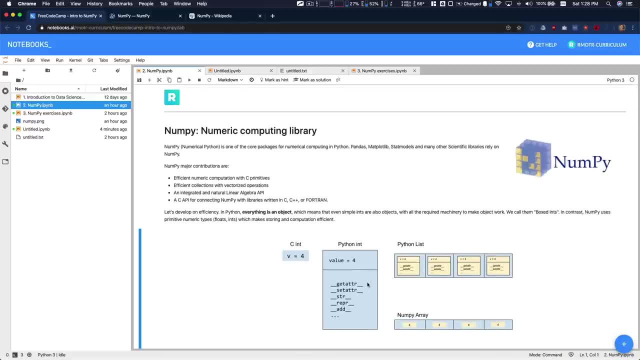 objects of Python. Again recap: you donate all this. if you want to get into more details, I recommend you to get a little bit more understanding about binary arithmetic and how numbers, or on computer architecture, how numbers are stored in memory, etc. especially for floats. 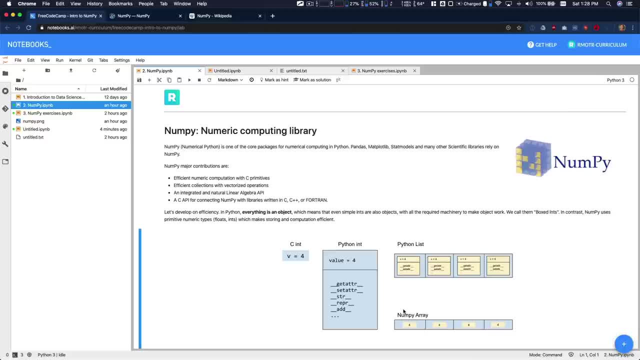 and all that's a completely different representation. So, with that said, we're going to see how we actually use NumPy without worrying so much about the low level details, And that's the beauty of NumPy. So we have already done our low level explanation of binary arithmetic. 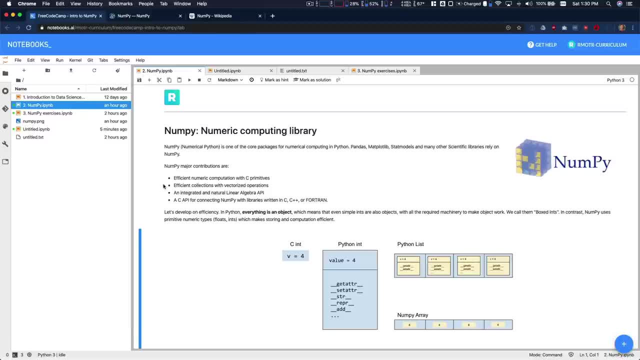 why are NumPy so important and all that? if you skipped it, that's perfectly fine. you will not need it. The reasoning was to include was that if you're in this tutorial, you're probably looking for fast and efficient options to process large volumes of data, And that's. 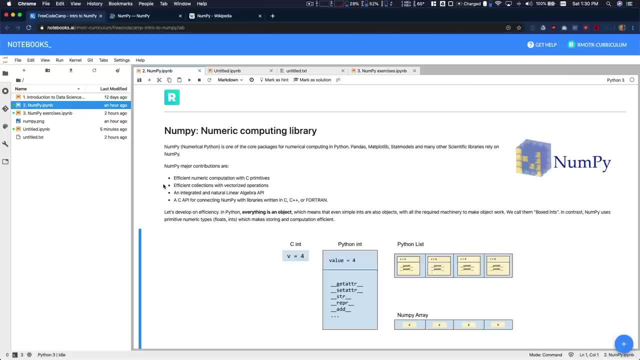 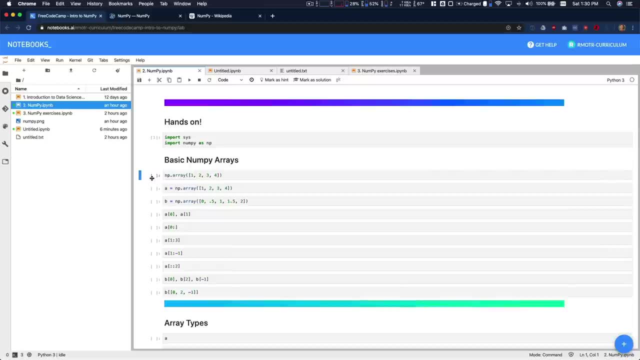 one All those things come into play. So let's, without further ado, let's just get started and start using NumPy as a library. So again, as I told you, NumPy is a very simple library for array processing and numeric processing. it has a few objects: numbers, floats, integer. 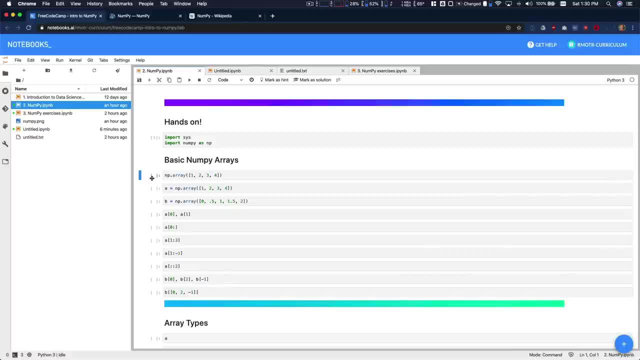 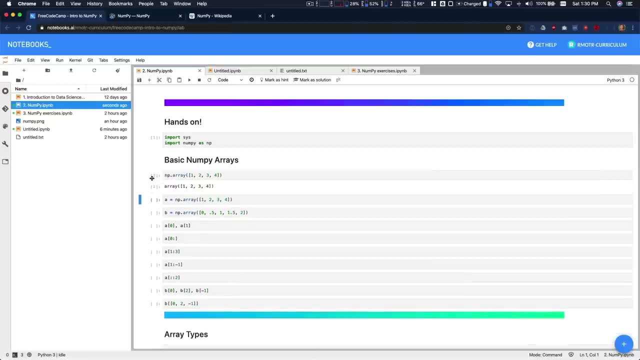 floats, arrays, and that's it, And it's very simple but it's extremely powerful. So in NumPy we're going to create these arrays which look a lot like Python lists, but they're going to be single significant differences. The first one is, of course, performance. If you go to the previous 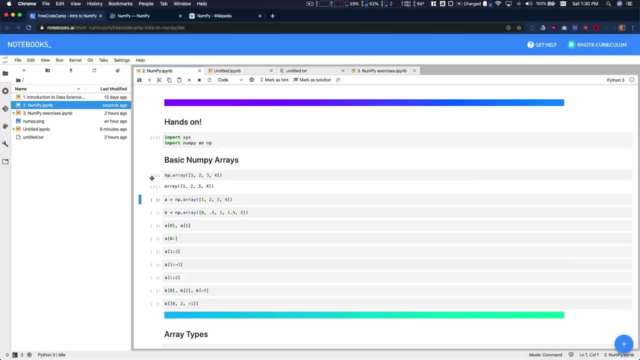 part, but we were discussing the binary representation of numbers in Python and NumPy. you're going to see the difference between them. So in this case we're creating two arrays And you will see right that the creation is extremely simple, The only thing that changes we need. 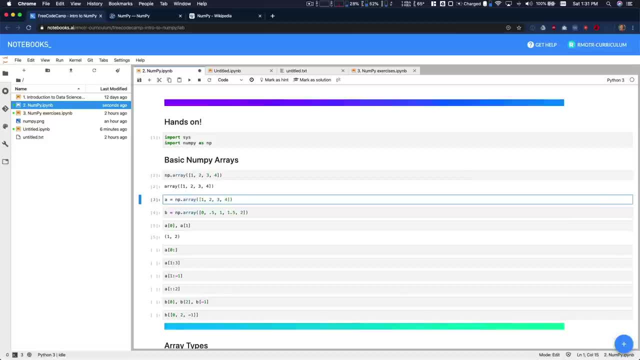 to add these mp dot array, and then we're passing, in this case, a list of numbers. This is something that we will usually be reading from external sources. Now, how can you access individual elements of a NumPy array? is this works in the same? 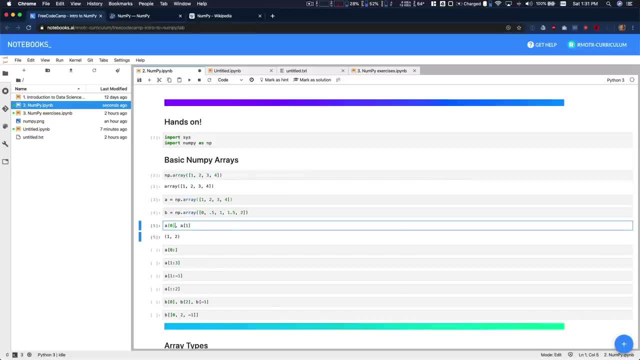 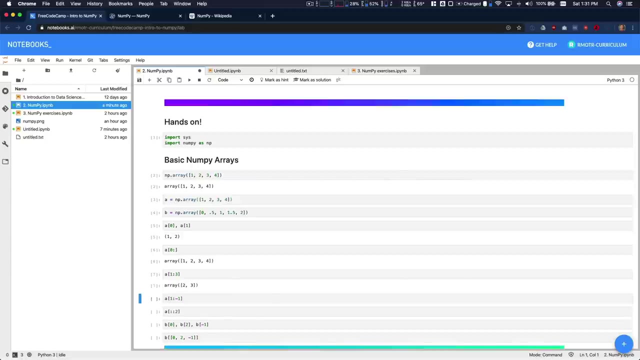 way as with a Python list, you can say: give me the first element, give me the second elements and it's zero. index, like again in a Python list. Slicing works in the same way. So in this case, up a zero to something, a one, up to three, right, just getting a low level. 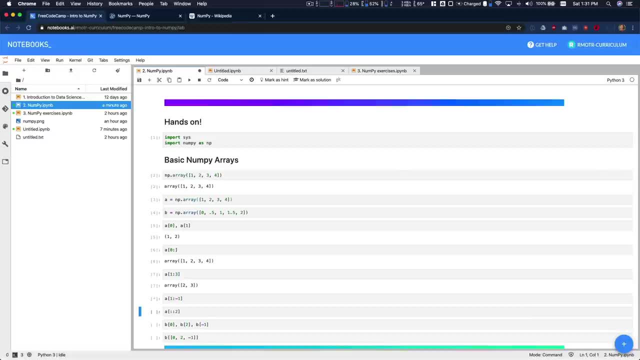 right and high level of the index. Okay, there's a negative indexing steps. they all work in the same way as with a Python list. So if you know how to use a Python list, you will know how to use a NumPy array There. 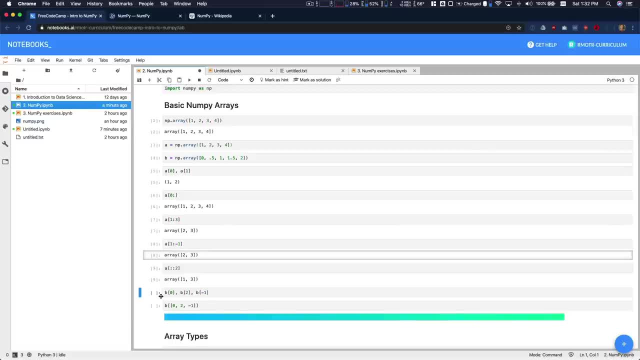 is one new thing right here's, differently from our Python list, And it's what it's called multi indexing. Let's say you have an array, this case B, and you need to extract three elements out of it. you need the elements out of it. you need the elements, the elements and things of that nature, And 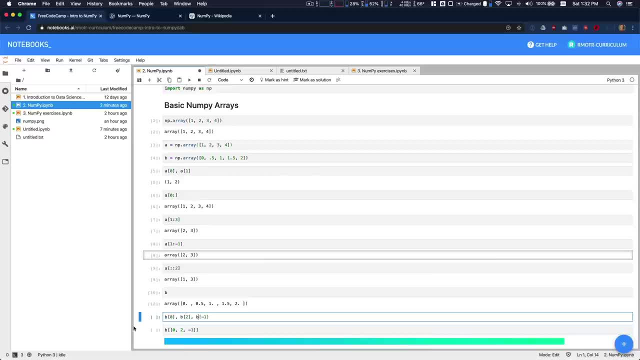 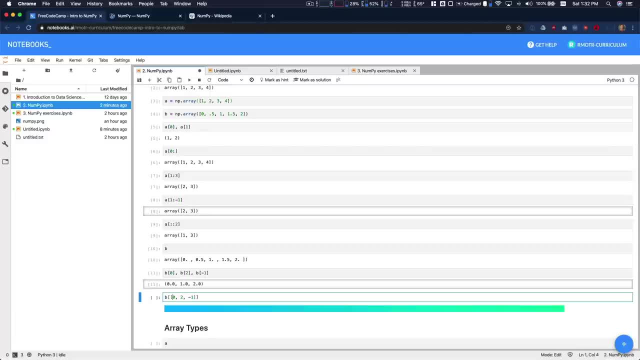 multi indexing, which is from B. I want to select the elements in zero, two and minus one: first element, third element and last element. right, so you pass it into another list containing the indices of the elements that you want to select And in this case, 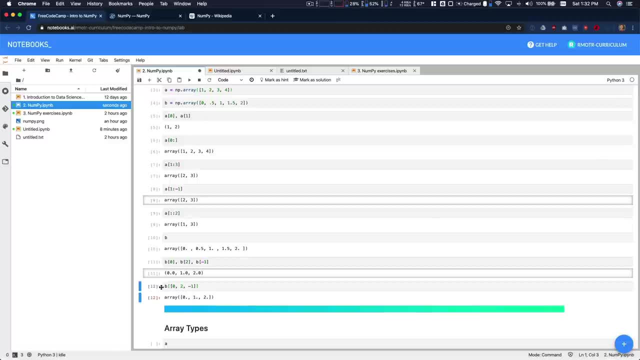 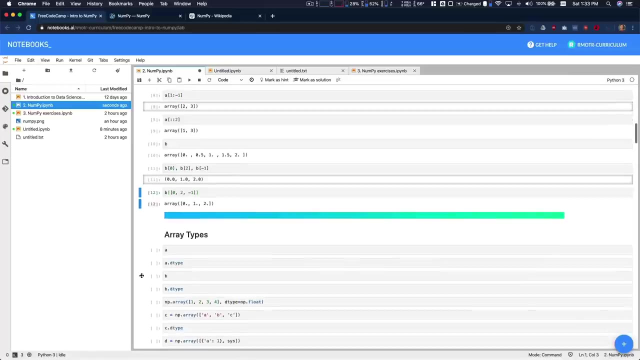 the important part is that the the result is another NumPy array. it's not just individual elements. you're creating another NumPy array which, again, if you're processing it's going to be a lot faster. So arrays have types associated And this is related to what we were speaking. 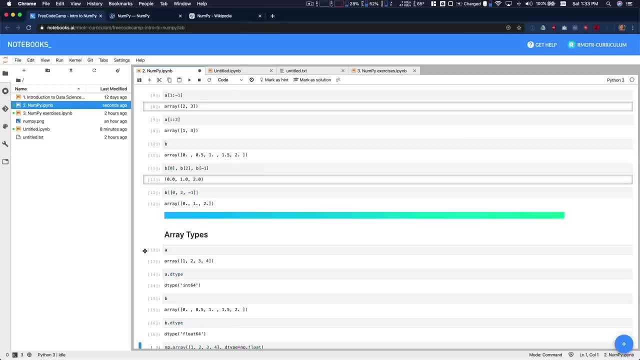 before. As a NumPy array is a continuous, is continuously assigned in memory. the NumPy library needs to know what's the type of the object you're storing. you can't just store you know anything- a string, a number- within it, because it will not be able to provide a performance and optimizations. 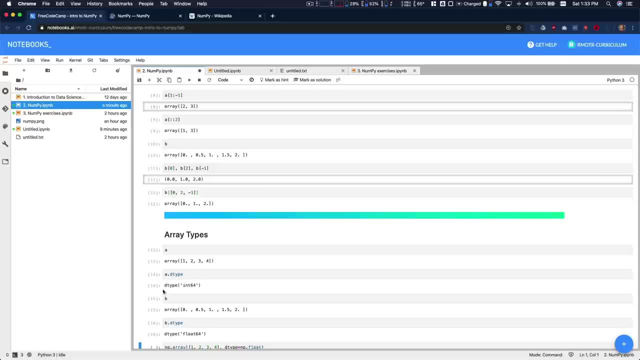 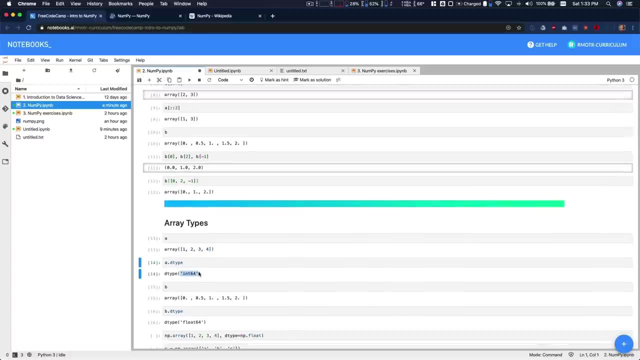 for arrays are not consistent in size. So, for example, when we create these array, only had integers By default NumPy selected in 64.. This is because of the platform. it's a 64 bit platform. you can tune this and you can select. as we're going to see other sizes in a sec When we 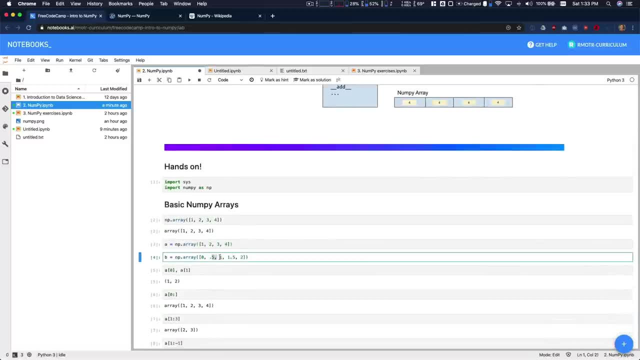 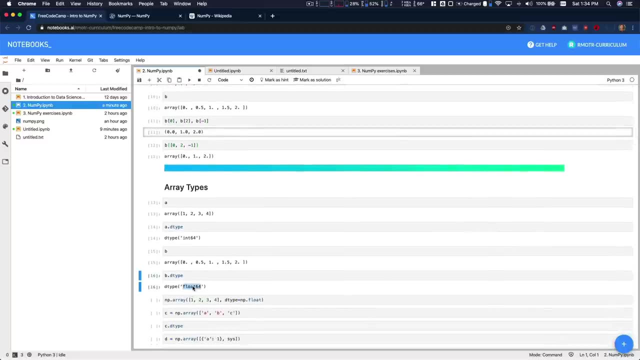 created the array B that contain decimals or floats. it assigned a different type, which is float 64. Again, the default type is always six, at least in this platform, that is 64 bit. it's going to be float 64. And in your 64.. 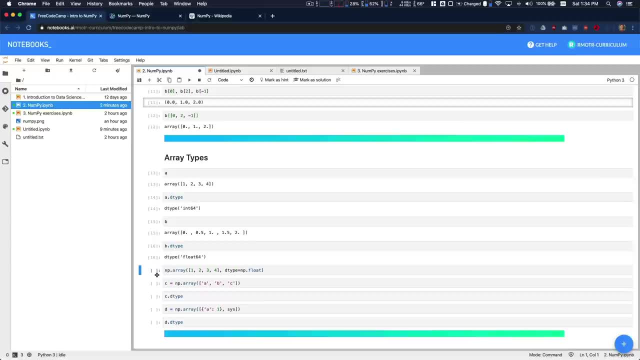 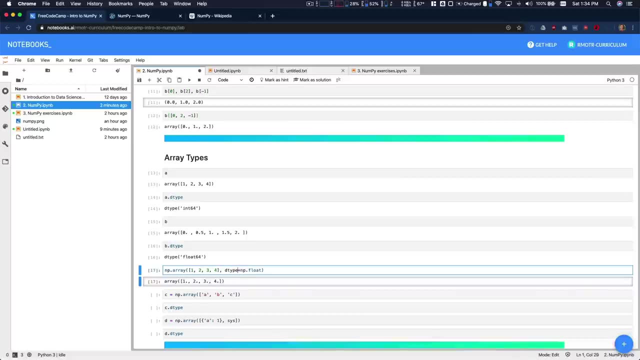 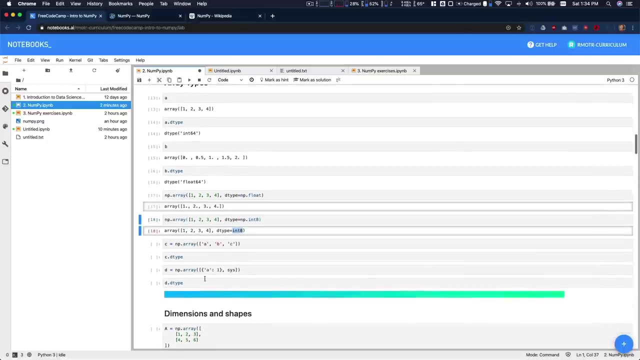 You can always change that. you can say: actually I want these. even though these are all integers, I want you to create them using a float type. or, as we saw in our previous video, we can say it should be actually type integer eight. so smaller integers for performance, for performance. 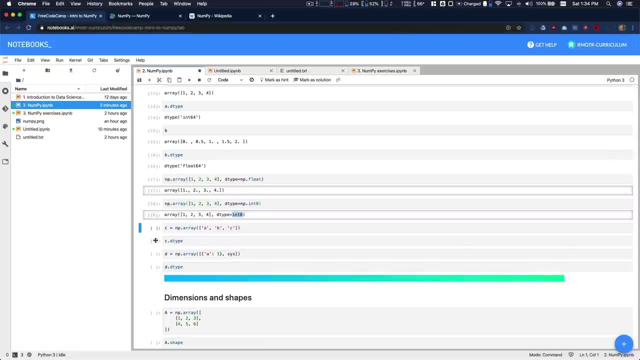 for better performance, sorry. So, moving forward, we were also going to see a few other types, like, for example, strings and regular objects, But as you're going to see this, there is no point of storing these things in NumPy. NumPy stores numbers, dates, booleans. 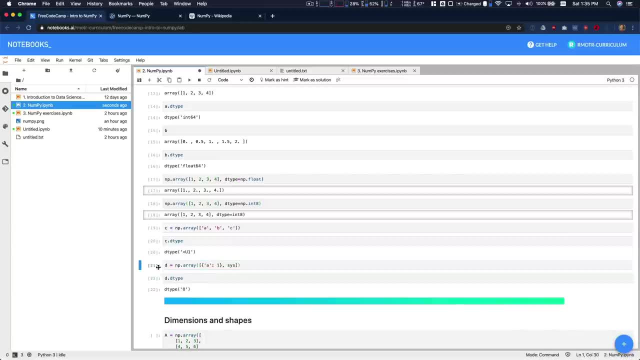 but not regular individual objects, as we're seeing right here. There is a way to store strings. it's perfectly valid and it has its own time, its own type, sorry- And it's related to the Unicode representation memory etc. 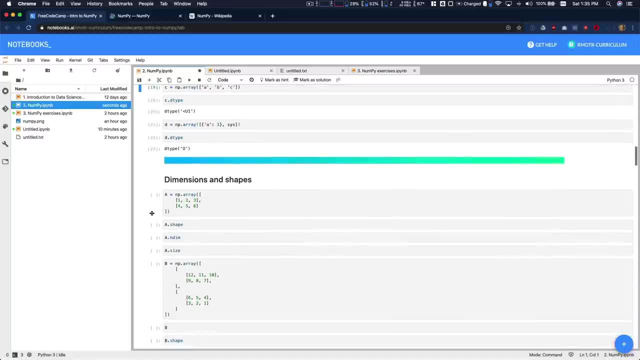 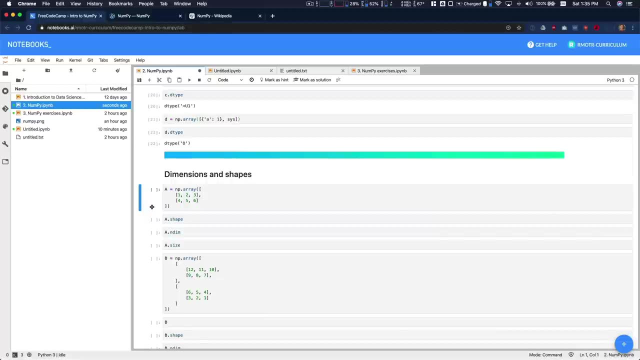 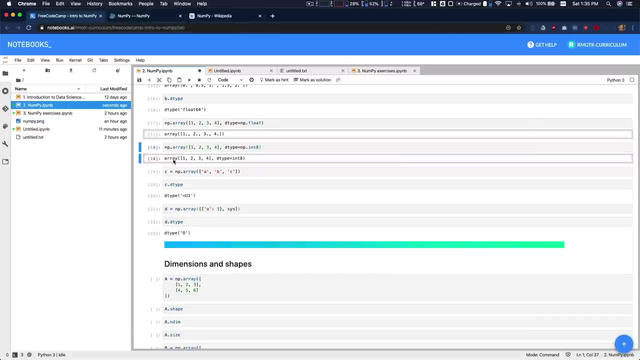 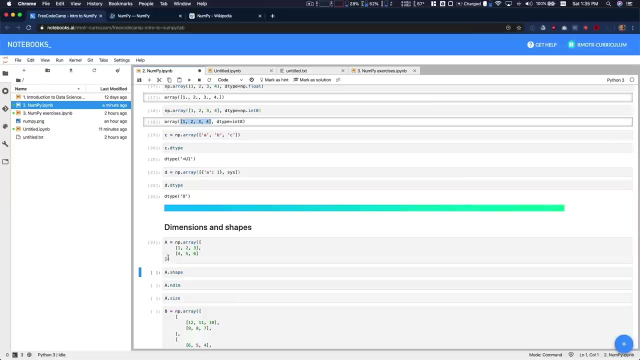 But again, NumPy is usually used for numeric processing. So the idea of NumPy is: we can create multi dimensional arrays. we can create the what we had created before. this is a one dimensional array, right, just one dimension. you can create matrices, which, in this case, 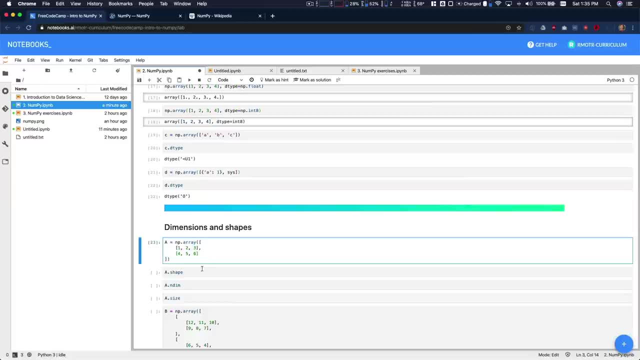 are two dimensional. we have two rows and three columns And NumPy. NumPy has a ton of attributes and functions to work with multi dimensional array. So the first thing we're going to see is the shape of an array which is two rows by three columns. 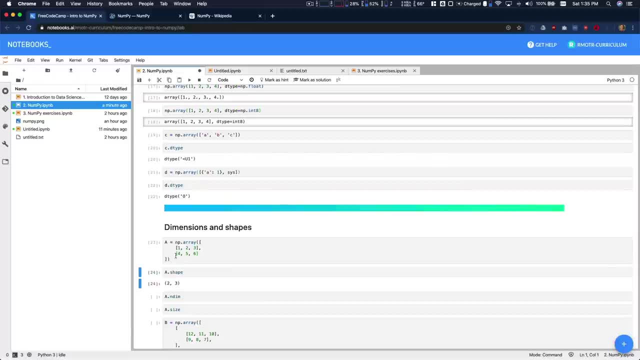 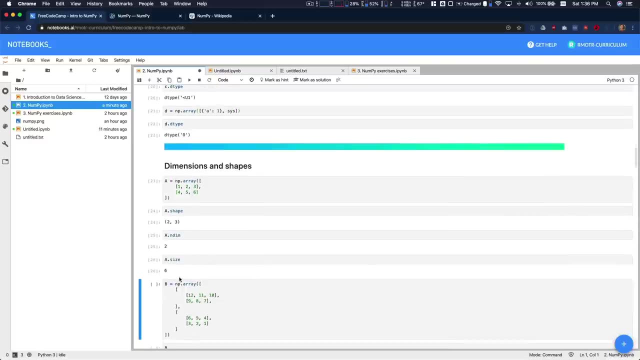 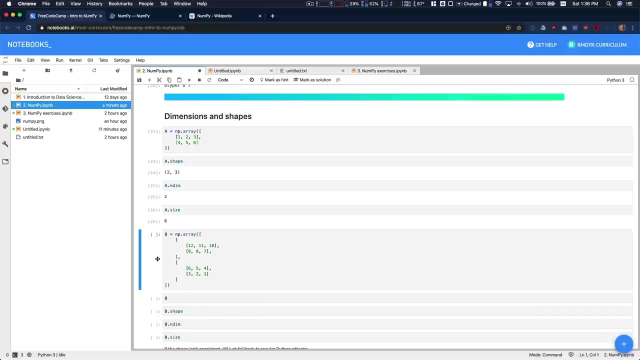 how many dimensions it has. it has one vertical and one horizontal. we have two dimensions And what's the total size of the array? In this case, the total size is six, the total number of elements we have. Let's go one dimension further. let's create a three dimensional. 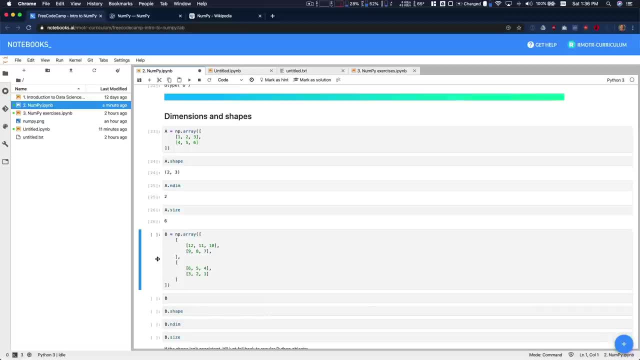 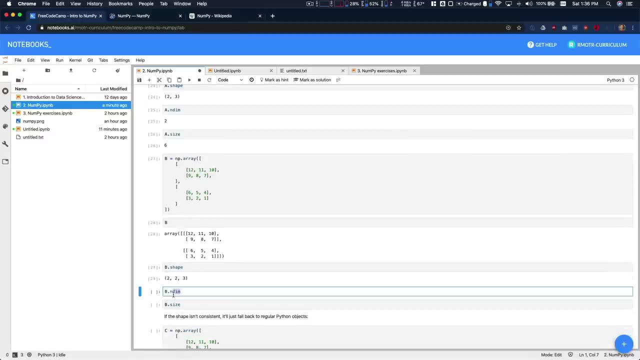 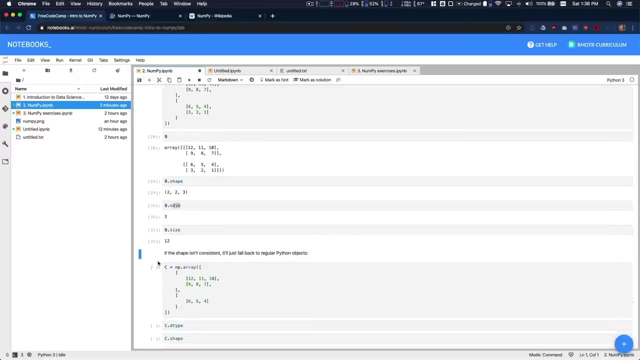 object: a three dimensional array which is basically a cube. In this case, for B, we have that the shape is two by two by three, the number of dimensions is three And the size is a total count of elements 12.. You always have to be careful when you're creating. 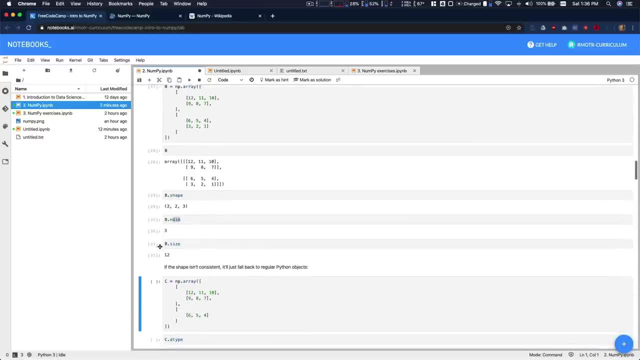 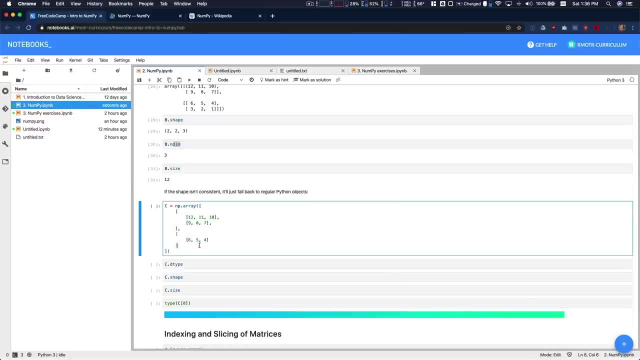 this multi, multi dimensional arrays. If the dimension, dimensions don't match, like in this case right here, where we have these second lists that only has one lesson in it- then the dimensions will not match And it will just take you, tell you sorry, that the array is of type object and the shape. 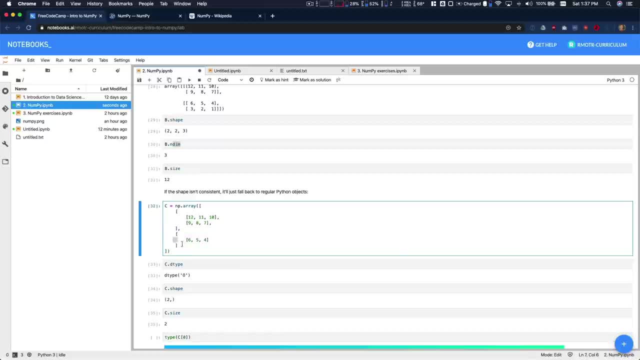 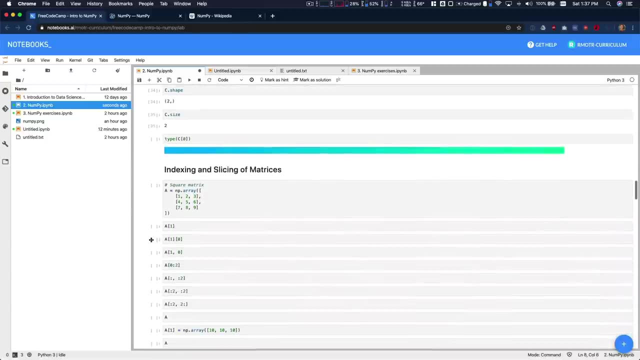 is only two, only has two elements: these one element and there's another limit. So in this case, we've done. we've done it wrong. basically, and you have to be careful when creating these, this objects by hand. So how can you index and slice matrices? we've done. 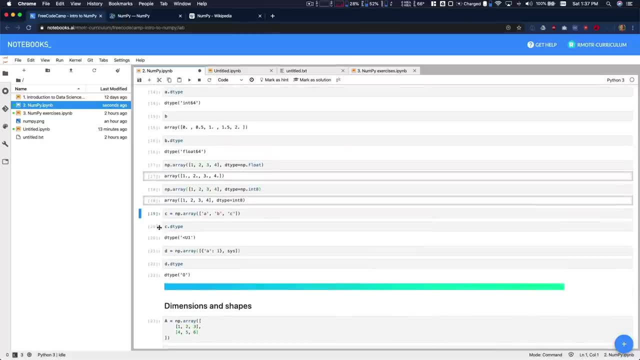 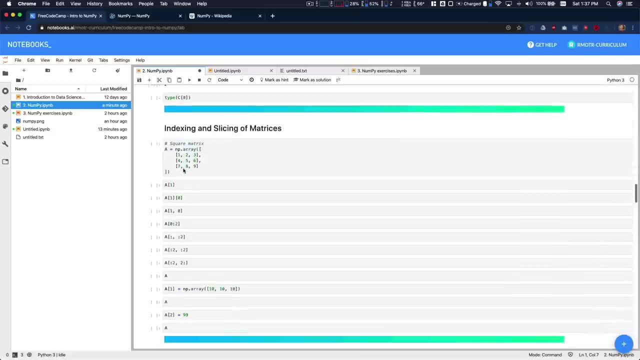 matrices. we've done it for a one dimensional array, So we were selecting elements, individual elements. give me the first element, give me the second element, etc. How can we do it with a matrix? With a matrix, what we're going to do is going to be very similar to 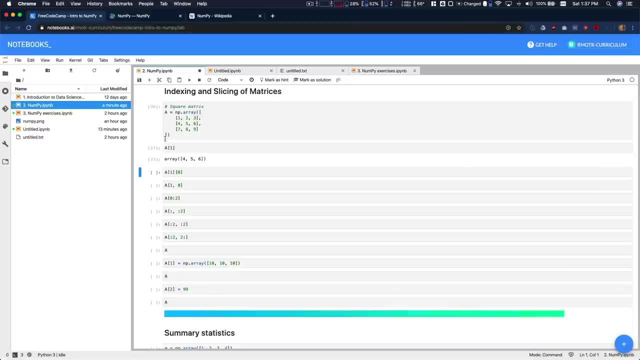 what we did before. The difference is that now we have to account for multiple dimensions. When I do give me a add one, is it the column at one or is it the row at one? Well, as you can see, it's the row. So this is going to be right here- 012.. Right, And there is also. 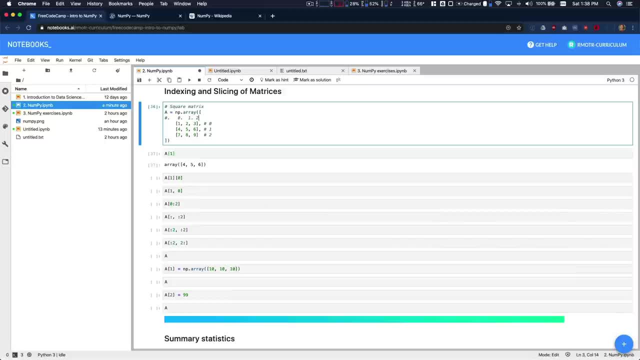 another dimension, right? So this is 012, in terms of index, index positions for our slicing. So here, how can you get the first element, the first element of the sequence? So here, how can you get the first element, the first element of the sequence? Well, let's. So here, how can you get the first element, the first element of the sequence? Well, here, how can you get the first element, the first element of the sequence? Well, here, how can you get the first element, the first element of the sequence? Well, in that. 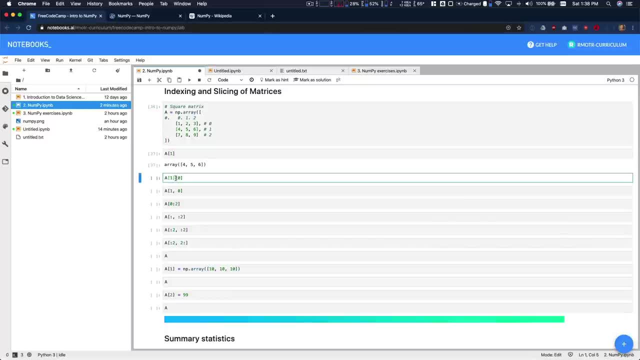 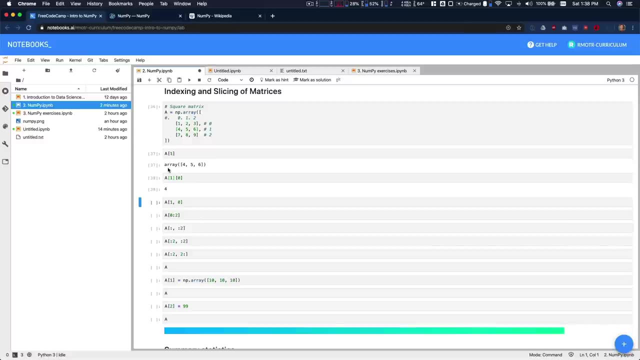 case, you're going to first select the first row- the sorry- the second row- and then select the first element, And that's what you get, number four. But there is a better way, which is by using the multi dimensional selection of NumPy. In this case, you're going to say: 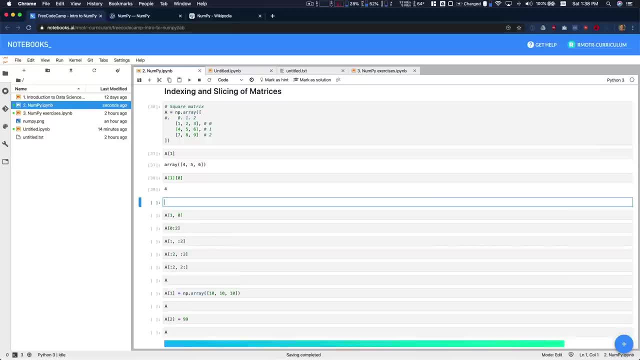 from this matrix, I want to select, and here you're going to pass a, in this case you're going to pass dimension one, dimension two, dimension three, dimension four, etc. And these are selectors for each one of those dimensions that you're passing, In this case. 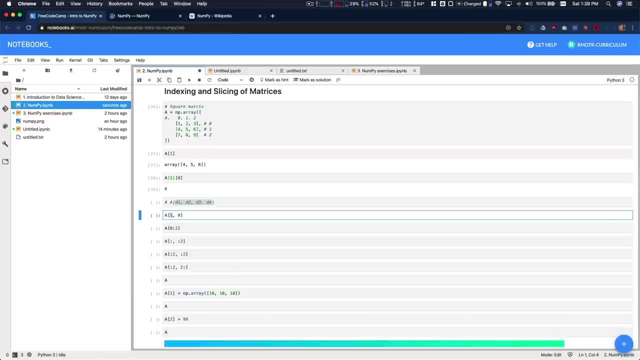 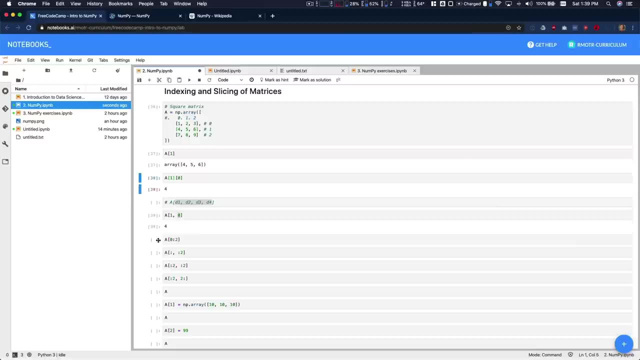 we say, for row level, one the element of position, one second element and for column level, we want the first element in it And it's the same thing as we did before. The advantage of this syntax and keeping in mind and reminding it, is that it will also let you add slicing. 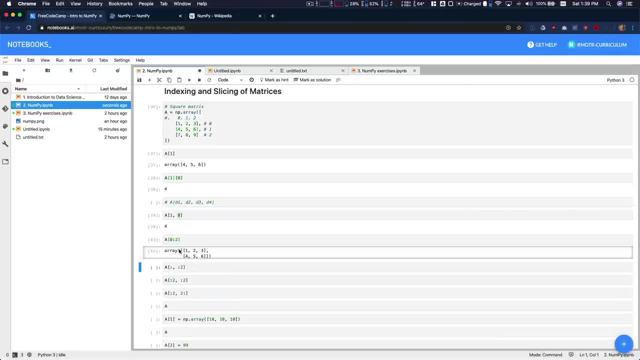 right. So you'd say: I want to select everything from dimensions: dimension one, which is rows, So in this case you say: from zero up to two, is these two ones, the two is not included. upper limit: the same as as Python, And then you can also. 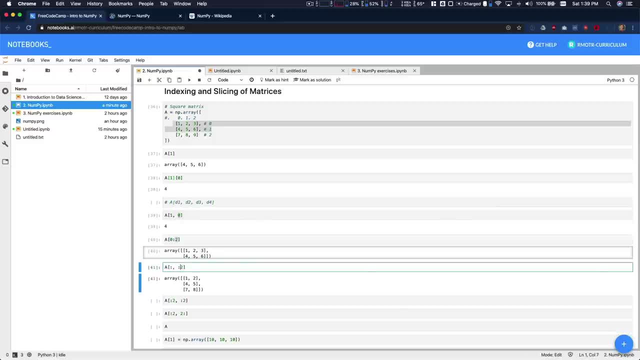 pass other other dimensions. you say I want to select every row. that's fine, But then I want to select from column level. I only want to select the elements up to two. So these two and these two and these two, right. 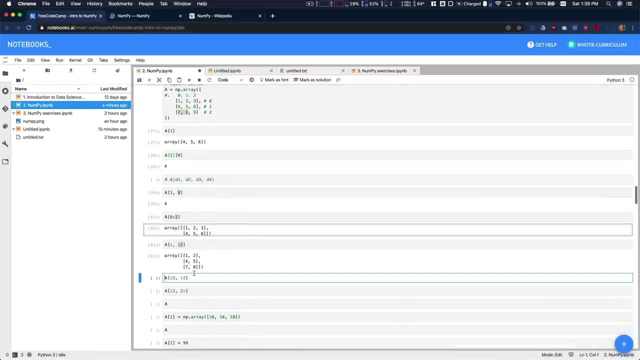 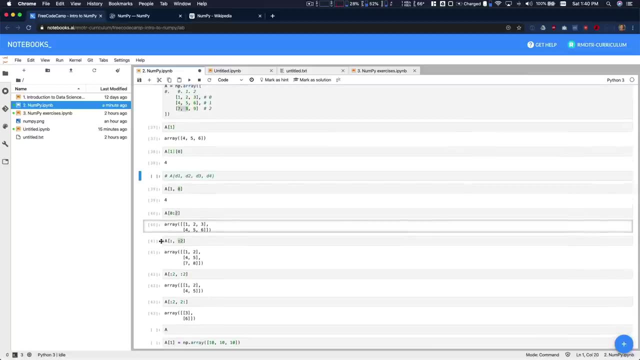 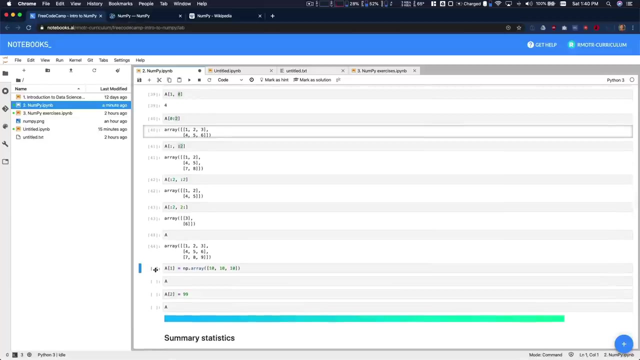 So one, two, four, five, seven, eight, These all works as intuitive as it gets. Remember: this syntax is the important that you need to keep in mind Moving forward for modification. you can say: I want to assign this new array to this entire row, right? So if the dimensions 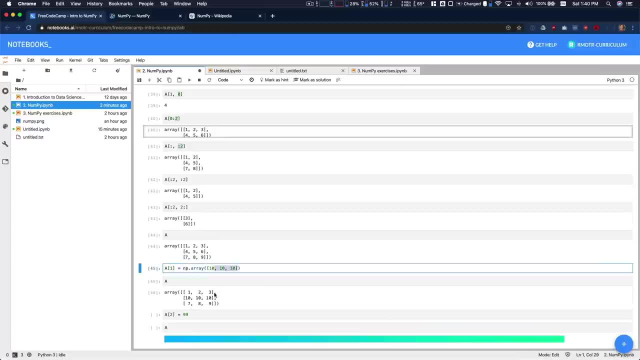 match. that's just going to work. Now, 10 is equals- it's added to the second row, or 10.. Or you can just use what we call usually an expand operation, which is going to say: for row number two, I want to assign the number 99. And NumPy is going to take care of expanding. 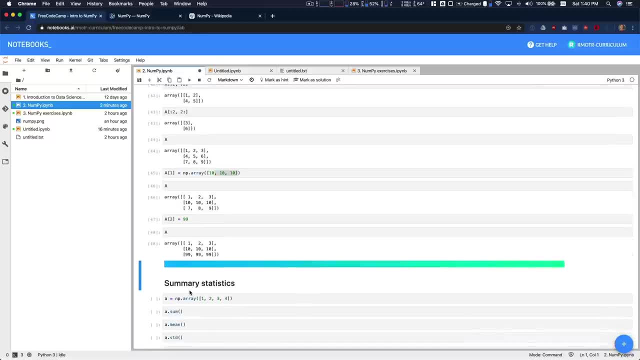 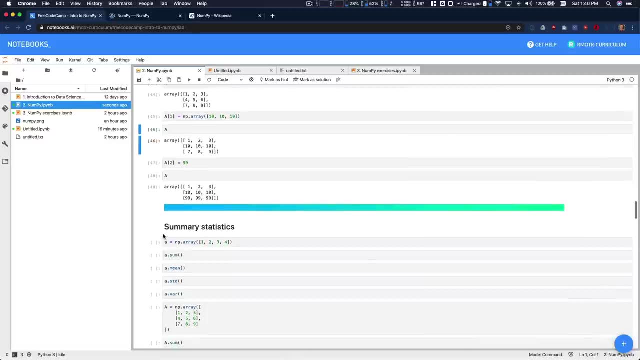 it into this corresponding array, given the number of dimensions that you have. So so far that selection. it's simple. we're going to see also is that NumPy has a huge advantage of containing a ton of operations you can perform. 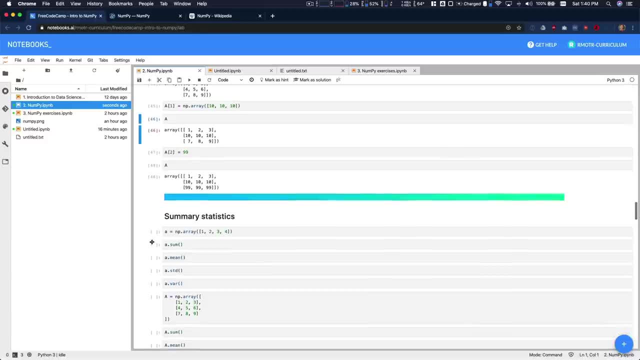 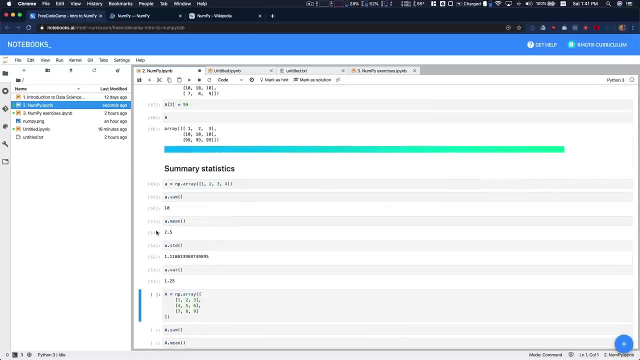 On top of your raise, your matrices, your multiple dimensional arrays in general. So the first one is the oldest summer statistic methods we have. So given an array. all these methods are already built in: the sum: the mean, average, right, standard deviation, variance, etc. 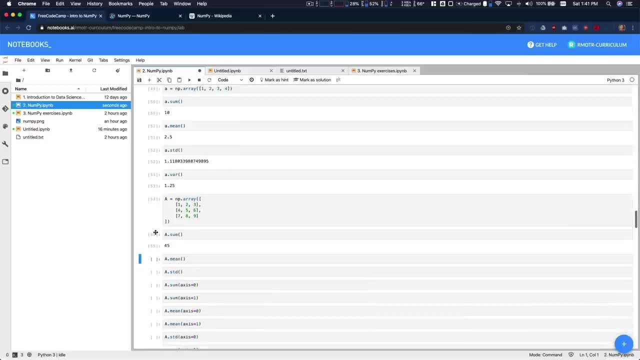 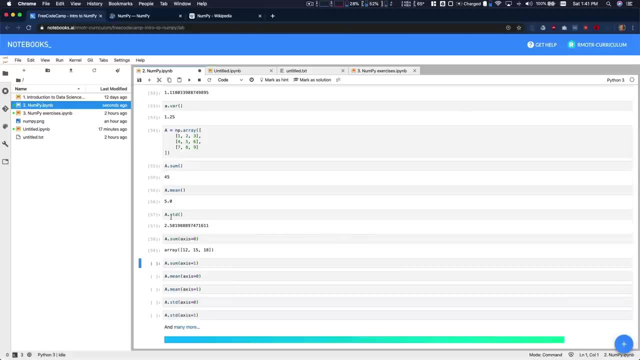 And that also works for matrices. So in this case we can get the sum, the mean standard deviation, or we can do it per axis. So this is very useful. we can get the the here. let's compare these two. there we go. we can get the sum of these. what is this? first column? 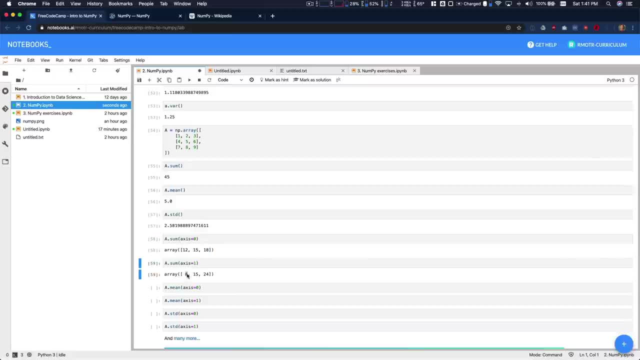 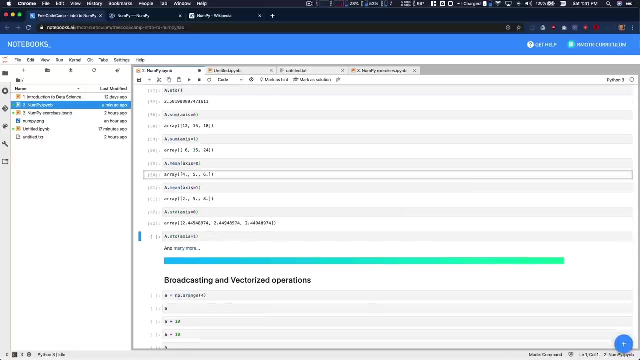 the second column or the third column. we can get it the first row, second row and the third row. So it's either this dimension, this dimension one, or it's a vertical dimension which is access equals one right. So per row, per column, or, if you have more dimensions, 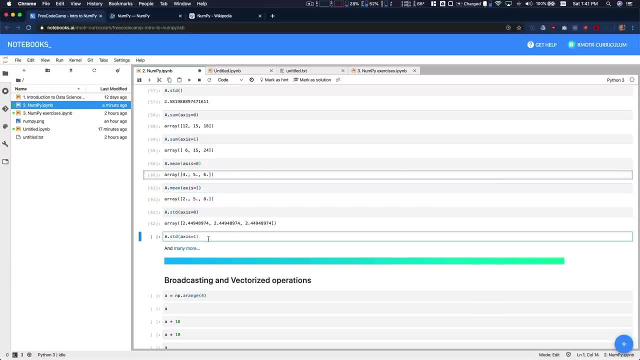 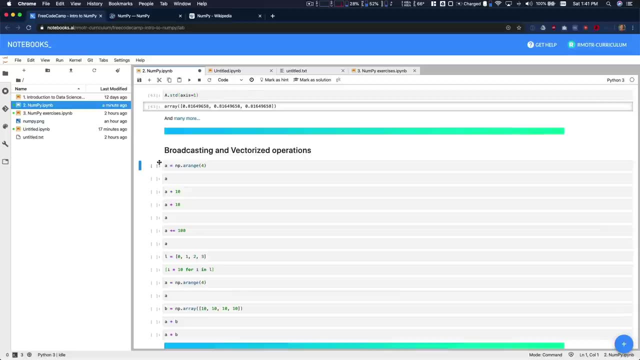 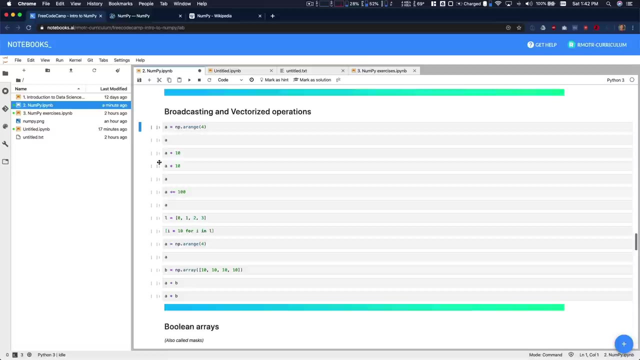 you can just keep increasing the number of this axis And that's just going to work as expected. Broadcasting a vectorized operations: this is a fundamental topic that we're going to talk about And it's going to be extremely related to Boolean arrays. These are a few new things that you have to keep in mind. we're working with number. 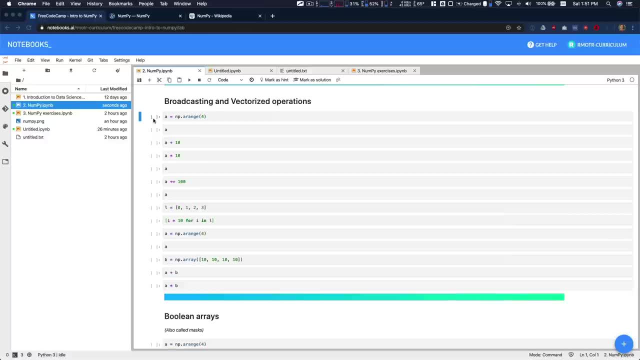 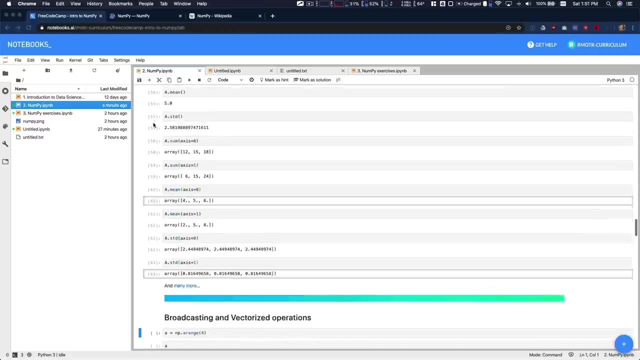 And now we're going to talk about vectorized operations and broadcasting, which can be a kind of intuitive topic at the beginning, but then you're going to understand how much sense it makes. It's one of the fundamental pieces of NumPy. we've seen how NumPy works In a very general way. we saw the multi dimensional 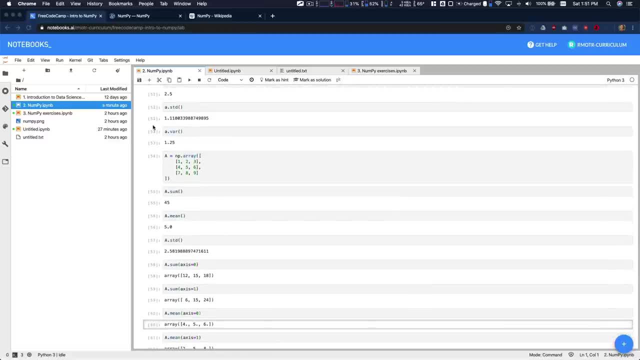 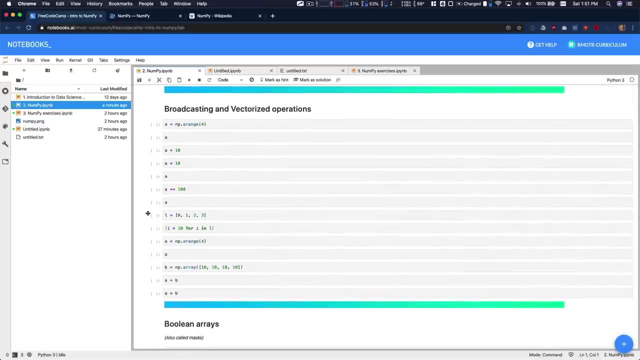 arrays and all those advantages. But you might be thinking, I mean, I don't need another library just to compute the sum or the mean, when I show you the vectorized operations, the broadcasting part. this is going to make a little bit more sense of why NumPy is so. 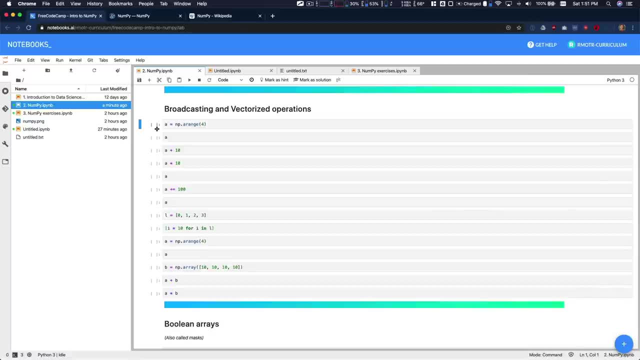 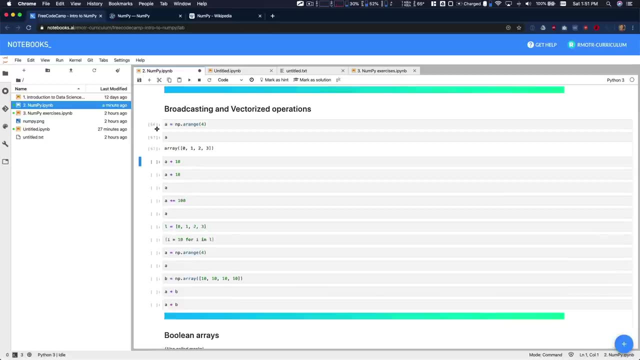 important. So, to get started, we're going to have this array, which is a right. that's just very simple array. vectorized operations are operations perform between both arrays and arrays, and arrays and scalars, like in this case right here, which are extremely fast. they're optimized to be extremely fast In. 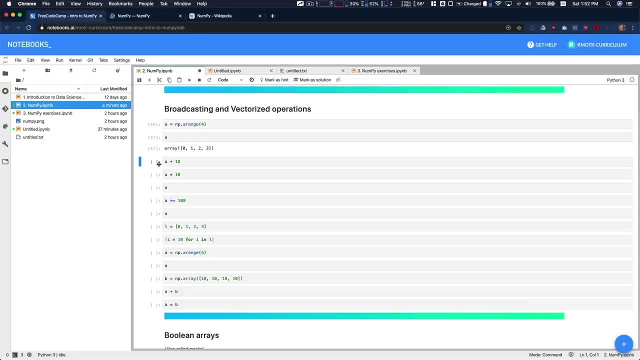 this case, what we're going to do is we're going to sum the entire array plus 10.. And what it means- we're going to see an example of what happens with that, with Python. But what it means is that let me show you the result that each one of the elements within 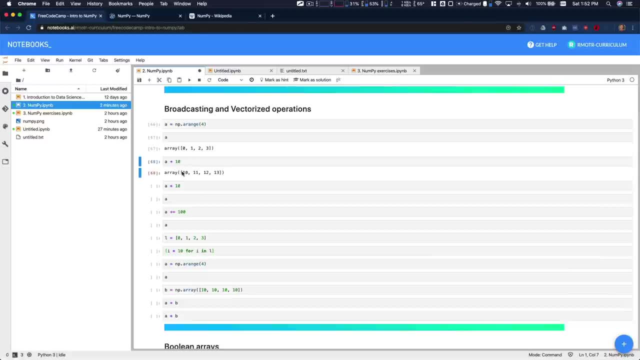 the array will be applied, this operation. So usually that's the concept of vectorizing an operation: you have the number and then this operation is applied to each one of the elements in here, or actually in these other one, right. so here and here and here and here, to result in this new array, the operation. 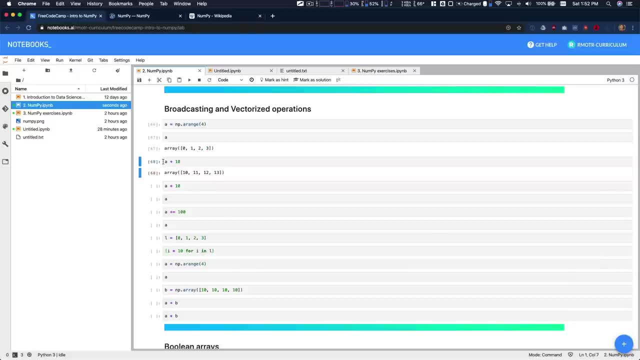 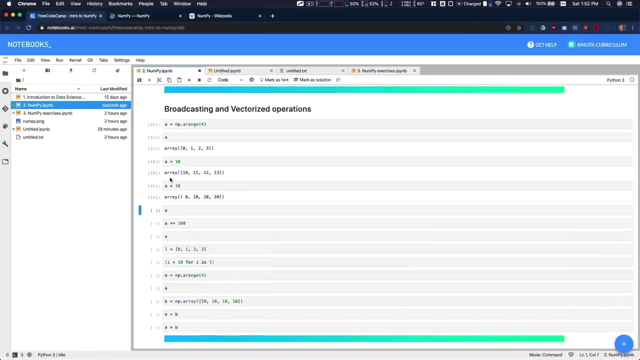 is expressed at an array level. right, we say a plus 10, that's it. But then again, internally, this is broadcasted to each one of the individual elements within the array. So in this case we have a plus 10, about eight times 10,, for example, which also it's. 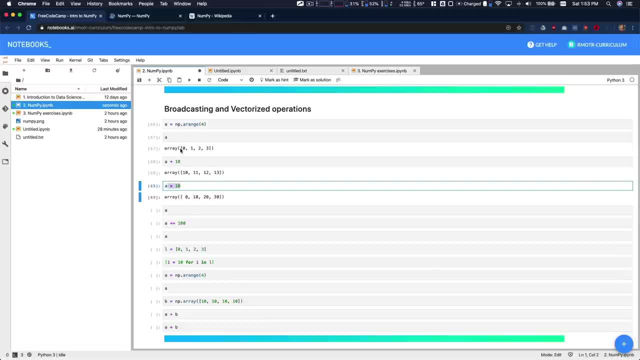 in this case is we're applying the times 10 operations to each one of the elements in the array, resulting in a new array with the result of that operation And these resulting in a new array is very important because, as we're going to see, NumPy is an immutable. 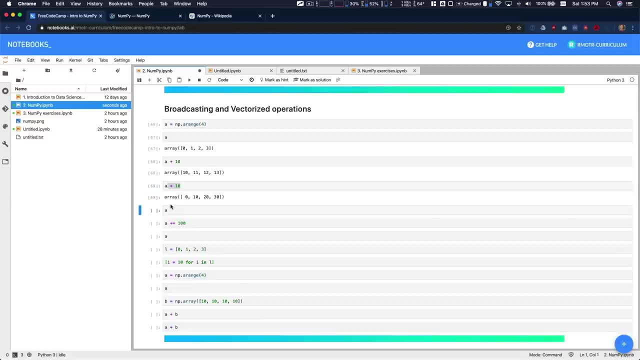 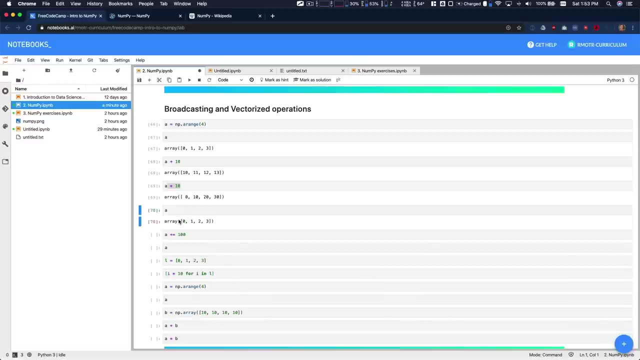 first library. it will not. any operation you perform in an array will not modify it, but it will return a new array. if we check the status of a, you're going to see that the elements are the same. it has never changed. we are creating a new array and returning it. there are ways to override. 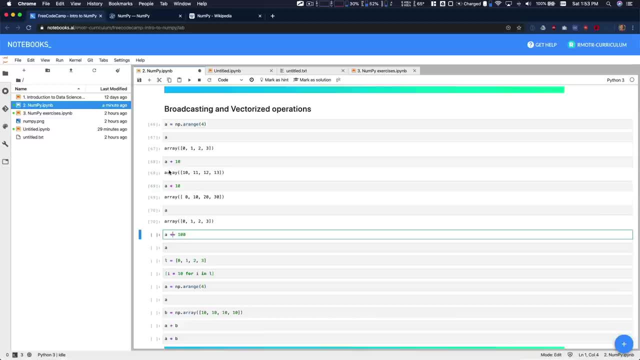 this behavior. if you want, And the all these operations were performing this way, also have the interface of plus equals, minus equals, times equals, etc. which will indeed modify their rights. So in this case, we're making a broadcasting operation, adding 100 to each one of the elements. 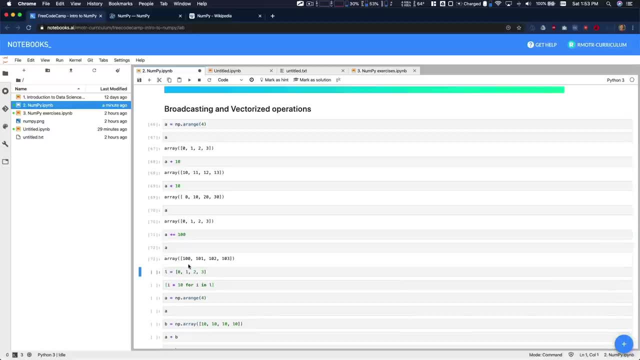 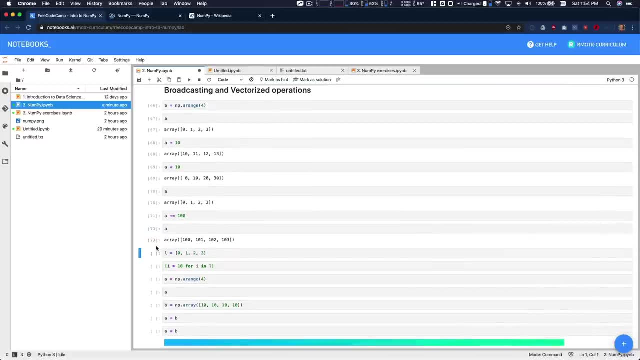 in this array And now this operation was immutable. a was modified and did it hasn't returned a new operation. If you remember from your pure Python skills right, The correspondence of vectorized operations are less comprehensions in which you're expressing an operation for. 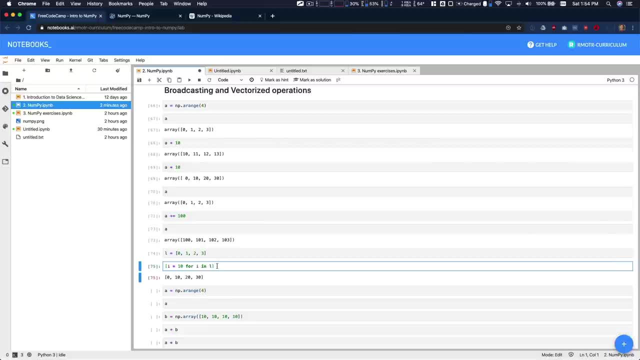 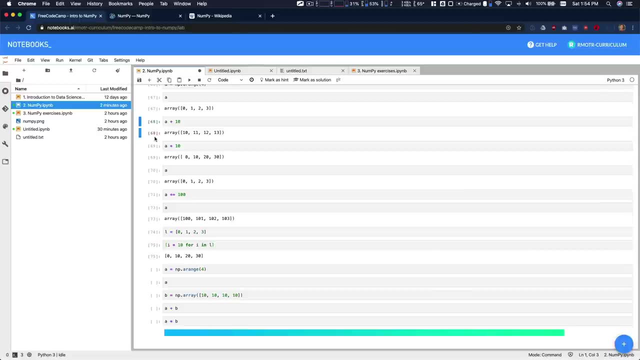 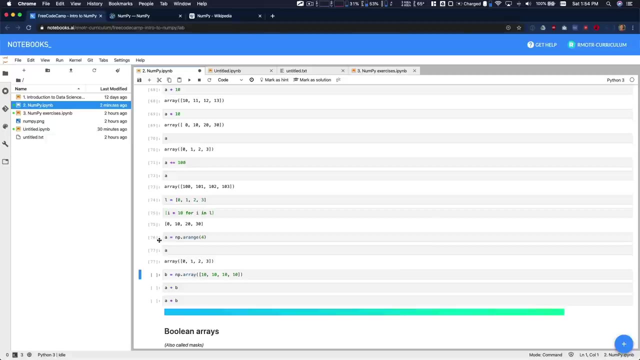 each one of the elements in your collection, right, So that's a less comprehension. It's a. it's pretty similar to what we're doing with NumPy, The main difference that this is all optimized and extreme. it's extremely fast, So the operations are these. vectorized operations are reduced, broadcasting doesn't. 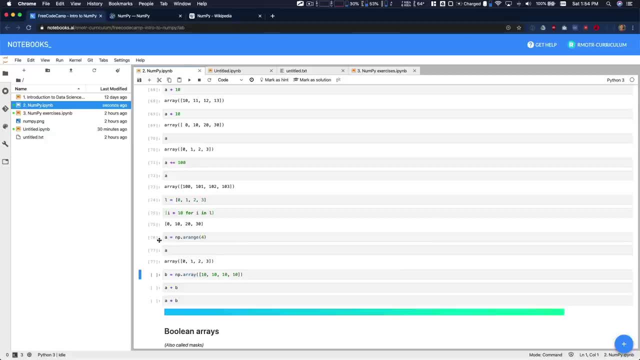 need to be only between arrays, and scalars can only be between arrays and arrays. So in this case we have a and we have B. I'm showing you right here we can do something like a plus B, And what you're saying is that if there is a number of arrays and you're 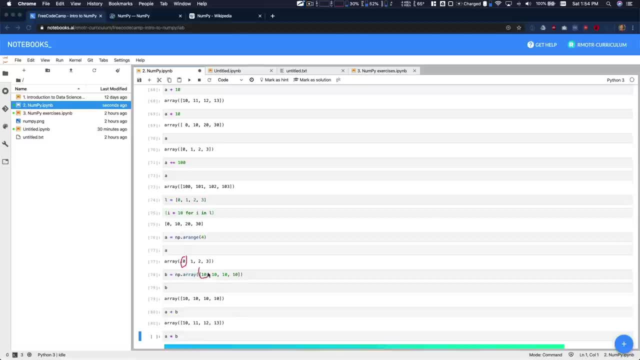 saying: there's a correspondence, right. so zero plus 10,, one plus 10,, two plus 10,, right, Let me. let me do it in this way: 110,, 210, and 310.. There you go, And that's the result. 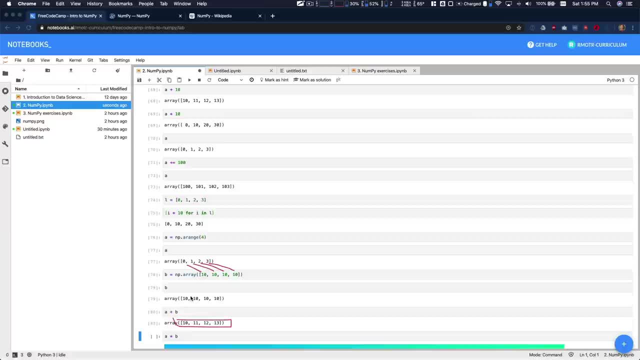 that we get right here. So this: for this to work, you of course need the arrays to be aligned and to have the same shape, But when that does work, then the operation is extremely fast in memory And it's aligned. it's a vectorized operations. 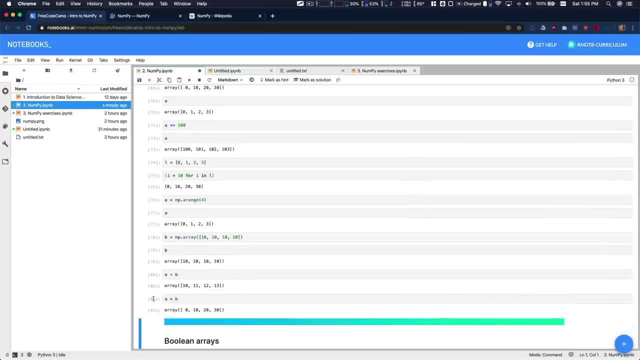 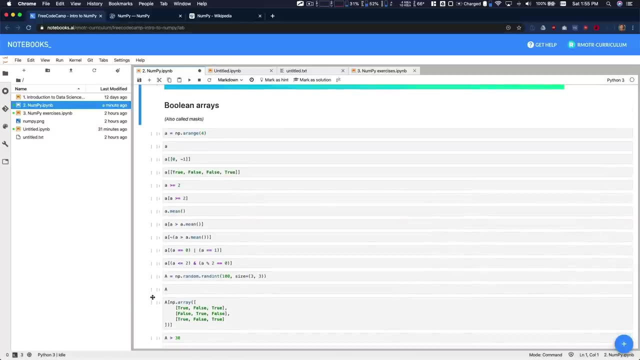 with seeing so far. why is this topic of vectorized operations so important? Well, because of the following, which is pulling arrays, And this is a very, very, very important thing. If you don't completely get it now, I ask you please to go and check the exercises we. 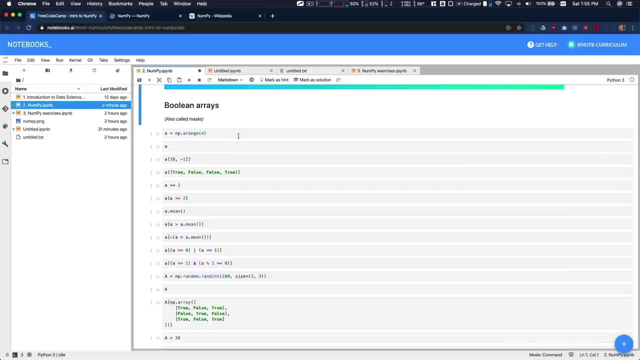 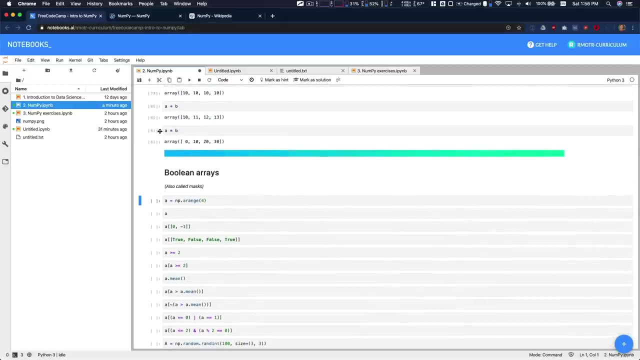 have for this lesson, because we're going to use it a ton, And we're gonna. we're gonna see that in pandas, the same syntax, the same primitives of Boolean arrays apply, apply and we're going to use the same things. So why are Boolean arrays similar to vectorized operations? Well, 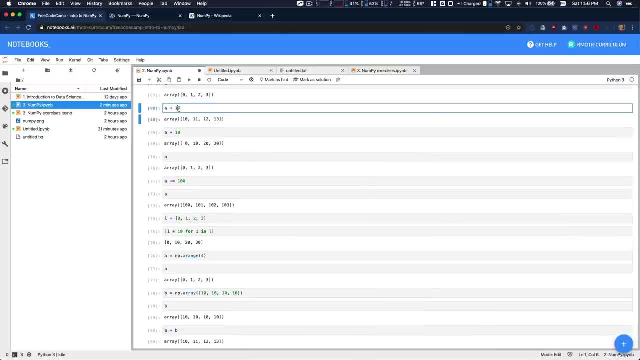 all these operations we've had performed here are just arithmetic operations, mathematical operations: plus something, times something, etc. If you look at the operators that you have in your programming language, it's it's not only mathematical operators like plus or minus or times, you also have Boolean operators. And the question now it's going to be what? 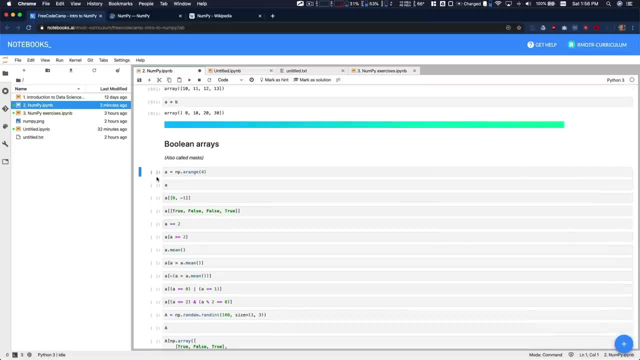 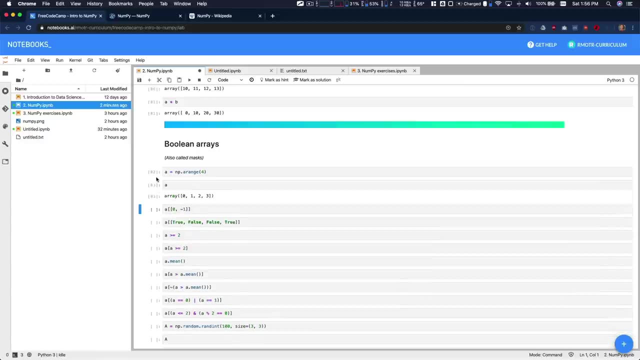 happens when you apply Boolean operations, when you apply Boolean operators to it. So, given our array, we had what ways we had to select different numbers. For example, in this case we need the first and last element. we do zero and minus one, That's. that's the 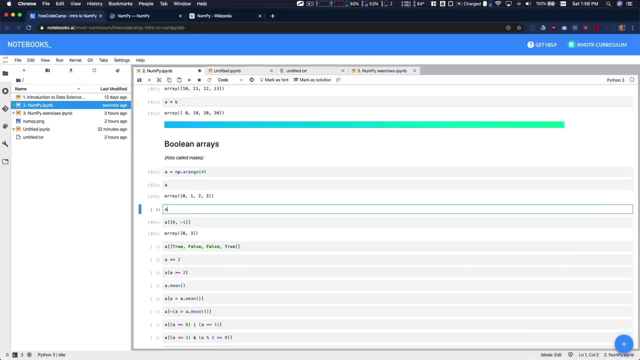 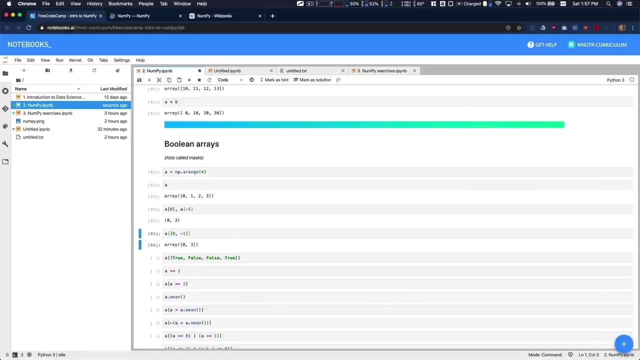 way we saw with an umpire. we also saw the traditional Python, one right. So as we can say a zero and also want to get a, I'm at minus one. So this is the first, the first way of selecting these elements. we know there's a second way with multi index selection. 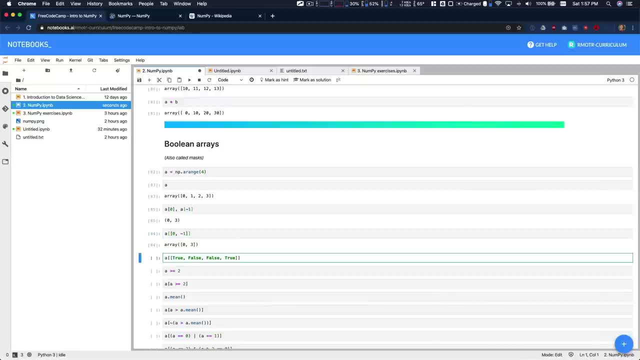 And there is a third way- And this is new- which is with Boolean arrays right here. So in this case we're going to say: I want to select the elements in this order, right, and you're going to pass either true or false if you want to actually select the element. 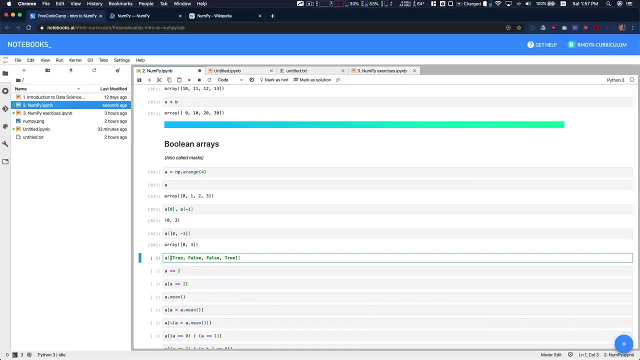 or not Right? So if you have four elements, you have to pass for Boolean values saying I want to select this element, I don't want to select these one element, I don't want to select this element And I do want to select this on right here. So I want the first one. on. 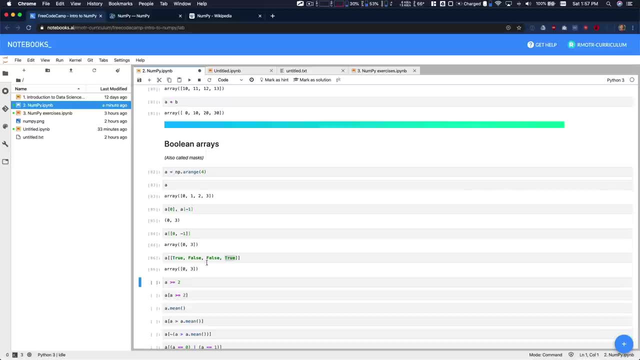 the last one, and the result will be the same: 030303.. So so far it's it's nothing terribly new, right? So this is new, but it's not extremely complicated. we are showing you a brand new way of selecting data. you can select regular Python. 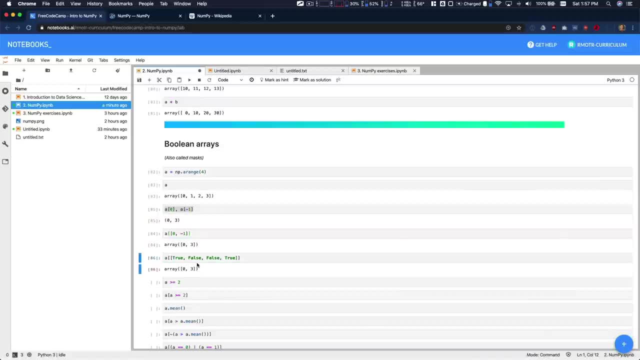 multi index or a Boolean array? Now you might be thinking: will I manually write true, false, false, true, true, false? for I don't know how many records. you have a million records. this is not scalable, right? You will not say to write all these true or falses. But 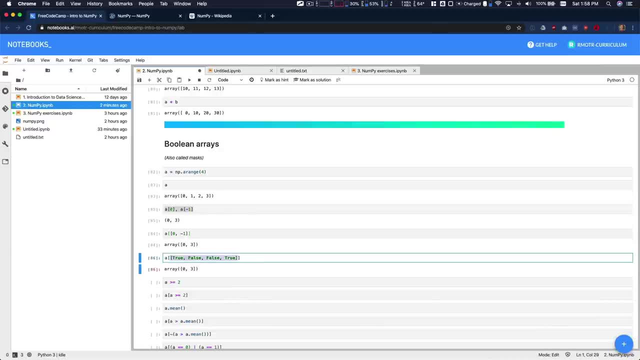 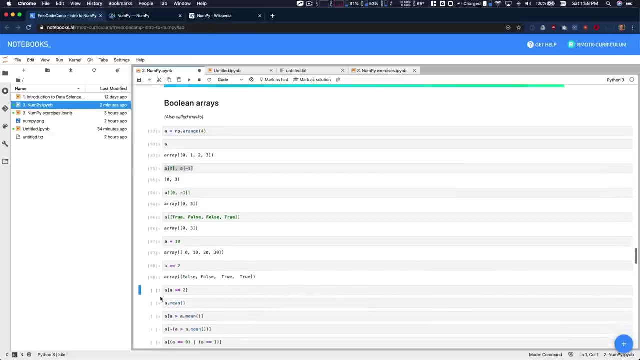 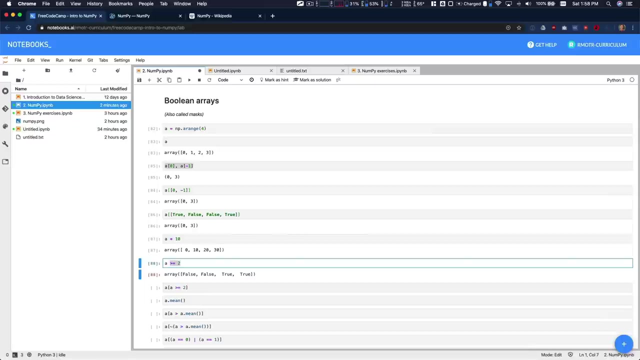 this is actually very important, Because these arrays are the ones are the result of broadcasting Boolean operations. So, again, regular arithmetic operation like this, But we also have it for Boolean operation. So what happens if we ask a greater than or equals to the number two right an array? 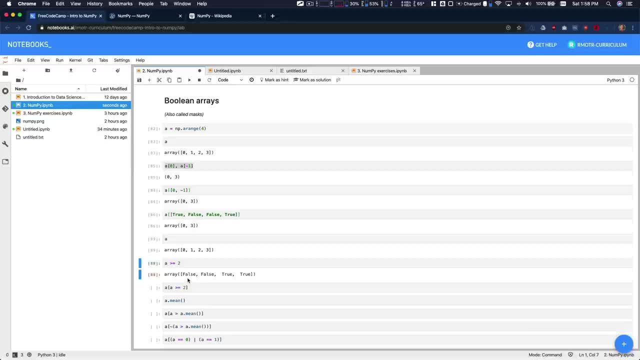 a. is this right? here is your 123,. then the result is false for zero, false for one, because they are not greater or equal to two, True for number two. True for number two, of course, and true for number three. So all the individual elements. 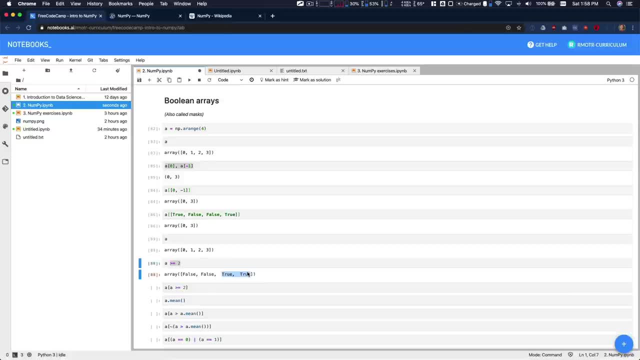 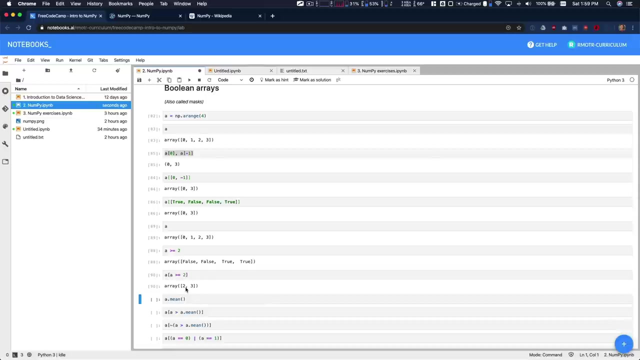 that match. this condition will have true and false in other cases. This is the power of Boolean arrays. we will be able now to combine these operations. So now we can do a greater than or equals to two right there. a equals a being greater than or equals to two. So 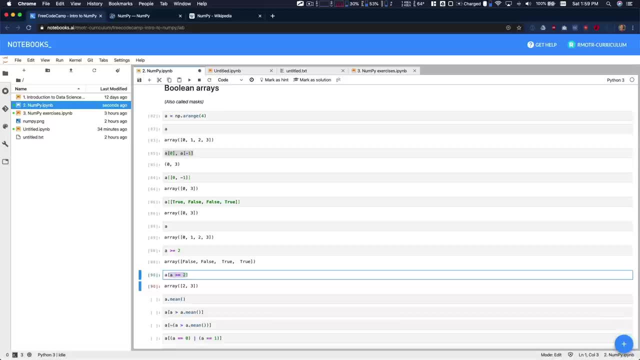 we're saying greater than or equals to the number two. The advantage of this is just filtering. we're filtering num, num, numeric arrays very quickly with a very familiar syntax: a greater than equals to two And we just provide that as the index of the operation. 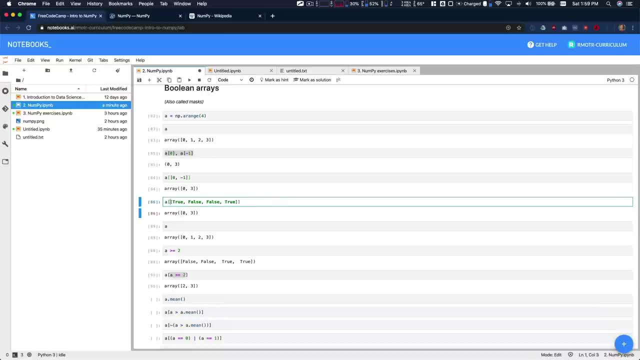 It's pretty much what is happening right here. We're saying: use this Boolean array. It's a Boolean list. right, There's a Python list with Booleans To filter or, sorry, to select elements based on that. But the question is: how do we construct? 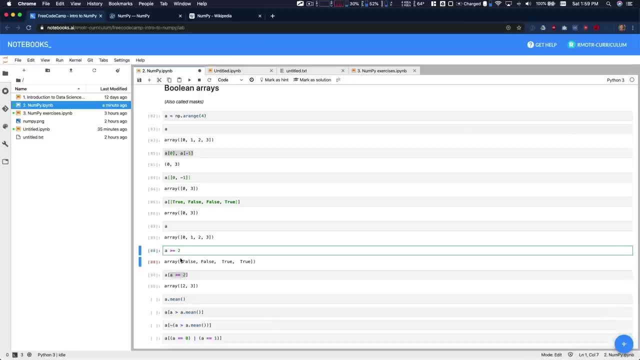 that list of Booleans. Well, in this case, we have constructed it by including a predicate, by including a condition that needs to be matched. The result, again, is filtering. it's a query method. you're looking, looking up some data. you're saying: give me all the. 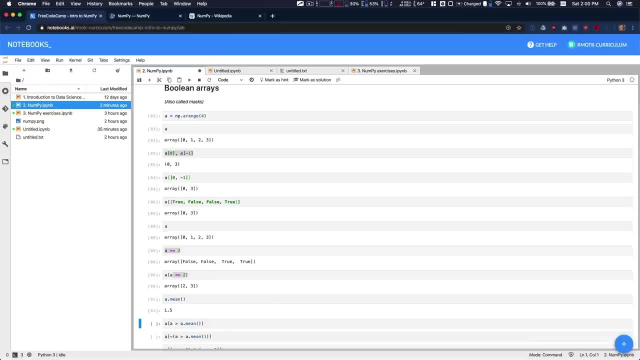 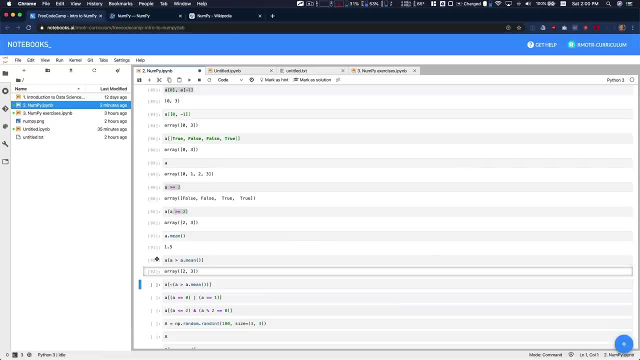 elements that match this condition. So you can say, for example, these values can be of course the same. So you can say, for example, these values can be of course calculated. you can say: give me all the elements that are greater than the mean, or 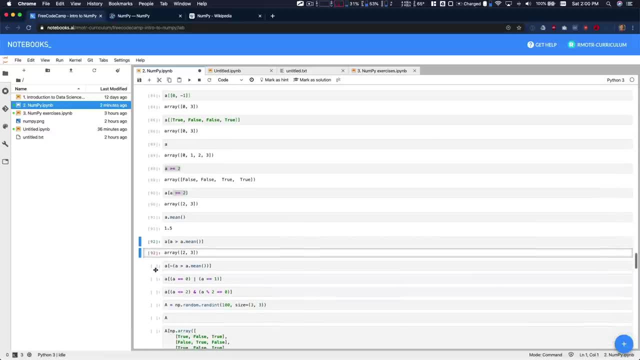 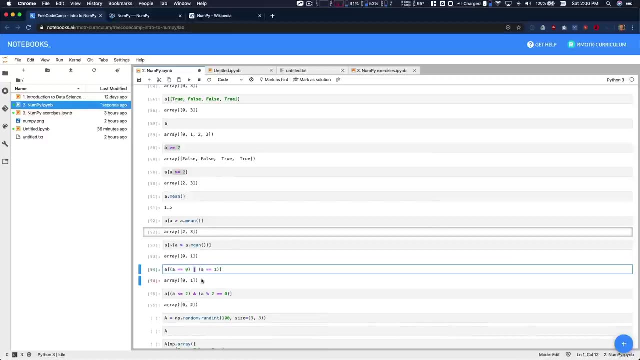 you can actually provide other Boolean appraisal operators, like, for example, all the elements that are not greater than the mean, so that means they're less or equals and the mean. or you can also include other Boolean operators like or, or, and so or, and and in NumPy are. 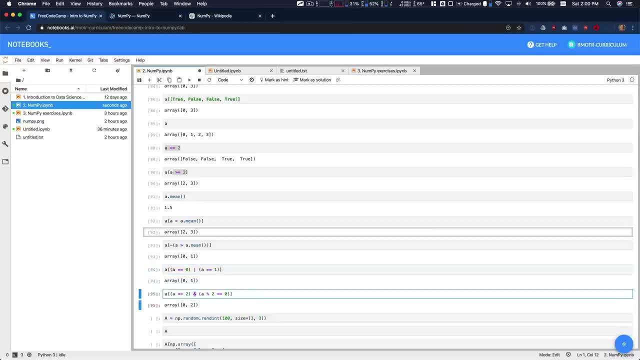 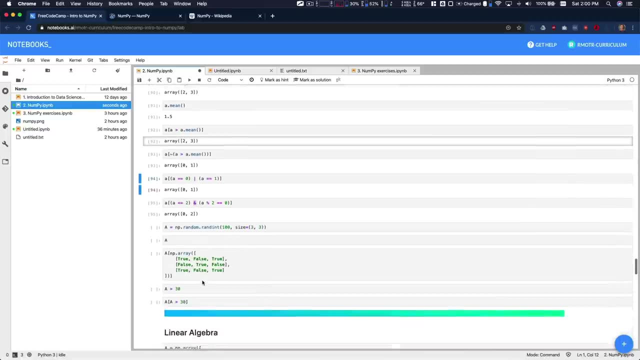 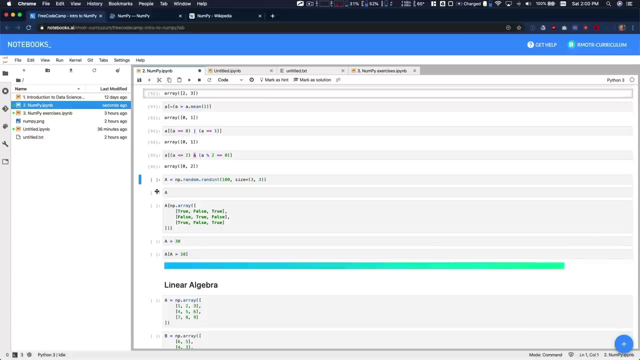 expressed with a pipe or an ampersand. ampersand because we can't use just the regular or and an in Python, And we can, but it's a good choice. they've selected this. So, again, this is the concept of Boolean arrays. we are going to construct these arrays that are just Boolean representations. 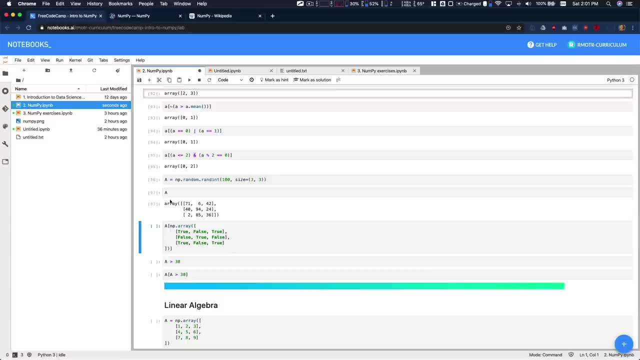 or Booleans based on conditions, right? So we have this matrix and we're going to say: I want to select these one and these one and this one, etc. So in that case, this is the result right here. This is the result of that, And we can generate a dynamic Boolean. 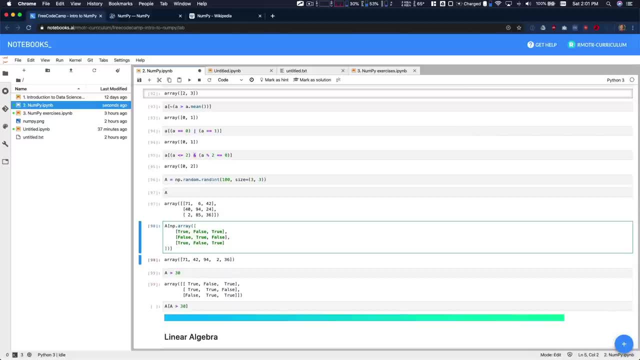 array. we never manually type all these right. we don't sit and say true, false, false, true, etc. We just run a query, filtering option, a Boolean operation which results in a Boolean array And now we can use it as filtering. So again, the idea here is that 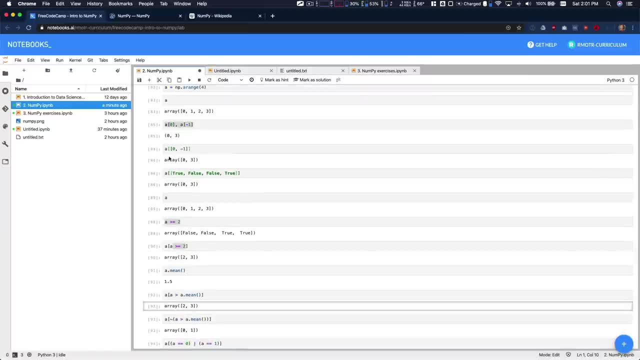 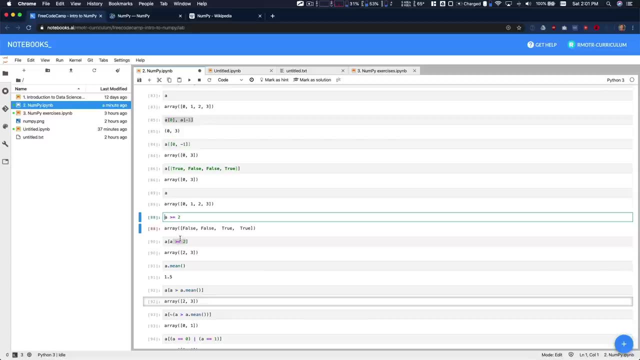 the operations we saw in broadcasting before a times 10 are also defined for Boolean Boolean operators. Boolean operators return Boolean arrays which can be used in filtering. That's the idea of all of it, And you can even combine these operations. you can say: 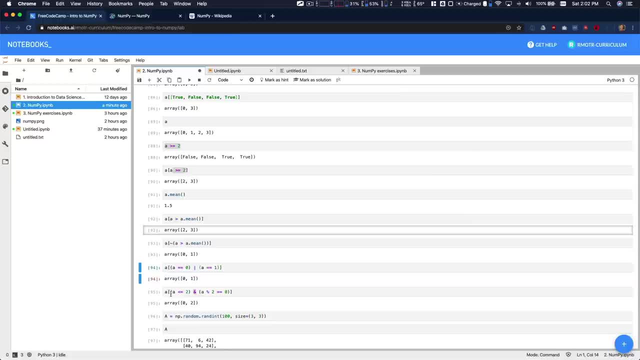 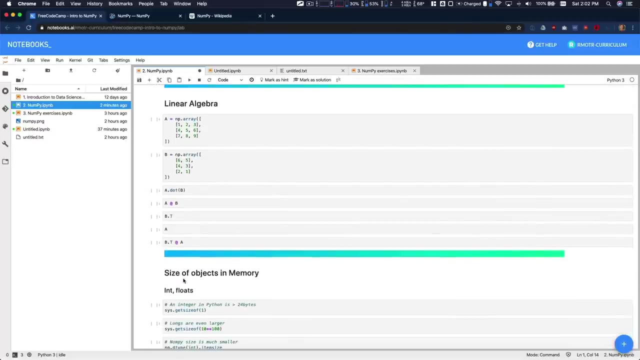 a equals zero or a equals one, a less or equals two, And it's also divisible by zero. you can combine all these queries, So now it looks a lot more powerful than when we we were doing before. So, moving forward talking about linear algebra very quickly, and this is we're approaching. 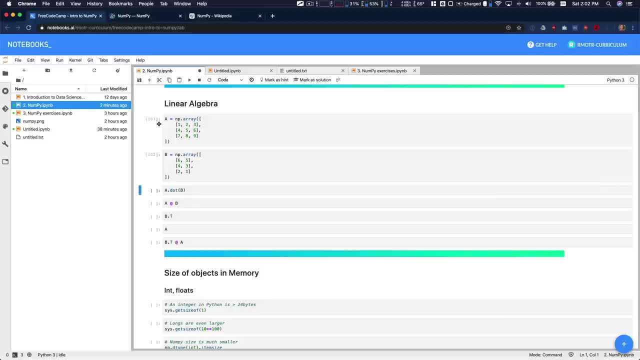 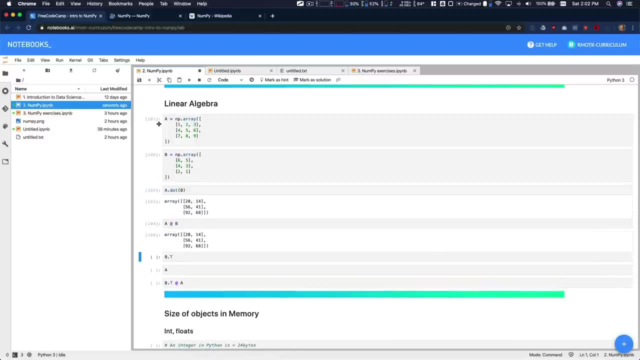 the end of the NumPy lesson, the port. the important part of the of linear algebra is that NumPy already contains all the most important operations for it. already optimized with low level semantics, it's going to be extremely fast. adult products, cross products and. 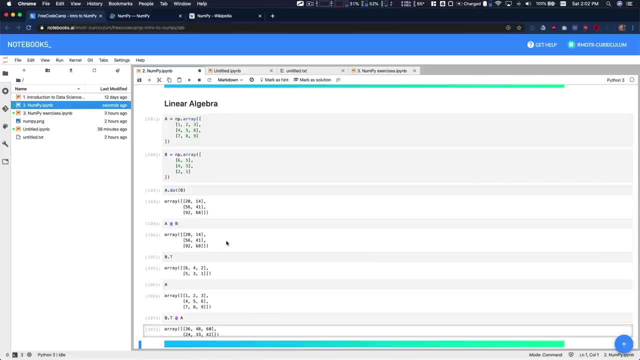 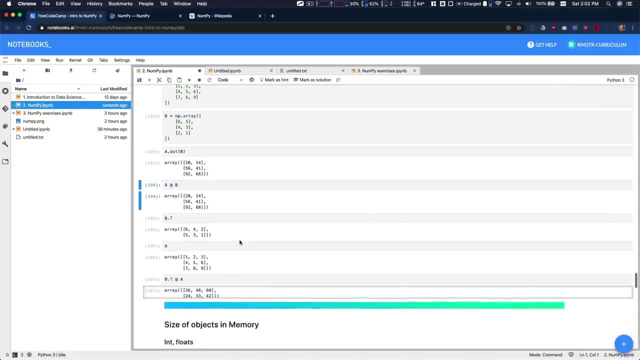 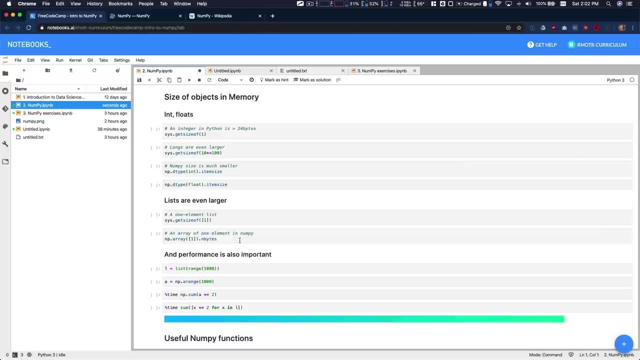 all that transposing matrices, all that works as expected- And again, this might be very, very important- especially, for example, machine learning, etc. It's extremely important. And finally, to wrap up what we saw in our, in our binary explanation at the beginning: 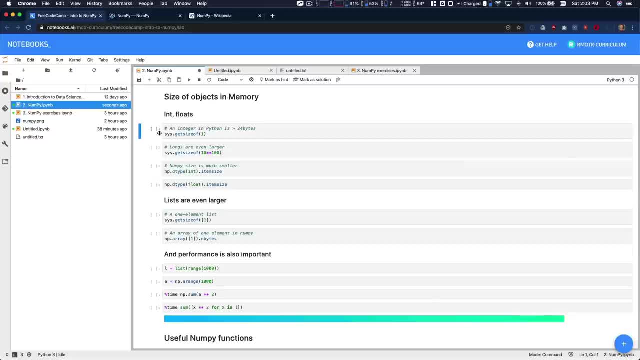 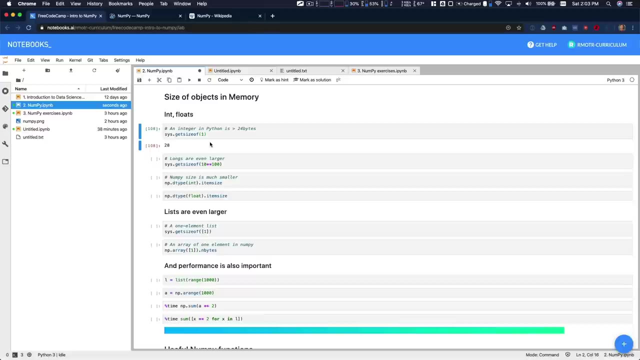 what you might have skipped is the difference in sizes between NumPy and Python, the differences in terms of performance between them. So in Python, a regular number, this is just a regular integer. in Python, That's size is 28.. Bytes in order, and just let this thing for a second: The total number of bytes. 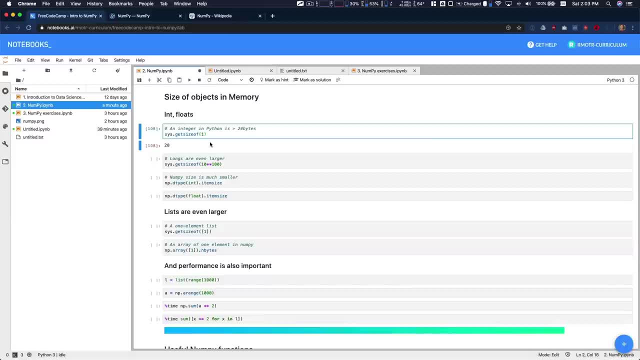 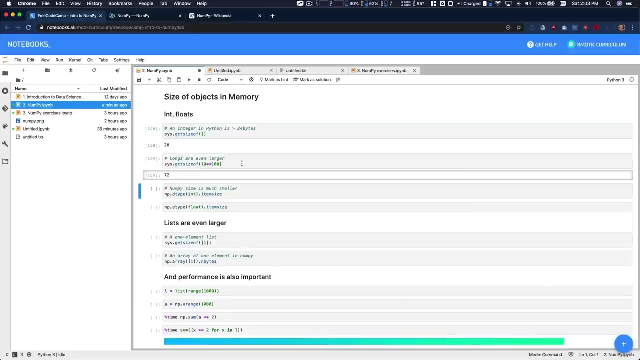 not bits. bytes that you need in Python to store a simple number, as the number one is 28.. You need 28 bytes to store just the number one is extremely space consuming, right? It's not very efficient. Larger numbers will even take more bytes to store them. What's the size of the integers? 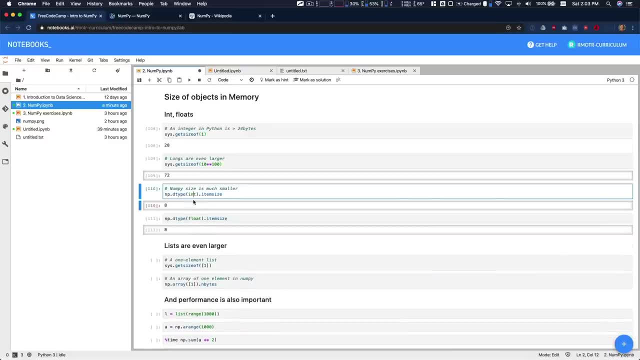 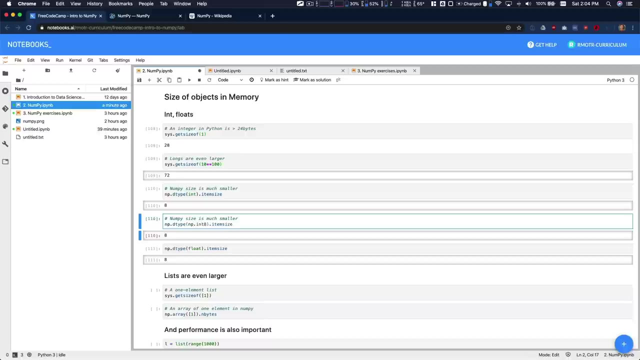 Well, we've seen it. we have. for example, we can create integers with eight bytes. we can create integers with one byte right, which were something like: here we have np Dot Int eight. we already know how many bytes has only one byte right. But you can have control of how. 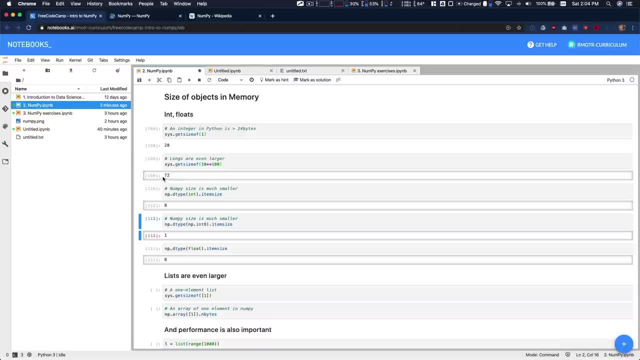 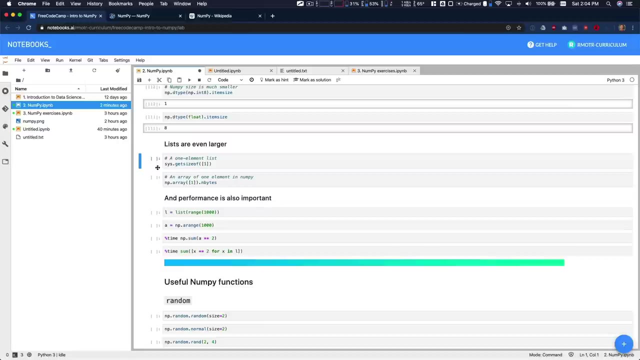 many bytes or bits, right, your numbers will take and you can see here the difference between the size of an integer in Python which is extremely large- 28 byte on NumPy- And also the difference in performance. let's say, for example: we want to hear you have the. 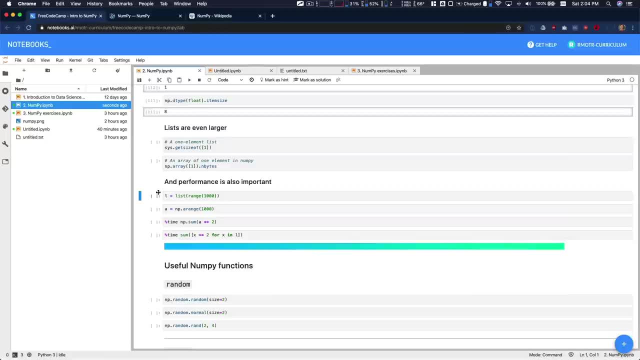 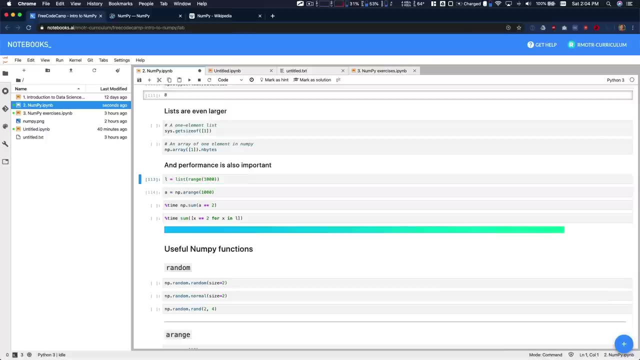 also difference in size of lists, which is also significant. but I want to focus in performance. we have two elements to have one list and has the first 1000 numbers and we have a Nempi array that has the first 1000 numbers. are going to perform the same operation in. 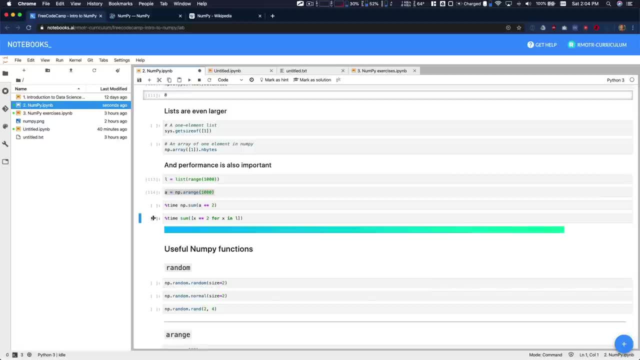 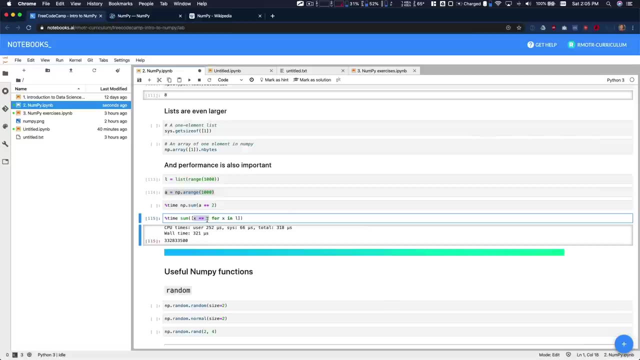 both of them. Let's use the Python one first. we're going to do the Python one first In this case, where we're squaring all the elements in the list. okay, the elements is squared, and then we're summing all the operations, right, So we express it as saying Create. 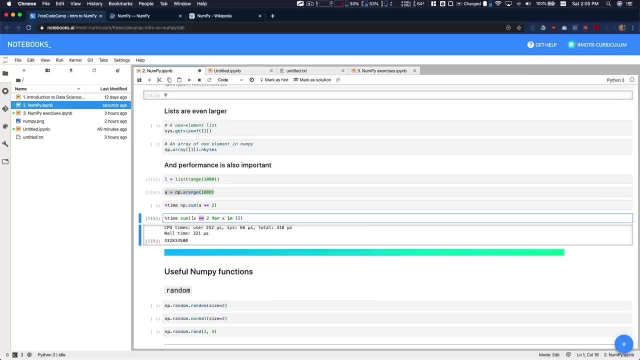 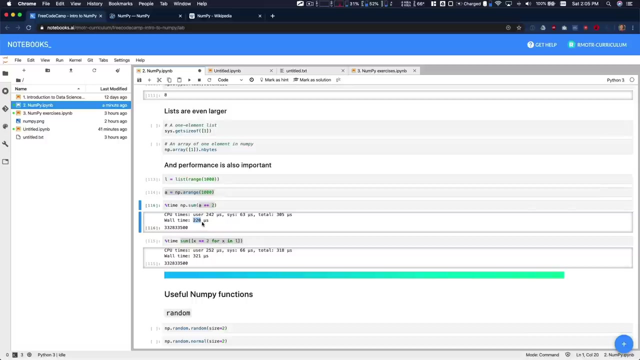 a new list, list x times x. sorry square for x in L, and then some everything. how much time it takes 321 microseconds. we're going to do the same thing with NumPy. we're going to say np, dot, sum a square, and you're going to see that it's a lot faster in the NumPy. 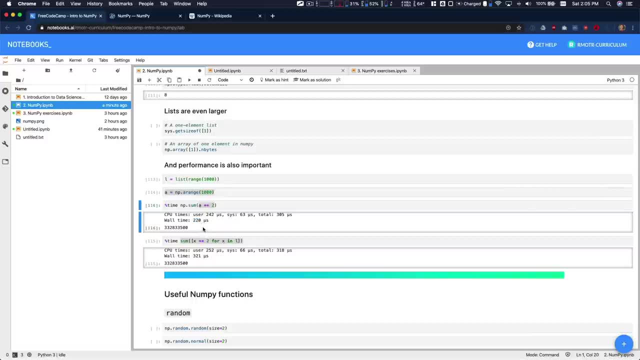 perspective than the Python perspective, And these are all very, very tiny, tiny operations with small numbers. What happens if we add more numbers? let's add two more numbers here, Let's add two more numbers here, And we're going to do the same two operations. So you, 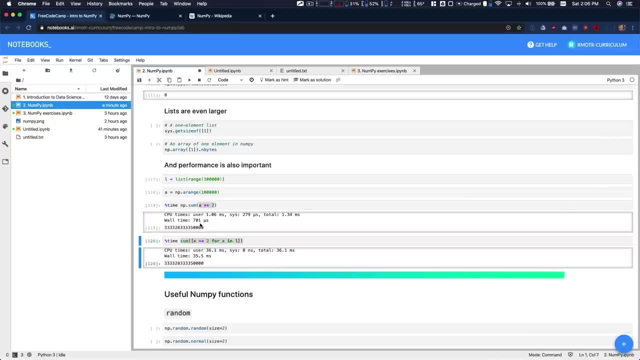 see here, the, the, the units have even changed. we're still in the microsecond layer here with NumPy And we've gone to the millisecond layer in Python. So as the size of your objects increase, NumPy will prove to be extremely fast compared to Python. So there are a few other functions you can see. 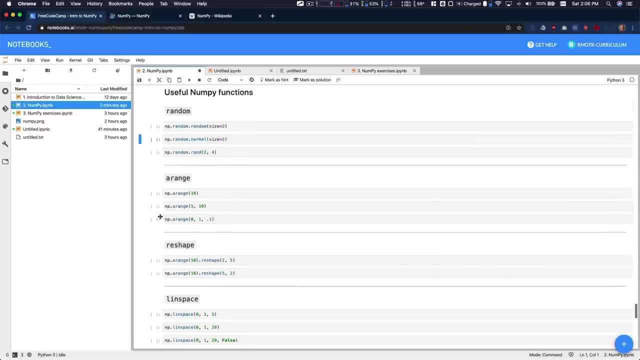 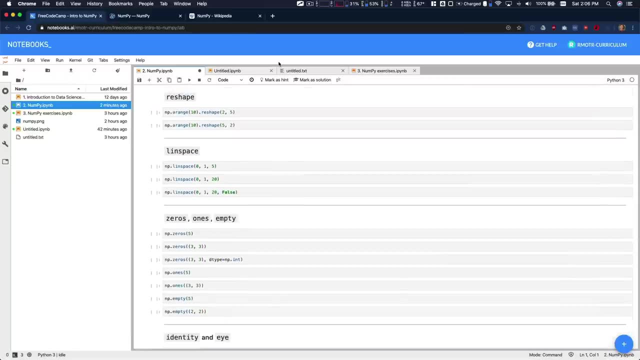 here, for example, extracting normal random numbers, etc. I'm going to let let these for you to look if you're interested in them, And remember you have the exercises which can help you solidify all the concepts we've discussed. 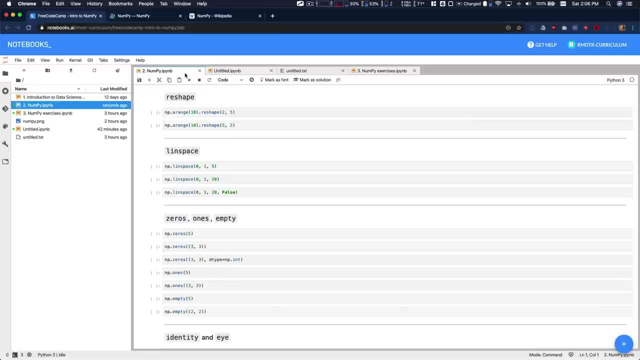 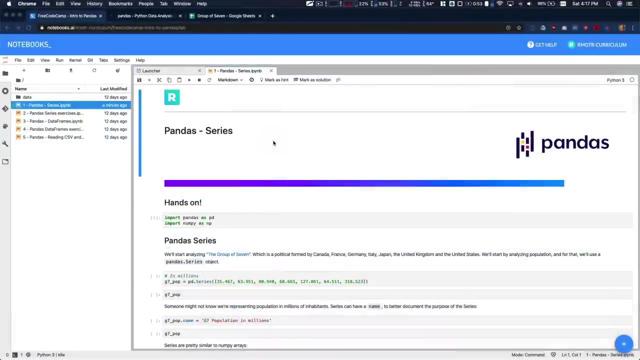 And we're going to move forward. Now to work with pandas, we're going to see also visualizations. we're going to keep moving forward this data analysis with Python tutorial, And now it's finally time to talk about pandas is the most important library that we use. 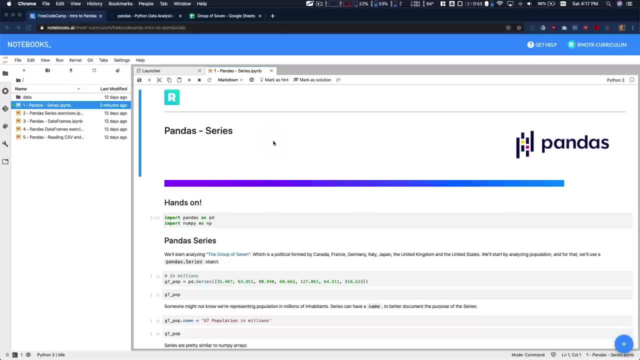 for data analysis in our day to day basis with Python. It's a library that will aid in the entire process, So let's get started. So you're going to start with the process of your data analysis project. you're going to start getting the data. step one: getting the data from multiple sources like databases. 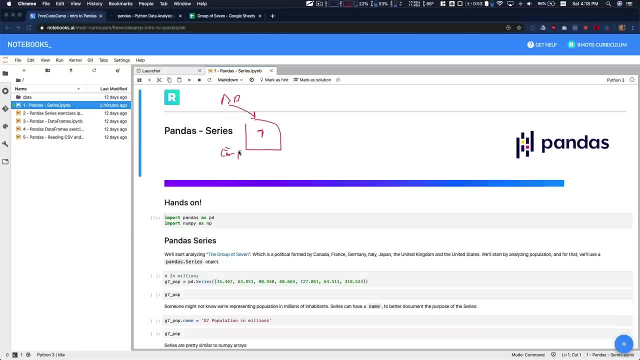 Excel files, CSV files, etc. That's all gonna get into pandas. you're going to be processing the data, right, so you're going to be combining, merging, doing different types of analysis. you're going to be visualizing the data, right, so a bar chart you're going to be visualizing. 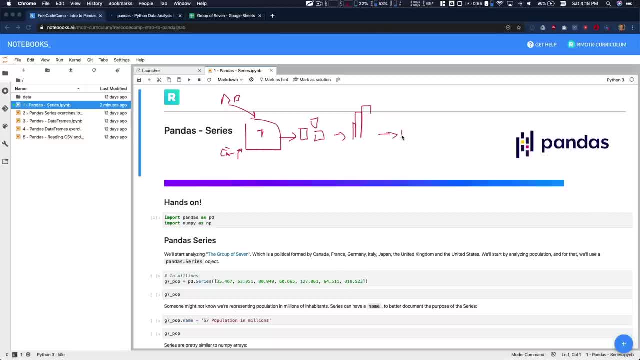 the data with pandas. You're going to be creating reports. you're going to be also doing simple statistical analysis. you're going to be doing machine learning, close to it, with the help of other libraries, but everything from the platform that provides the pandas library. it's again. 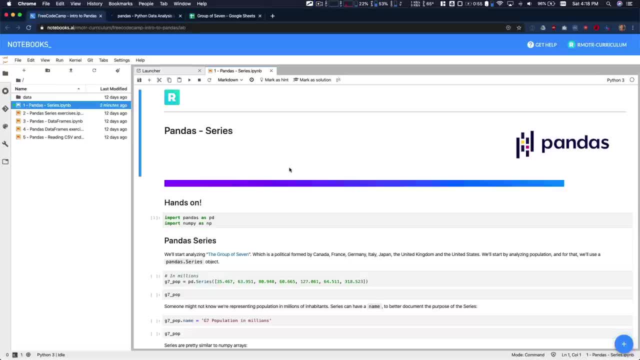 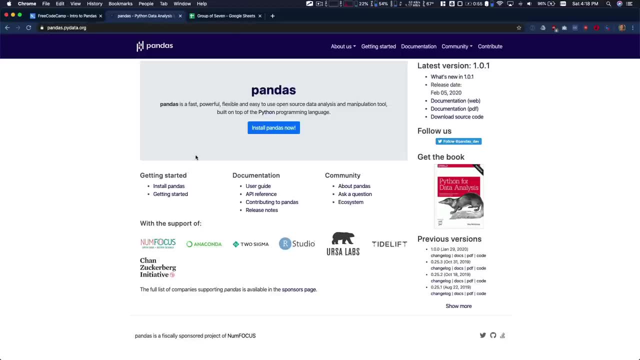 one of the most important libraries in in in the data analysis, data science ecosystem with Python. pandas has recently released the version 1.0.. That's the latest version of pandas. That's the latest version of pandas, So we are talking about a very mature library. 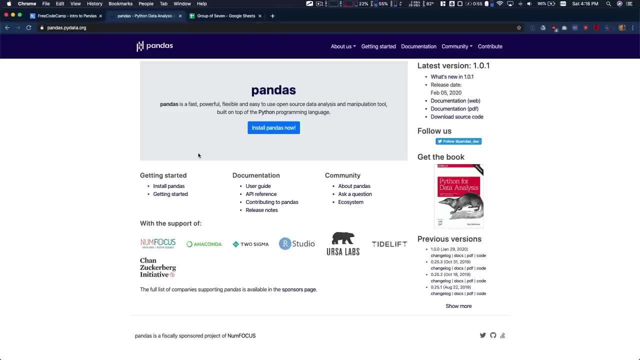 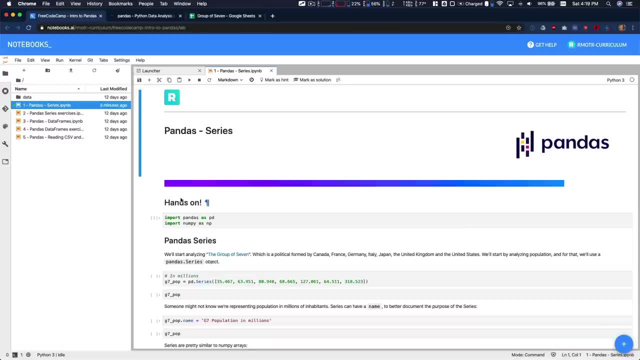 It's been around for a long time now And again, it's the primary library that we use in Python for data analysis and data science. So I'm going to do a quick introduction to the data structures that pandas has, and we're going to understand how they work. 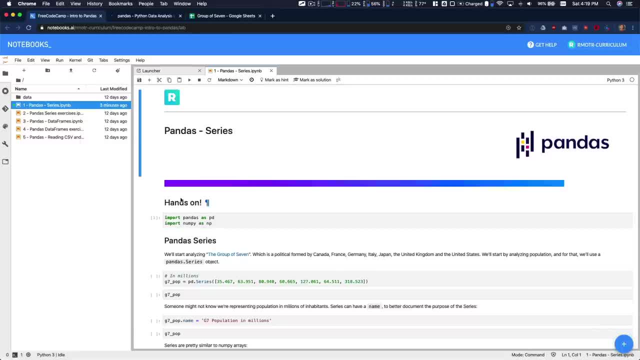 So you can start building right the phone. we're going to start building the foundations. I need you to be very familiar with the way the data structures from pandas are processed, And then we're going to move into other things like reading files, grouping data, etc. 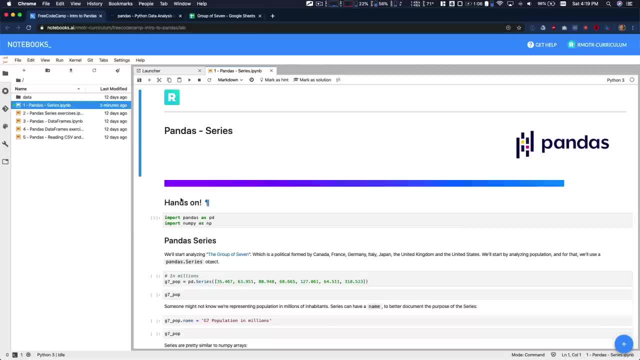 So, to get things started, we're going to talk about the first data structure to pandas has, which is the series. In reality, pandas has two main data structures that it uses all the time, And it's the series under the data frame. the data frame is the one you will probably 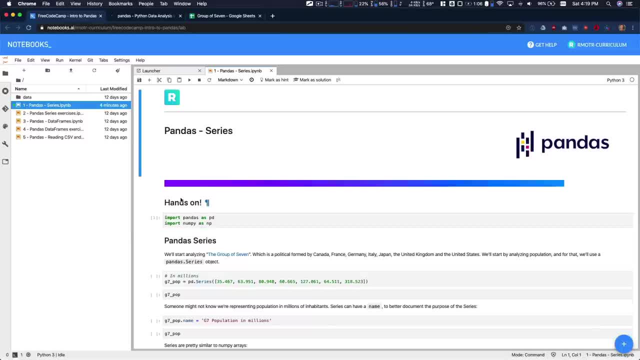 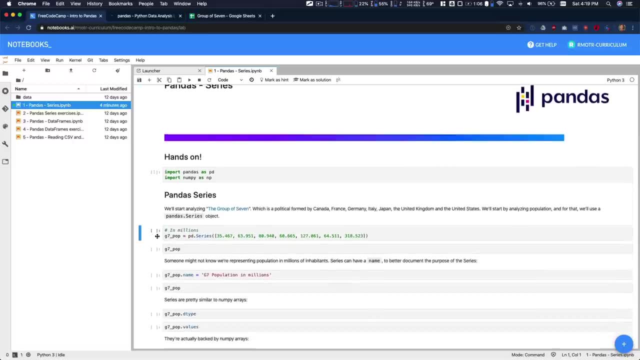 be more familiar with. it looks just like an Excel table, But we're gonna start first with a series. Okay, so just stay with me here. We're going to talk about a series for a second. In this case, we have imported pandas. 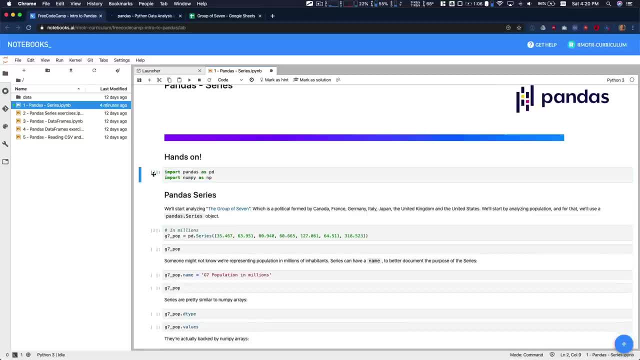 And we have also imported NumPy, as, as you might imagine. as I told you before in a NumPy part of this tutorial, we were saying: NumPy is fundamental for data analysis because every other library- pandas, matplotlib, they all sit on top of NumPy. 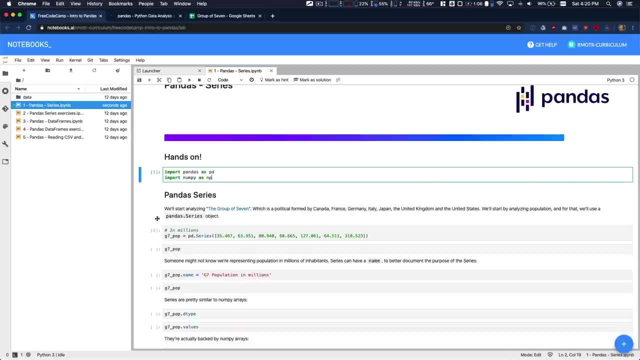 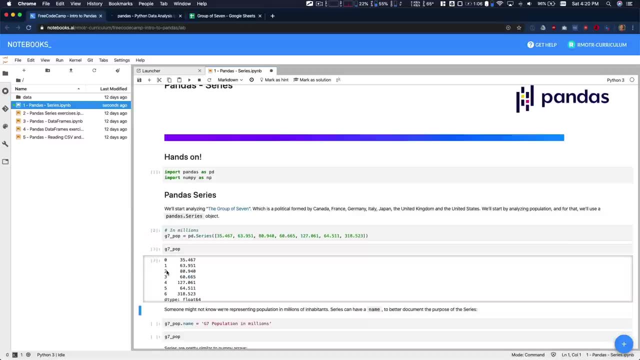 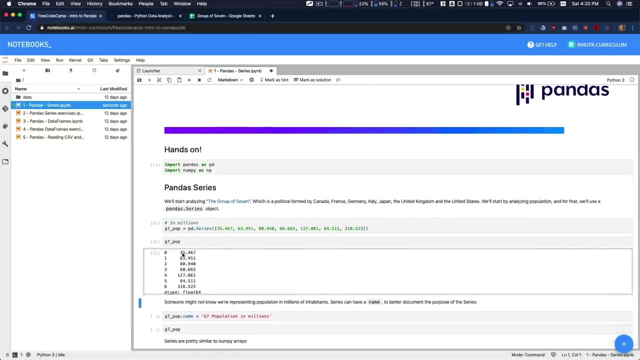 And you can see it right here. we're going to be using some features from NumPy within this lesson too. So this is a series in pandas. What do you see right here? It's the concept of a series. is this ordered sequence of elements, right? 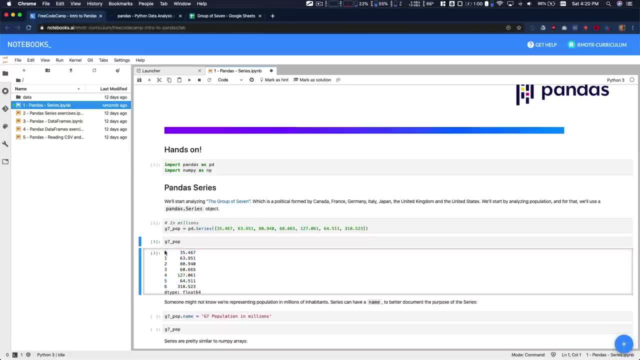 All indexed, right with. they are all indexed by a given index, of course, And you might think that this looks a lot like a Python list, right? So in this case, we're storing the population of countries right in millions of inhabitants. 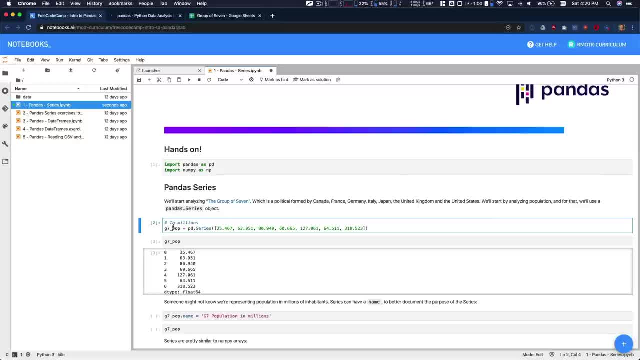 In this case it's Jeven Jesus. Jeven pub is because we're getting the population of the group of seven. you can console the Wikipedia page, But basically we are storing population in here in this series And again it looks a lot like a list but we're going to find a ton of differences in. 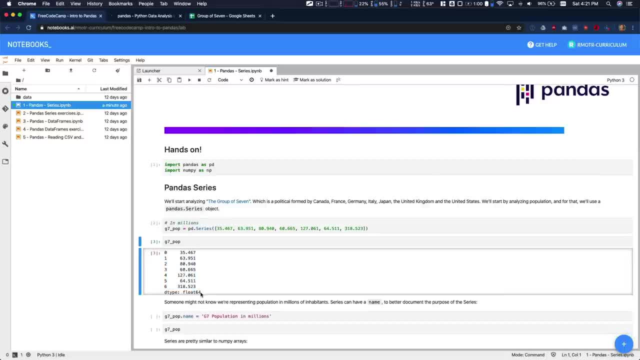 here. So the first one is that the, the series, has an associated data type, And this is something we saw in NumPy. when a NumPy array couldn't hold different type of objects, We were all. we were only having one type of object. in this case it's float 64.. 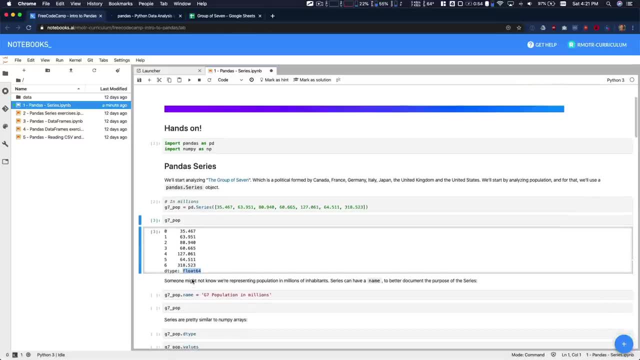 So all the numbers of the series will be of type float 64.. The underlying data structure that pandas is using to store these objects is a NumPy array. So a second difference we see very quickly is that a series can have a name right. 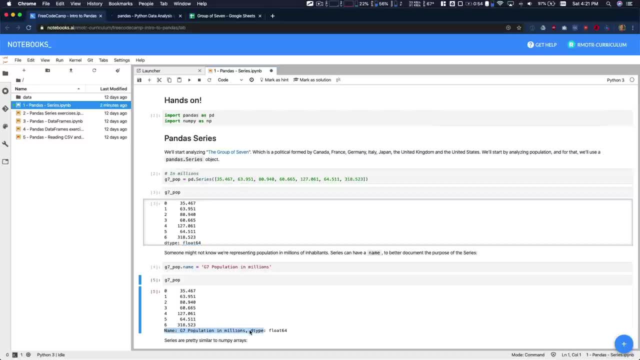 So now, when we display the series, we see that it has a name, and now it might not make a ton of sense, But once A series is part of a data frame in the form of a column, then the name is going to make. 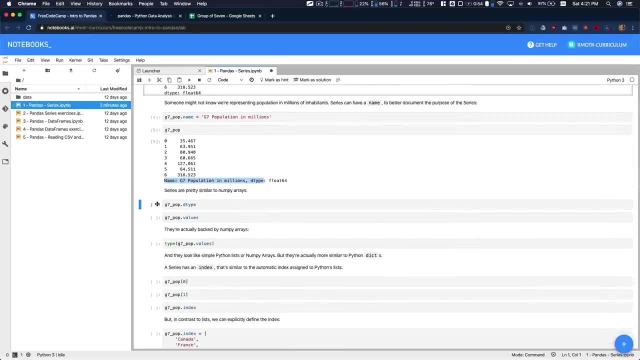 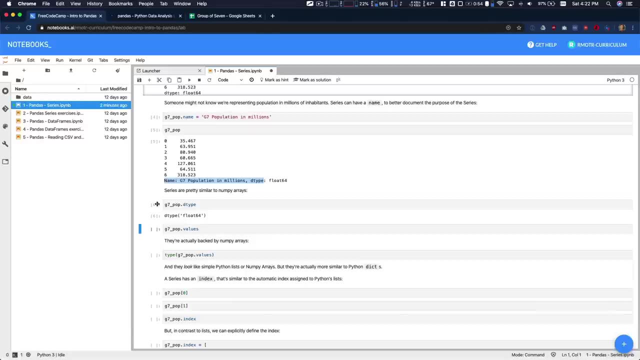 a lot more sense. So, moving forward, again we saw that it has a type And again this is because the box, the data, is boxed by a NumPy array. you can always consult, you can check values of a series and you're going to get the array that it's. 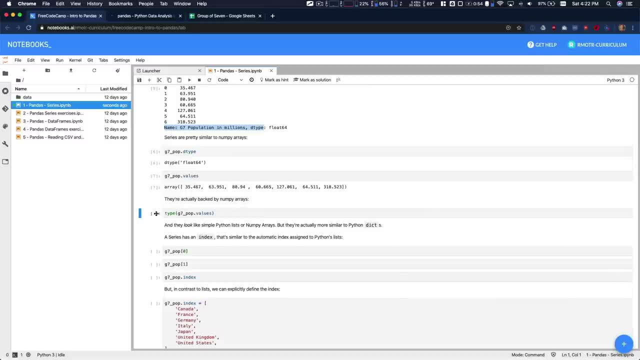 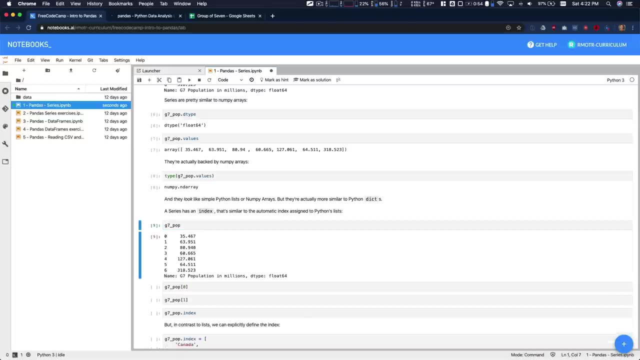 backing up that pandas series, right? so you can see that it's a NumPy array. Once you have these series we were just consulting here- This is on pop- you can in. you can select elements as you would in a regular list, right? 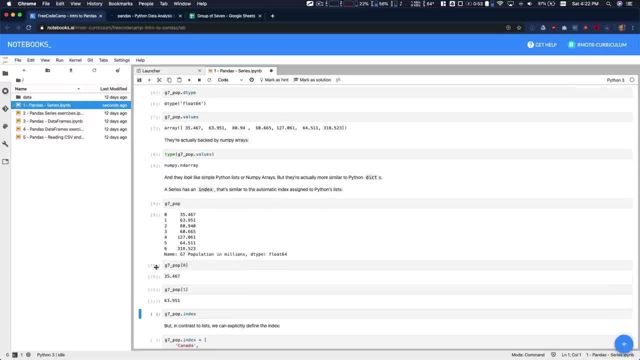 So, for example, give me the first element, give me the second element, the last element, etc. And that's because a series in currently has an index similar to list, a list, when you create a list in Python, right? so if I create, l equals a, b and c. 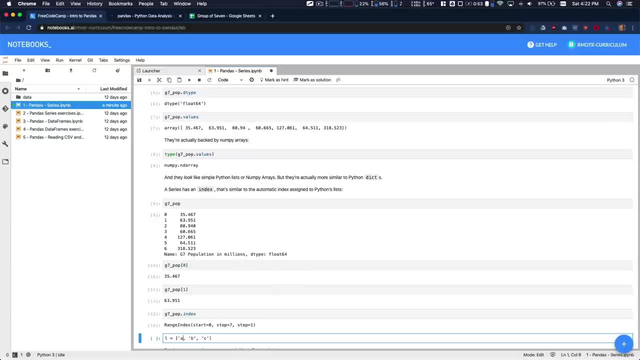 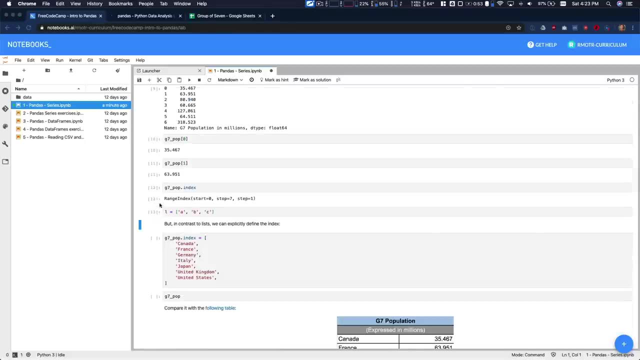 There you go. there's something wrong here, missing a quote this list. we don't say it right, But the idea is that there is an index here: the zero, this is one and this is two. right In the pandas series, this is a lot more explicit: each element has an associated value within. 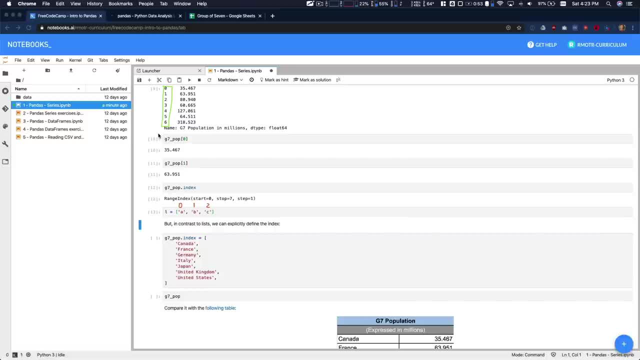 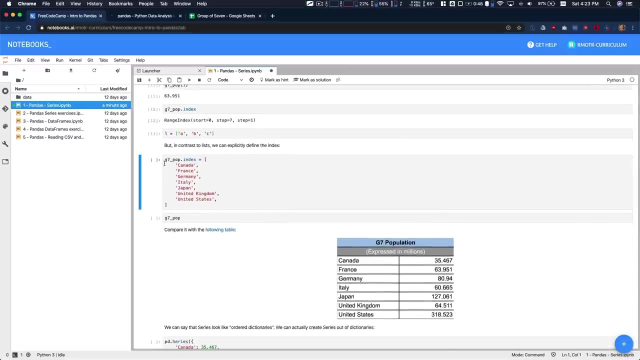 it And you might think that That is pretty much the same thing. They're all. they're both the list on the series. they're both sequences. they're ordered sequences of elements, But we're gonna see that there is a fundamental difference on is that we can arbitrarily change. 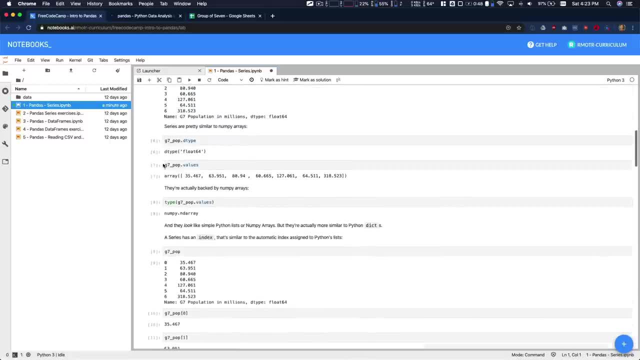 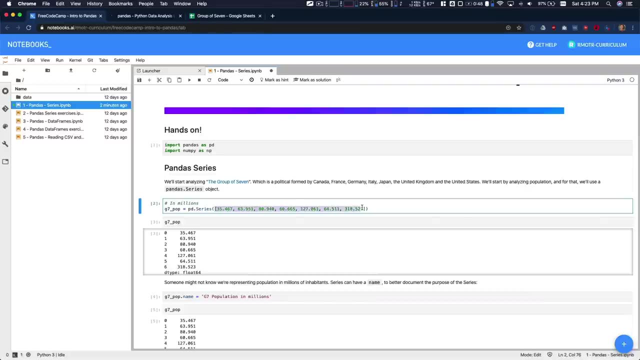 the index of a series. So by default when we created it we didn't assign any indices. So by default it was a range index from zero up to n minus one elements. But you can see that it doesn't make a difference. 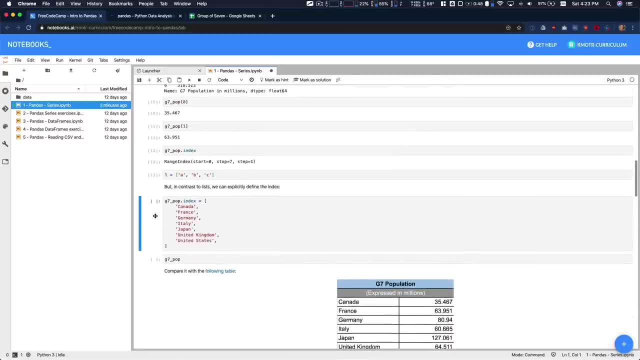 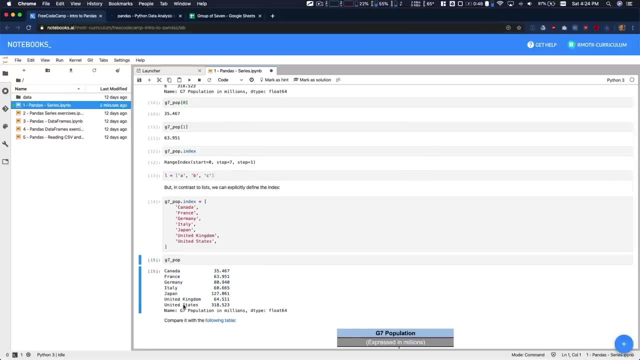 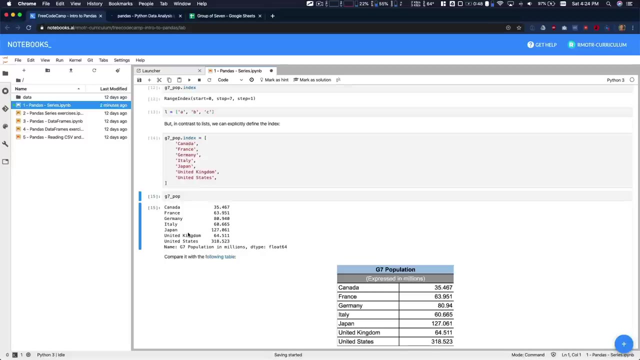 So we can change the index. you can actually arbitrarily again say what is the index of your series And in this case, these data structure. this series has now these indices that we're saying right here. Why is this important? because now we're going to be referring to these values not by a. 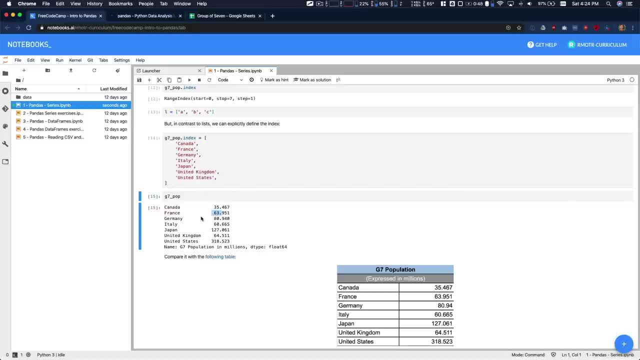 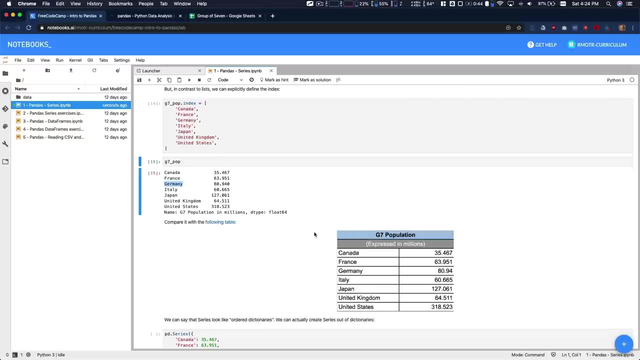 sequential position, but by a name, by, by a label, by the index which has a meaningful name for us as humans. Okay, so now these thing looks a little bit more like a dictionary, we could say then a list. we started thinking that a series was similar to a list. But now 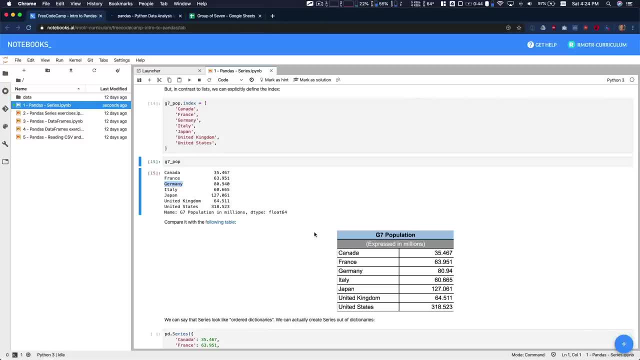 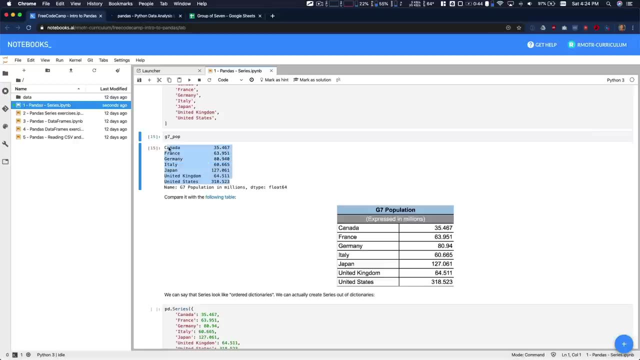 we can think that a series is limit similar to a dictionary. But wait, don't get me wrong here. The series has a fundamental trait, And it's that it's still ordered, something that didn't happen with with dictionaries- dictionaries in Python. 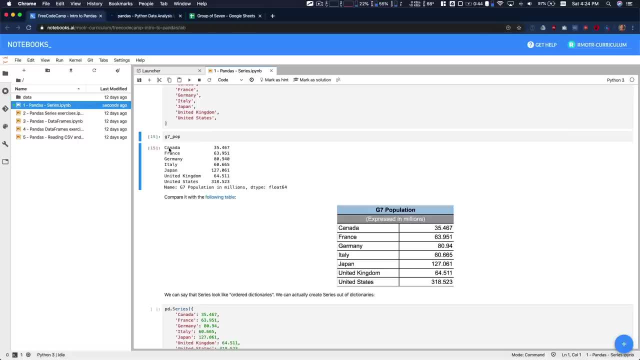 are not Ordered. actually, in Python 3.7, they're ordered, but we shouldn't be thinking that they're ordered their unordered data structures. In this case a series, is indeed order, So it has both those advantages: It's ordered. 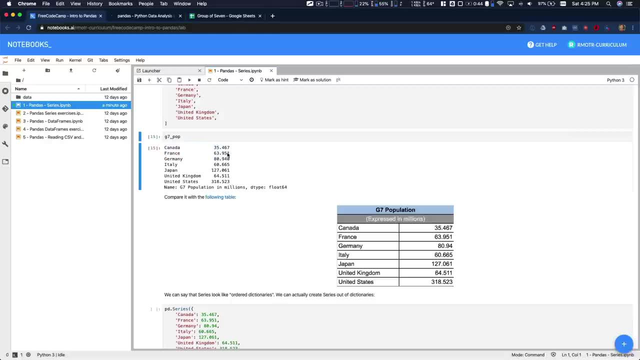 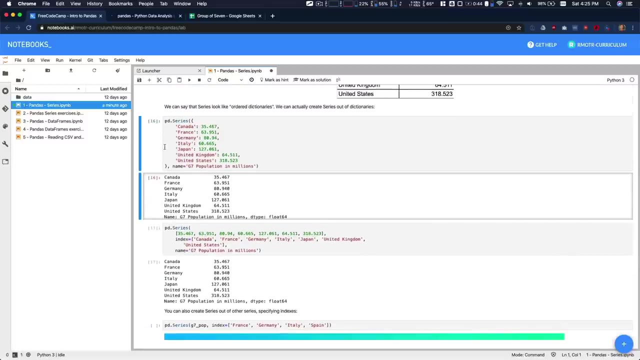 Kennedy's always before friends. That's as we decided to create it. But also it has names or labels or keys associated with the values as a dictionary. So this is creating the series from a list. scratch right, all these methods. you can see that you can create a series bypassing 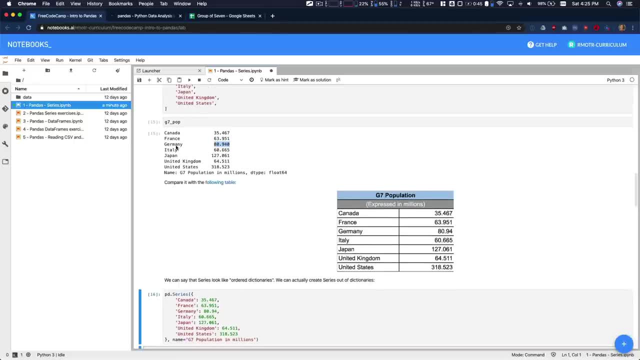 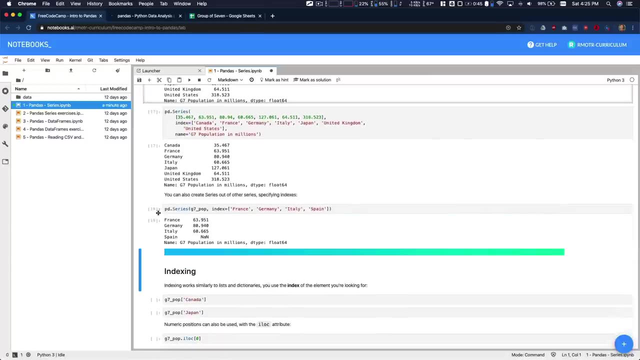 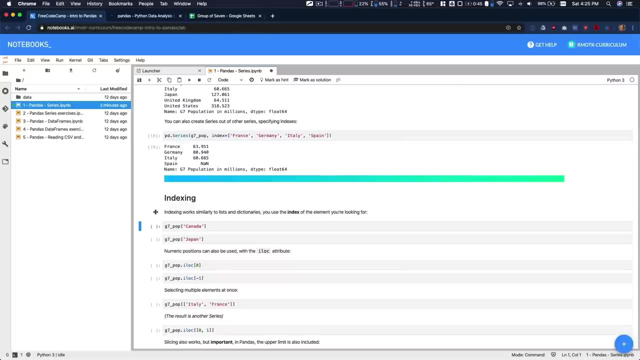 the index. it doesn't have to be a two step process where you first create the series and then add the index. In this case, you can do everything at once And the indexing is now going to be done by those indices, right? So those labels that make up the index. 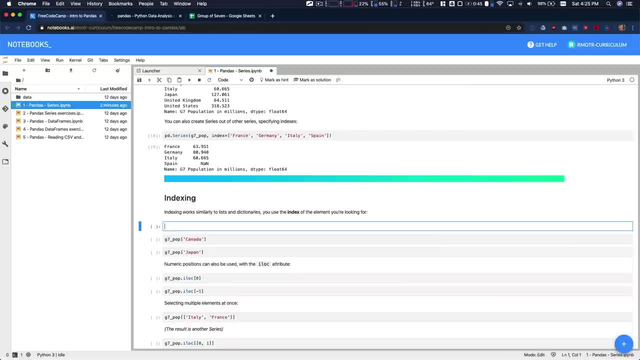 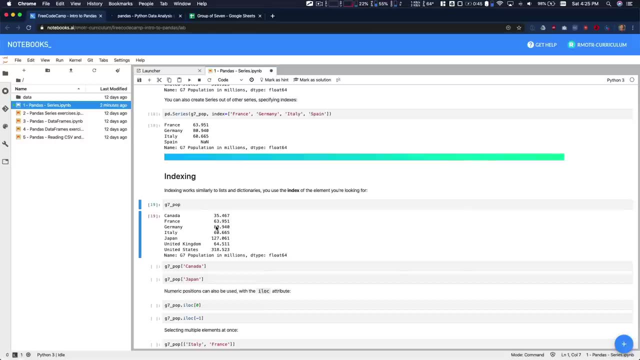 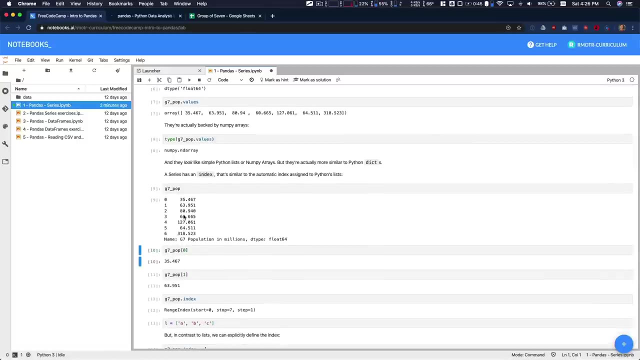 will be used to index specific data. So g seven pop, we see, has these countries with these population. And now, before the index, we were saying I want to get what's the population of Canada. And then we had to remember what was the position of Canada. Oh, it's the first. 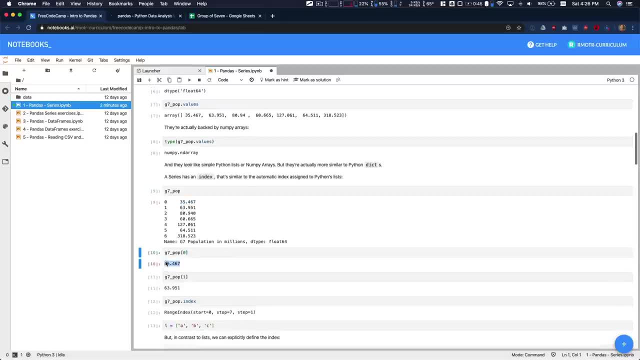 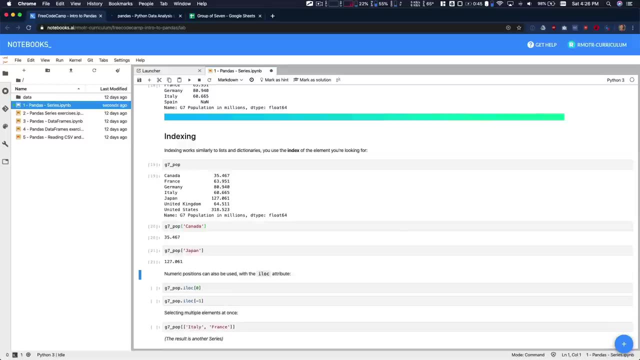 help countries. we have to do g, seven, pop and zero with the index. Now we can just consult: what's the population of Canada, What's the population of Japan And, as you can see, the syntax is the same as with the Python dictionary: just pretty. 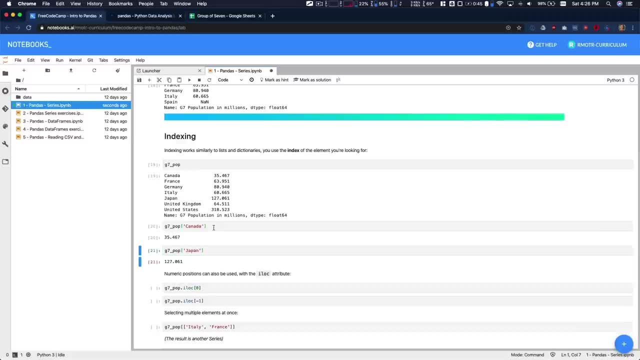 much same. you pass the key and it's going to get the value. So again, summary: the advantage of a series is a is a ordered sequence of elements backed by a NumPy array, very efficient, very fast. But it also has an index that can take any labels as we pass. So it's going. 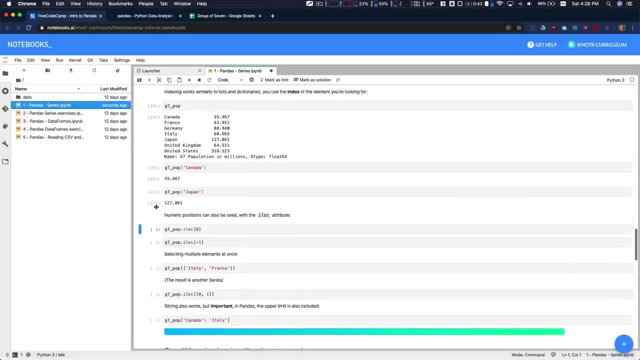 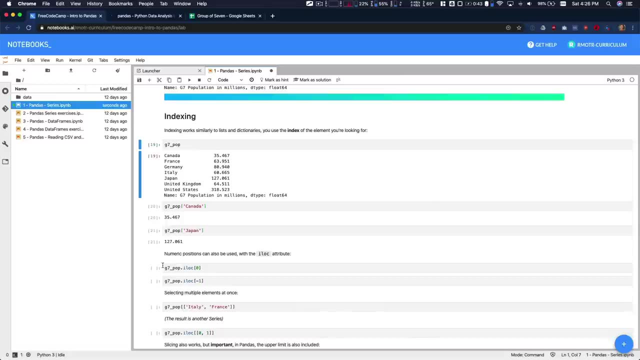 to make it a lot better for indexing. you can steal. when you have a series, you can still get the elements by the sequential ordering. After all, it's a sequential data structure. it doesn't matter if you have in an index. you can still say: hey, I know, we have an index, but if you want, 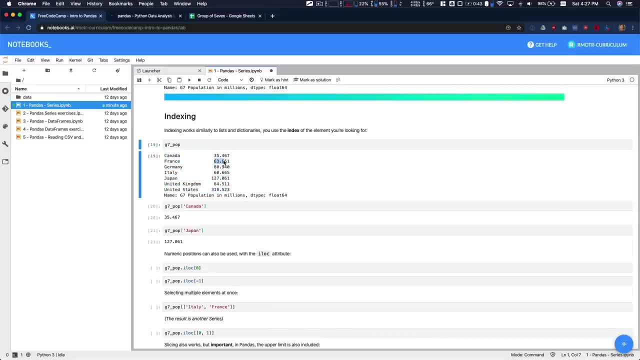 to get the last element, or the first element or the second element, and you're going to do that by using the attributes I look. okay, so you can say to this series, from this series I'm going to- I lock, locate by sequential position these elements: the element in position zero. 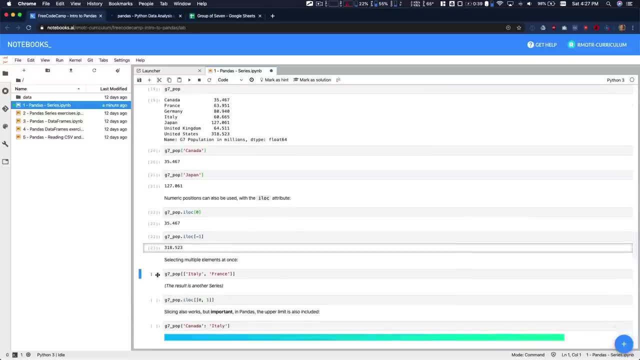 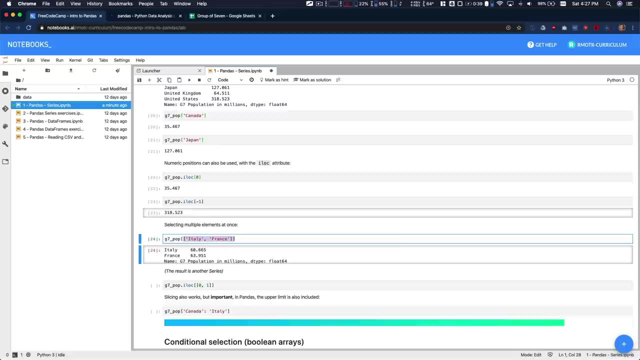 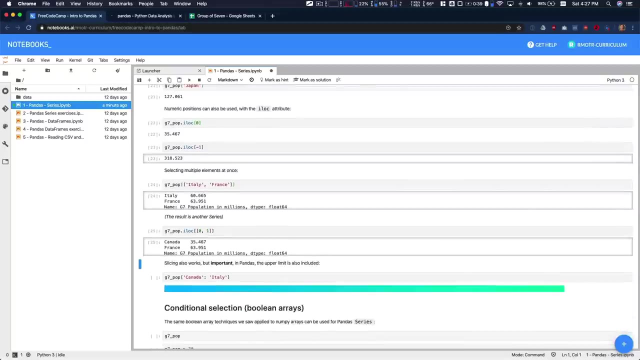 or the last element, And that still works as expected. series also support multi indices, as we saw with NumPy. So in this case we can get two elements out of two, three, n, any elements. you can pass multiple indices And the same thing happens with more, with sequential. 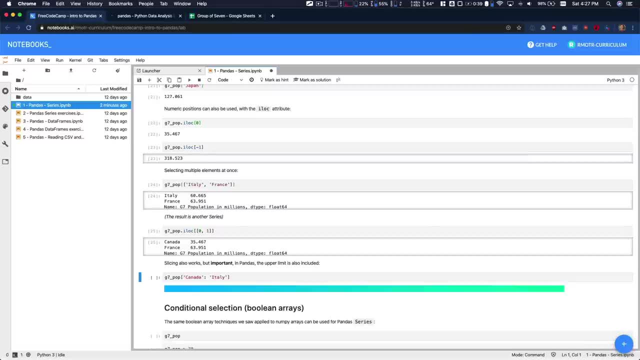 multi index series also support range or selection or slices, but there is a fundamental difference here. this is very important. pay attention. there's a fundamental difference with Python And it's that in Python the upper limit of a slice is not returned. So from our list. 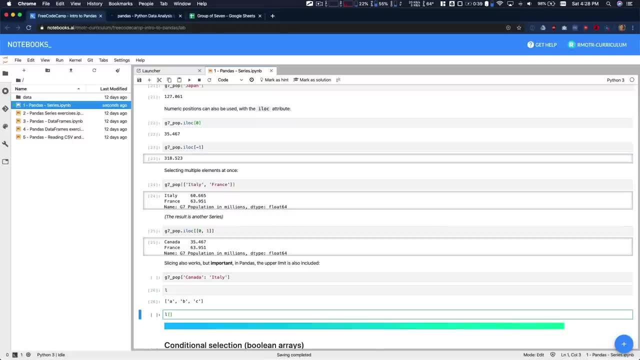 that we created before. if I do L up to number two, I don't get the index C right. So this is zero, this is one, this is two. two is not included In a pandas series. the upper limit is indeed included. So if, when you ask from Canada up to Italy, 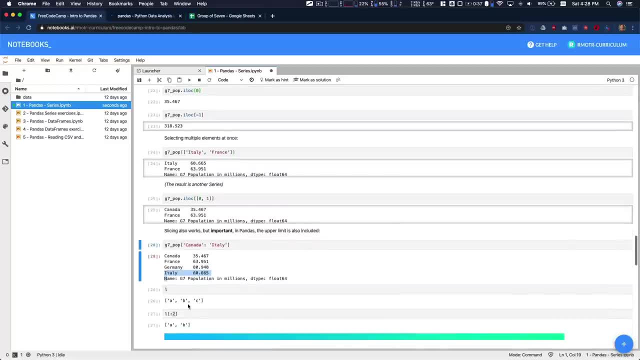 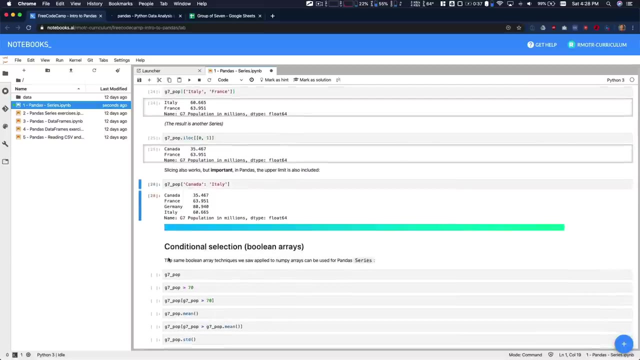 Italy is in the result Okay. so this is something to consider when using index selection in pandas. I think this is still violent. It's very I understand the reasoning behind. it's just different from Python, So you should remember Boolean arrays, which was a topic we discussed in our previous lesson of NumPy Boolean arrays. 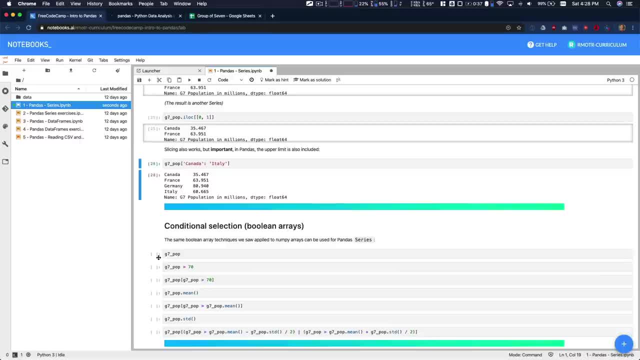 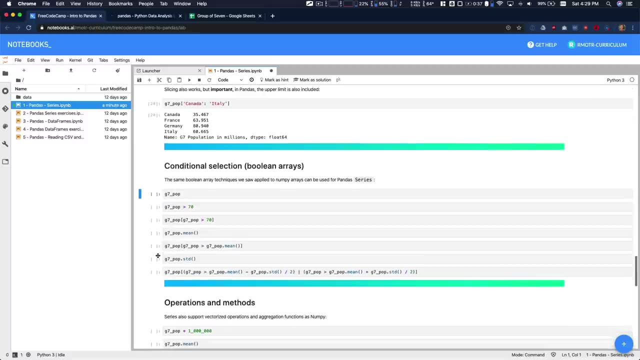 is still a thing in pandas. the difference that we, instead of saying Boolean arrays, we should say Boolean series. right, The idea is that we will be able to perform operations on top of series. So, for example, right here we have mathematical operations on top of. 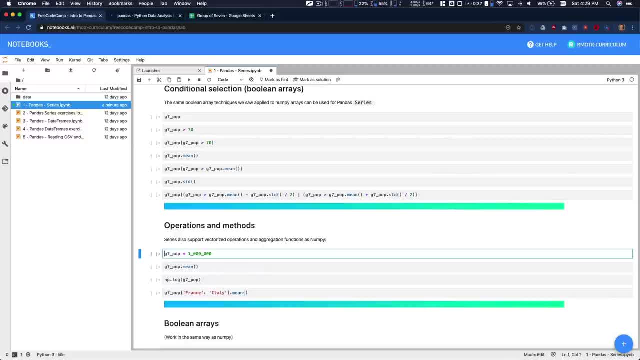 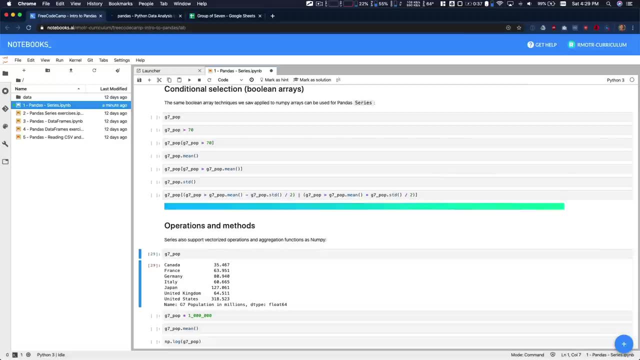 series. In this case we have the zero G seven pop which, as I told you at the beginning, is in million of inhabitants. If we want to get the series of in just units, we will need to do G seven pop times one million, And there you go. now is in terms of units. 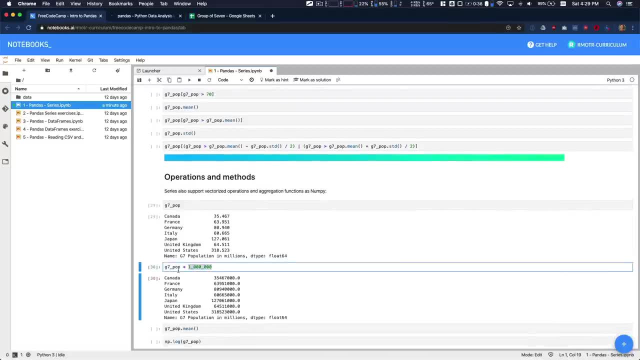 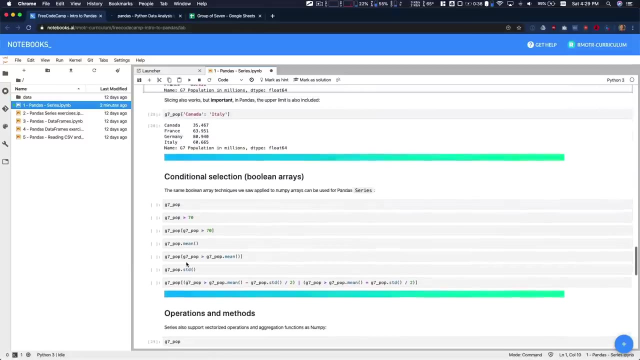 These operations- right, these vectorized operations that brought these broadcasting operations- can also be performed with Boolean operands. So instead of a multiplication, a summing operation, we can also perform Boolean operations. So instead of a multiplication, a subtraction, etc. we can add, we can use a Boolean operator. So in this case we can. 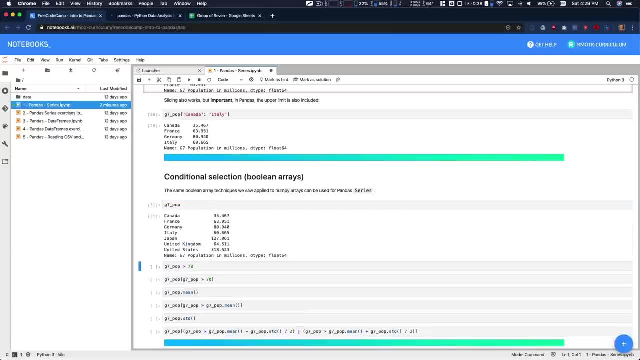 ask: what are the countries that have more than 770 million inhabitants? we will receive the result is a Boolean array. it's not a braille right, it's a Boolean series, you know, but basically it's the same concept of with us with a NumPy Boolean array: Canada. 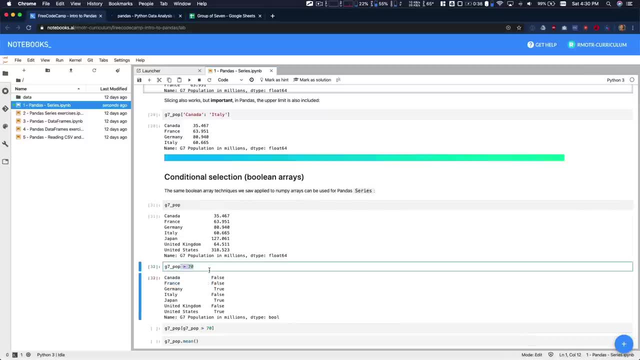 France, they do not have more than 70 million inhabitants. In Germany does have seven, more than 70 million inhabitants, here 80. And the same for Japan. So Japan here is the same on the same for the US. The US also have has more than 70 million inhabitants. So again, 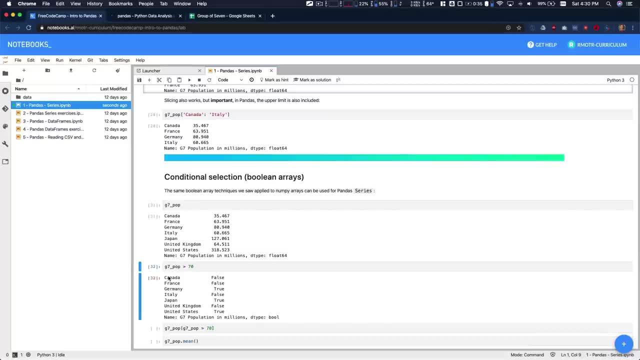 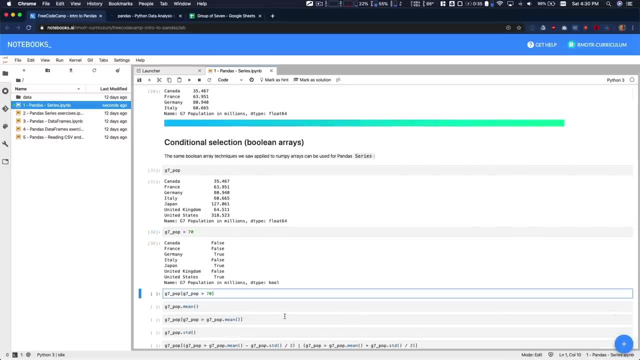 the Boolean array or Boolean series in this case, works in the same way as with NumPy And selection. It also applies, So I can now select. I can say: give me from these series just seven, pop all the countries that have more than 70 million inhabitants. the value is more. 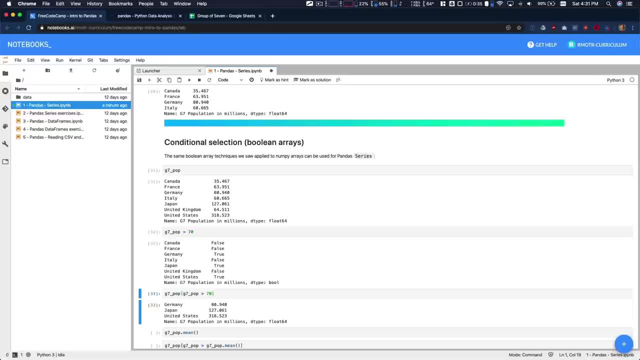 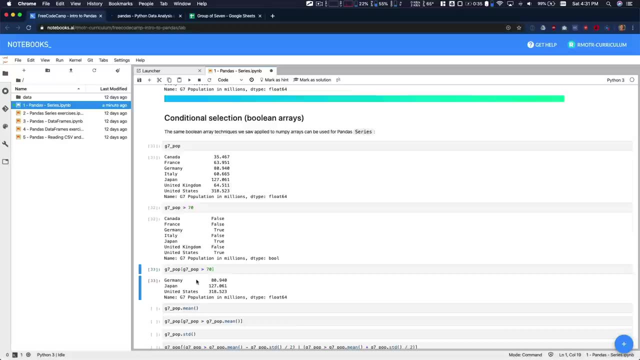 than 70. So now again, we are building filtering, we're building a query language, if you want, on top of pandas, we're selecting data based on this condition: Remember when. if you ever have trouble, remember all these, the idea is that you can always track down the way this index is. 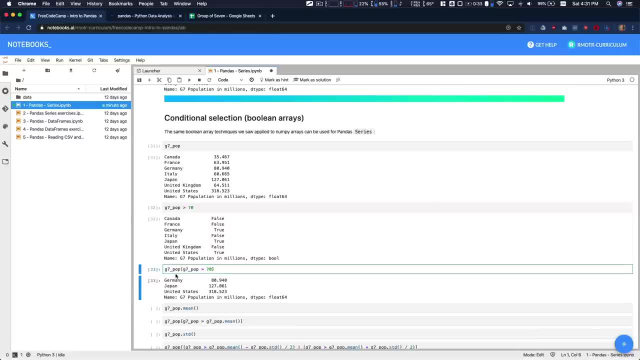 being built. In this case we are. it's not that the selection knows anything. this first election knows anything about how to select countries with more than 70. This operation was performed first, which resulted in these series, And now this series will be indexed. 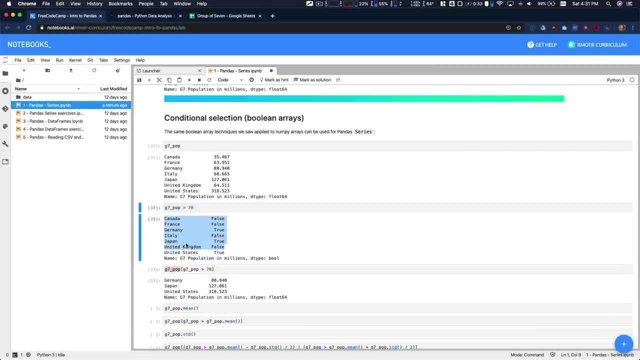 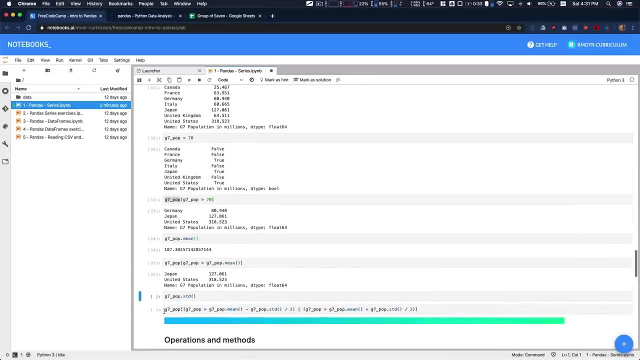 by these array, these Boolean array, And the result is as you can see it. and again, these operations can be run with calculated methods and all the operators we saw in our previous lesson- which was not, which was, or this regular pipe, or and ampersand, which. 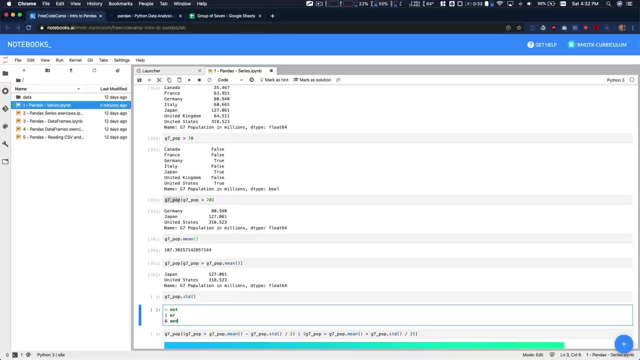 is the end. all these can be applied in any order that you want. So if we read this thing, which is complicated on purpose, it's worth saying: give me all the elements that are above the mean minus two standard deviations, or below the mean, actually above the mean. 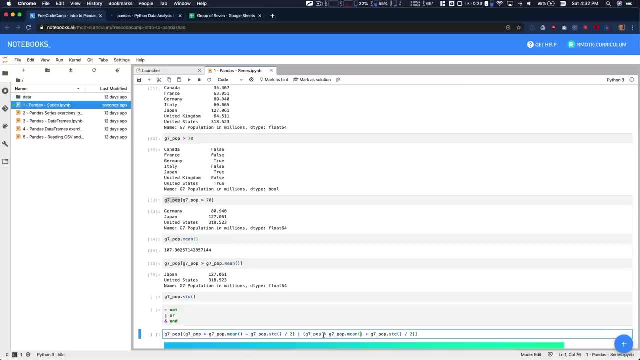 and here was below the mean or if this is incorrect, but it doesn't matter, It's just an or operation between two ends of the. it's. actually it's above the mean minus two standard deviations, The standard deviation. so we are applying this operation or right that operation. 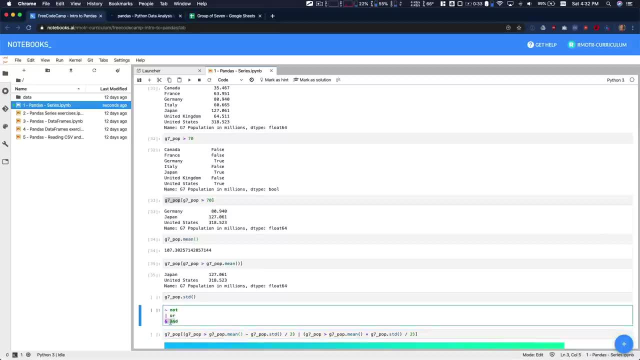 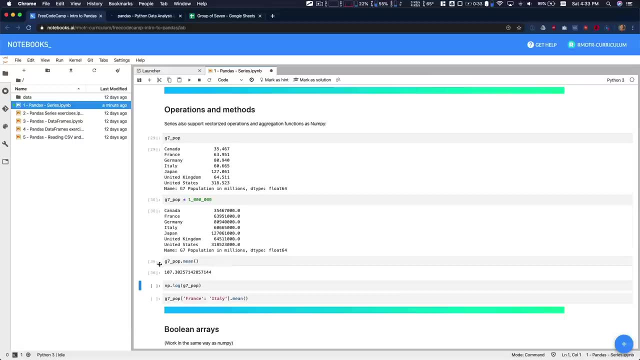 we have before. So they're not the or and the and they all work with Boolean selection as well. The operations we saw from a mathematical perspective mean in statistical operations we saw in NumPy some mean average standard deviation. we were actually using standard. 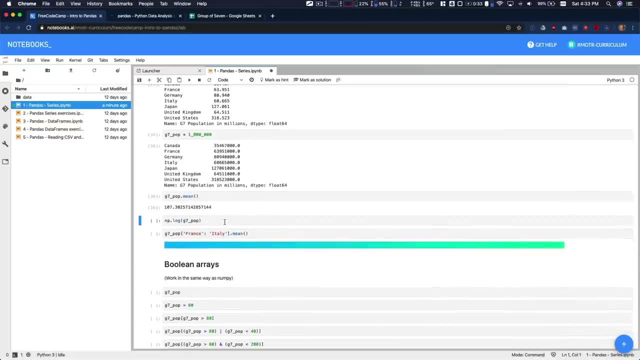 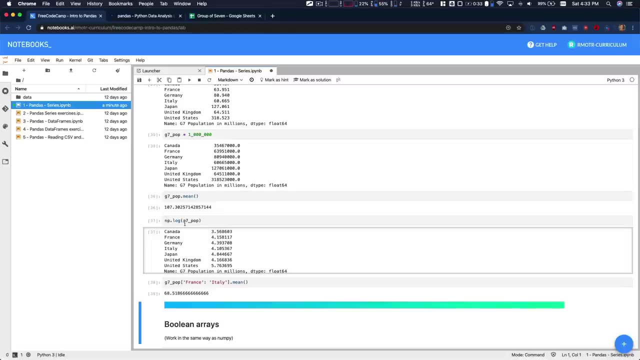 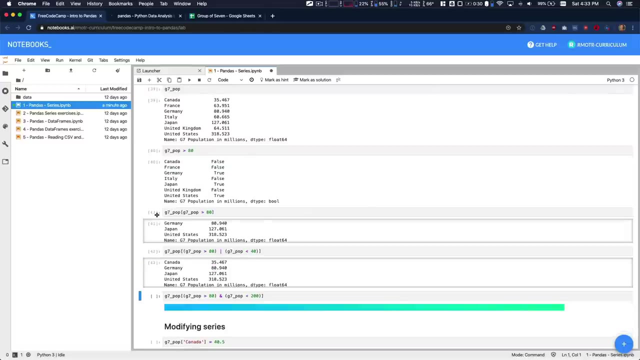 deviation before they're all still relevant in this case. but also you can use traditional NumPy functions with pain the series, because, again, append the series is internally backed by a NumPy array. So this is all the same, as you can see. here's a an example that it's 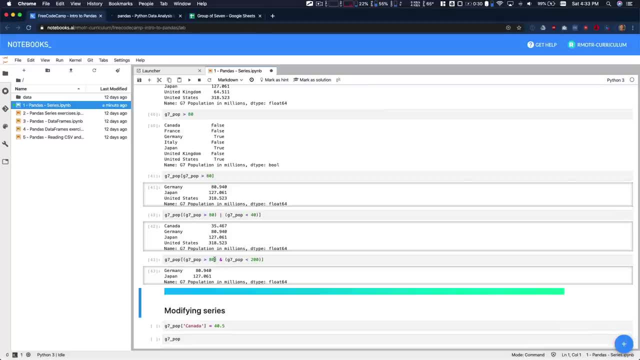 a little bit more clear. we're getting all the countries that have more than 80 million inhabitants and all the countries have less Less than 200 million inhabitants, So it has to be above 80. But it also has to be below 200.. Okay, or in this case we say either above 80, or below 40, or below 40. Right. 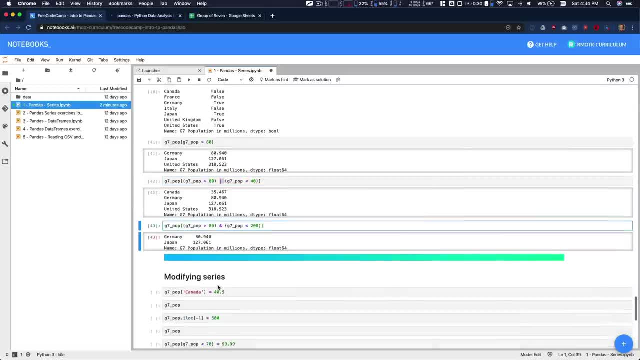 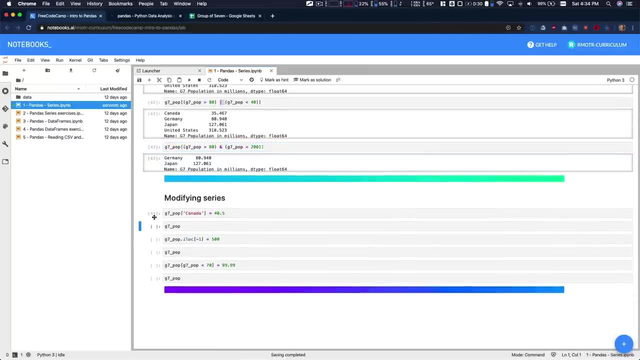 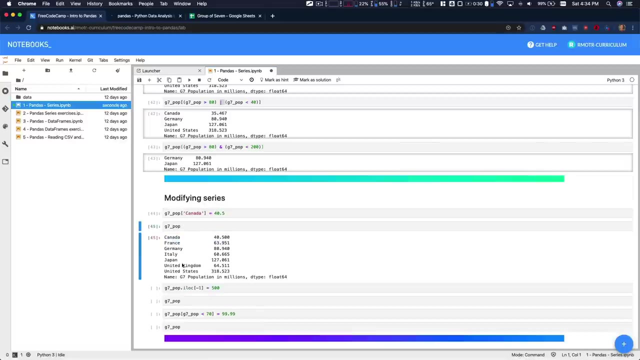 So that's with the or operator or the not operator. Modifying series is relatively simple. Whenever you have a value, you can just assign it all together. In this case we're saying Canada is now 40.5.. I don't know why we just wanted to do it. This is by index. you can. 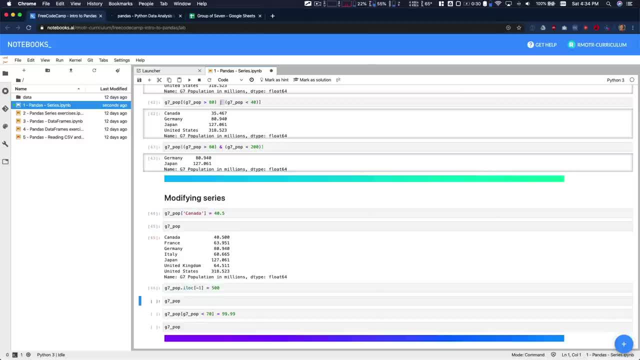 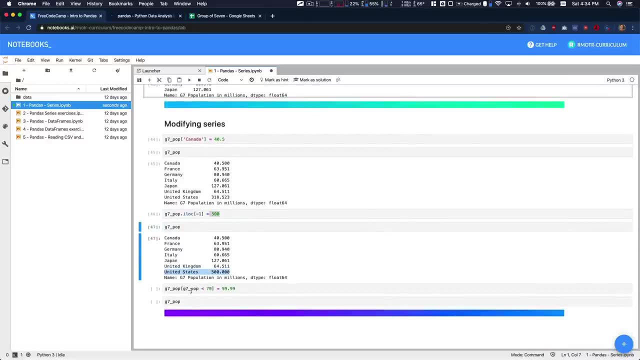 also do it by sequential position. So in this case we're going to say the last country should have 500. Now. So we're going to see right here, the last country has 500. Now. or you can also modify elements based on our Boolean selection So you can say all the 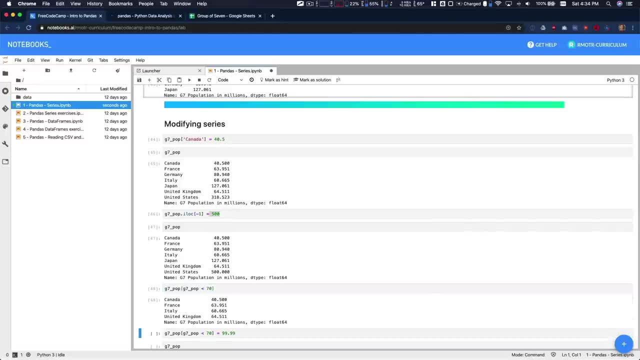 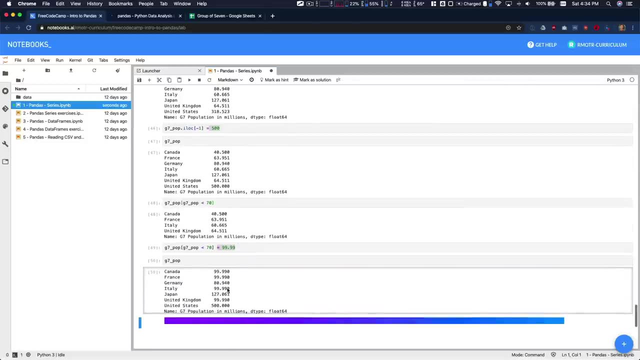 countries that have less than 70 million inhabitants. all these from our previous case. we're going to say 99.9.. Query: all these will now be 99.9.. So, as you can see, it has changed all these countries. So this, the assignment, works by direct indexing or also works by Boolean. 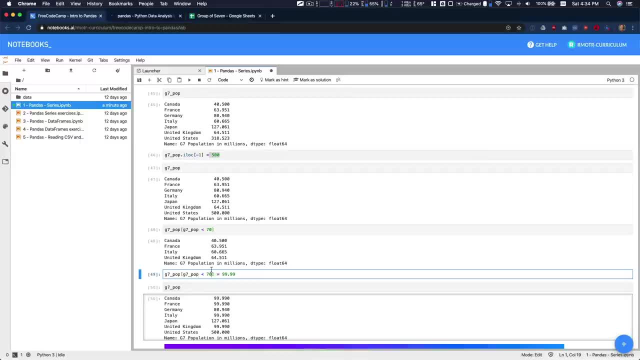 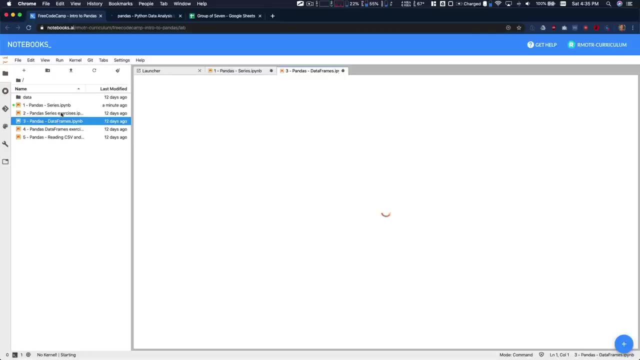 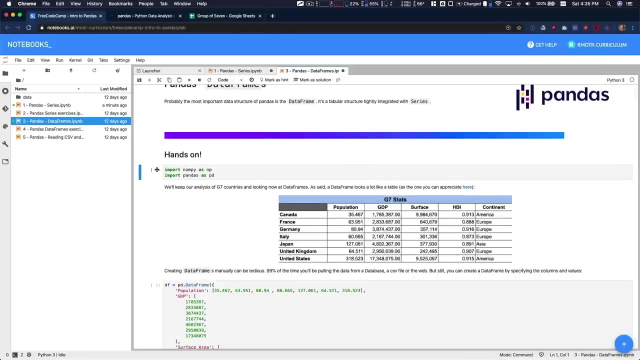 indexing, And this is going to be extremely important when we are cleaning data. So let's move forward and start talking about data frames, not before you have exercises in four series and also for data frames. So our I recommend you to check them out. So, talking about data frames, this is what a data frame 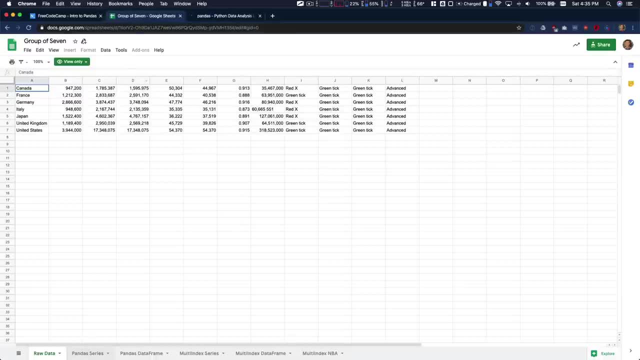 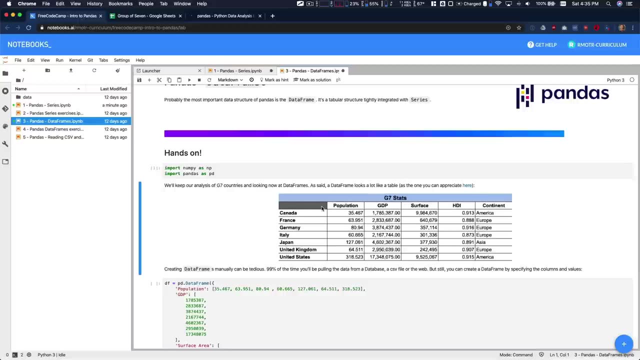 is going to look like. It's pretty much the same thing as an Excel table. So this was our series And this is going to be our data frame. It's a table, So it looks a lot like an Excel spreadsheet And actually it's very common to create pandas- data frames- out of. 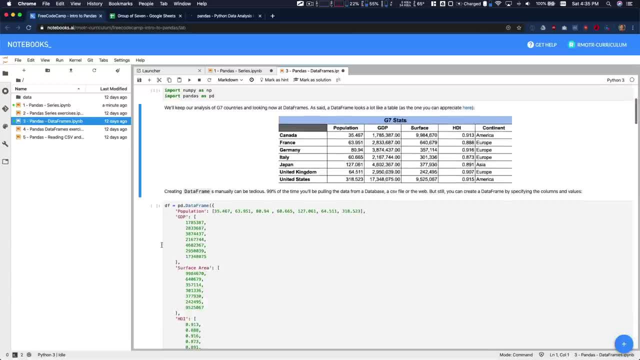 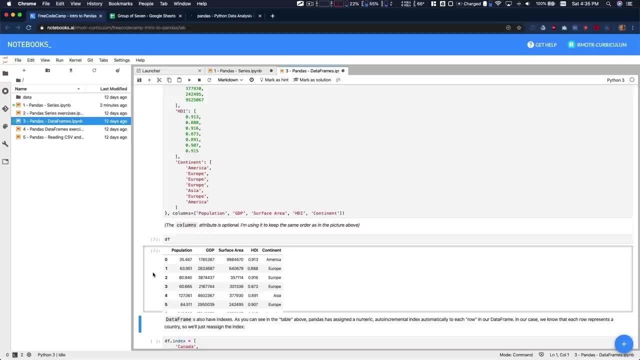 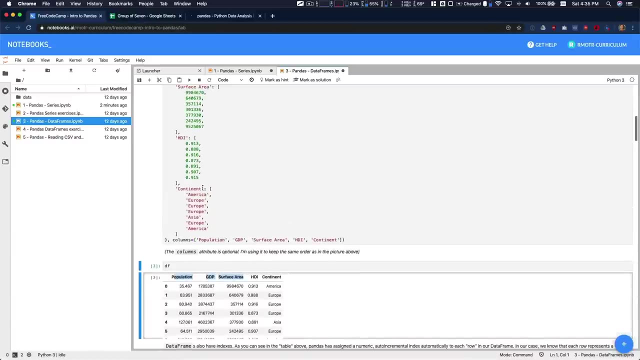 CSV files, which are tables basically, And I'm going to create it. we created with these data frame object and I created, there you go. these are data frame And, as you can see right, it has columns that we have assigned. 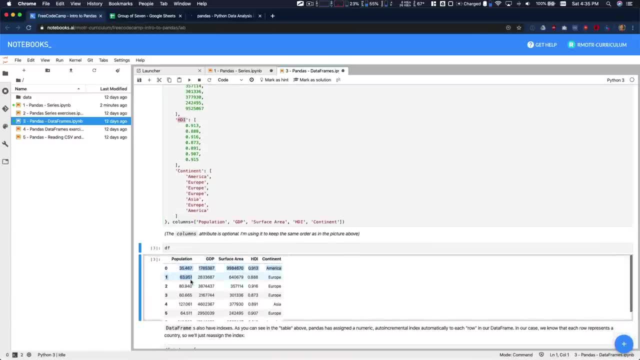 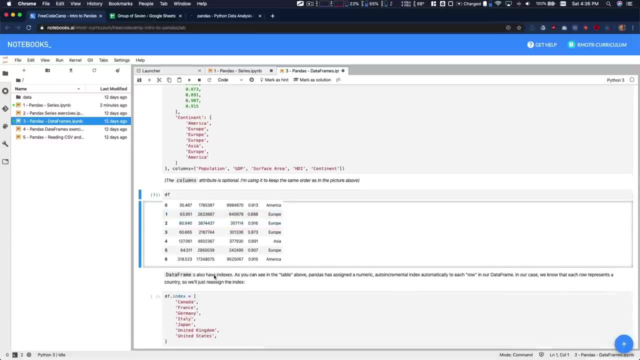 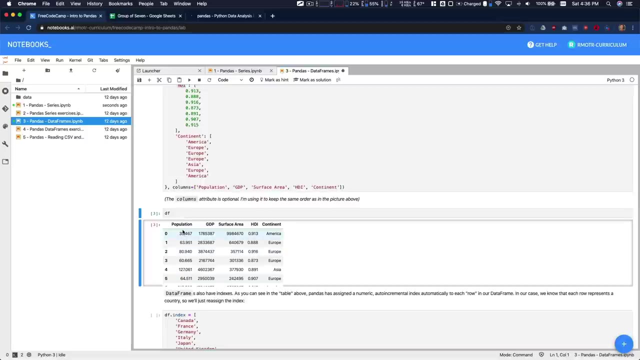 In this case, we were designing the columns And we have rows of values right below each one of these columns. Why What's the similarity with with series and it's not a data frame column? So a data frame will be basically a series, So we can think a data frame as a combination. 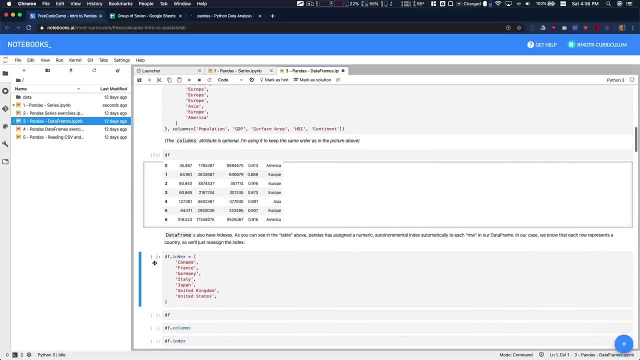 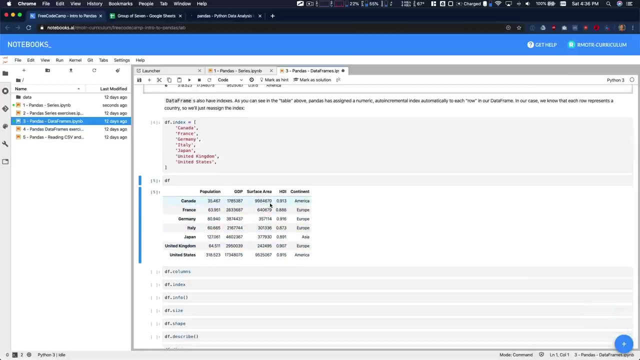 of multiple series, one per column- we're going to assign an index to the data frame, the same way that we did with our series. So in this case this is our data frame. sorry, right here. this is our data frame that has the index right And it has the columns as we. 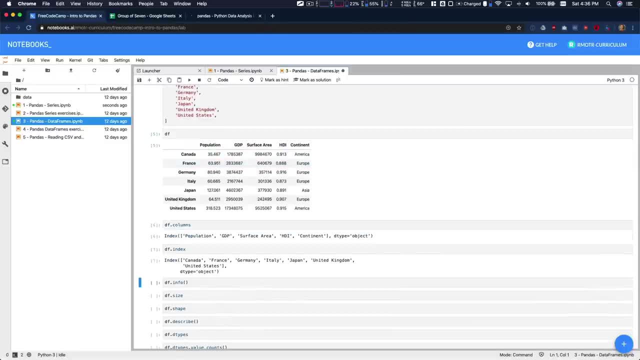 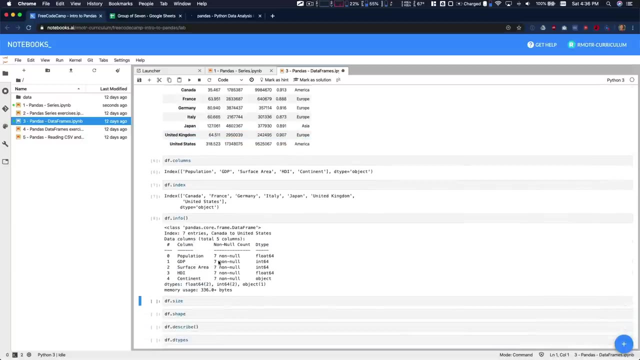 had before? What columns do we have? So what's the index of the data frame? these are all attributes that you can consult. there are a couple very interesting methods from data frames and we use all the time. The first one is the Info method. that's going to give you quick, a quick information about the structure. 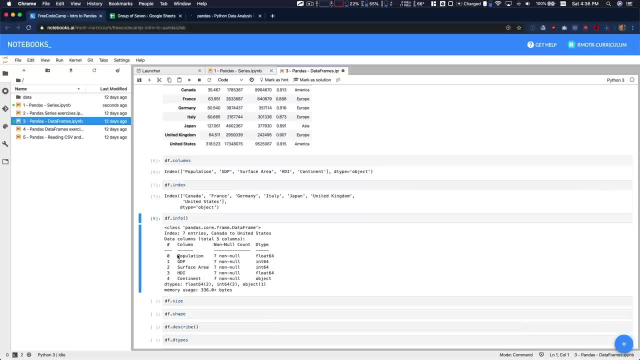 of your data frame right. So it's going to tell you what columns you have: Population, GDP, surface area, HDI, continent on. it's also going to tell you the types and how many no volumes you have. It's actually telling you how many non values you have, So you can. 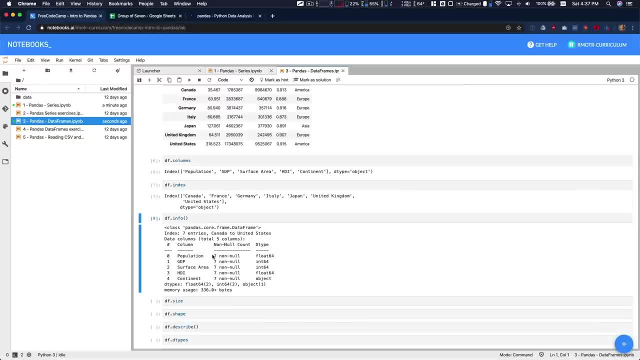 do that information right from the top of your data frame editor. Now, sometimes myывать the refund date is actually: let's see, Look up the content and it's just a nice easy know values you have. But we use this when we're cleaning data to quickly identify those. 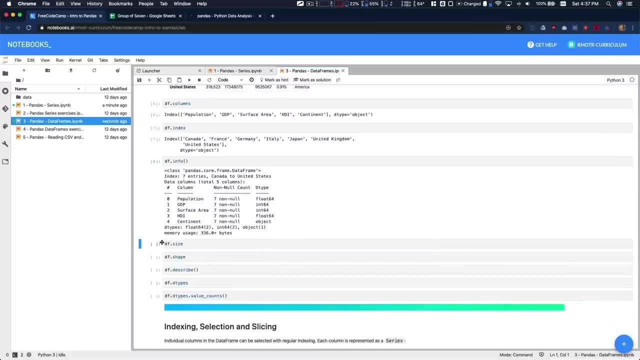 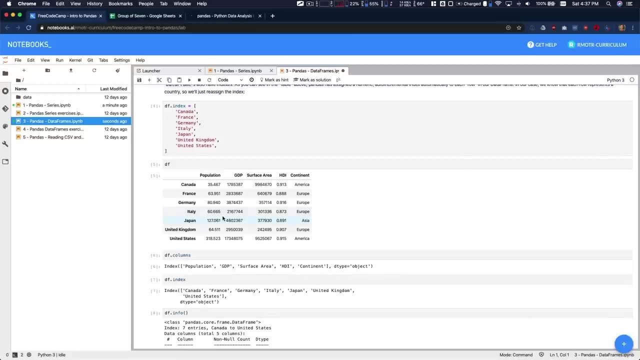 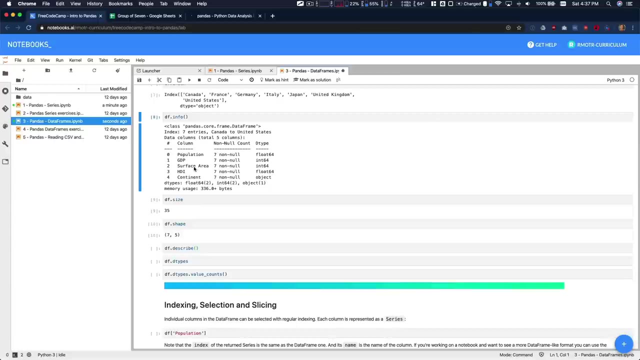 columns and have missing values. we can check for the size of the data frame, we can check for the shape And this is similar to a matrix, right, a two dimensional array in NumPy is pretty much a data frame And also similar to info. that was again to check a summary. 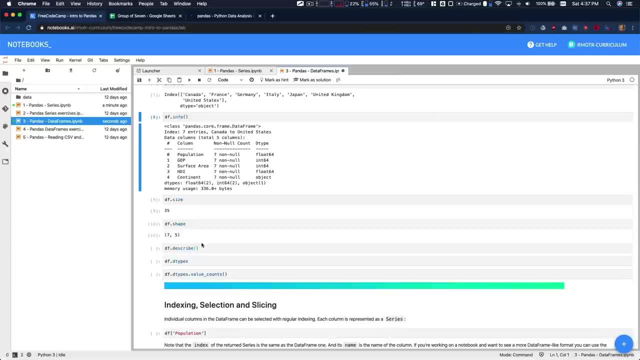 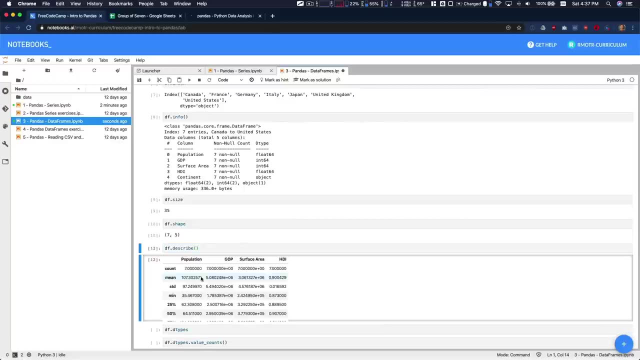 of the structure of the data frame. we can also use this tribe, which is going to give you a summary of the statistics of the data frame, And in this case, what we see is that for each numeric column, only those columns are numeric. continent is not here, for example. 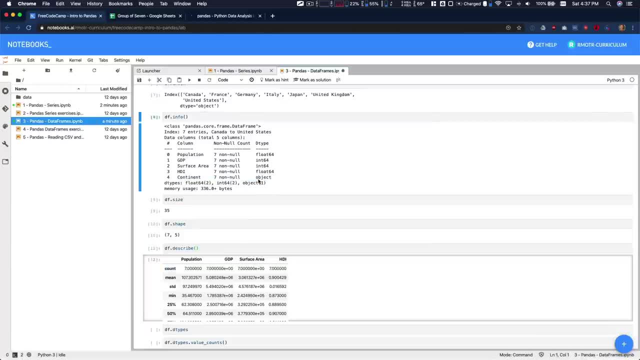 this is continent, So you can see the type is, object is just, is a string, basically all the numeric columns. we're going to have some more statistics for them, So for example, for population, how many elements we have. what's the mean? 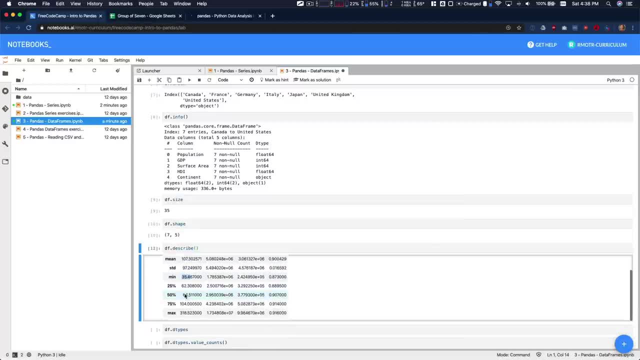 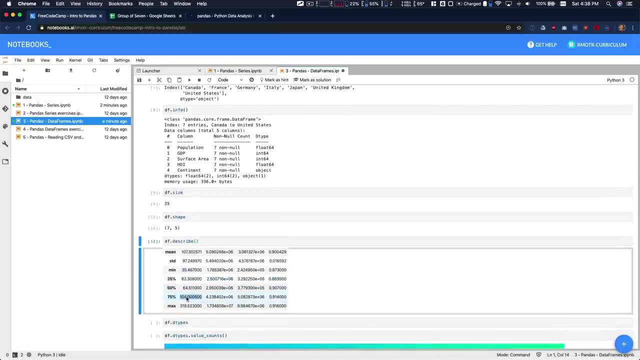 Right. What's the average value, What's the standard deviation, the minimum, the maximum and in between a couple of percentiles: 25th, 50th and 75th percentiles. So this is quick summer statistics And we do these a lot. So keep in mind is crime method is very popular. 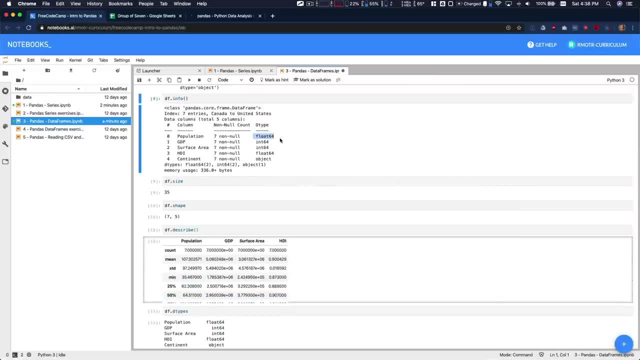 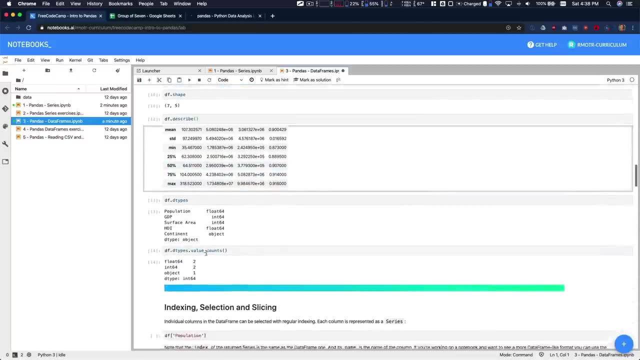 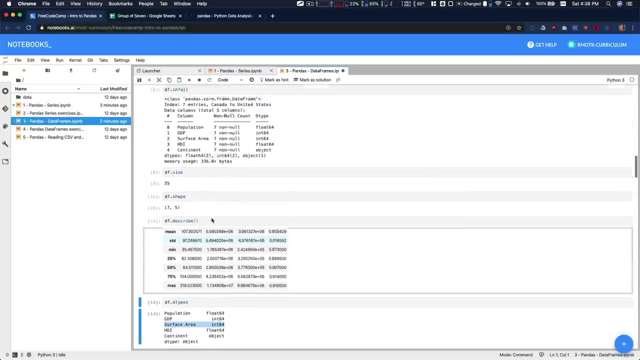 As you could see in the in the info method, the columns have associated types. Okay, so this is very important. The continent is an object. that means that it's basically a string, HDI is a float and surface area is an integer, And that's because NumPy- sorry pandas- is automatically through. 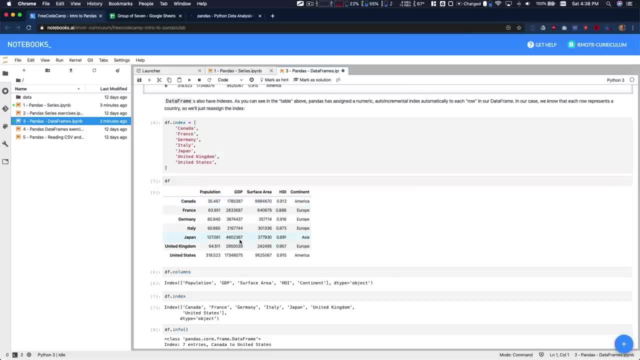 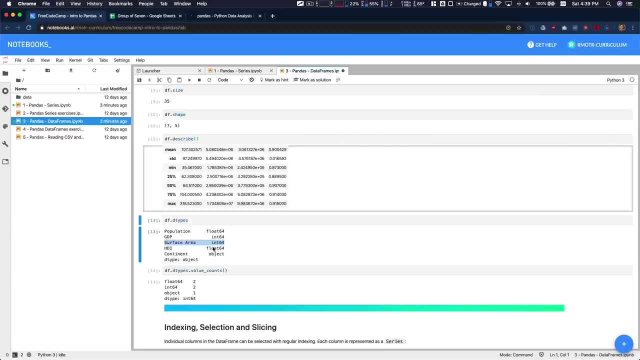 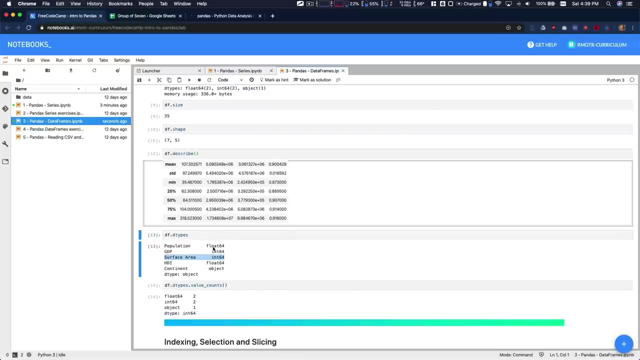 NumPy is automatically recognizing the correct type to assign to each one of the columns. This is similar to what we saw with series, in which the series contain an actual data type. A series was part of a given data type, So that's something you cannot change, And in this case, check checking value. 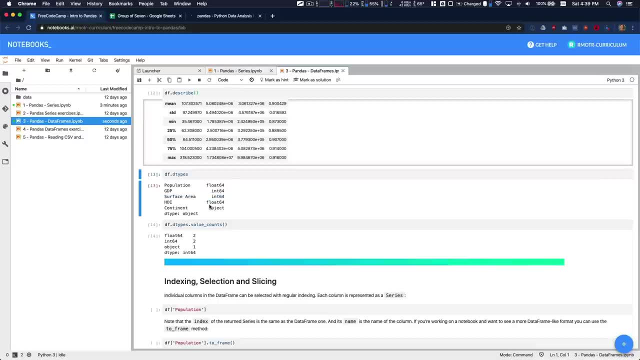 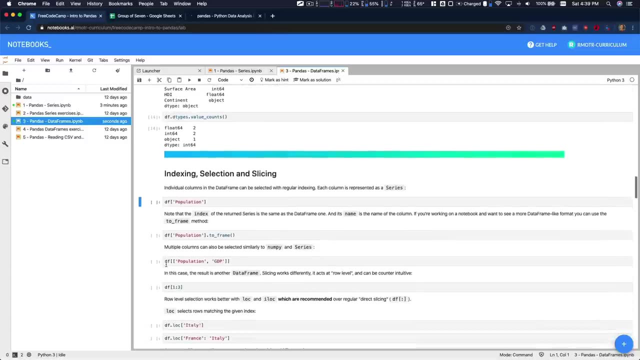 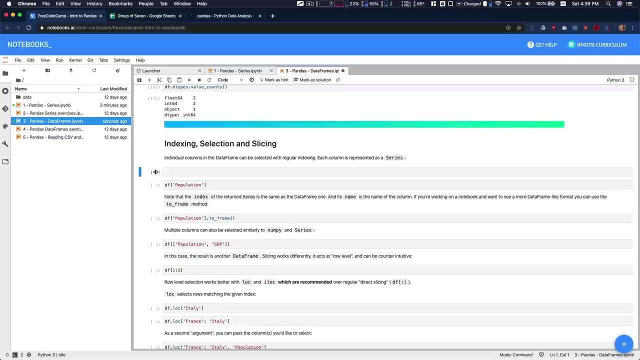 counts, you can have a quick reference of the types of your series. So, moving forward, how will we? we will be selecting data from series. Well, there are a couple of methods, And this is might be a little bit confusing. So what I'm going? 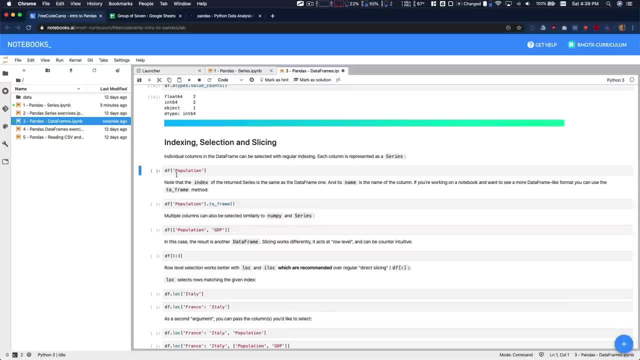 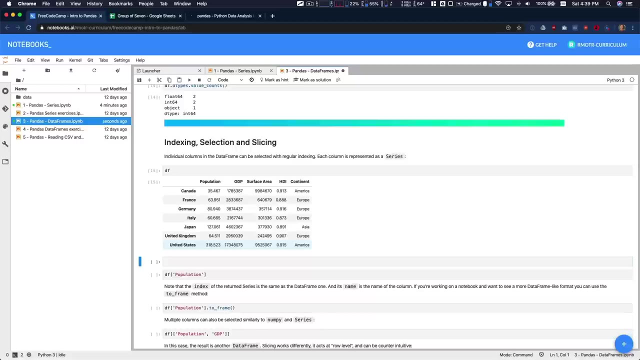 to do is- I'm going to skip and just going to give you a quick reference first And then. then you can read, if you want, through the process we follow here. Given a data frame- and this is just two quick rules- given a data frame you're going to select by index. 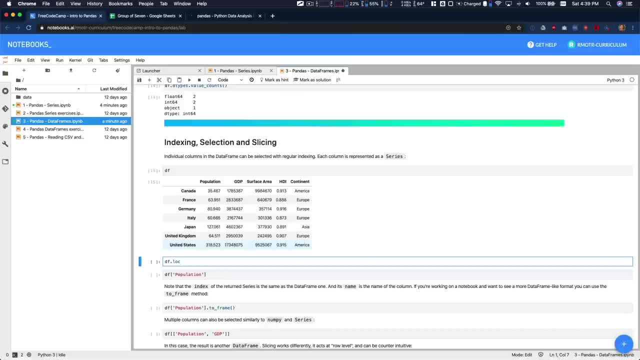 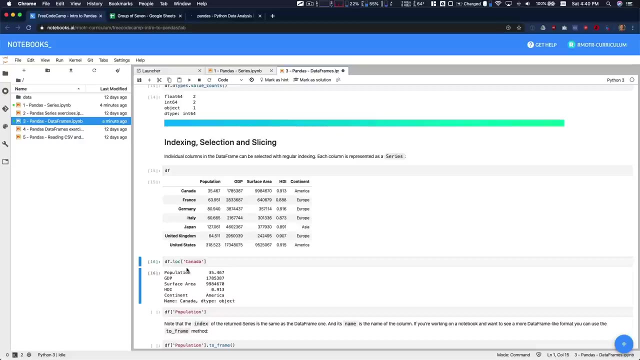 using the lock attributes. So the lock attribute is will let you select individual rows. So, for example, we're going to get Canada, Canada, Okay, that's great, that's the value of Canada. The I look attribute will let you select similar to the series. 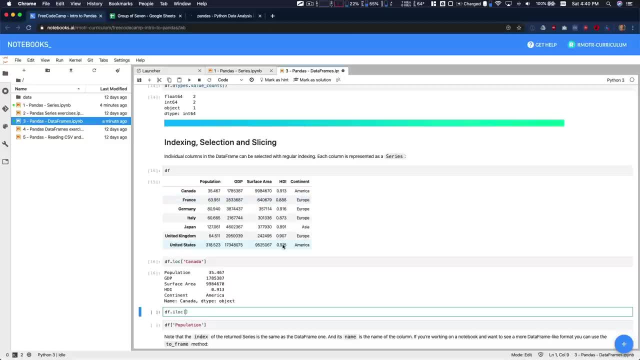 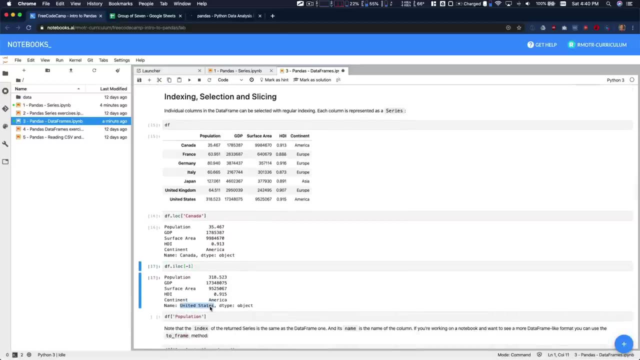 the row by sequential position. So let's say we want to select the last row. In this case it's the United States of America. So again, look, let's just select. select rows by: by index. give me the row under this index. I look, will. let you select rows by sequential. 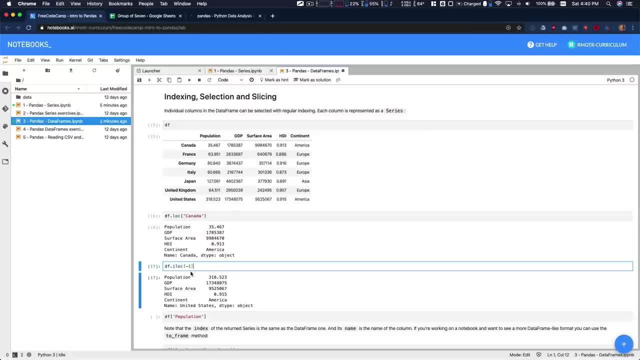 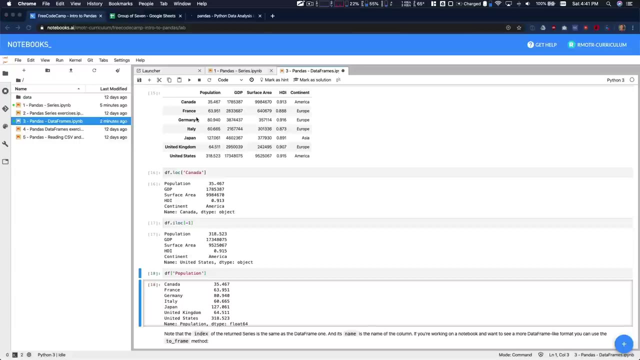 position. give me the last row, the first row, the second row, etc. And finally, without using lock, without using I look, just by saying df, at something. you are selecting that column, give me the entire, give me the entire column population, right here, the entire column population. 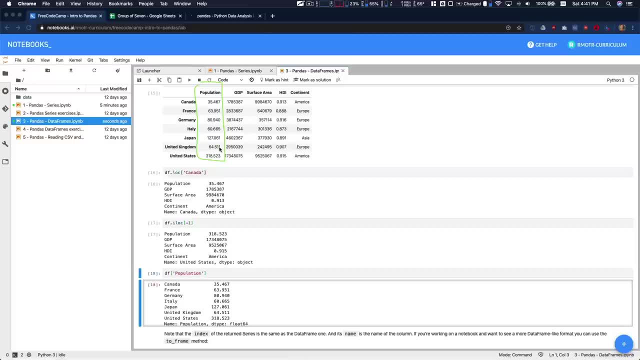 So what you're saying here first, first of all, this is a quick reference. dot dot lock will give you an element by index. I look will give you an element by position, a row by position, And just doing df at something is going to give you the element: the column. 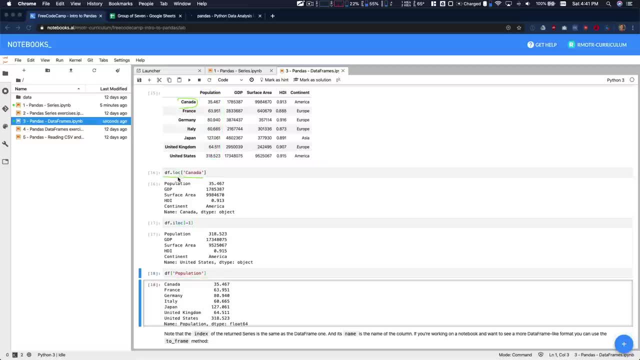 sorry that you are passing. So it's like both look and I look, look and I look. work in a horizontal matter. Give me this, While df at whatever works, you know, in a vertical model. just getting you a given. 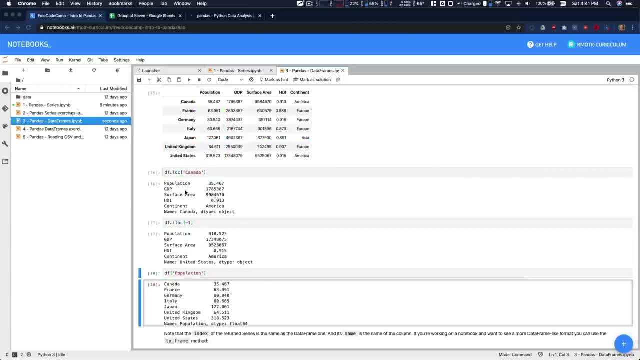 row. But something more interesting here is that all the results- this one and this one and this one- they're all series, what are being returned, our series. So that's what we saw before, And the way it works is first, if we focus in this last example, we're going. 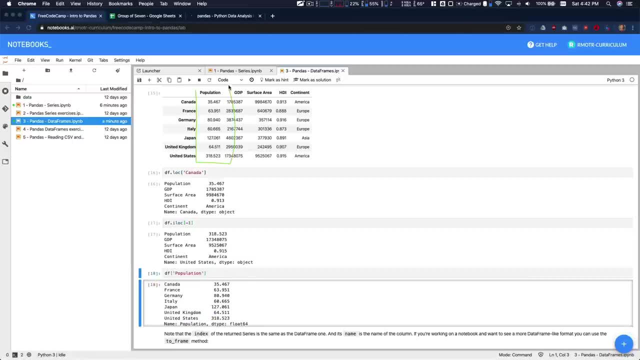 to see that it's pretty standard. There's just these series right here was is one return, And remember it has a type and everything. So that's, that's fine, If, if we ask for a row, like in this case, we 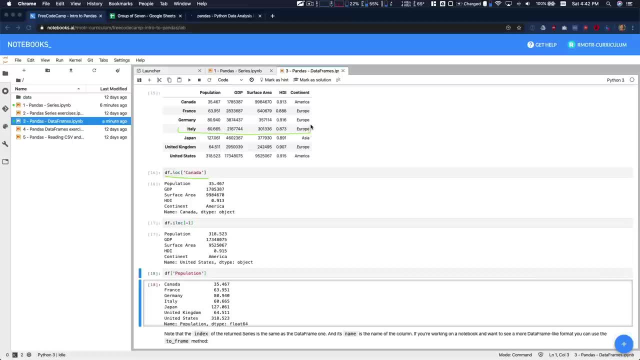 can get, for example, here, Italy, There you go. The result is also a series, But what you can see here is that this thing is kind of transposed In a way that here was the values of the series. Population is here And GDP is here. 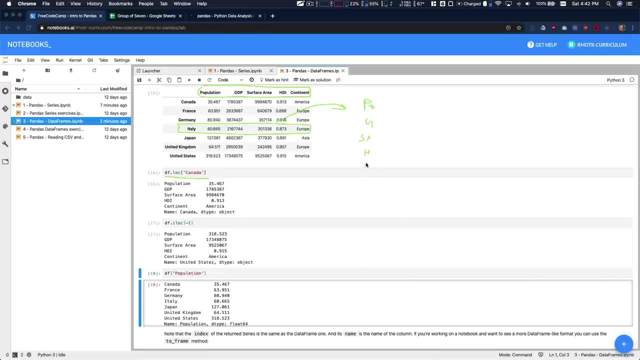 and surface area is here: HDI on continent. and here you have the values. So it's again. it's being transposed right from vertical to horizontal in a regular series manner. On the index of the series is extracted as the name. 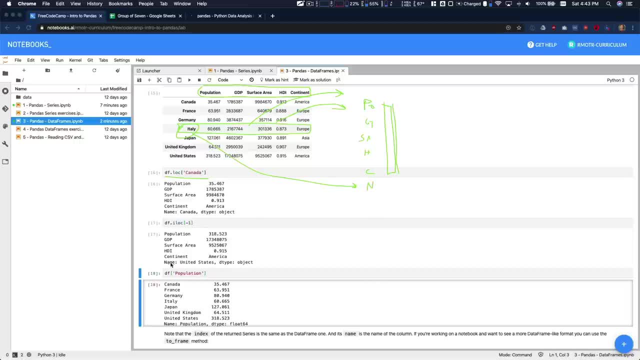 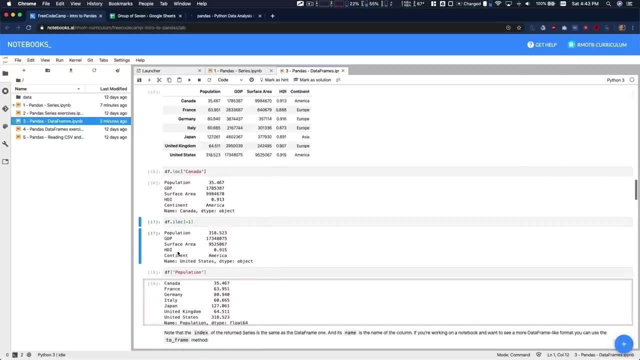 That the, the column hot. So in this case the name right there is the value of the index that it had. So you can read more about it right here. But I just want you to remember these rules. dot log is like by index, dot i log is like by sequential position, the F at something. 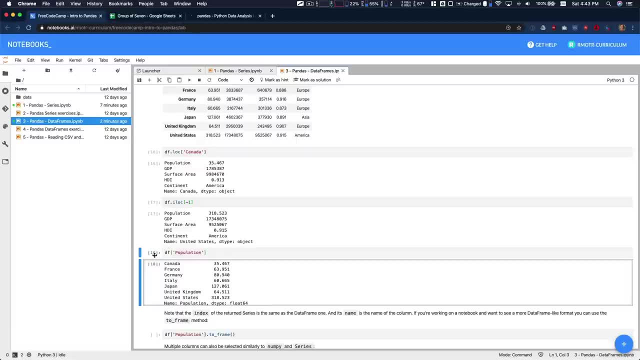 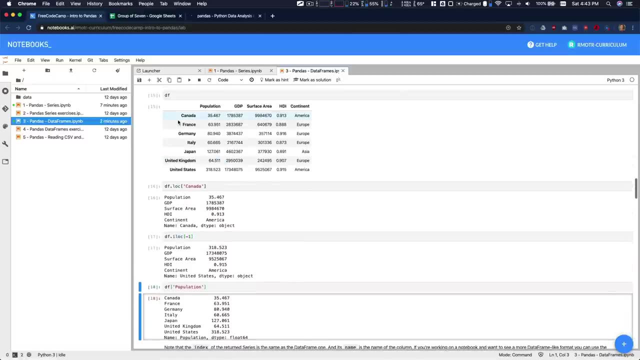 you go by column, there are times when these might not apply, So or not want to apply. there will be some issues. So, for example, if you're rose, if your index is numeric, you might have issues with these form or that form. Just respecting these three for now. 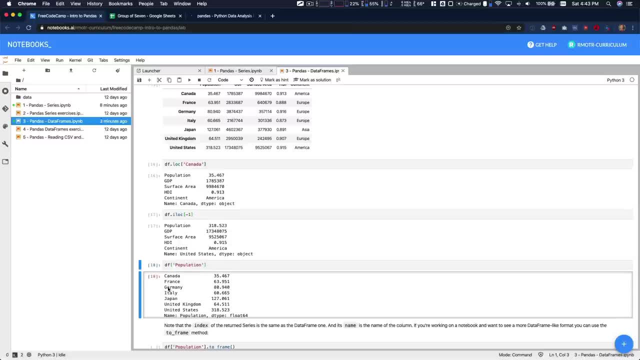 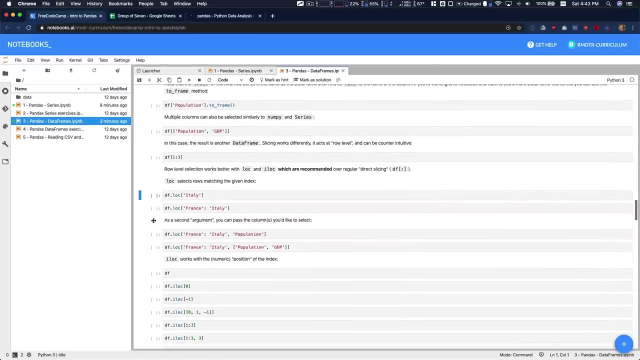 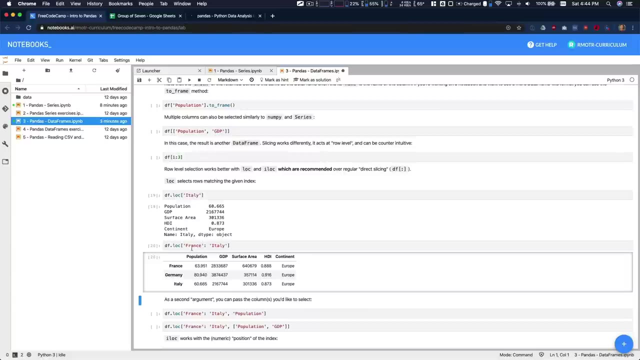 it's going to get you any elements you want to get, either by row or column. So, from what we've seen, the oldest slicing also works as expected. So we can get, for example, Italy, or we can get France up to Italy. So the upper limit is included. 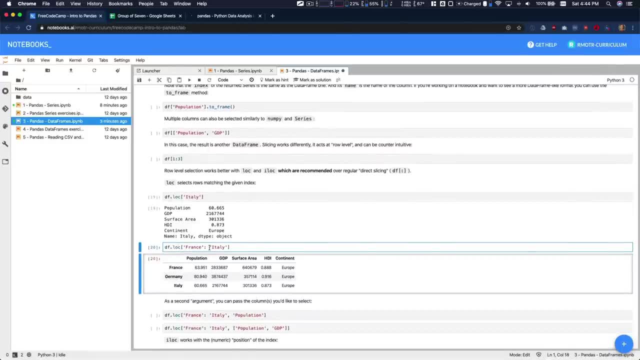 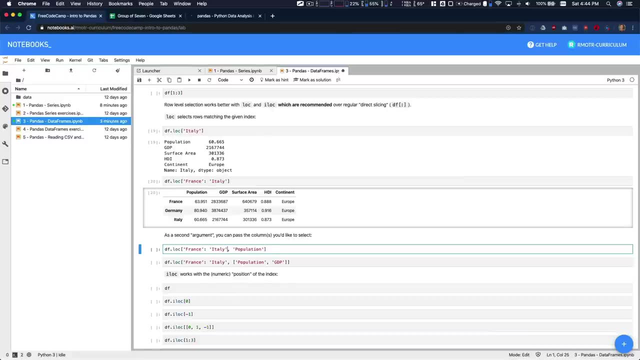 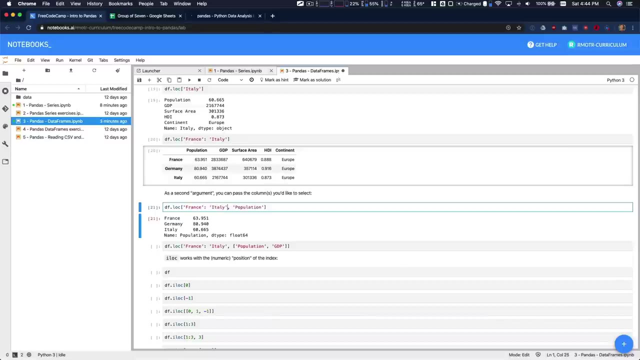 But again it's dot log and we selected by indices from France to Italy. We can also do the second dimension, similar to the way we worked with NumPy. we can do second dimension here And we can get all the countries that are from France up to Italy, including Italy. 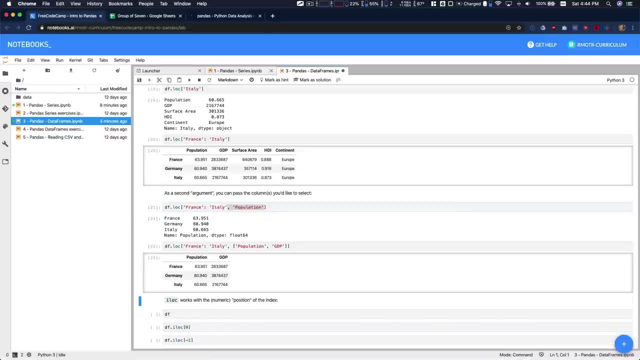 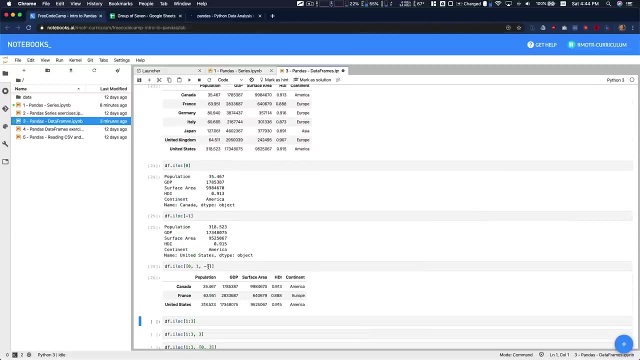 but only the population column or population and GDP. So here you can see this second dimension being applied at the concept of of multiple dimensions in selection being applied also to payments, For I look it works in the same way that in that, the multi index and the slicing. so 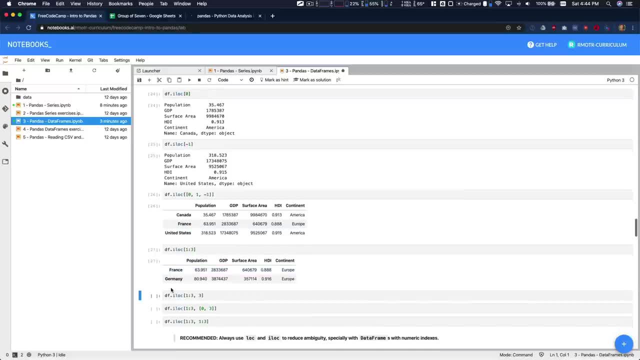 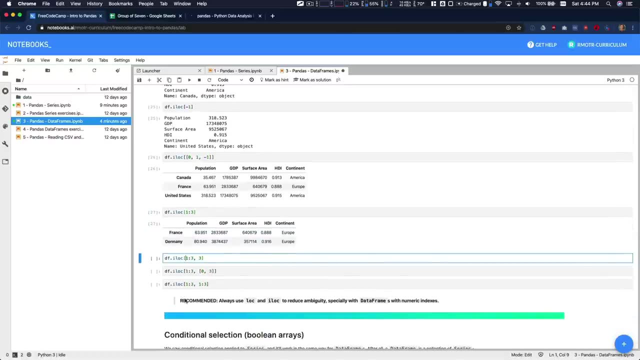 we get, for example, from one to three right in sequential positions. In this case the upper limit is not included. So that's another difference from what we have. And we can also do multi dimensions. we can say: give me the countries from 123.. And the column should: 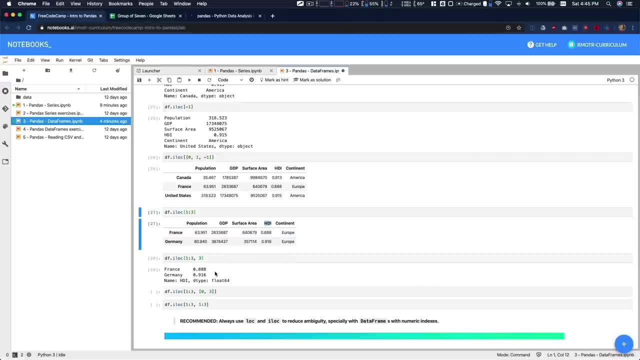 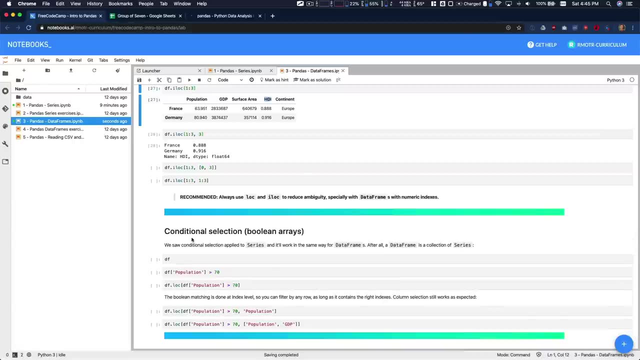 be. 0123 should be the third column. Now the fourth column, the column under index three, which is HDI. So that also works as expected And again recommended. always use lock. I look to select rows and just use the naked data frame to select columns, as we saw before. Now moving forward: conditional. 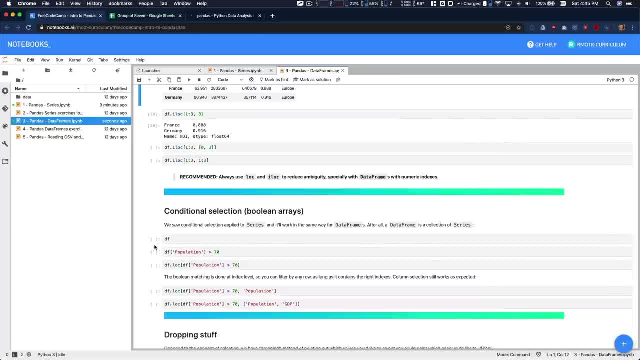 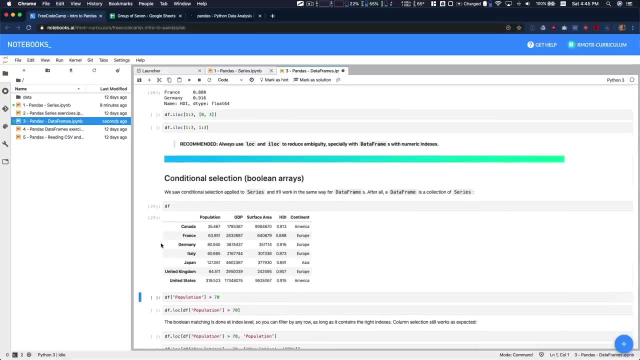 selection, Boolean arrays, Boolean series, whatever you want to call it. This also works for data frames, And it's very important. It's a way to filter data. it's a way for us to consult data when the when we need it. So in this case, what we have is: we want to. 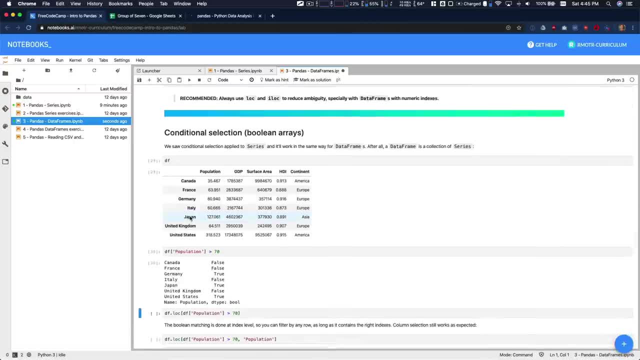 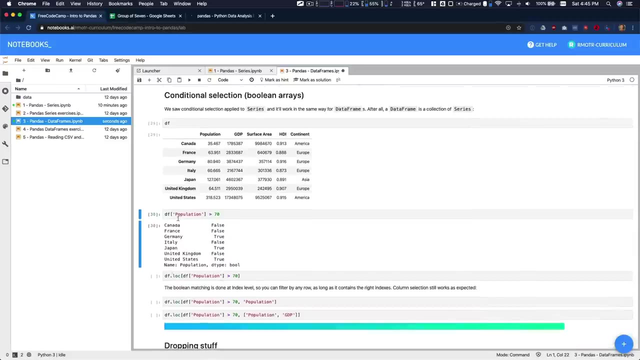 select all those countries which the population is greater than 70. Okay, so all the countries that have more than 70 million inhabitants. similar to what we were, we did with a series, But in this case we want to do it with the data frame. So what you're going to see here, 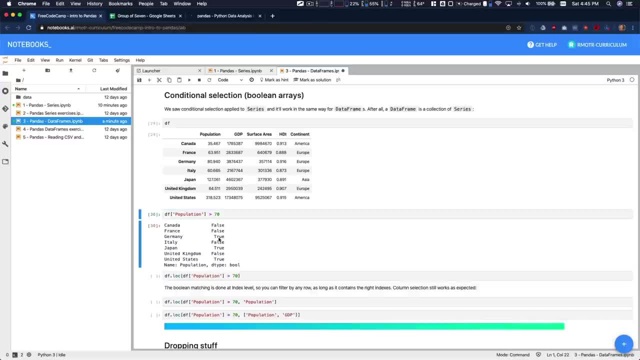 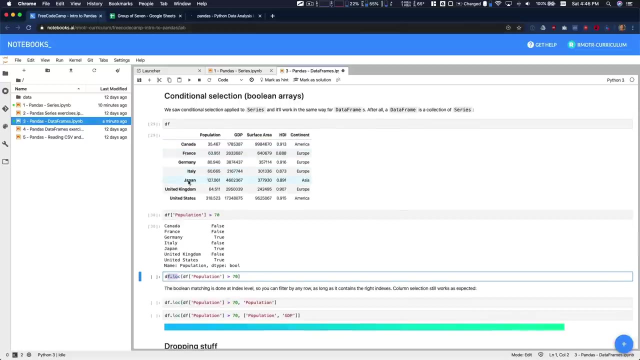 is that we're going to construct a Boolean series, as we did in our previous video, right? So we're going to inject that result 70, false, false, true, false. And we're going to inject that result, that Boolean series, in a dot lock selection. give me all the countries which. 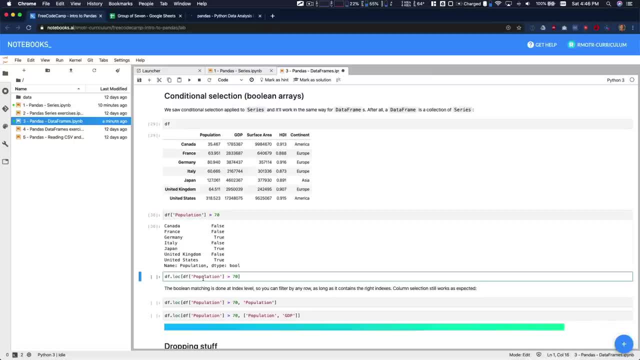 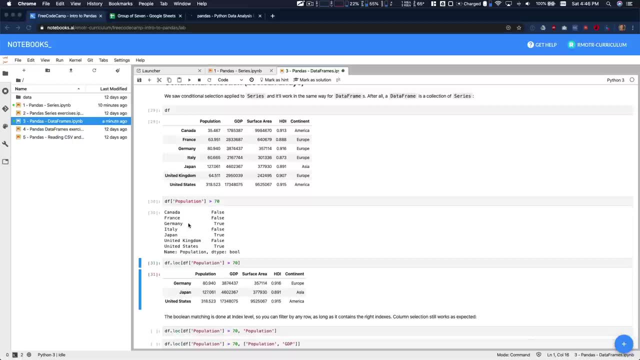 much here than the true value in it And remember just this is kind of a mnemonics or a way to remember. the way pandas knows how to filter things is by matching this index right from the resulting series with these index of the resulting data frame. These are: 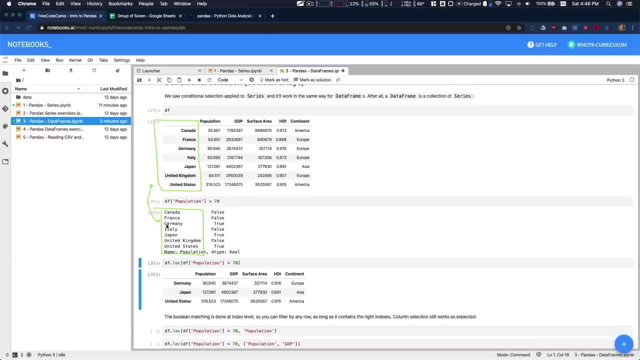 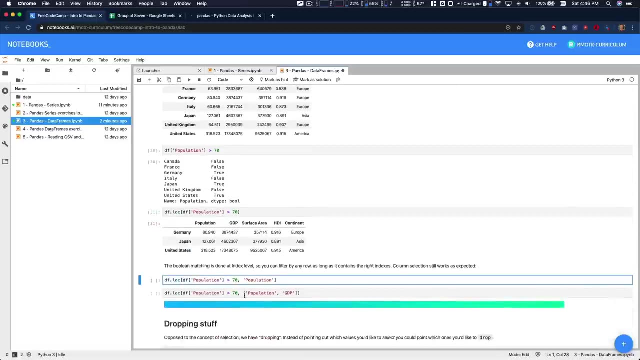 two different objects. they are completely different objects, but their index much. So. here Japan match Germany match. So here Germany and Japan, they are the same, And that's why that thing is working as expected. This is just the first dimension, which is: 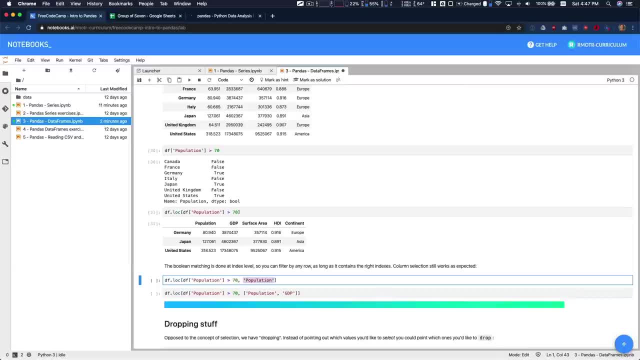 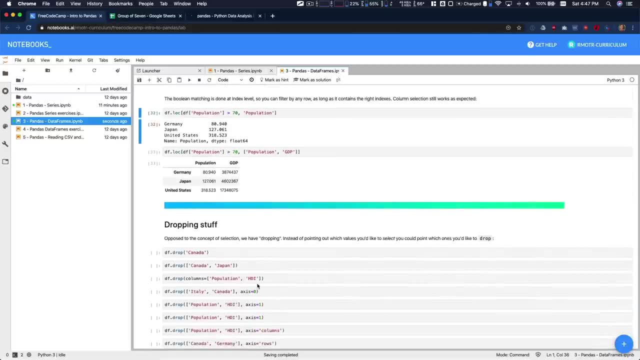 give me these rows. you can also pass second dimension, saying: give me the index of the column or these columns, right? So that's still. that still works as desired. So what about dropping stuff? you can say: whenever you have a data frame, you can say: give me. 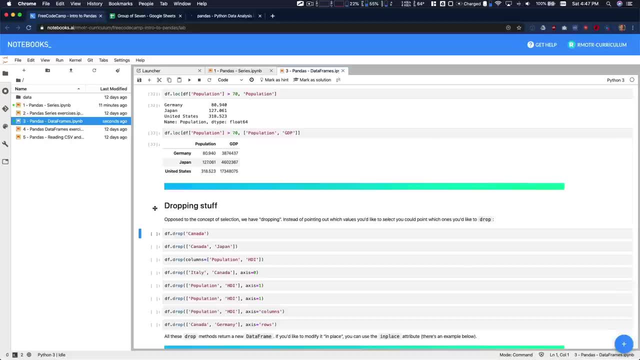 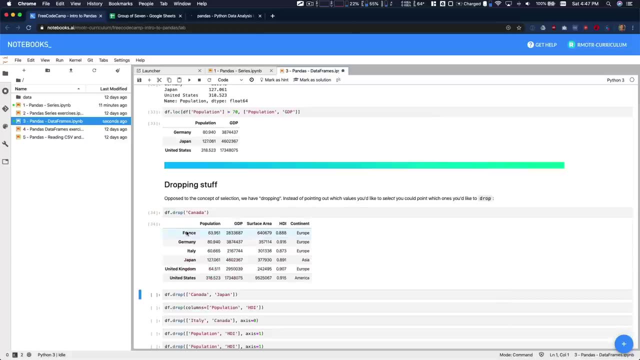 just these pieces. or you can say: drop the others. right, It's just pretty much the same. Dropping is very simple. you can drop by index, drop this value, drop Canada altogether, period or drop these indices: Canada and Japan. 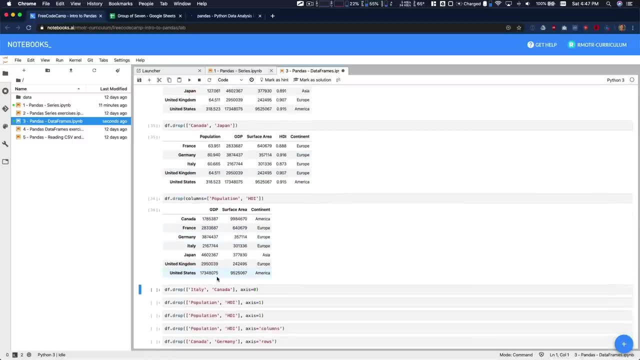 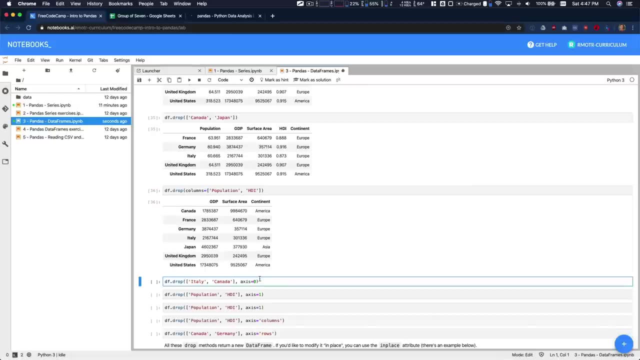 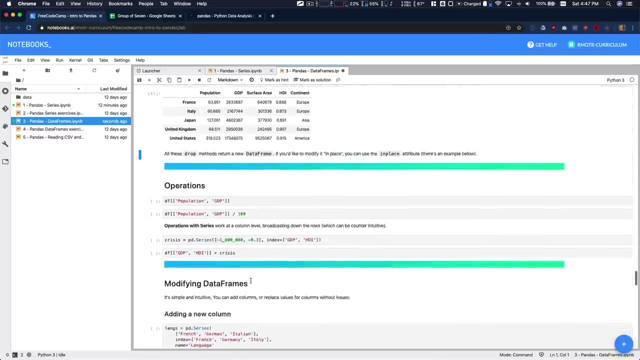 Or you can also drop columns, drop population and HDI as columns. These ways also have a more advanced usage, which is, with the axis, similar to NumPy. I don't recommend them so much, But you can still use them and see them in here. So all the operations we've seen so far, they're. 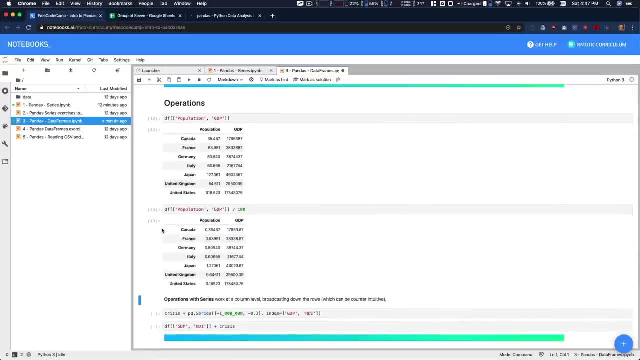 all working. The most important part here is the broadcasting operation that we're going to do between series. So we're going to create a new series crisis and I'm going to show you what it looks like. So we have here crisis And we're going to 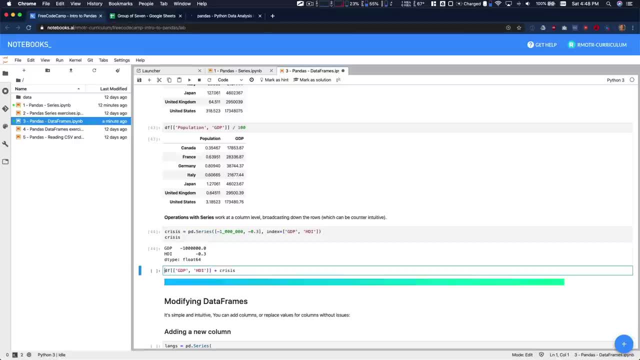 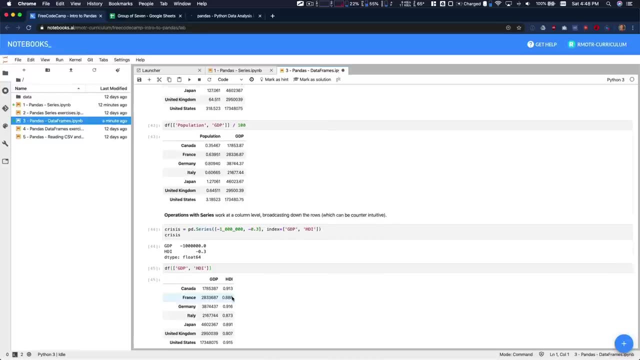 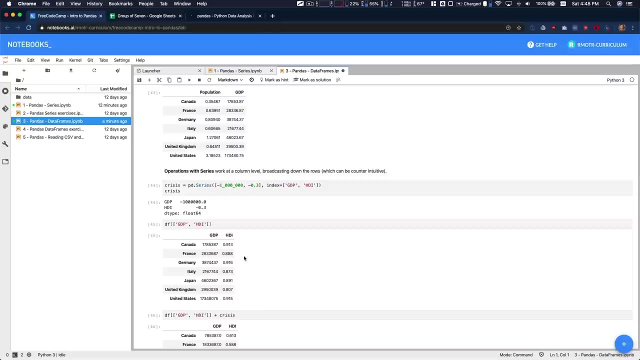 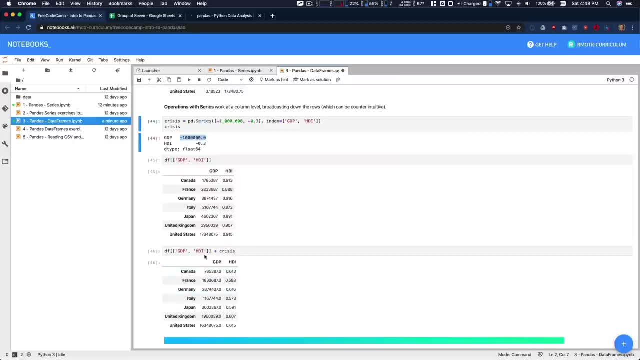 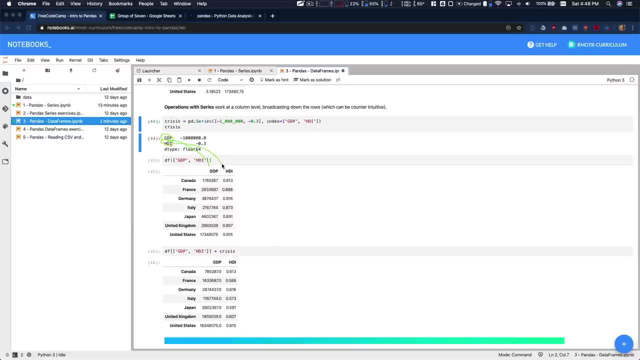 matched with these GDP and the HDI is matched with these HDI. So there are two different objects to independent objects. the series and these data frame here, But when we compare, combine them with an operation like this: the- the columns in this case are aligned- GDP. 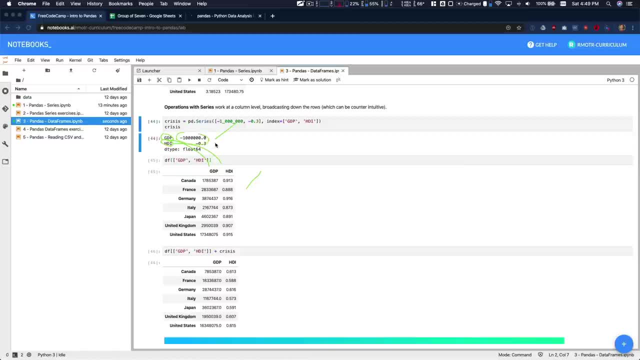 and HDI and they work together. So the you're going to subtract these value in all these column. let me remove this. you're gonna subtract these value in all this column for all these values. I'm going to subtract these value here in these column for all these values. 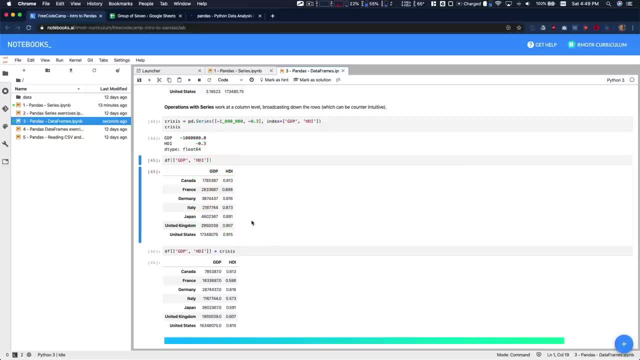 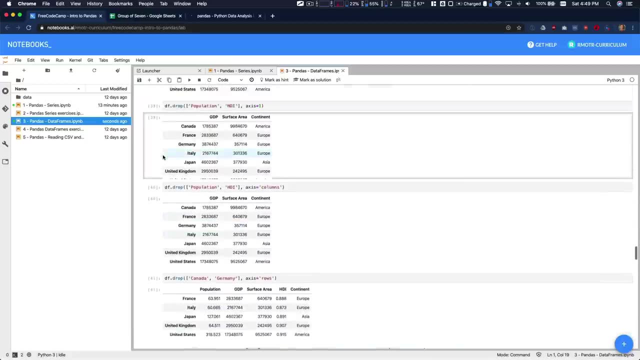 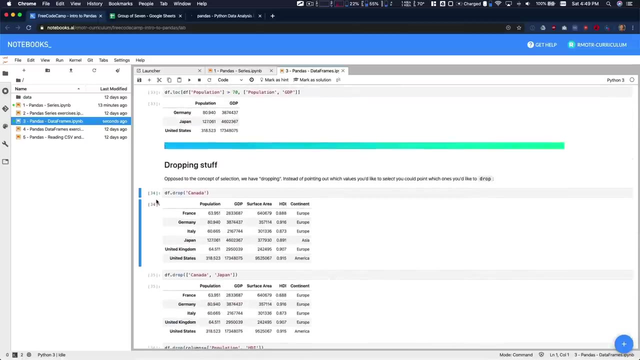 That's the way it's going to work. So moving forward. what about modifying data frames? they want to. I want to show you something, And it's when we were dropping stuff before we were not actually modifying the data frame. So here we did, df, dot, drop Canada, but the 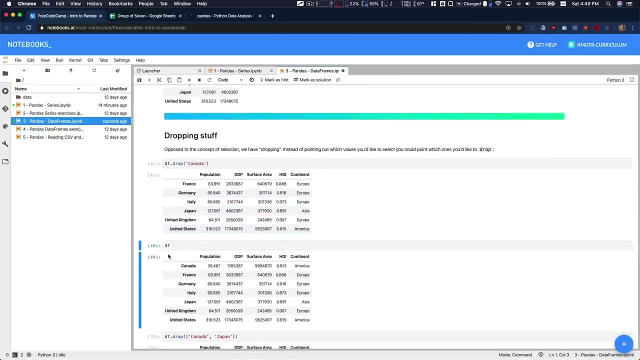 F steel has Canada in it And that's because, similar to what happened with numpy, These operations are all immutable. They are not changing the underlying data frame we are storing. we are storing, we're creating new data frames that store the result of the given operation. So in this, 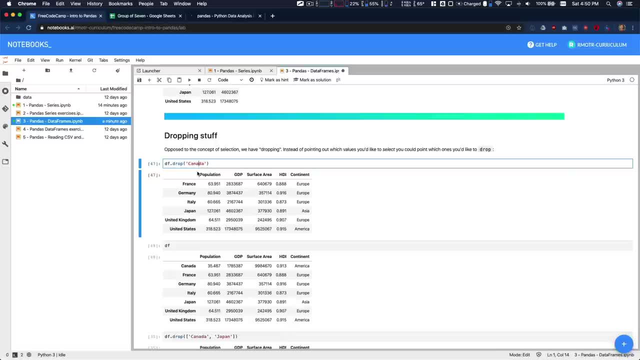 case you have to drop Canada. the result is that the this new data frame, but the underlying data frame is not changed. That's because, again, they are immutable. operations: 99% 9.9 operations in pandas: it are immutable. there are ways to change it. there are ways. 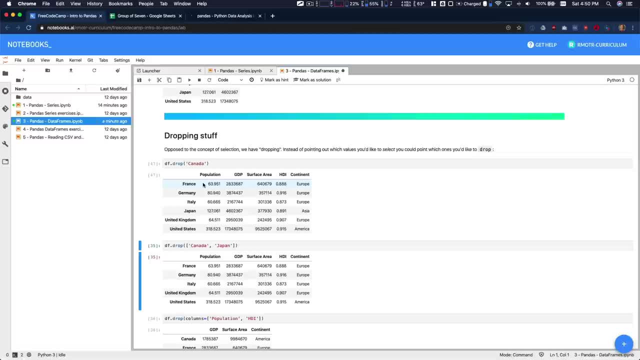 to make the changes permanent, But for now, I want you just to think that everything is immutable. Whenever you want to perform an operation, it's going to create a new series. If you wanted to keep track of this, you will just need to do something like df two equals. 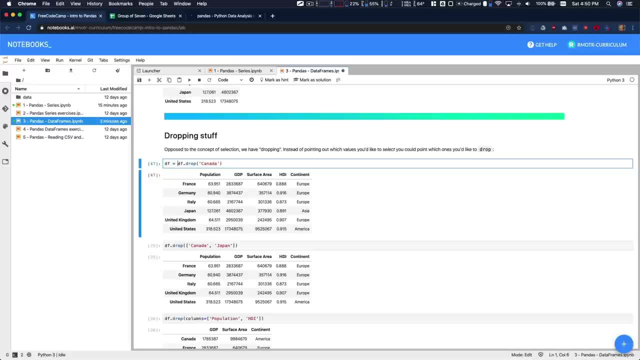 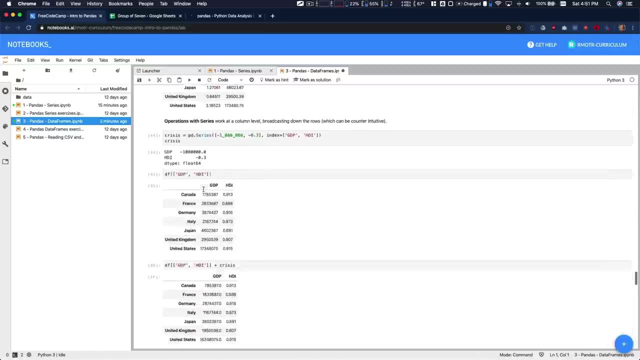 that, or even the F equals, you know, just to modify the current data. Again, there will be a way to not do that, But we're going to save in a second. So modifying series more explicitly, that, I'm sorry, modifying. 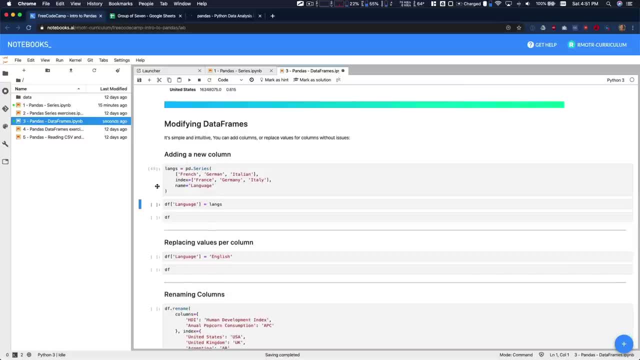 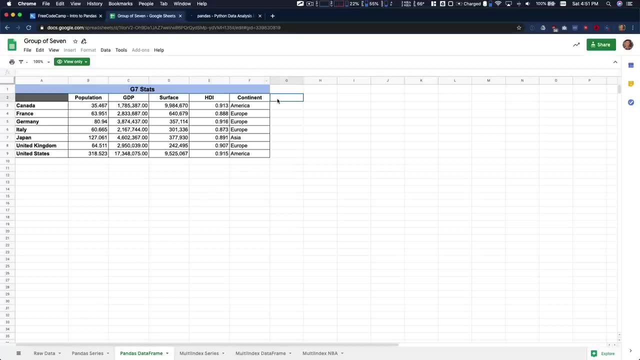 data frames more explicitly. how can you create a new column? Well, very simple. I signed the column as it is say in this, this column, right here. it's similar to say here language, Oh, it's just read only. But if I say, language equals and I can just write whatever I want. 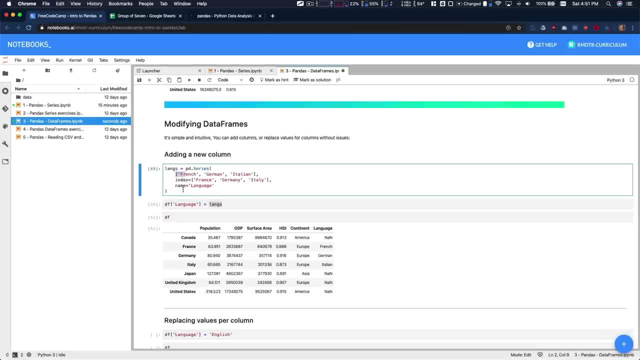 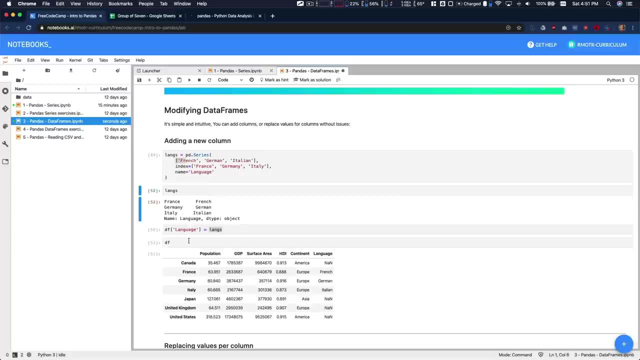 In this case. what do we do? What we've done is that the language- let me show you what links had In this case- was a tiny series. it didn't have elements for all the indices in the data frames, But that doesn't matter. pandas will match all the indices that actually exist And it will leave. 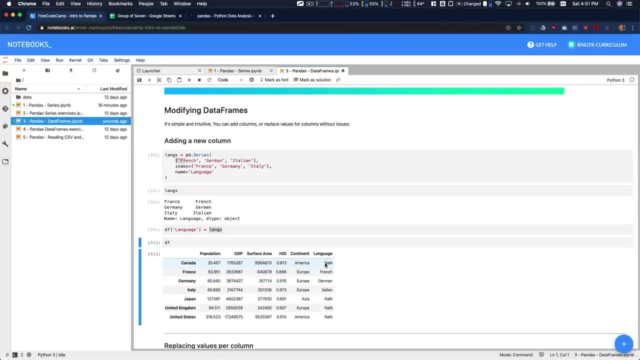 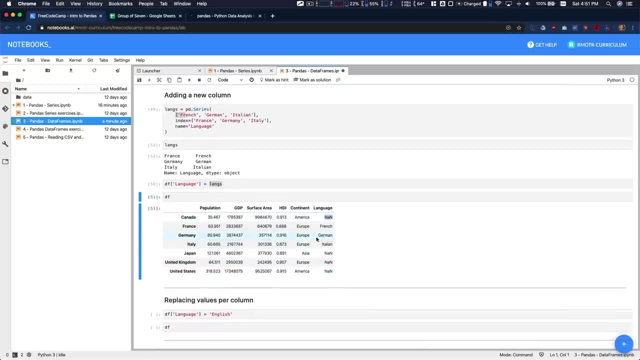 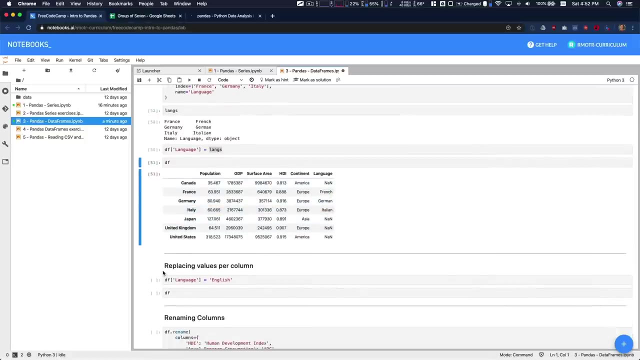 blank. the rest, This nn is what we use for a blank. it's a, not a number from Mumbai. we're going to talk more about it when we start doing cleaning data, data claims, Sorry. So again, links: friends: Germany, Italy. you can see the values are all up there. What happens? 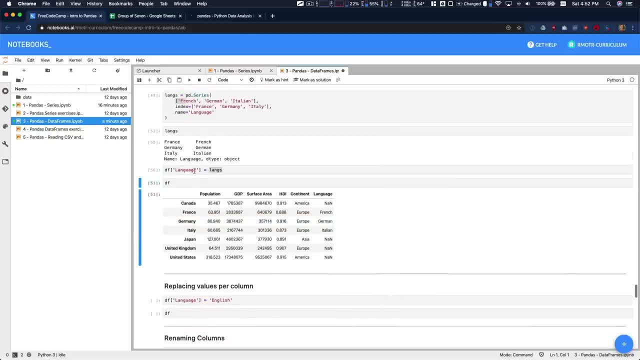 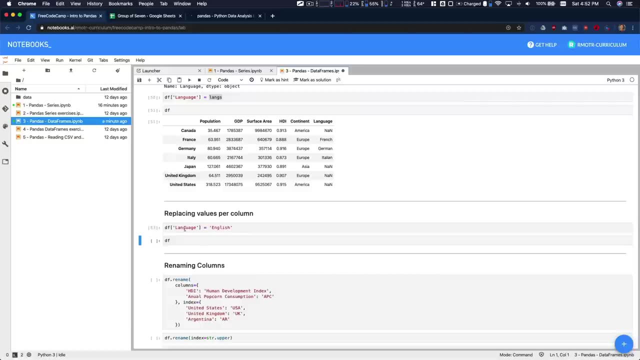 if you want to change a value, the language series already exist, you want to change it. or column already exist, you want to change it. So in this case we're going to say DF language equals English. So we're going to change it all together And DF now will be. 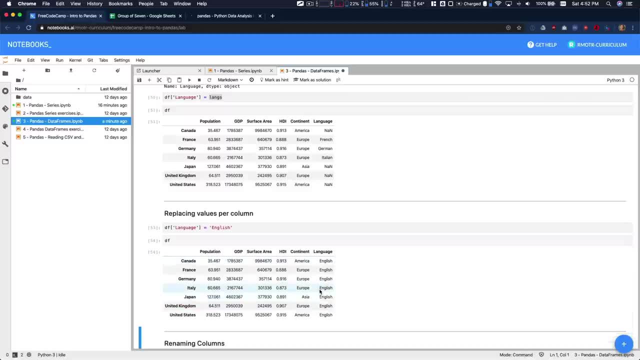 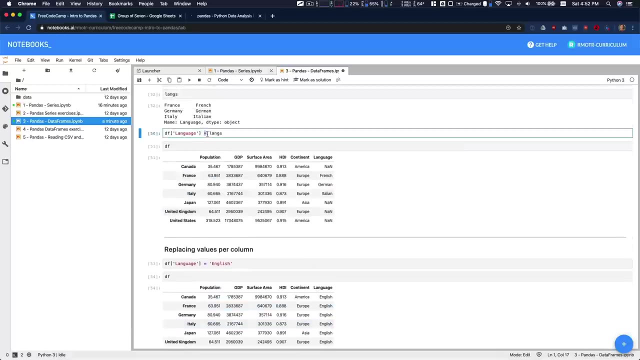 affected And all the values of language will be English. How can you relate, How can you realize when there is an operation that is changing the underlying data from the underlying series or the underlying numpy array? it's usually when you have an equal symbol, remember. 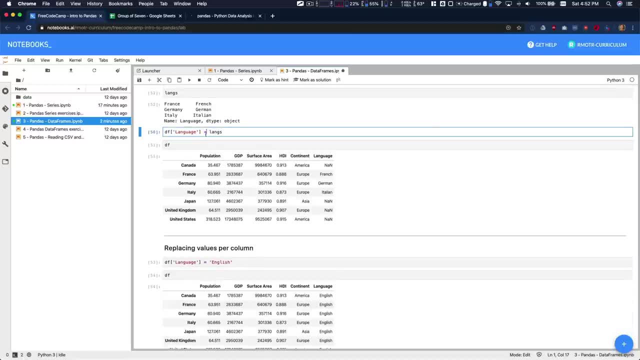 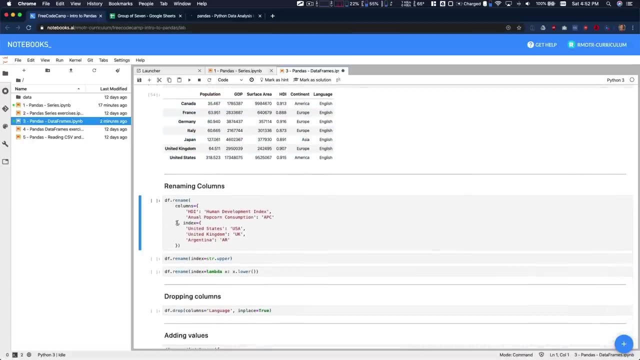 numpy, we saw something like plus- equals. In this case, whenever you have a plus and equals symbol is you are modifying the underlying data frame. So, for example, check this out- the rename function or method of a data frame. We'll let you pass columns and indices to rename. So in this case we want to change. 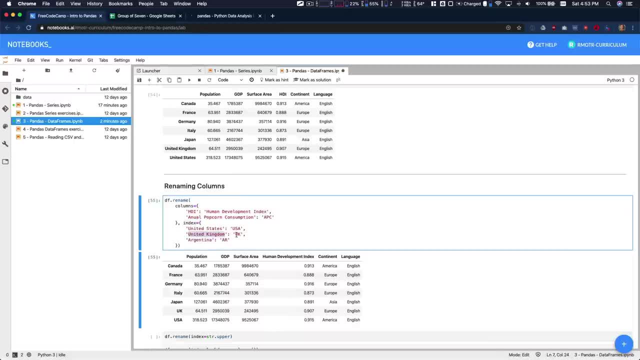 the United States to USA, the United Kingdom to UK and Argentina to AR. Argentina doesn't exist in this data frame, But that doesn't cause a problem. That's why we want to show you the US- UK were modified correctly, And HDI was modified correctly And APC, which 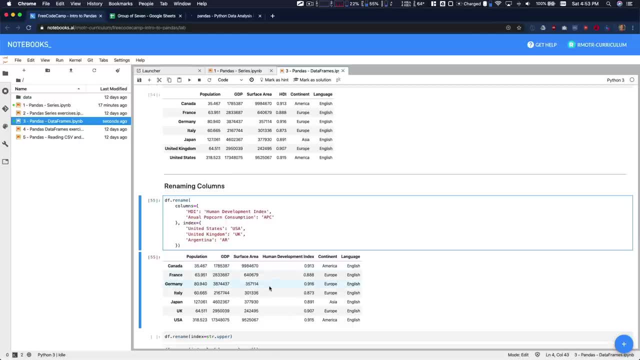 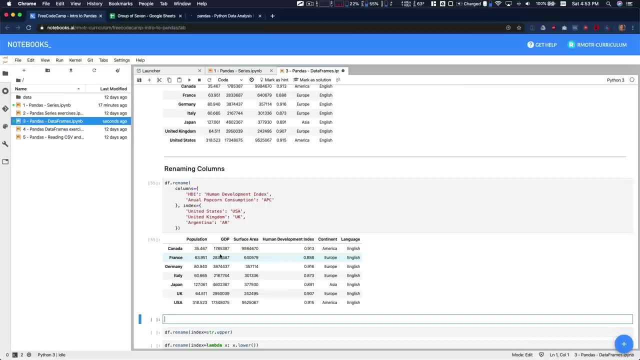 doesn't exist, Didn't cause an error, Any problems. Now, why am I showing you this? because, remember, these operations are immutable. If I check what's the state of the data frame, we see that the original data frame has not. 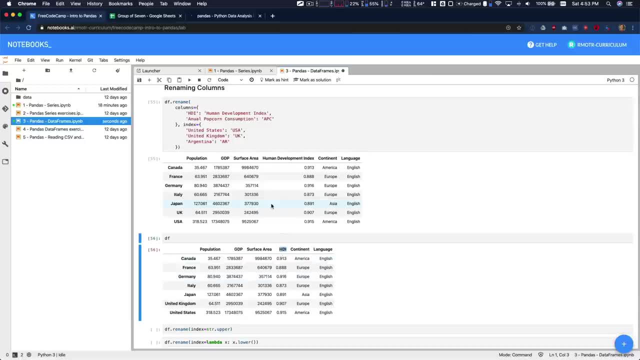 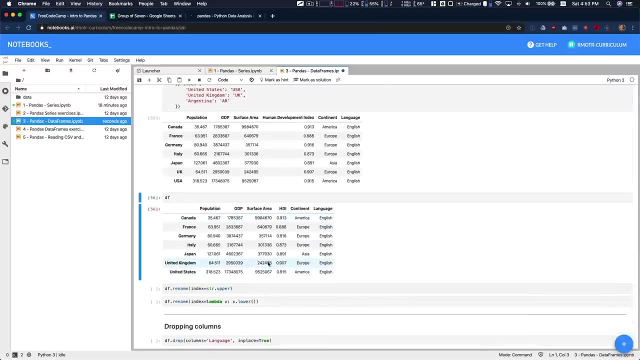 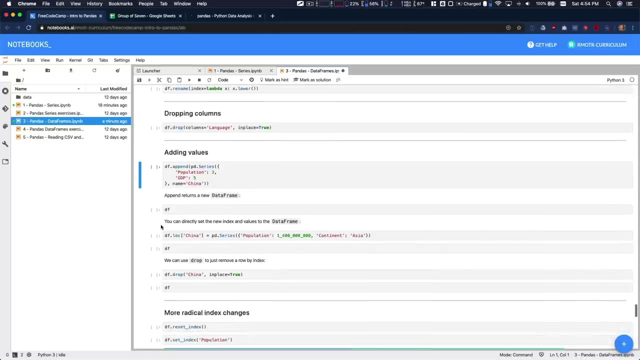 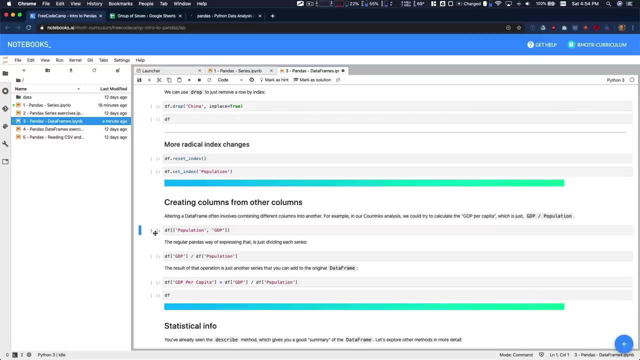 been changed. HDI is still HDI, it doesn't matter if we renamed it before. it's still the same data from the same thing for this indices. all these operations are immutable. Now let's look at a few more examples of modifying data, just for you to look at, And 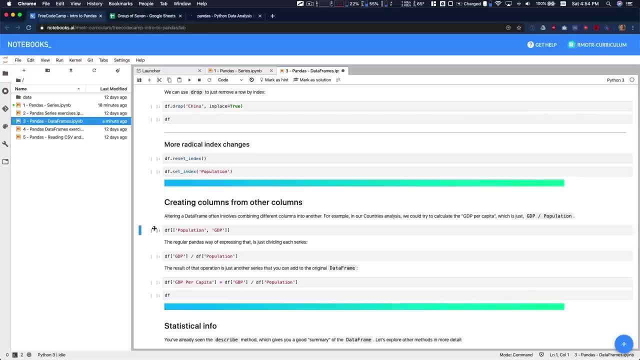 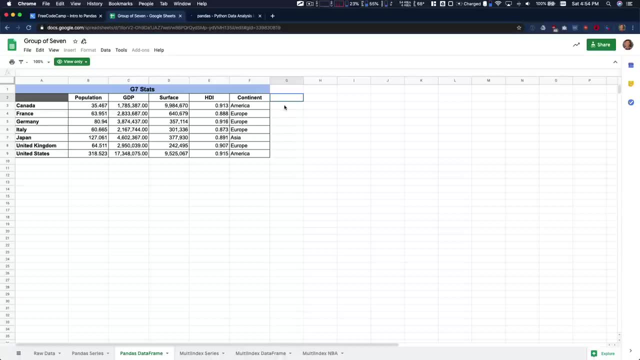 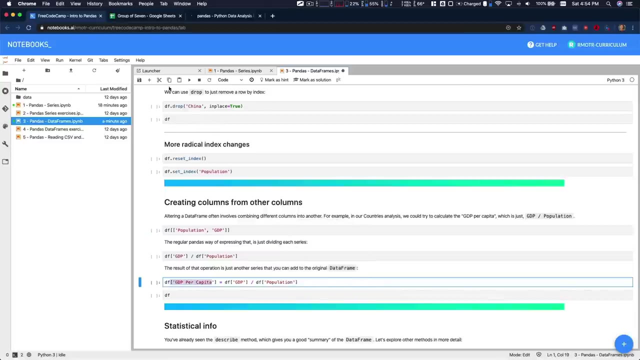 something that is very common for us is creating columns that are combinations of other columns. So again, this is read only, but you can. you can imagine that I could do here something like, for example, GDP per capita. right, if I go here and I do GDP per capita GD. 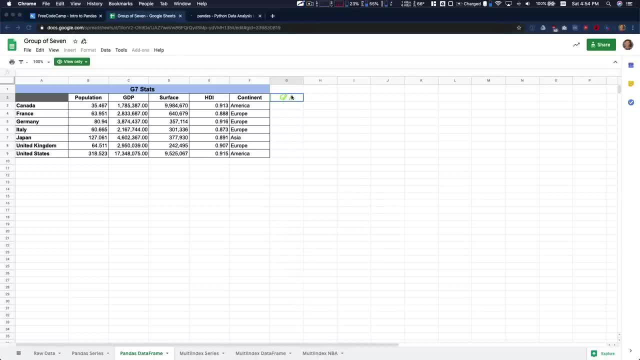 per capita Right, P per capita capita, And here I say is equals to the GDP, this column divided by these column right. so I do something like B, B three, actually C, three, C three divided by B, three right. 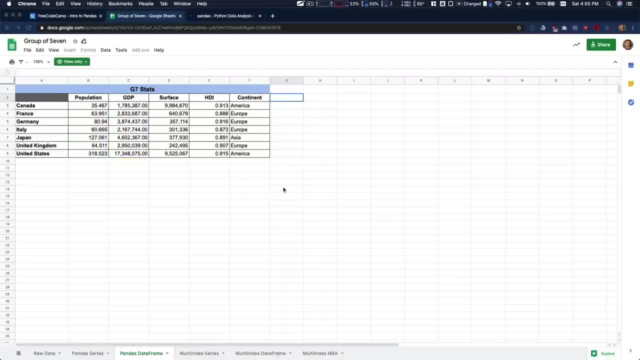 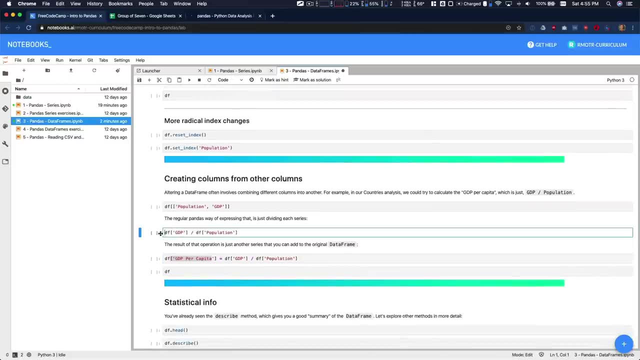 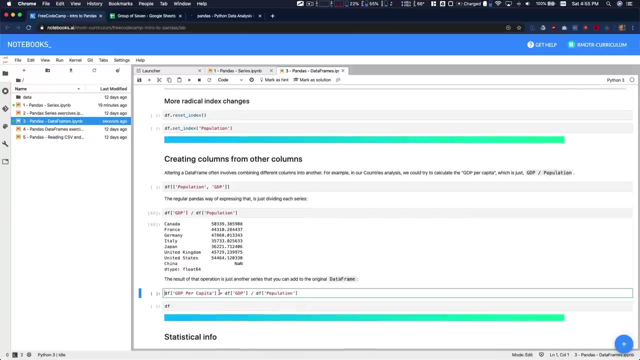 And then we would extend the value Right All the way along. here In pandas we do something very similar. we can do just any column. we can just perform operations, broadcasting operations between them, in this case GDP by population and 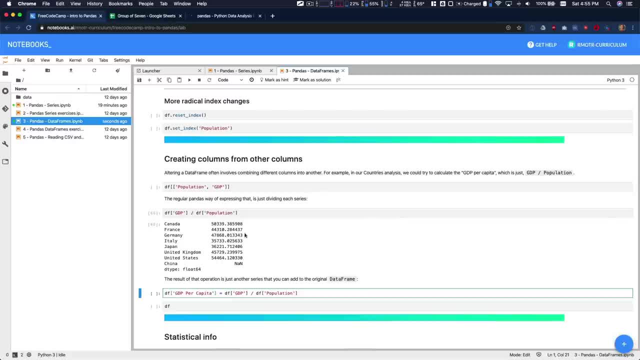 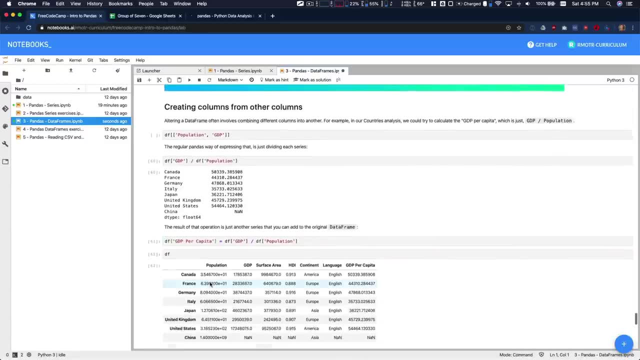 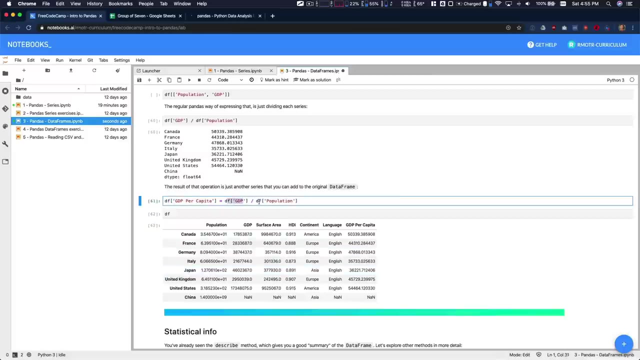 we can assign that series. which is the result, right, the results, the series. we are going to assign that series to a new column. So GDP per capita. there you go is now a column of our column DataFrame. Again, all these broadcasting operations are extremely fast. they are backed by their non 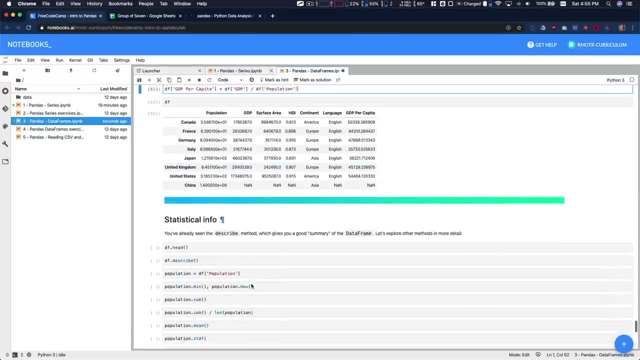 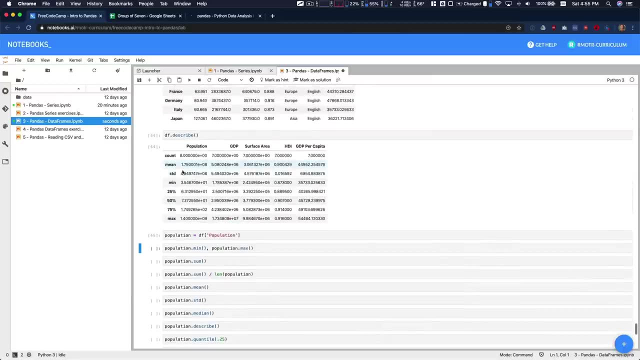 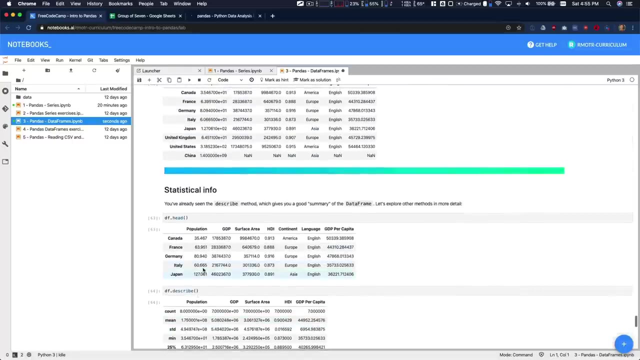 pi array and they result in a series, So very quick statistical information, a few methods, right to the summary statistics. we saw them with the describe method, but minimum, maximums mean median. all that works as expected, Something that I want you to note here, if possible. 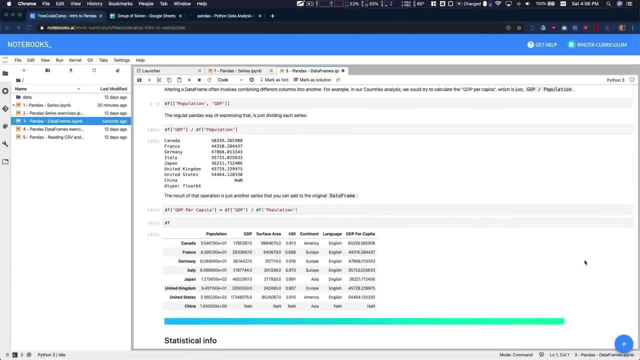 Is that with pandas? we have- I'm going to change colors here, we're going to use red With pandas. you have this concept of a data frame, right? data frame that has multiple columns and multiple rows And these operations are resulting. operations are resulting in just one series. 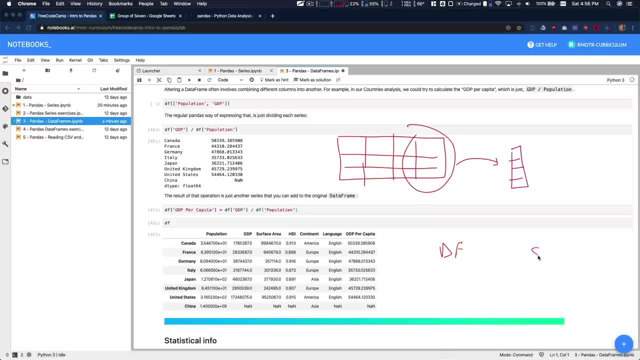 So in pandas you have your data frame and you have your series And we could say we have individual numbers And it's like always the data frame is always resorting back to this. it's like some operations will just return a series and the series can be used in a data frame, right? 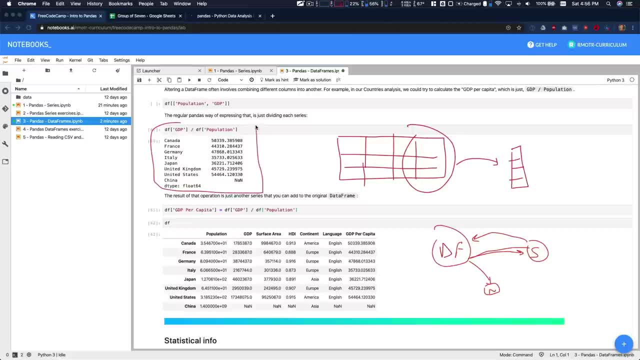 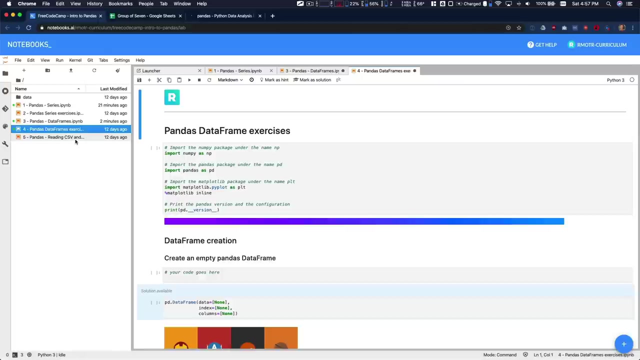 So in this case these resulted in a series, But then we immediately use the series to set the value of a column right. So that's why understanding series is so important. So there are a few more excitement exercises for you here, So you can check them out and complete them if it's going to make a little bit more sense. 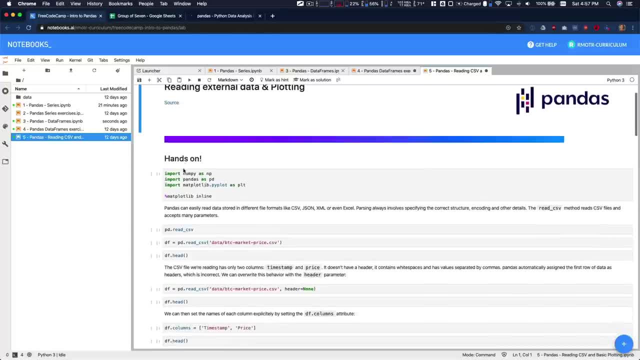 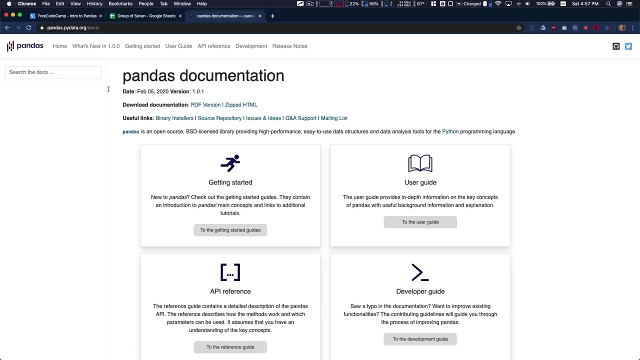 once you're working with it. Finally, I want to give you a very quick introduction to reading the external data and plotting, And to do that we're going to use a few methods that are very popular in the. maybe we can look them up very quickly here. 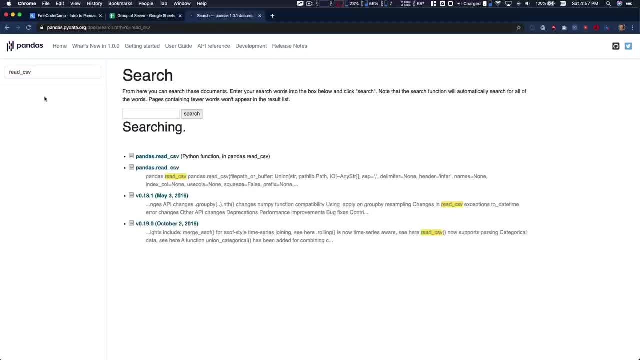 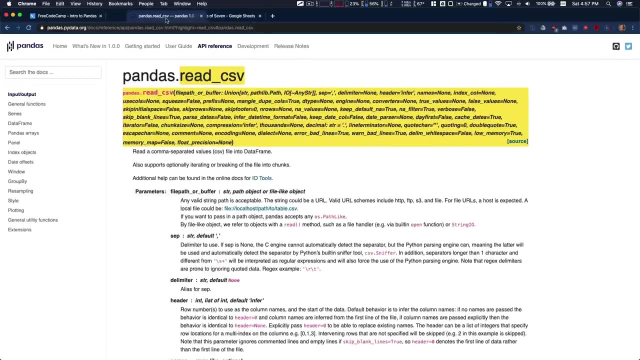 We can say: read CSV, use the read CSV function from pandas. So these function read CSV. And as we have read CSV, we actually have a few others. read SQL, read Excel, read XML. there are multiple JSON, there are multiple ones. read HTML. we will be able to automatically. 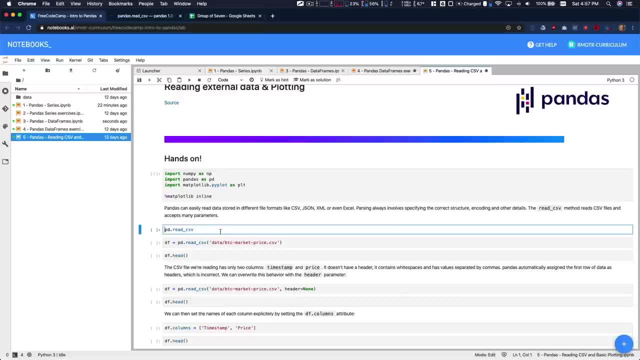 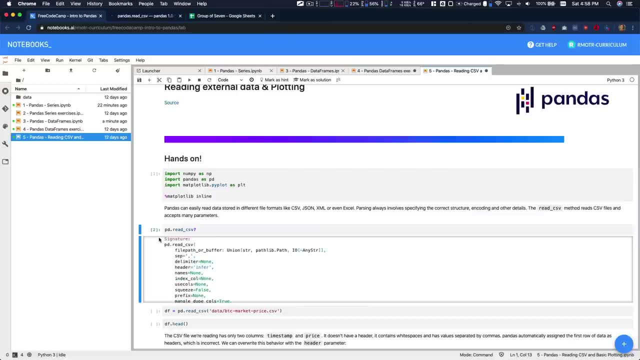 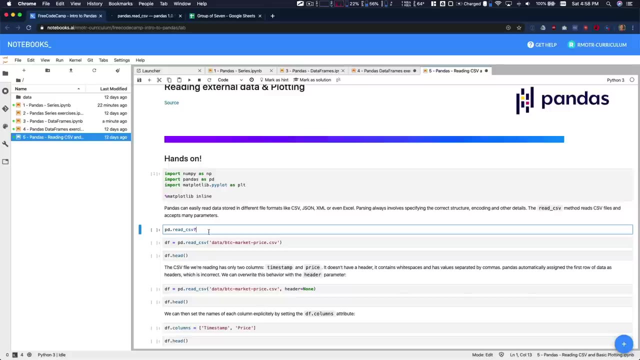 parse an HTML page and read it. So a few functions like these, like what we're going to do with this. we're going to do a few things with this. read CSV, right. here's the structure of it. A few of these functions will let us import data from an external source into our pandas. 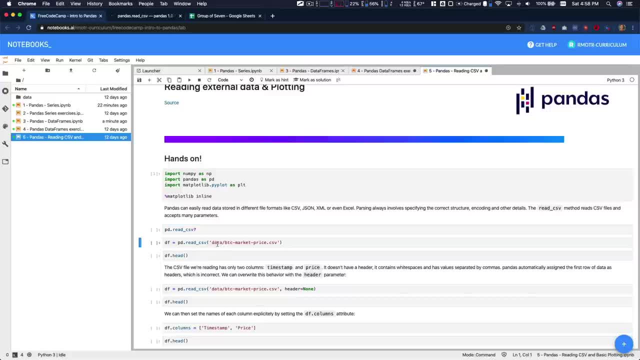 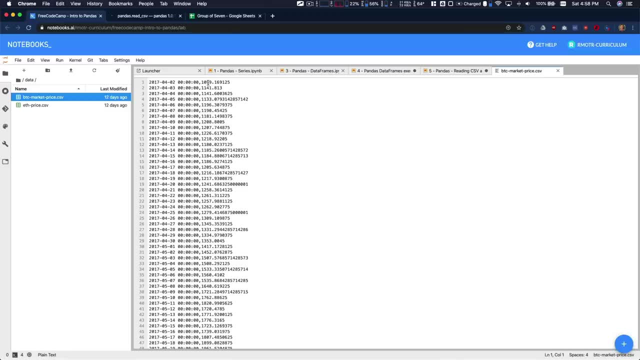 workflow. So in this case, what we're going to read is this BDC market price value. So it's right here. If I open the CSV, this is what it looks like. It's the date of the price taken, or read, and the value. 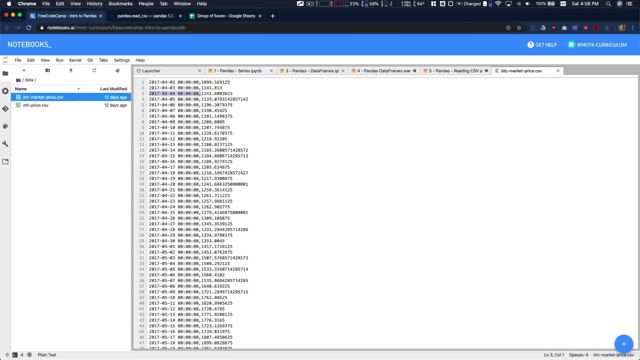 The top value, The top value, The timestamp And the value, the timestamp of the value. Note aside the price of it going 2017, and now it's close to $9,000,, I think. but just a note on the side. 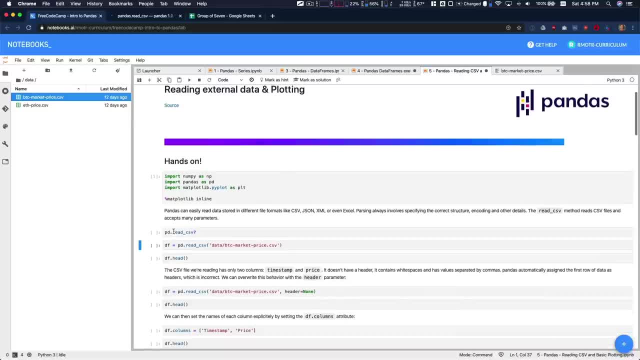 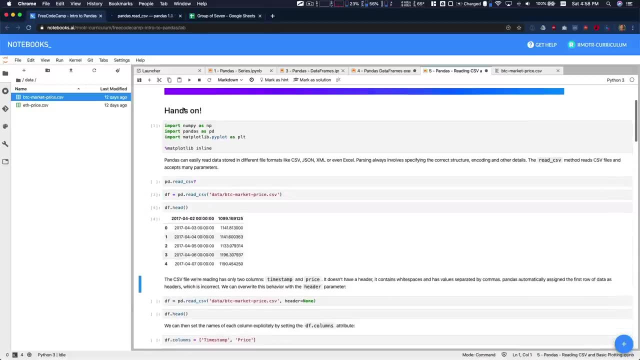 But again, this is a CSV and this is CSV that we're going to be reading. To do that, again, we're going to use this method: read CSV. The method will automatically parse the CSV as expected. And there you go. 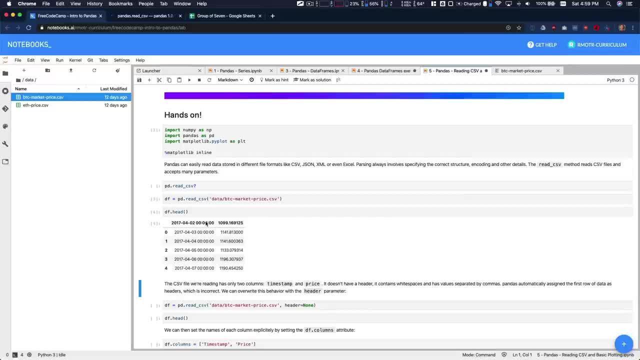 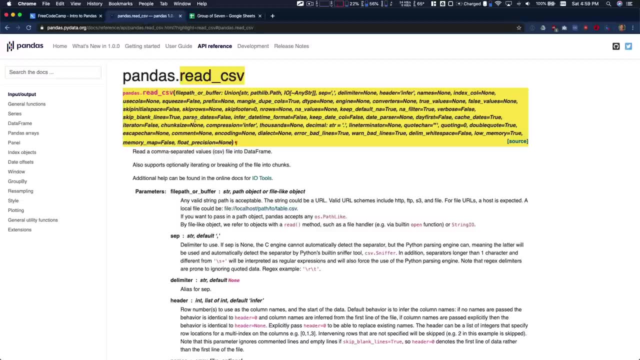 And the process Now will be for us to start tuning it to get to the right point. So I'm going to show you a few customization, as few customizations we can do with the red seat, red CSV function. So the first one, and sorry, let me tell you first we have a ton of attributes here. 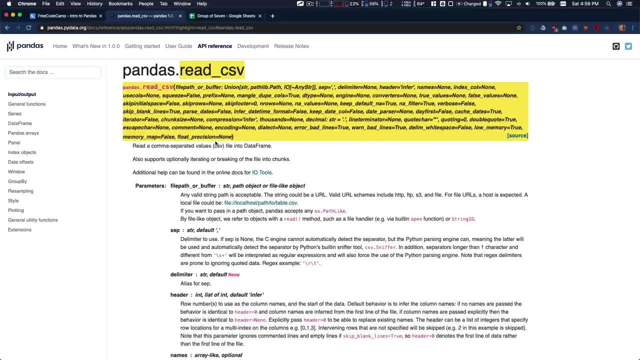 So we have a ton of customization to do with the read CSV. you will not remember all this. you will not remember everything out of the top of your head. So don't worry, you can always go back again to the documentation. I'm sorry. 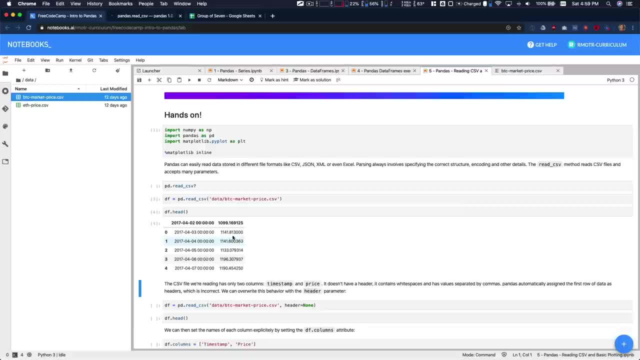 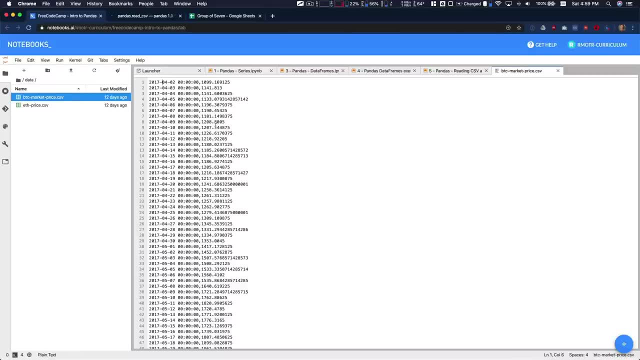 We just practice. it's going to come naturally. So the first thing, the first row of the CSV was considered to be the column names. So in this case this file doesn't have a column name. let's say, I added, I'm going. 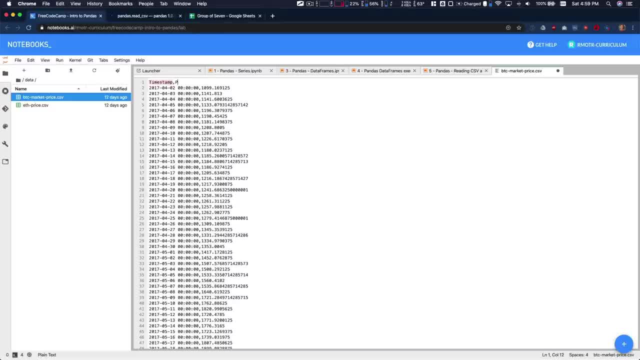 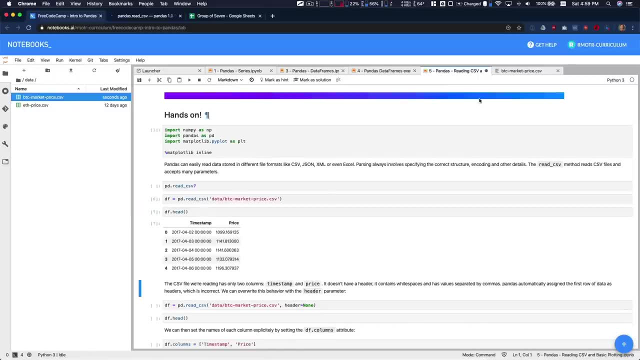 to do timestamp, timestamp price. I'm going to save it. I'm going to read, read the file and read it, read, read it. There you go. So, by default, pandas is assuming that the first line of the CSV file is going to be: 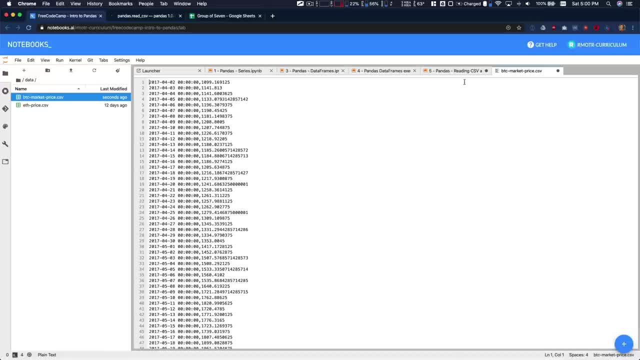 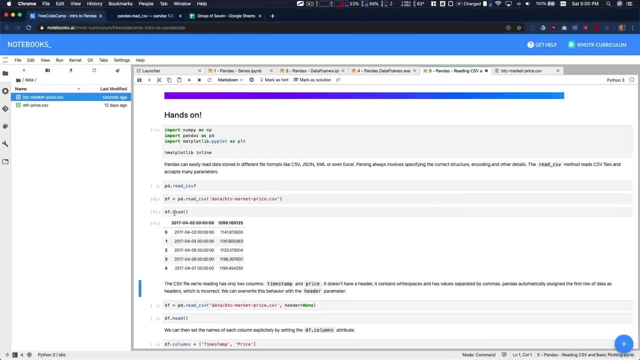 read. So the first line of the CSV is the Rd columns. I'm going to go back into what it was right. I'm going to show you Again. that's the assumption that pandas is doing. we're going to, of course, of course. 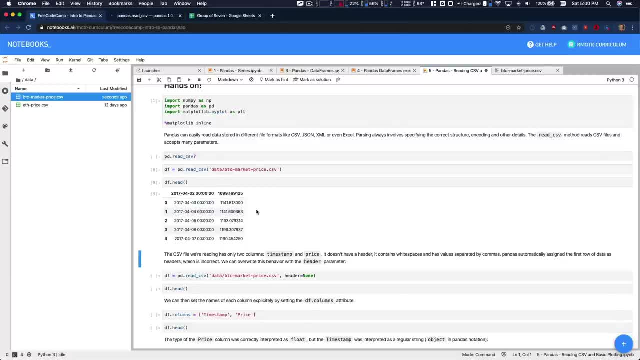 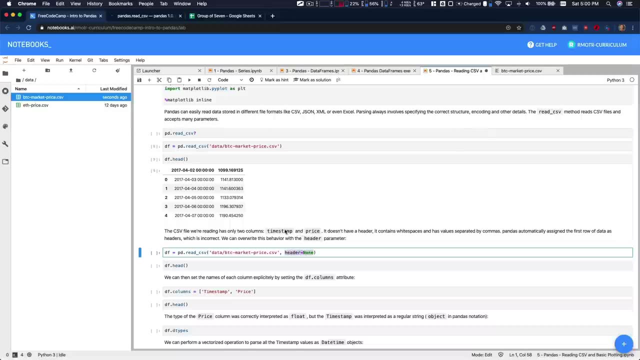 change that assumption because in this case our CSV file does not have column names. So we're going to say heather equals none. And this is when we start seeing the attributes that we're going to use from the read CSV function: read CSV. and when I do, heather equals none, for us it's going to be none. 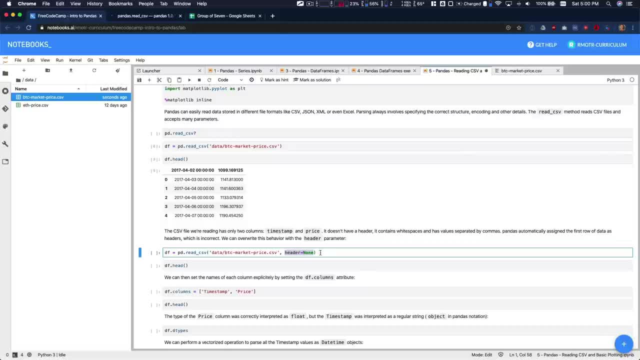 So we're going to say header equals none. And this is when we start seeing the attributes that we're going to use from the read CSV function: read CSV. So we're going to say heather equals none, So the column is going to be none. 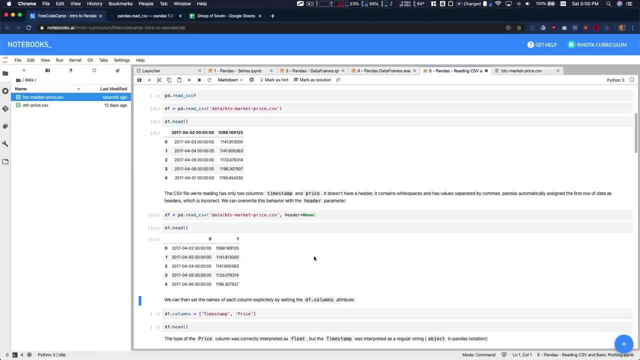 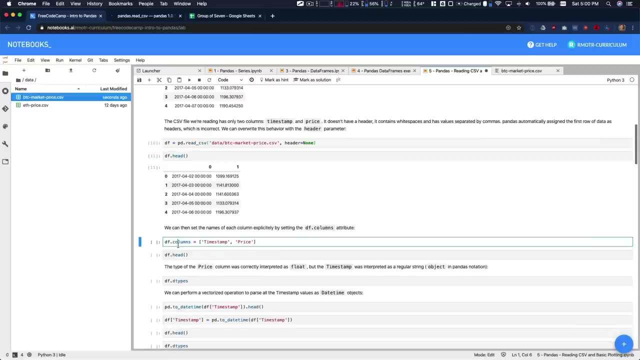 That means: don't infer, don't read a header, don't try to infer a header, a header from the CSV file And the columns are zero and one. So now I'm going to change the columns And I'm gonna say: actually it should be time, summon price. 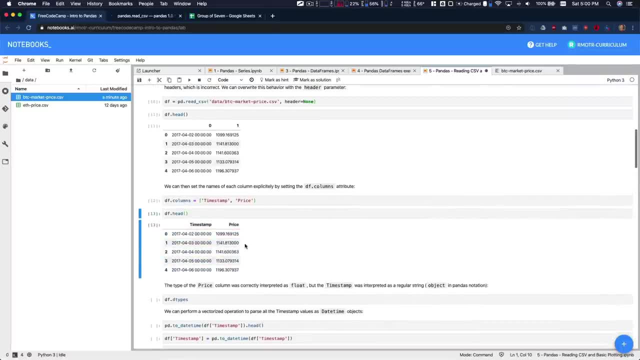 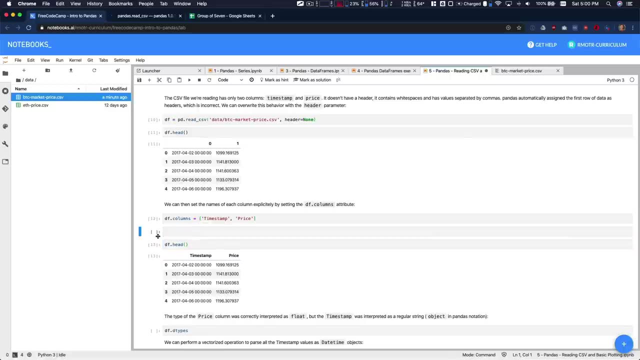 And now what I'm going to do is show you the first rows. So you're saying here that I have this df dot head method. that I'm doing That's because this is a significantly large file. So we're gonna say not, not that long, but it at least it doesn't. 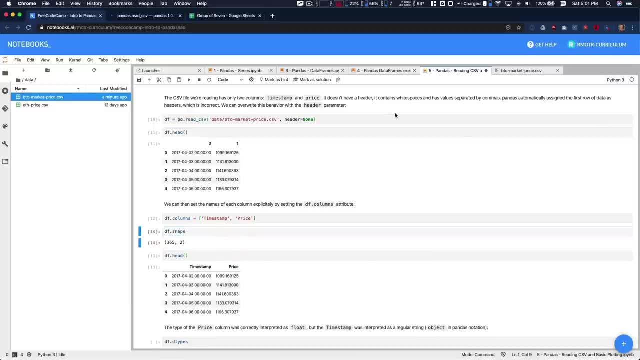 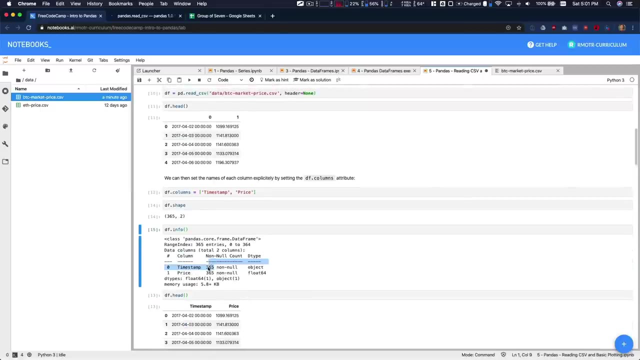 fit in my screen. What's the shape of the, the CSV or the data frame? it has 365 rows and we have two columns, So we can do the F info, for example, to have a little bit more reference about it. we have 365 values. there are no, no values and price is actually. 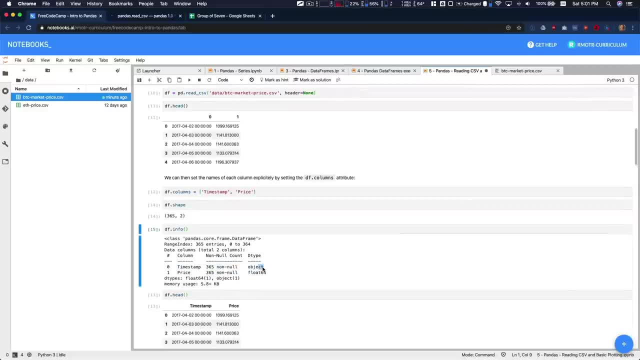 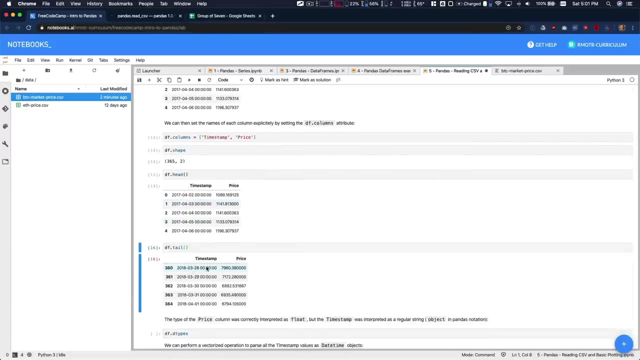 float. the timestamp is an object and we're going to fix that in a second And sorry, the DF of head on the F dot tail are the methods we use to get either the first and files or the end row, sorry, or the last n rows, which are five rows by default. you can change. 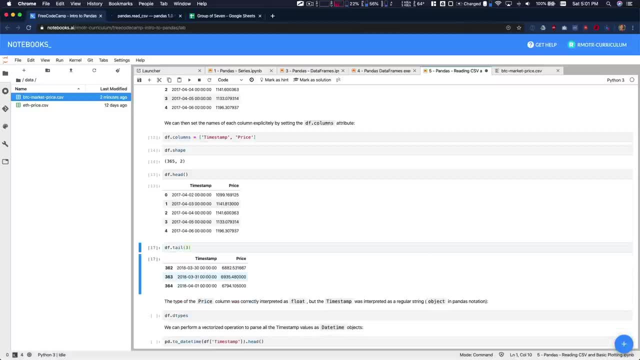 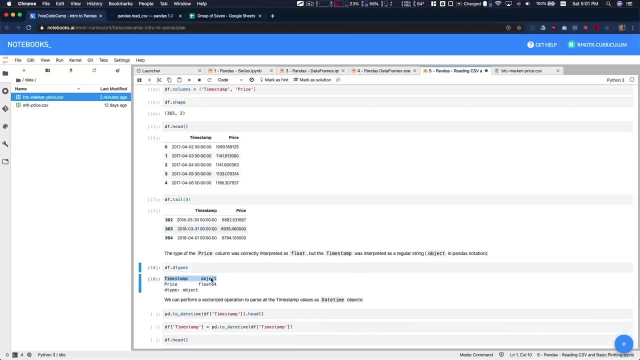 that and say: show me the last three rows, for example. that's something you can do. And again the types. So the types is the timestamp. In this case the timestamp column was not properly parses date. it was parsed as an object, as a string. 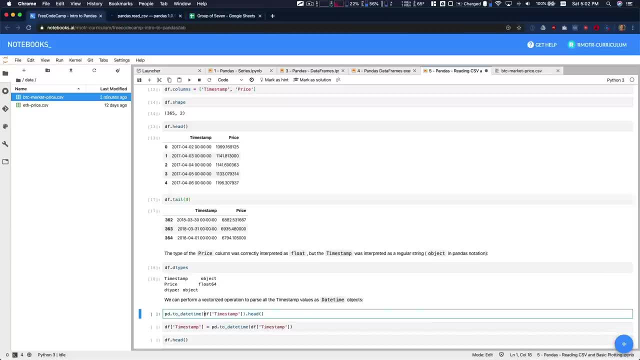 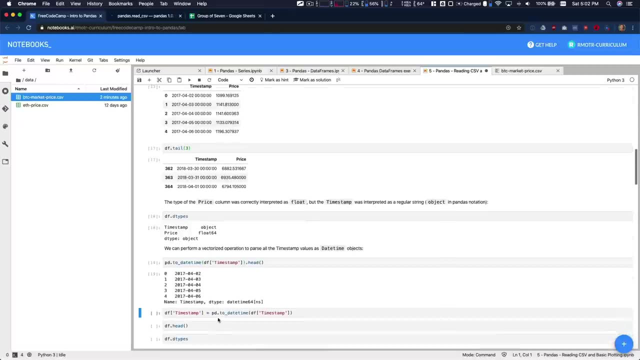 which we don't want. So we're going to use the function PD dot two day time, something we're going to explore in more detail in reading in the cleaning data, cleaning course, part sorry of the tutorial tutorial. we're gonna use it to daytime function to turn these column. 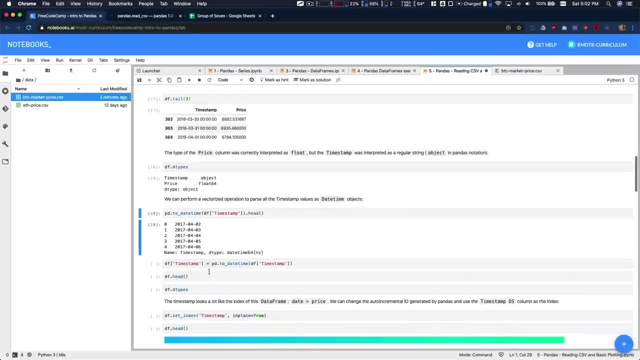 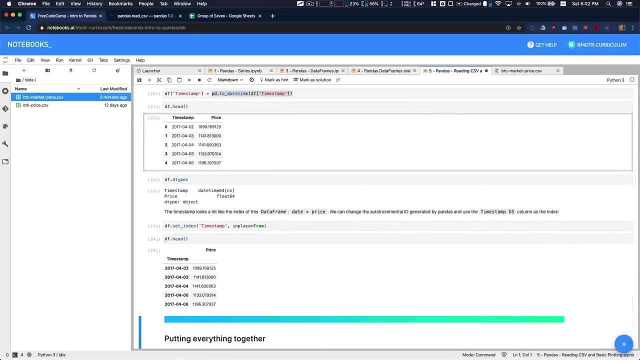 DF the timestamp into an actual date, And now we're going to say the F dot timestamp equals to this function resulting: And now everything looks as expected. there is one more change that we want to do, And we want to set the index of the data frame to be the timestamp, Because by doing so we can quickly 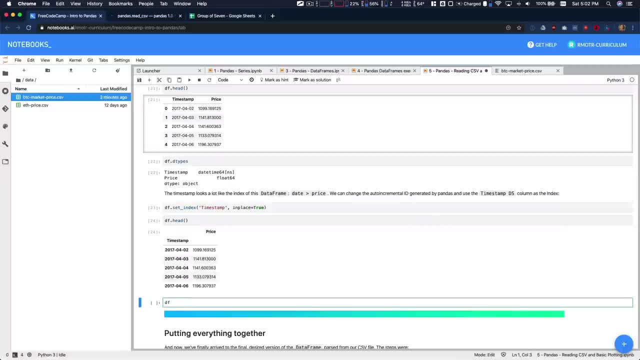 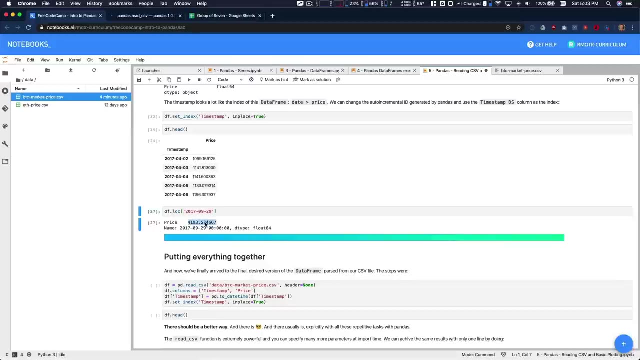 access price information. Let me see what was the price of of Bitcoin In 2017.. Oh, 929.. And I make a mistake here: I forgot the DO, the LOC. There you go. So we have the value of Bitcoin on this particular date, forgot lock. remember that to get value. 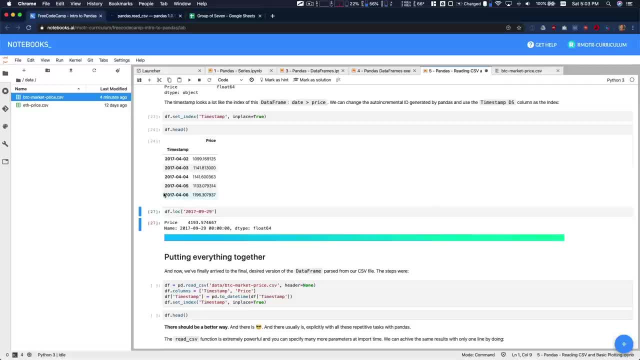 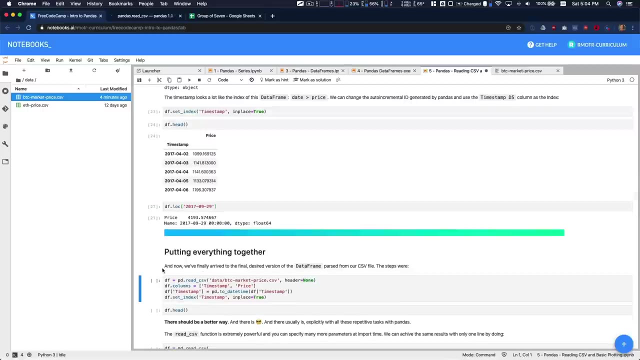 from a particular row, you have to do dot lock. There we go. So we are getting dodge particular value. Because we've made the timestamp the index, we can access the value directly from the index. So what happens? if you want to turn this thing into an automated script, for example, want to run this process? 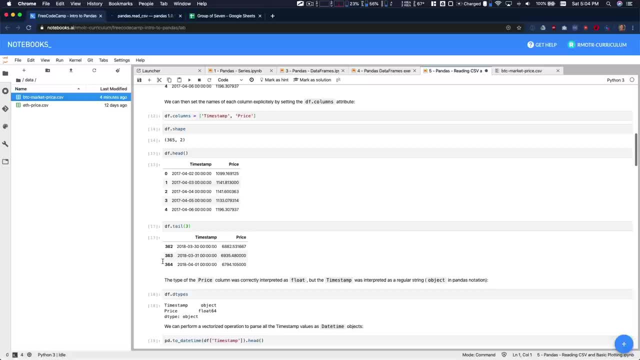 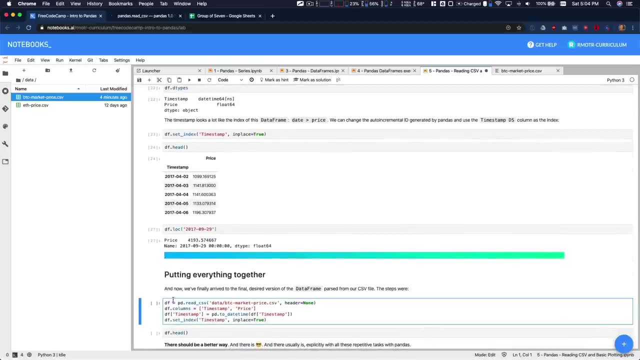 every day at 5am. whatever we can want to read the CSV, strip the columns, rename them, turn into timestamps, etc. This is what we've done so far: read the CSV without a header, create the columns, turn it into a daytime, timestamp into a daytime and assign it to. 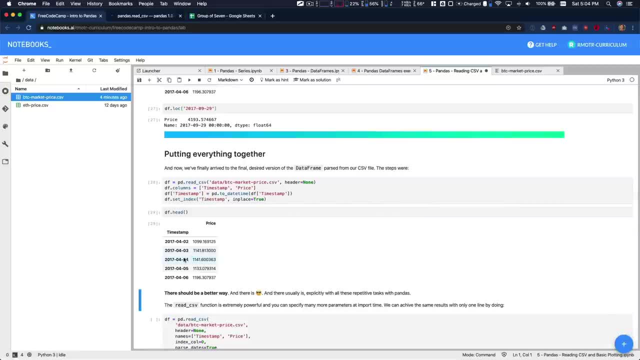 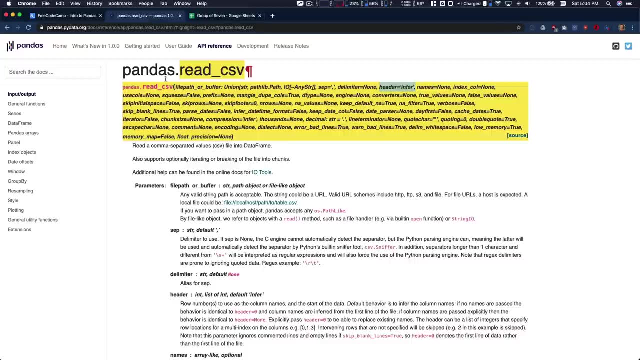 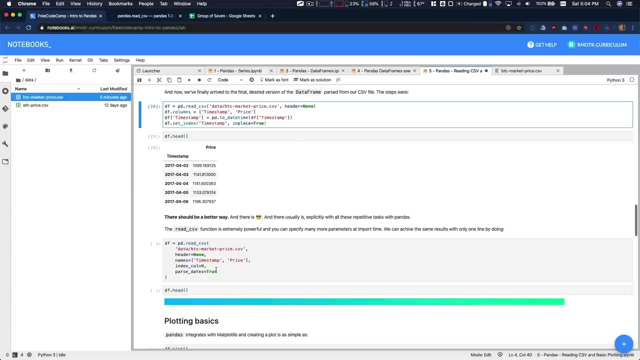 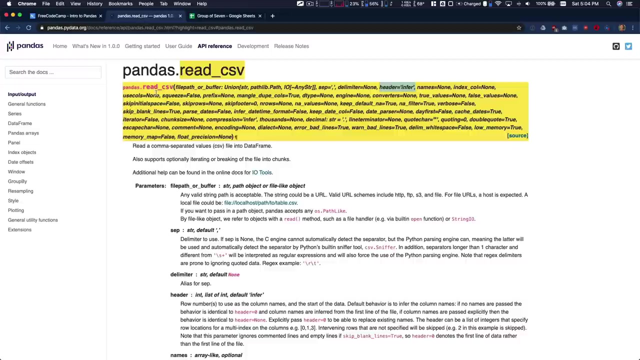 the index, And that's the result again. Well, actually the read CSV- or sorry, the read CSV method is so powerful that it will let us do all these actions in just one call of the read CSV method. We there are parameters that will let you customize the behavior to. 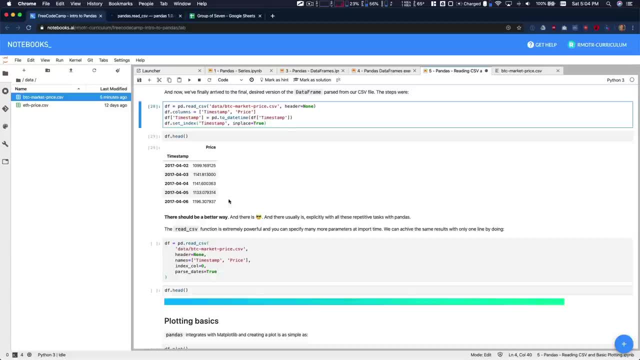 achieve the same results that we did with four lines of code right here. So we're glad we applied that here. So in this case we're going to say: read this CSV, don't assign a header- that's something we don't saw already- or don't infer a header from the first line. These are the 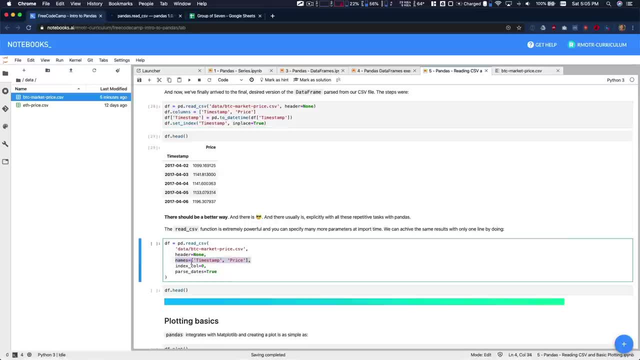 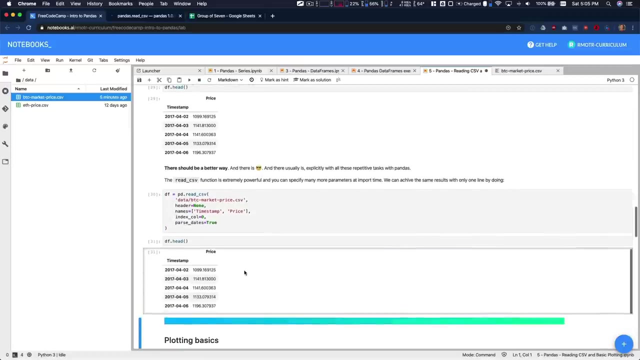 column names, So we don't need an extra line, we can just say these are the columns names. Oh, and, by the way, the first column is going to be the index of the data frame. Oh, and also parts of date if the index it's a date, so parts of date, and we have the same result. 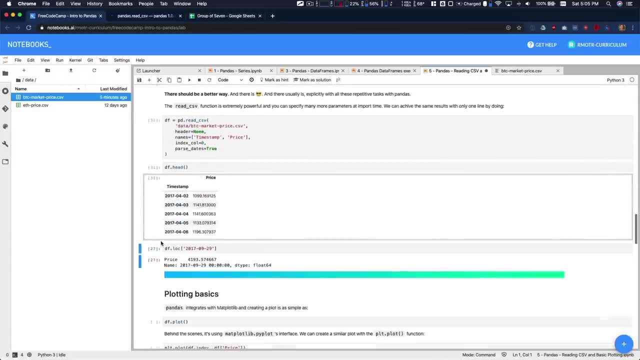 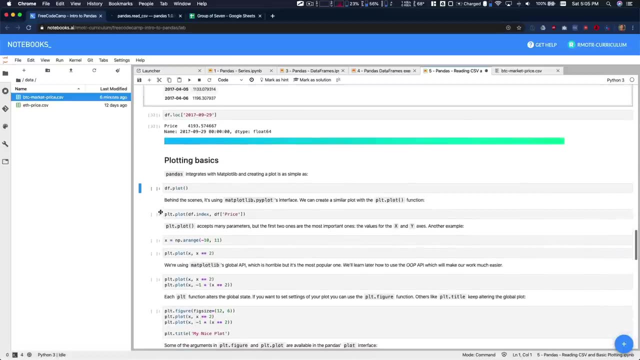 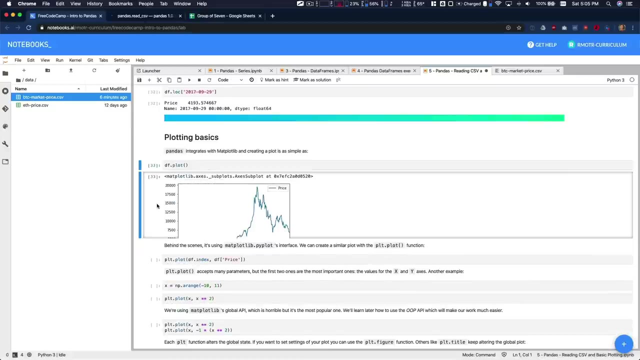 as before. So now I'm going to try the same thing. There you go, So you can see it's working. So very quickly. pin this plotting Alright. so we're going to be doing here is. I'm going to show you very quickly. I don't know what's this thing is. 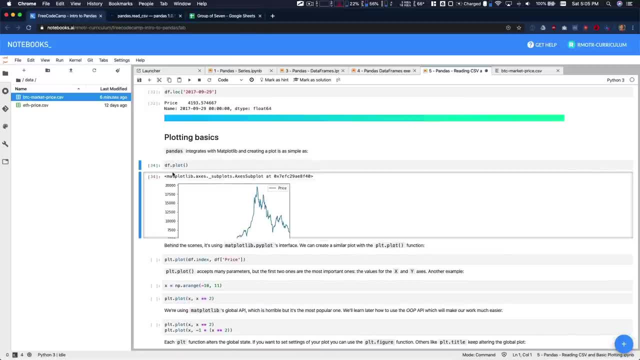 As a vertical scrolling. I want to show you very quickly that you can create plots with pandas. interest a breeze. it's so simple to create plots. So in this case, what we're going to be doing is, given a data frame, you can always invoke the plot method And the 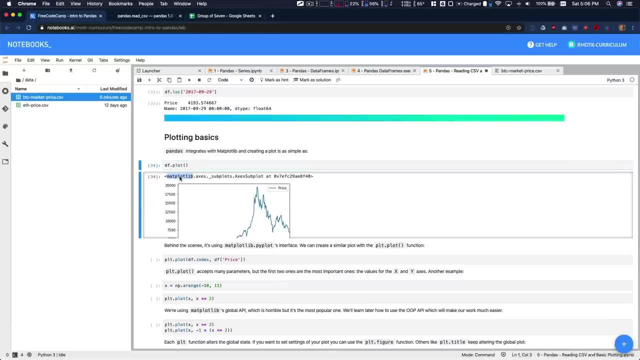 plot method. what it's doing it's using the map plot live library, something you can check, if you want, in the docs, But for now it's not necessary. with this we're going to be more than enough. What it's doing is it's creating a plot, And what it's doing is it's creating a plot, And 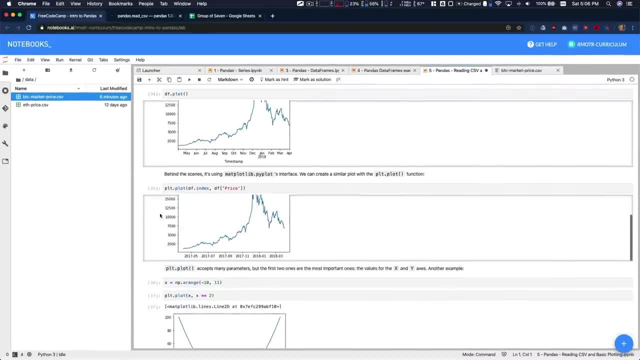 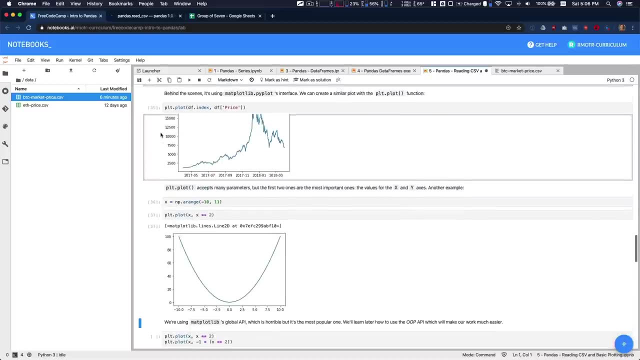 it's creating a plot And what it's doing is it's creating a plot, And what it's doing is it's creating a plot, And what it's doing is just using again the regular plot library, as you can see the map of the library, which is part of the standard pi data stack, And 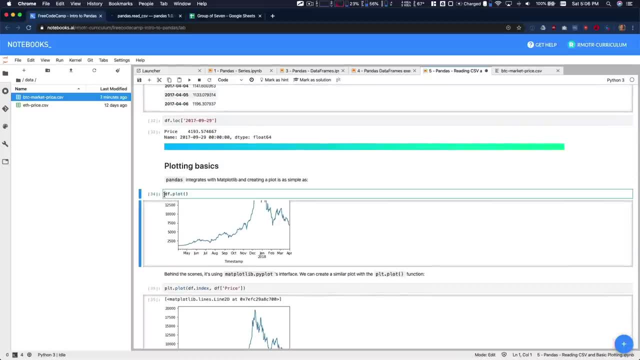 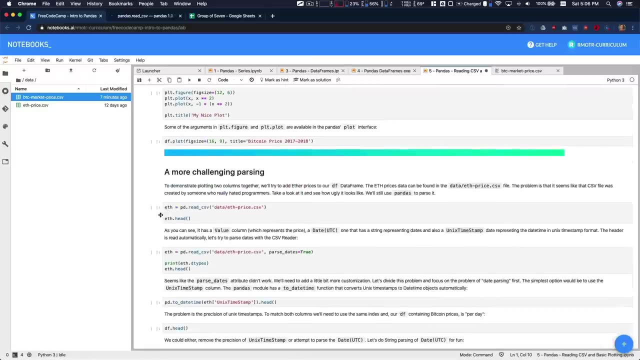 again for us to access using pandas. extremely simple, just the f dot plot, you're done. you can set the plot as you want. we're gonna see more details of mapla lives- don't worry too much about that- later. So there is a more challenging example here that I can just run. 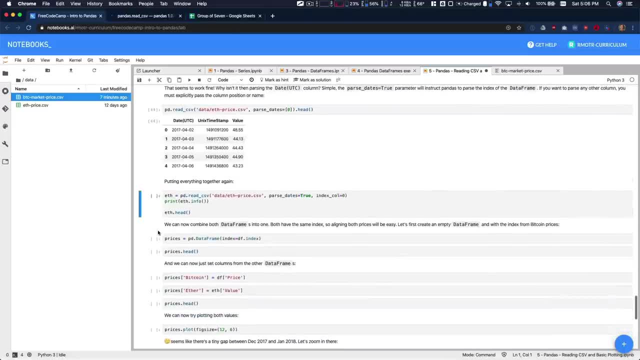 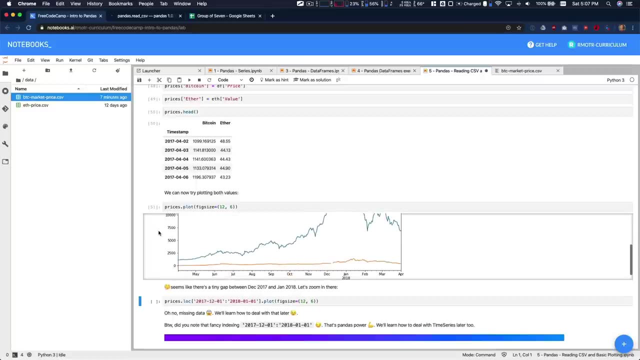 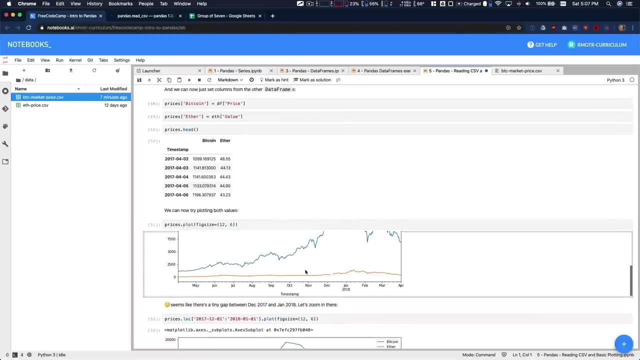 very quickly. So you're going to inspect the process we follow to fix the data, But this is what we have. there we go, And what you can see right here is the difference between the Bitcoin and ether in this period of time right here, and they are both loaded in the same chart. 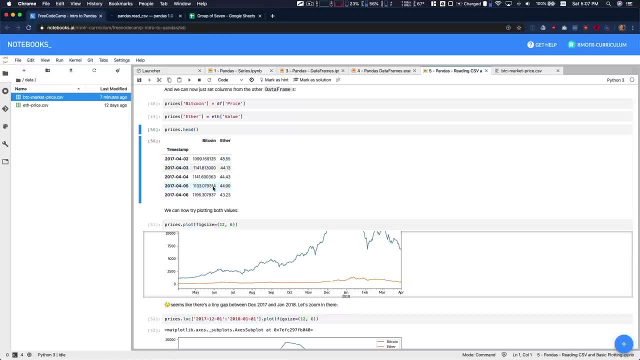 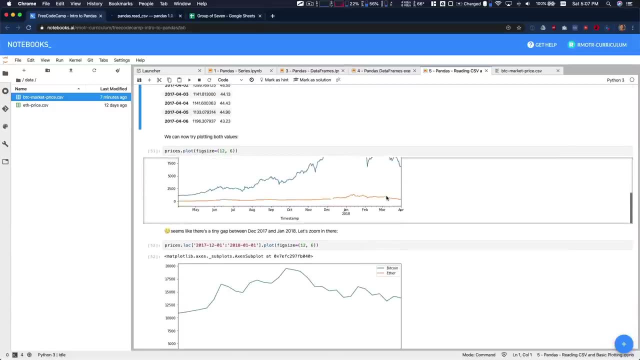 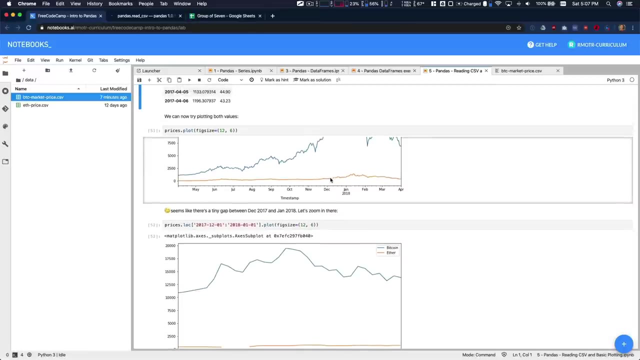 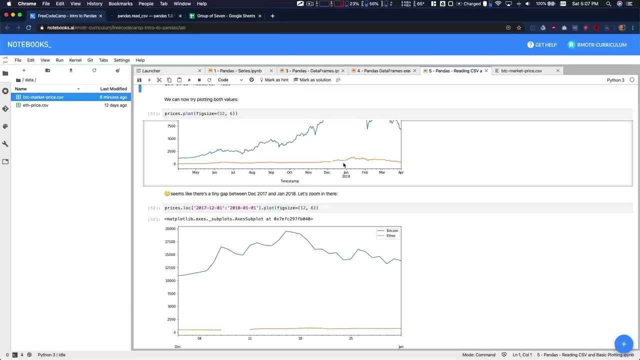 And that's because this is the resulting data frame. we have Bitcoin one side and we have ether on the other side, and we are plotting it Right here. we're creating one plot with all of it And we are noticing these empty value right here. So what we can do is we can go from December- the first- up to January. 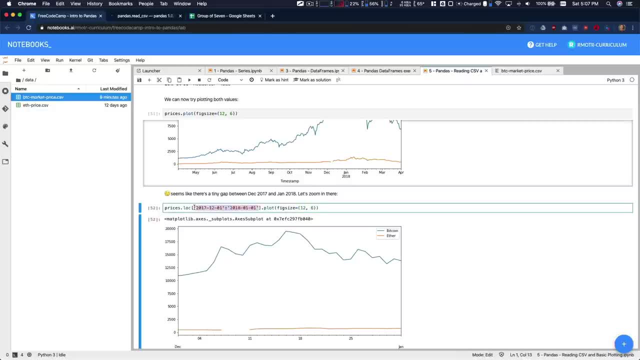 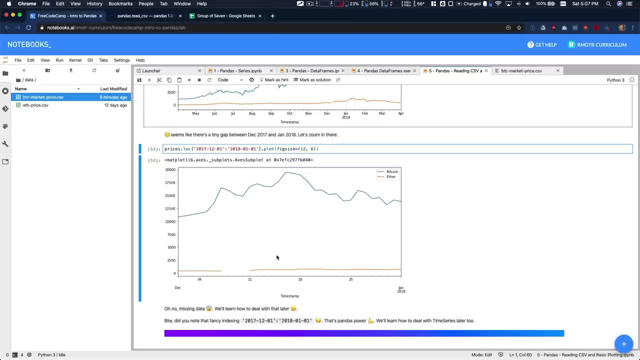 the first, this period, So we can select that period, is in that block And we can just go ahead and plot it again. And this is what you see right here, the gap that we're seeing. So, again, this was the introduction to pandas. we have a real life example of pandas following: 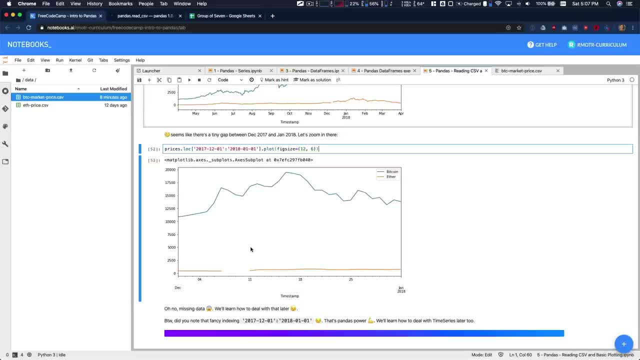 up. Also, we have a little bit of made it more data cleaning and reading other interesting files and sources of data for in getting more data into the pipeline right. So the idea is going to be showing you how you can import data from Excel, from SQL, and then do the 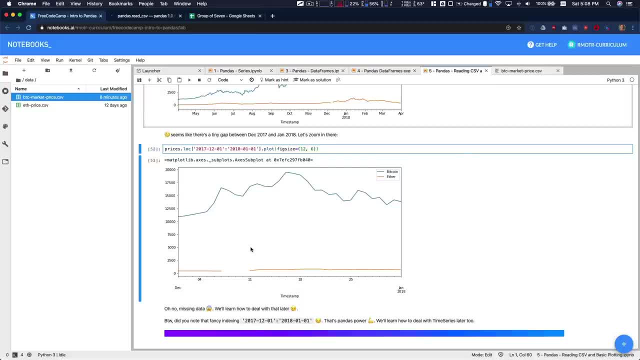 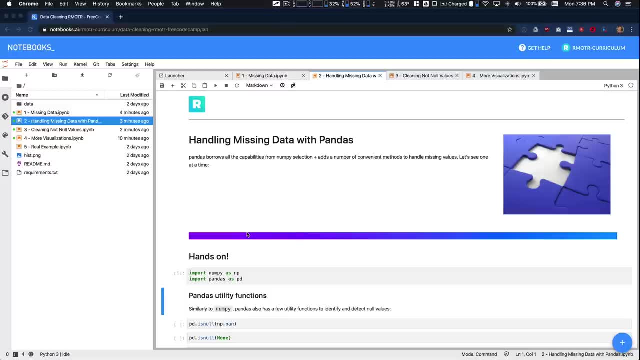 actual processing and analysis. Now it's time to talk about data cleaning. we have arrived to that point in our tutorial, in which we have pulled the data. I've shown you how to manipulate it with pandas- the beginning, at least the introduction to data manipulation with pandas- and now it's time. 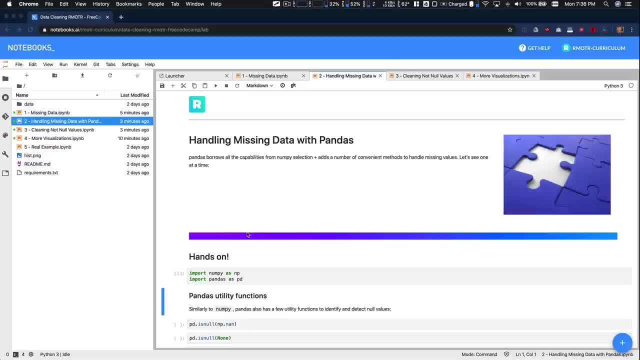 to properly fix it. For the sake of brevity, we are skipping a few parts of the process of data cleaning, especially. you're going to find in this first notebook that we talked about Analytics, conceptual missing data with Python, with NumPy, And we're going to miss a few. 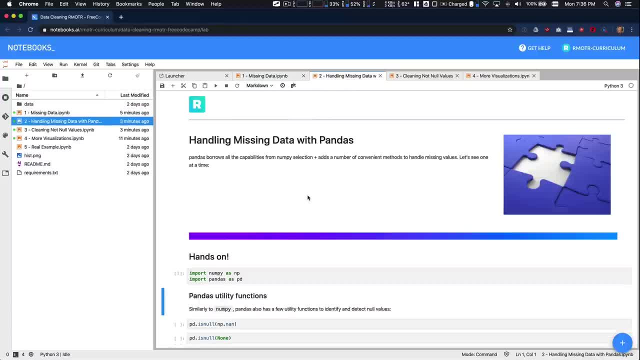 other things, But I'm just going to mention them pretty J in a pretty general form, And then you can, of course, dig deeper. you can check our courses if you want to know more about it. Usually, when we talk about data cleaning, where it's in from a more conceptual 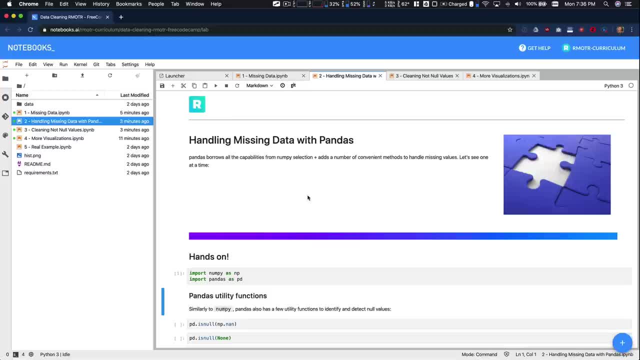 level. we're going to talk about a four step process. The first step is usually finding missing data, which is the simplest problem to identify, Identify it from a data set when something is missing. So you have car sales data And there is a car that has no name right. Or there is a card has no price right, So there. 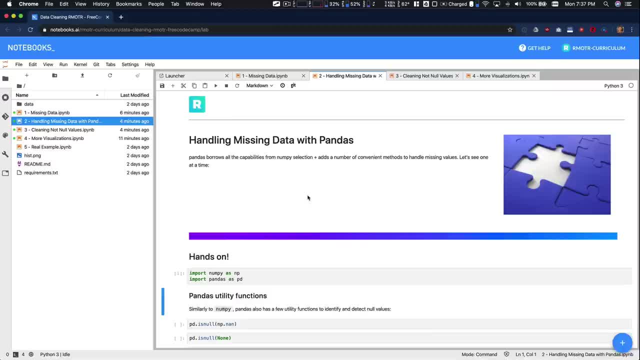 is a number of missing, or there is a category missing, or there is a string missing, And of course, each one of those is going to have a different meaning. how to solve, how to fix data set that is missing data. it can be very simple If you can just, for example, drop: 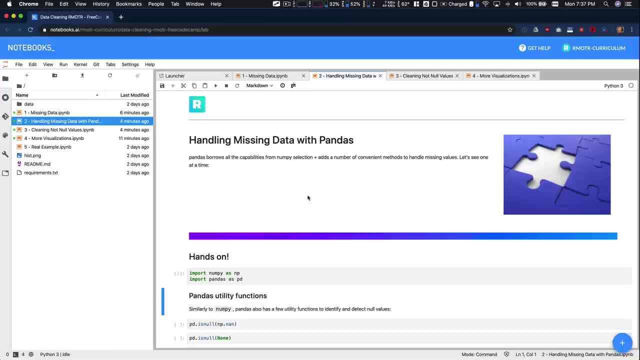 the record value right. So, for example, the prices fail and is missing, you can fill it with the average value of the sales data or something like that. Or it can be very complicated if the value is important, if you can't move forward until you actually find that missing value. 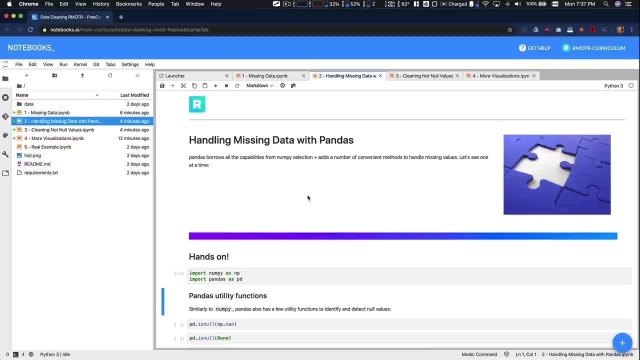 And it can involve something like picking up the phone, calling your ETL team asking what's going on, that the data is missing. Or even if you're buying the data, you have to call the vendor ask them why there is, if you're paying for that and there's data. 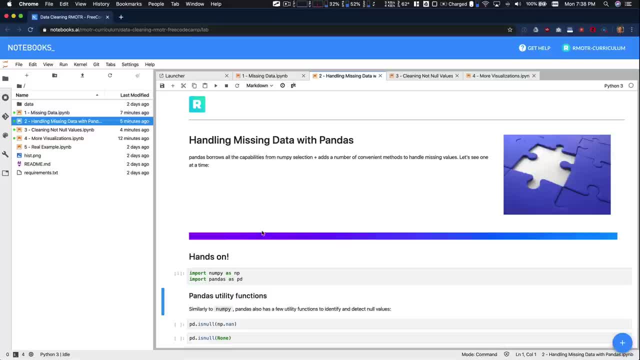 missing etc. So it can be a very political process. It depends what's your use case. But again, from a technical perspective, identifying missing data and fixing it is going to be extremely simple. Once you have fixed the missing values, then you're start looking. 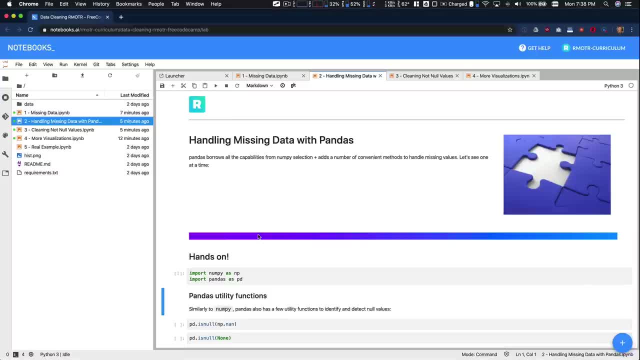 for the data is an assuming. the data is not clean. yet in this process of data cleaning, The second step is when there are Invalidities. Invalidities: So you have, for example, column that is price and there is a string within it, right? So you're expecting only numbers and there are strings in it. So then it's. 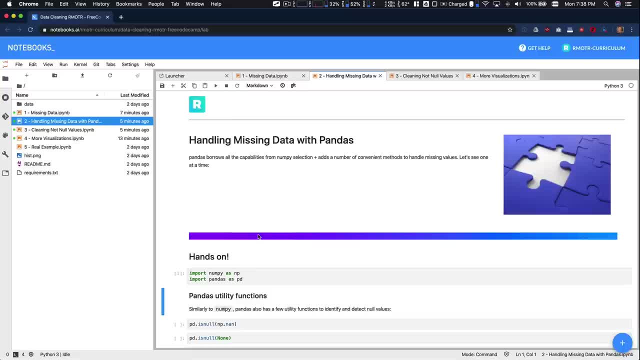 not going to be that complicated to identify. it's not going to be that complicated to fix it, But again, we're increasing the complexity Until, at the end of these data cleaning process, we're going to reach problems that have to do with the domain of the data you're looking. 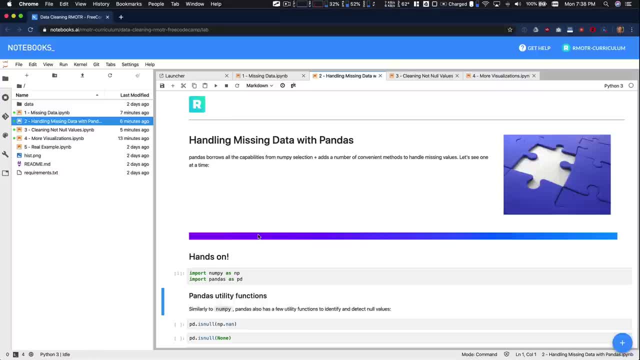 right. So, for example, you have a column that is it's customer age and there is a value that is 170.. Right, So that is not an invalid value, It's a perfectly valid integer. The problem is that, given the domain right, we're speaking. 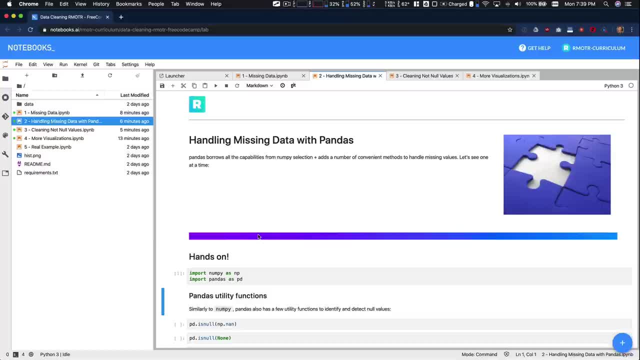 about customer age is highly unlikely that a customer is 170 years old, right? So in that case the value is completely valid. there is no missing data, there is no invalid values, etc. It's just about the domain, And this is when things get very complicated. 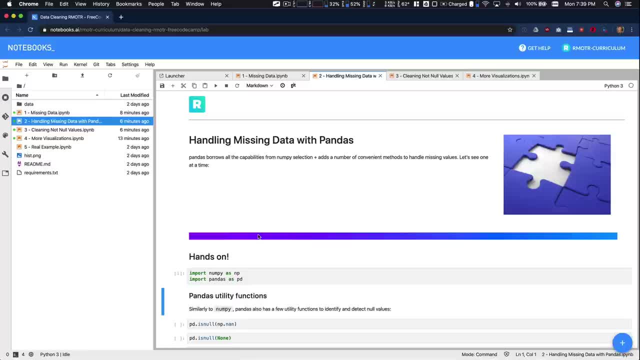 Because, in this case, the example of age is something that resonates with all of us. we know about age of humans, But if you're working in a domain, if you're working as a data analyst in a domain that you don't know much about, right then you might not. 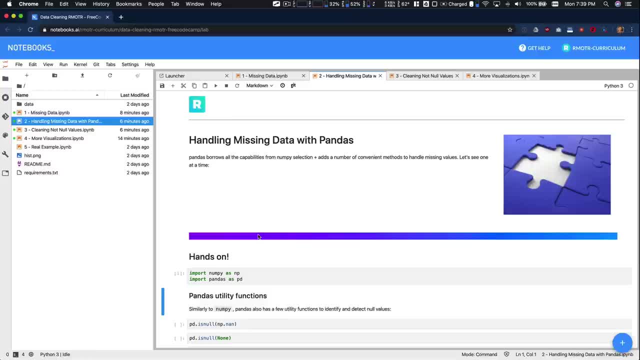 be able to judge if a value is invalid or not. If I am working in a biology lab and I have something like white cells count per milliliter of blood, I don't know what's. what's a good value. That's an invalid value, right? So it's. it's something you need to know the domain So. 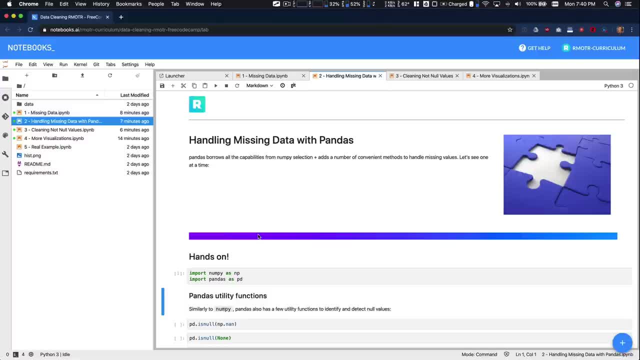 that's usually the most complicated part of data cleaning. when you reach the limit of everything is valid, everything checks out, And now I need to make sure that these value is valid for these domains that we're working. So, again, this is the spectrum that we're. 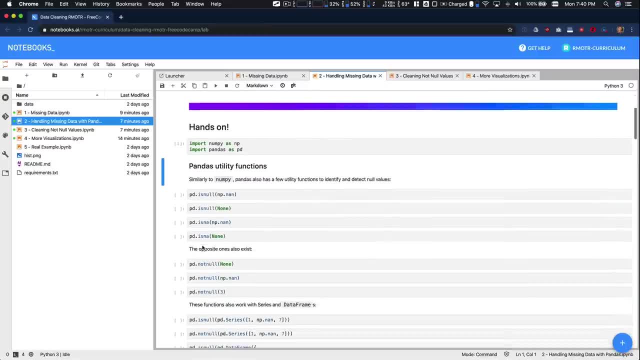 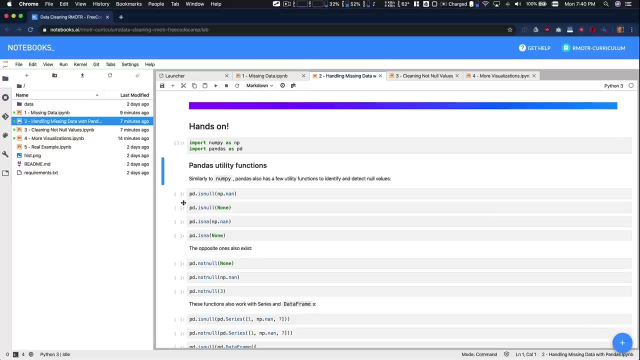 going to be revisiting today. So, to get things started, the way pain this works with no values is is it has four functions, which actually there are synonyms. it's going to be. it's going to be relatively simple, just trust me on that. There are a few things. First, everything that pandas. 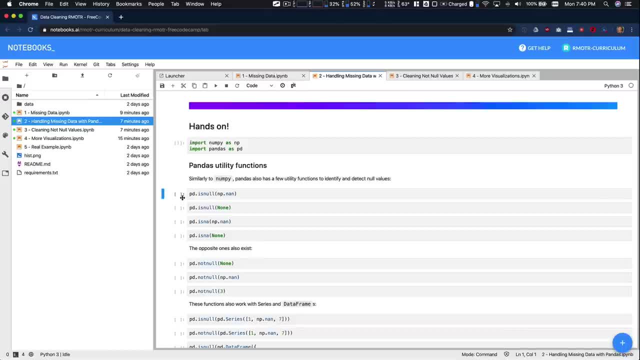 does in the process of missing values is related to the way known pi works. So again, we're skipping it. you can go to that notebook, check it out by yourself. But it's extremely simple. NumPy has these objects na, n, not a number, to identify a missing value or no. 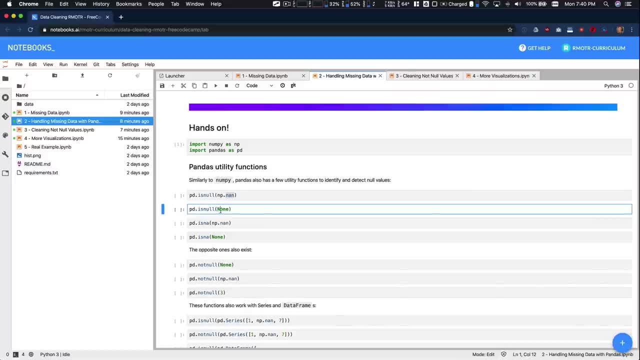 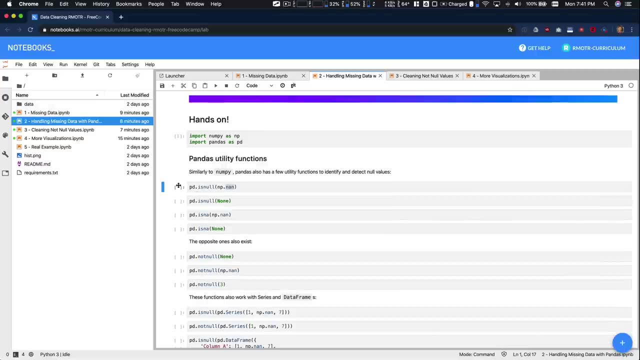 value. In Python we also have the non value, But again, in pandas and NumPy we're going to use na, n, none, And there are, in this case, at the beginning we have these two functions: is no and is na, which are complete synonyms. 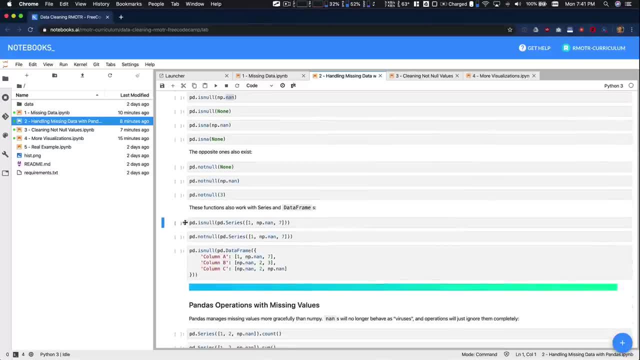 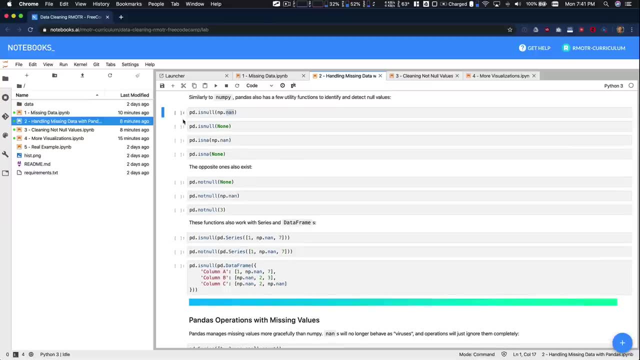 we're going to find also is no, and I don't know if we have it is na, and they're also complete synonyms. So no, an na for pandas is the same. you can use the one you prefer. Sadly, I like is na, because it's the way I learned it, I think, for my students. I usually 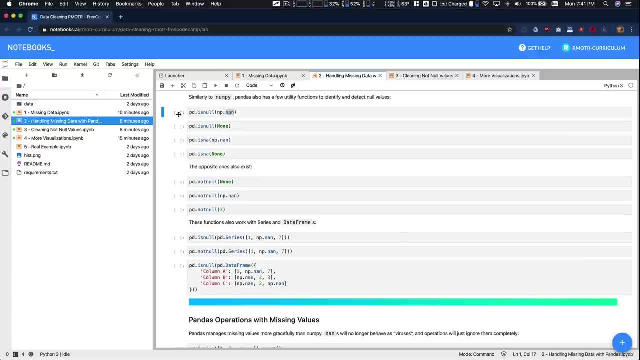 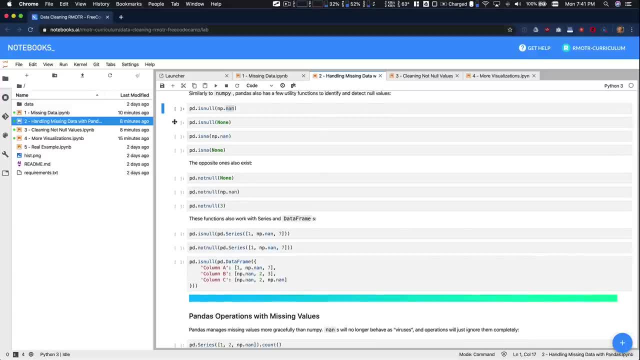 more self explanatory. So you can use the one you prefer. if you can use is no, I think that's gonna be better. if you get used to is na, then you're going to be on my side. just do whatever you prefer. So again, is not going to say true or false, depending if 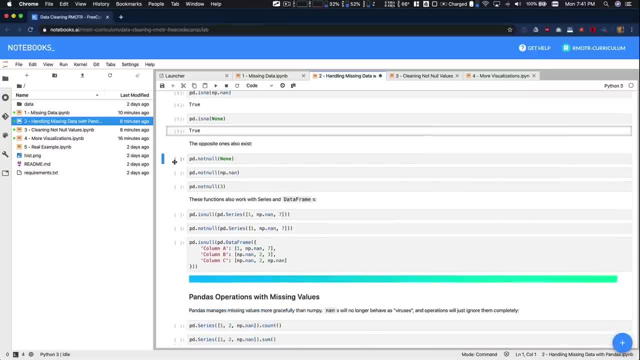 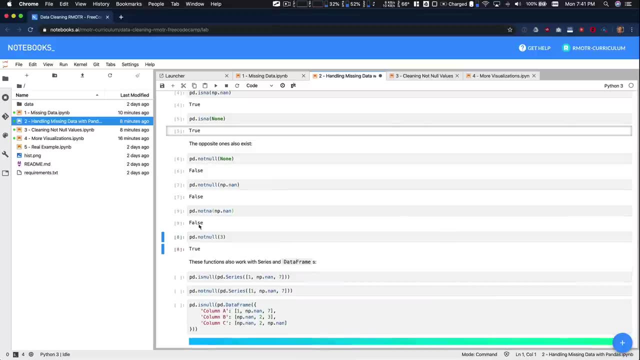 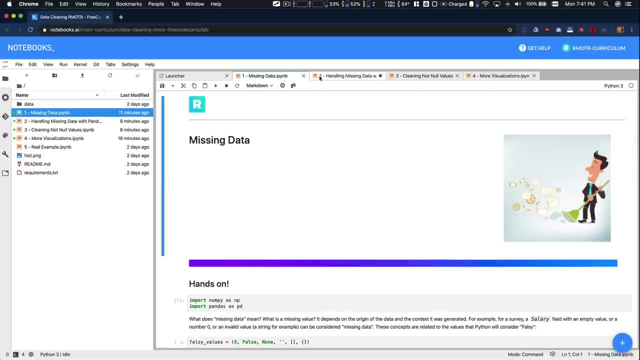 the value is no or non right And of course not null is going to be or not na is going to be the opposite. So not na of not a number is false and not na of three is true. If you get to this first notebook you're going to see it: all the false values on the truthy. 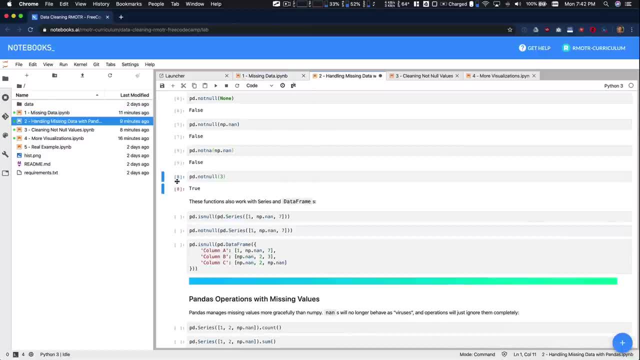 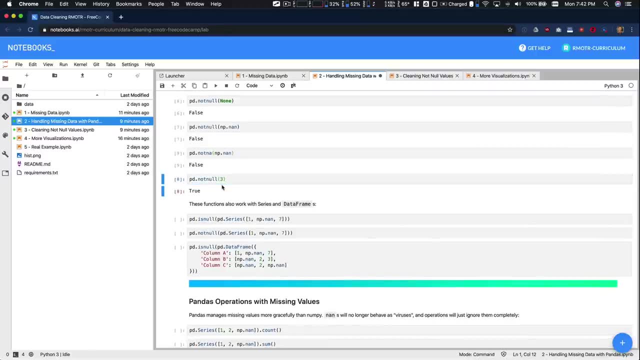 values in the. in terms of Python, anything that is not empty or none, etc. is going to be considered to be truthy. So anything you pass here, that again it's not an empty string or a null, is going to be considered a truthy value. So it's null and not null. 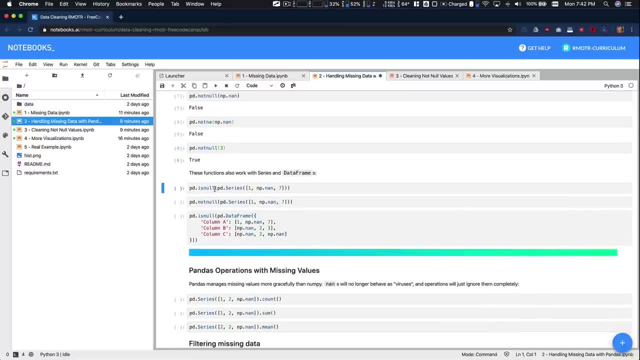 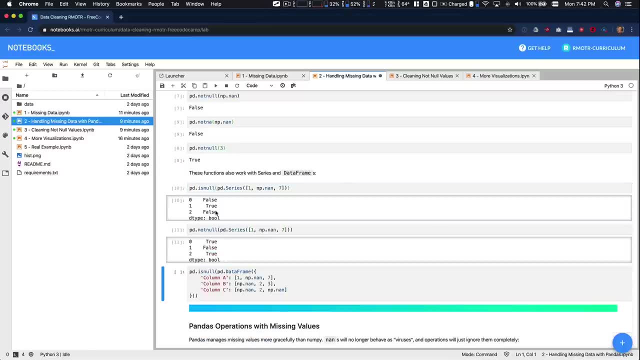 or isn't a and not an A. they both work also with entire series or entire data frames, right? So it's not just for one off value. you can pass an entire series And the result back is going to be: if the series is, if the series, what values in the series are either 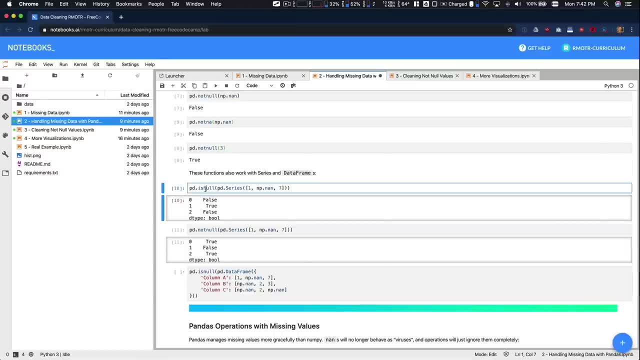 no or not. no, depending what's the question you're asking. either is no or not. So in this case, we say: which values of these series are no, this is not no, this is not no, this is no. So this is only true And the opposite. for the following method we are going to 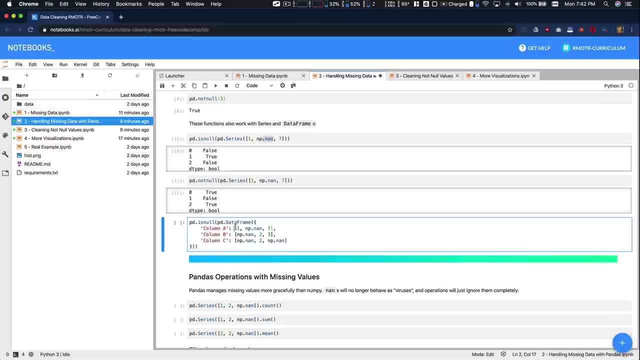 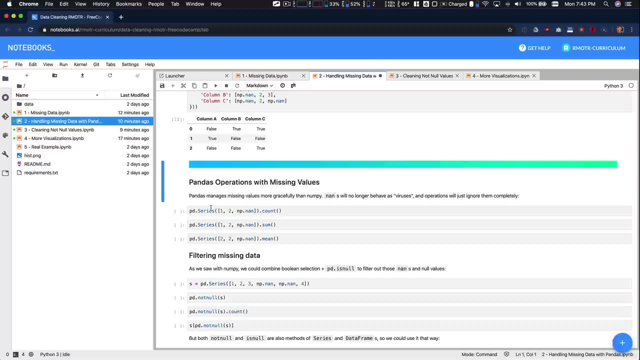 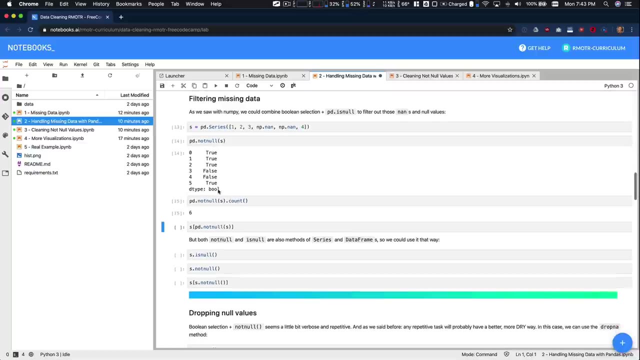 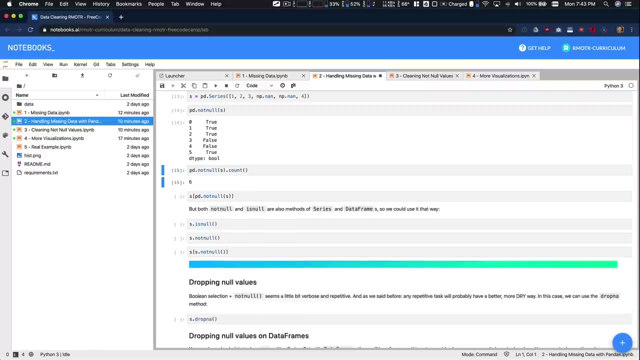 are applying or actually function, And again, the same thing works with not entire entire data frame. So something we do usually is, if you look in to no, no and no, a few hacks that we usually apply are the count and actually this be the sum of all the no values or not. 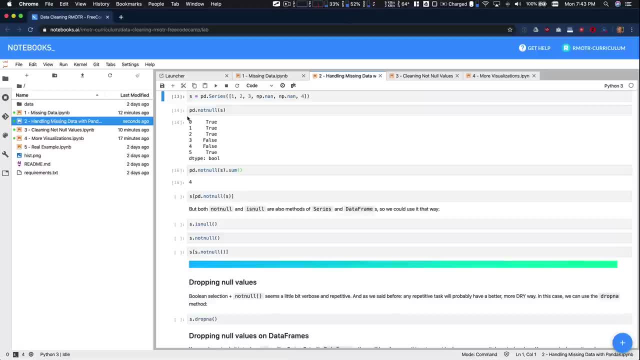 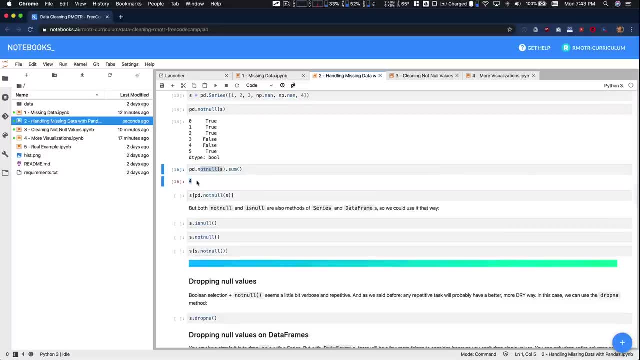 no values. So we have this entire series. we can say how many not no values we have And if we sum those not no values in this case, we're going to get a result out which is the entire, the entire summary of the not no violence we have asked, And the same thing is going. 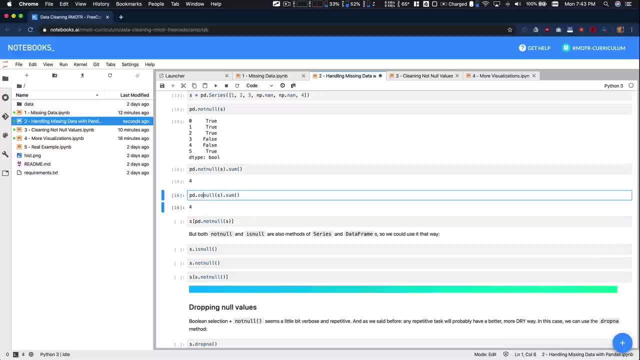 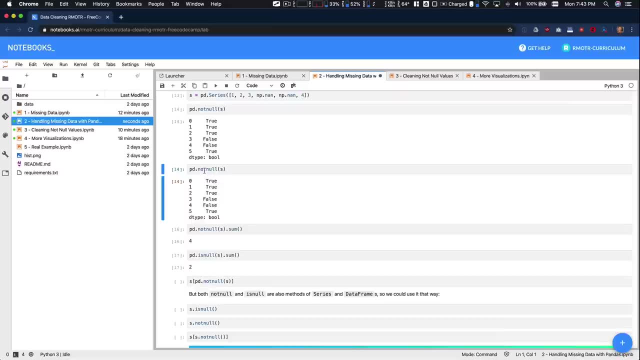 to happen if we say is no, So if I do, here is no, some we're going to get how many no values we have, And it's pretty much the opposite Of this question is no, And the way it works is in Python. booleans are pretty much integers. 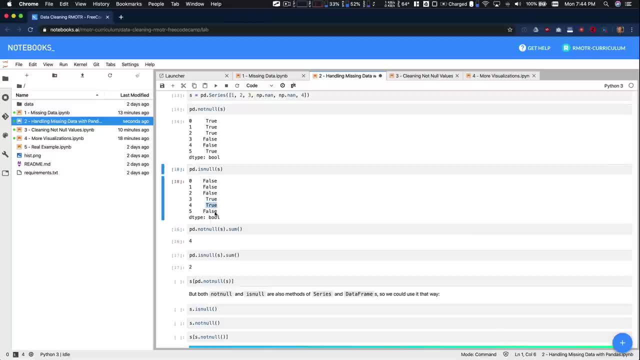 there are ones and zeros, So every true file is going to count as one and every false going to count as a zero. So if you ask for the sum of a Boolean series, you're going to get out the result of the number of truths that are available in dot series, right? So 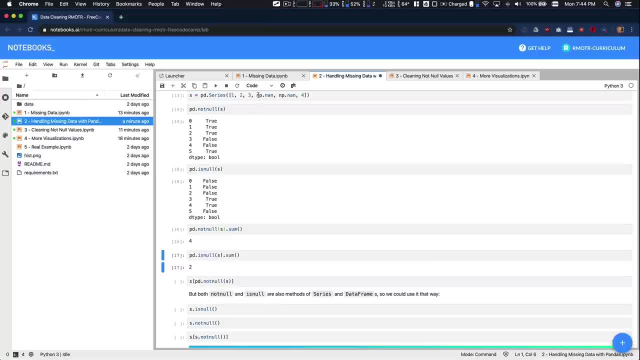 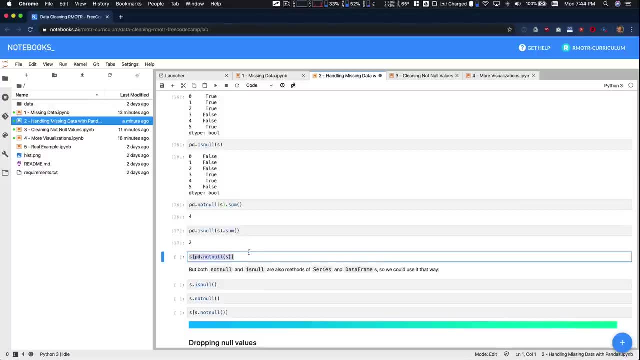 in this case we have two no values. we ask how many no values we have. And if we say, ask how many no values we have, is no dot sum we get to out. you can use these tricks to filter the data with a series. So in this case we can say: give me all the values that 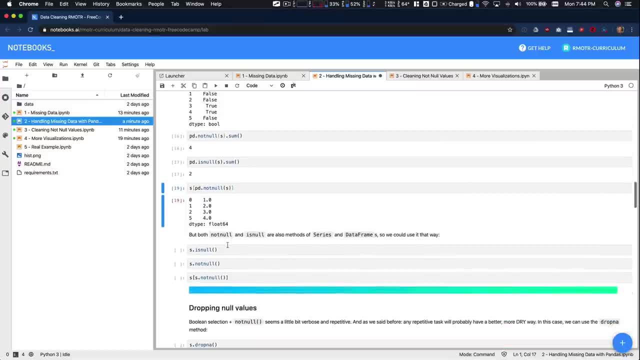 are not no rights, just not know. Also, something interesting is that both for data frames are for series the not not normal is. normal is an a, not an, a methods also sorry, functions also work as methods. So in this case we can say instead of: 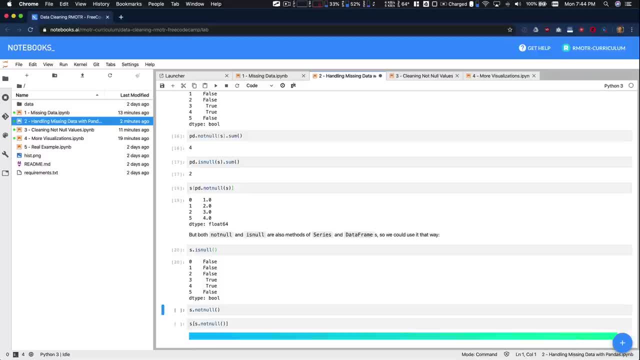 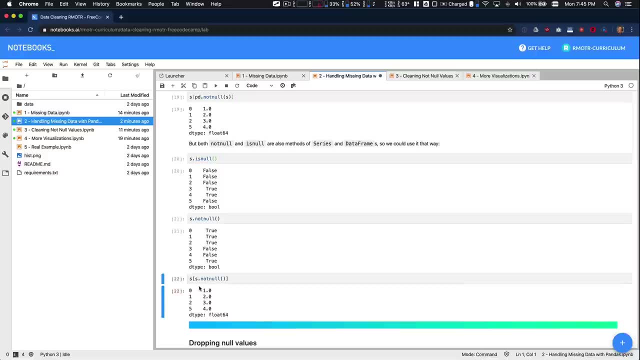 PD dot, not no. we can say: s dot is no, s dot is no. So now it gets a little bit more, a little bit simpler. But if the final objective of these call s equals, sorry s, selecting only the values are no, no was to drop the no values. then there is a simpler form, which 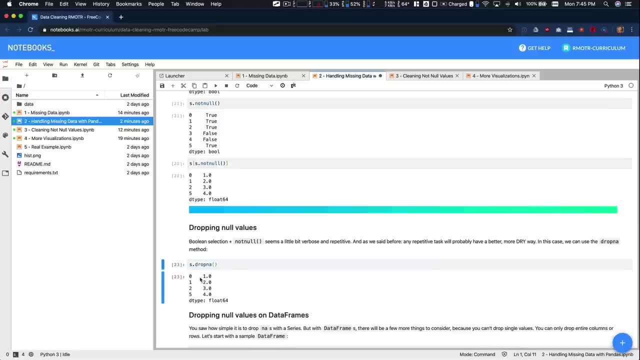 is drop an A. Okay, so in this case we can say: s dot drop an A And we're basically invoking anything that is happening here. we're missing. we're just excluding, sorry, all the missing values in the series or the data frame, because this also works for data frames. So what's? 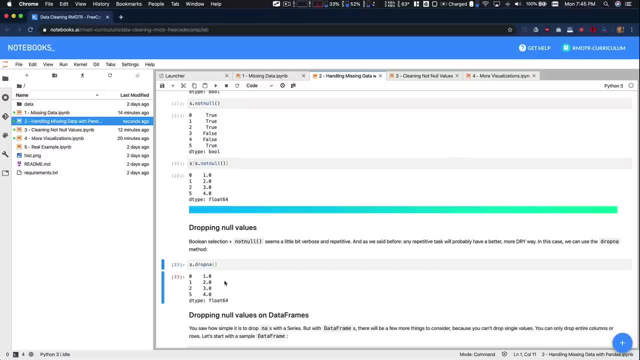 the one. one important thing to remember here is that all these methods are immutable. we are not actually changing or modifying the original series. the underlying series is not being modified. there is a new series that is returned. So if I invoke s, I'm going. 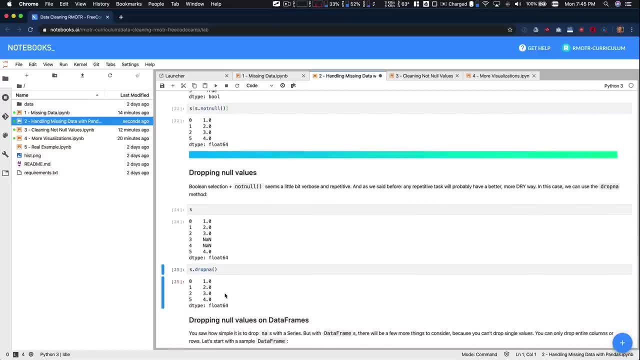 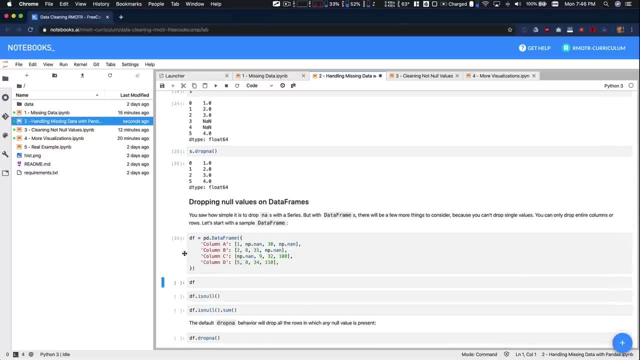 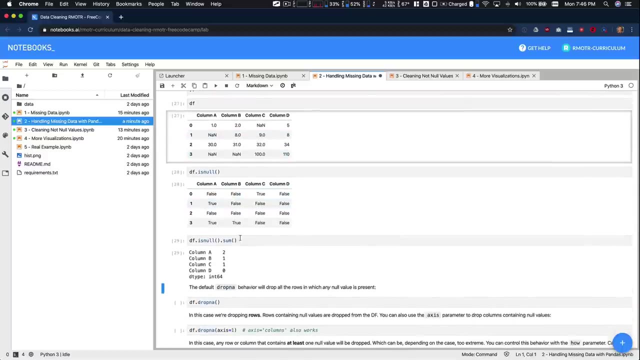 to say s again. this thing has is not modifying their series. you're creating a new series And that's the one that hasn't. that doesn't have the missing values. Everything we've said also works for data frames. So right here, with this data frame, we can say how. 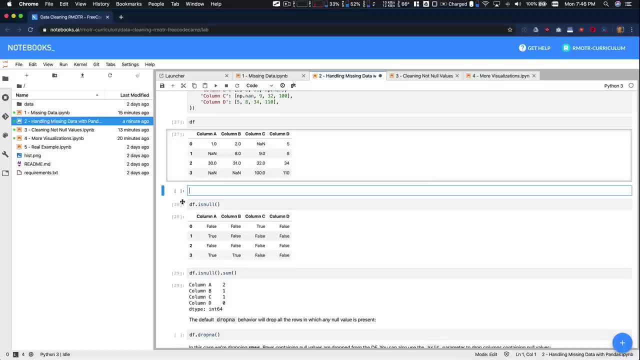 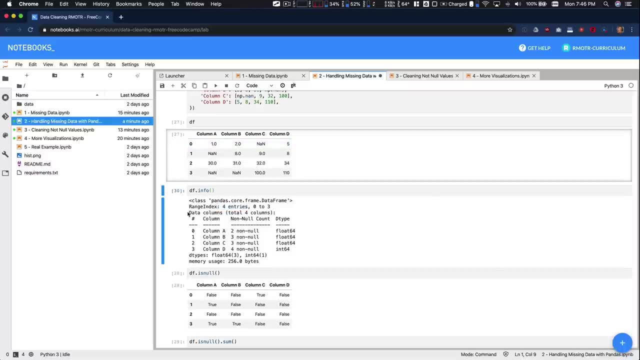 many, right? the first thing usually is to start with an info method, right? So we have info And we see that there are in total four entries, four rows. we can also do a shape If we, if we need more information about the structure of our data. So there are four rows. 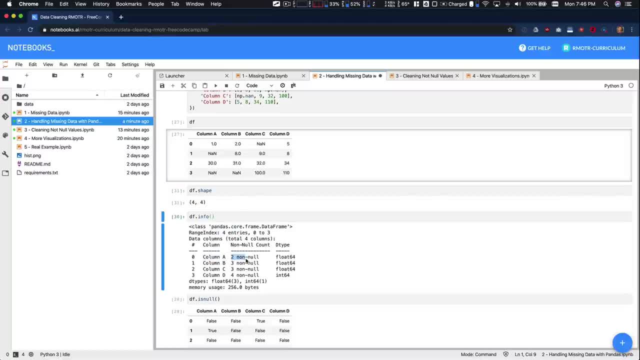 four entries in our index. column A has only two non, no values, So that means there are two values that are actually no, no, sorry, no. there is column B that has three no, none, no values, So that means that one value must be known, And that's for column B again. 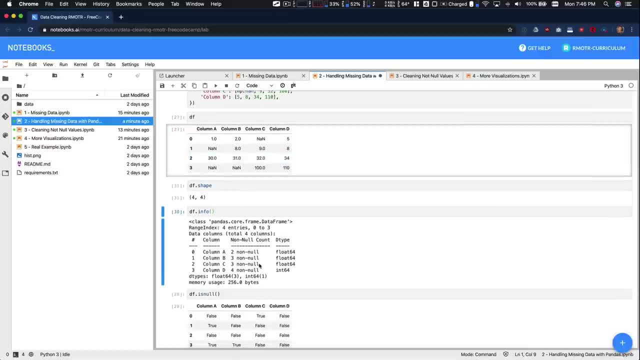 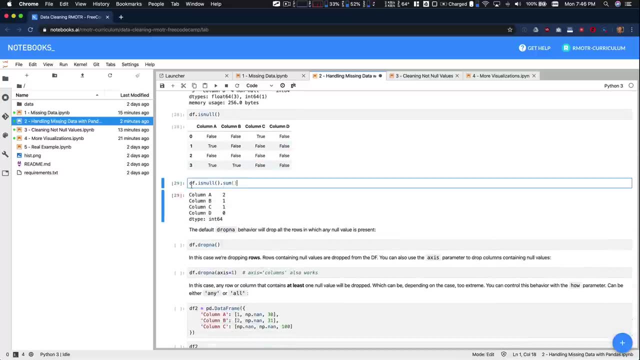 So usually info gets you very close to understanding the structure of the data frame. So if you understand the structure of your data frame and how many values there are missing, the same thing happens with some. we can just do: the F dot is no is an A, and then some we're. 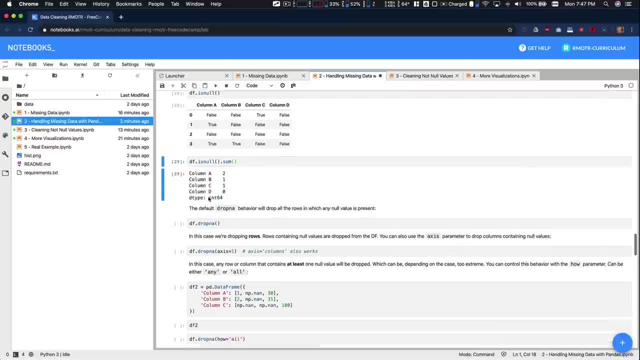 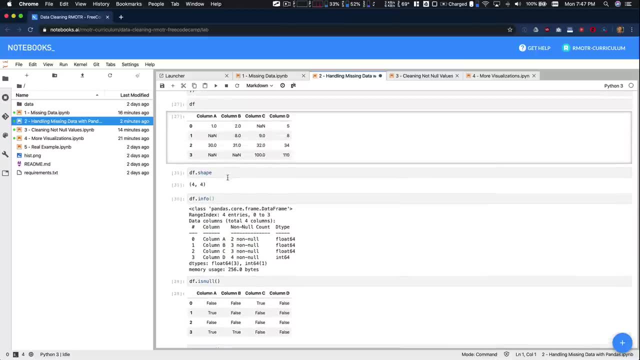 going to get a quick reference of how many no values we have in that given data frame. drop an A works in the same way, But there is a significant difference. The way drop an A works in a data frame by default is by dropping any row that has at least one value. 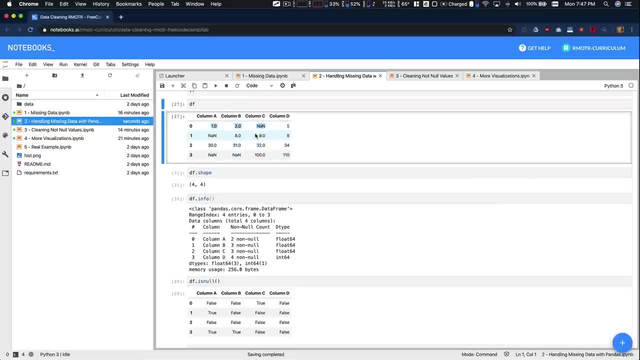 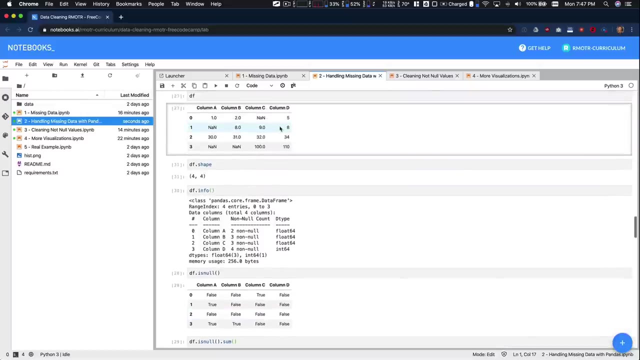 No value. So these row has a no value dropped. These row has a no value dropped. These row has two no values dropped. This is the only one that it's not being dropped Right, So it's very harsh in that respect. You can change that to make it to the column: only only keep. 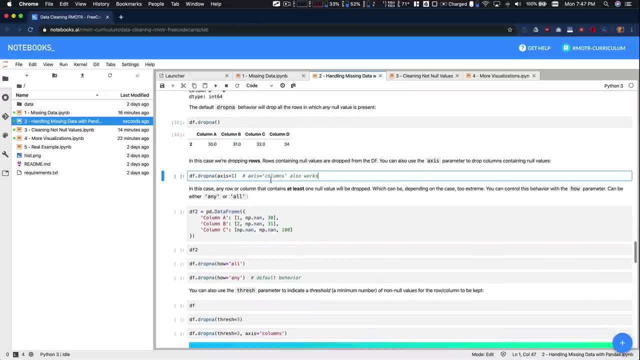 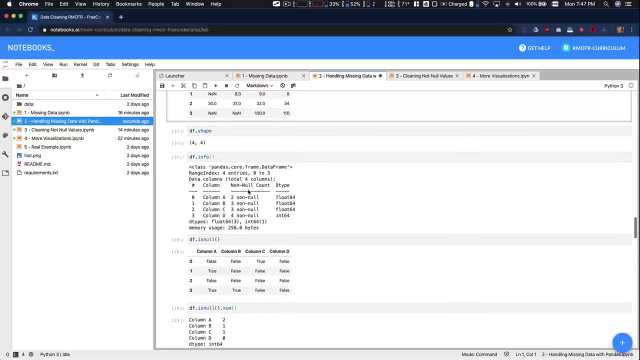 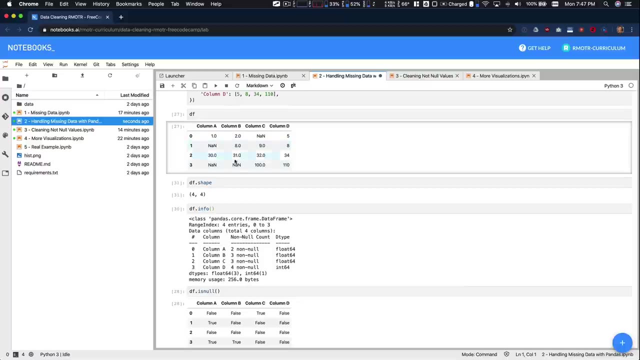 the column that has no, no values, And that's by switching the axis, equals to one, And there is also a way to select: select a subset or threshold, So only delete rows that have less than three valid values, For example. in that case, you're going to use something like the strategy of the drop in. 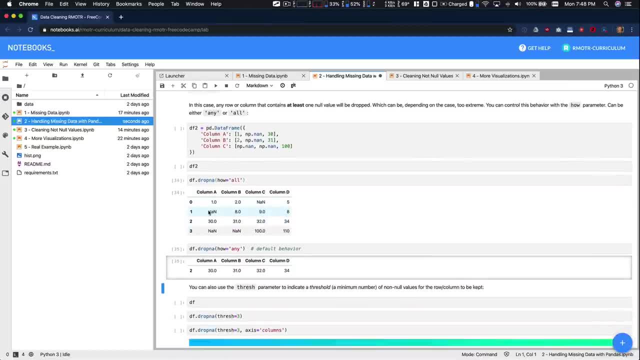 a you're going to say: drop the columns, the rows, sorry, or the columns, because it is also works for columns that have all the values and no, or drop the the. this is the default hey behavior. drop all the rows that have any. 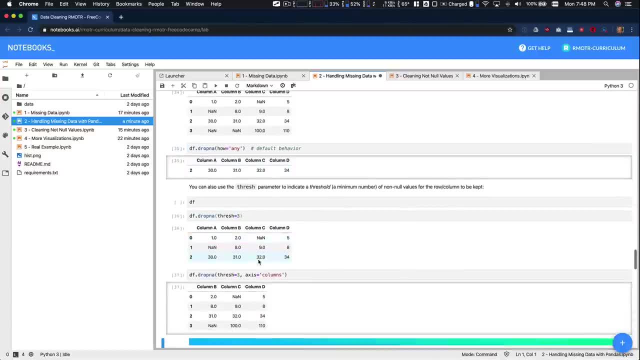 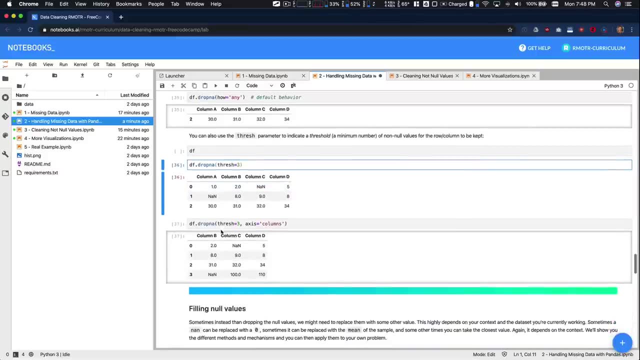 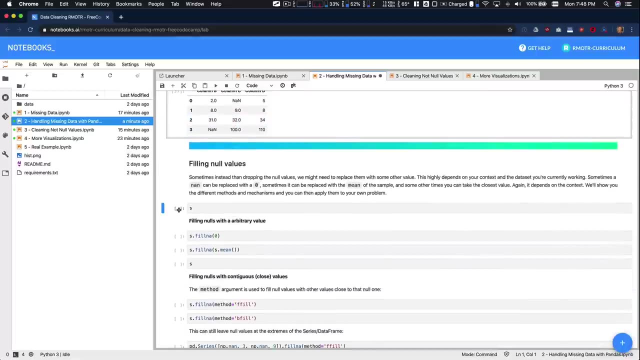 value in an a or specify a threshold, which you are basically saying: I need this amount of valid values in order to keep the the row. It's the way it works, not which wants to drop is which wants to keep, based on the threshold. So once you have identified the no values, it's extremely. 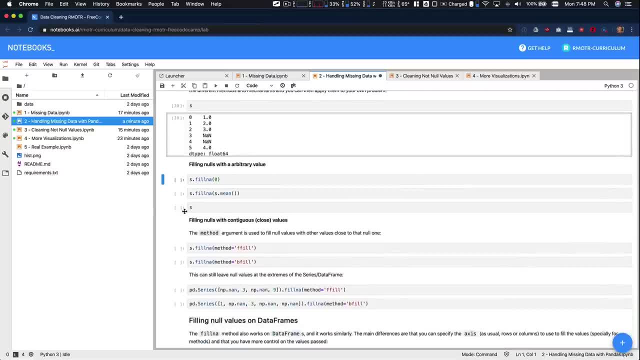 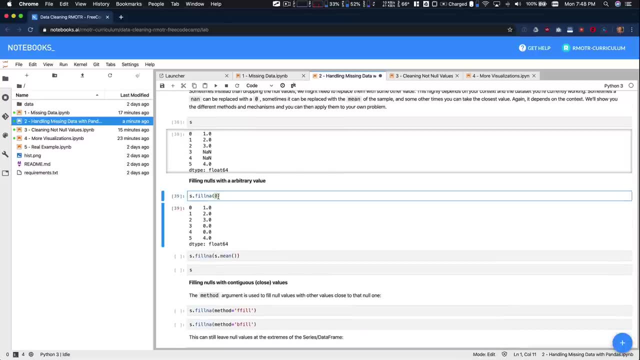 simple to clean them, to sort of fix them. So the first method we're going to see is filling a within a particular value. we're going to say from this series: I want you to fill the blanks or fill the missing values with, or fill the ns, fill them with our number. 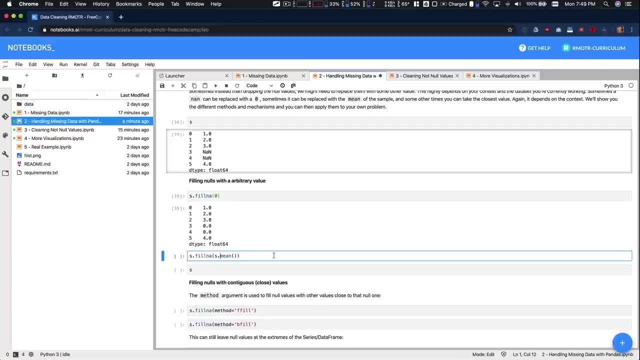 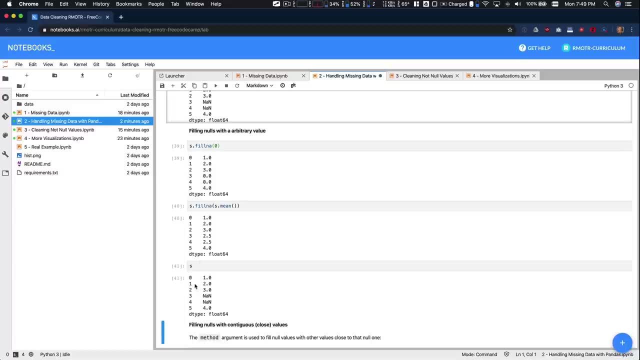 zero in this case. So these two are number zero. or, of course, you can use any statistical method you want. In this case we can use the main. Remember this is not altering the series. the original series is still the same. we're not changing it, It's creating new series. 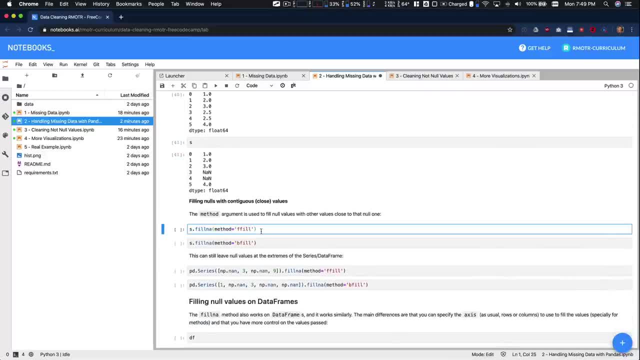 because all these methods are immutable. The following method is: or this the following following way this method works is by passing a method which is for field or backward fields. these are the possibilities And basically the way it works is it's overflowing all the. 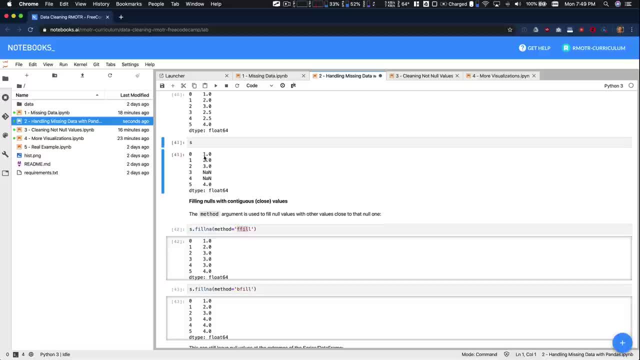 values top down, at least in for field right, starting here, it's dropping this value here, dropping this value here and dropping now three here. as this thing is a none, it gets replaced. So this thing is three now, which gets dropped here, And now this thing is three. 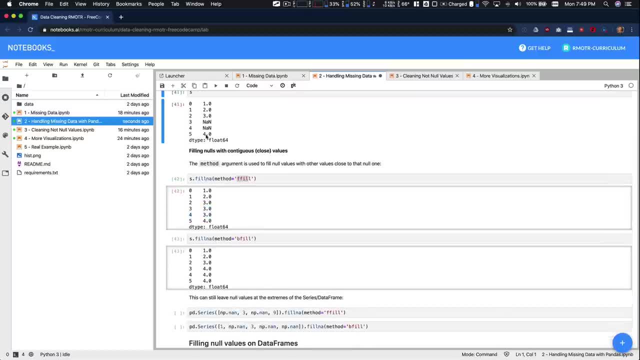 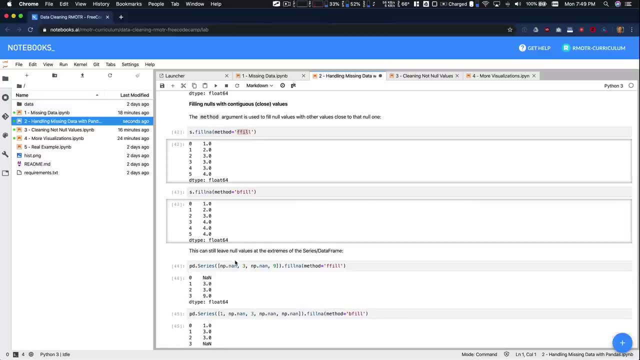 again. So that's what we have right there. And of course, backward fields works in the other way: starts with four and movies moves it here and then moves it here, etc. You have to be careful when using these, because if you have no, no values at the beginning or 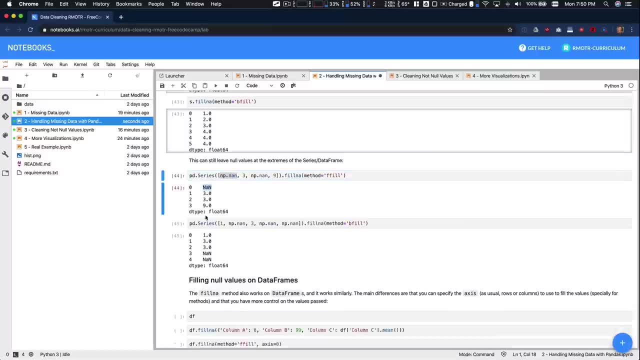 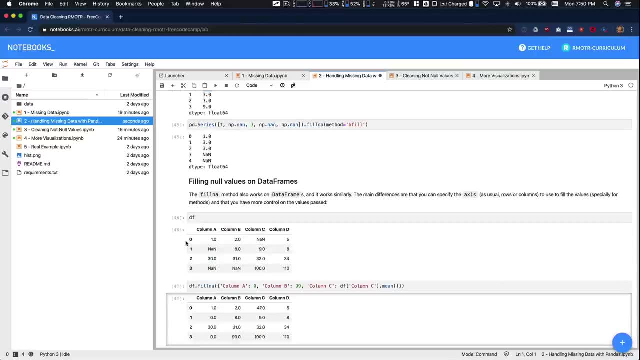 the end, then you're going to end up again with no values because there is nothing to feed forward, Right? This is the first value you have in there And all we've seen also works for data frame. So both backward field, forward field, for both in terms of 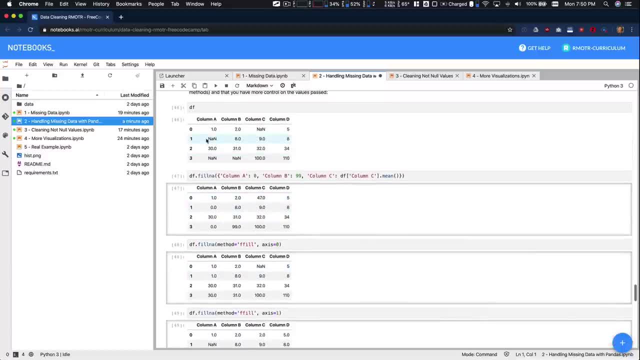 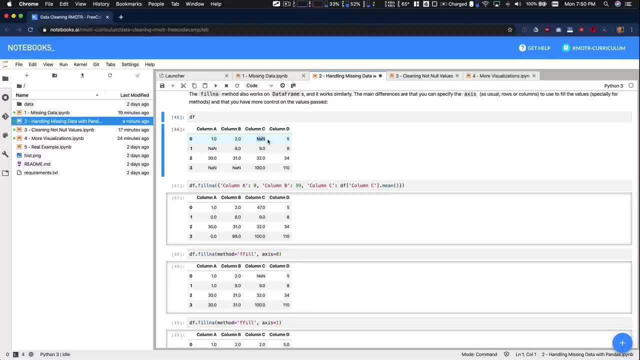 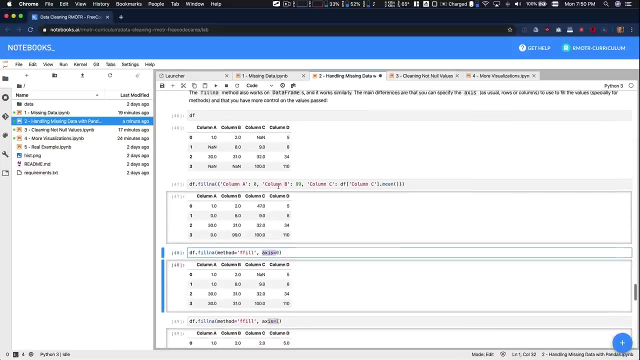 rows for filling right. so we have. we have these values data set. So we do for field row base going to be 122, here two and then five right, so that's going to be for field axis one. if you use for field axis zero, then it's a vertical filling right. it's. 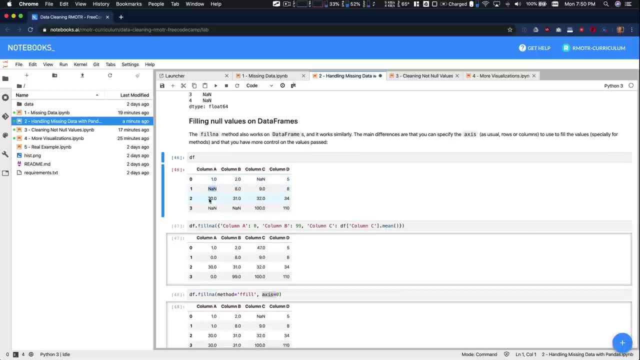 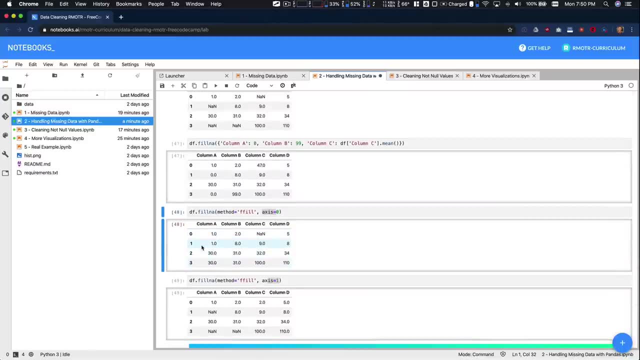 going to go here: 1130 30.. So that's for the column that is right here: 1130 30. So it's either for for filling in in- sorry, this direction for filling- or it's going to be in this direction. 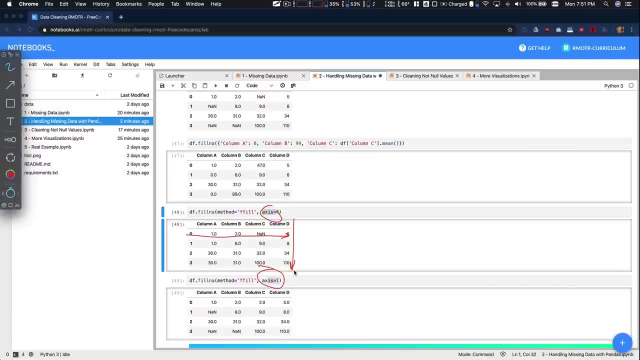 depending on the axes that you are passing, And actually let me we're going to put the correct forms. with axes equals zero, it's going to be columns. it's going to be this direction. with axes equals one, it's going to be row based. So it's this direction, right. 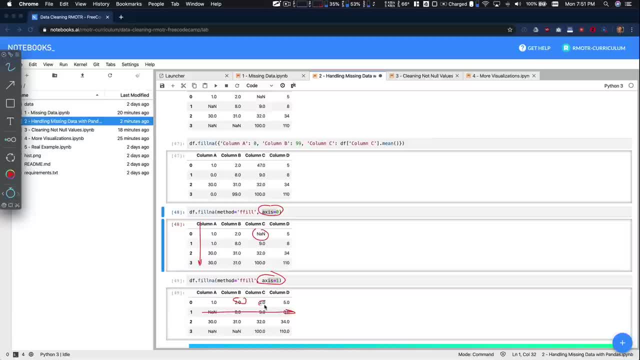 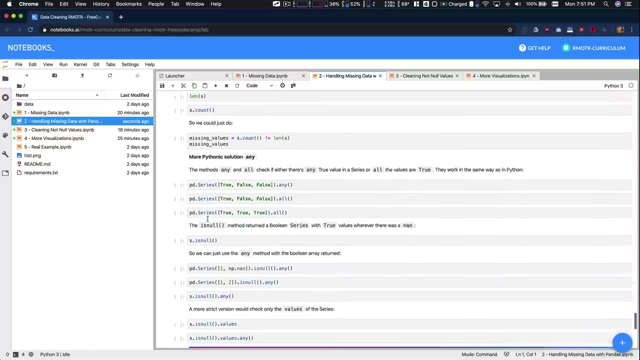 So we had a no value here, that code, So we're going to fill in this way. Okay, moving forward, we what else we have? we have here checking for values, And we're pretty much saying this already. you can use the. 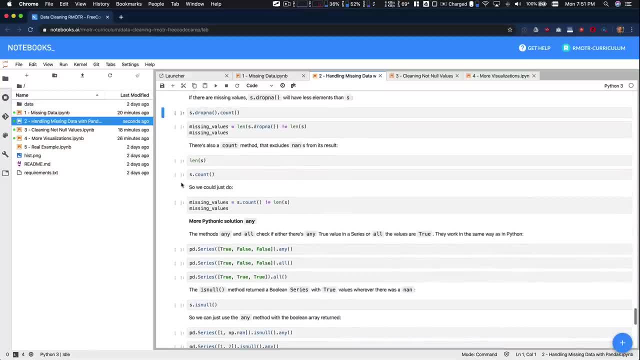 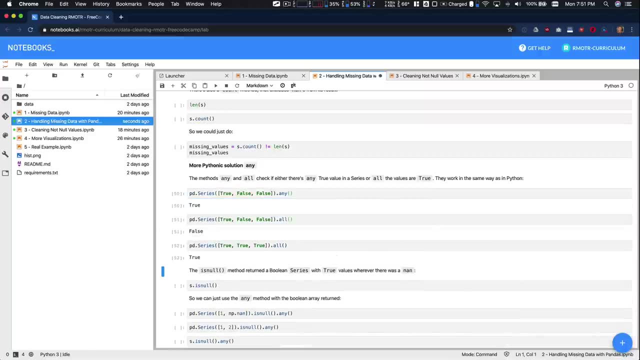 is no the some method to get how many values you have. And there is also any and all which will give you very quick. These are usually called Boolean tests. you can say, ask if there are any values are valid or if all the values are valid is just to build more complicated. 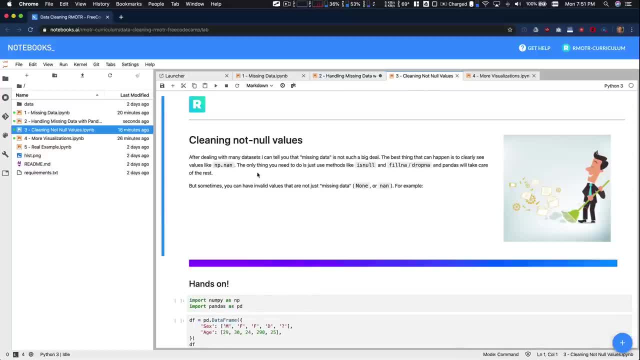 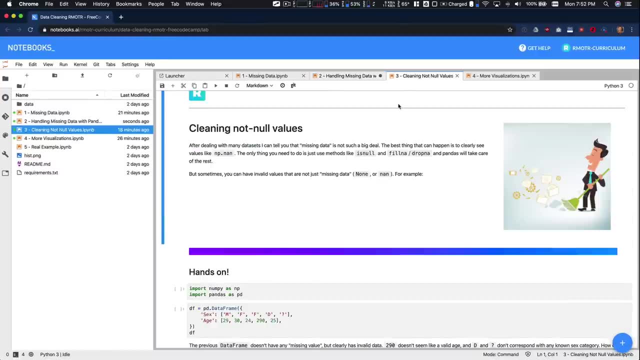 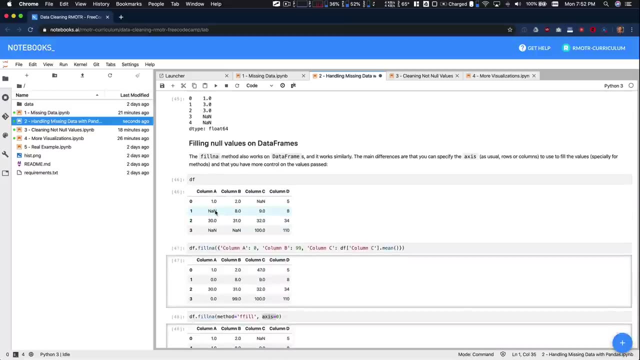 queries. So so far, so good. So the the process we said was at the beginning we were fixing missing data, missing values. there is nothing in there. we have read a data frame- where's our data frame? right here. we have read our data frame from CSV, from a database, and the 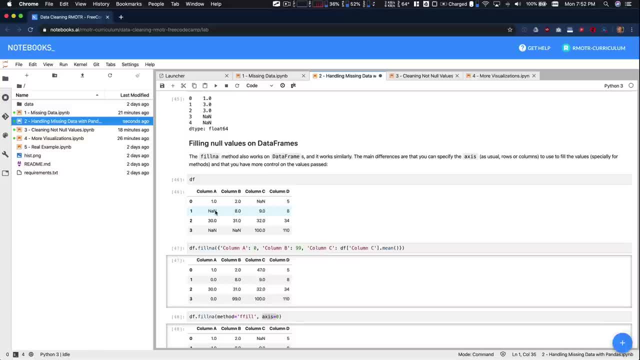 value is missing. No, there's a hole in it. So we have quickly identified it with is an A or is no. We were able to drop the ones we didn't want to keep- drop an A- or we were able to fill the values we wanted to fill. fill an A. that was simple. isn't a drop in a filling a? what? 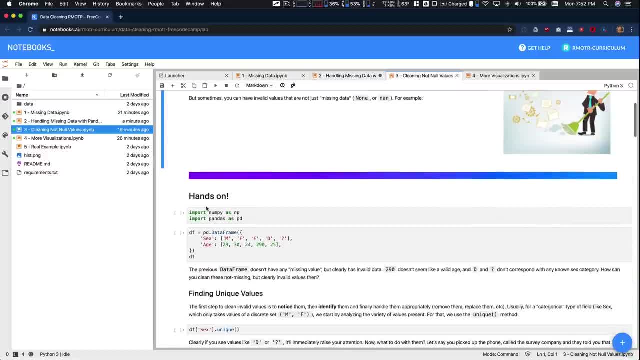 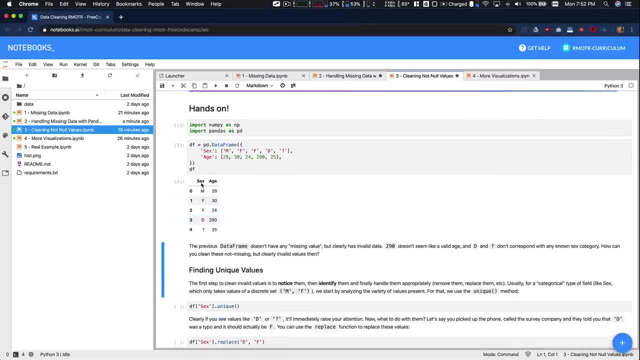 happens when you're cleaning data that actually has a value, so there is no nothing missing, But those values are invalid. So, for example, here the sex column is a categorical column that only accepts m on F, D, on question mark, Though we don't have a question mark. And 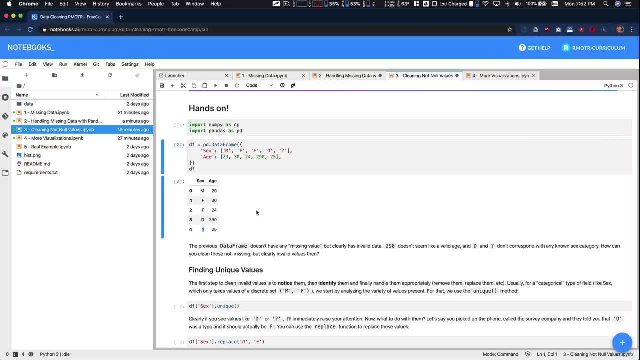 those are invalid. they are. it's very simple to see an invalid value here because it's completely out of the scope. The same thing as we have, for example, question mark in the age column, where we have. we have a string in the age column. it's very simple to identify. 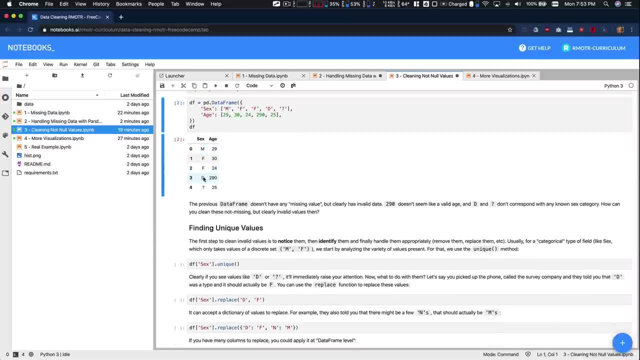 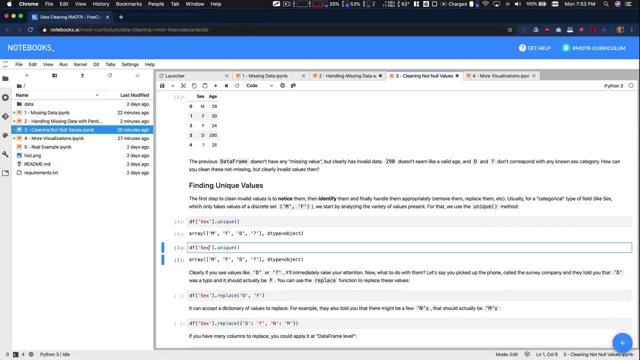 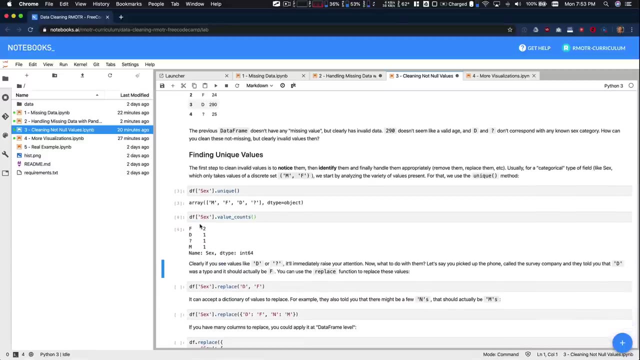 that how we're going to clean those. let's start with sex first, because it's simpler. in this case, The first check we can do is with either unique or with value counts. I'm going to use value counts. we've seen this method before. it's a quick summary of all. 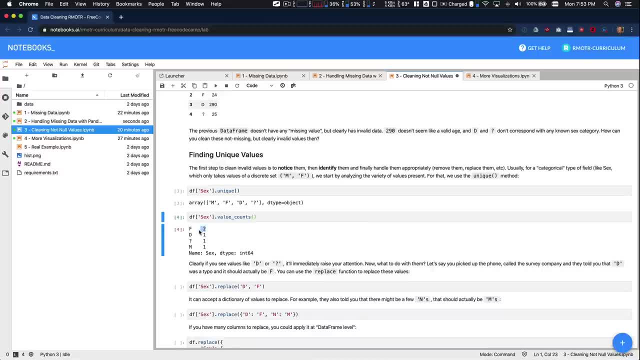 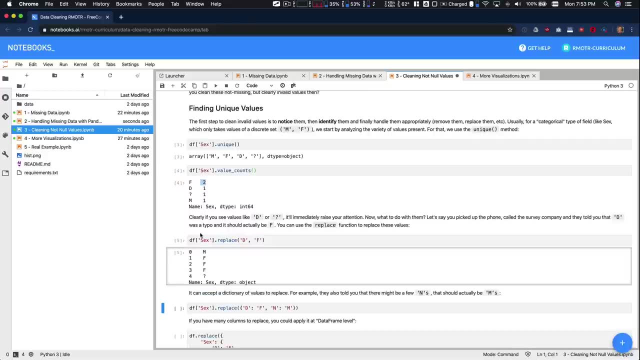 the unique values you have And in this case, finally, counts, also gives you a total count for those values. How can you fix them? Well, there is a replace method which is extremely intuitive. you can just replace. in this case, we're changing all of these two F's and all. 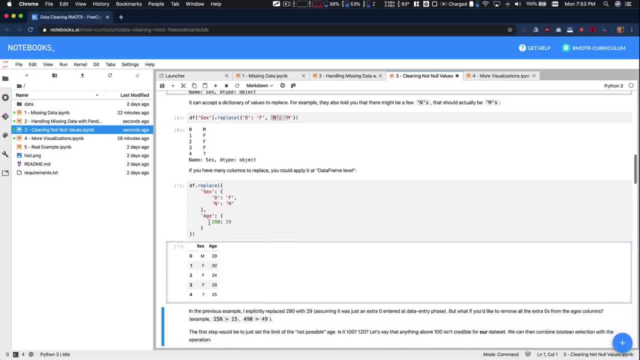 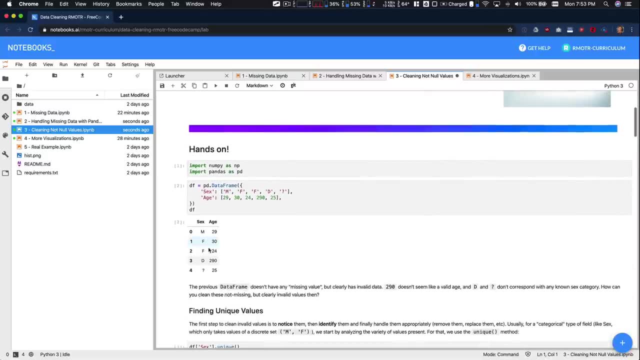 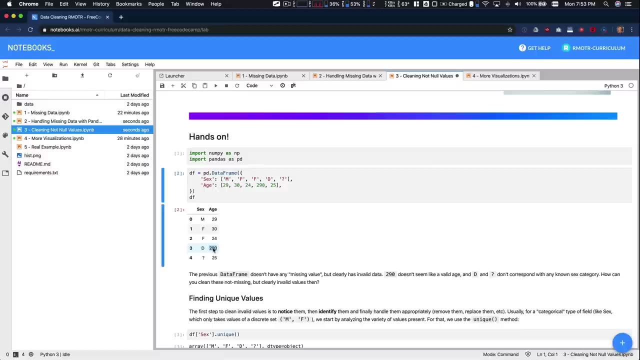 the N to Ms And it can work in multiple columns For those values that, again, we said were more complicated to fix, like in this case. we know age- in this case is 290. And we know, because we know the domain, that 290 is an invalid age. 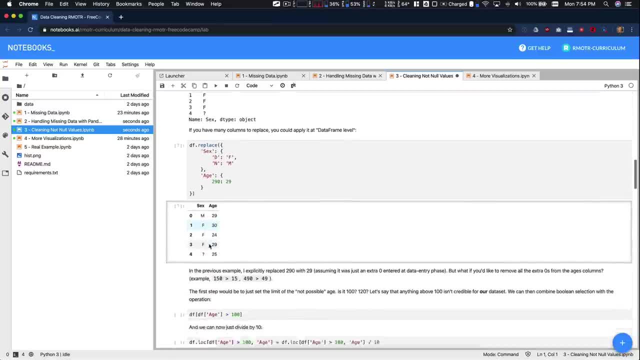 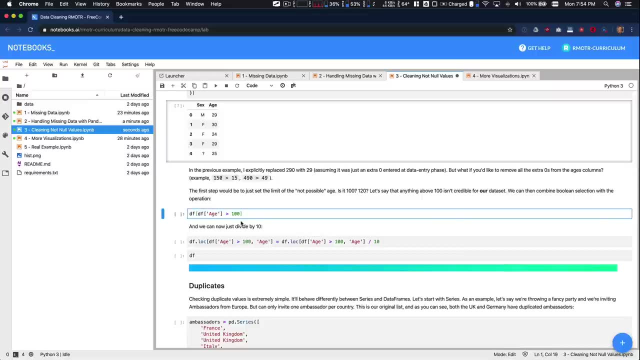 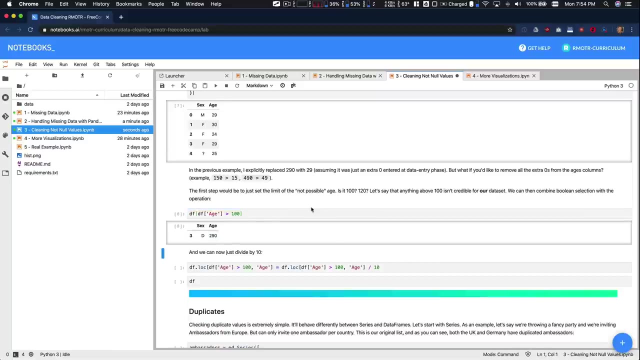 for a human. So we will need- usually in those cases we're going to need- more complicated fixing and it will involve more programming. That's the reality. you have to be better at coding. In this case, we know that this value is invalid because it's probably an extra zero. 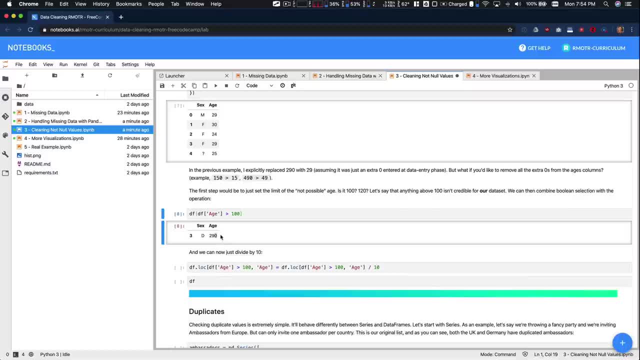 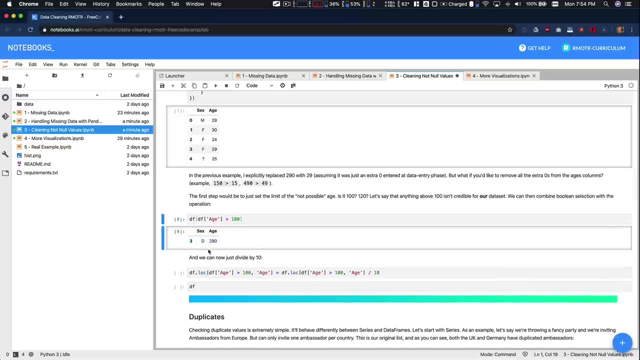 So all these values, you are pulling a CSV with ages and there are a ton of 180, 290, 30 to 320,, for example, invalid values out of 100, right in the hundred places, And that's because there were typos when they were creating the ages. So how are you going to fix that? 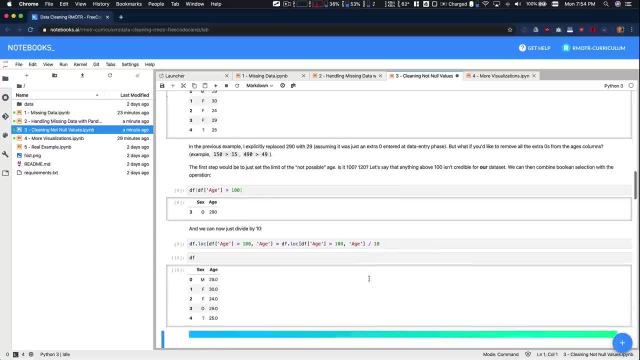 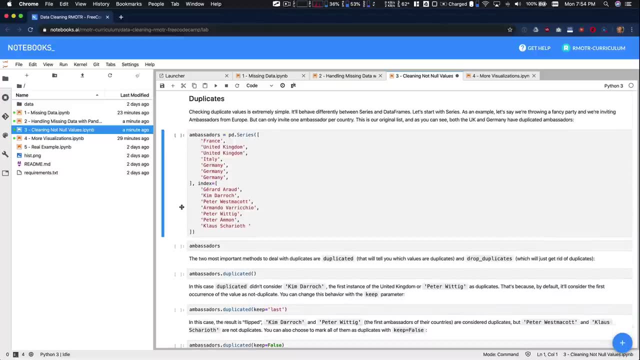 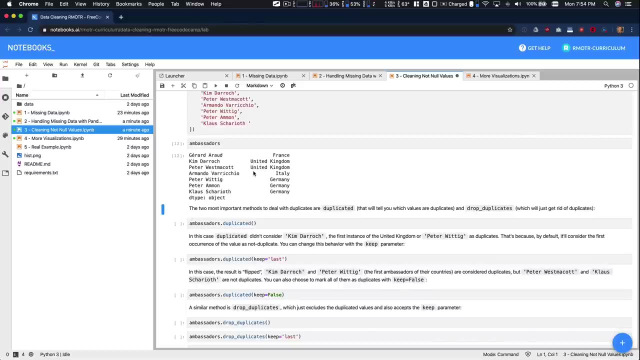 Well, in this case it involves a little bit more programming. we're dividing everything right By 10. So also something that might be useful is dealing with duplicates, And we need to first define what's going to be a duplicate value. So this is. this is usually a little bit more. 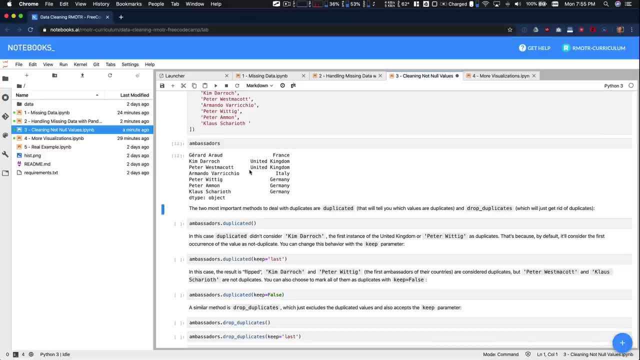 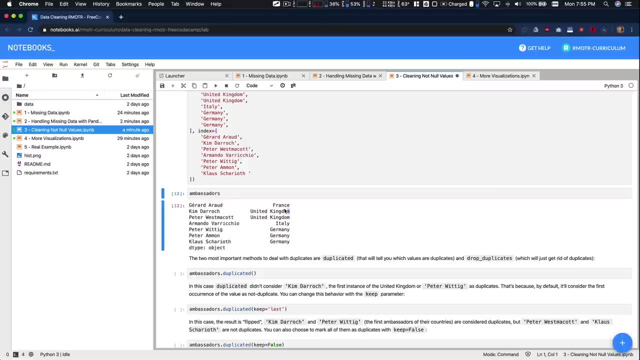 political, if you want. you have to define what's going to be a duplicate. In this case, we have a series that contains ambassadors and each the ambassador is the index. the country of the ambassador is going to be the value right, So this is usually the important. 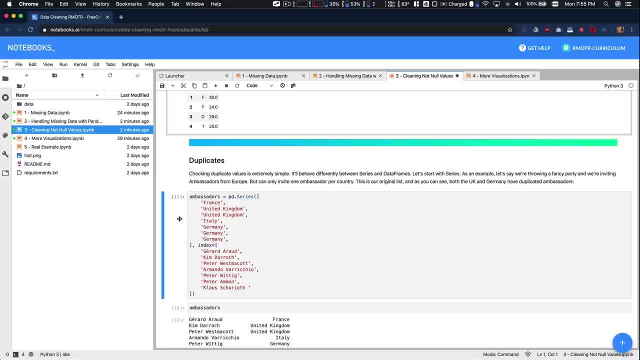 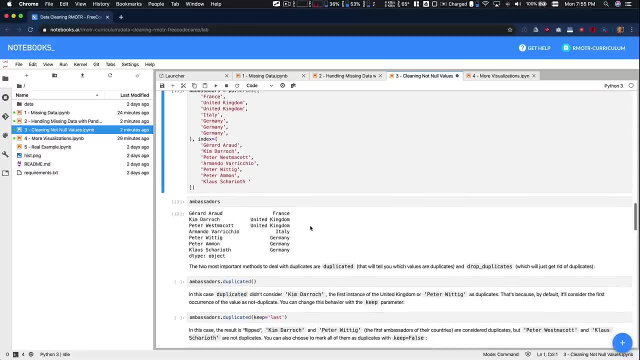 part. the reading here says the word conducting a party and wanting to invite one ambassador per country. we don't want to repeat ambassador ambassadors. So in this case, what's going to happen is that these two, in our human eyes at least, we can click clearly and quickly. 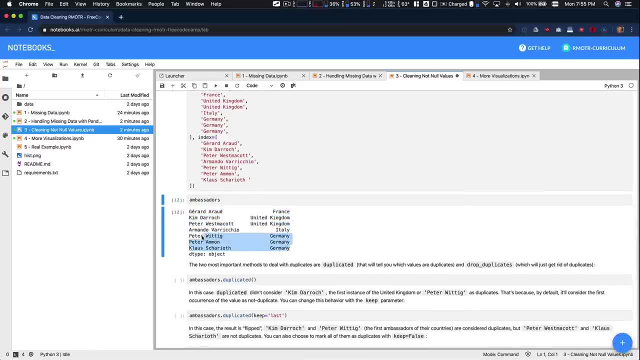 see that these two belong to the same country and these three belong to the same country. But here again we have to define which ones are the duplicates, if you want, and which ones are not duplicate. So, for example, maybe we're going to put a duplicate in here and 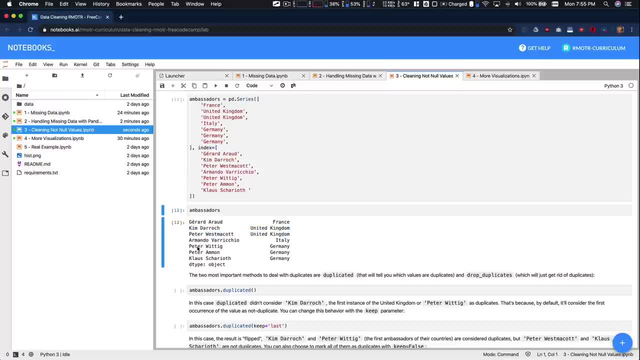 we can say the first one is duplicate, or we can say the last one is duplicate, So this is the first one, not duplicate, And or actually we can say this: the last one is the one I want to invite. it's not to duplicate, So we're going to have political rules if you. 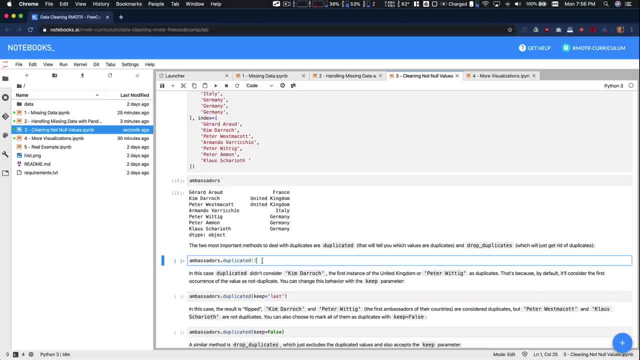 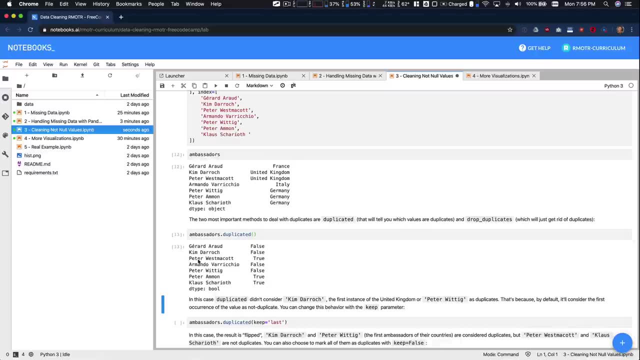 want for each one of those. So let's see the duplicated method and the way it works by default. By default, the duplicated method is going to return true for duplicate. for all the it's it. I'm going to invert it. it's gonna not treat as a duplicate as the first. 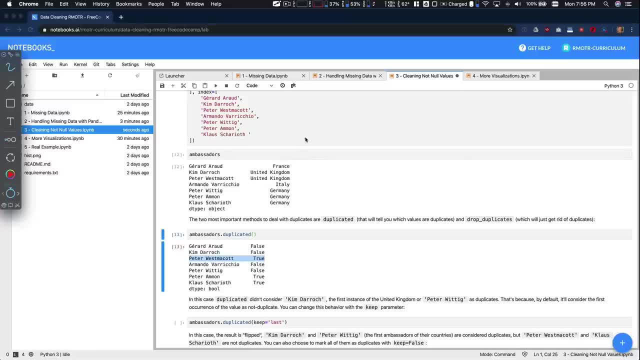 instance, that it says: So the method is actually walking top down right And it's saying: do I have friends? No, I don't have friends. I'm going to keep it here because I it's the first time I see friends. Do I have the UK? No, I don't have the UK is going to keep it. 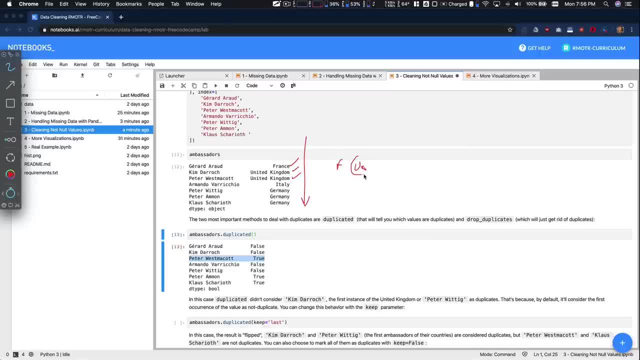 here. Then it sees the UK, again, realizes the UK is already there, It's a. it's already there, It's already present. So this one is going to be considered a duplicate. Italy is here, it's fine, The first occurrence of Germany. it's fine, writes down Germany, but then it 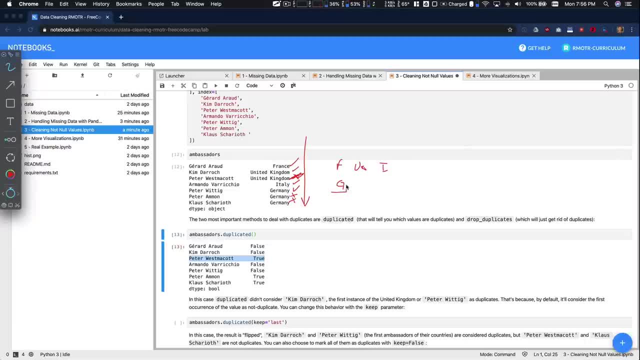 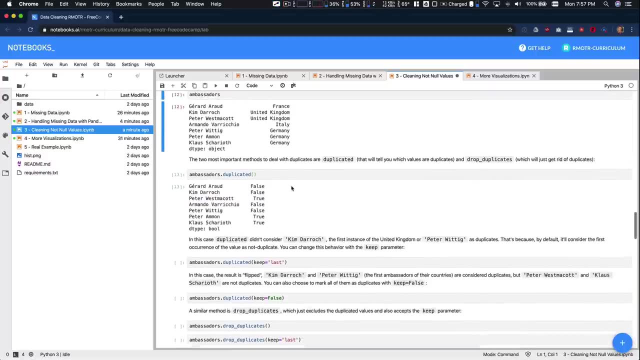 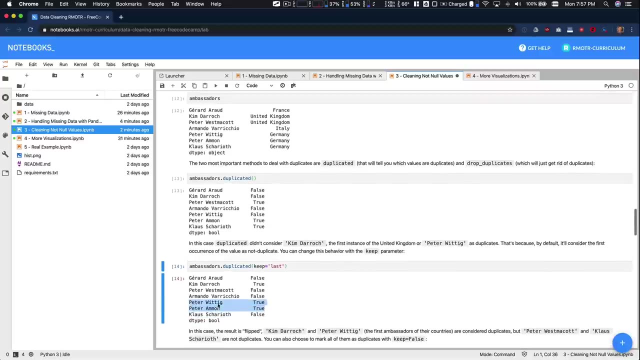 says Germany, two more times And it realizes that Germany was there. So those are now duplicates. That's the way it works By default. we can change that and change it to last. So the last element is not considered to be duplicate And the other two are considered to be duplicates. 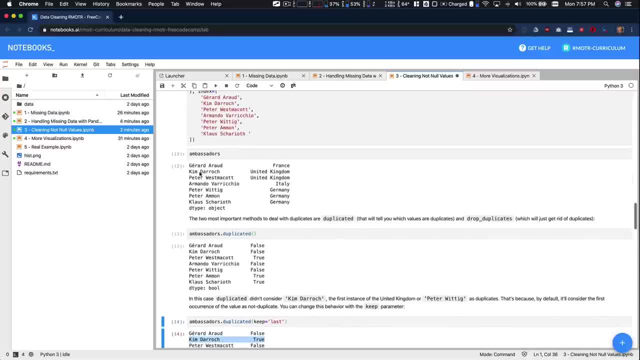 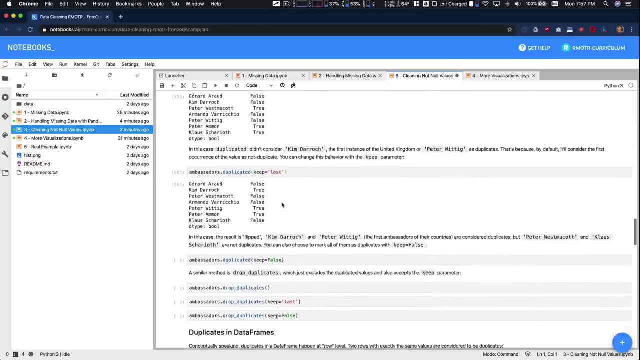 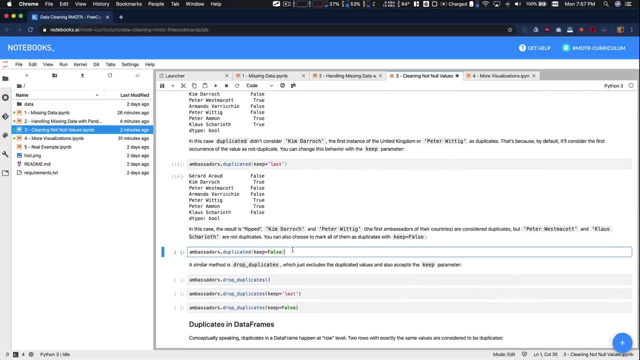 And the same thing here, Kim. here is the one considered duplicate. So it's either top down or bottom up, depending the way the parameter you're passing. it's either keep default or keep last, Or you can be a little bit more harsh and say everything duplicated is actually. 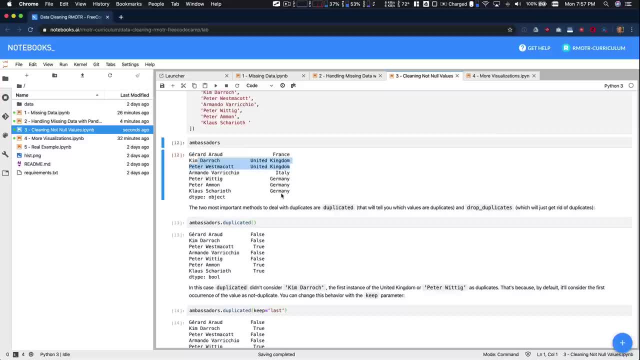 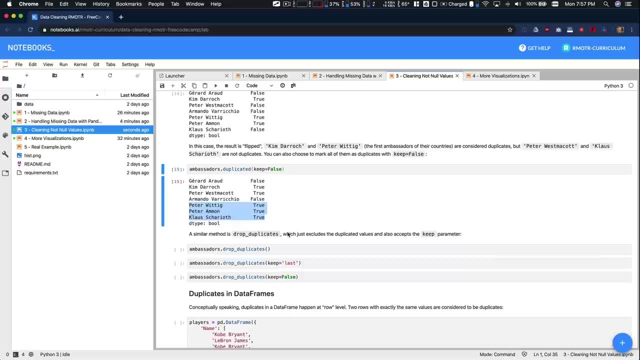 to be needs to be considered duplicate. So these two are duplicates And these three are all duplicates, As you can see right there, Similar to the duplicated method, which pretty much tells you which values are duplicated. It's it helps you identify them. You also have the drop duplicates And in this case, 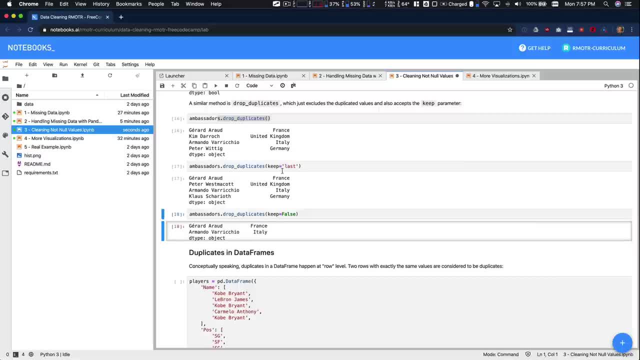 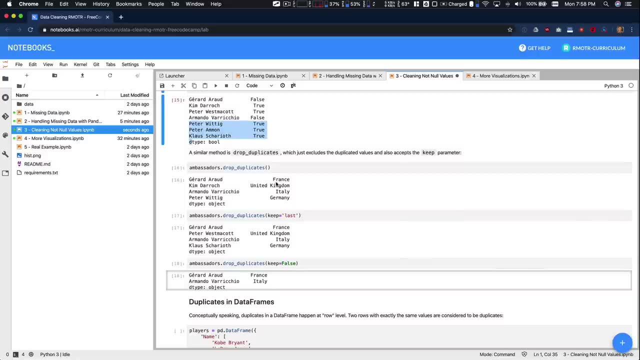 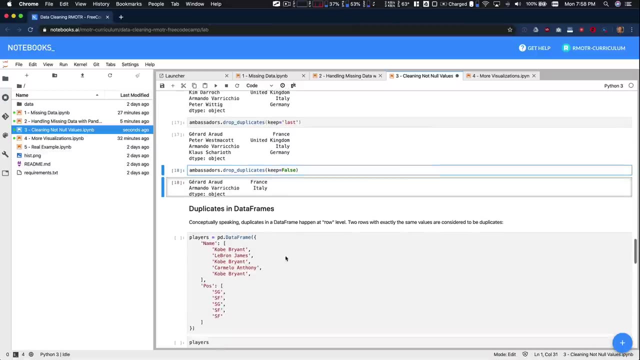 what this method is going to do is basically the same thing as before, but dropping all the values that check for true. right of the method is: if the violence is missing, it's going to just drop it, And the same rules apply: default, last and false For subsets. in this case, what we 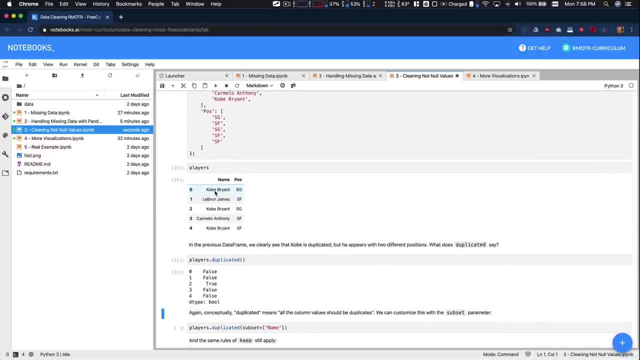 have is we have multiple. we have multiple players in the data frame, But what happens is that this player, Kobe, is present three times. for human eyes, we see Kobe three times. what is going to happen here is that the way we're going to think about duplicates is by 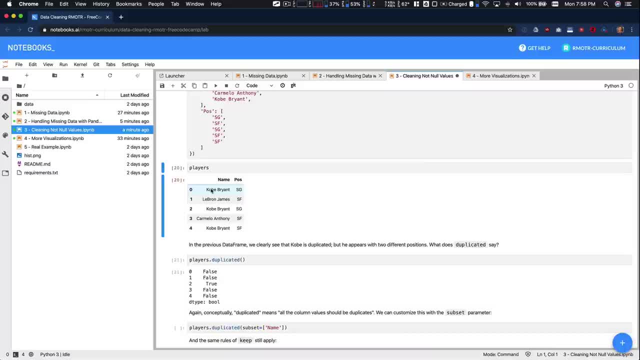 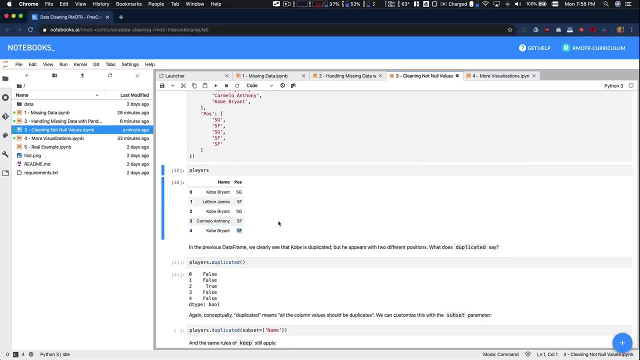 understanding the correct subset that we should check. In this case, Kobe playing as an SG is duplicated two times, but Kobe playing as an SF could be considered different player, if you want, because maybe it's a different season or it's a different, a different position. 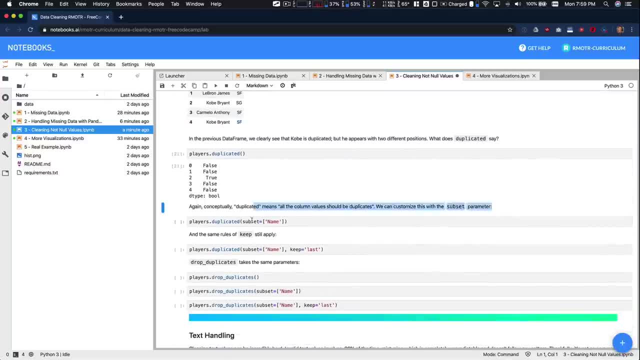 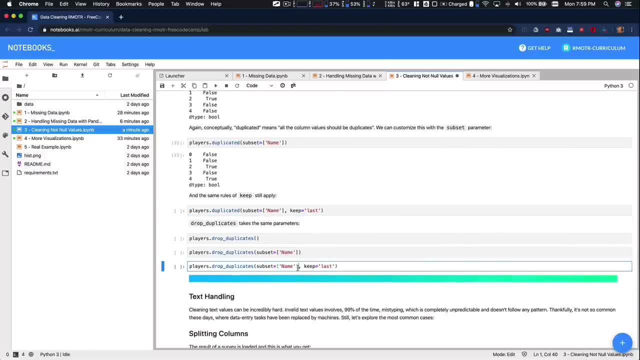 they played. So in that case we need to pass what's the subset that we are going to consider duplicate, only check for the column name, or check for the column a name And then, or not check for the column name, which is the default. it's going to check the entire. 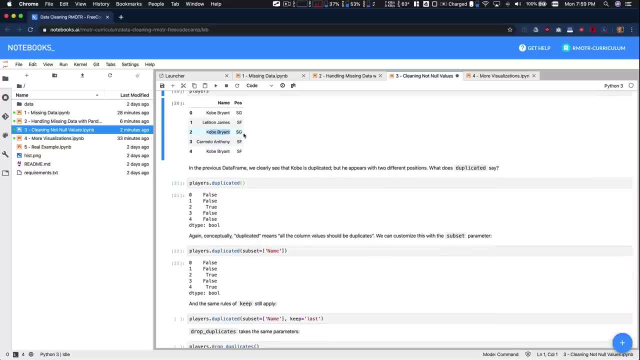 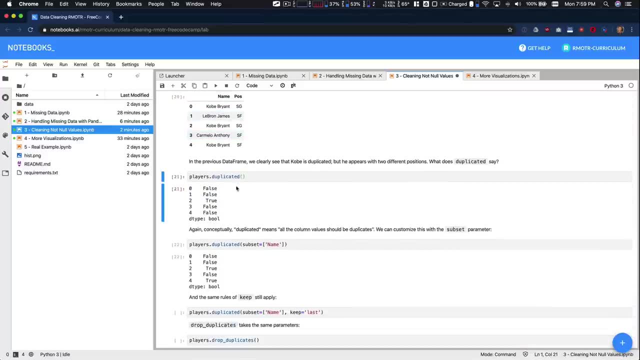 data frame, And when that happens, then these two are considered to be duplicates. So these one is a duplicate. with this rule, if we put keep last, sorry, keep falls, both are going to be considered duplicate. So the second occurrence is the duplicate one And the last. 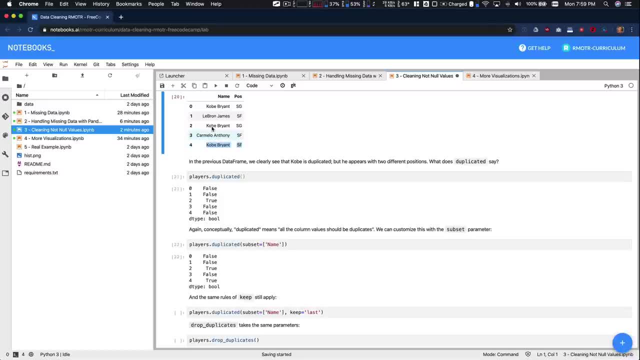 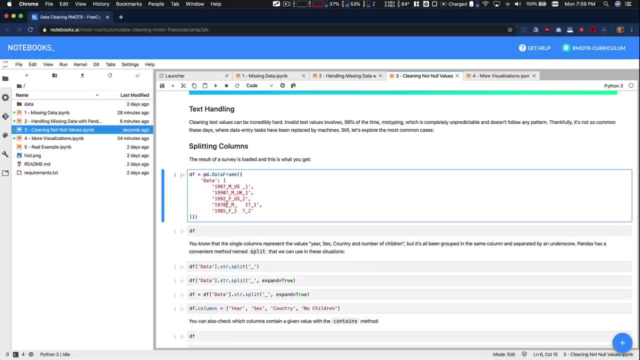 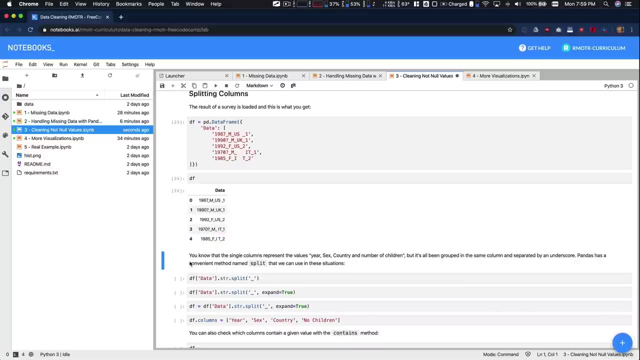 one is a completely different row because the the value in position is different. That's a way It works here, Moving forward with more cleaning of values, we're going to talk about string handling And this is a very neat feature of pandas that special types of columns will. 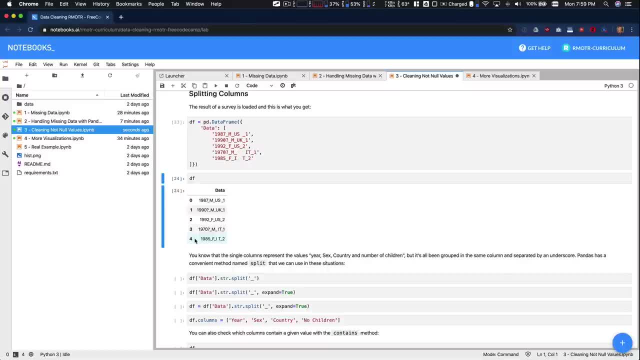 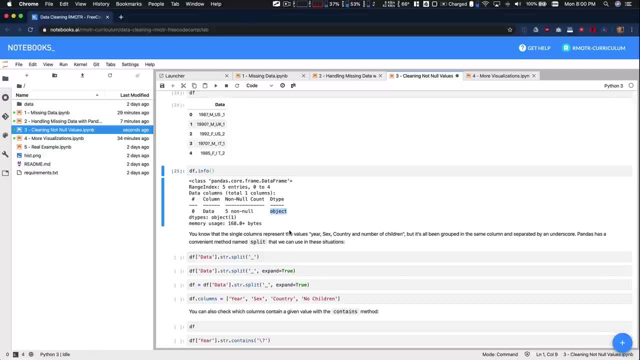 have special attributes. So, given the column type, so the f info, which is an object, which is a string right in pandas, that all the strings columns are going to have this special attribute which is STR, all the daytime columns, something we're not going to call it, but 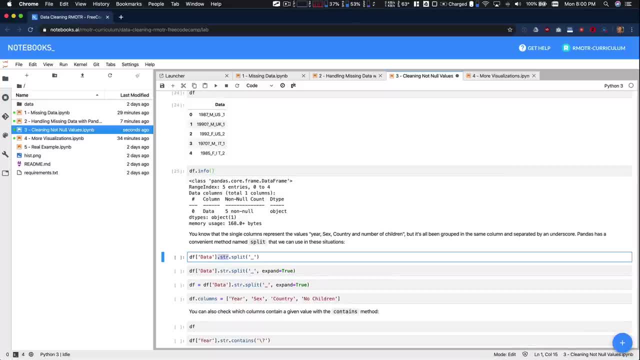 we're not going to call it a string. So we're going to call it a string And we're going to call it a cover. But you need to know: all the daytime columns have a dot DT, math attribute. all the categorical columns don't have a dot c at cat attributes And those. 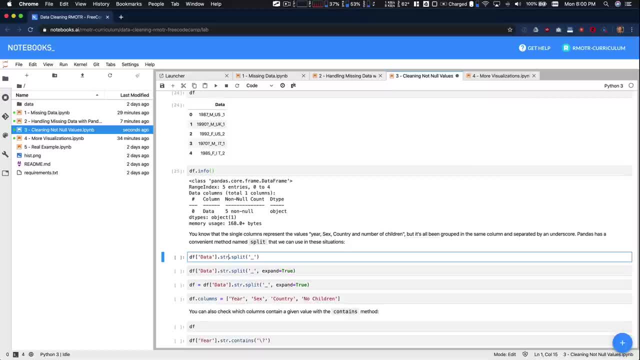 attributes: str, DT, cat. they have a special methods associated with the domain of that column. All the methods associated with string are, of course, for string handling, or the methods associated with DT are for daytime handling. So in this case, we're going to 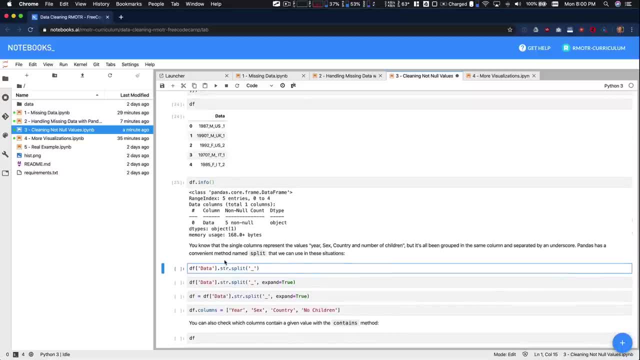 review. all- not all- have very good subset of the string methods we can apply And something interesting is that all these methods have a very good, have a lot of relevance and are related to the ones in pure Python. So if you have a pure Python string, there is 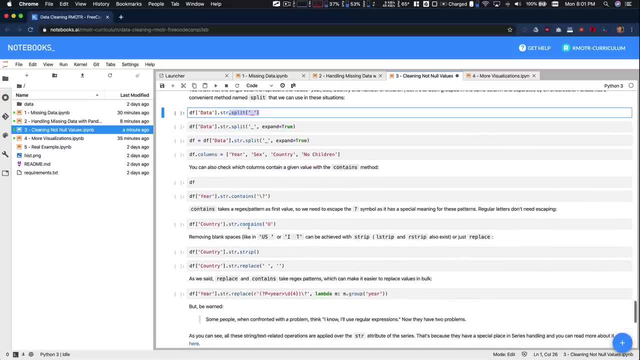 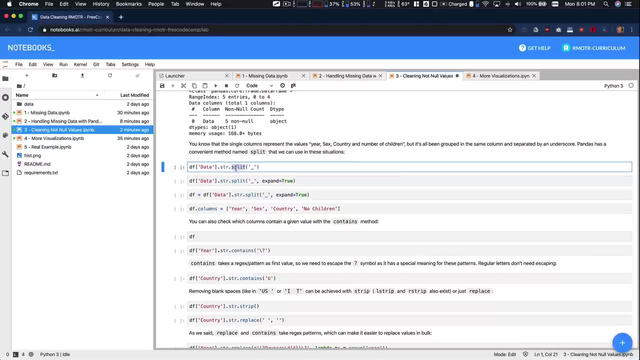 a split method. there is a contains method or I don't know if there is a contain actually. it's actually I think it's the in operator, but there is a strip and there is a replace right. So all the methods under the STR attribute in pandas have have an analogy in the standard. 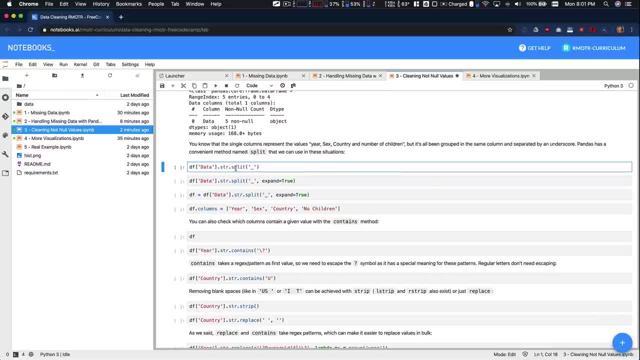 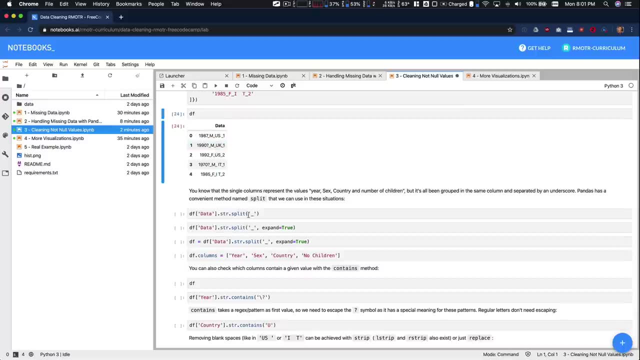 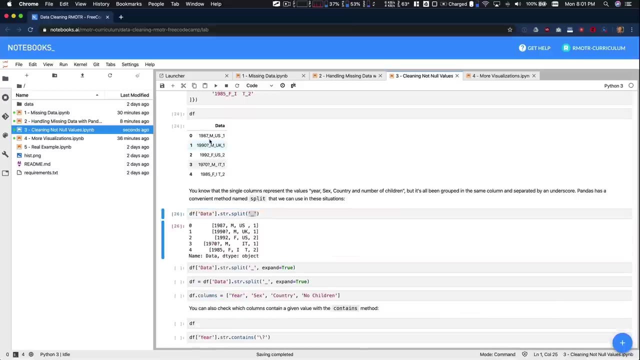 library of string handling with Python. So, starting at the beginning, this data we have. I'm going to delete this. this data we have. what we are going to do is split the values right by an underscore. So in this case, that's what we have. we have split all the values. 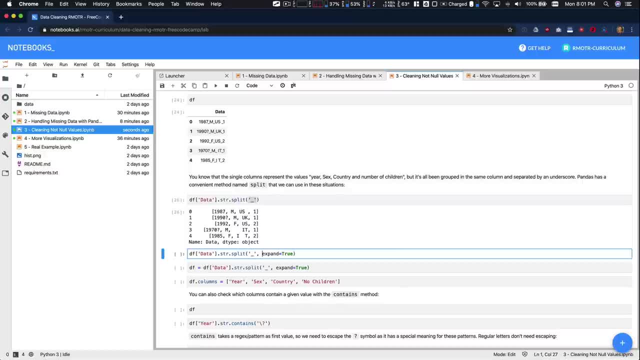 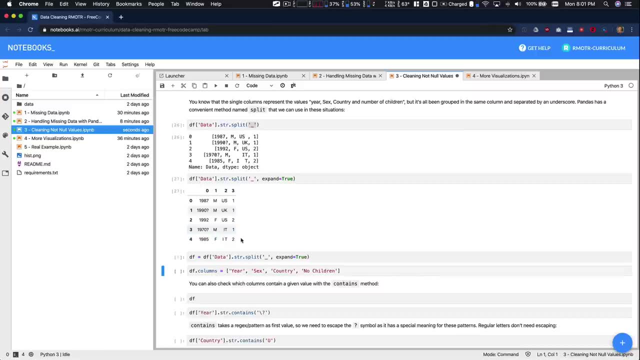 with that underscore And we're going to use the special attribute is expand. expand sorry equals true, And what it's going to do, it's going to create a data frame out of that. So we create a data frame with 70 columns, And this is what we have now, So we can keep applying methods. 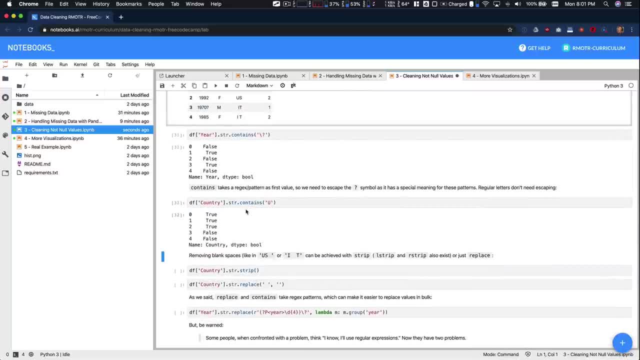 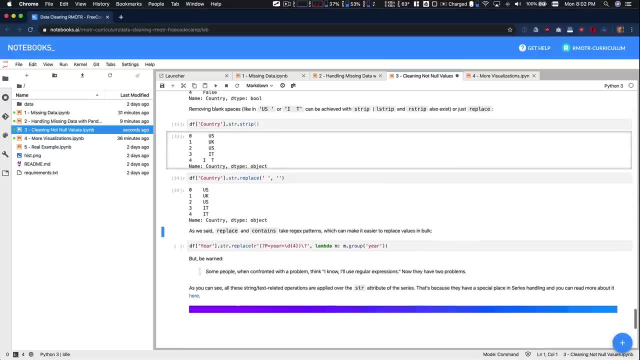 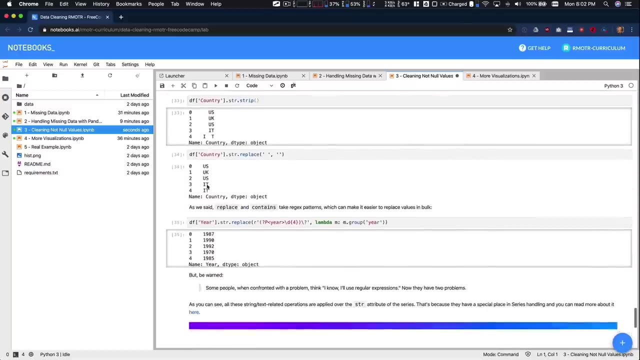 So, for example, contains or contain, contains regular or contains with regular expressions rights. for you to see the power of it: we can just trip, replace And we can do even regular expressions with replacing. So we could fix Something like this question mark in a string. we could fix it with regular expressions. 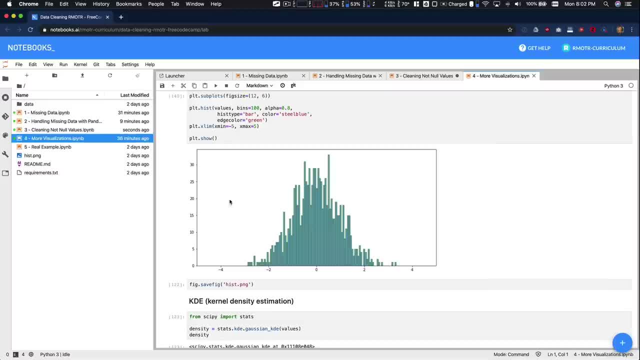 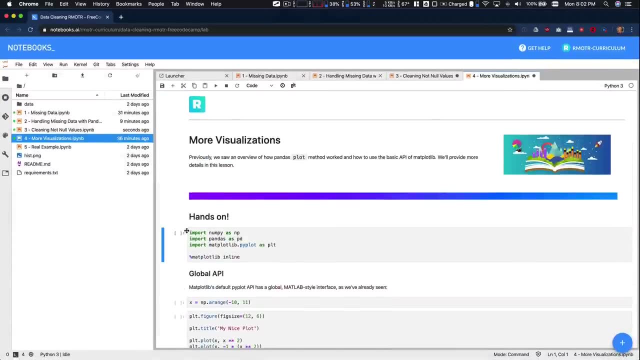 if you know how to handle them. And finally, something that is going to be very helpful when you're doing data cleaning is looking at the data from a visualization perspective. Data clean has a ton to do with statistical understanding of your data: to when a value. 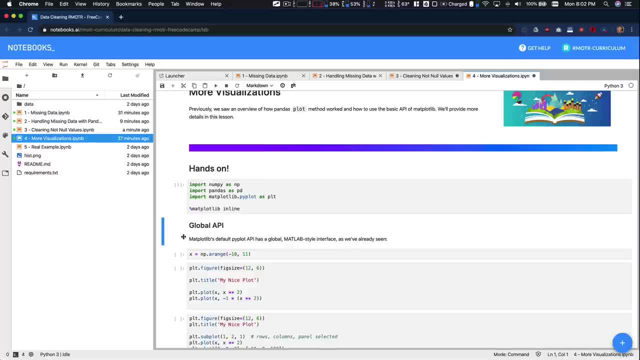 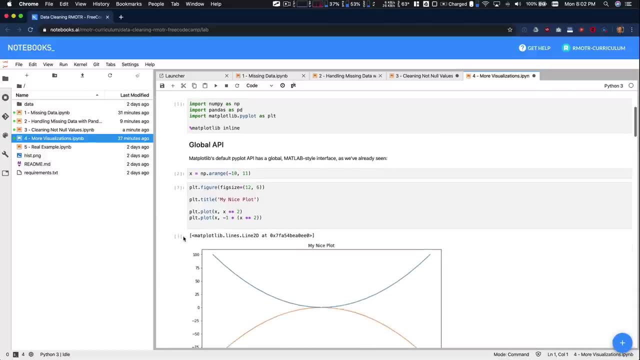 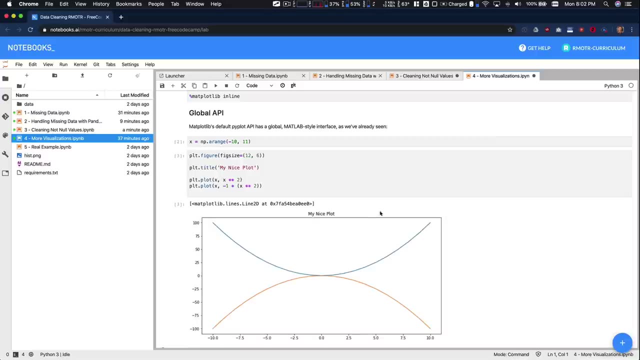 is considered an outlier, for example, it might be invalid and you want to clean it, So. but that's a lot more about statistics. In this case, I want to show you very quickly the matplotlib library that I've been promising for some some time now, the matplotlib library that so far we've accessed it directly from. 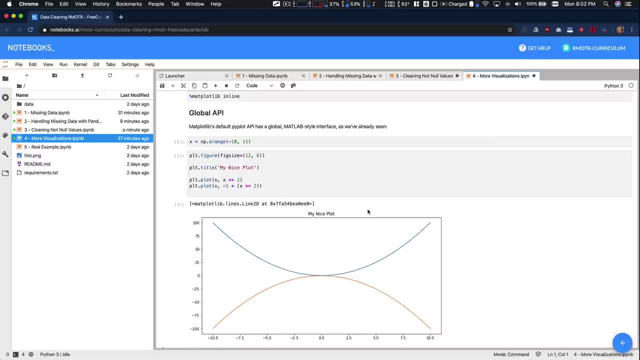 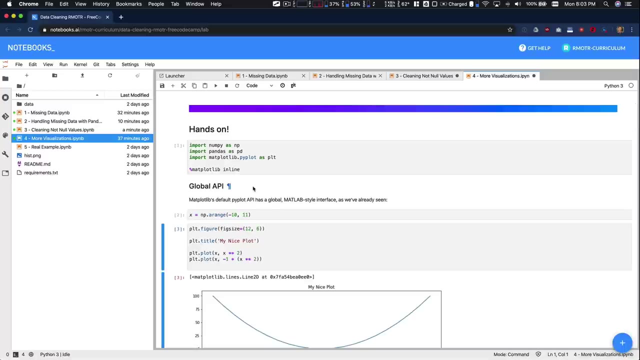 pandas from pandas. right, we were doing a data frame dot plot. It's these library. matplotlib is the one backing all those methods And we're going to see how to use it directly now. The matplotlib library has two important API's. we're going to call them. One is the 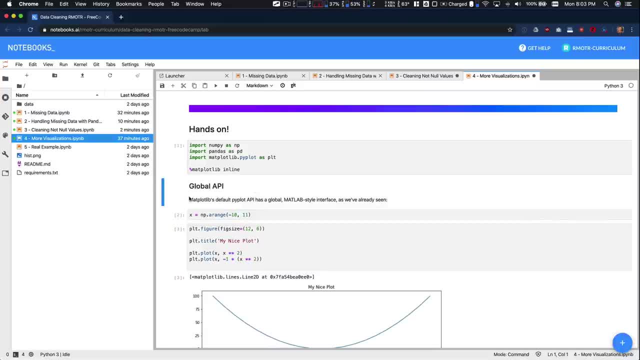 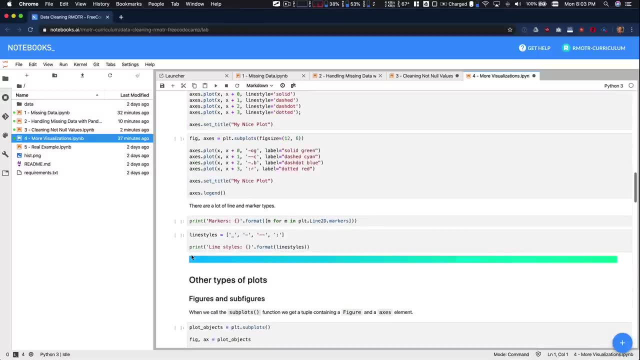 one that I don't prefer, which is the global API, But it's the most common one. it's the one you're going to find around- the global API- And the second one is the object oriented API. So it's around here And usually there are. there are ways. it's just two different. 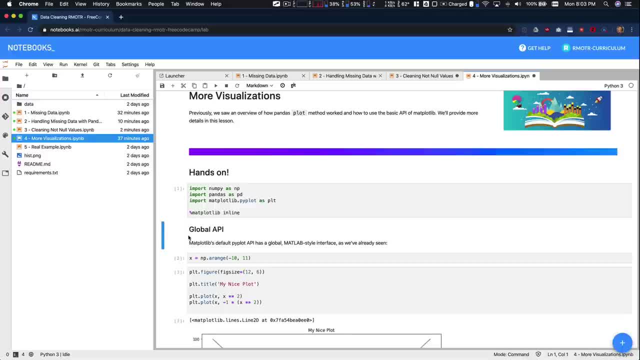 ways of doing the same thing. Okay, the global API is an API that it's, in part, inspired in MATLAB. It's been around for a long time And, sadly, most of the answers you find in stack overflow- tutorials, books- will be using these global API. the way, the way, the one I prefer, the 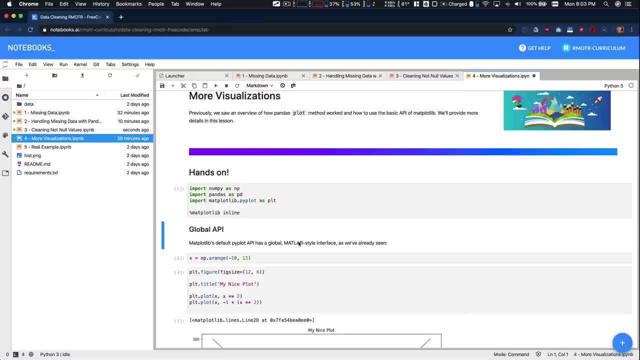 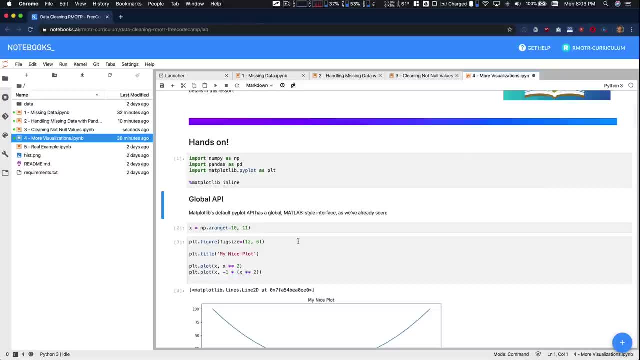 most, and I'm gonna explain why in a second. it's going to be the object oriented API, but I want to show you both, So you have a reference. If you follow me in this feeling of preferring the object oriented API, you will always have to translate global to OOP. 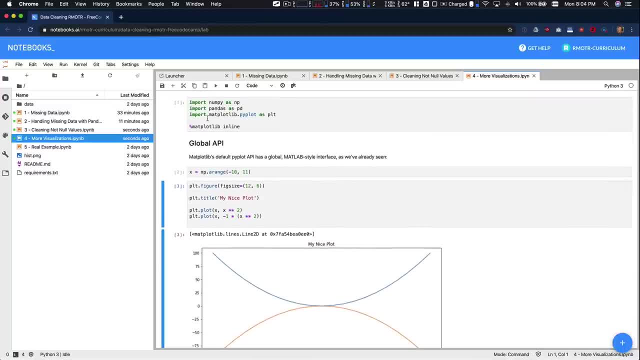 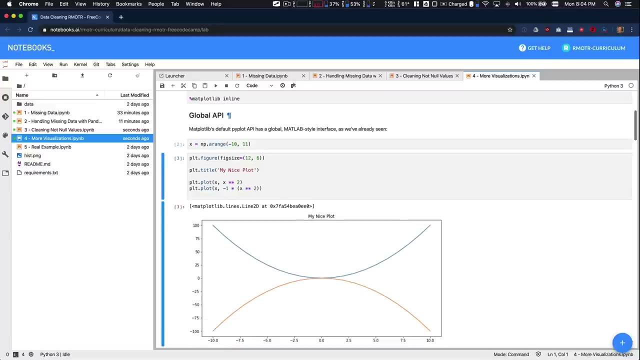 Why is it considered a global API? Well, we have imported matplotlibpyplot as PLT, So we haven't imported the whole module module, the whole Python module. depending how much you know about Python, programming is going to make sense or not. we have imported the whole module, And now what we're doing? 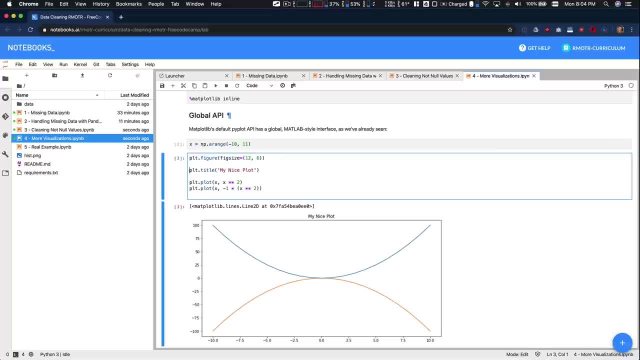 is, we're invoking PLT, that figure and final, and then we're going to do a title And then, finally, we're plotting two things: we're plotting x, our plotting x squared and minus x squared. And why is this global? because we're invoking functions, are at at module level And the 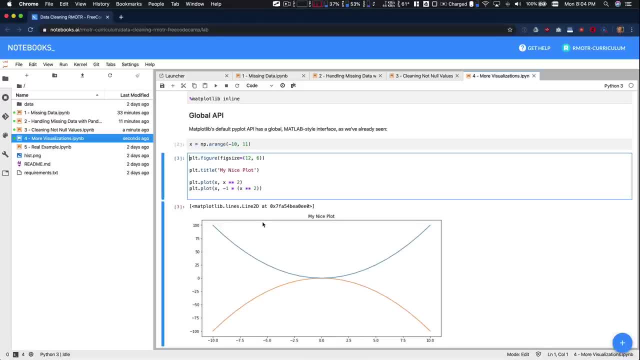 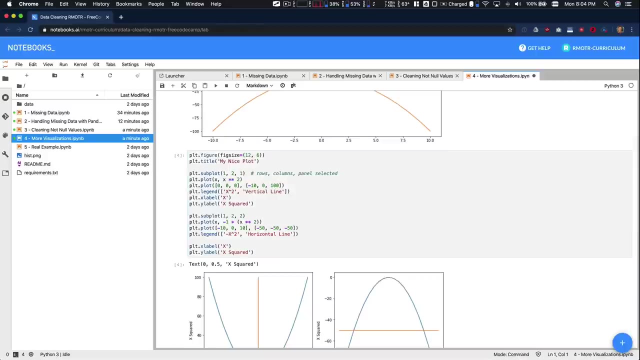 reason: object: the final plot that is being modified by these very generalistic and global calls right. So by by doing this call right here, I'm modifying the final result of the plot. Let me show you a more complicated example So you see the problems with the global API. 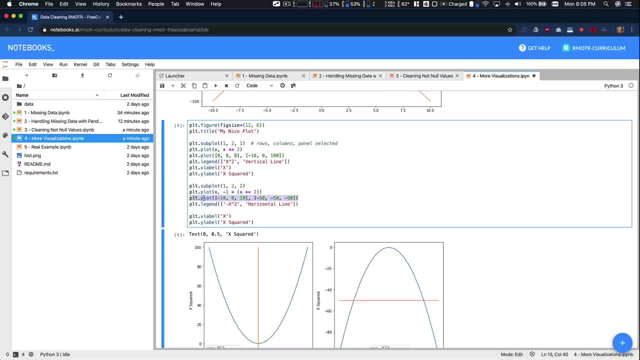 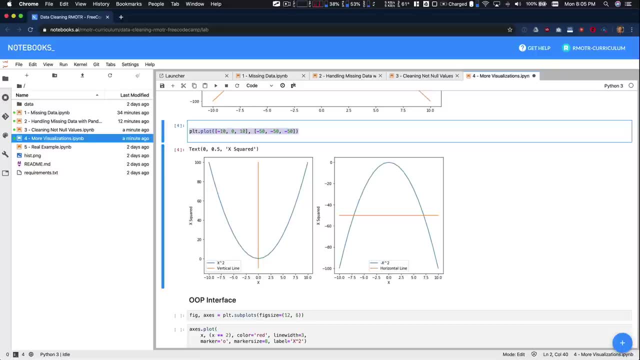 If you look at this line, if you could delete everything, let's actually delete everything. What is this line doing? Which plot is affecting? You do not know. There is no object oriented way of saying in this second plot, the plot on the right, or the figure on the right, or 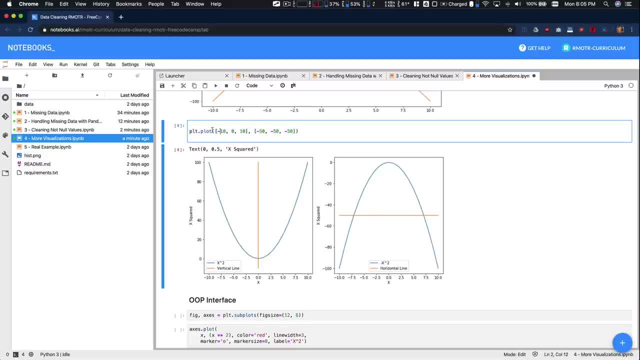 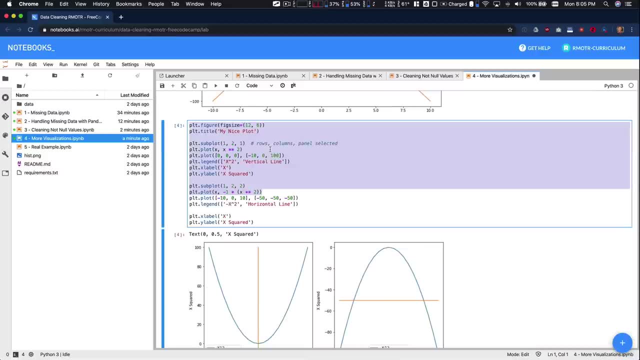 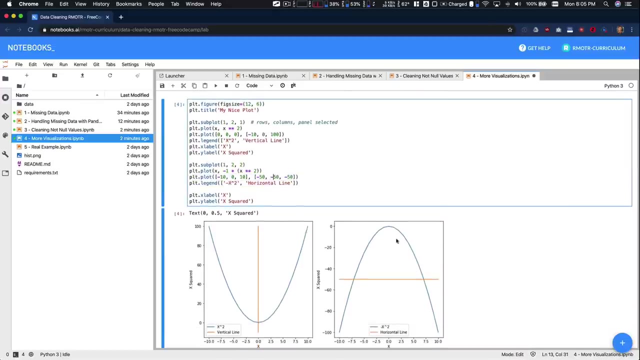 actually the subplot on the right. I want you to plot this thing. You're just saying it to the entire module And, depending the order that you said, it is where it's going to To land that particular figure, where it's going to land, in which plot it's going to. 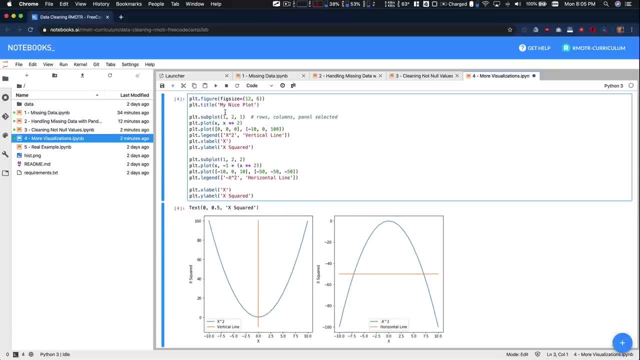 land. Again, it's a global API. So we start saying: I'm going to create a figure, trust me from. so, from now on, I'm going to start drawing on it. there's going to be the title And hey, by the way, it's going to have one row, it's going to have two columns And I'm 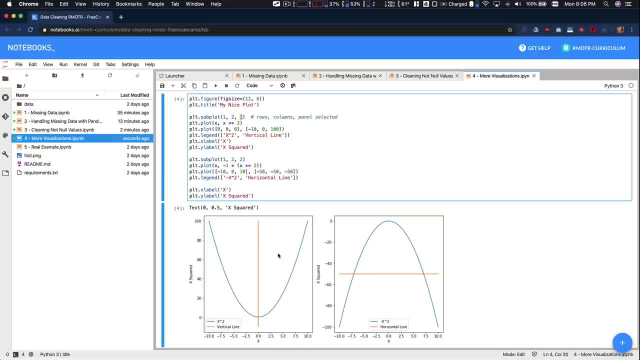 gonna start drawing in the first plot. these were right here. these were right here on the left, So now I have kind of activated. if you want that plot, it's active. So now I'm going to start drawing on it. So every action that happens after this line is going to be affecting. 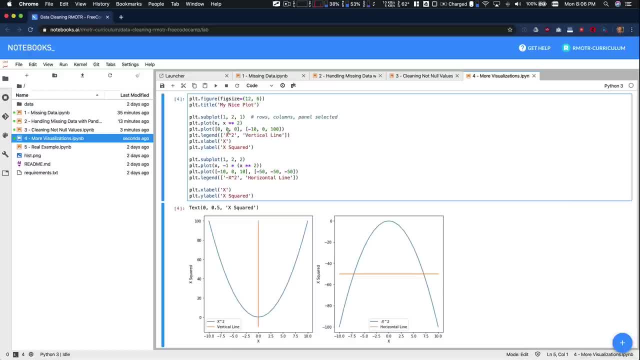 this plot, this plot right. So then I plot x and x square, I plot this vertical line, I put a legend, I set labels, etc. And at some point I just stop and say: Hey, now I want to switch the plot. I want to now start plotting. sorry, I want to start plotting. 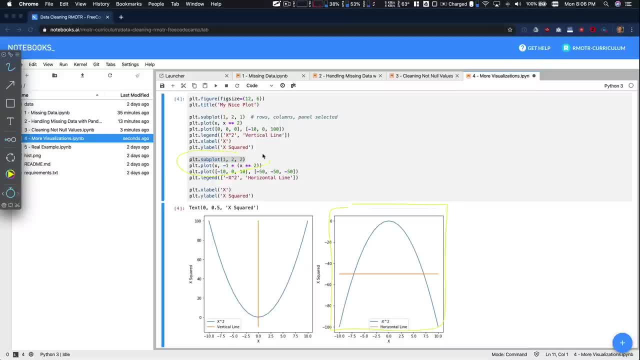 here in this second one, because I have just changed dots. the first line, this one. Oh sorry, the way it works is by saying the first row, second column, but second plot. So now I want to start plotting in here. every successive line will affect that plot And 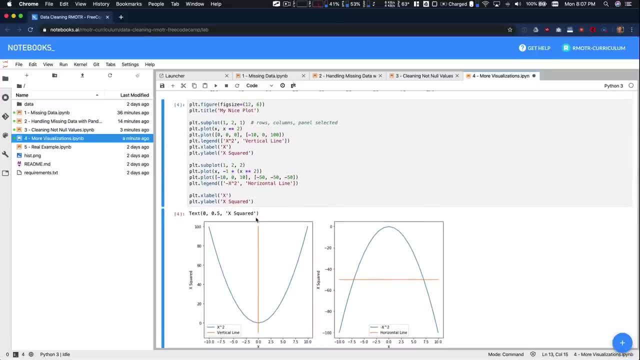 again, you can see that understanding a code given the order, the, the order you're going order in the sequence of lines, is very hard. If you have to debug a report that has a plot that takes 100 lines, then you have to keep in your brain what's happening top down. 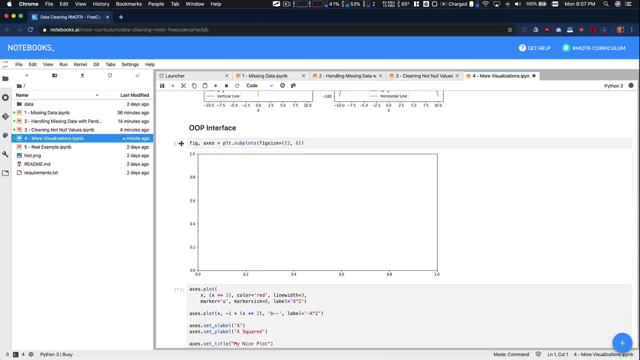 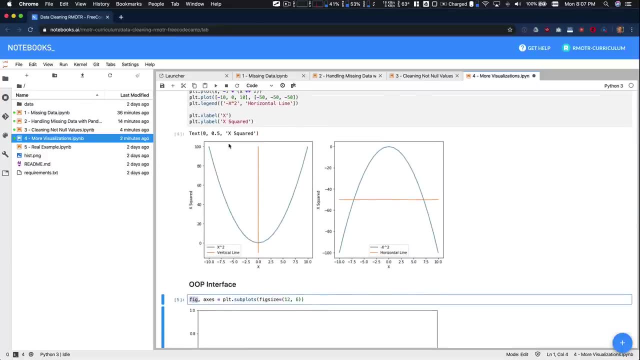 A different approach is going to be the object oriented approach, in which we're creating a figure and we're creating access. So in this case we have, in this case we have right here one entire figure in red and we have in here Purple. we have two axes. 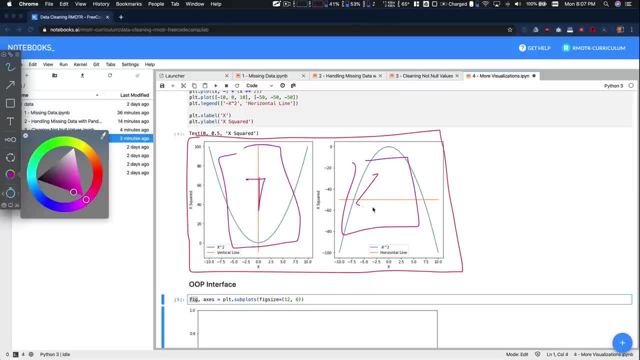 So this is axis one And this is axis two. So we have two axes. we are going to create those using an object oriented approach and we're going to keep references to them. So we've done the same thing. So we've done the same thing, And then we're going to go and 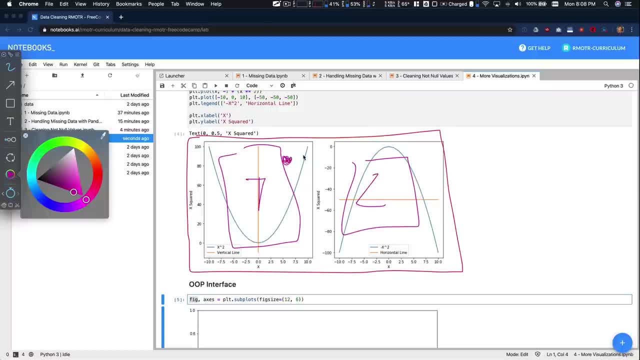 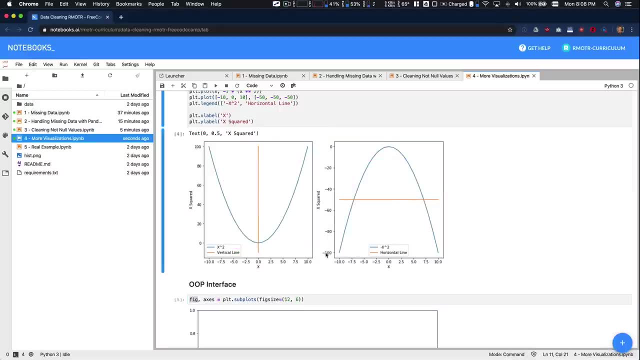 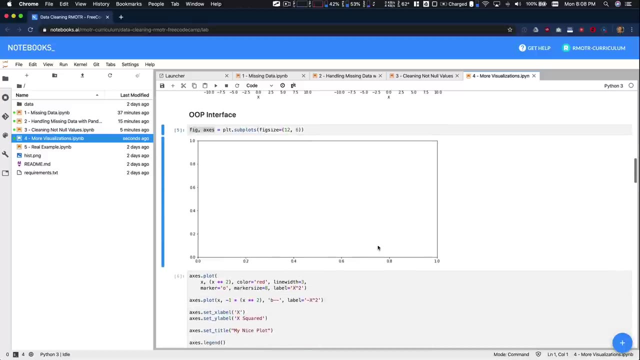 So we're going to say later to these plot, to these axes: sorry, I want to plot something And that will be very explicit. it's going to be an object oriented way. So the first thing is creating the figure on these, the axis. In this case we have just one axis. 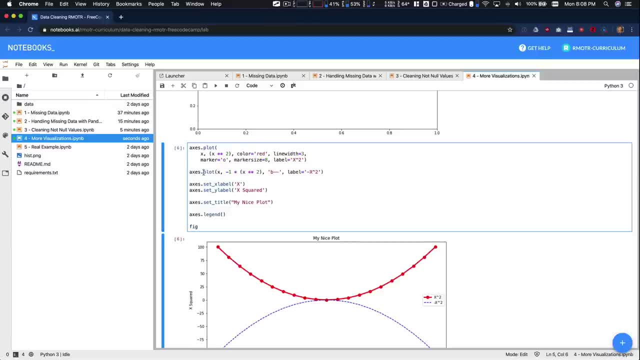 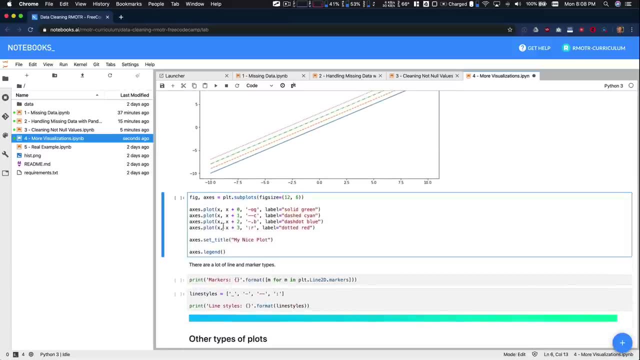 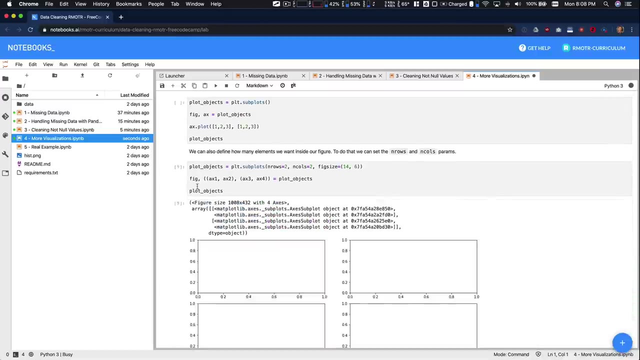 that's it. But you can have more. and then you say: in this axis, I want to plot this thing, in this axis I want to plot that thing, etc. When you have multiple axes, a site could show you. I'm going to go back again to that in a second. But in these case in which we 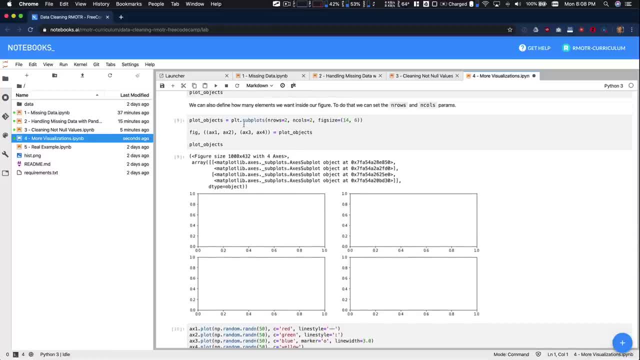 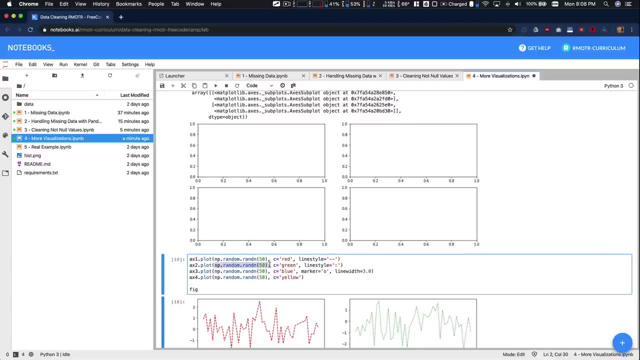 have four axes right. so we create one figure and it has four axes. we do it with the subplot method, saying n rows and columns. Now we say to the axis number one: I want to put this thing to access number two, I want to put that thing right, so it's 1234.. And now we 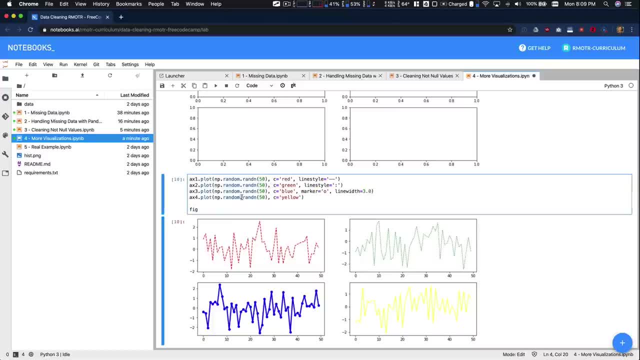 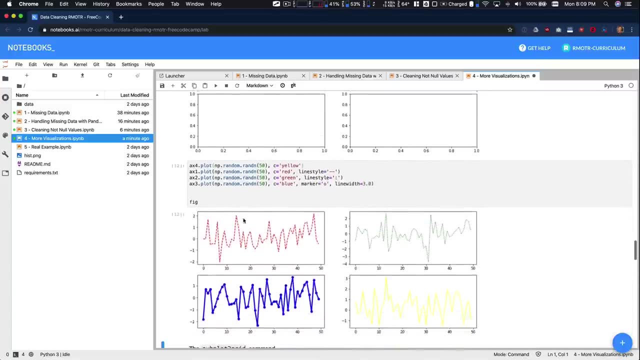 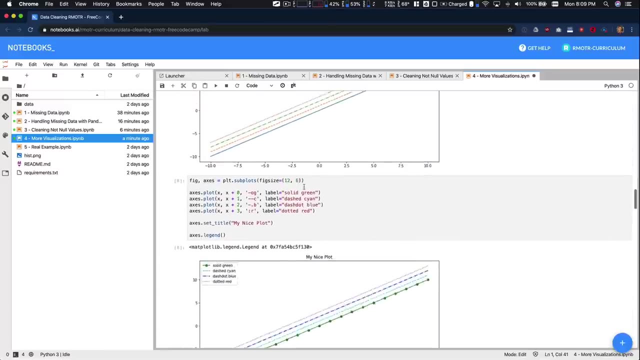 Now it's a lot more explicit. it's not depending on the order- I could change this order, that doesn't matter There- that the results are going to be the same. Access number four has yellow, regardless of the position that we're following. So the map will live. And now that 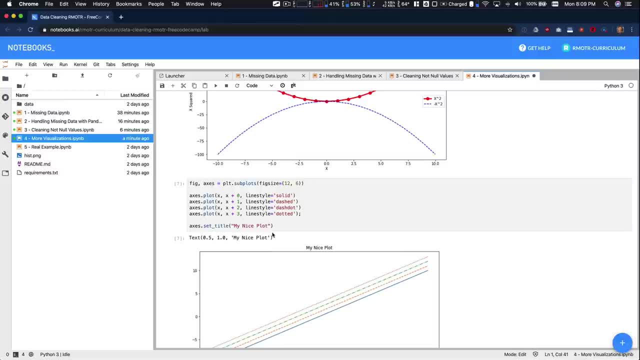 we have clear out the differences in both API's. My belief has these very simple plot function or method, depending optical inter global that will plot something that you specify. In this case, we're passing all the values in x and all the values in y And in. 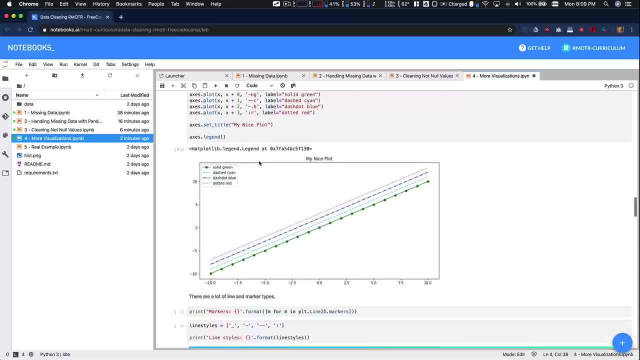 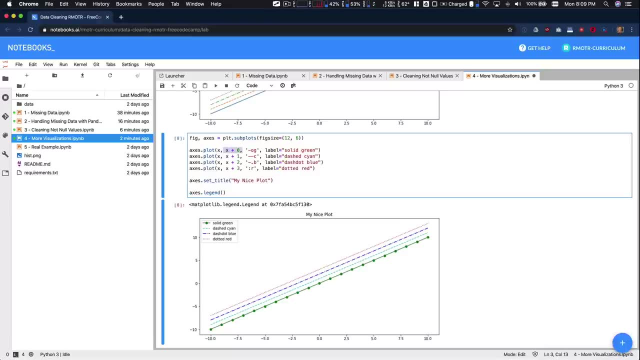 this case we're passing a given line style. this can change. with these type of syntax, you're saying: I'm plotting this thing in x, I'm pulling this thing in in y, second parameter in y, And I want you to use a straight line. it's straight line, Yes, With this, this is. 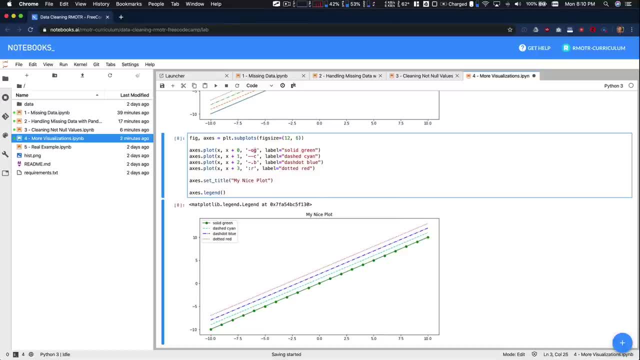 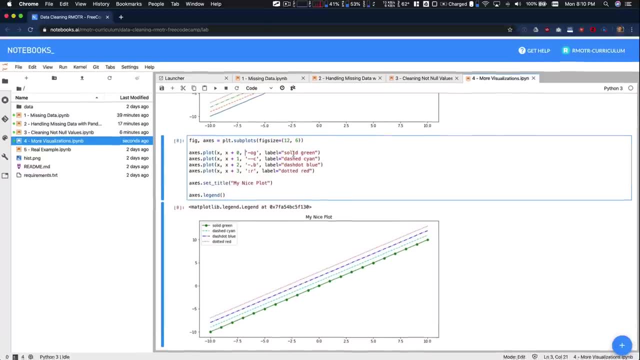 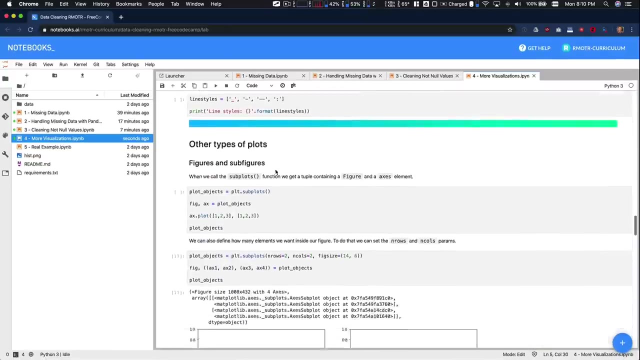 this marker, the dot and in green. So this is if you are very familiar with it. if you're very familiar with my poll live, you can use the syntax. In other case, you can just say: line style: market marker: sorry color, specific keyword arguments for each one of those. So 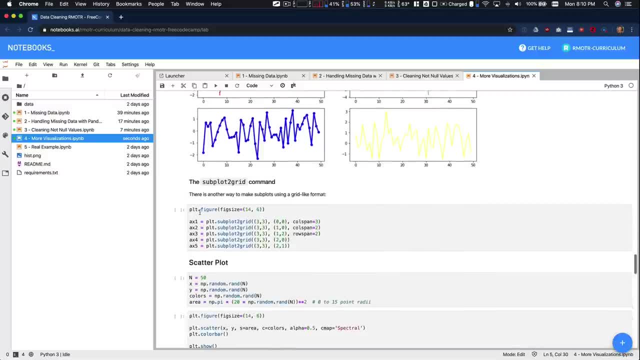 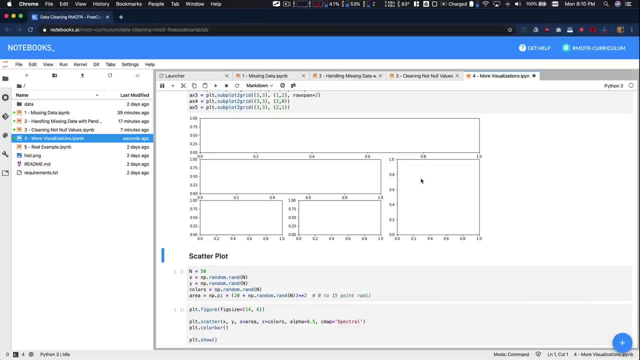 do we only have line plots in Apple live? No, of course not. We have a huge variety of plots And, by the way, there is another one here. if you want to see more than plugins, our grids. you can create these grids and put different things in it. And again, 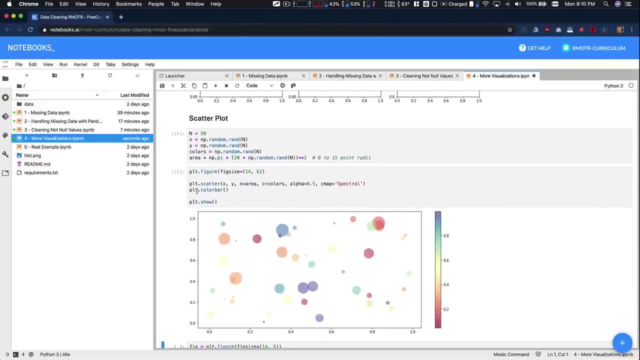 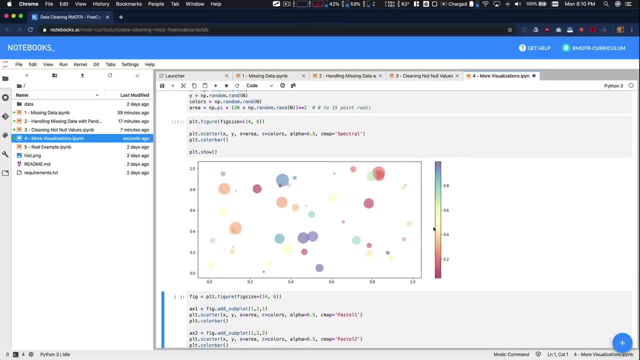 not only line plots. One good example is a nice scatterplot. So basically we're plotting x and y correlation And there is also a value, a color map, right? So given the value, there is going to be a change in color. So this kind of lets you plot three to four dimensions. 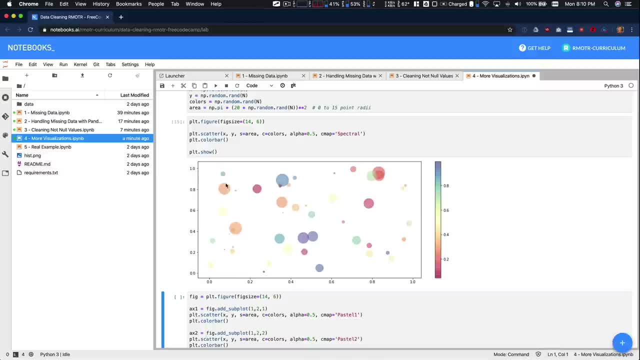 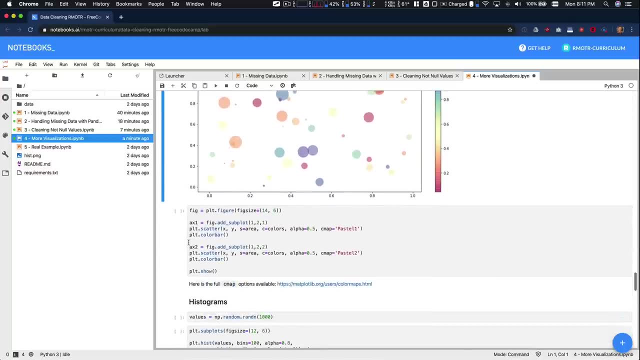 of your data: the volume x, the volume y, the size of the bubble and the color of the bubble. So we're- you're pretty much encoding four dimensions in just one figure, right? So in this case, we're just using two different scatter plots. 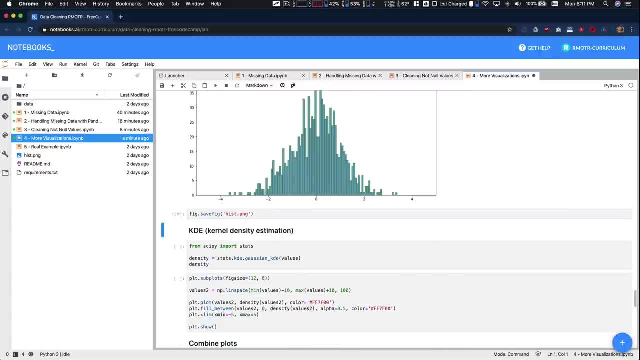 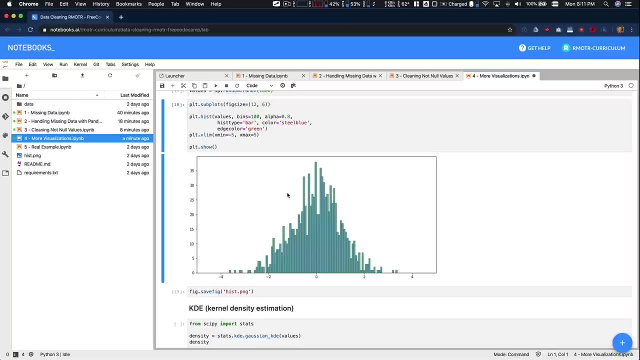 there's more information here. we can also plot histograms. We've very quickly seen that with pandas. with pandas is is very simple, was just plot type histogram, kind histogram, hist. actually you can look it up in our previous lessons. So just go back into the 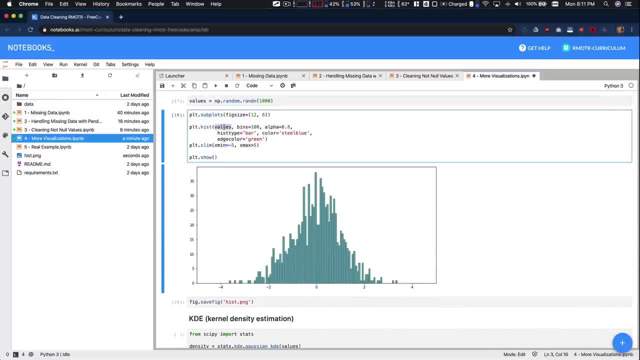 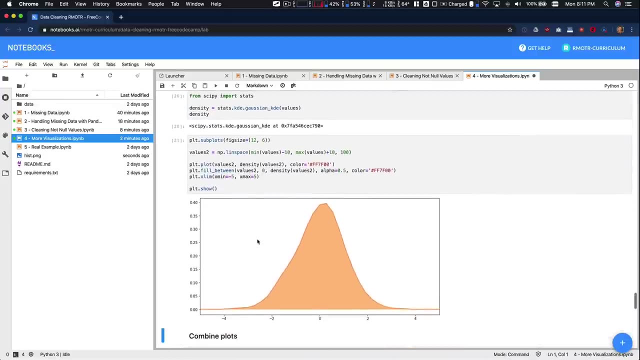 index in the video And the histogram is extremely simple: just text, the values you're plotting and how many bins you want. There are some more advanced arguments here, like the alpha level etc. But it's simple And similar to the histogram. you can also create kernel density estimator. 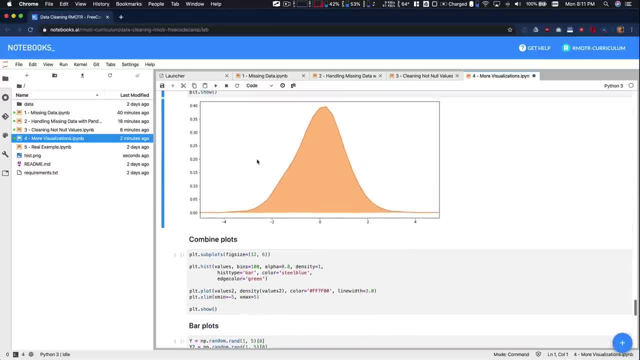 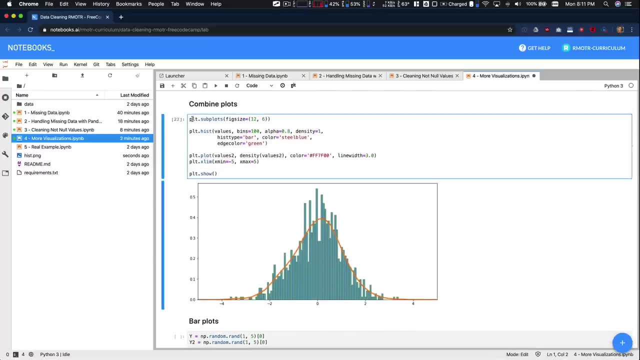 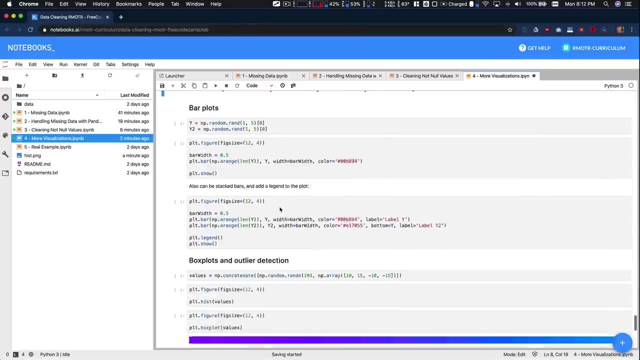 diagrams, which is very similar to our distance to simulate. if you want to continue distribution, You can combine these plots if you want. In this case, we are creating the plots, we're plotting a histogram And then we're plotting the lines And then we're plotting our changing the limits. But 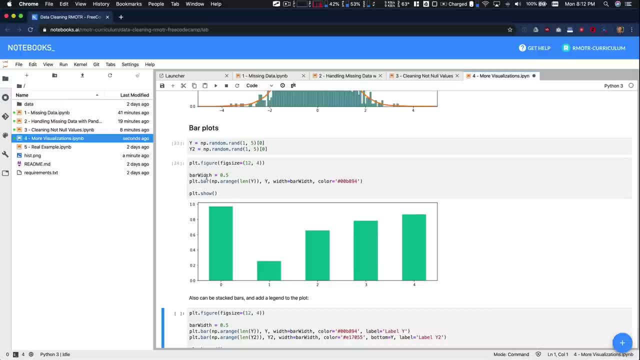 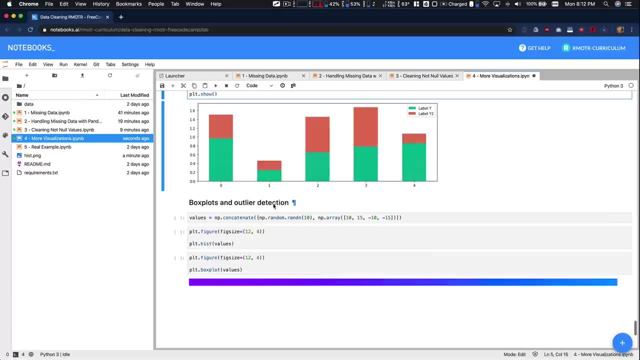 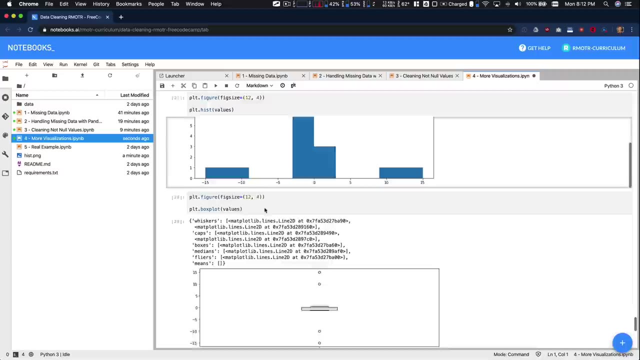 that's pretty much it. And you can also create bar plots, right? So in this case we have PLT dot bar, or here we have two bars are stacked right. That's the different way to look at it. And finally, checking out layers, you can always plot histograms or box plots. 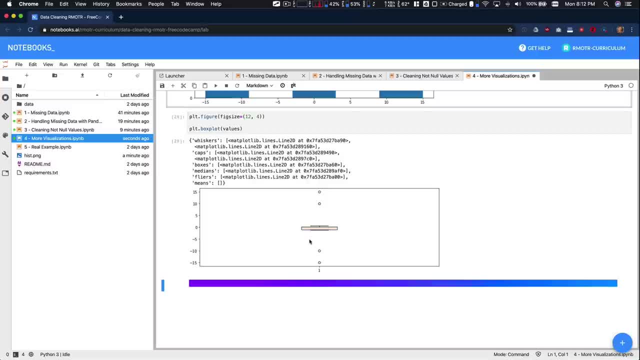 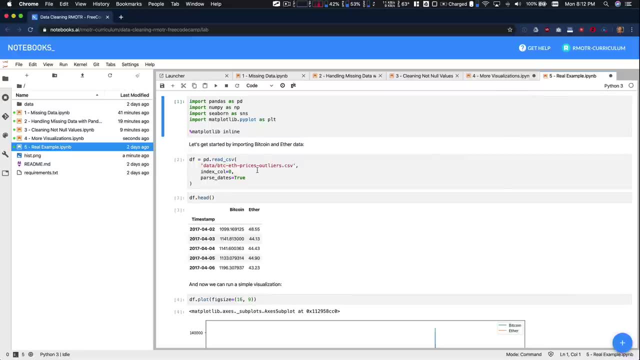 right. So box plots are also a nice feature to have in here. So this was all with data cleaning. We're going to keep moving forward this tutorial. I want to mention one more thing here And it's there are notes here for kind of a task. 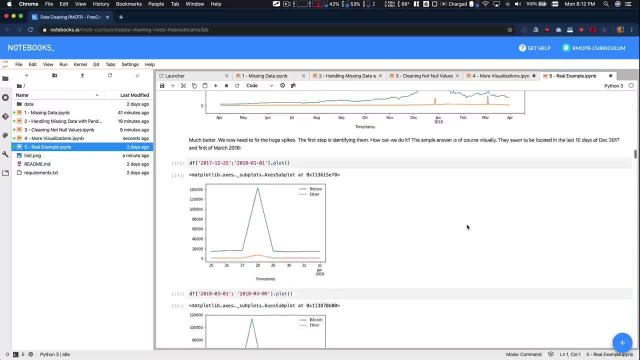 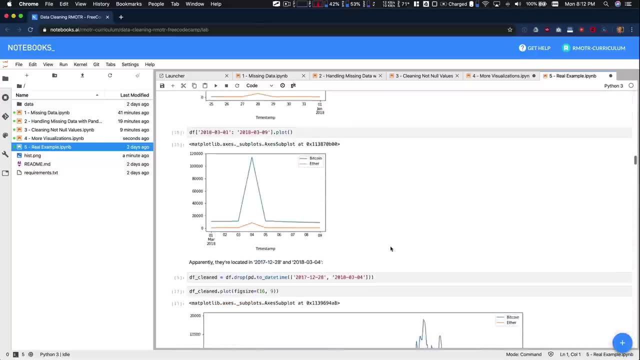 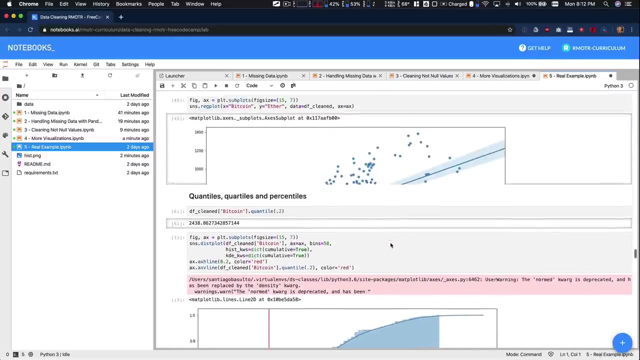 that you can follow with data cleaning, which we're we are identifying. We're identifying missing values in given positions with is no less than a and right. here we're looking into more detail about some statistical properties of the data in case we needed to clean up. 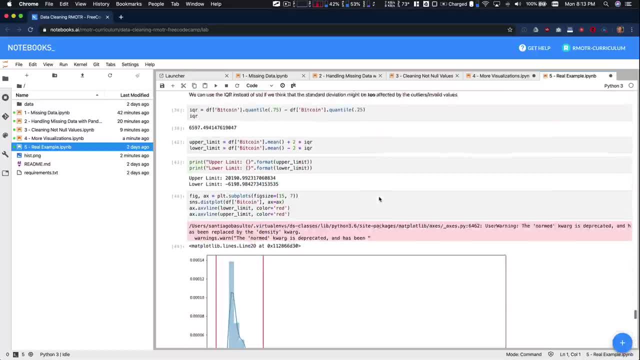 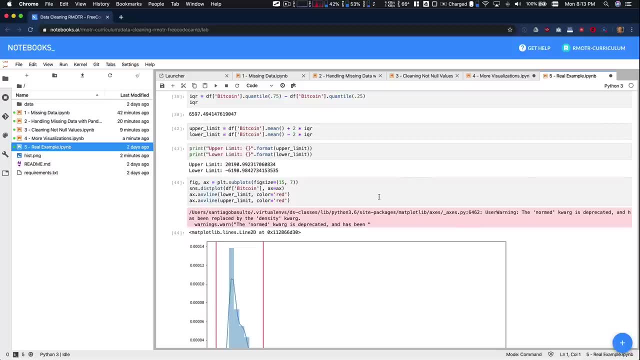 it. Okay. so this is a little bit more advanced And it's it's related to the concept of cleaning data, given the domain. So the statistical analysis can tell you that this value is an outlier for this distribution. the value might be valid. So, for example, a human being is: 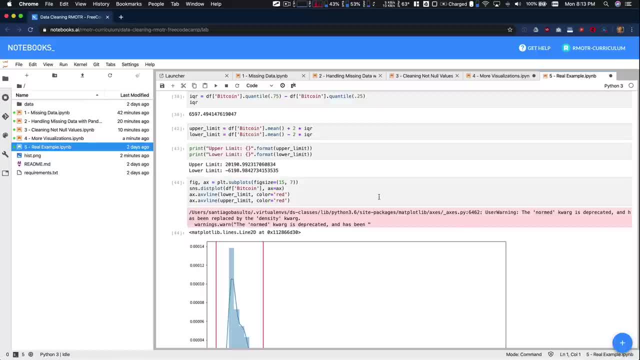 90 years old. that's, that's valid. that's a valid age. But if you're analyzing data about high school students and a human, that it's 90 years old, it's going to be completely invalid or it's going to be an outlier in that distribution And you can treat it as. 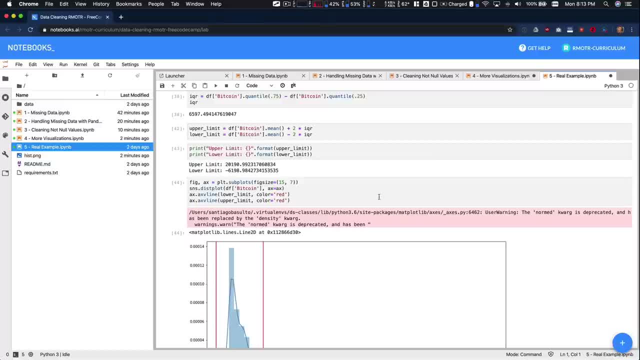 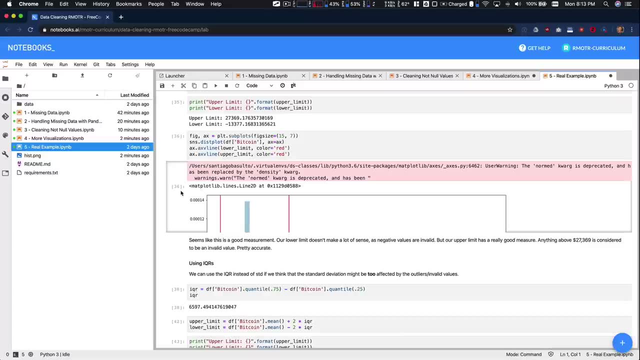 an invalid valid and clean it out, remove it, for example. So that's, that's still a little bit more, with the whole statistical analysis that you can follow here. it's a little bit more advanced for this, So let's move forward with the rest of the videos. 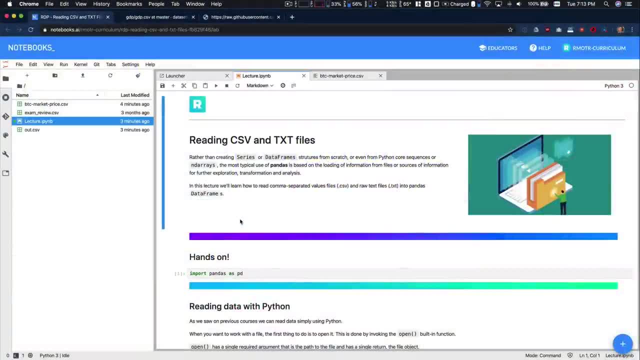 And now it's time to get into more advanced features of pandas to import external data. So we've seen already in a real life example the way we can import data from CSV files and from SQL databases. right, we had actually those two lessons, the objective of these. 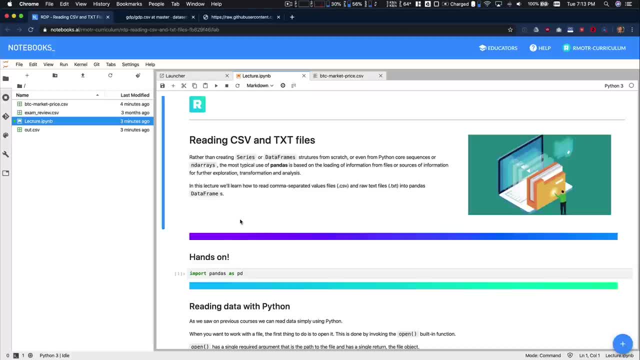 part of the tutorial is to show you how you can improve or get into more advanced use cases of importing data. So we're going to start, for example, with CSV and text files. And again, you've seen there already, but here we're gonna give it a, an extra twist, So I'm going to show you. 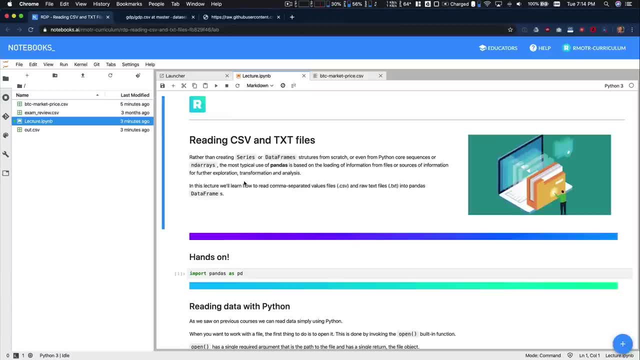 more advanced features And for special use cases. TXT files. CSV files is conceptual speaking. a CSV file is a text file. It's just human readable text right that it's encoding information. The idea of a CSV file is that it's tabular right, So it's a plain text. 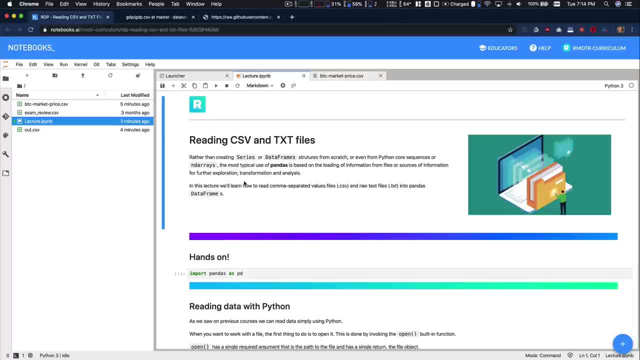 file, tabular data in it and it's separated. CSV stands for comma separated, But it can be the separator. can be anything. we can see more examples later. But basically the idea is that it's text file, that it's tabular in a tabular format. So those both CSV files and 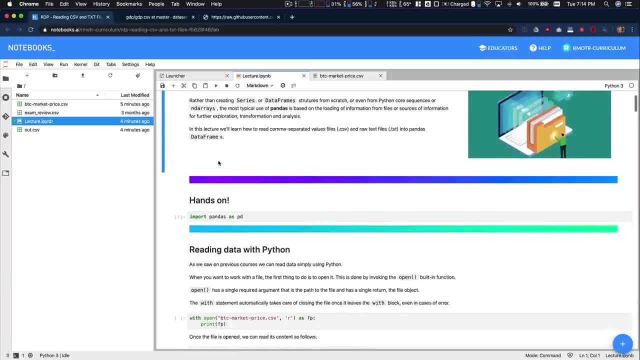 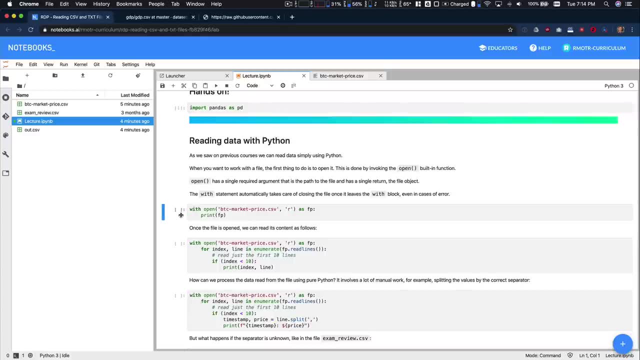 text files will be read with the same method. So, to get things started, I want to show you the basic way we import, we read data from from from external sources, using Python, without even starting yet with pandas. So you don't need to know this. it's usually. it's usually. 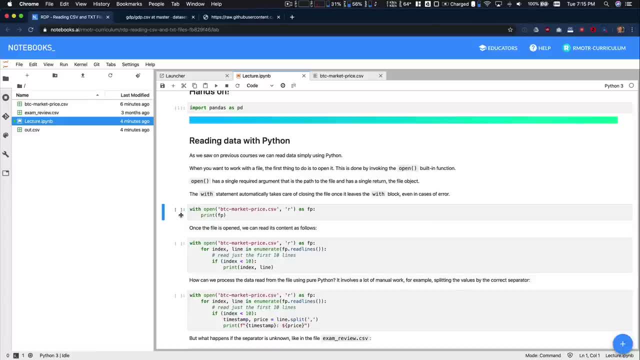 productive, if you want for data scientists or data analysts to understand a little bit more how file reading and writing works in computers, because there are multiple, multiple concepts aligned here. they involved operating systems, processes, your language. right, it's not the same thing to read a file with our or with Python or with another language. 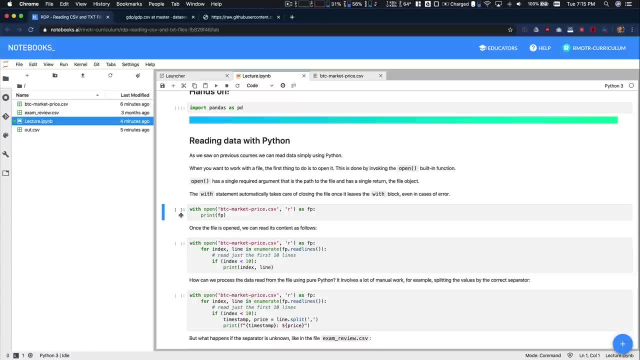 So there are multiple concepts here And even though pandas, in this case, can make it seem very simple to read and write data, you can get a little bit of a more advanced use case if you know the internals of, again, both the operating system processes on your language. So this is the way we read data. 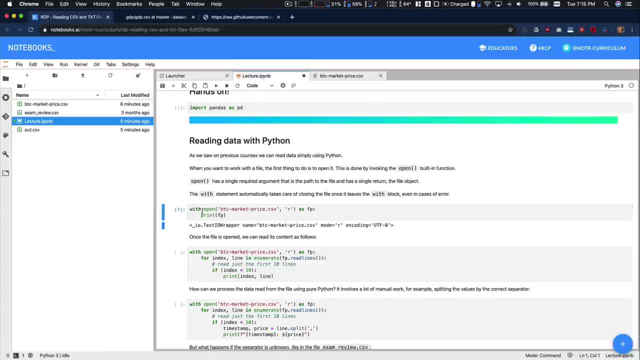 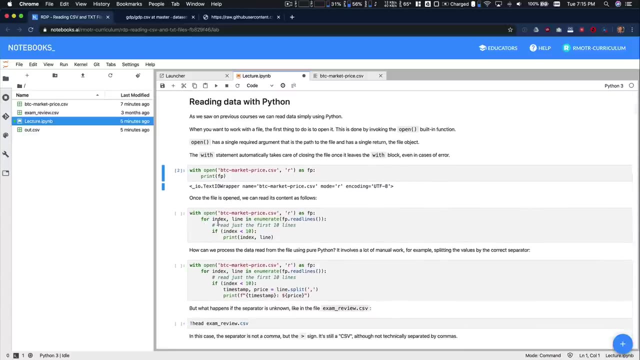 with a reader file. Sorry, using pure Python we use the function open And in this case we're using a context manager, just a security feature, again related to to the advanced use to of reading and writing files. But it creates a file pointer right And with the file pointer. 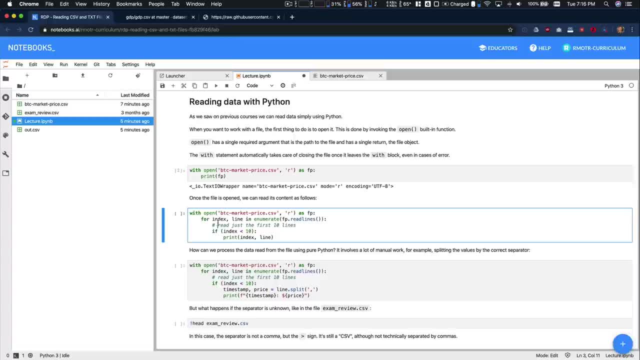 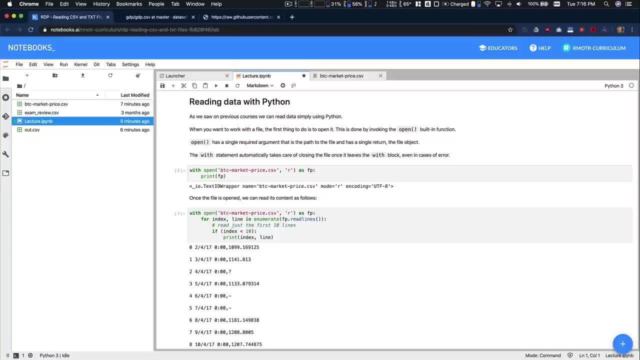 you can then use the very simple API point post but that but that pointer, which is something like read line, read lines, read a number of bytes or characters. or you can just even treat FP as an iterator. just do for line in FP, But basically we're going. 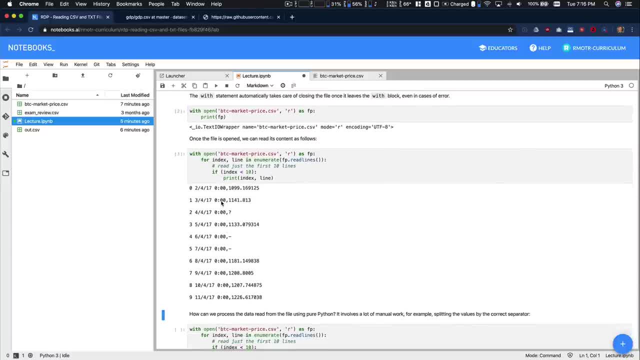 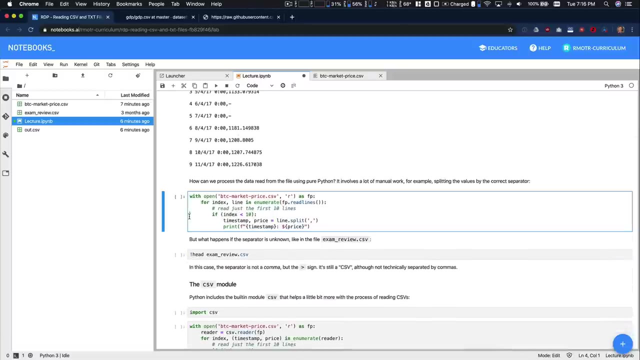 to do something like these. we'll start reading data From top to bottom just until I don't know we hit a given end. In this case, we're doing it just for I don't know a couple of lines What else we can. it gets very difficult when you're reading. 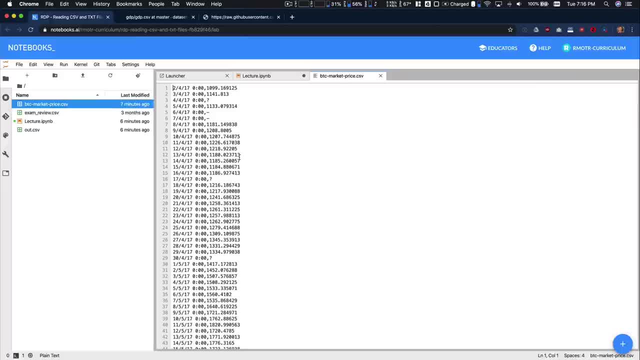 text files, to process them, because it's usually hard to parse the structure of the file. So it's not the same thing to have a file that is separated by comma, separated by columns, separated by pipes, spaces, etc. So you're going to see that once you want to get a file. 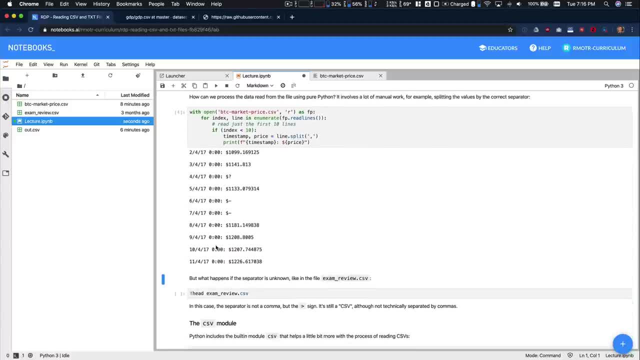 it's a little bit more, I don't know- a little bit more with an advanced usage right or a little bit more. fancy your calculations and and the way you parse the data, it's going to be going to get harder. So that's why we're going to use pandas Or I'm going to show. 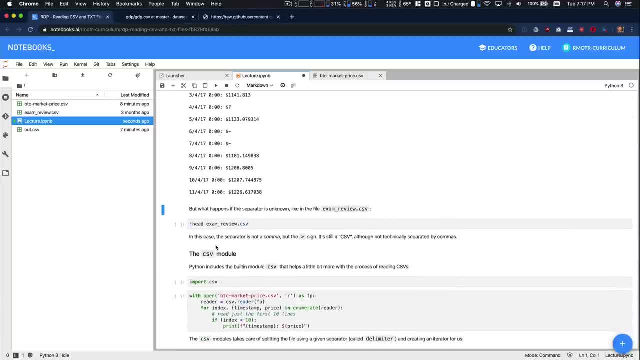 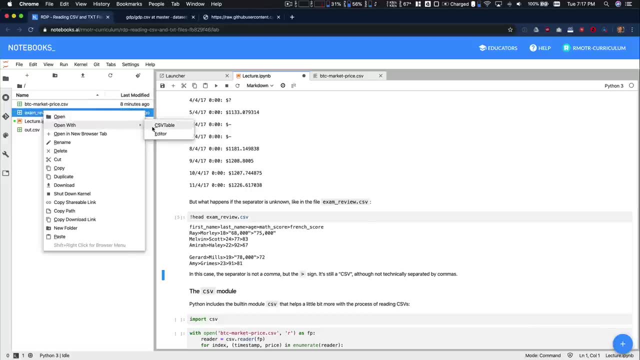 you in a second. this is the module that is part of Python, So this is the file that we're going to be reading. it's the XM review file and I'm going to open it And even though it doesn't look like a CSV, it is indeed a CSV. The difference is that here, the separator 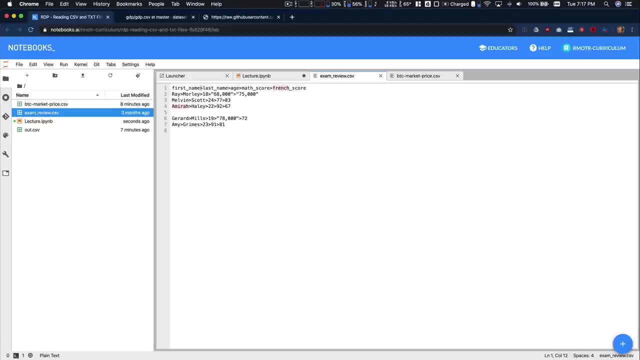 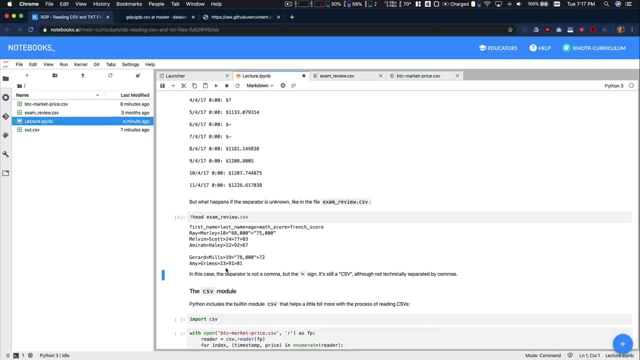 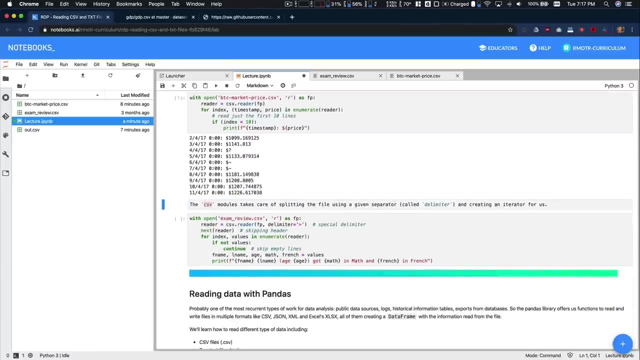 is the greater sign. it's not the comma, it's a greater sign. that's going to be what marks the delimitation between different fields in our CSV file. So we're going to use the CSV module And the way right here to parse the data using that module is by passing a. 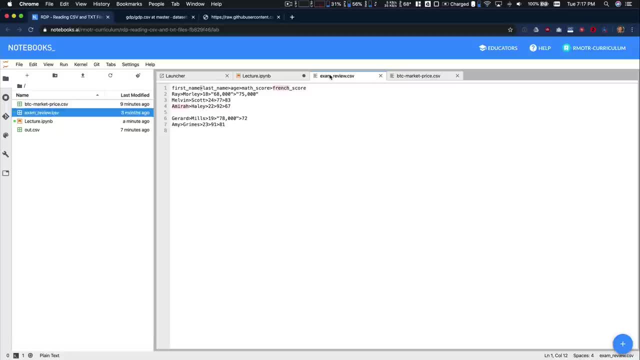 special data delimiter right. so that's going to be the type of work that you might need to do when you're parsing data. It's not the same thing to have a delimiter day: it's a greater sign. it's not the same thing to have numbers, for example, that are enclosed in quotes- all. 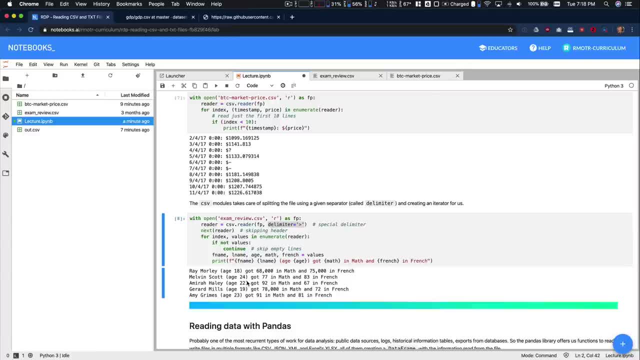 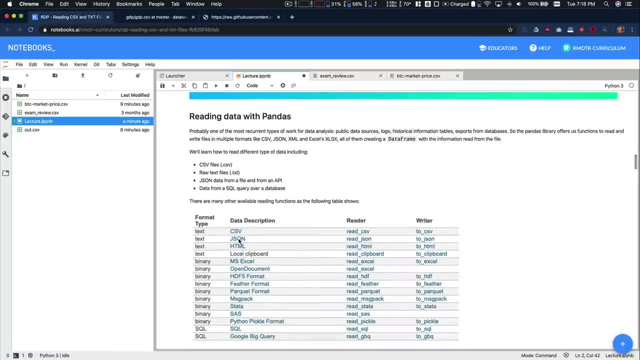 those things right will change the way you work. And all this is going to be abstracted away by the pandas module. So to get things started again with pandas, at least pandas has multiple read underscore something- methods that will work for different sources, right? So we saw already read SQL. 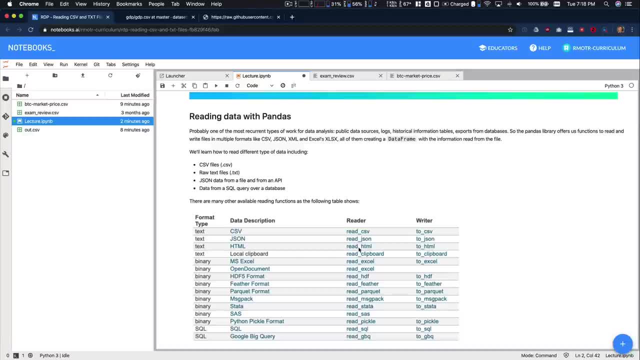 we've seen, read CSV. there's also a read HTML to directly parse information from a table. it's literally you can just you pass a website, it's going to read information from a table. or read JSON, read more advanced formats like Parkett or Stata, etc. And again, each. 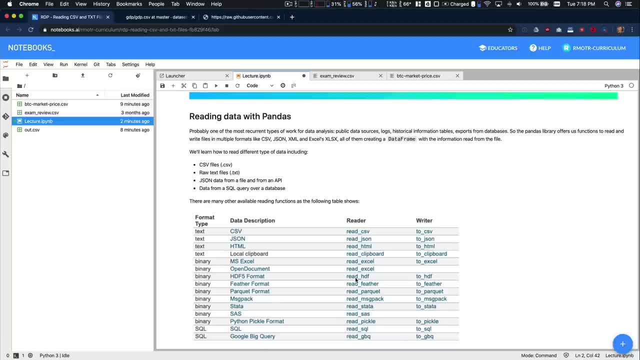 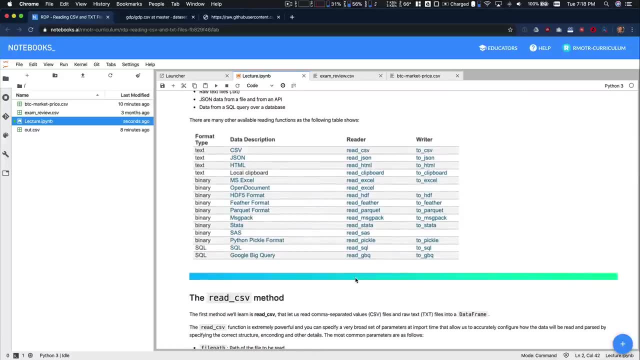 file format will usually have a correspondence In pandas it's. I've never had the chance to rewrite my own stuff. to be honest, the same thing is going to happen for something like Excel, which might need external modules. it's not directly provided by pandas, But by installing those modules you can easily 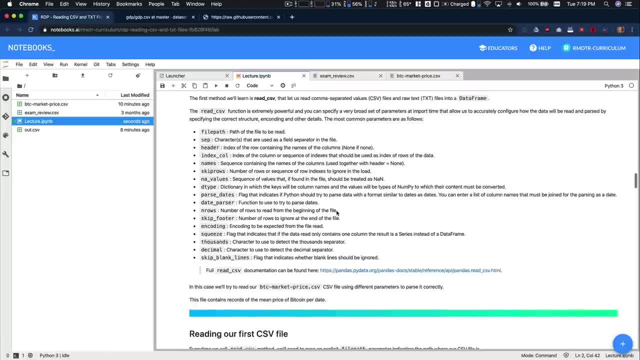 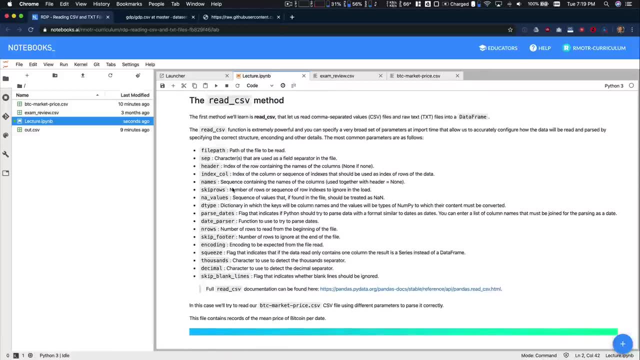 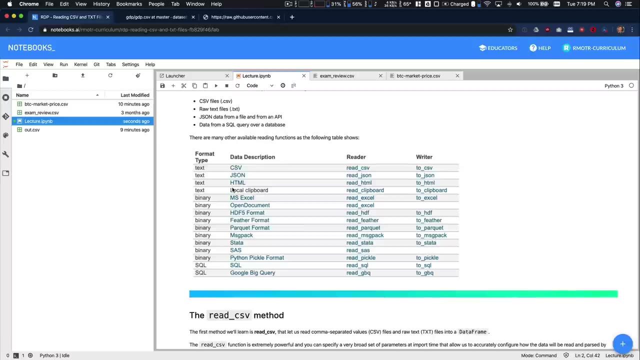 incorporate Excel files in your day to day work. So the read CSV method- sorry- has a ton of parameters. So this is the the main characteristic of all these read something methods, Given the amount of possibilities that you're going to have with these files. 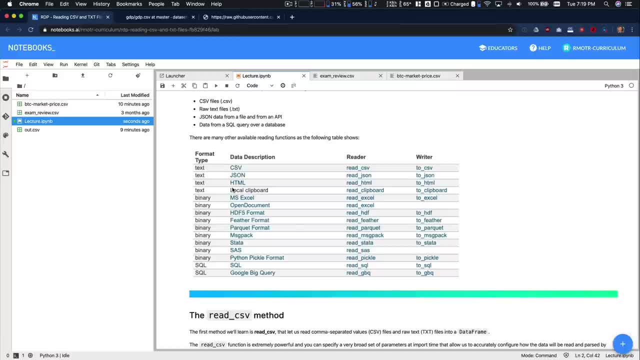 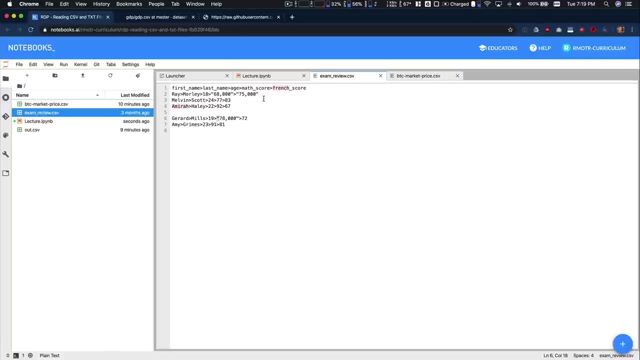 there exists a ton of different ways to customize the method invocation Right. So again, CSV files. we saw there are multiple things that happen- CSV is a pass ahead- that have a header or don't have a header, different delimiters, different enclosing of strings or numbers. 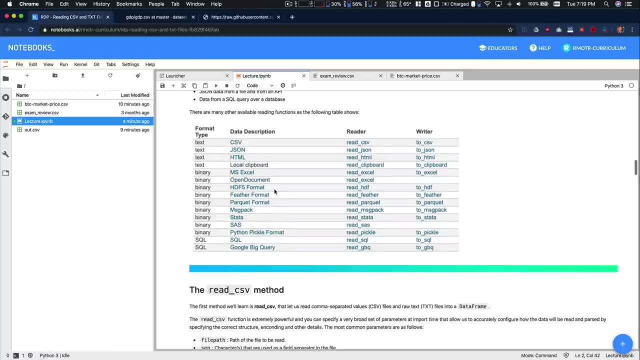 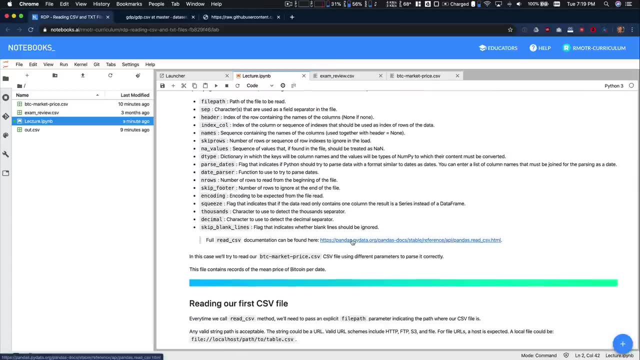 multiple things, blank lines, etc. Multiple things are going to happen And that's all you're able to customize. So it's very, very easy. And also, if you want to customize the, customize all that with the read CSV method. So this is the reference of all the attributes. 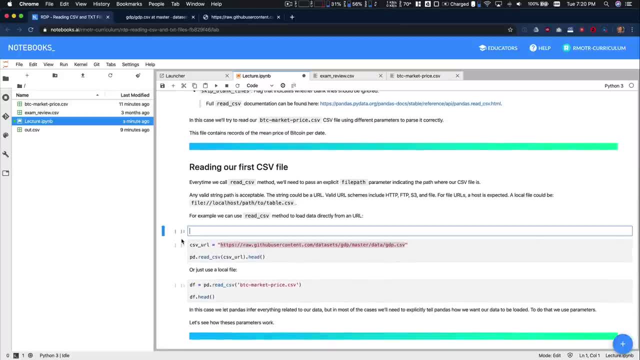 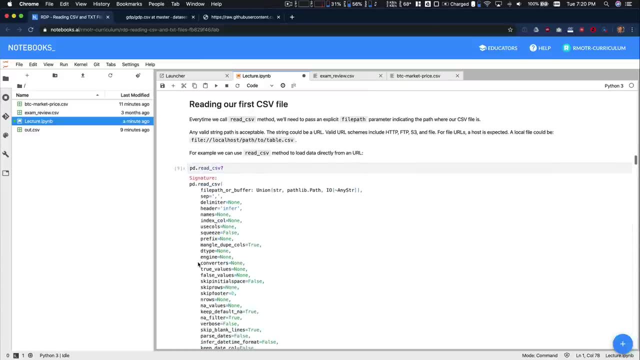 you can pass to it. Usually something that I do, and I do this very often and I use pen this a lot- and I still do something like read CSV and I get the documentation right here to look into the, the parameters that I think I need to pass to my particular use. 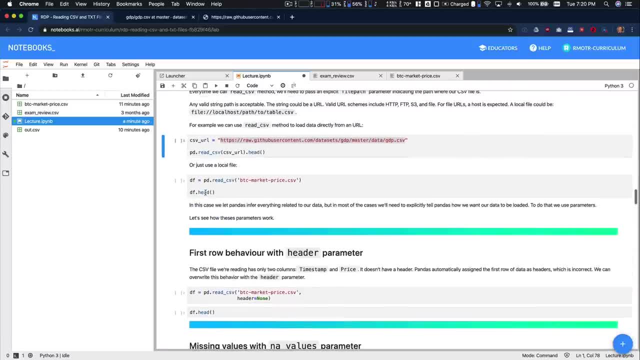 case. So keep an eye always in the docs, because it's impossible to remember all the parameters in the CSV. So in this case, what we're going to do- it's something very interesting- is we're going to parse a CSV file, but it's not located in this computer, it's not locally. 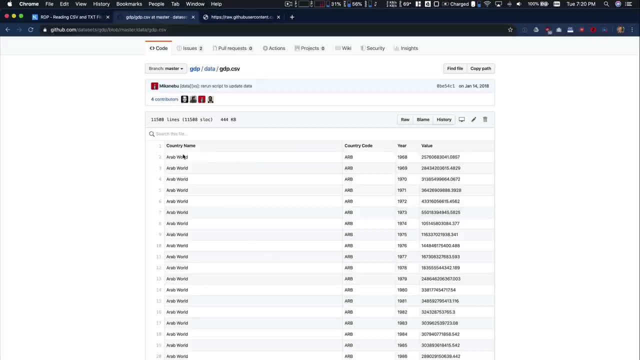 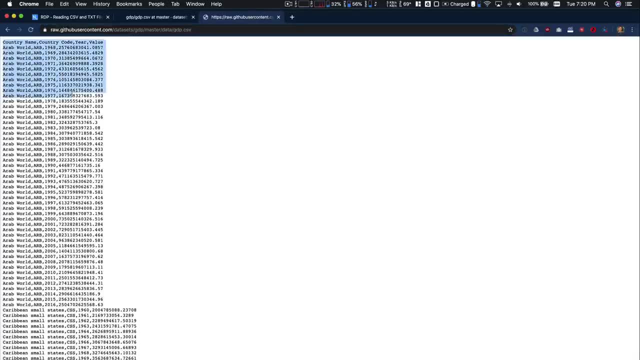 available in the computer. the CSV file is this one right here, which actually is the source. if I get the raw version is this thing. So this is a CSV file. what I could do here is download the file right, So just do. 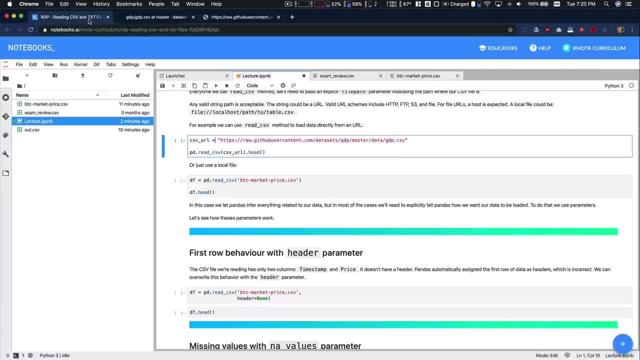 File save. get the CSV file on my computer uploaded here, right, so just copy and paste here, drag and drop it here, But actually pain. this has this nice characteristic that it will read a CSV, that it's either locally, as we did with BTC market price, or it can. 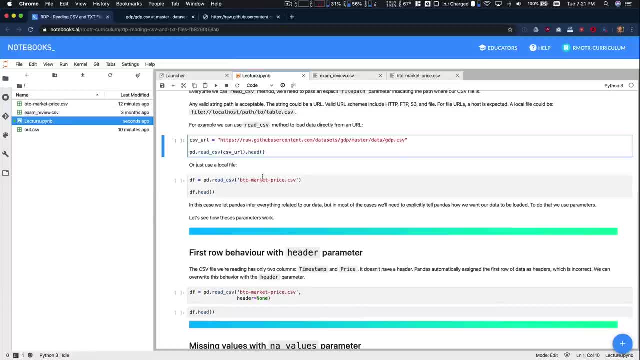 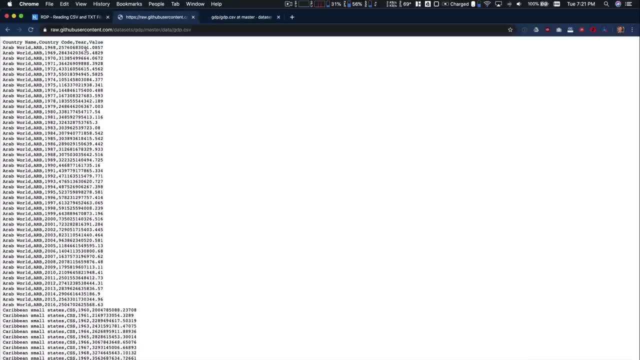 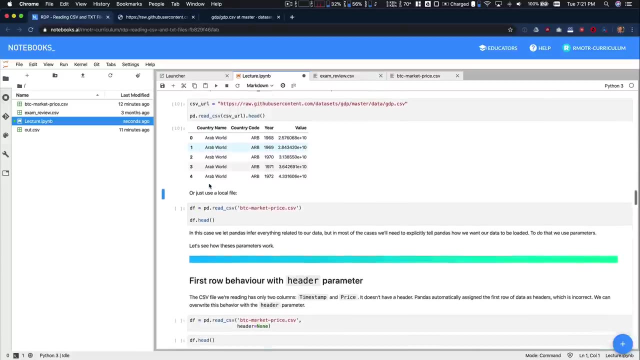 also do it remotely. it's automatically going to download the content of those files And it's going to provide, it's going to save it in memory for further usage. So there's a very neat feature. And again, this is the, the CSV file that we are using. And again the same thing. if it's 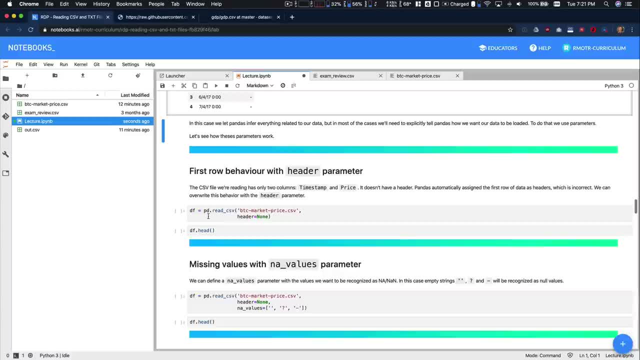 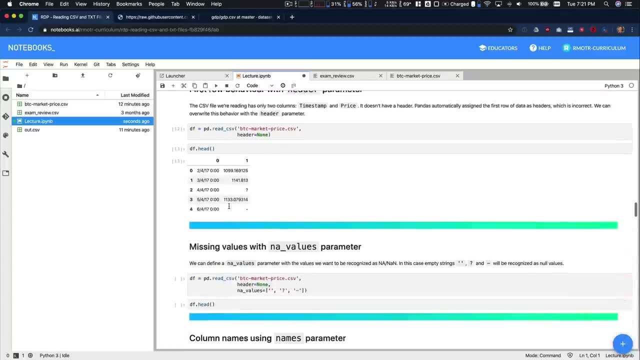 a local file. it works in the same way. So a few features you've seen already. in this case we can do a header known. if you don't want to treat the first row as a header. or what about missing values? we can treat some of these values like a question mark or like. 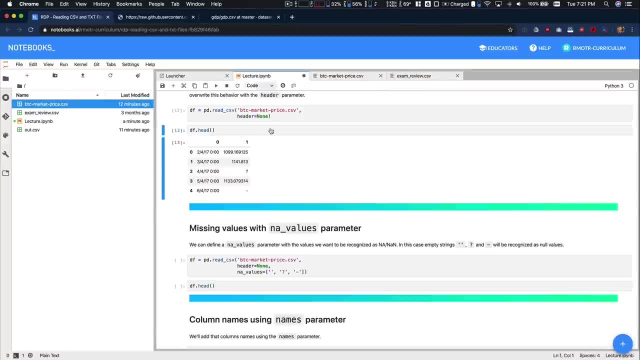 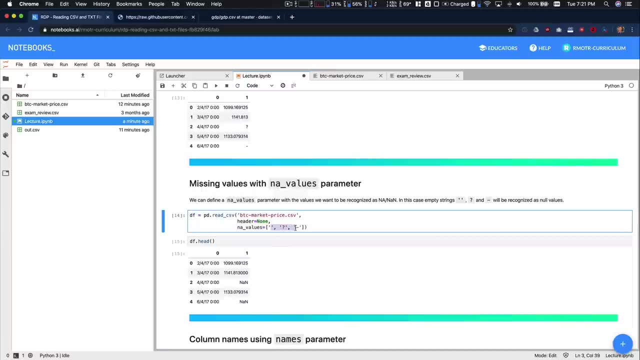 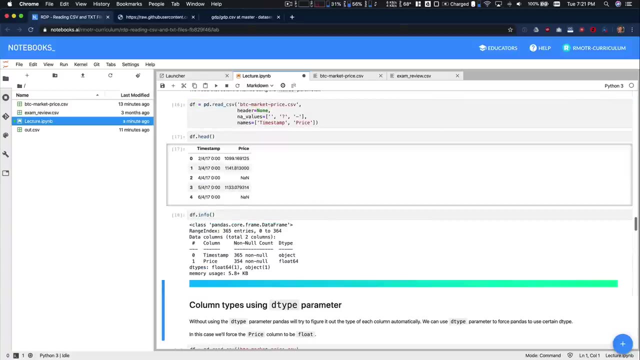 an exclamation mark or dash, etc. as not a number, number, a value, right, so as a missing value. And now any of these values we have passed will be transformed into another number for easier and easier process cleaning. we can pass names, which is going to be basically. 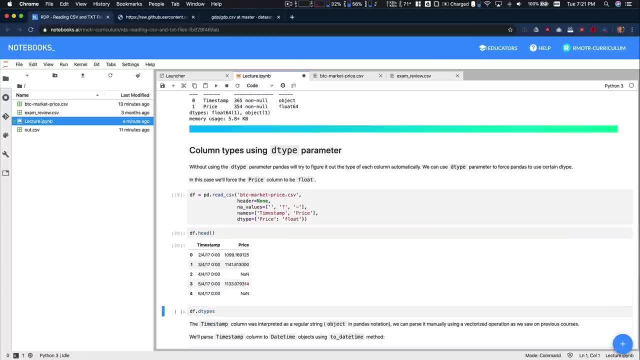 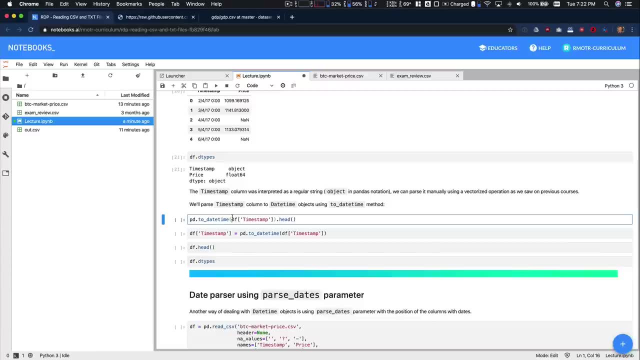 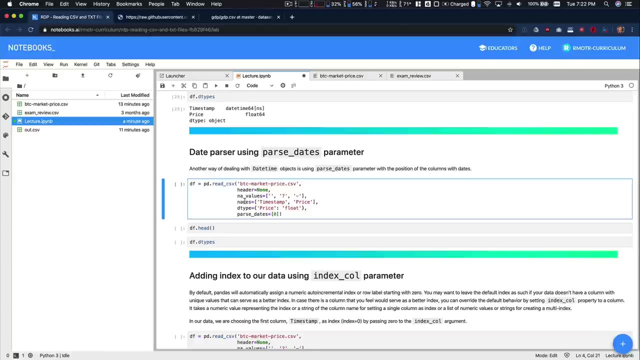 the column names for each one, And we can also specify column types, as you can see right there. So now the types are going to be float And object. we've done this already in one of our lessons. we are parsing the time and there you go, So putting all together. 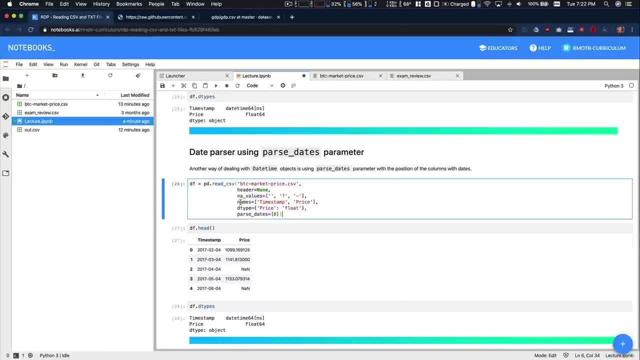 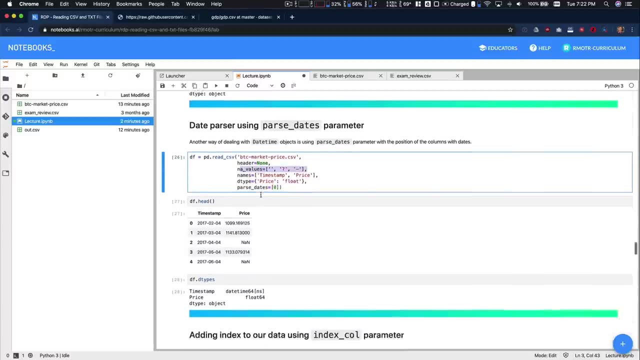 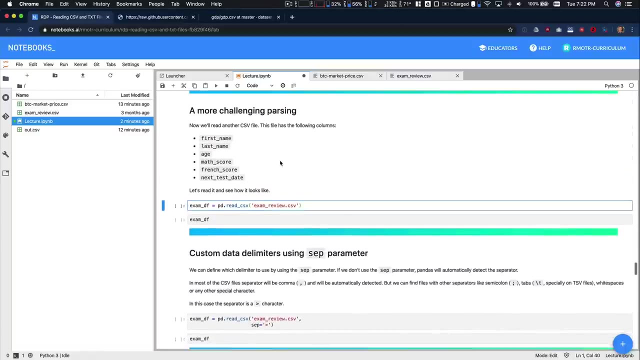 we get to these advanced forms of reading CSVs where we're passing column names, we're passing types, we're asking to read dates, we're passing no values, headers, etc. So this is a pretty common thing we are doing. So what about XM review? if we try parsing this thing, we get this very ugly. 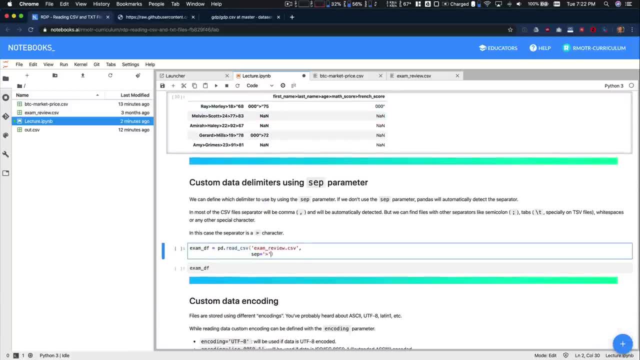 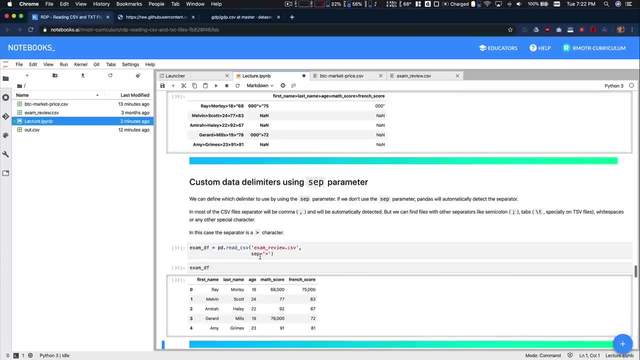 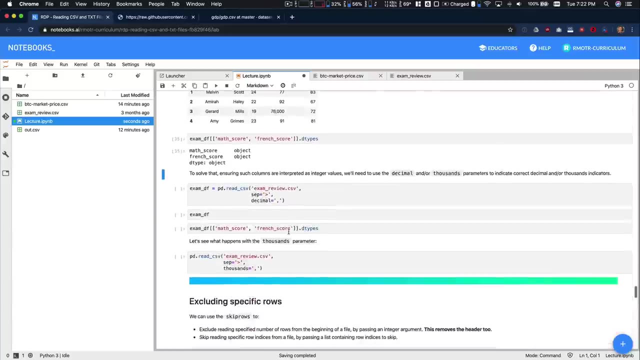 format, In this case the parameter to specify the what we used to call delimiter in CSV is now set from separator. So the separator is going to be the greatest sign and that just works as it needs. So a few more examples you can check on here, the most important: 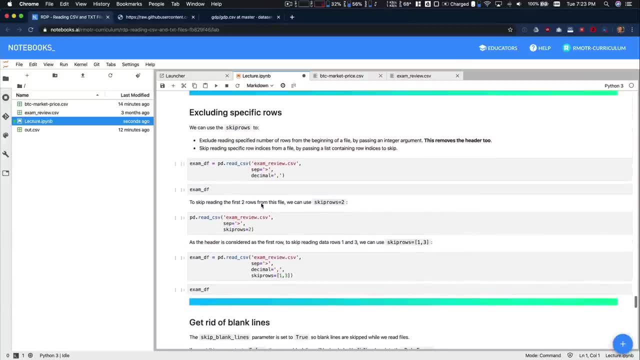 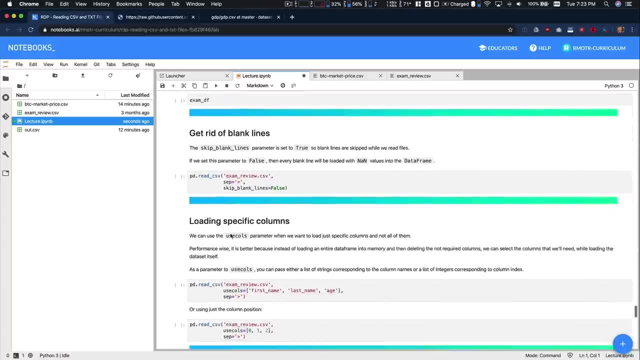 part is following right the documentation to find those particular use cases that you are having. So, for example, something like skip blank lines or whenever there are like empty rows at the beginning, right. so if you have empty rows at the beginning is something. 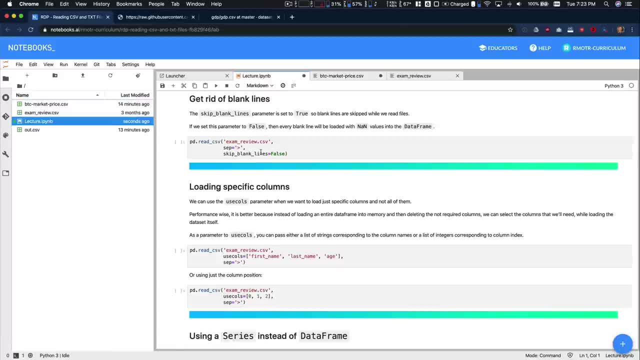 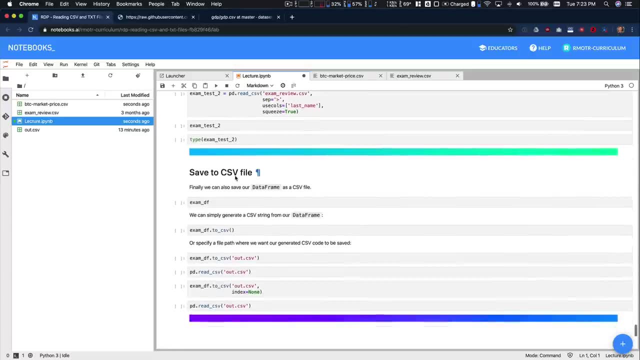 you can also say skip rows so you don't need to parse those, it's not, it's not going to break, etc. So that is all part of the read CSV file And to finalize this part, at least CSVs I'm. 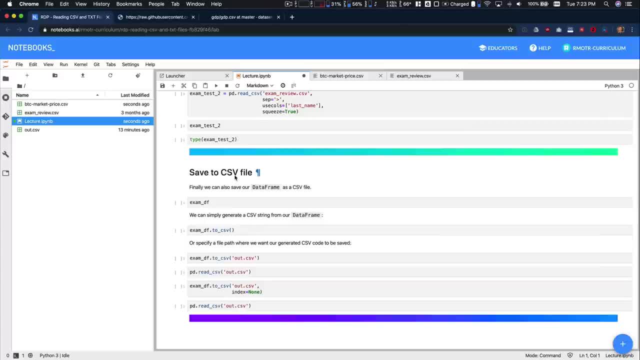 going to tell you something that applies to pretty much every other data format. as you have a read something method, there's going to be a two something method. it's basically the process of writing, So you can do read CSV or you can do two CSV. So with these, 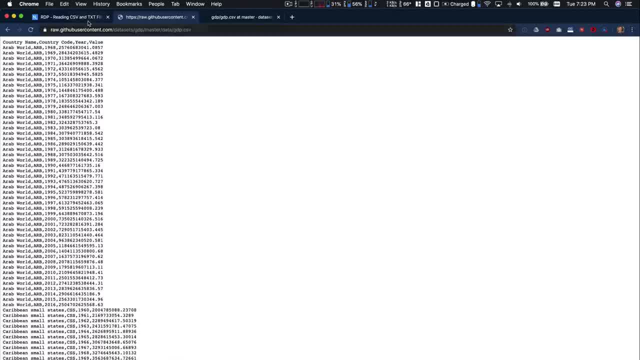 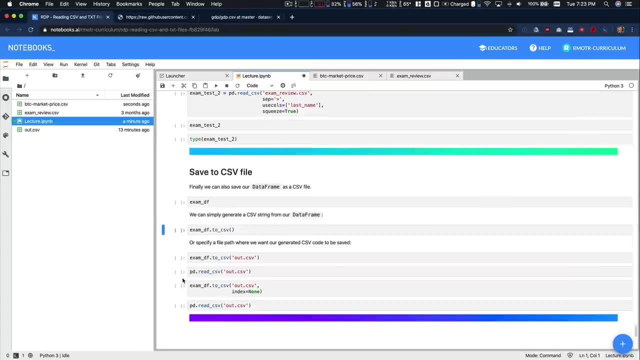 CSV that we imported from the external source of the remote source. they can just do two CSV and it's going to store it locally, All right, And there are multiple options also to pass to CSV the delimiter or actually the separator, if you want to include a header. 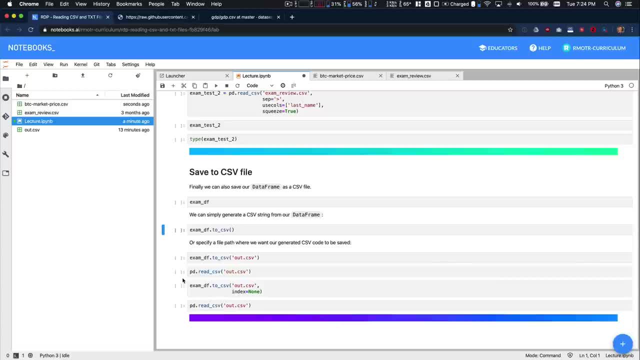 if you want to include an index, etc. they're pretty much the same as the other one, But the idea is that for every read something method there's going to exist a two something method. that it's basically the process of writing. So let's move forward with a few. 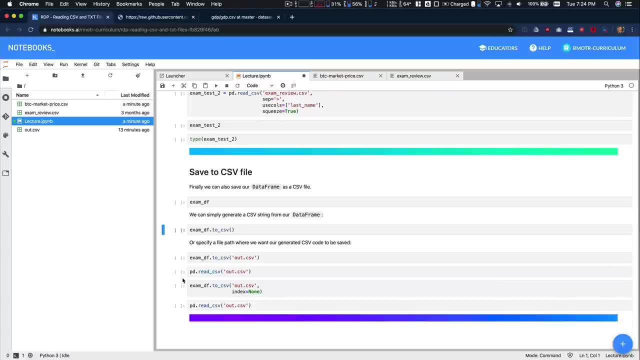 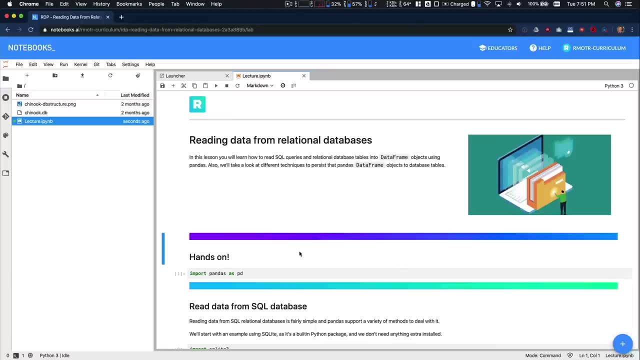 more data formats And interesting. we're going to get to read directly HTML pages in just a couple of minutes. And now it's time to read data from databases. we have already done that in our real example with pandas- part of the tutorial- But I want to show you. 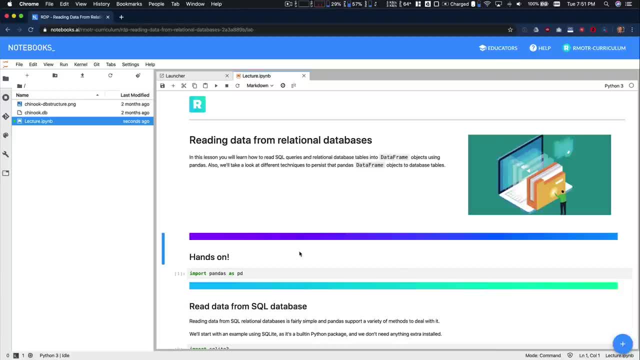 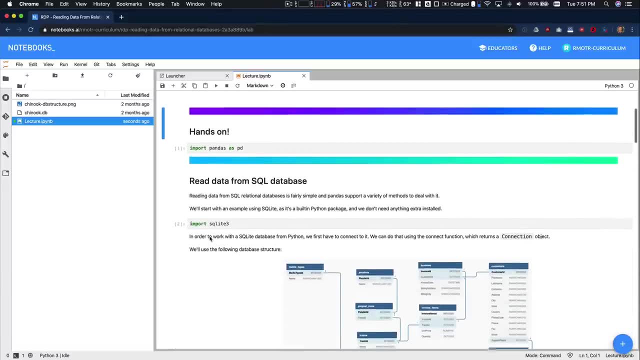 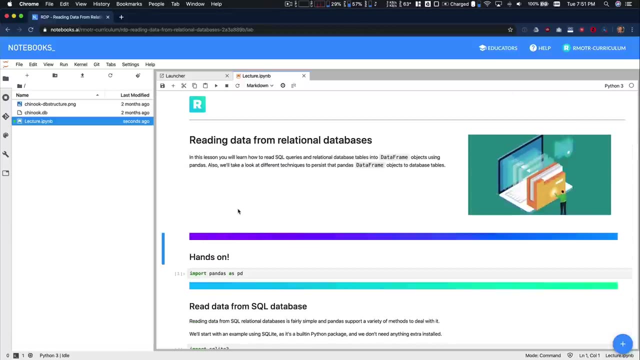 a little bit more details. details So you understand how data is being processed, in case this is a common scenario from you importing data from databases. So the libraries you will need first thing, depending on what database engine you're using: Postgres, MySQL, Oracle, etc. 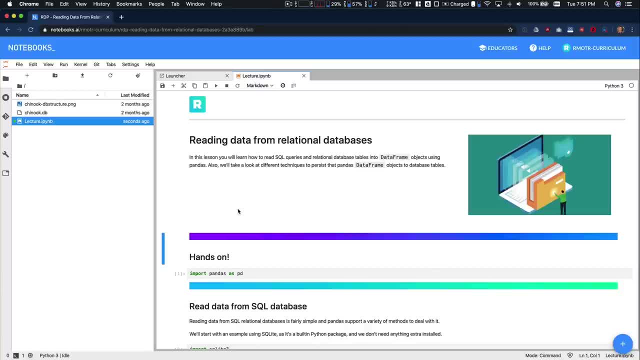 you will need to install different libraries, But the API is. once you have installed, those libraries are going to be the same. there's actually PEP from Python that actually defines the interface for databases. libraries and pandas can work with pretty much any- any database. 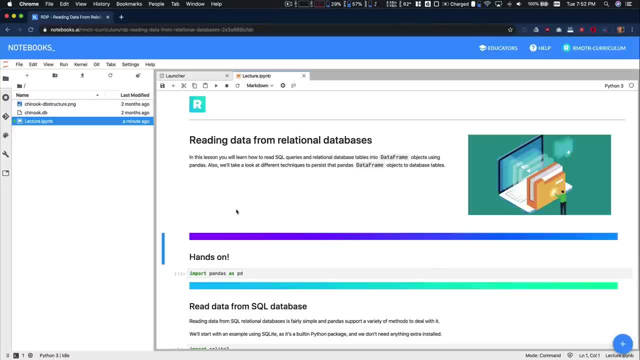 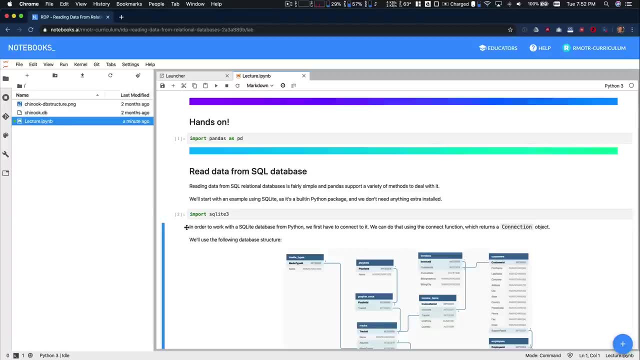 of these SQL common database that comply with that interface. In this example we're going to use SQLite Because the database- right here, there's nothing, no server to connect, etc- is extremely simple to get started And the example we're going to use, or the database example we're going, 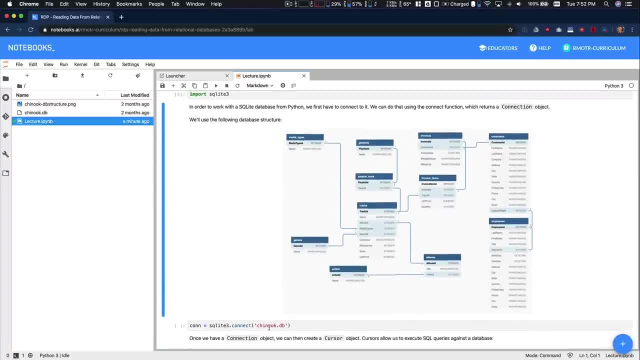 to use is actually different one from our previous database rating. In the previous one we were using Sakhila. In this case we're going to be using Chinook, which is a smaller both in structure and in size, So it's going to be a little bit simpler. So to get things, 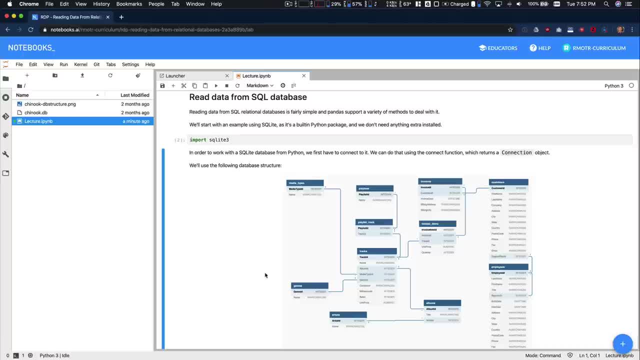 going here. the same thing that we did with our previous part, that was, how to read data from files. I show you how to actually read data using Python. So forget about pandas for a second. I told you, if we go back again to the beginning of time, there was no pandas. This was a way. 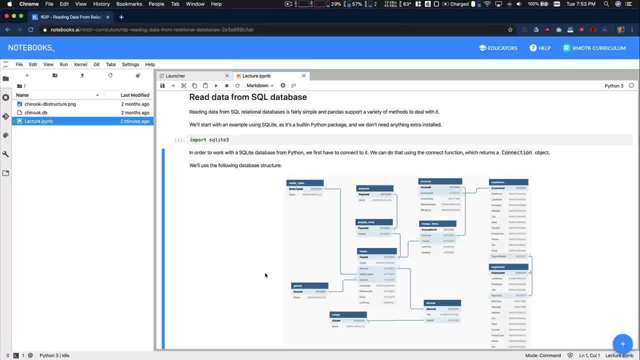 we were reading files, open FP, FP, read lines, etc. So I now want to show you what predates to pandas, what was the default way to read data before pandas, which is with the regular- again- interface from Python. So the way it works is: we're going to import SQLite three. 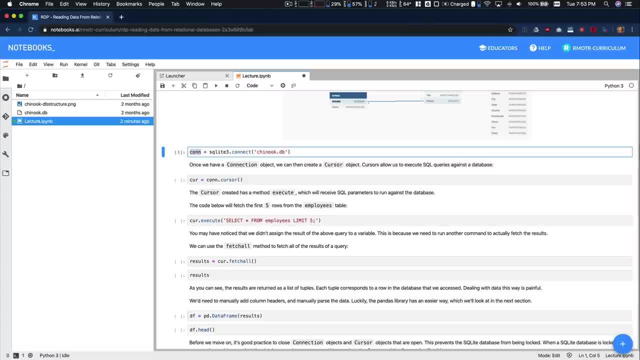 we're going to create a connection And now with this connection we have these common interface. that again is going for pretty much any other database that you're used to, And the default behavior is we're going to create a cursor And we're going to execute. 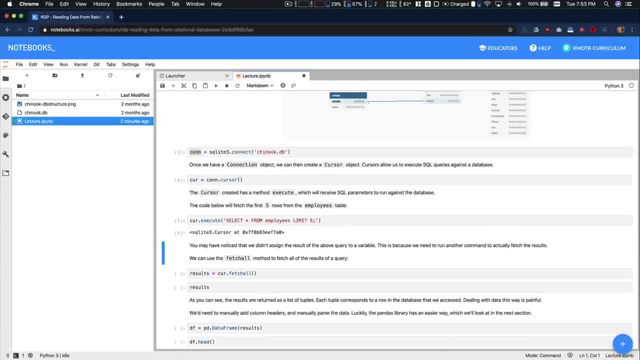 queries using that person. In this case, we're going to execute a regular select star from employees limit five, so we want to have five, five records out of the table. employees, Once you have executed the query, it's like they're waiting. 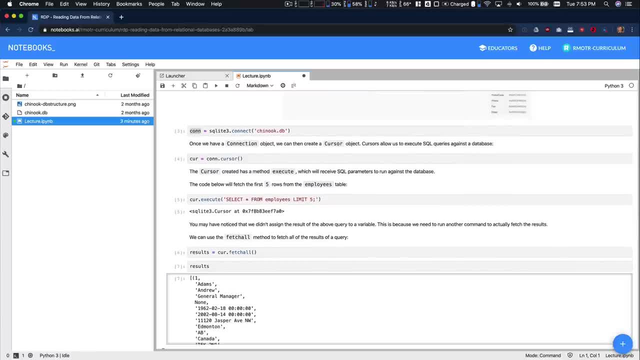 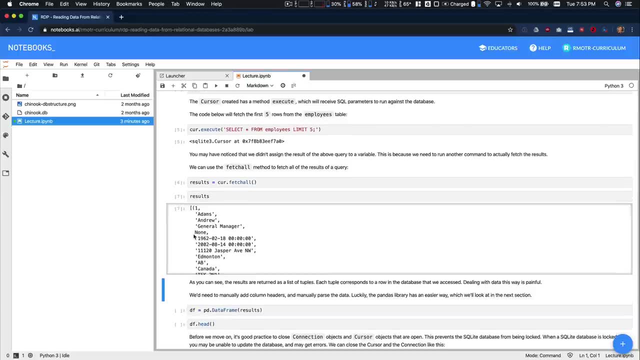 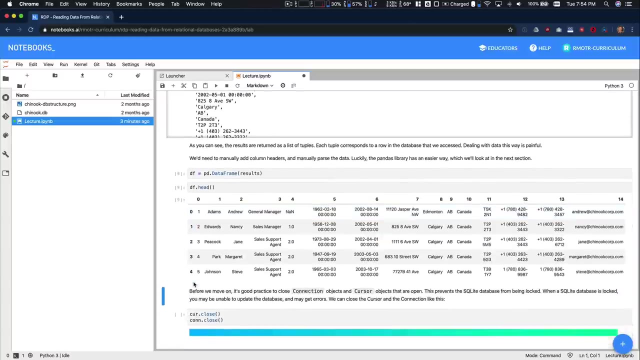 You can do a fetch all to get all the results of that query. And here are all these results. As you are noticing, this is the result is a list of tuples, So it's not extremely useful. Now, if you combine it with pandas, you can just create a data frame out of that info. 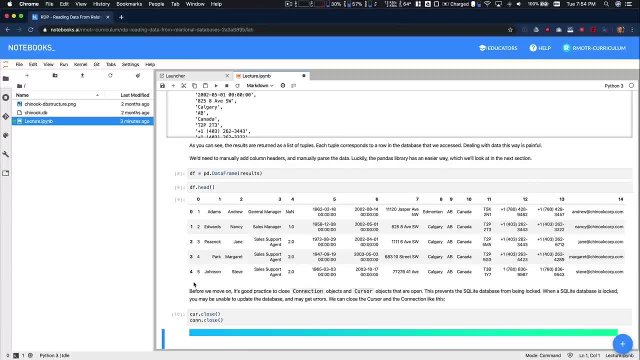 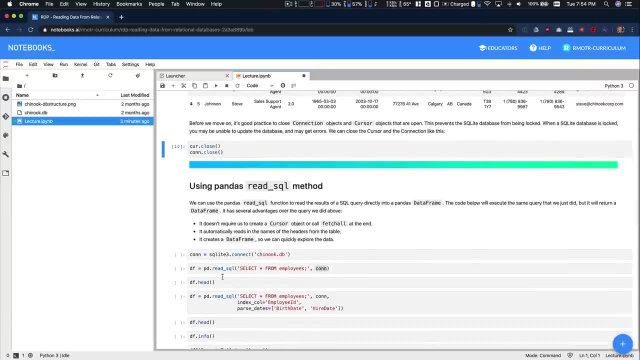 And we're close. it's not perfect, but we're close. So let me show you now, before we were going to close the curtain, the cursor on the connection. Let me show you now how we work with pandas. With pandas we have, as we have, a read CSV. 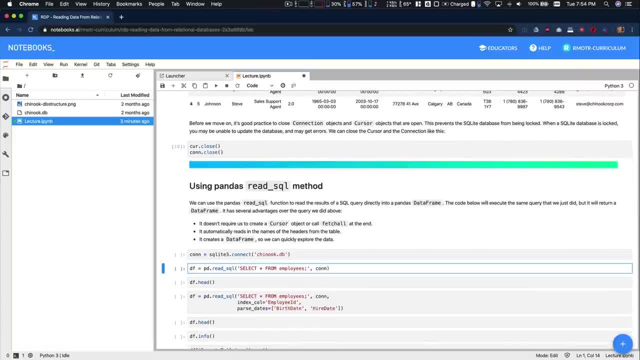 method. we also have a read- see as read- SQL method And in this case, what this method is going to receive is: the first parameter is going to be the query that we're passing in. the second parameter is going to be the connection, that the object, the connection. 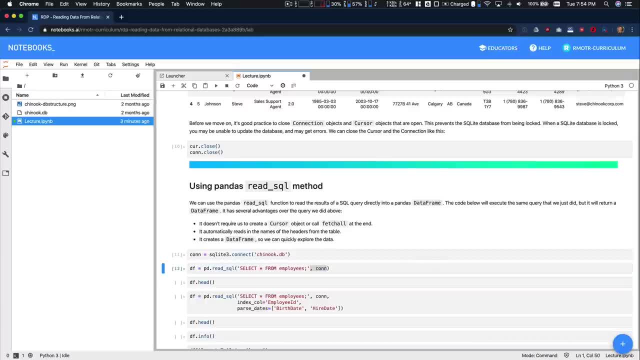 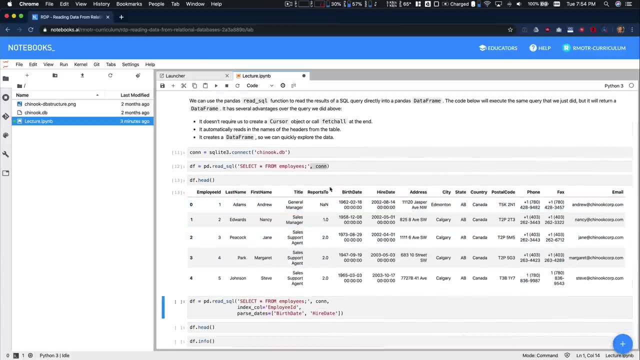 object to actually issue the connection by pandas. So it gets as simple as writing the query, And now everything has been imported into a data frame, including column names and all that. if you want to get a little bit fancier, you can either specify the: 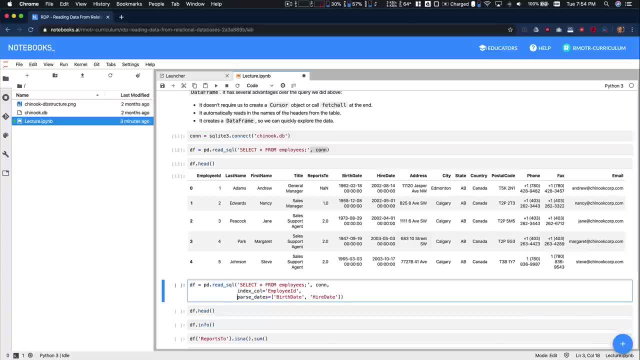 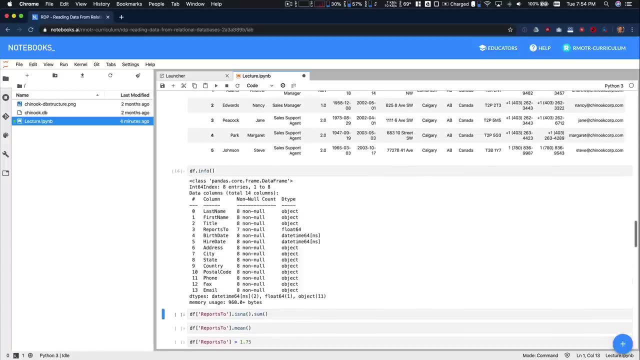 index column that is going to be used, of course, as the index, and and also what types to parse for a specific column. So now we have pretty much all the work down. So we're going from something very manual as processing things with a cursor, etc. which might also 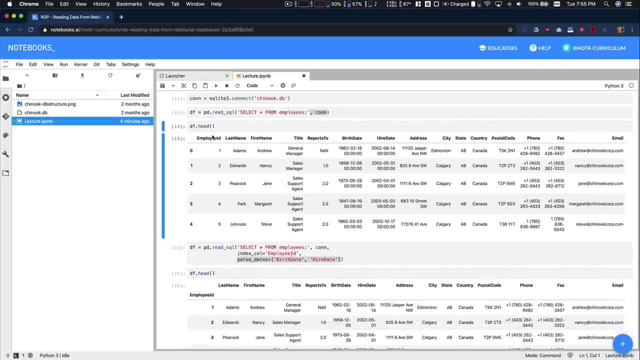 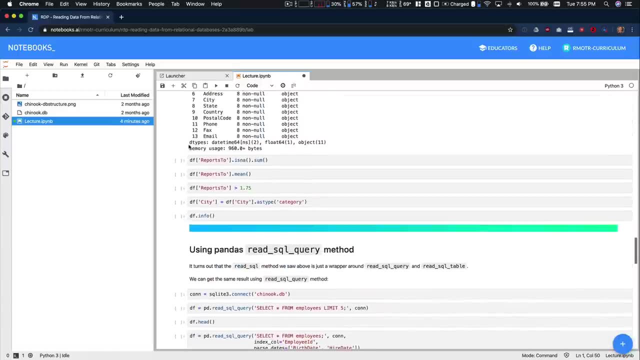 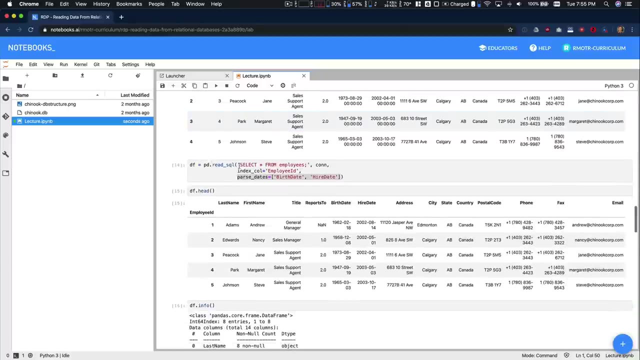 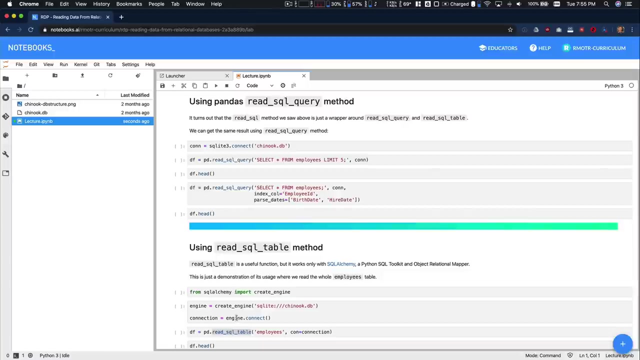 be slow to using pandas to directly import the data from the database. There is actually a caveat here that I'm going to tell you is kind of a very deep detail of the way painless works, And is that the read SQL method is actually a shell for two other methods: read SQL query and read SQL table. Alright, so read SQL table. 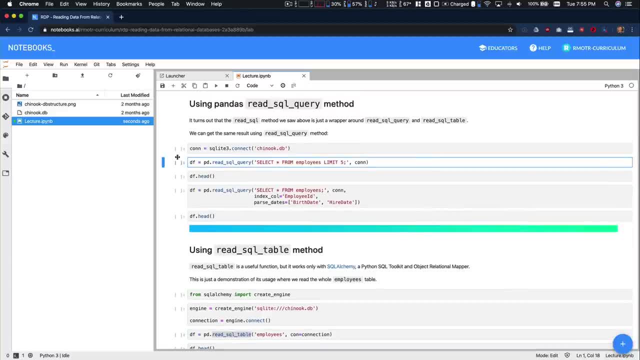 and read SQL query. When you're using read SQL, it's actually kind of forwarding the work to either query or table. Read SQL query is the default behavior, what we've done so far. So in this case it's just going to issue a query and the connection is going to read. 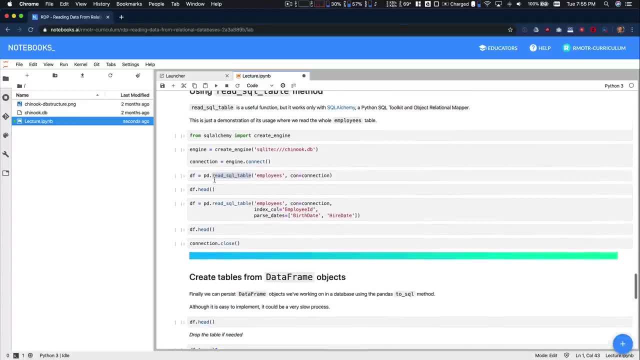 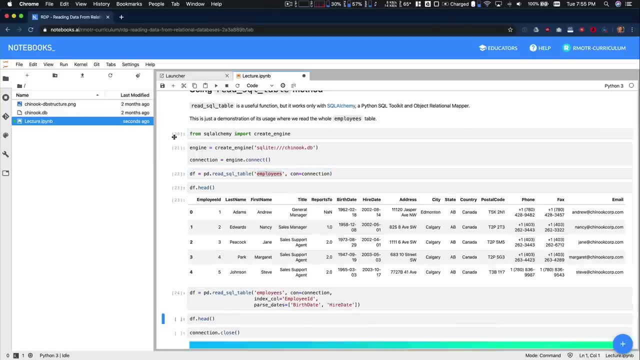 it for you. In contrast, SQL table is going to read an entire table. you just pass a name and it's going to automatically give you all the information for it. So in this case, all the column names, etc. So it's. 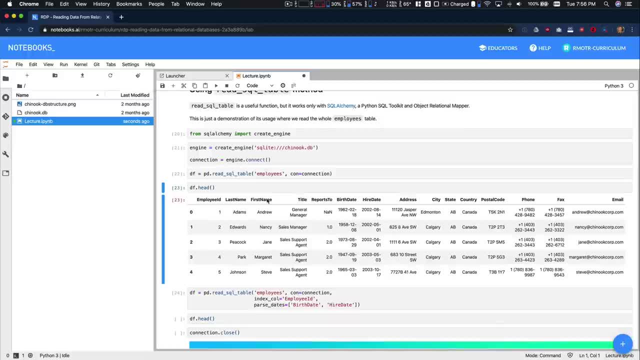 a lot simpler to read an entire table. the only thing to keep in mind is that to use this method, you need to install these libraries, SQL alchemy and the connections generated from it. So in this case, we create an engine and we create a connection: objects. And now 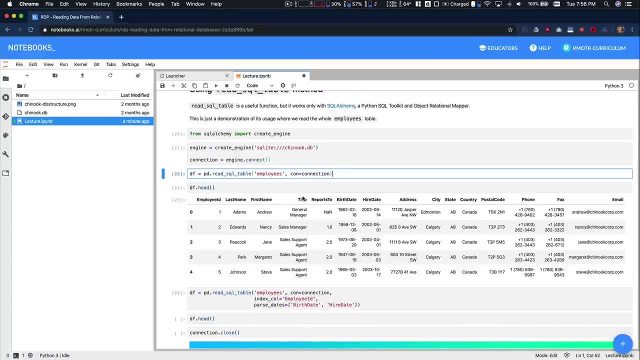 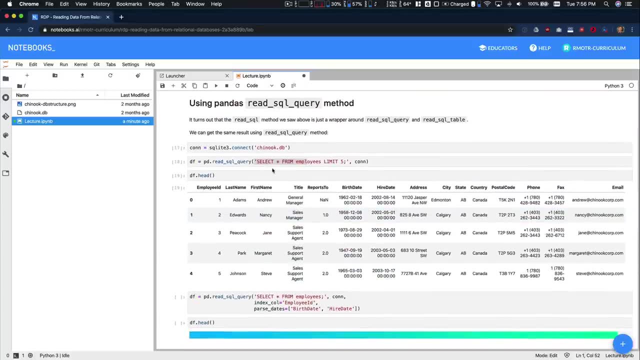 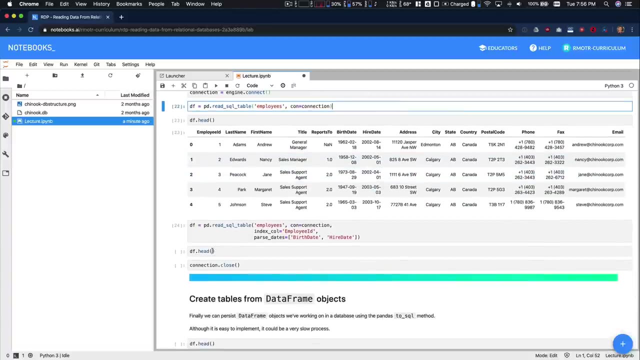 we can pass the connection. object: object: sorry for pandas to do it. So again, it's pretty much the same. If you find yourself doing red star from this table or red star from that table, it's a lot easier just to read SQL table. and that's gonna do it just once. 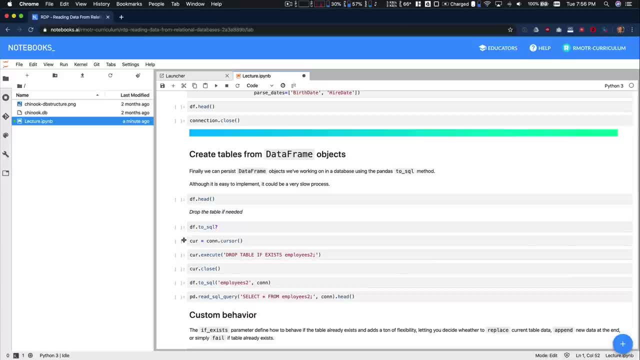 As we saw that read CSV files had to CSV. sorry, read CSV method had a to CSV method. the same thing happens with read SQL. there is a read SQL And there is also to SQL. what's what it's going to let you do is get the from the database. 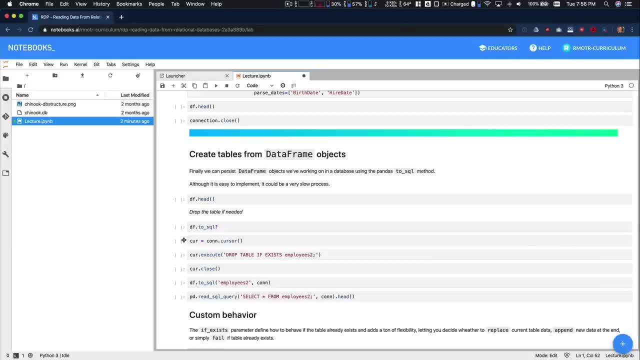 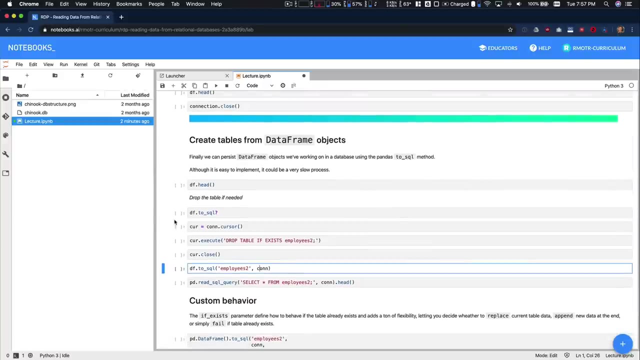 and write it down into a database table directly. So it's going to also receive the connection right. So to SQL is gonna receive what table name of these data frame? what table name is going to be on a connection object? Now, something to keep in mind is that to SQL has an important parameter, which is what? 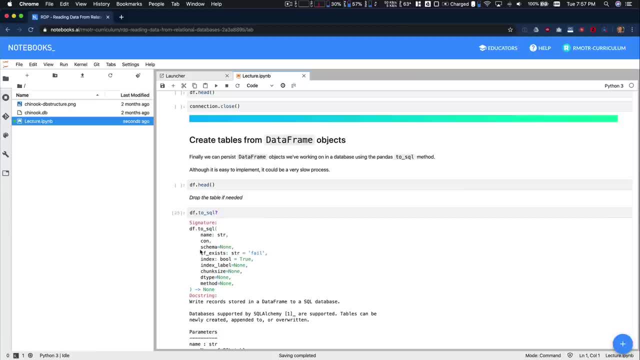 happens if the the table already exists, that in the default way it's going to fail, just going to throw an error when you are trying to save data to a table. And this makes sense because, as data analysts, we're usually reading data and processing it, we're not so much writing. 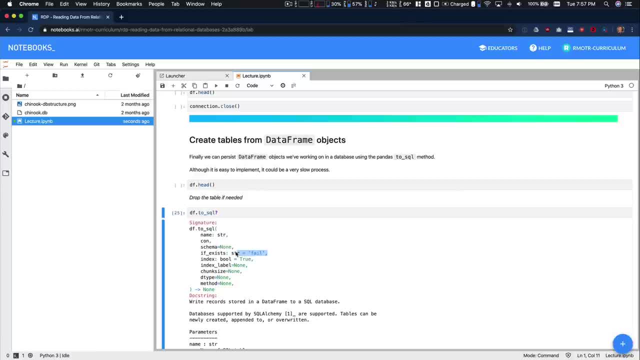 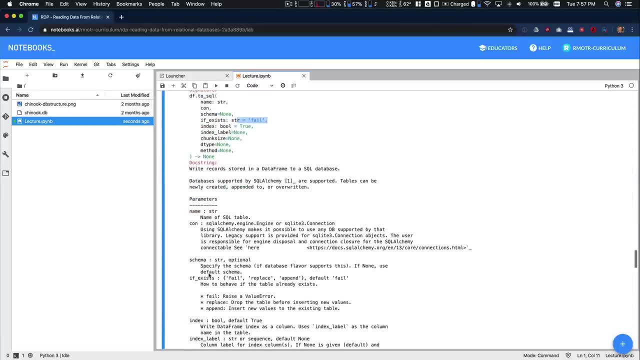 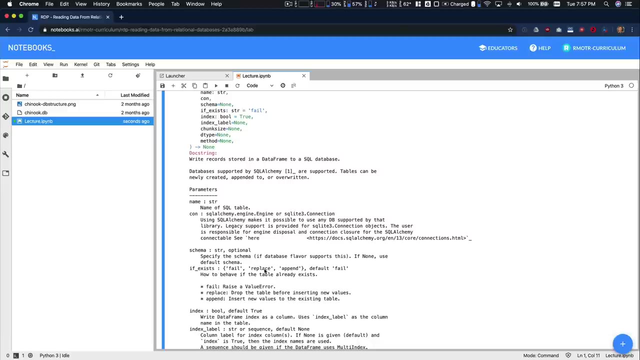 it. So we want to make sure that it's not by mistake. But if you do actually want to write data, you can just change this parameter, if exists, to something like replace or append. usually we're writing to intermediate, intermediate tables. Again, you can choose either to replace. 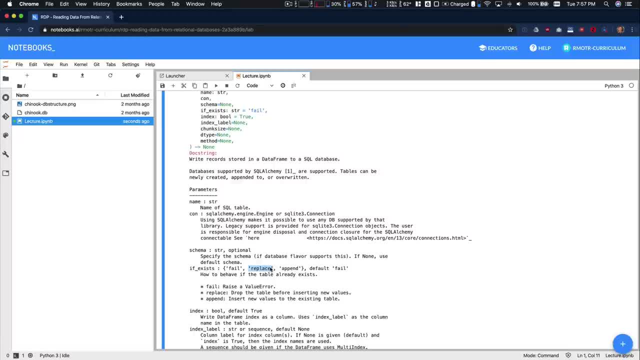 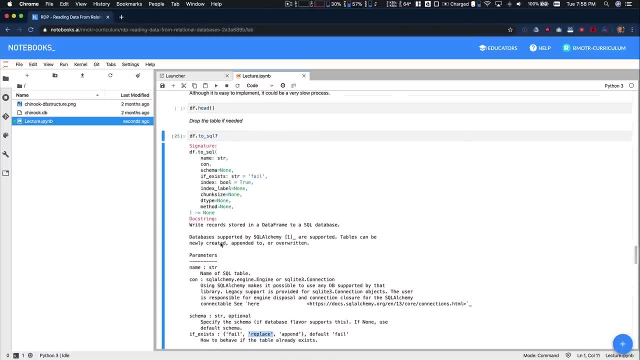 the whole content of the table. be careful here. or to append right, just write it at the end of the current table. So that's just for to see. So this was the way to read data from databases. Of course we're not touching on anything like SQL and all that, but it's. 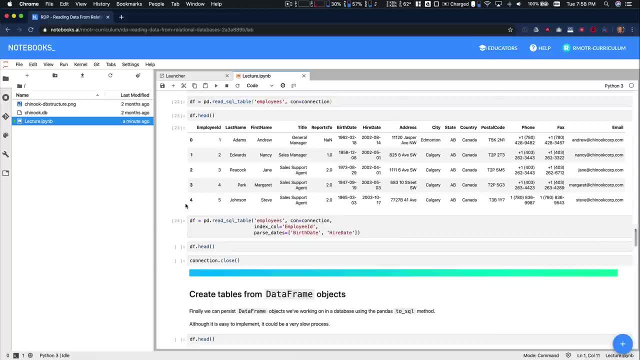 a lot more advanced. It's just for you. If you already know SQL, if you're already working with databases, you can pretty much copy and paste what we're doing here And you're gonna- you're gonna get your data imported into Python. So let's move forward to read some. 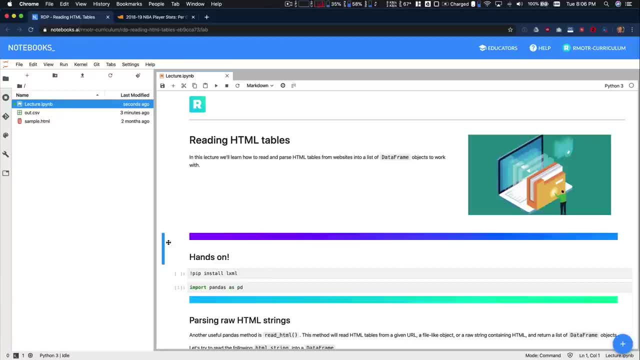 HTML files. And now, very quickly, I'm going to show you how to read tables or data frames directly from HTML web pages. To be honest, this is a simple method: is going to be just read HTML, But it depends a lot on the structure of the web page. So if it's not well structured, 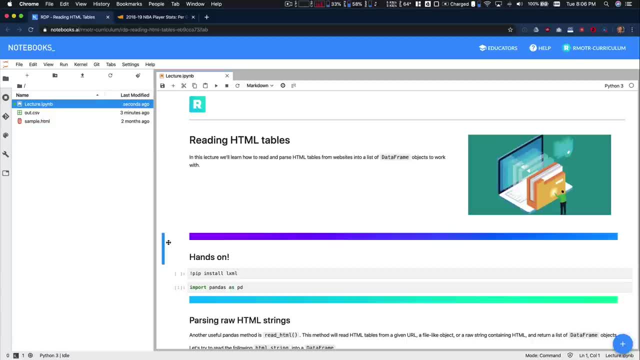 the tables are not correctly created, you're gonna have issues and you will have to do a ton of data cleaning. In my experience, whenever I try to parse a table from a well structured site like Wikipedia or some stats site, it usually works very well And it's a very quick way of hacking. 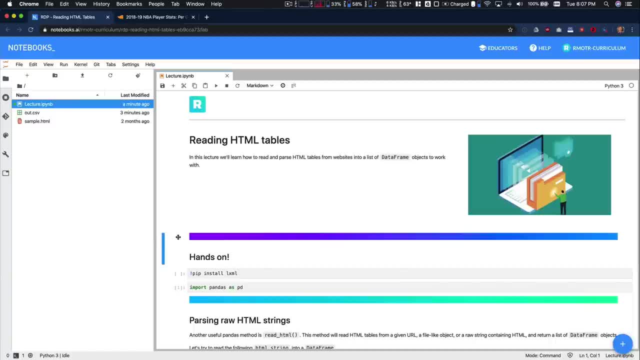 you know, whenever you have questions, you know, like I don't know, I need to know the GDP of countries. instead of looking for a GDP data set, you can just go to a Wikipedia page. there is usually a table there. you can directly parse it and you are done So. 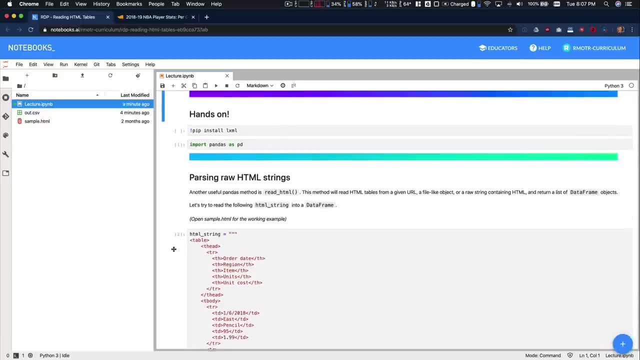 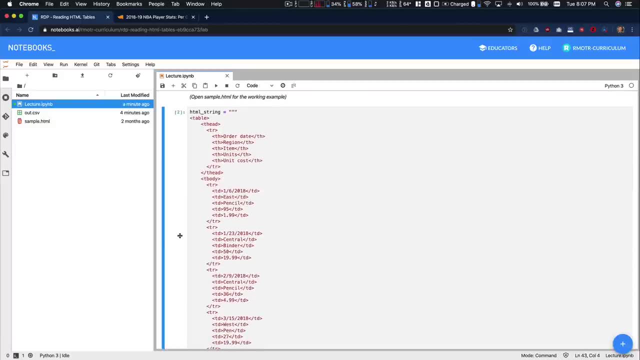 again it's. it's a relatively simple way to get some data For quick hacking and exploration. The way it's going to work is we have these HTML created. It's just for testing purposes, to get us started. Usually, of course, you will try to read something. 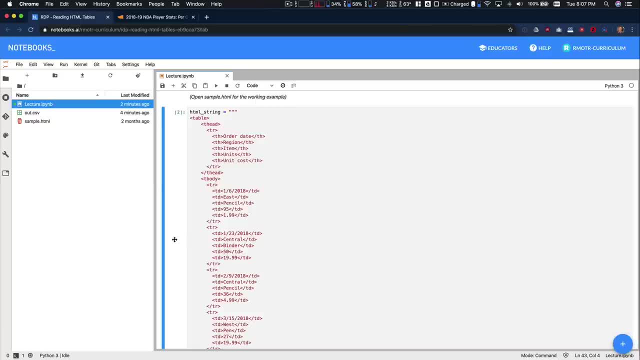 from a live website. So you're going to pass the URL to the read HTML method and the read HTML method will download the content of the page and parse it. Let's suppose we have the content already, the HTML, And this is what it looks like. there's a exactly the same HTML. 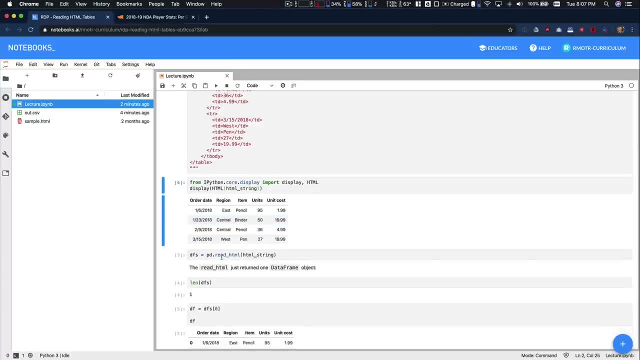 we have on top, So we're just displaying it here in the notebook, And what we're going to do is we're going to invoke the method read HTML. the read HTML method is going to parse the entire HTML and look for multiple tables. not just one site will potentially have multiple tables. 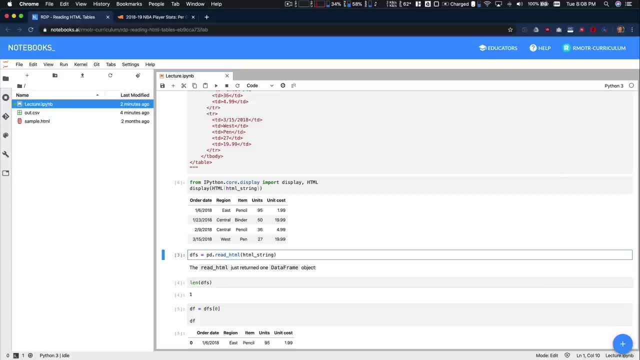 Even if you don't see them, the it's a common way to structure things in HTML to use tables. That's why it's going to parse multiple tables In this case. we store them all in the DFS. multiple plural right. multiple data frames. 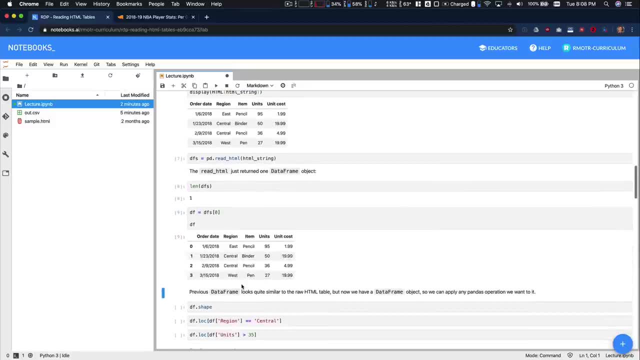 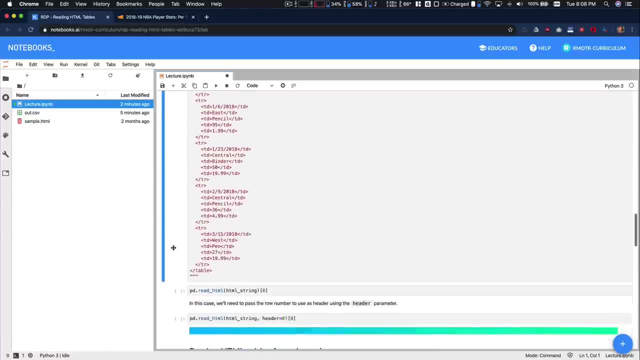 And we see there is only one. So in that case we're just going to get the first out of frame And it has correctly parsed what we had before. just working in the same way, The same is going to happen with, for example, things for heads and all that if the table doesn't have a header, it's going. 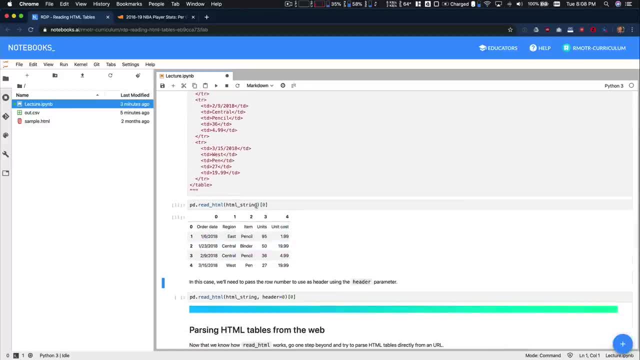 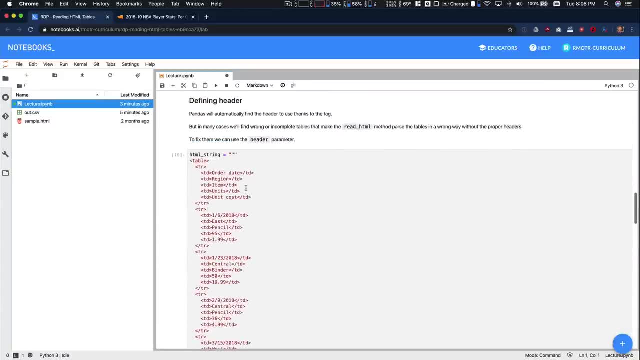 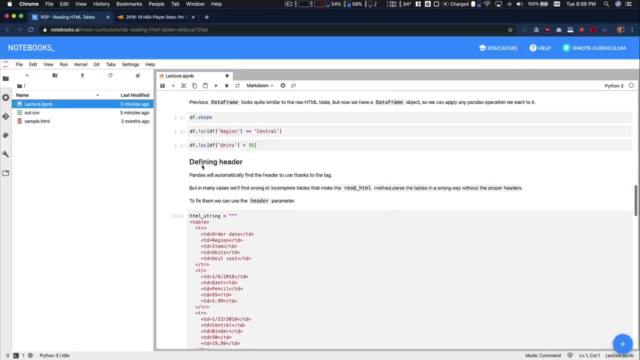 to automatically write. understand that in that case. So that's pretty much as we know it already. In this case, what you're going to see is that what I told you before about data cleaning process Is that these table does not have a header like the previous one that has a T head, T. 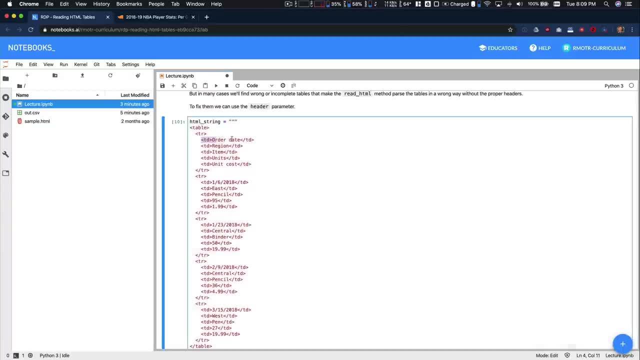 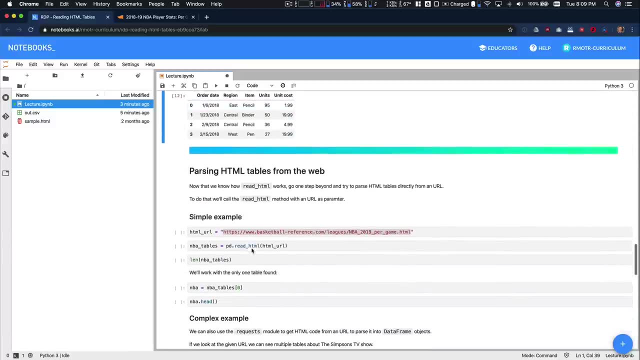 head attribute. in this case, a header is just another row, So that's why read HTML is going to have issues and you have to provide a little bit extra information. So let's see another, more realistic example And we're going to parse data directly from a website. let me 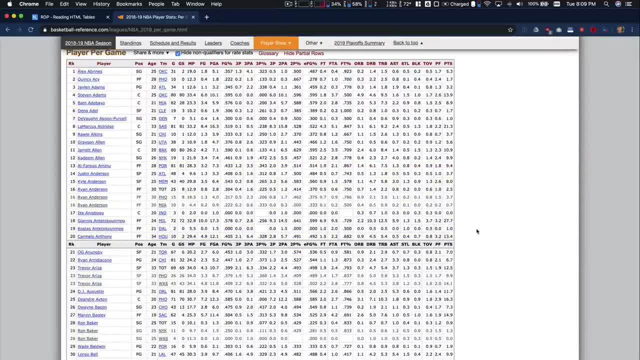 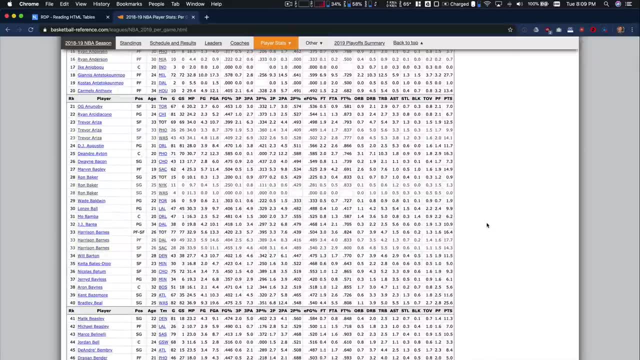 tell you here, just just for educational purposes. you always need to understand if you have, if the data is public so you can actually see it. You can actually parse it Again for Wikipedia, at least what I do- the content is created. 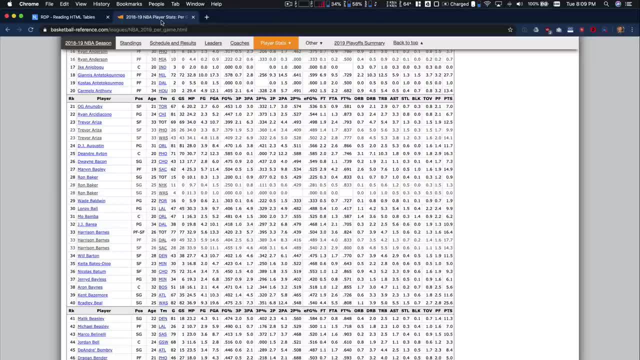 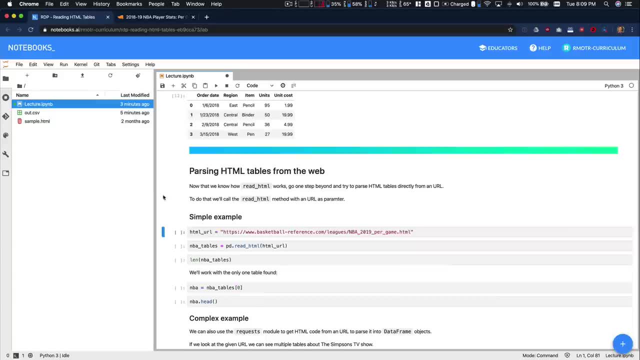 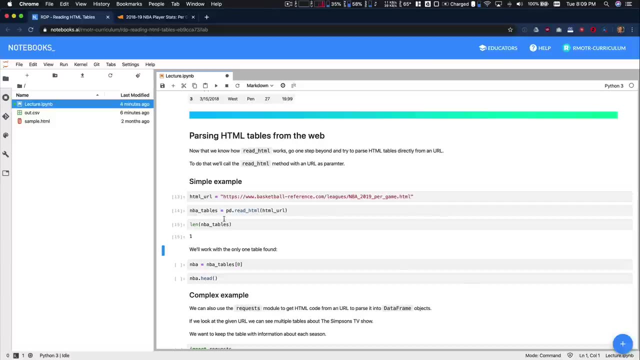 comments so you can get a hand on it. The what we want to show you here is that a very complicated table that has multiple headers, etc. So that's why we're using this example, So we're going to get the URL and we're going to directly do: NBA tables equals. read HTML. 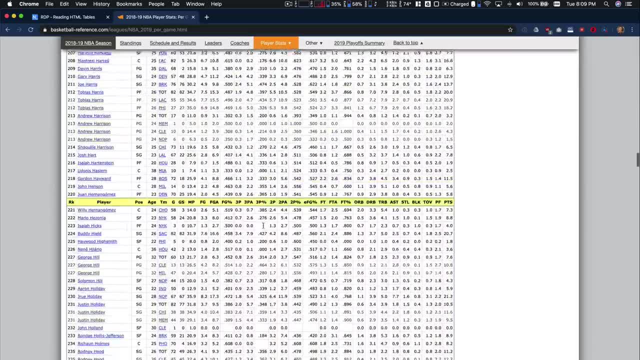 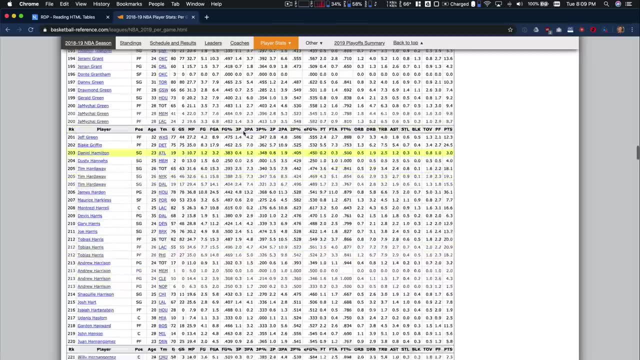 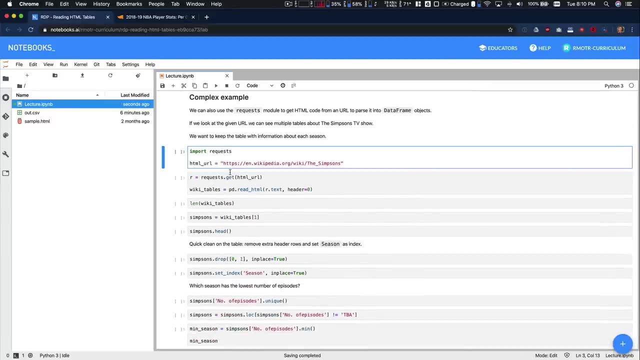 the only table in this page is this one, the large one, And now we're going to get NBA is going to be that, and we see that the all the players in this case have been parsed. What about something else? Let's actually open this page. 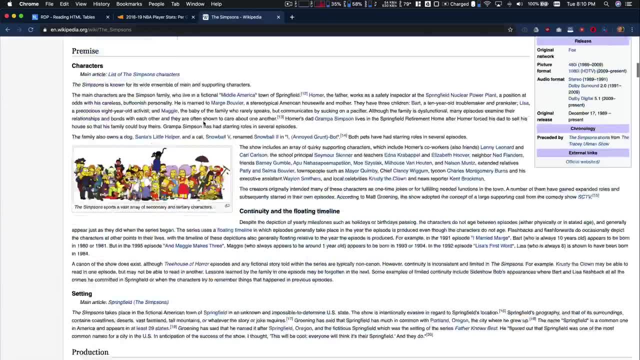 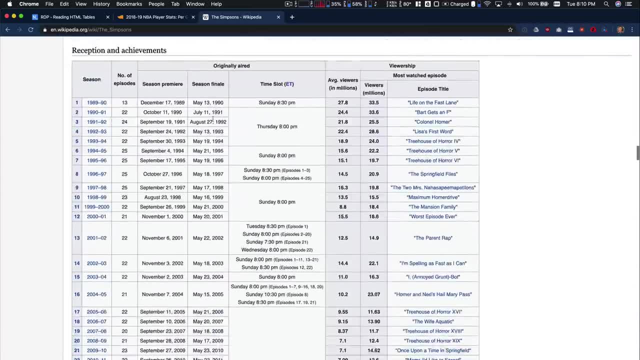 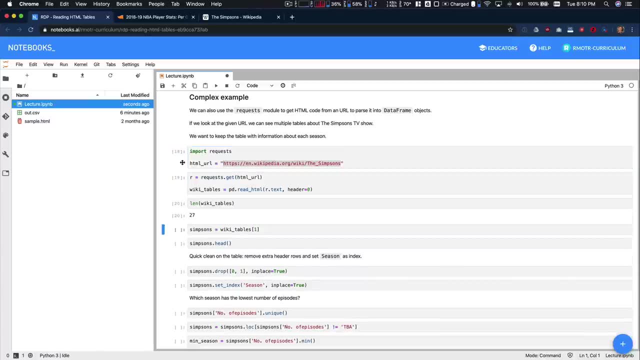 right here the Wikipedia for the Simpsons, And here we will probably find several tables. See, we have one right here, this one, So I'm going to import it. We have 27 tables. Again, you don't see it. You don't see them, sorry, but they are there. And the 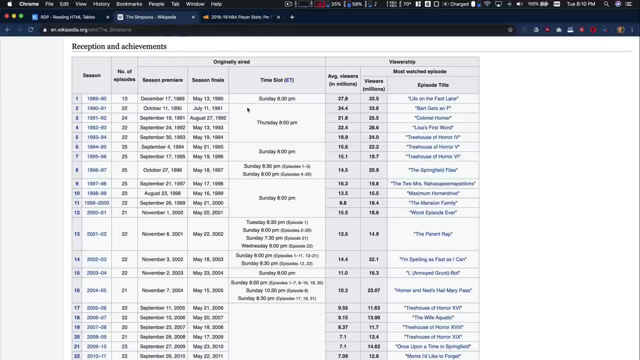 most important one is the one we care is this one right here. So the problem you're gonna have with this table is that it's using both columns, pounds and rows pants. So in this case, this column here spans for 123 columns And these row here spans for 123, at least. 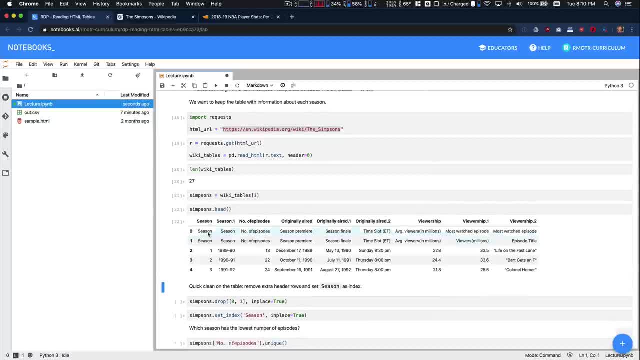 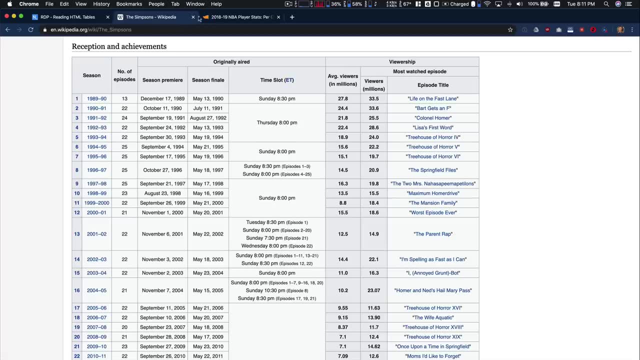 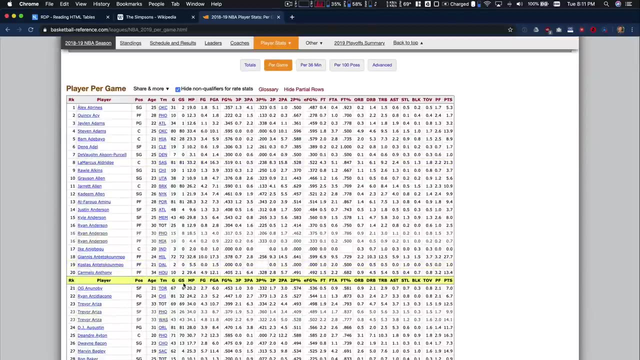 three rows So that column stands, results in these very ugly data frame and you will need a little bit of extra cleaning. So the problem you're going to find with HTML tables that usually there are: things are not well formatted for machines, they are formatted for humans. So, for example, in this case, 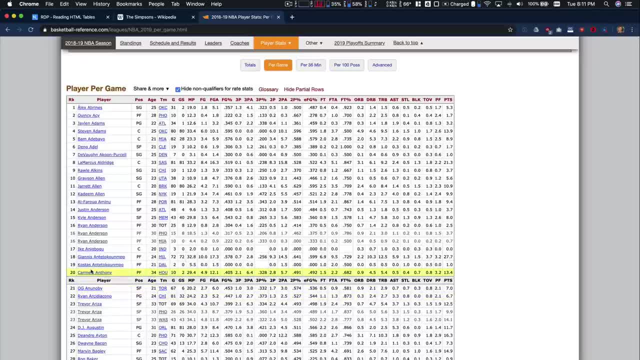 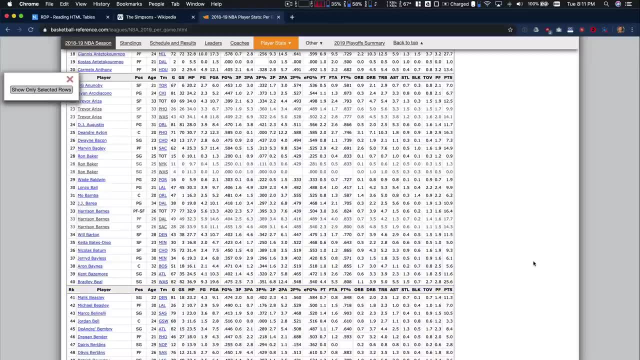 we have this header repeated. when you parse this data, you're going to find that every 20 rows, there is going to be a header row and you will have to clean it. every four, in this case, 20 rows, you will need to drop it, you will need to clean it, So you will. 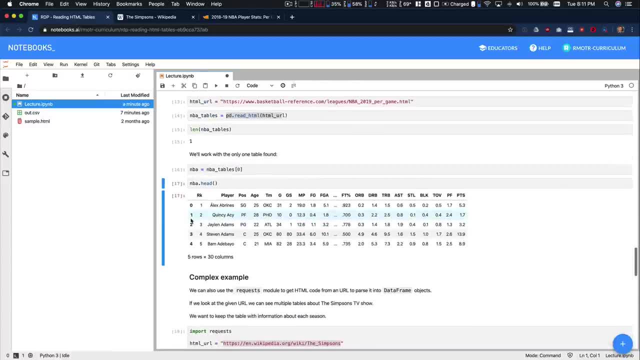 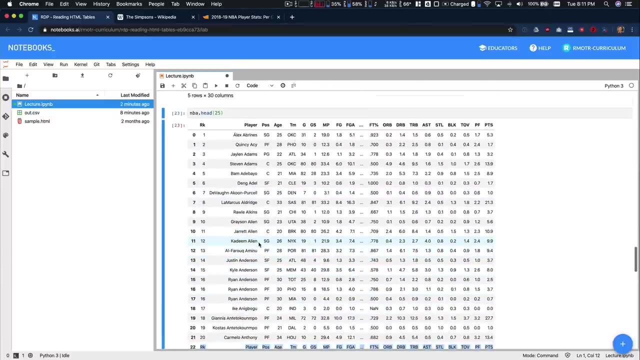 need to do something like D, f to drop. let's see, actually, if we can see it. I haven't tried this, But let's just do it. live dot head and you're going to find 25 records now. So here, record 22,. we find that header. So what we're going to do is you will need 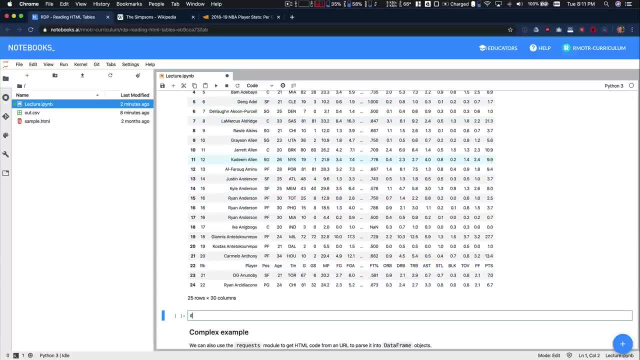 to do something like d, f the drop, the f dot drop range 22,, starting in to the top 12.. 22, up to the f, the shape, zero, right, these many rows plus one, plus one and every 20. 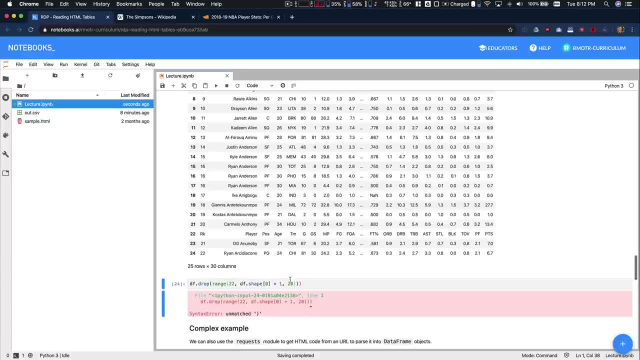 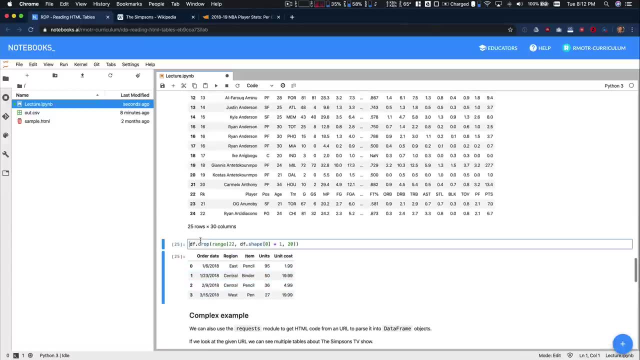 rows. I don't know this is gonna work. let's just run it. Oh didn't, it didn't even work, It didn't compile There. Oh, this is MBA actually. There you go, So maybe it works. 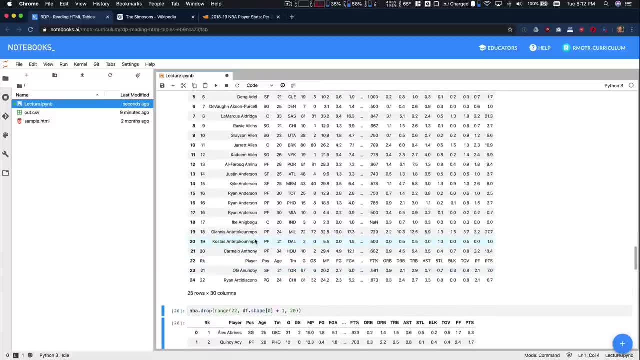 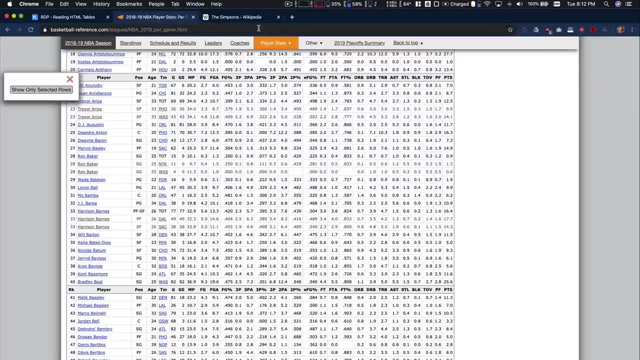 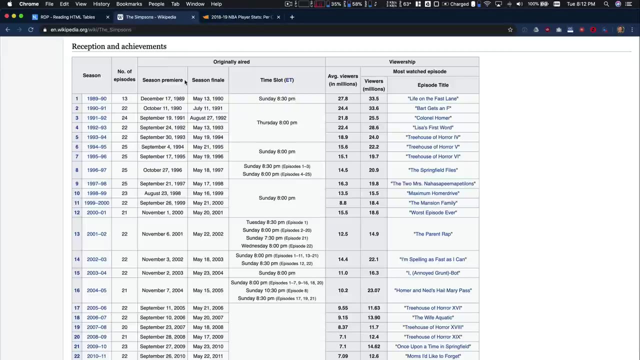 you can check it, But what I'm going to say is, again, there is some cleaning to do, because HTML pages are optimized for humans, not for machines, So usually it's going to take a little bit more time. The good news is that there is usually a service associated that 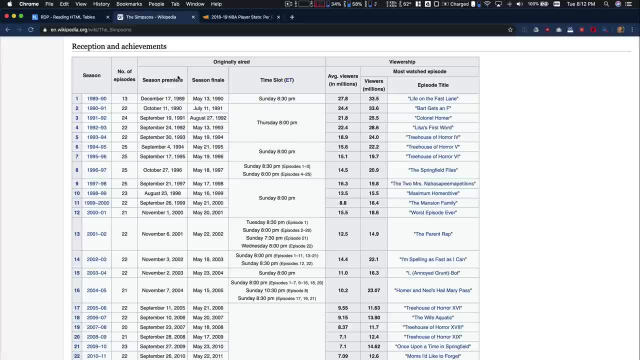 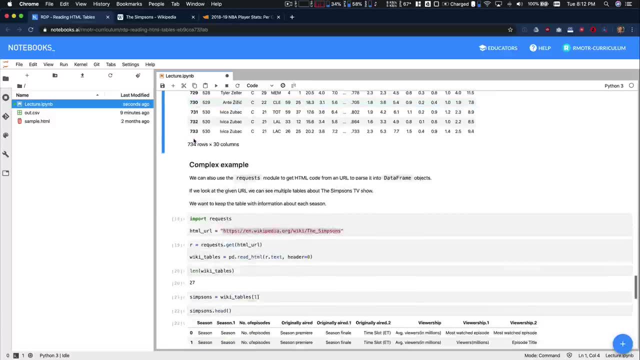 you can consult. So, for example, there is a Wikipedia API that you can use instead of a page, But again, sometimes it's just easier to pull the data directly from Wikipedia. Yeah, So that's it. you can also write data to CSVs, of course, or HTMLs. That's pretty much the. 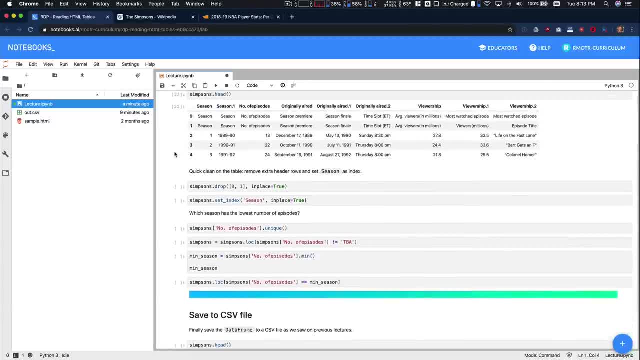 standard. As we've said, this is up all we had for the read data portion And we're going to move forward now with a few other methods, especially what we call data wrangling. we're going to do a little bit of grouping and keep moving forward with our tutorial. we 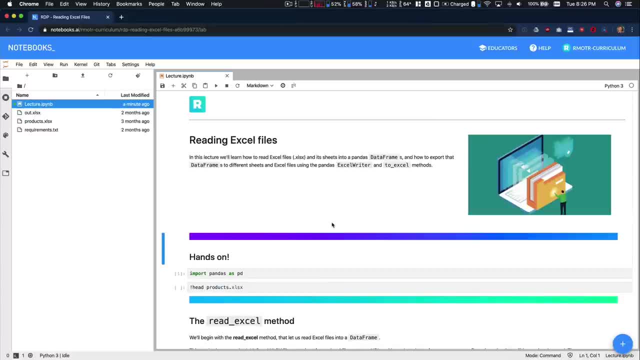 have decided kind of last minute to add a final source of external data, that it's going to be an Excel file. it's just a common Excel files. you know it because we imagine that you might come from an Excel background So you can just export the data you have in your Excel. 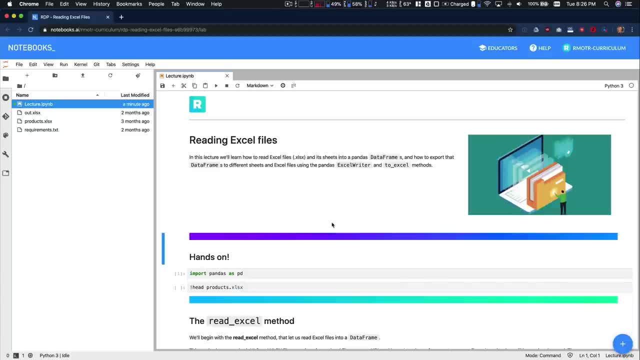 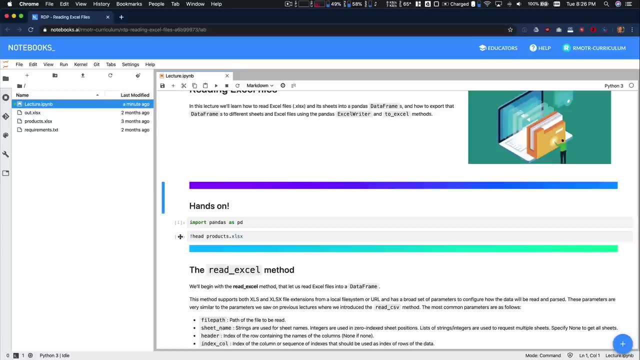 files, spreadsheets, and load them into Jupyter Notebook and start working with them with panless. So you can try things out and kind of draw the parallelism between Excel and what you do with pandas in Python. So the first thing is that an Excel file is not a 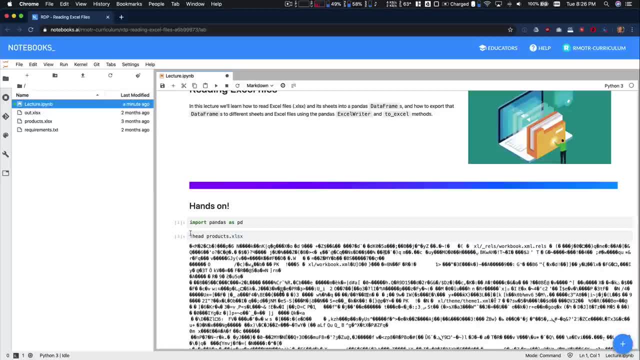 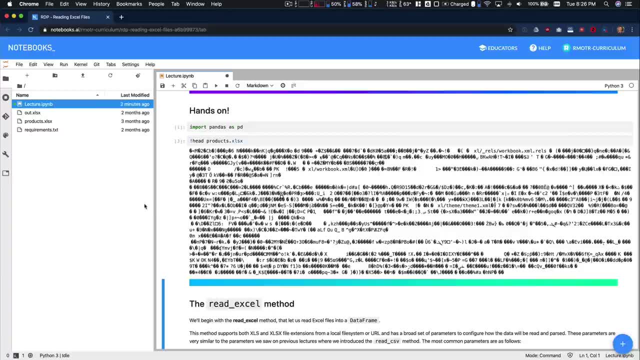 text file. So if you try getting the Excel file, it will not work. But if you try getting the content of it, It's not a text file. it's not so simple to parse it. So that's why it's going to require external tools, that they are already installed in notebooks- AI- they 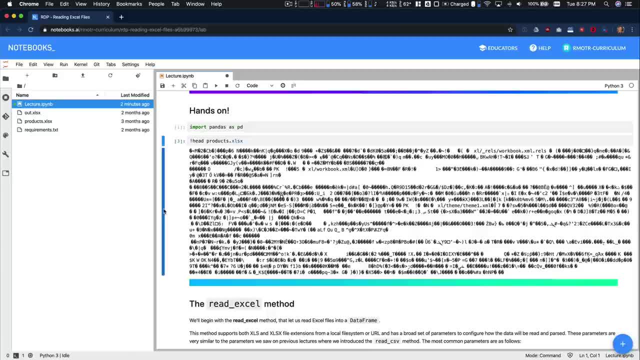 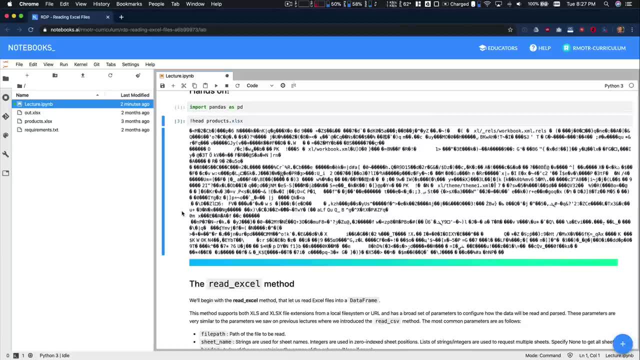 might be installing go up, but it depends on your computer how you're going to install it. So just keep in mind that there might be issues when importing data from Excel if the if there is low compatibility between the library you're using and the spreadsheet. 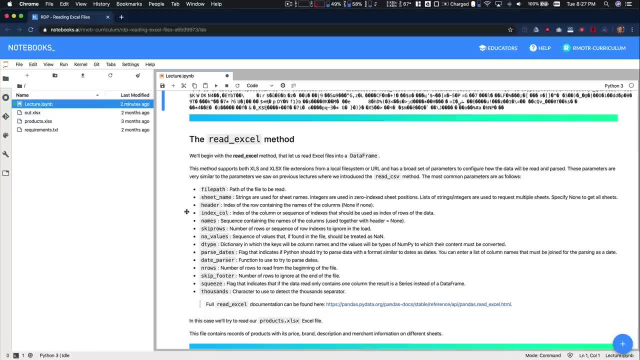 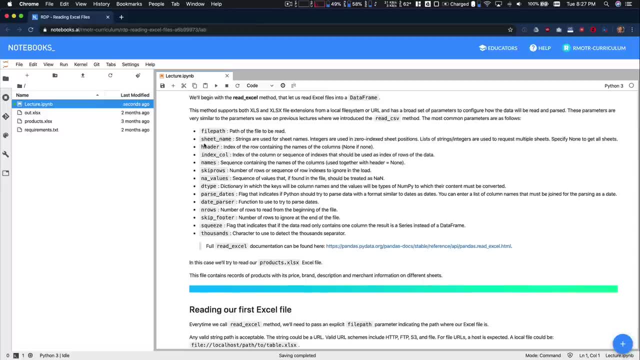 version you're using, But without those, without getting into those details, there is this read Excel method, which pretty much takes care of everything for you. has different parameters, like finding the, the sheet that you're reading from, of course, a path, etc. So we're going. 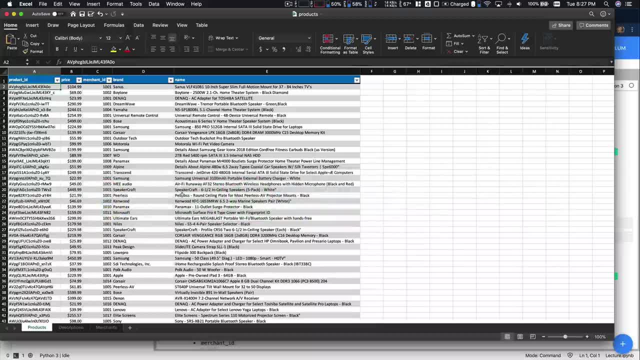 to start reading these file, which is products file, that has three sheets: products descriptions and merchants, And it's actually something we use in an Excel file, to sorry, in our data analysis. from Excel to pandas course to show how to merge data and all that And from the 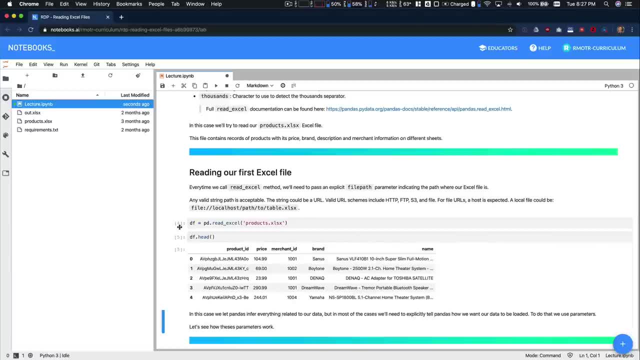 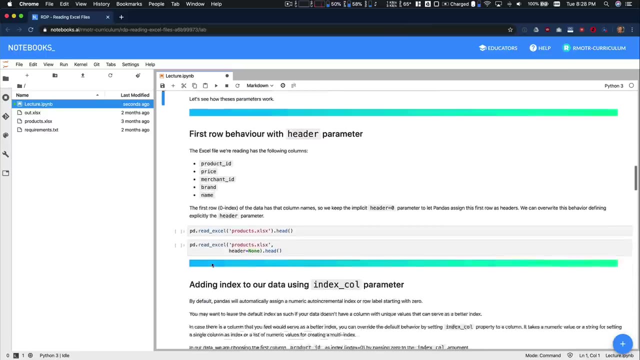 from this file. what we're going to do is just read Excel, And what you're going to see is that it reads the first sheet of the Excel file. I mean, a data from is just corresponds to one sheet, only, right, And the first one is product. So that's what we are writing. 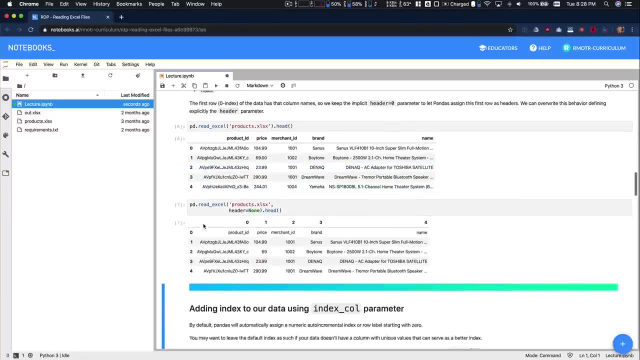 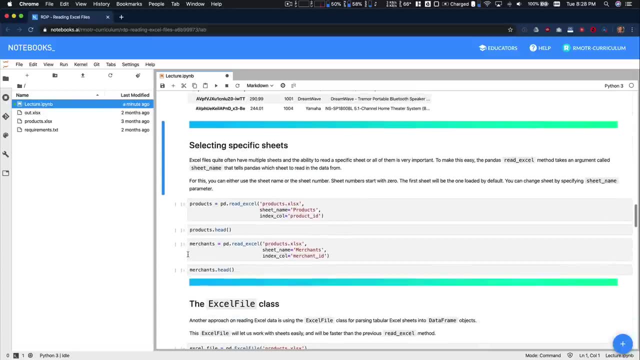 There are different behaviors for it. you can change the way you parse, heathers, etc. you know it already. defining and specific index, that's pretty much everything we have. Okay, We have seen so far. it's selecting specific sheets is simple, just pass the sheet name. 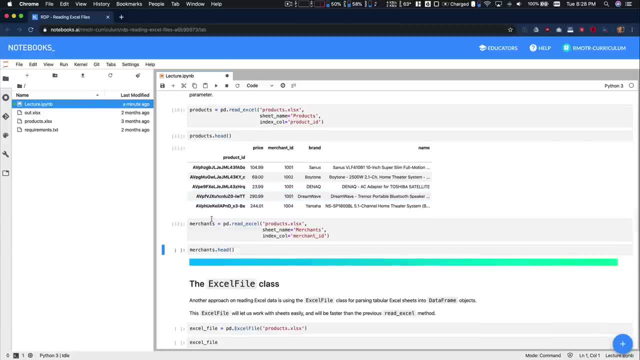 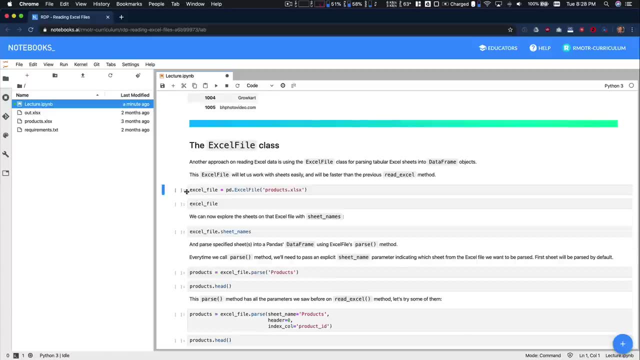 And you can read: sorry, either products, merchants, whatever sheet is available in the current Excel file. There is another format or a specific class that it's a little bit more advanced, that it's the Excel file class, So it's not as we were doing here. read Excel directly. 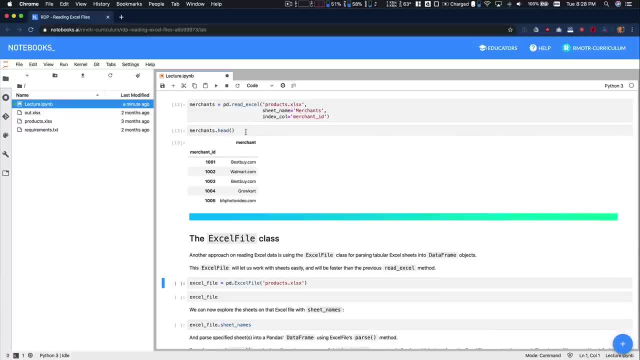 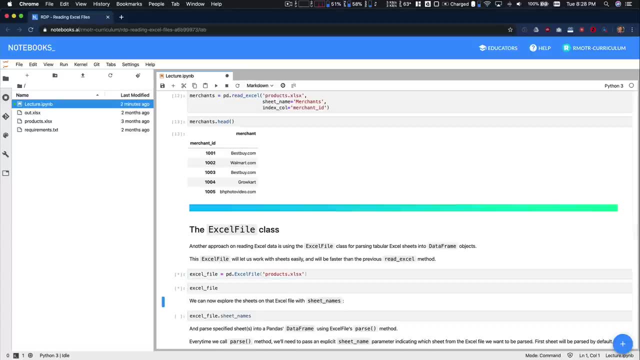 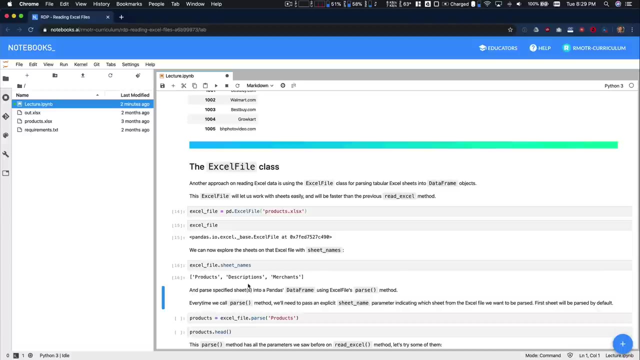 is going to read that Excel file into a data frame, but you're going to instantiate this Excel file class with the parameter being the file name. And now these files can have just a reference of everything you have In this case we can do, for example, sheet names. it's gonna tell you have products. 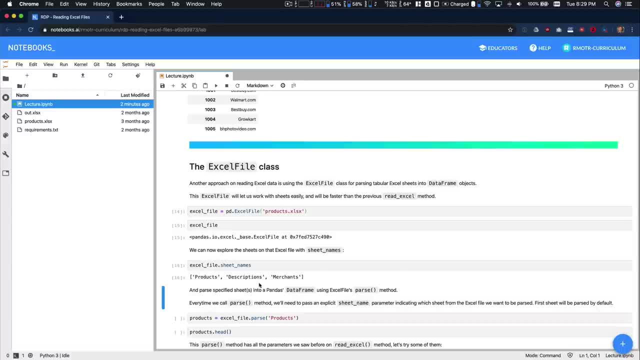 descriptions, merchants. this is a little bit more of a explanatory data analysis. So let's say you can't use Excel to actually see the contents of the Excel file. this is going to be helpful. you're going to first parse the Excel file, get the sheet names. 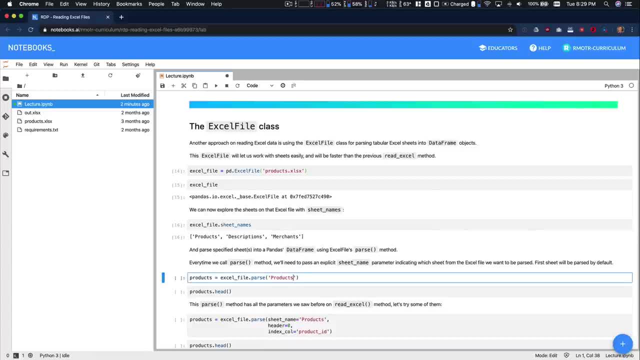 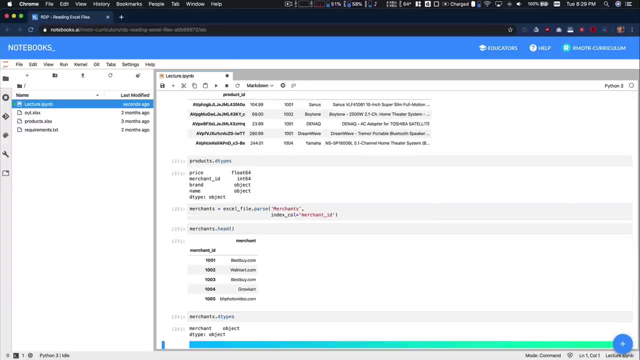 and a little bit more understanding of it. And now we can say from this file we have previously parsed, it's right here, or instantiated. we can parse the product, the product sheet, and that's going to get you that data frame. And the same thing is going to happen with all, all the parameters. 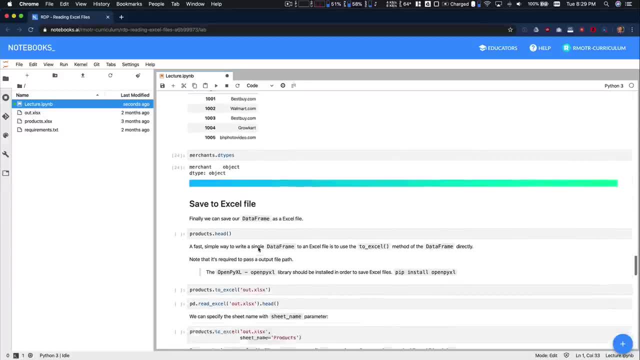 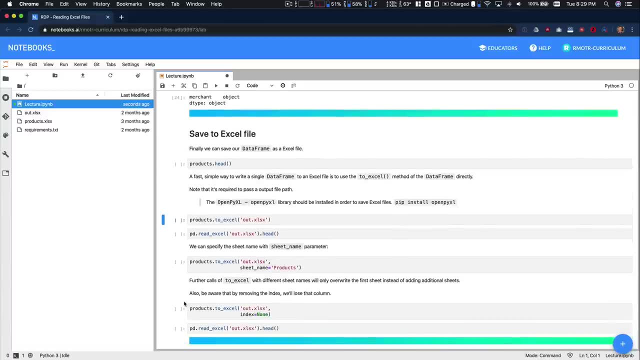 we can pass. they are the same as read Excel. Finally, you can see that there is also two Excel file And it works pretty much in the same way as to CSV, you know, decide if you pass an index or not, And also you can define if you're going to pass a sheet name or not. 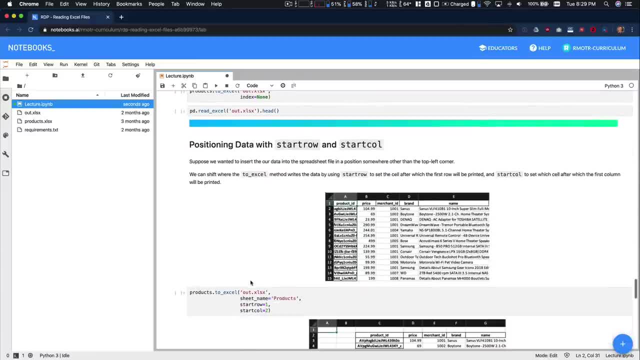 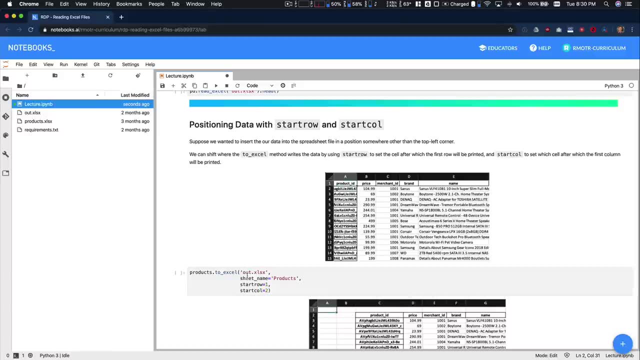 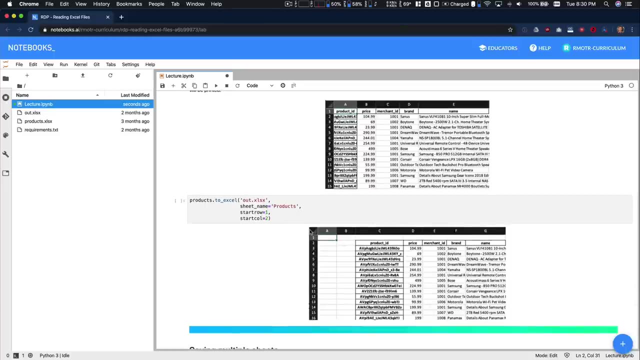 or just going to be the default one. So, as you can see, getting your data into from an Excel file into CSV data frame- sorry- is extremely simple. There are more customizations to do. let's say all your file is shifted right. either rows or columns you can change. 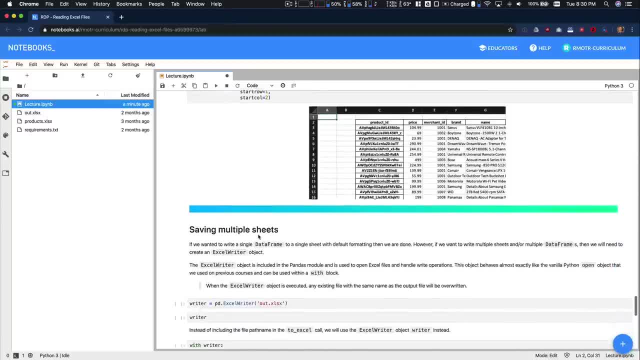 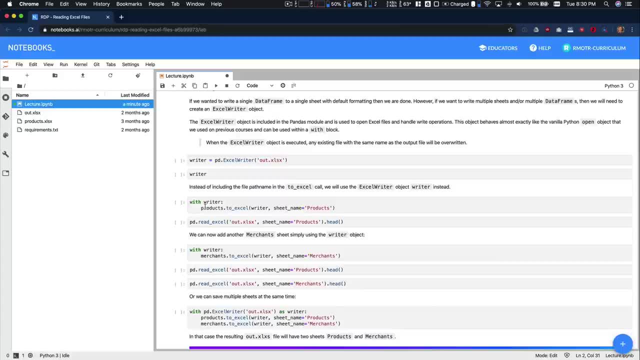 that with star row or style column. that's going to work too. So that's pretty much a. The only thing we need if you're writing process is a little bit more complicated, like, for example, you want to write specific sheets, you know multi sheets Excel file. 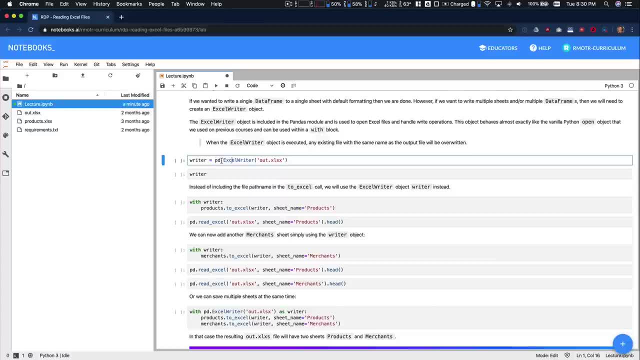 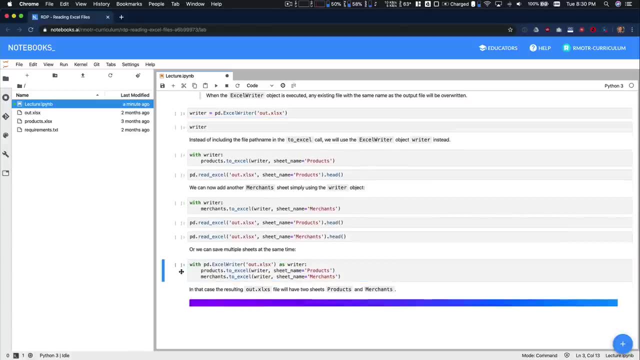 you can use what we call an Excel writer, And it's also part of pen, so you instantiate the writer and then you can start to write process, saying which sheets you want to write with each one of those data frames. So again, reading and writing data from and to Excel. 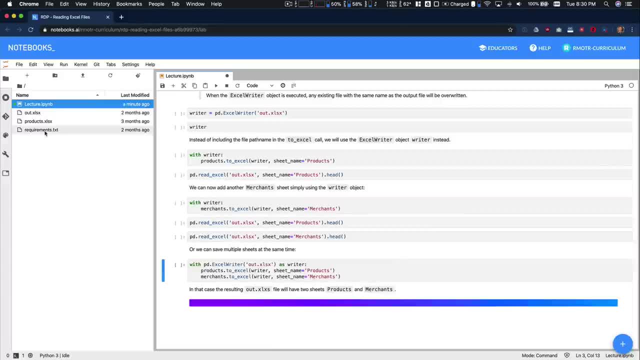 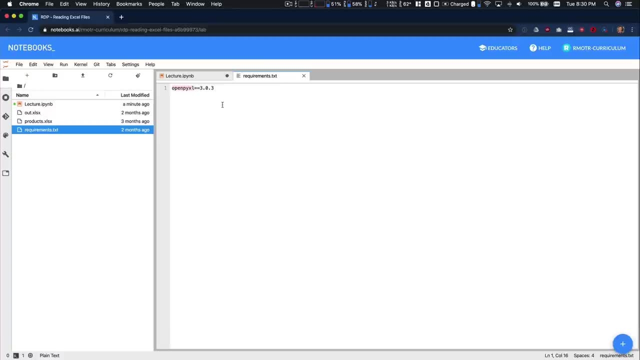 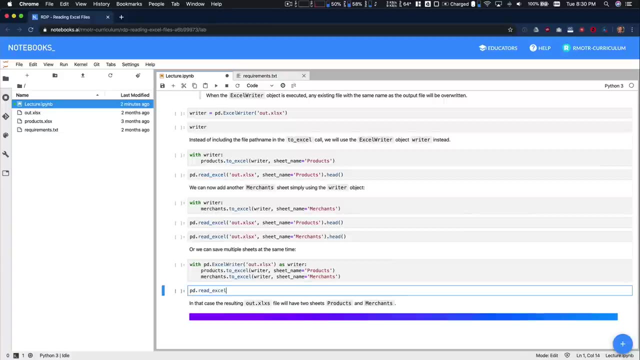 files is relatively simple. It all depends on the libraries are installed. it depends on on what libraries you have in your current environment, if it's Windows or if it's a Linux slash slash Mac. the documentation of PD dot read Excel might have more details. 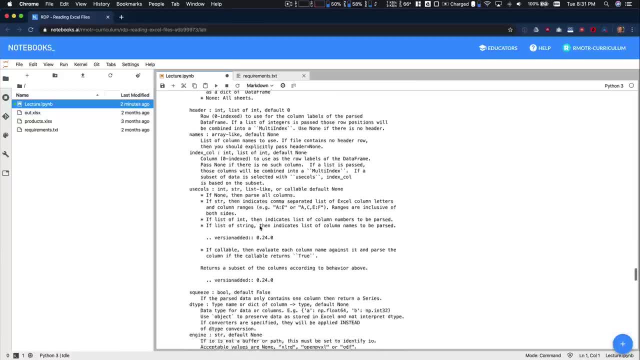 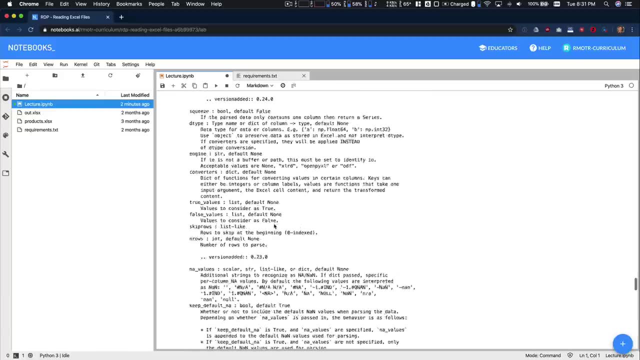 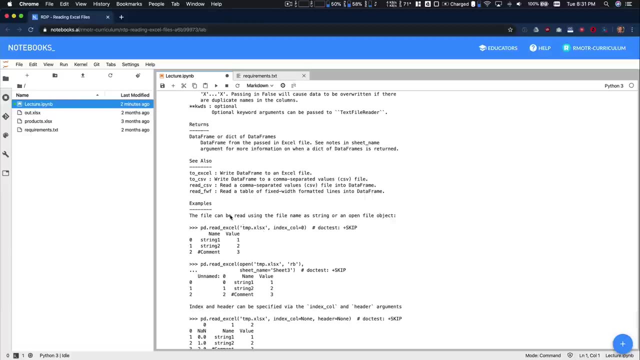 for the given platform that you have. So let's see If it names per document. if it's not here it's going to be in the panels documentation, But there might be requirements for each one of the platforms that pandas is supported. 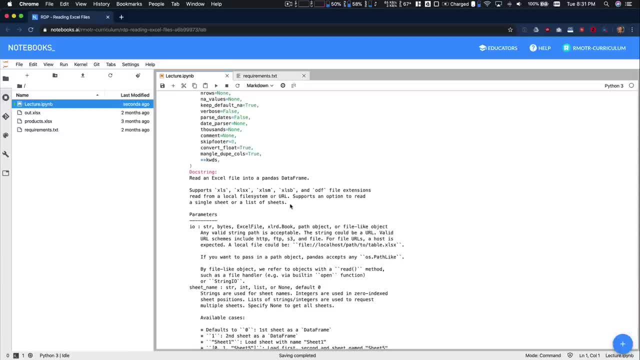 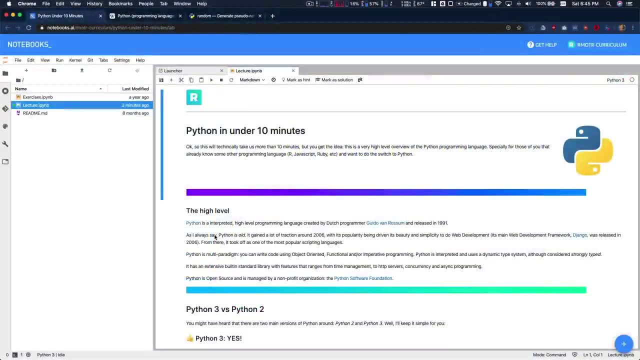 So just check it out. Check for your own, for your own platform- if you're in Windows, Mac, Linux- how to get those libraries installed. So, in case you're just getting started with Python and you might come from another language, 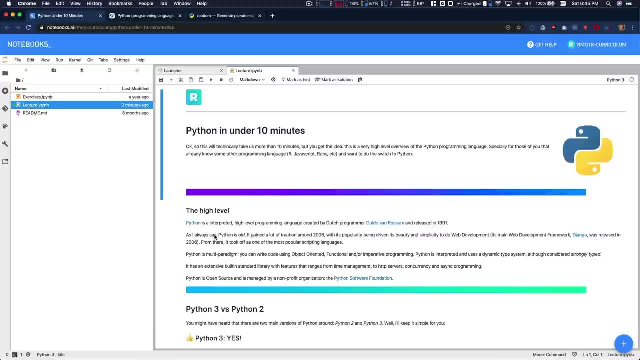 the objective of this video is to show you how to get those libraries installed. Now of this quick section is to show you Python, Ideally in under 10 minutes. I think it's going to take a little bit more, But there's a very, very, very quick reference of Python. 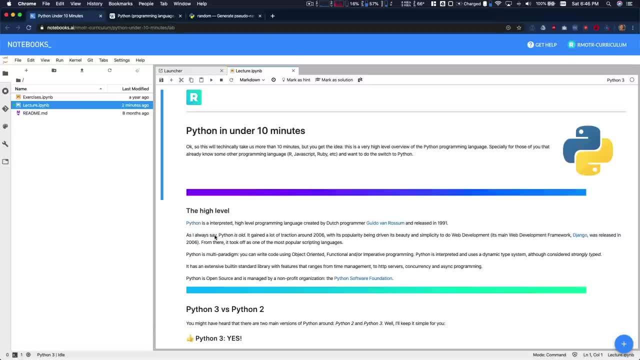 again, just the high level features of the language, how to use it, how to code functions, how to import modules, variables, data types, collections, etc. You can just scroll through this notebook if you want to take less time. I will be providing explanations on top of. 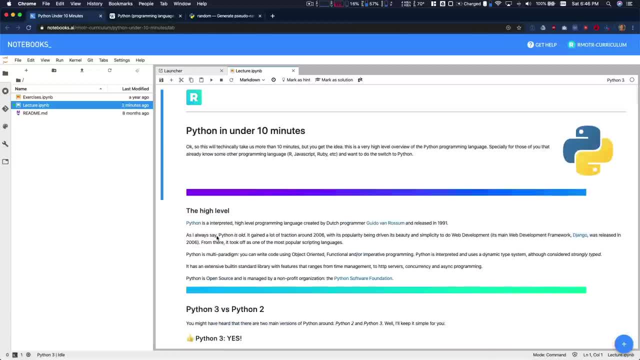 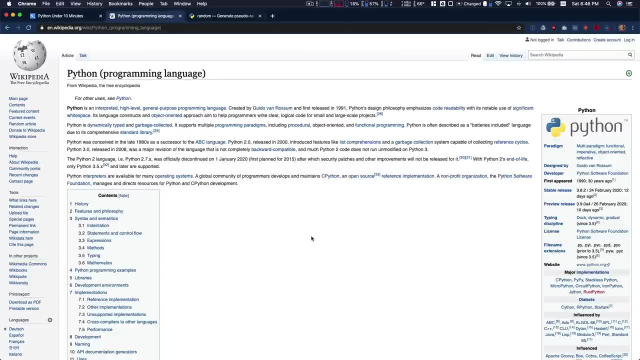 all the topics, But there's a very good reference of the entire language. So, to get things started, Python is an old language period. It has caught it has caught more attention in the past five to 10 years, But it's a very old language. It's even older than Java. It's up here in 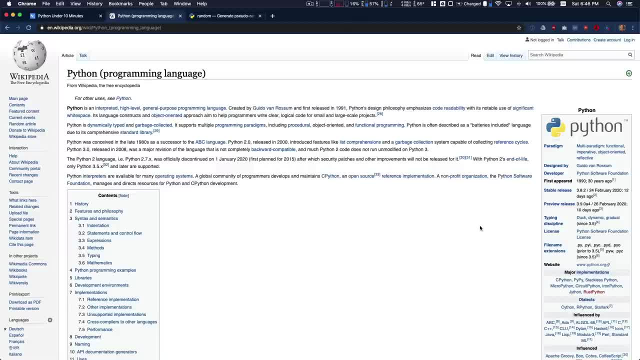 1990s And it was created by this person. get away with Gita van Rossum- And it's an important actor in our X ecosystem. He's used to be- I think he's still the one deciding discussions, etc. When it. 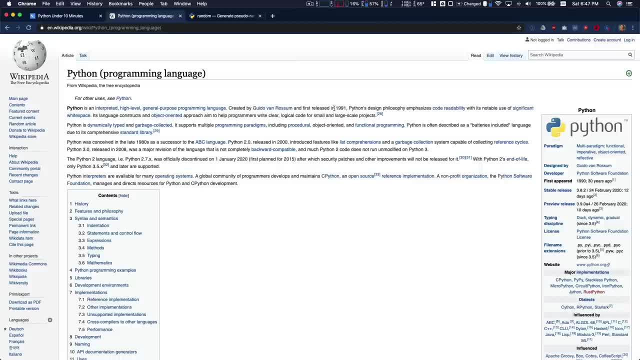 comes to defining features of the language, etc. Python is a high level interpreter, dynamic language, And this means a ton. Actually, if we read this entire sentence, interpreted: high level, general purpose, this is basically high level programming language. it's object. 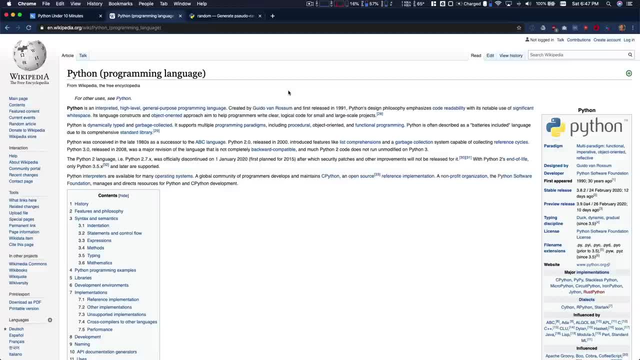 oriented And it's also includes functional attributes or functional features, like functions as first class objects etc. And it also, of course, it supports imperative programming And it has a wide variety of applications. you can do web development with Python. you can do scripting. it's a lot used. 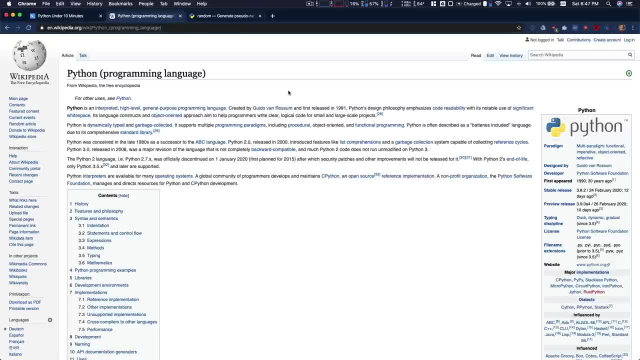 for system development, for configuring machines in in general, And of course you can also do data science. So it has multiple applications. it has a couple of features. For example, it has a couple of interesting features like indentation for defining blocks, etc. that 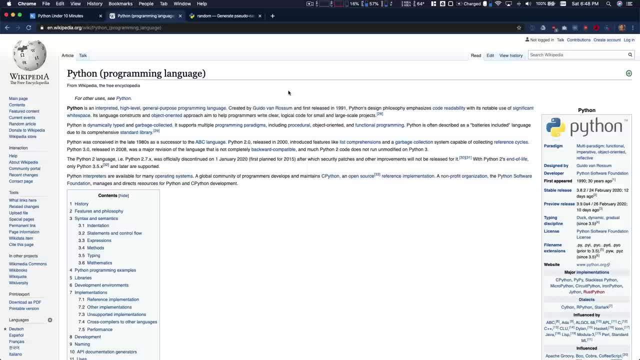 make it, and in a very good language, to get started with programming. So if Python is your first language, you should be comfortable with it. It's a very good idea. For me, it wasn't my first language And I hope it was- It wasn't- But I have taught people programming. 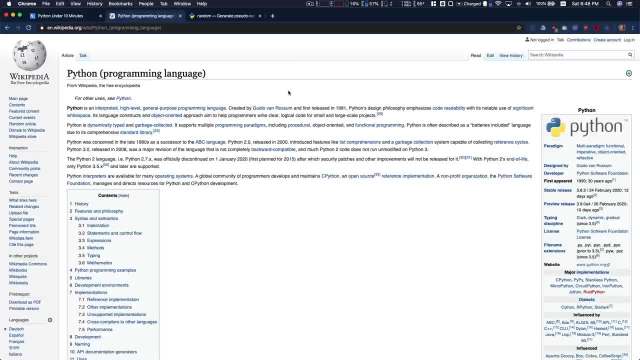 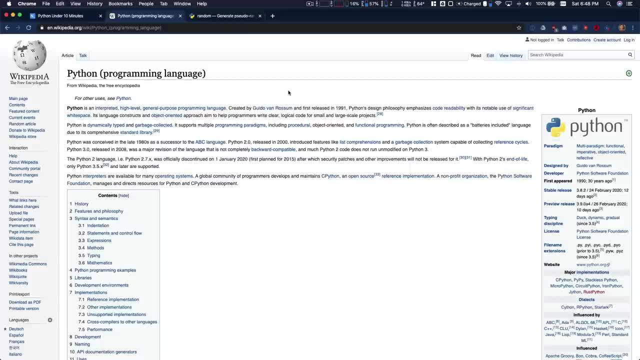 And I hope you can use it. I think it's been very good for them because Python doesn't have weird things like my having JavaScript or Java, So it's a very concise language and consistent language, to be honest. So let's get started very quickly. First of all, when 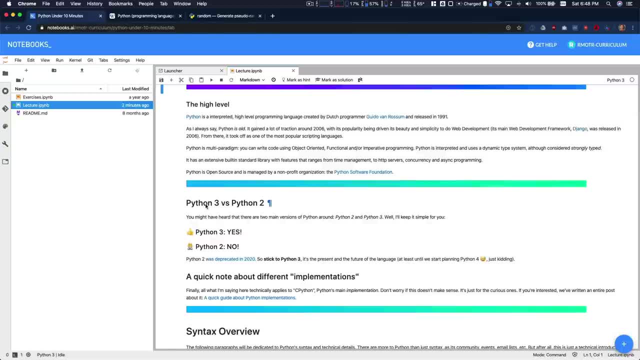 you're going to install Python your own computer or you can use notebooks, Ai or Google call up. But if you're installing in Europe your own computer, you might see that you can install either Python two or Python three, reading tutorials online, etc. you might see Python two and Python three. the reality is: 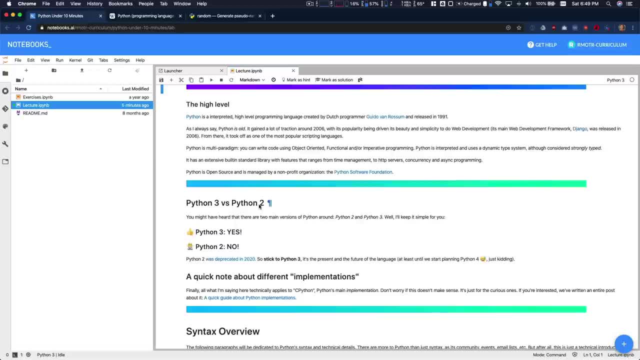 that Python two was deprecated in 2020.. So the you cannot, you should not use it anymore. there are still ways to install Python two, but it was deprecated, So you shouldn't use Python two. you should stick with Python three, which is the evolution of the language has. 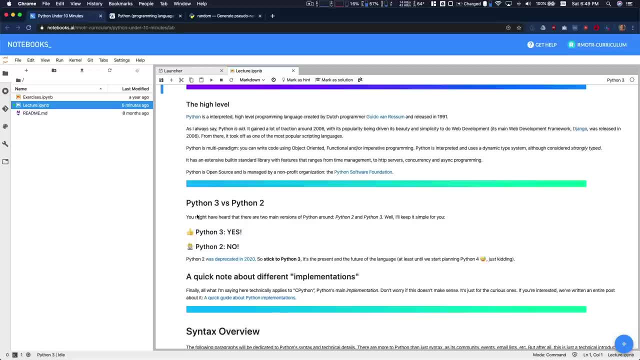 a ton of fixes from Python two that they were weird. things happen in the language and used to confuse beginners. So that's no longer a problem. Python three again is what you should use. you will read in multiple tutorials etc what that they are using Python two. 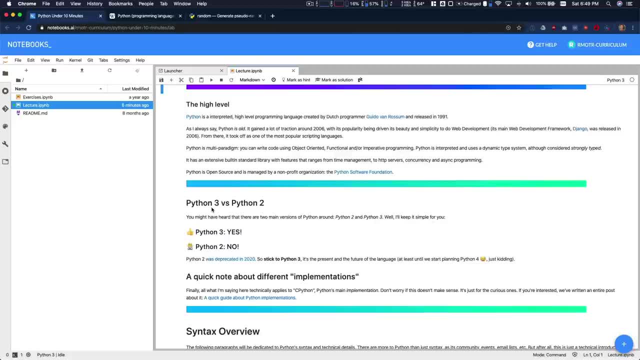 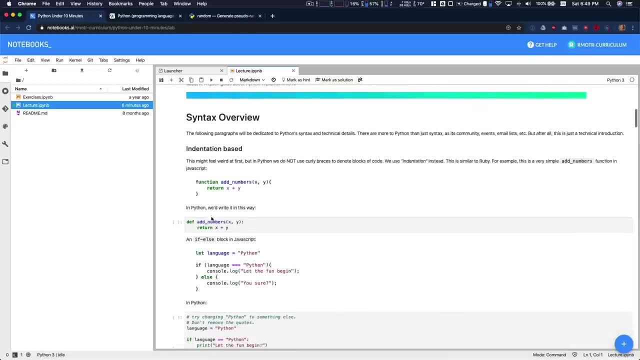 you should try using Python three, and sometimes the code will break, But the changes to fix it are not very hard. So to get things started here, I will be drawing the parallelism with regular syntaxes. For example, this is the way you will define a: 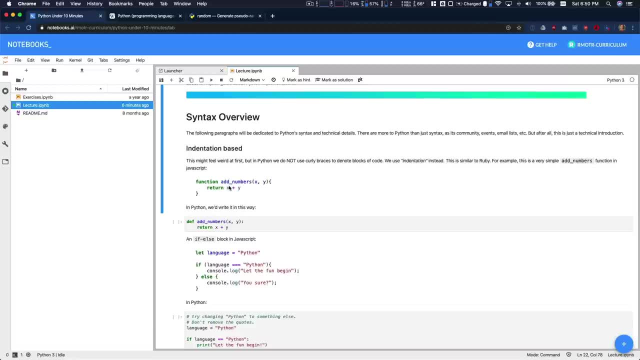 function in, for example, JavaScript And it's also very similar to something like C or Java based languages. the function keyword curly braces, etc. So I will be drawing a parallelism with these sort of languages So to get things sorted out, the way to define. 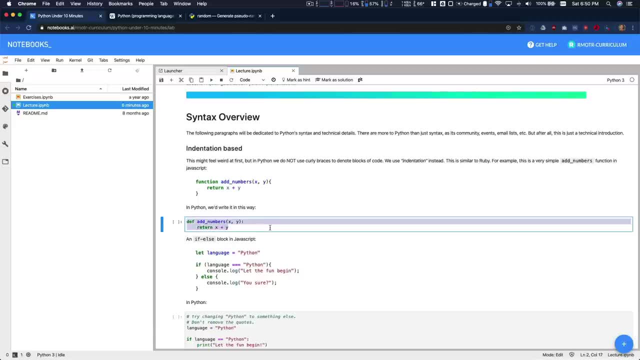 a function in Python is in this way, And the main characteristic of this language is that the way we're going to define blocks is by using different indentation levels, So this is a valid function. in Python, def is a key where we use the name of the function. 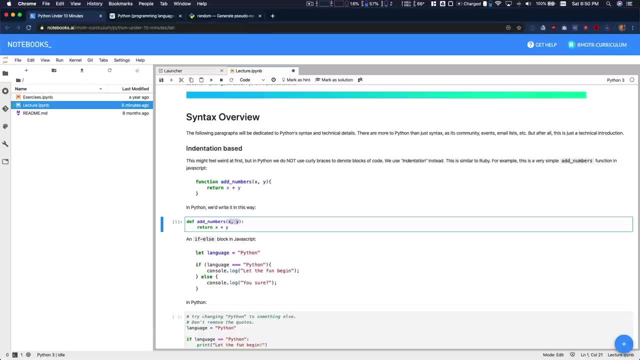 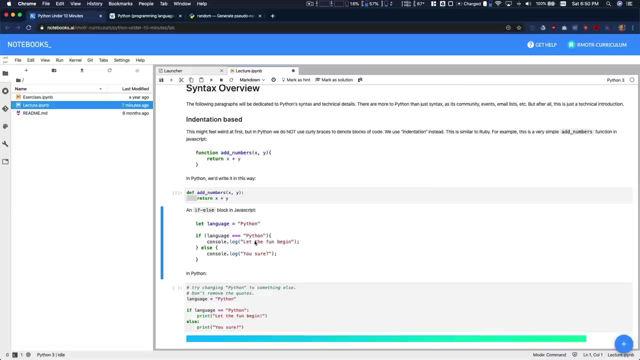 the parameters it receives. And the way to define the body of the function is by just indenting everything one level to the right. Usually this is just force basis And another, for example, is an if else statement. So if this thing happens, 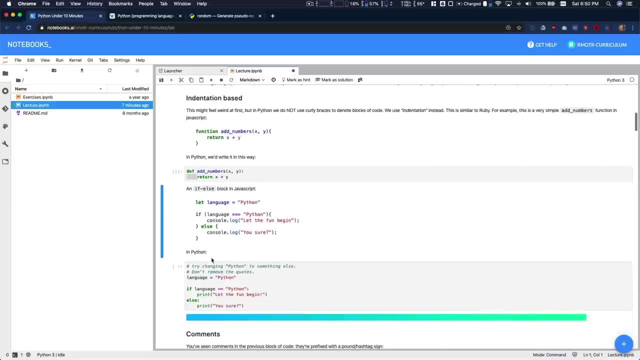 do that. if else, do something else. right is JavaScript In Python, again, it's defined by indentation. If this thing happens, we indent one level to the right. do this, else, do something else. If there was another if statement here, if I don't know language. 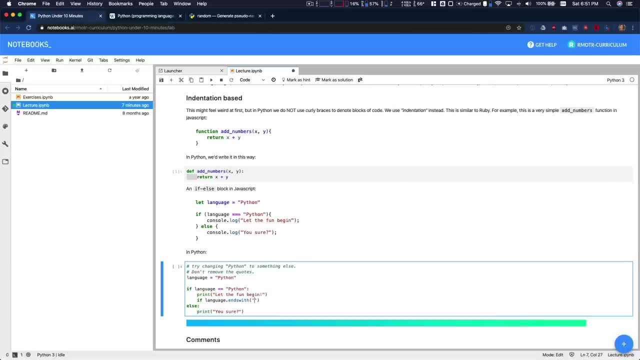 ends with something like I don't know three. then do something else. print pi three, for example. So we're indenting everything to the right. every time we start a new block, whenever the block finishes, it's just when. 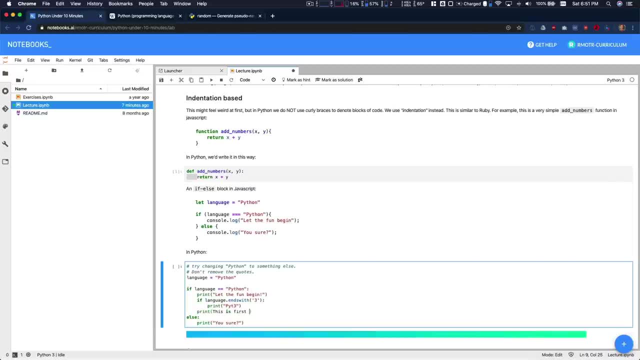 you go back again print. this is first block. right, That's the way it's going to work, by indenting our blocks. This is very good because first we don't have debates of where we should place the curly braces And also because it makes it a lot more readable. 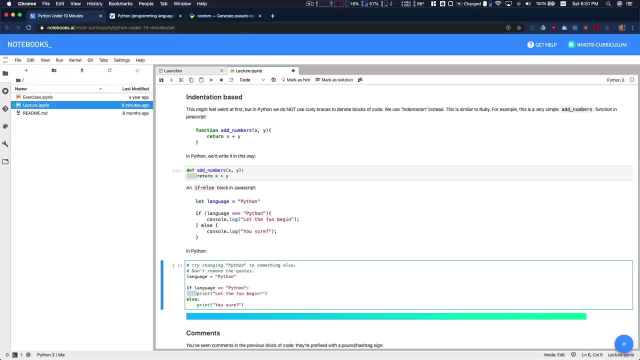 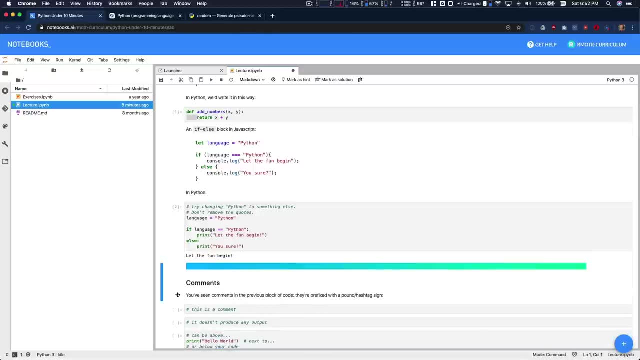 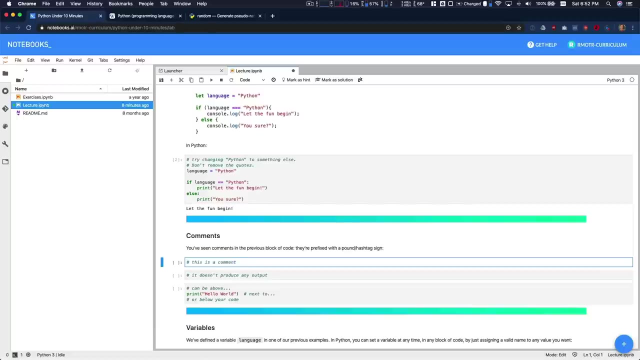 it's a lot easier to read these code because there is obligated, obligatory indentation to even make the code work. So, as you can see, that's that's just how it works, How we're going to make comments in Python, just by using the number, the path symbol, there. 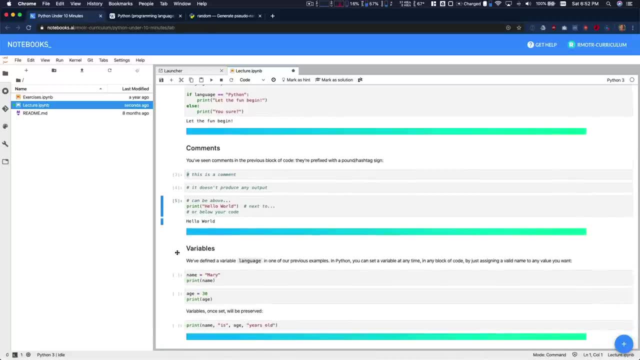 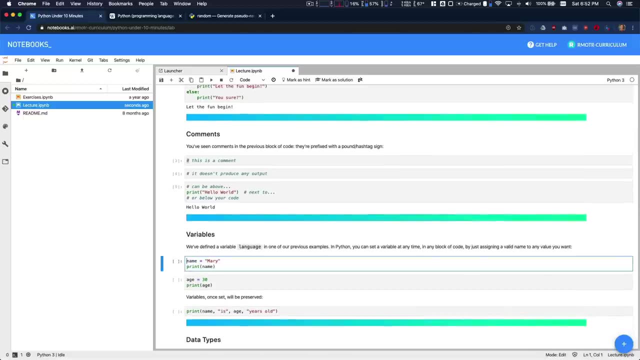 we go And the. the way to define variables is just by specifying the name. So it. Python is a language that you don't need to declare variables. you just declare and define everything in just one pass. you know, you find a variable as it goes. Python is dynamically, dynamically typed. 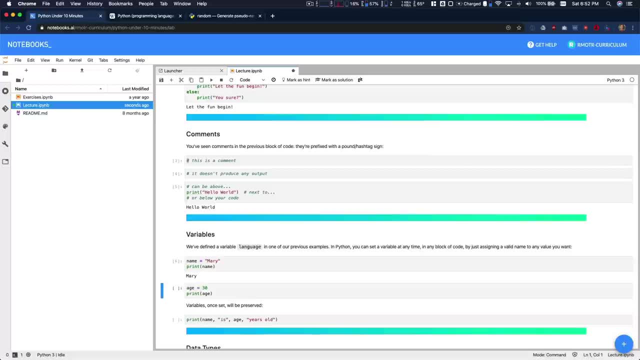 but it's also strongly typed And these might kind of cause confusions. But basically you can assign variables to any value you want And you will see that collections etc are heterogeneous in terms of types. etc is a very dynamic language. Talking about types, I'm going to show you the most important types. 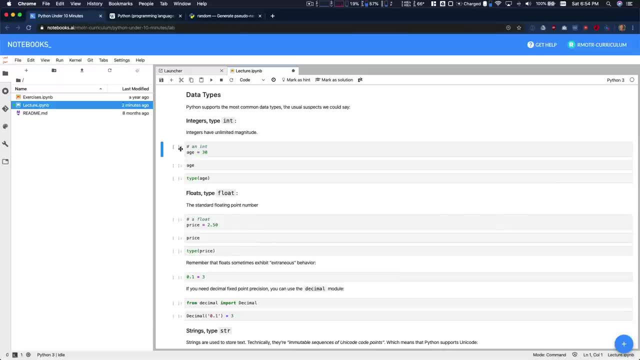 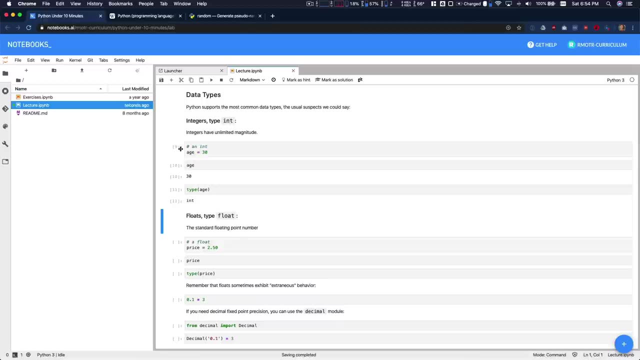 that we have in Python especially. we have numbers, of course, integers. we don't have so many like like you might find other languages like different precision sets, or we have integers. there is also the concept of longs. that has changed with Python to, to be honest, 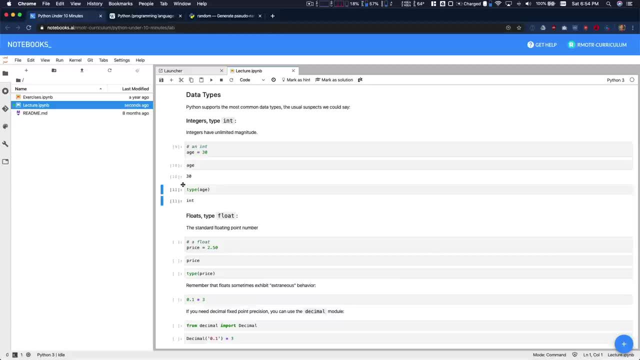 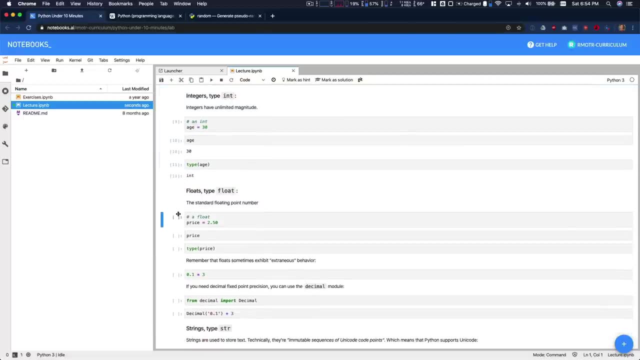 and Python three. to be honest, We use just integers. That's the way we work. It's a. it's a smart enough type to save storage when needed, So that's that's good. And we also have floats right, which is the regular. 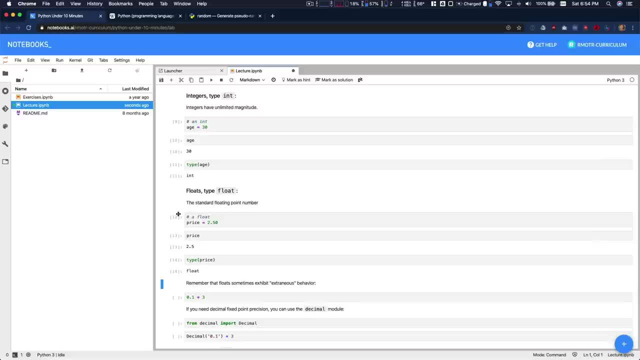 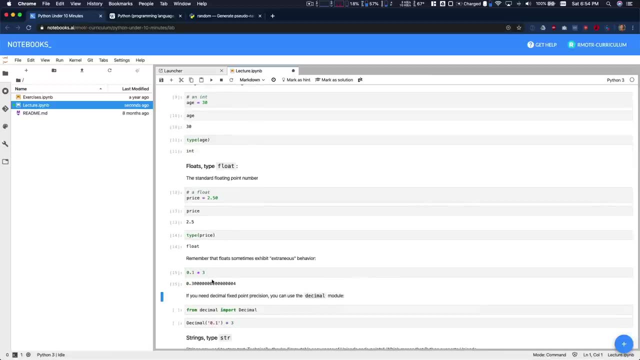 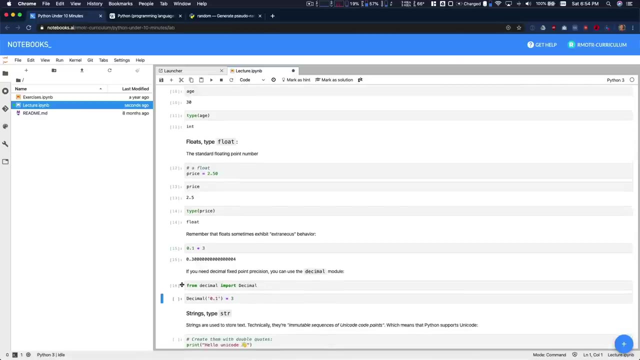 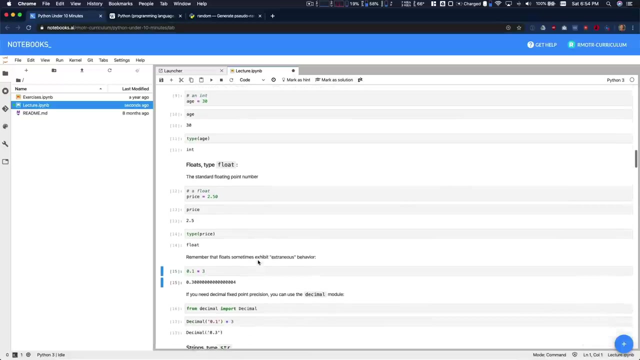 float type for floating point arithmetic in other languages And of course it suffers, if you want, from strange behavior from floating floating point arithmetic, like in this case. you can prevent that by using the decimal module Which, as you can see, doesn't suffer from from these issues. So numbers, we have integers. 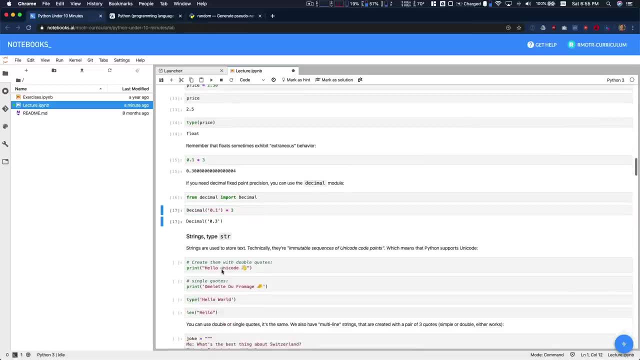 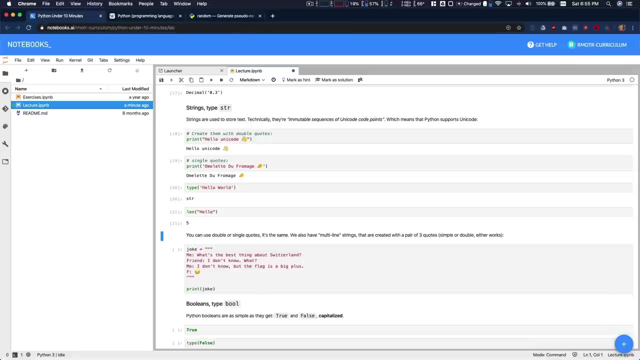 floats and we also have decimals. Strings are just the type STR and they are defined literal, right as in this, as you can see, right here you can just type the string as it goes. There is a difference between- there was a difference, sorry, in Python two between: 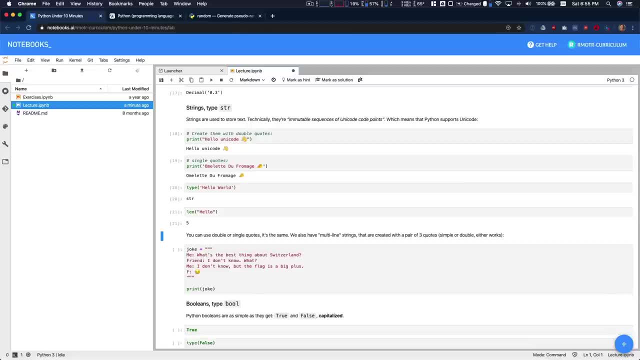 Unicode and strings, etc. In Python three This has all been fixed. So in Python three this is all Unicode And there is the concept, or the difference in terms of the concept, of something being the type the Unicode code points as it's. this string and the underlying encoding will turn it into binary. So in Python, 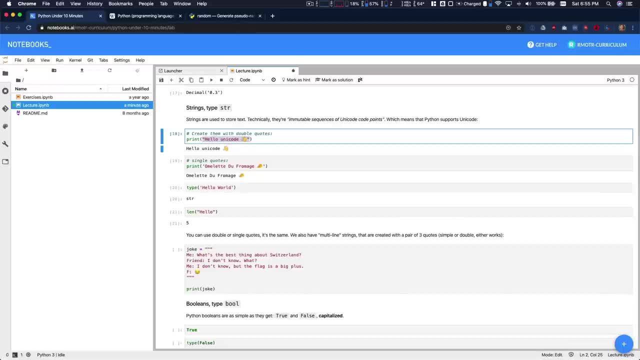 three still had. we have a few ways to differentiate between what it's a binary string or what it's a text based string, For you shouldn't worry about it, I just want you to know. if you're reading a Python two tutorial, for example, you might find the difference between Unicode strings and 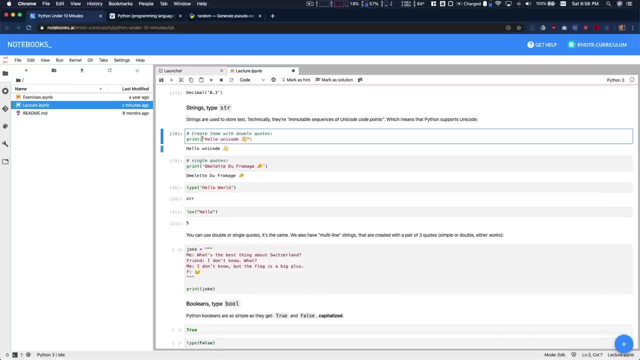 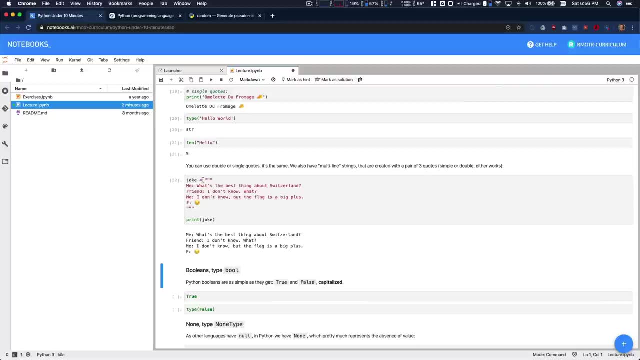 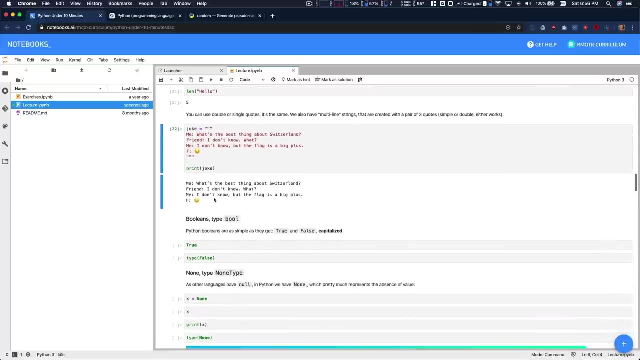 regular strings, which is is no longer something that we should be worrying about. If you have a string that it's too long and it expands multiple lines, you can always write it using three quotes. can be double quotes or single or single quotes. So just to create a multi-line. 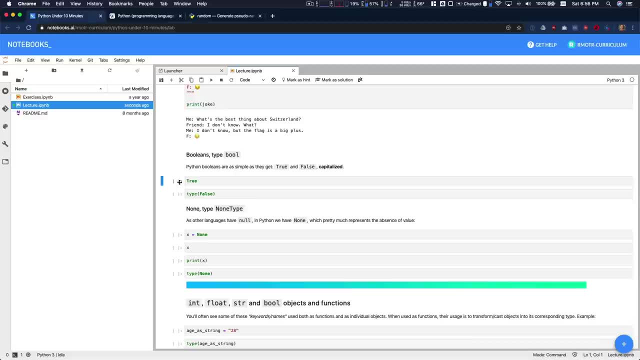 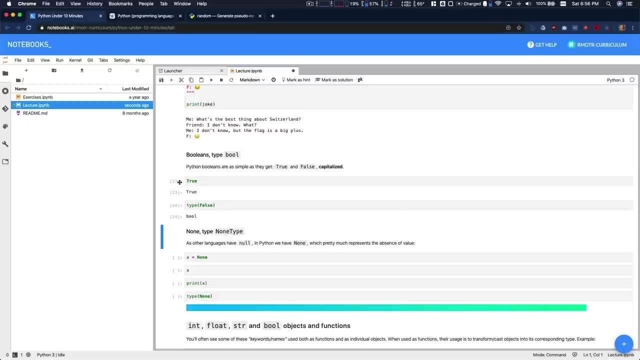 strings is extremely simple: booleans. There are two boolean type do. boolean objects are unique, right, It's kind of a singleton, which is the true or false objects, for example, and they are of type bull. There is also the concept of no in Python, which is none. we 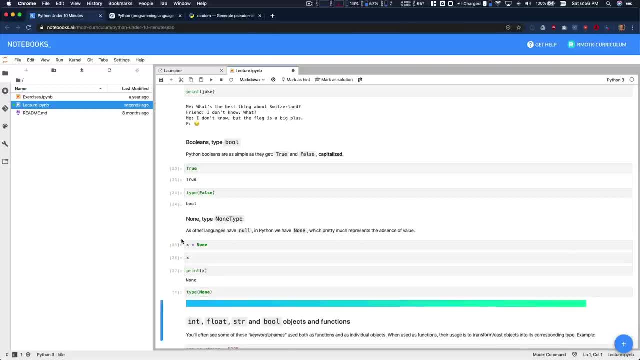 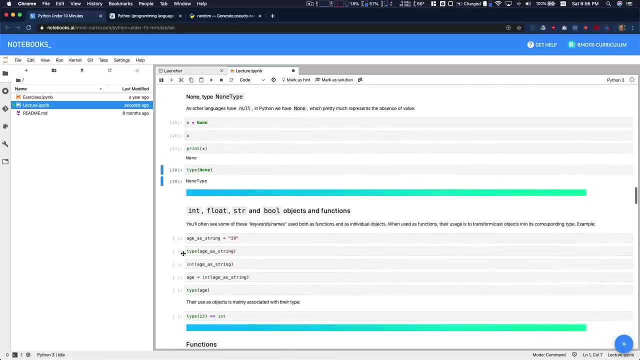 don't have. no, we have none. but it serves pretty much the same purpose. In Python, everything is an object, So even this exchange, strange objects like none will have an associated class, if you want. everything in Python is an object, So all these types of we find you. 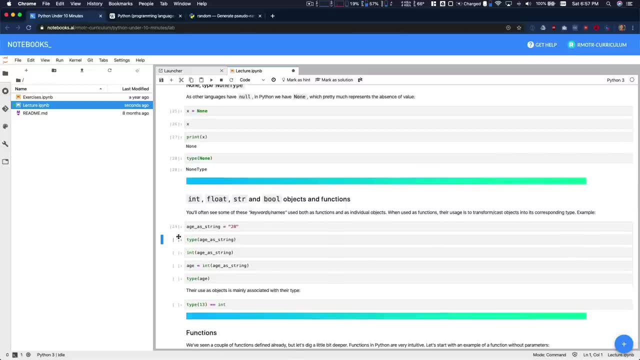 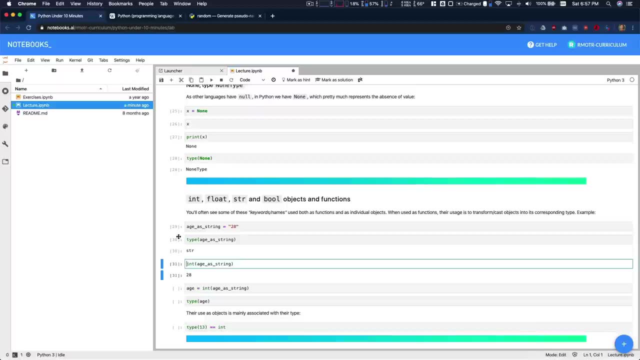 have seen. so, for example, we have this string, which is h of string, the type is STR. you can use the int str, float, bool types, right, but it's the result of the type also as function. So in order to cast, in this case, 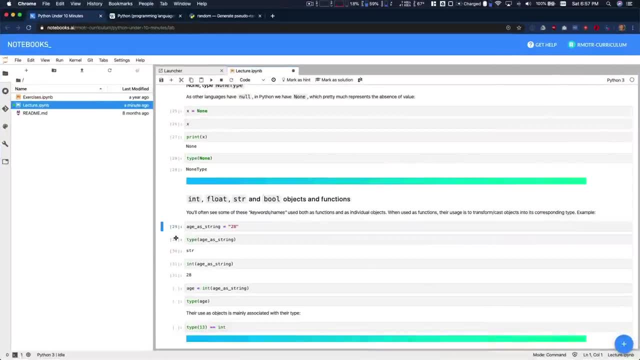 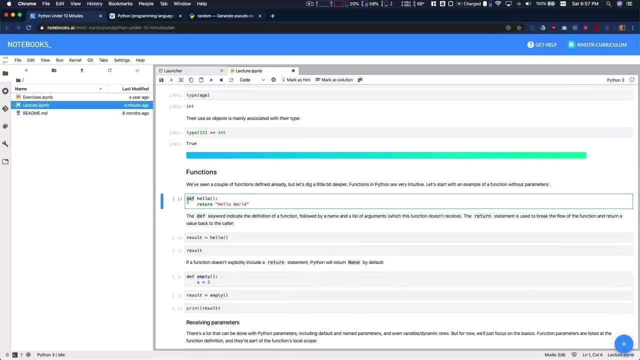 a string into. in order to cast a string into an integer, you will use it. you will do it using the int function, which is the same thing that you get with these, for example. So this is the same as this, as you can see, what we have just shown. So functions again. 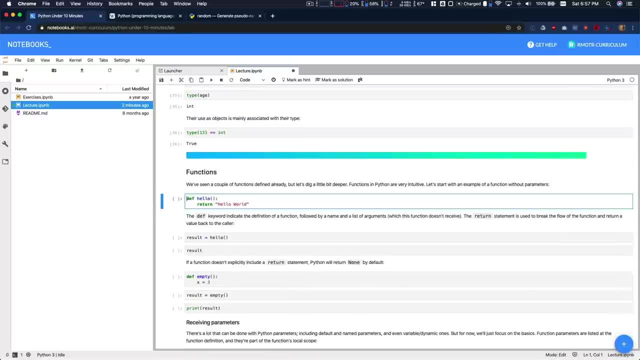 death is the key word we use. we don't use function, we use death. I you can use. define as a mnemonic the name of the function. parameters are optional and finally, have the return keyword. you should always include a return. you usually 99% of the time your function. 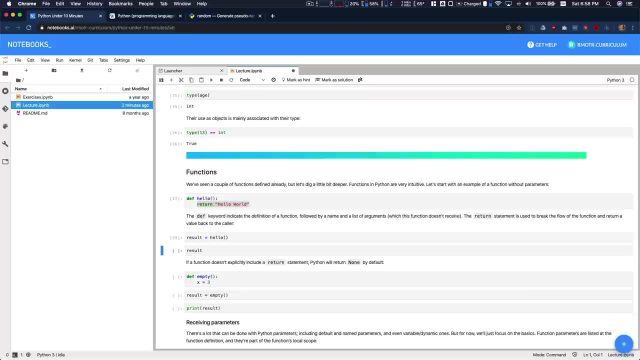 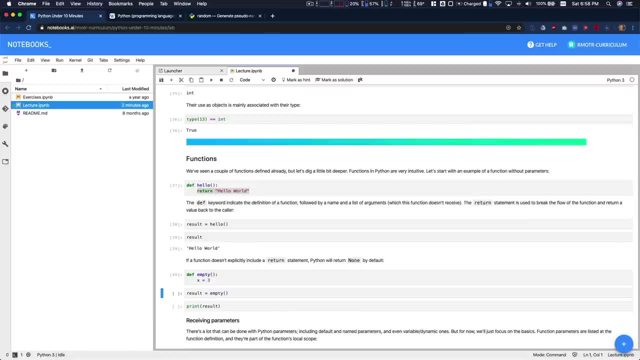 should return something, Because that's going to be the result assigned once we invoke the function. just this is pretty regular: If your function doesn't return anything explicitly, if that means if you haven't written down a return statement anywhere in your function. 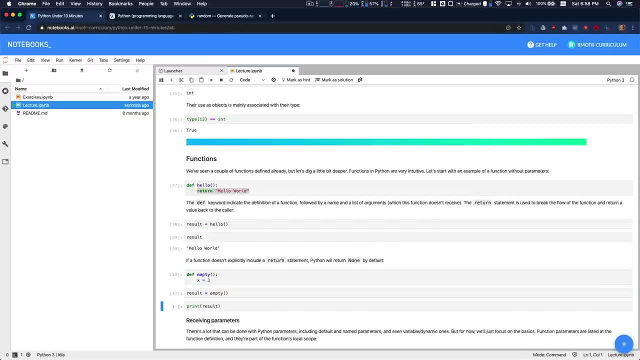 the function will still return something, so that the the fact that you haven't included a return statement explicitly doesn't mean that the function is not returning anything implicitly, And actually it is returning something. it's returning none, right? So, by default, if you don't include a return, Python will do this, just for you to know. 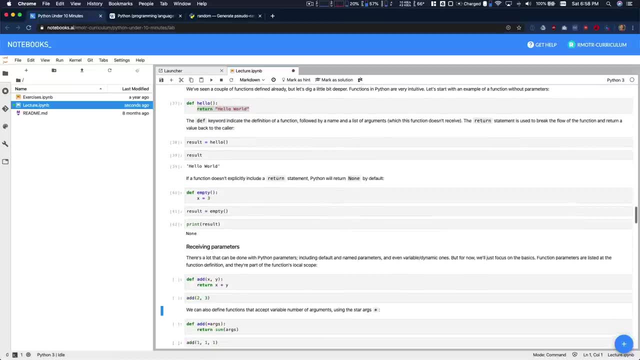 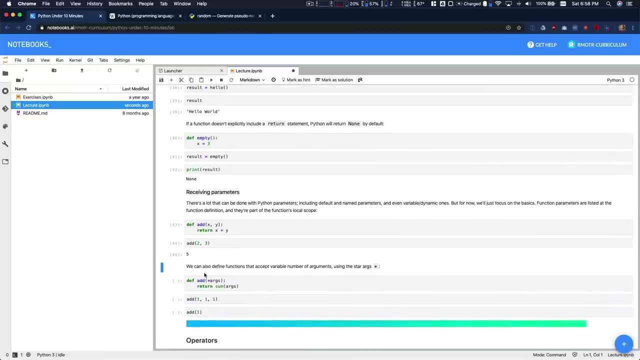 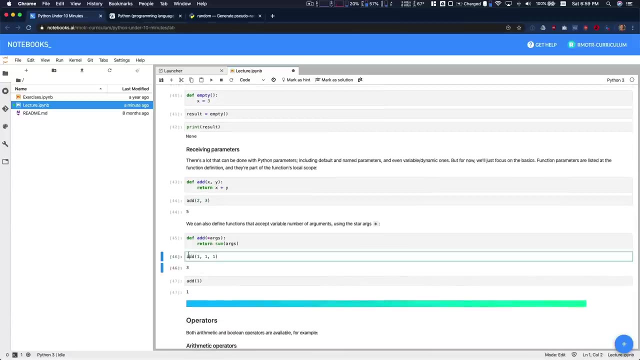 a function always returns something. Specifying parameters and passing parameters is pretty standard. Python has some advanced features with parameters like, for example, variable length arguments. we can pass as many arguments we want to make it very dynamic- keyword arguments, named arguments, etc. 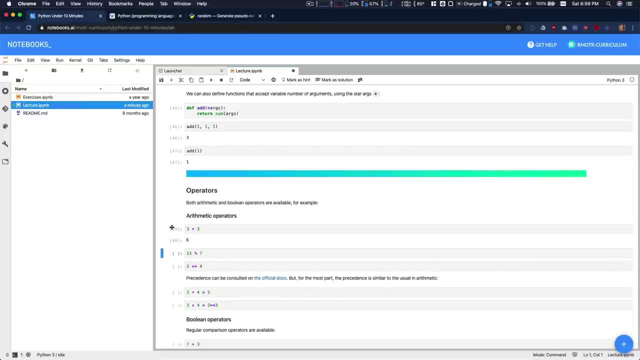 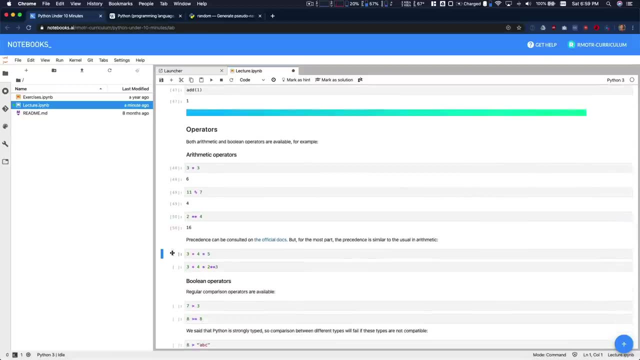 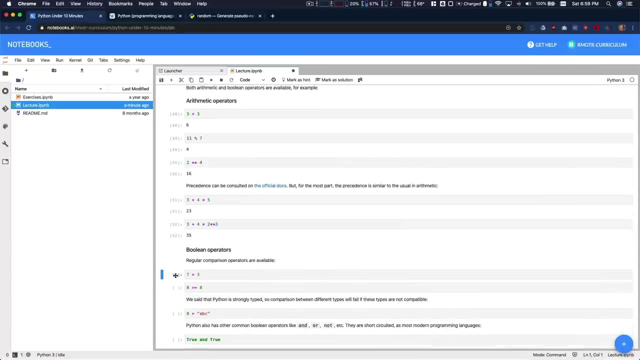 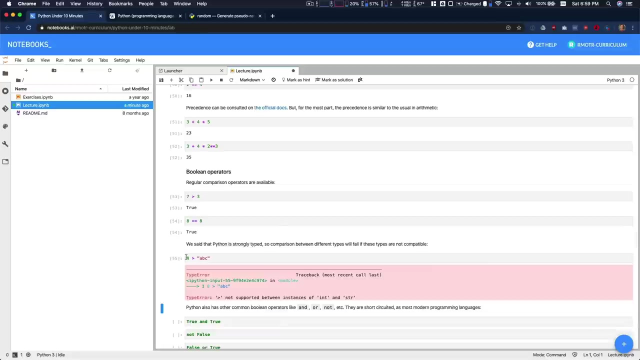 So all the arithmetic operators you know already: addition, modulus. In this case we're doing a power It's operation. All this is pretty standard, And the same thing happens with all our Boolean operators: greater than graded, or equals, then, etc. There are type checking. So this is when we have the strongly. 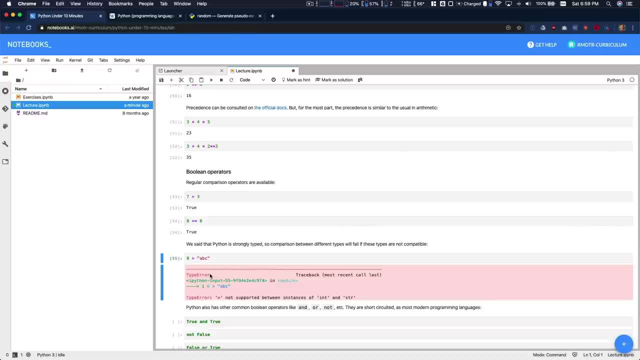 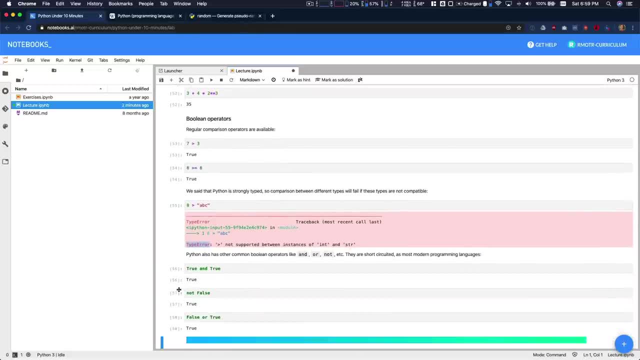 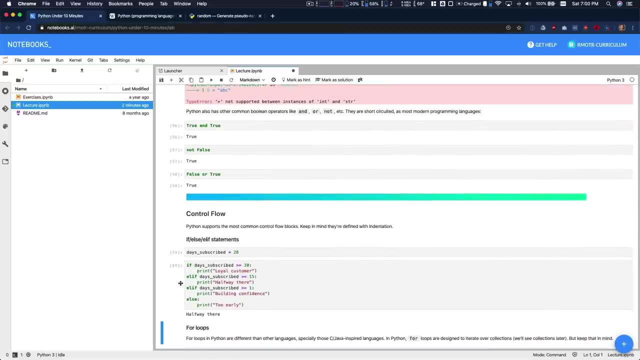 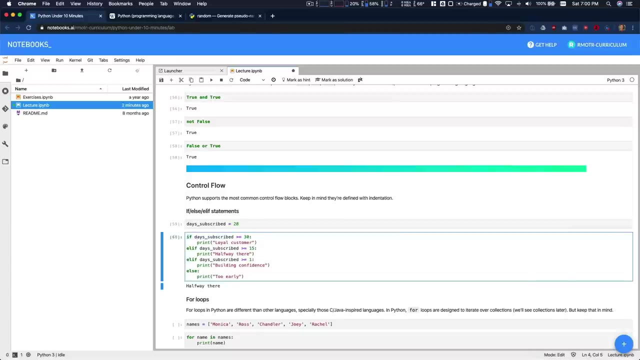 type error was raised, And the same thing with booleans and not an or operators. As we saw before, control flow is defined by the indentation, So every new block is defined with an indentation level. Python includes if else, and also l if, which is very convenient. 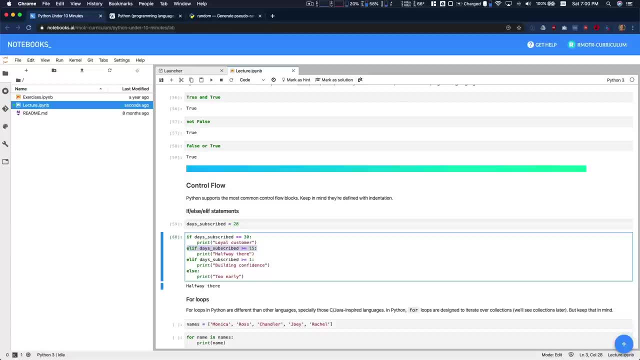 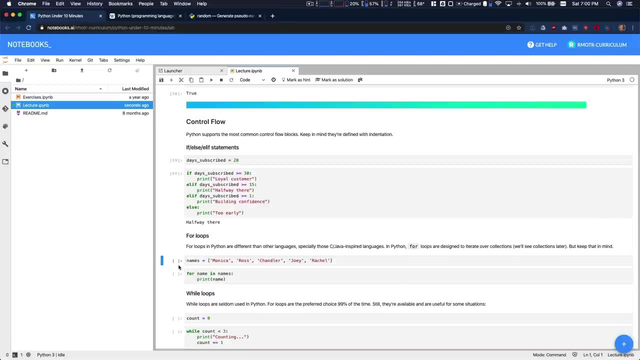 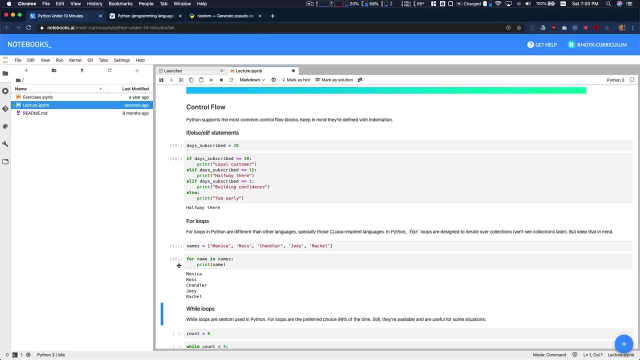 And this is an example. if this happens- l if, l, if, etc. Python does not have an error. So if you have a switch statement, for example loops, how are you going to loop through something? in Python? loops on lists or collections in general are very interconnected Because 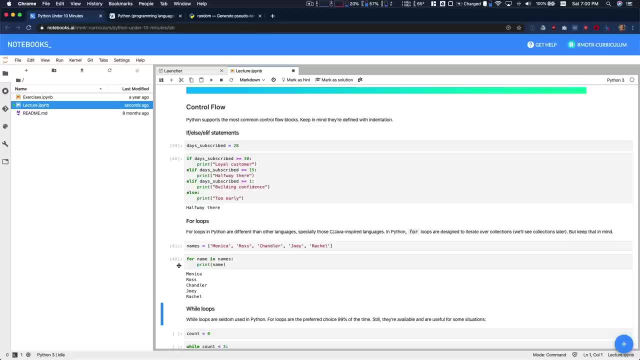 in. in reality, when you're looping the Python, you're not doing a regular. in Python, we don't have something like in in Java, you're going to have something like int. I equals zero. What else? It's been decades and I- this is, I haven't. 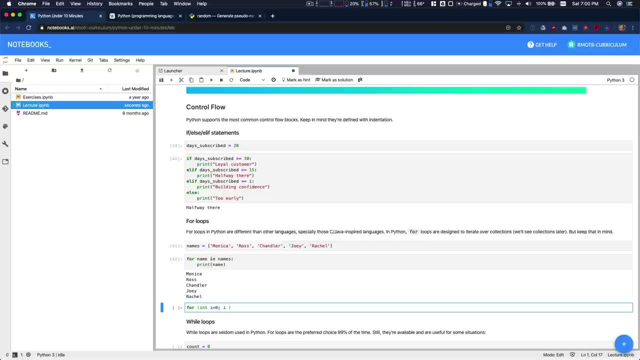 coding in Java. So I, I don't know. minus 10,, less than 10,, less than 10.. And here we do, I last, there you go. So we don't. we don't have these in Python. we have a way to mimic. 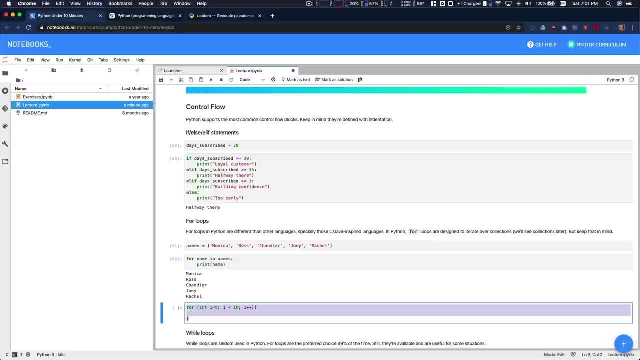 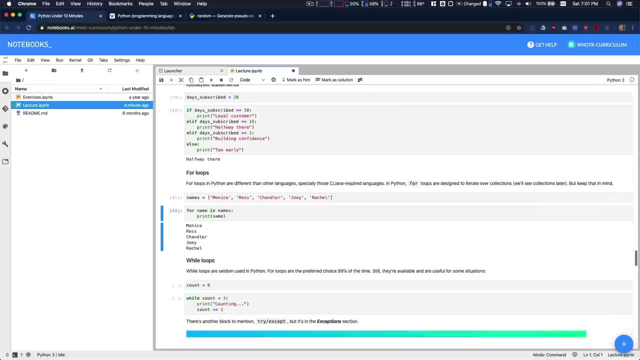 it. But we in Python, we always iterate over collection. So what we're going to do is we're going to create a range element and we're going to iterate over it. So the way it works is very close to another language is going to be a for each right. So in this case, 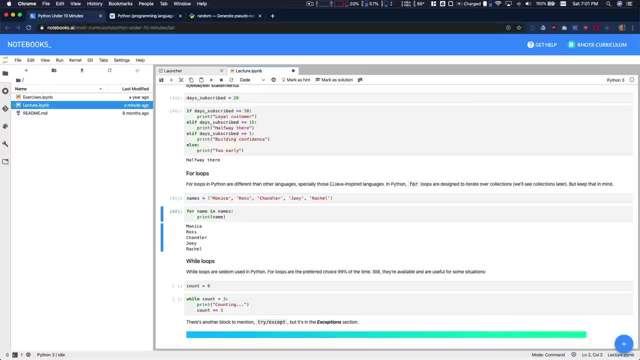 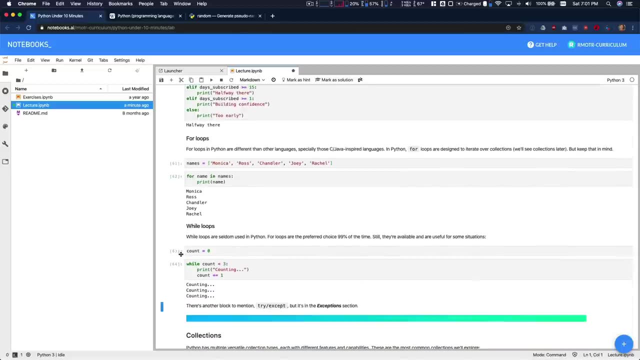 we have all these elements and we're going to do for name in names. that's it, And at any moment the name is going to be associated with an element in the list. While loops are part of the language, they're usually discouraged in favor of for loops, if something can be. 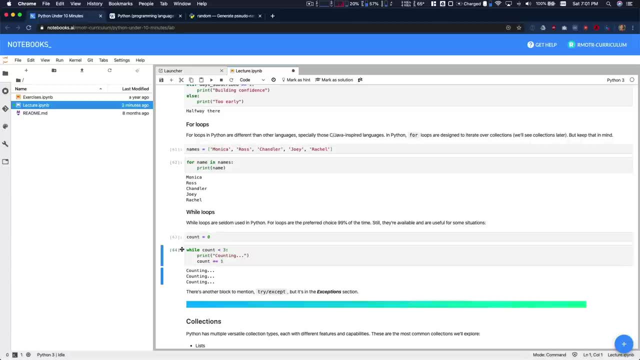 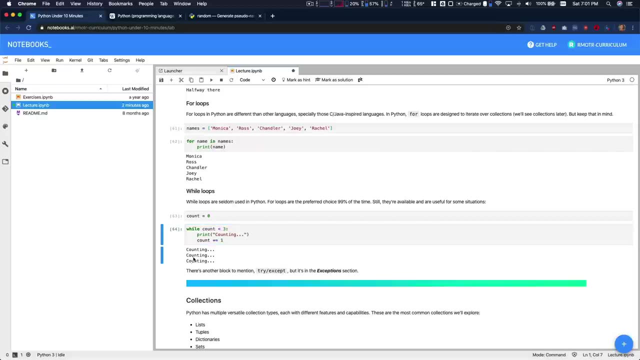 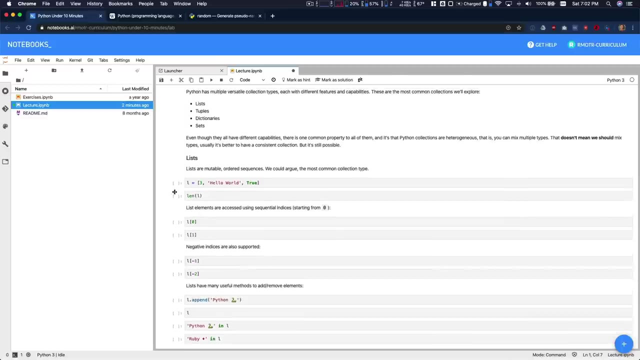 coded with a for loop, For loop. it should be coded with a for loop and not a while loop Because, as you might know already, these my trigger, or these my result in an infinite loop if you're not checking the conditions correctly. So the collections we have in Python are the fundamental. 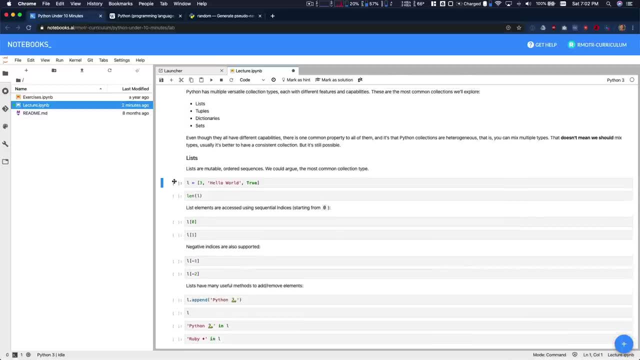 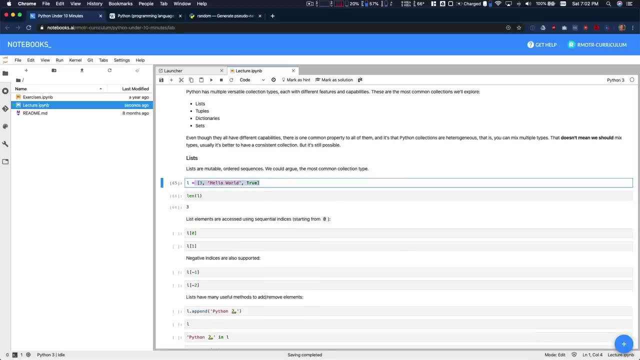 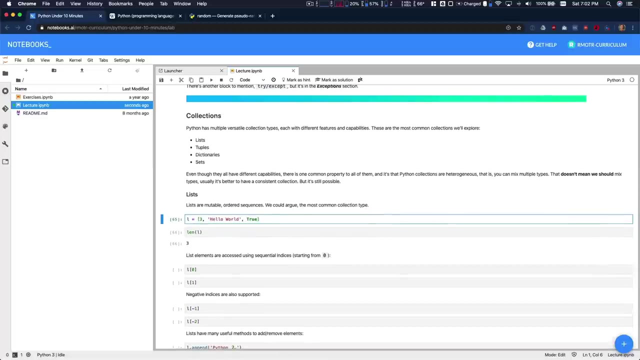 ones, the primitive ones. the most important ones are first the list. Python is. we do a heavy usage of lists And it's just an heterogeneous data structure, So you can put anything in it And actually all this collections are heterogeneous. you can mix values as you want And in this case we have. 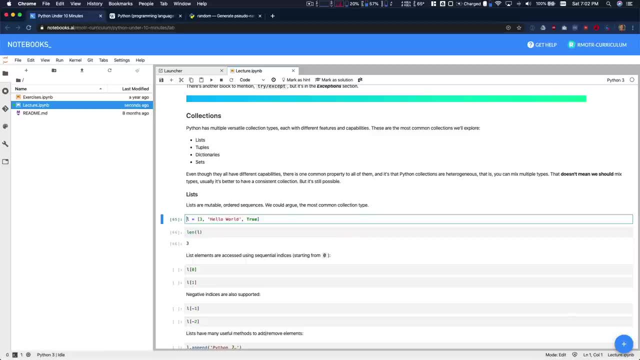 three elements. we have added one string, one integer, one string and one Boolean. And let me say something here: even though pythons- Python supports mixed types in the collections, it doesn't mean that you should do it. To be honest, we should use- usually avoid mixing. 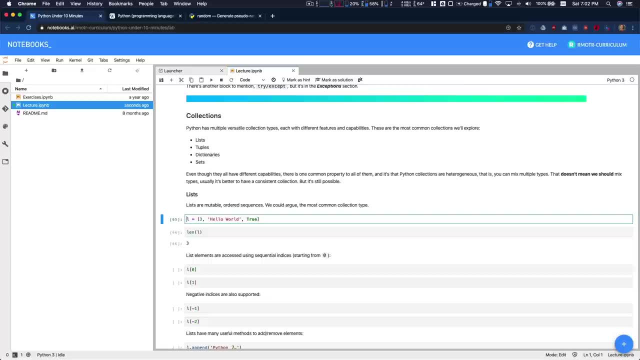 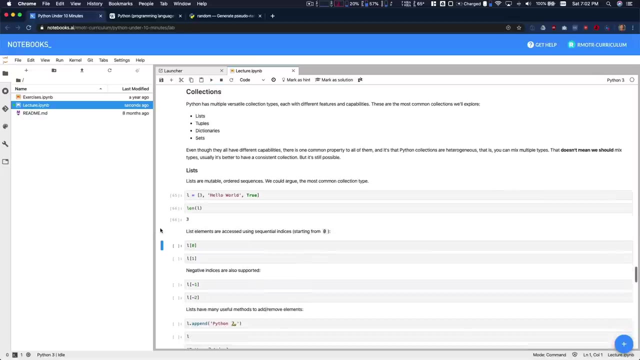 types in collections, because that means we don't- we don't know what we're putting in it. right, It should be consistent, So it's possible revisit your code if you have too many different types in it. Checking the length length function accessing elements is by by zero indexed. 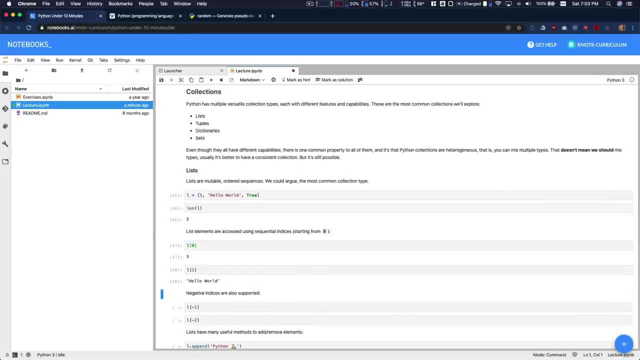 and we use square brackets. So in this case, give me the first element, given the second element, and also we can index starting from the from behind, from the end. So in this case, minus one minus two, minus three. So in this case, minus one minus two. again, give you. 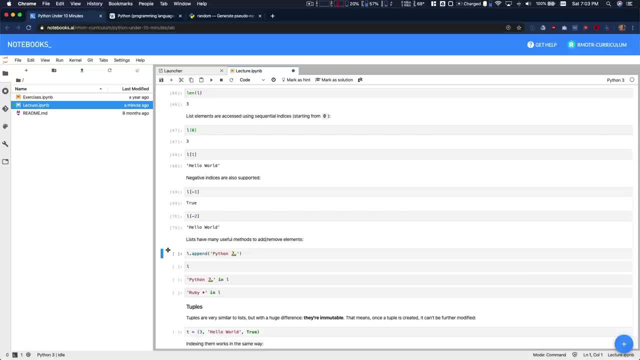 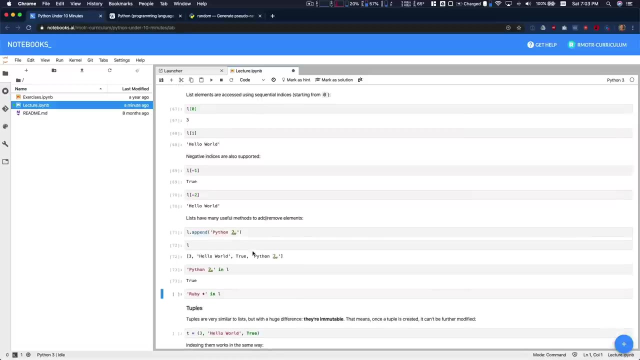 different elements. You can check the operations associated with all these elements Very quickly. a list is l dot append. we're going to append the new element, So the list now has an element at the end And we can check if that element is part of the list. In this case is true. 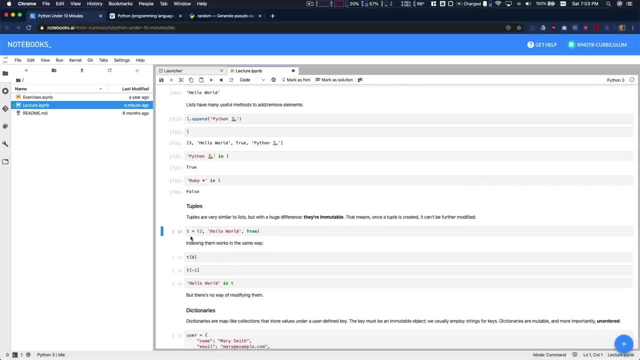 In this case is false. tuples are similar to lists. they are also consequences, But the main difference is that they are immutable. there is no way to add new elements to a tuple or remove elements from a tuple once it has been created. So 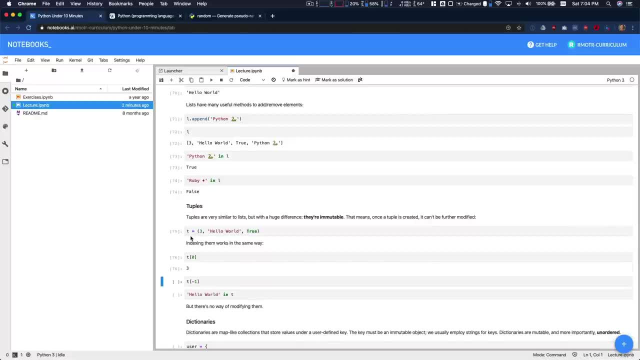 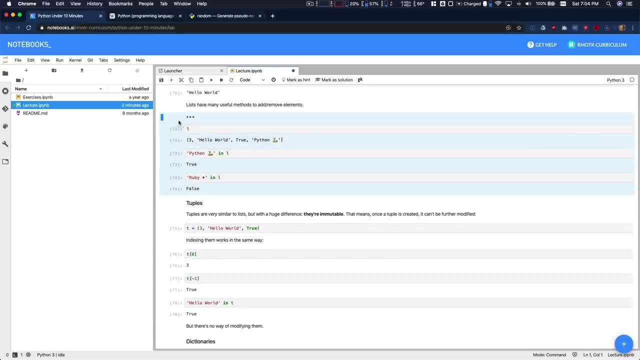 in this case, we have created a list with three elements, a tuple, sorry. with three elements. we can access it, we can check if something is in it, in the same way we did with a list, But in this case with a tuple. again, you cannot modify. tuple never changes. 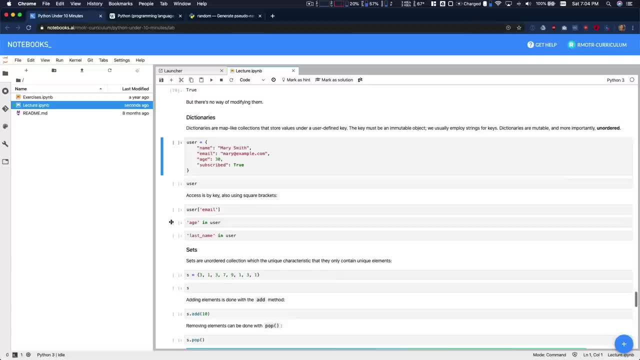 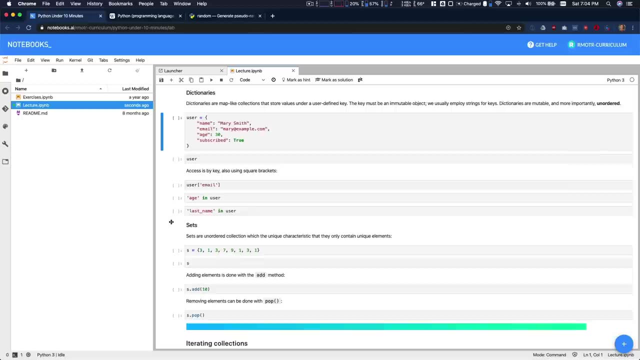 you can't add elements to it. Another important data structure is a dictionary. in Python, A dictionary is a key value right mapping. it's similar to an object in JavaScript or hash table in in Java. it's a key value mapping type And in this case we are going to associate values to names, So you can see. 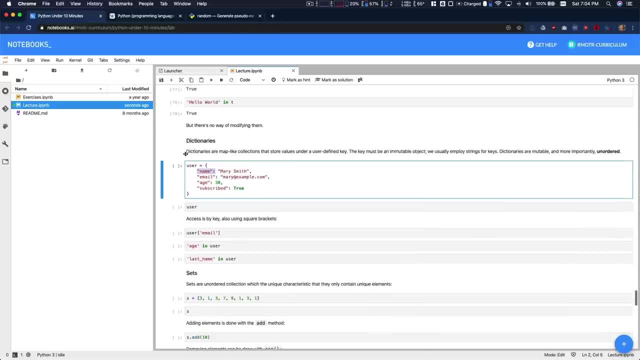 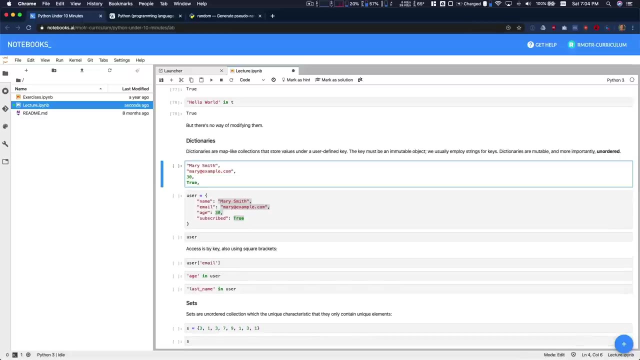 this. the way I like to explain it is: if you create a tuple, a list, right. so let's say, we're going to create a list out of all these elements. give me one second. We're going to create a list. There we go, we're going to copy these elements And I'm 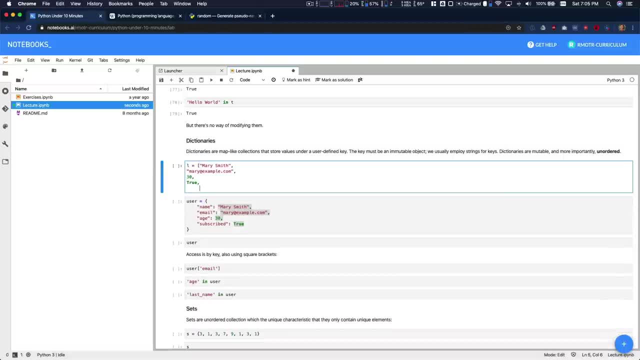 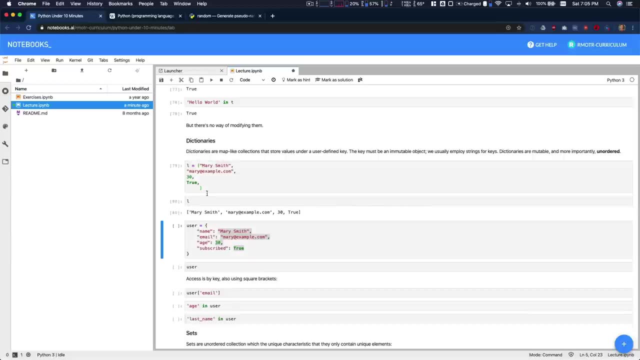 going to associate dots to our list. There you go. So these are lists. We could very well store the information about our customers in a list. right that that works? I mean I can get it done. The problem is that whenever I need to access information about this list, 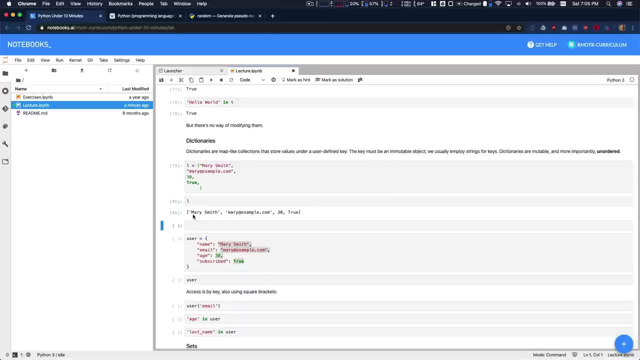 we're going to say, for example, I don't know, I want to give me the email of this customer. I have to remember the position that the email is located, So in this case, it's going to be position number one If this information grows, instead of having 1234 values or four pieces of information. 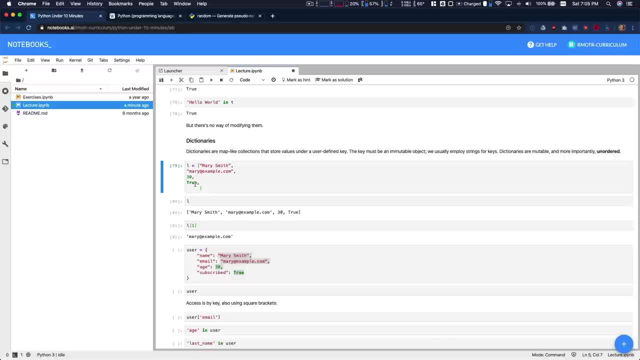 for a user. we have 100, right then it's going to be very hard to access those individual values. So that's why we create dictionaries. dictionaries are collections of values. the important part is on the right, the important part is the value. But they are instead of just indexed by the position we give them. 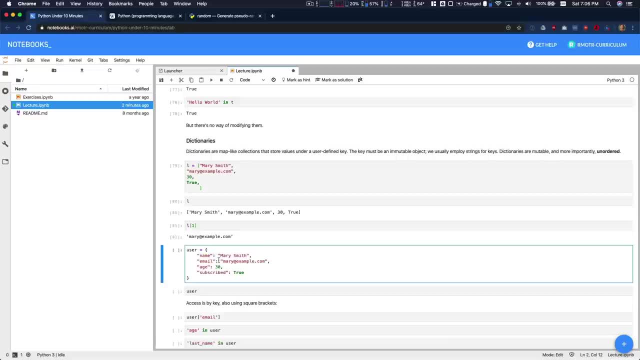 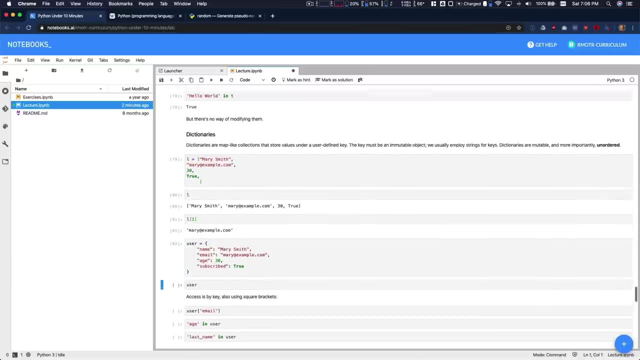 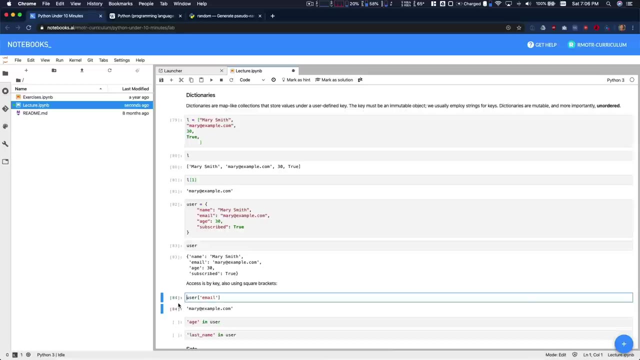 arbitrary names. we tell them very explicit names. this is the name, this is the email, this is the age and this is if they're subscribed or not. So once we create this dictionary, we can access those values By the name. give me the email of this user. or is the age present of the user is the last? 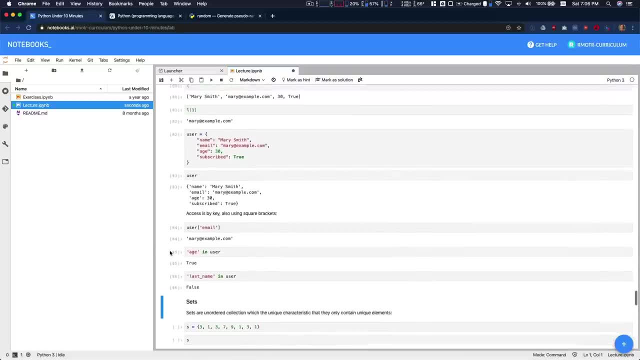 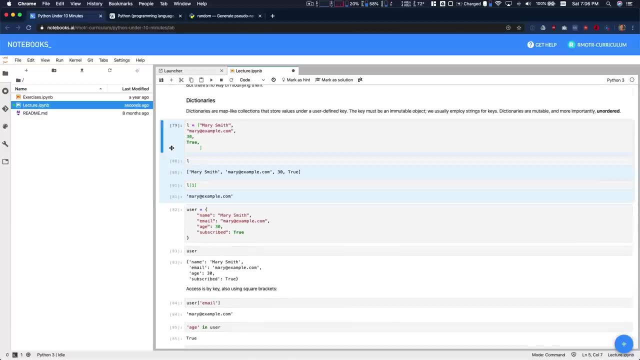 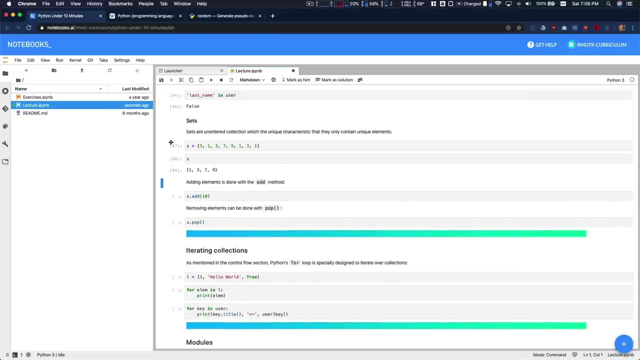 name present of the youth in the user in the user dictionary. So again, it's a way to store information associating labels in order to make it simpler for us later. Let me delete this and I move forward. sets: sets are very common. data structure is when you're learning about collections and 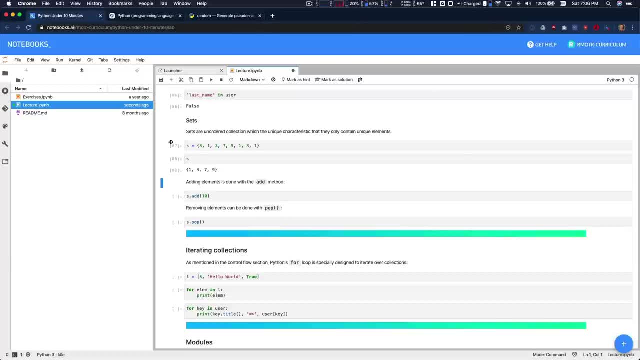 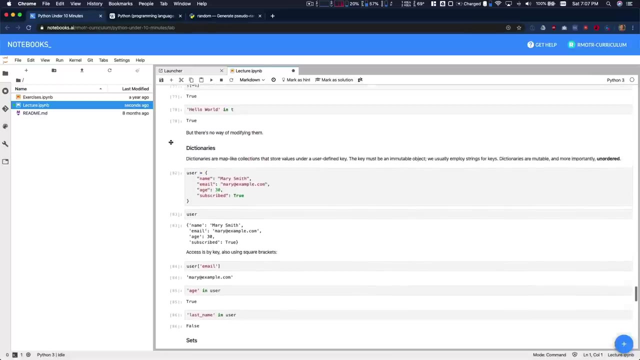 and and, yeah, data structures. in general, It's not so common in too many languages, I mean, it's not very popular in Python. we use it often because it has a very interesting feature. First of all- and it's something that I forgot to tell you- about dictionaries, both sets and dictionaries. 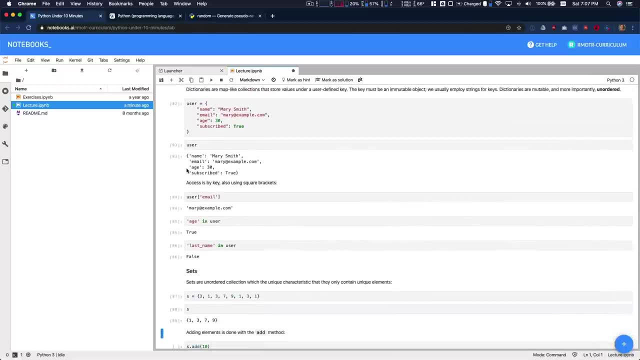 are what we call unordered data structures. you never know the order of the elements In Python. with recent versions There have been changes which make Python dictionaries ordered, But for now I'm gonna say you shouldn't rely on it. you should think your dictionaries, as they are completely unordered. 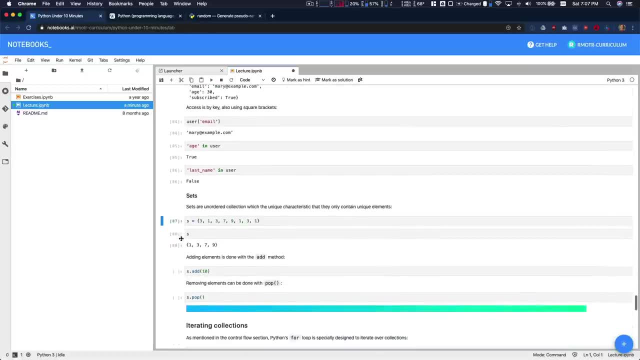 data structures and the same thing for sets. Sets are- it's a bug that contains elements. you know it's a big bug. you keep throwing elements inside of the set. there is no order in it And what's going to happen with it? you're gonna add elements, for example, to the set. 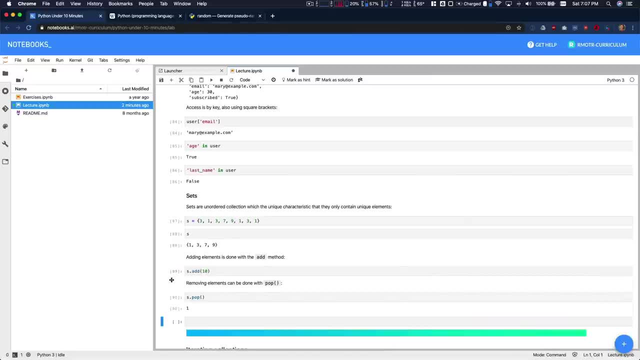 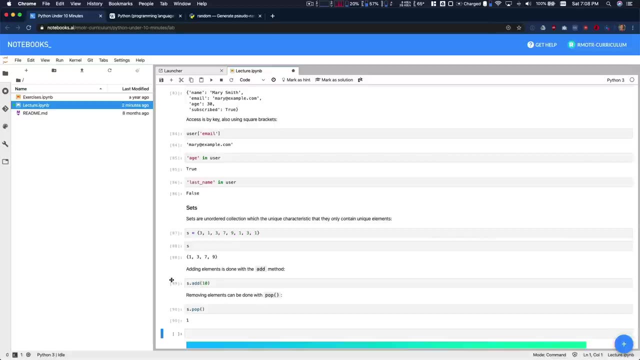 or you can remove elements to the set, And there is one important thing that makes the set so useful, And it's the membership operation. I'm going to write it down here: membership ship operation. There you go, So you can access this notebook later. So in the membership, 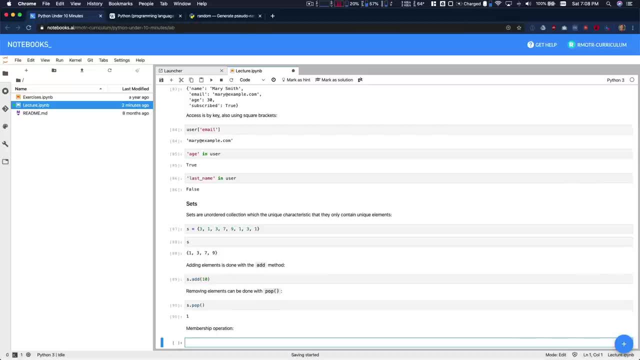 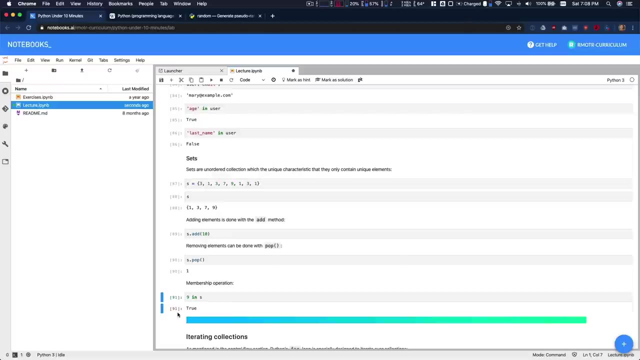 operation, the, the, the process of checking the set. you're going to have to do a lot of things, For example checking if something not nine in s, the process s of checking. this is extremely fast, it's what we call Oh one, And this is because, as you might have seen here, when 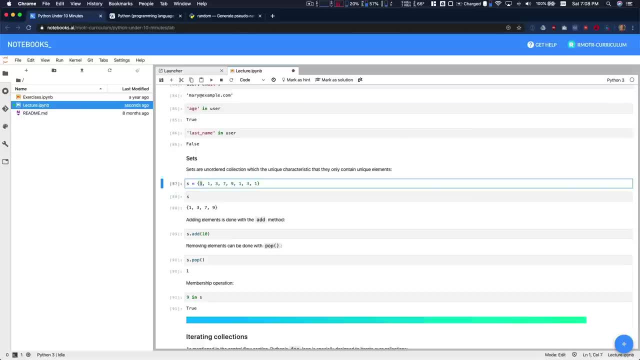 I created this set, I included a couple of repeated elements: 333.. Right- 11179.. The resulting set doesn't have those repeated elements. These are two features of the set. the set will only contain unique values And, by the way it's implemented behind the scenes, will 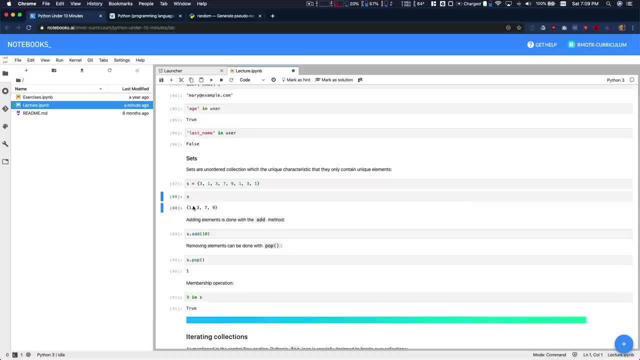 make that these unique values are extremely simple to check whenever you pass these. membership operation is extremely simple, or sorry, it's extremely performant. It's very fast, different from, for example, a list, So keep it in mind. sets are very, very useful when you're checking for membership. So, again, 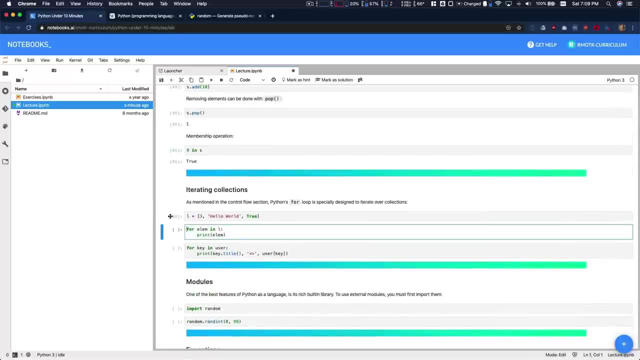 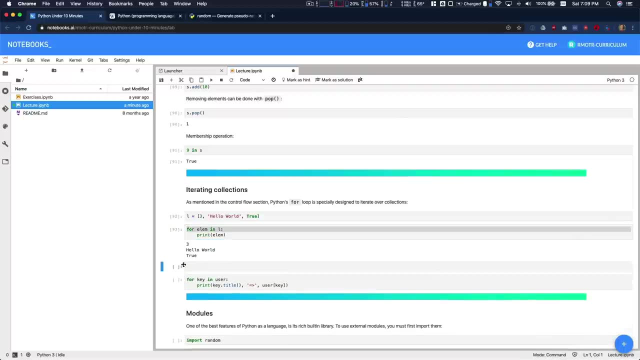 as I told you before, we're going to iterate over collections with a for loop. So in this case is, if we have a list, it's going to be for element in list. there you go. If you have a user dictionary, a dictionary- sorry, in this case user, we're gonna the default. 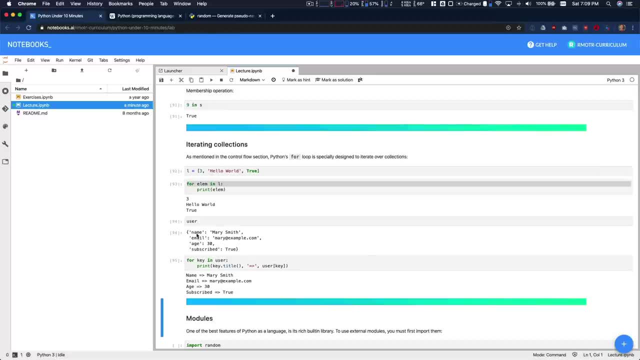 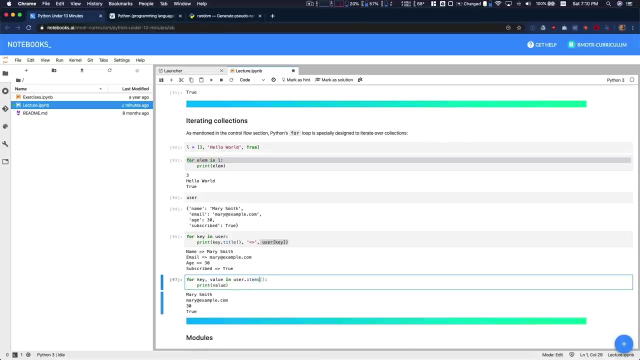 iteration is by key. we're gonna get for name And email, age subscribed And we have to extract the value out of the of the dictionary. we could also do for value in user dot values. Oh, there you go. Or you can iterate over both key and value with items, key and value. 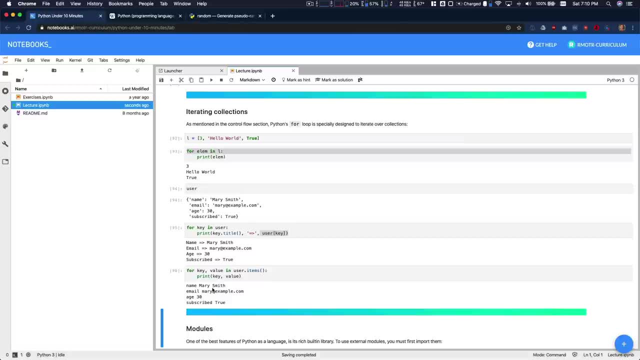 Okay, There you go. So iteration in, in in Python is very readable, to put it in a way. And again, remember, we're always using the for loop. that assumes that you're iterating over a collection. we don't have the for E. I equals zero equals zero. I equals zero. I less than 10 times less than. 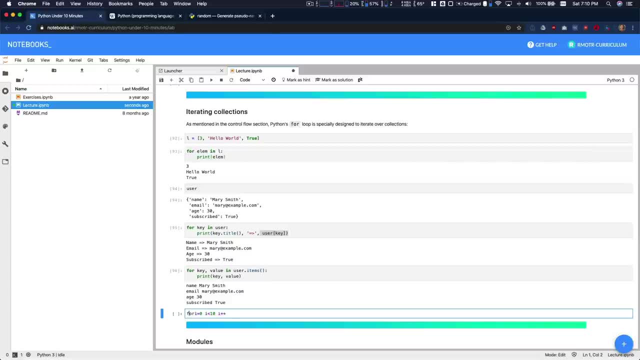 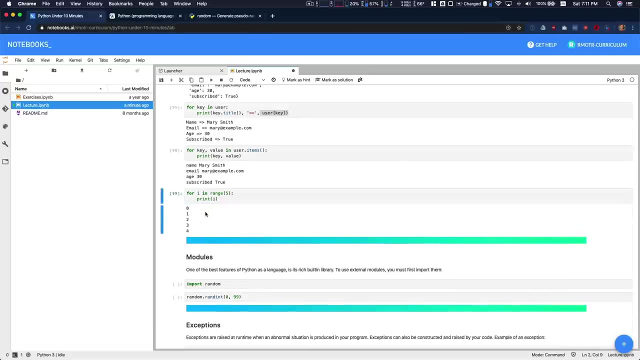 10. I plus plus. we don't have that right in Python. we can simulate it with for I in range five, for example print. we can simulate it with the range function, which generates pretty much those elements. Something that you might have heard about Python is that 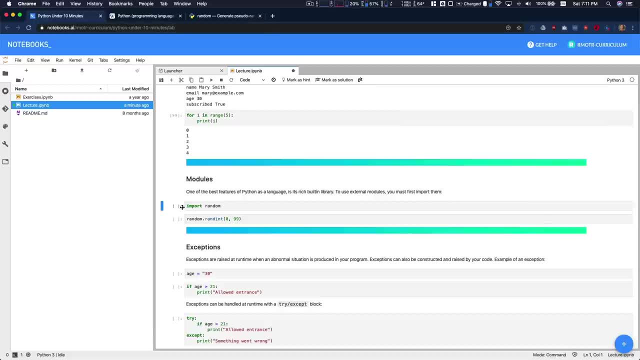 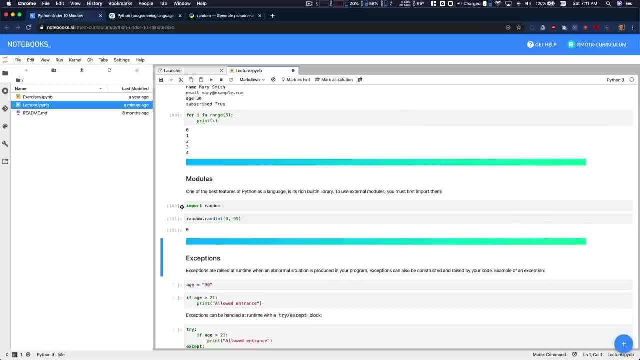 it has a huge library of built in modules, right, That you can just import. it's just gonna work. there are so many things already coded in Python that it makes it very simple for you to create something on top, Do you want? 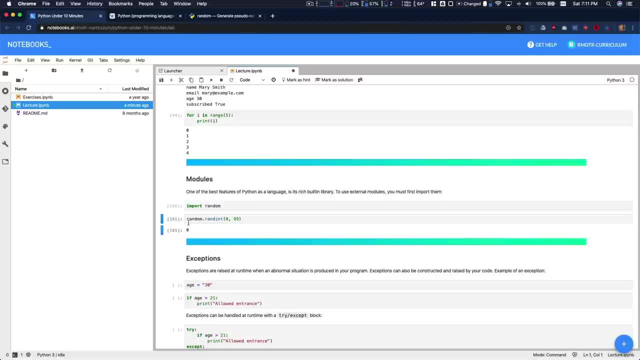 an library for, I don't know, security, cryptography, math, numeric processing, NumPy right, Machine learning, web development, creating games. there's pi game. do you want to create a graphical user interface? Whatever you want, Okay. 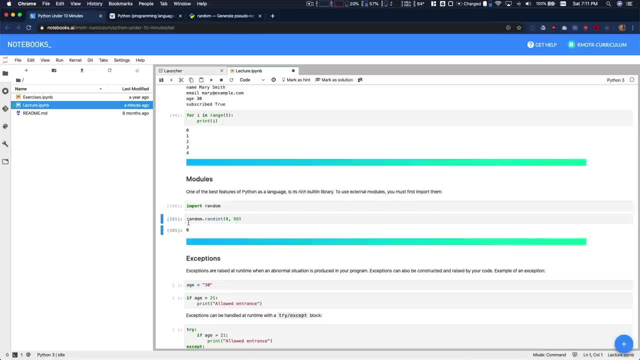 So, what you want to do, there is usually a library that has already been coded and will make your job easier. On top of that, the built in standard library right, which is already included with Python. it's not third party In this case. it's already created. 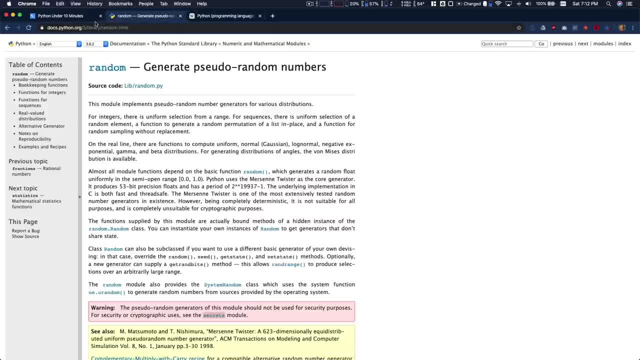 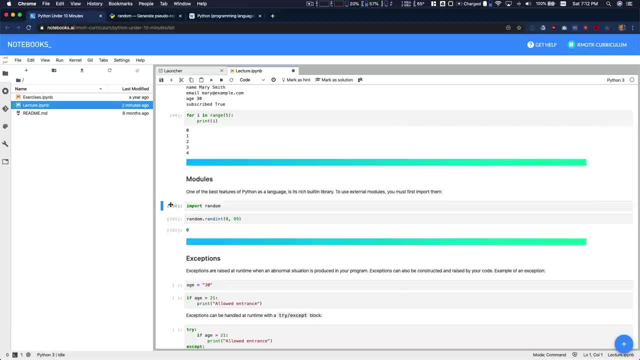 by the Python core team. It's a huge library, so many modules, And the way it works is by importing this module. So this is the way we're gonna work with Python. We're gonna work with packages and modules, or differences between modules and packages. 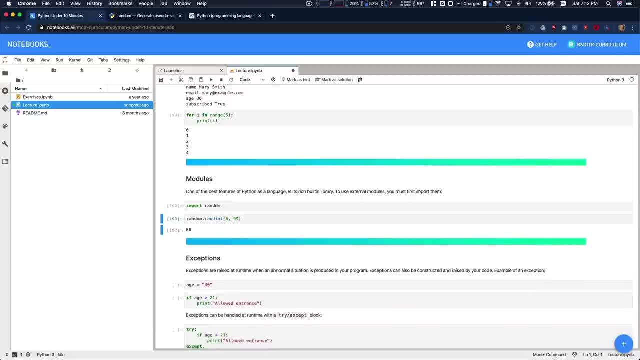 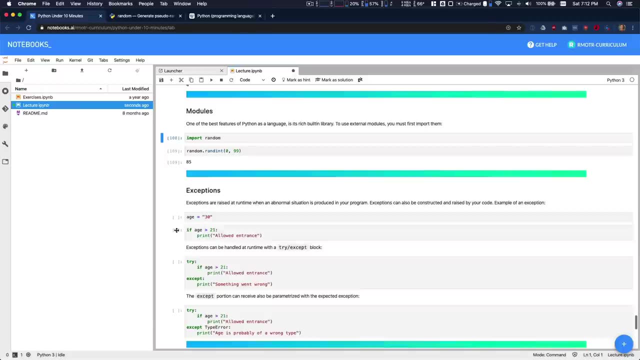 third party built in this a little bit more advanced, But again in this case that random number generator. it's already built in and you can check the docs right here. Exceptions whenever you do something that doesn't work. So in this case we say if the age is greater.